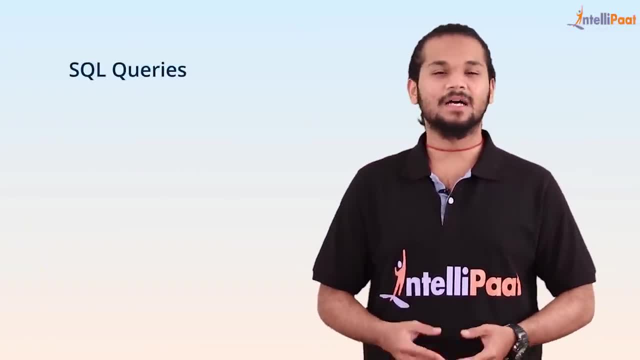 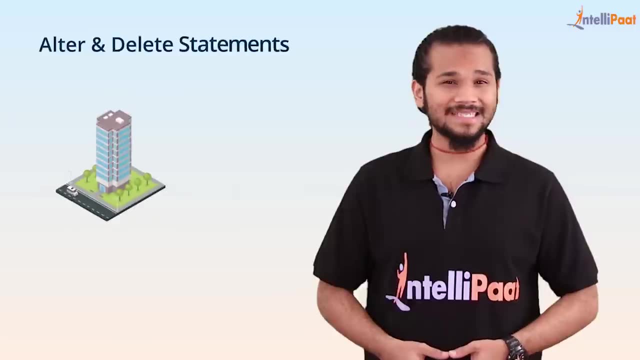 learning the SQL query syntaxes, such as statements which involve select commands, group by having order by and much more, And after this we can check out the alter statements and delete statements as well, And, followed by this, we can learn everything there. 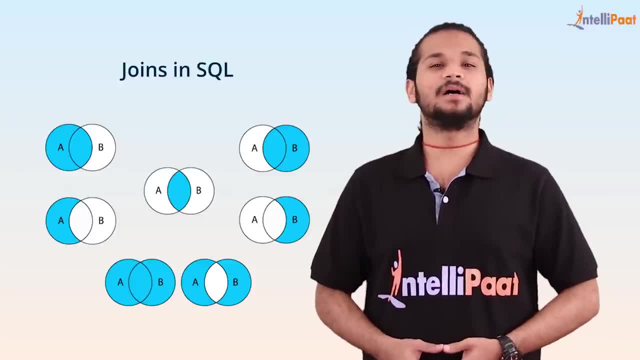 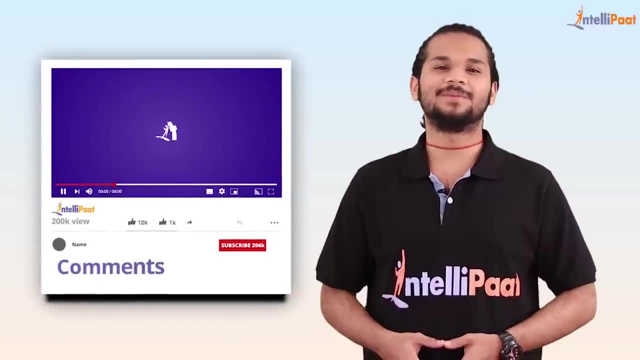 is to know about joins in SQL, And after this, guys, we'll be learning about unions, merge statements and many, many other operations. If you have any queries at this point of time, make sure to head on to the comment section below and do let us know and we'll be happy. 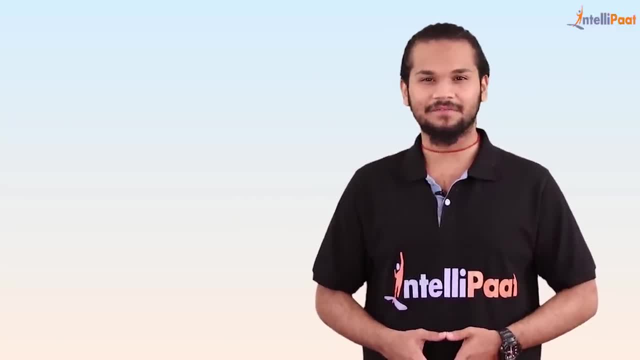 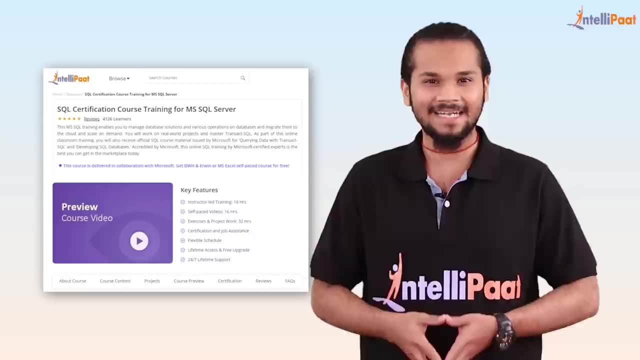 to help you out there, And if you guys are looking for end-to-end core certification in SQL, Intellipath provides the SQL core certification training program, where you can learn all of these concepts in depth and earn a certificate at the same time. Well, without further ado, let's begin. 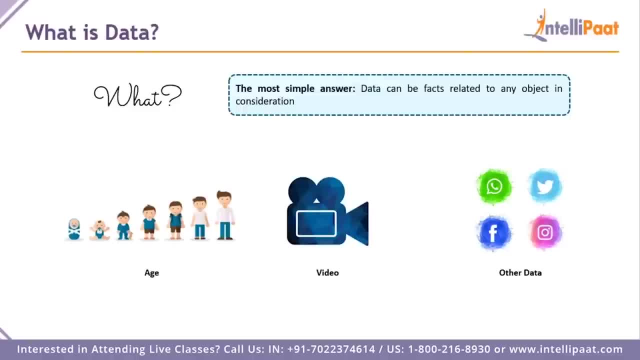 the class. We live in a world which is surrounded by data, right? So what is data? In my opinion, data can be considered as the facts which are basically related to any object which we are talking about. So you know, data can be age. Well, age is a data. 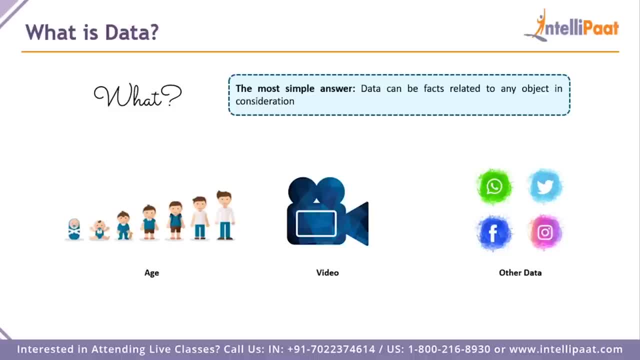 You know you can put that in numerics, You can put that in a form where people can take note out of it and, you know, make sense out of it. Because you know age can be anything from 0.1 all the way to 100, and much more as well. right? So age is a numeric in which 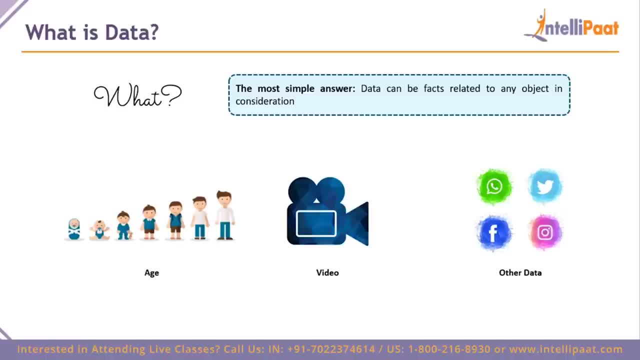 we can gauge something and get something out of. And then, if you're thinking about the other forms of data again, we have video data as well. right, So video is what we call as unstructured data. But then if you do not know what unstructured mean, do not worry. 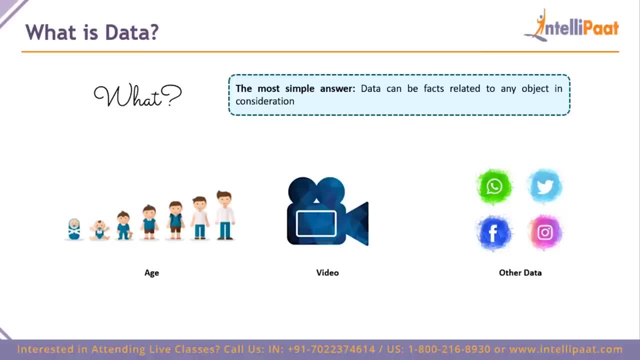 At this point you need to know that. At this point you need to know that pretty much you know, video is a form of data as well. And then there are other data as well, And when you think about all the data we generate, 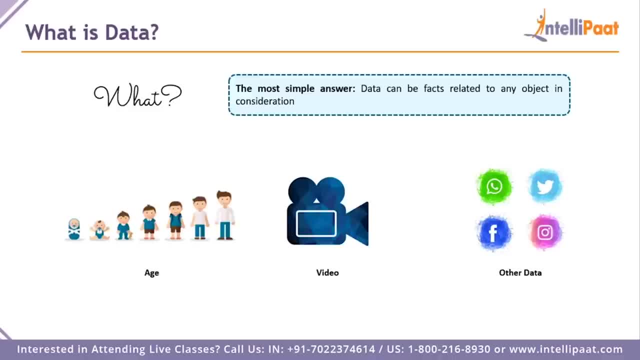 by you know, leaving messages to each other on WhatsApp or leaving tweets on Twitter, sharing photos on Instagram or putting some updates on our timelines on Facebook. So all these stuff, and lots and lots more, is what we call as data guys. So this brings. 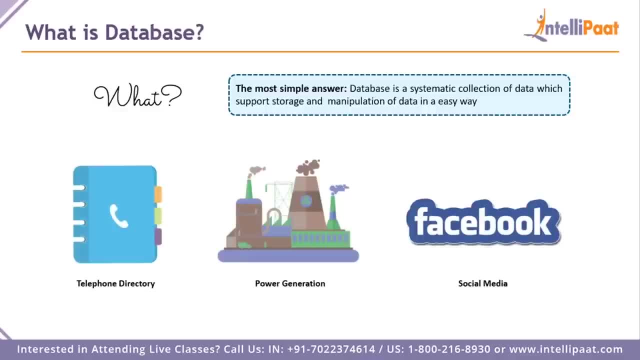 us to the question: what is a database? You might have heard of data. So if you've heard of database, guys head to the comment section and put down the comments as usual. We all love an interactive session, So, and you guys are very good at it as well, guys, So head. 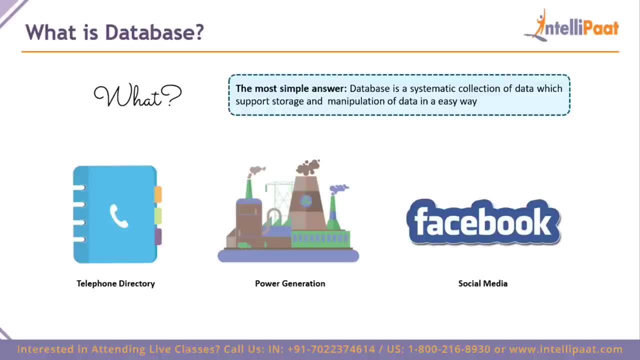 to the comment section and put your opinions down. So what is a database? Well, a database is basically nothing but a very systematic collection of data, in the most simplest terms. So why would we go about needing the systematic, you know, collection of data? Well, it's pretty much to, you know, support, some sort of storage. 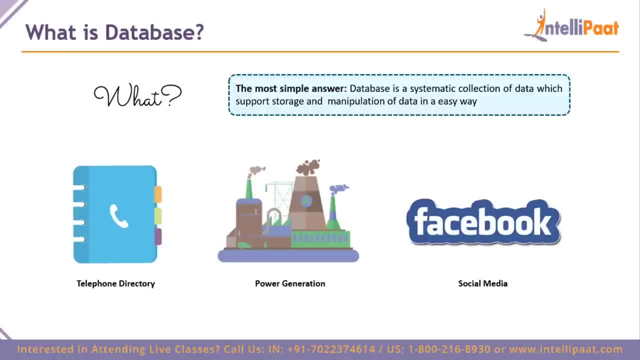 where we can hold the data, We can maintain the data and eventually we can. you know, we have to have the ability to manipulate the data in a very easy way, to be honest. So to give you examples of what databases actually are, if you guys remember when we were, you know, a couple of years- 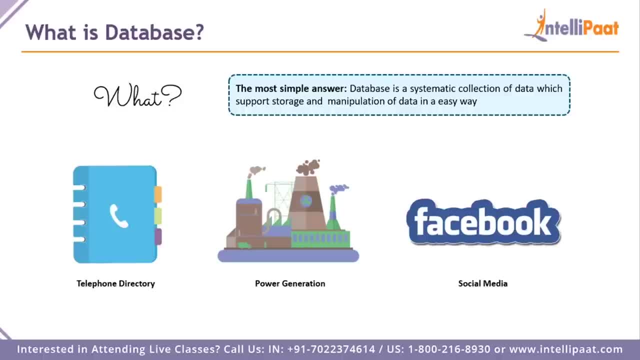 ago we used to get these telephone directories where they used to be all the numbers. It's called yellow pages in a couple of countries as well, So that is a very good example of a hard copy of a database, And the contacts option on your mobile phone right now is also. 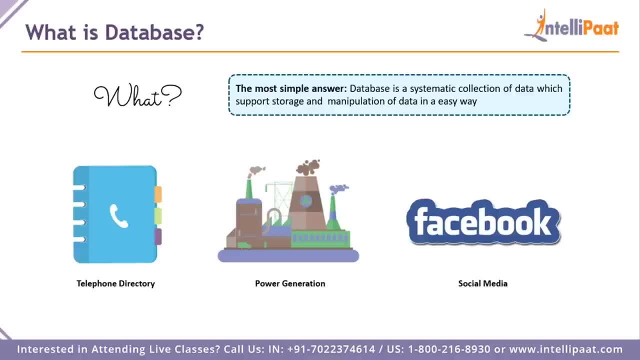 a database. Coming to power generation, power generation, you might not know, has a huge database of you know what power is being consumed by what house and whatnot, Because, again, at the end of the day, you get billed for the power you use And this data goes to your. 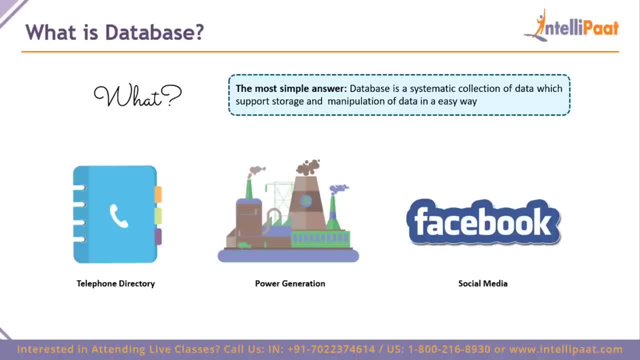 local electricity power supply board And again, this forms a very big database as well, because pretty much they need to know what the power they're generating versus what's being used, and many, many other details as well, guys. And then coming to social media, 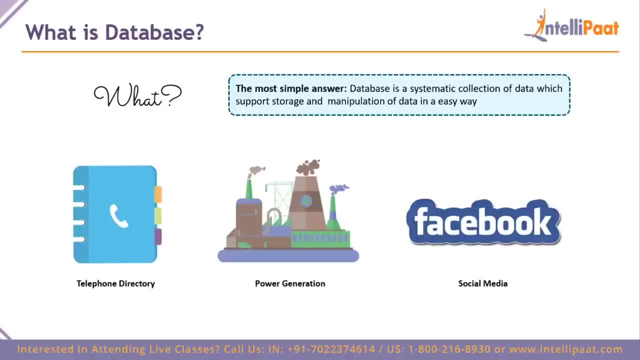 as I just told you, uploading images, uploading statuses, you know, uploading stories, whatnot. so all of these are stored in a database, in secure data centers, what we call, especially when it comes to social media and privacy things. So, pretty much you know all of these. 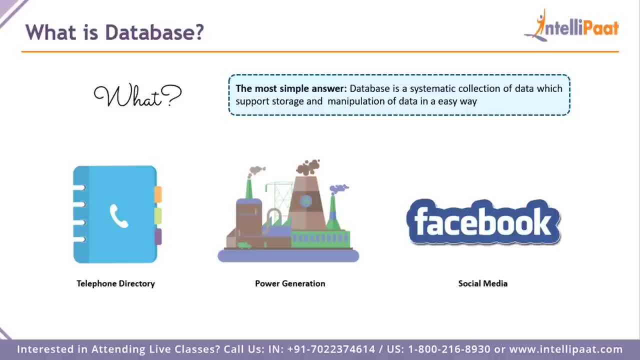 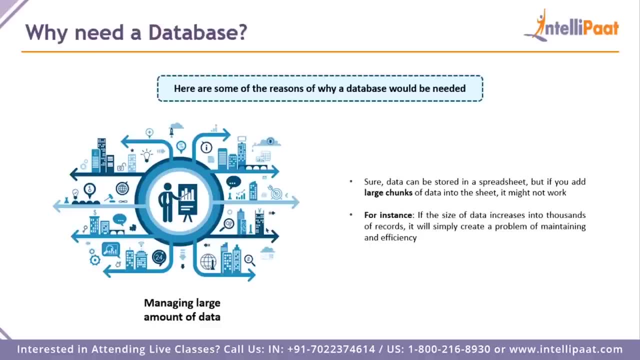 are stored in the database, and it is stored securely, guys. So, basically, this brings us to the question: why would we ever go about needing a database? Well, I've pretty much tried to keep this session very simple, And this is these. these are the reasons that. 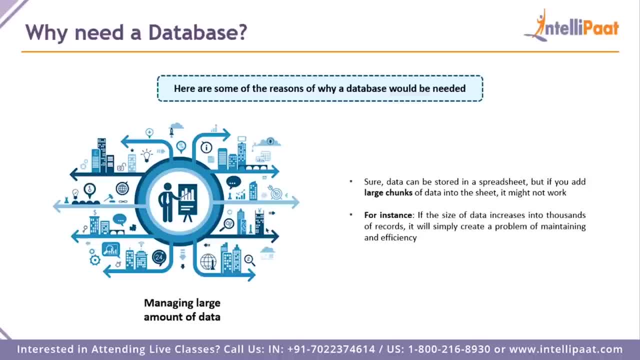 I could pretty much think of of you know why are pretty much we would need a database. The first thing, in my opinion, is that we need a database because managing large amounts of data is a hassle, because you might say: you know what, I can store data in a spreadsheet. 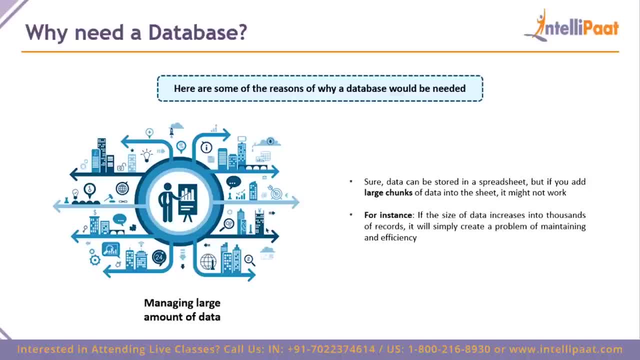 and it's going to be fine. But then when you think about very, very large amounts of data, large chunks of data, and throw it all into one sheet and make it work, it might not work or it might be extremely difficult, even if it works right. So you know, let's say the 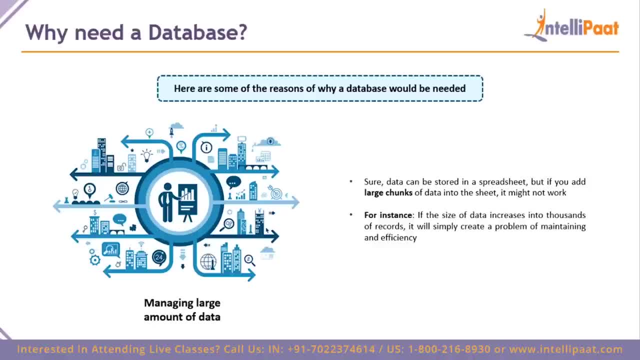 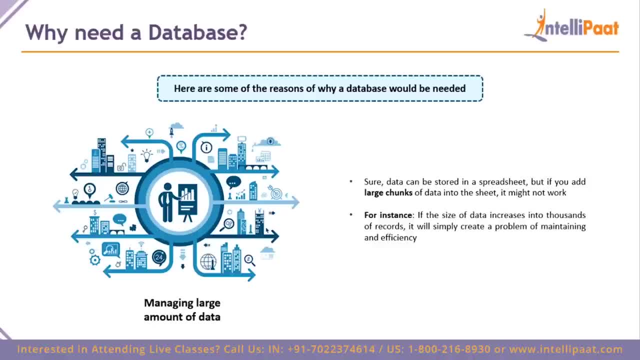 to thousands and millions of records. so when this happens, you know it will create a huge problem if you're using spreadsheets to maintain this data and at the end of the day, it is gonna hurt with respect to efficiency, time and what not as well, right? so this is the first point of why you need 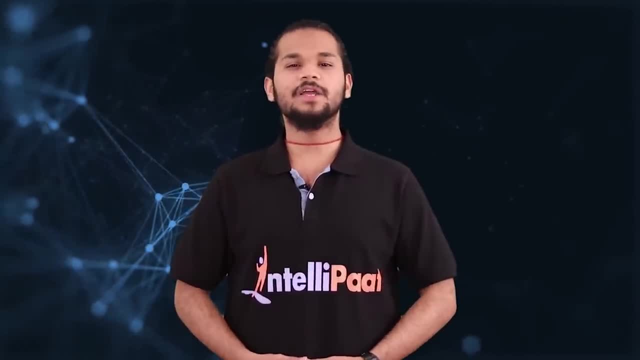 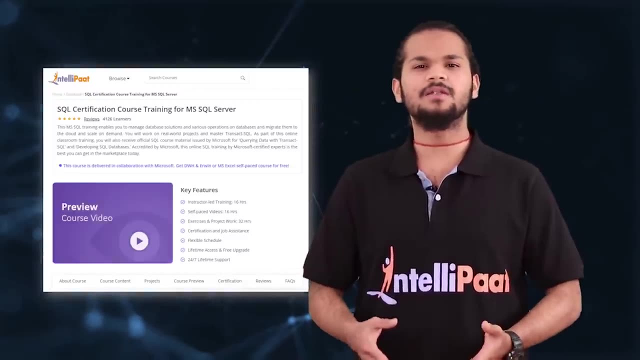 why you should need a database. just a quick info. if you guys are looking for end-to-end course certification in SQL in, telepath provides the SQL course certification training program where you can learn all of these concepts in depth and earn a certificate at the same time. the link is: 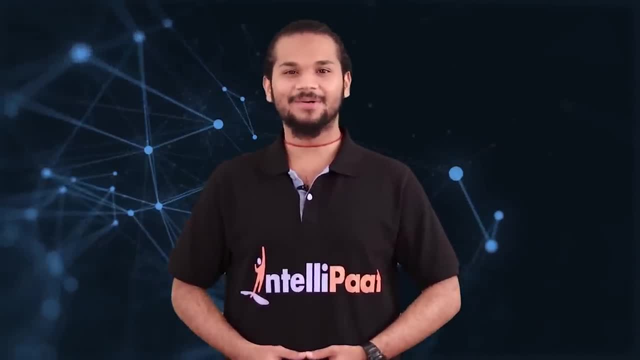 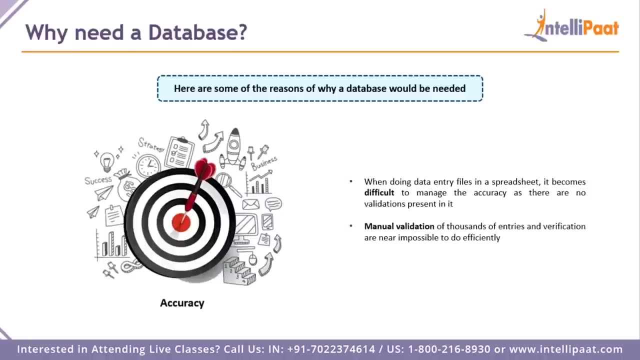 given in the description box below. so make sure to check it out. and on that note, let's get back to the class. and the second thing is the accuracy of the data, because when you think about it, doing data entry pretty much into a spreadsheet sounds very easy, but then it becomes extremely difficult. 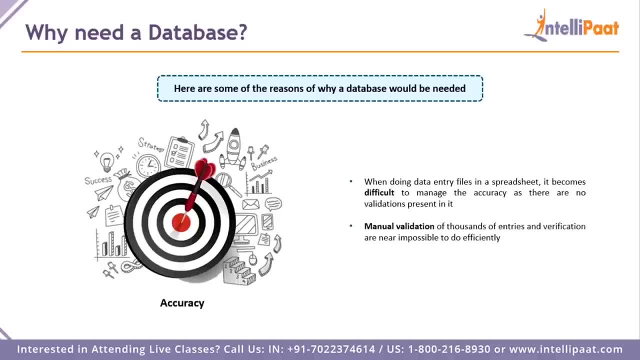 to pretty much track how accurate the data is you know on the spreadsheet. because, at the end of the day, if you cannot have a method where you can validate the spreadsheet to find out a the data is accurate or not, it doesn't make sense. and again, think about this manual validation of 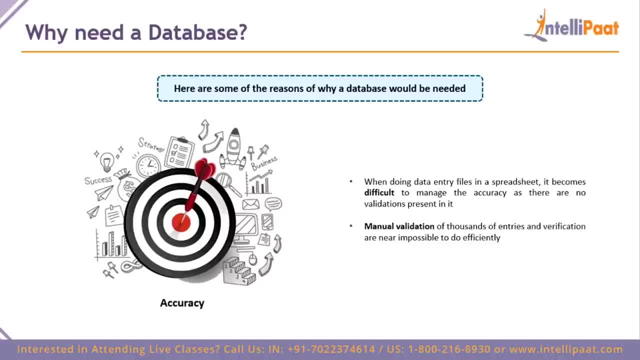 thousands and millions of entries and verification of the same. it are pretty much near impossible. and even if they were possible, pretty much it brings the efficiency right down to zero, right in my opinion. so this brings us to the third reason of pretty much why would? we would need 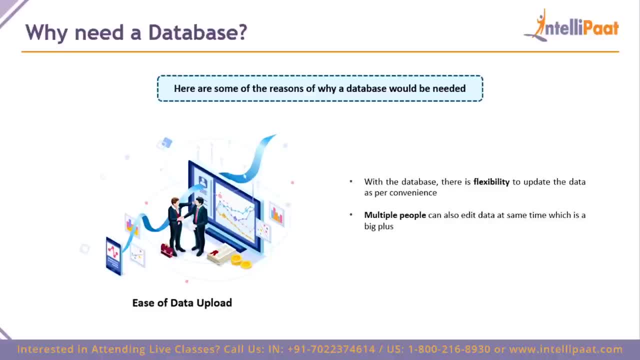 a database guys. so in my opinion, again, it's the ease of data uploading, because with the database you have very good amount of flexibility to pretty much you know: update the, update the data present, manipulate it, play around with it, create and delete it whatever you want at your convenience. so you do not have to wait for a the person who created the spreadsheet. 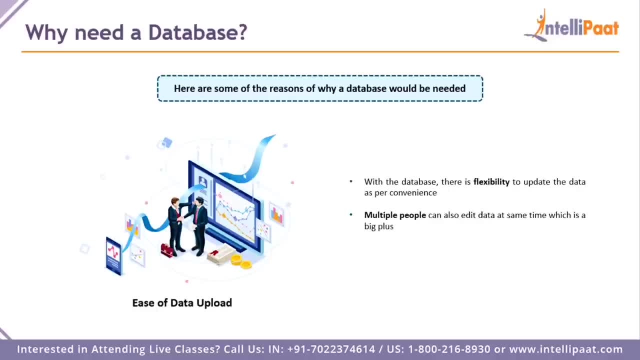 go through millions of entries and do all of that. so again, you know, the best advantage of a database is that multiple people can edit the data at the same time. be, this brings up the efficiency and pulls it from zero to hundred. you know, almost hundred in my opinion, guys. so 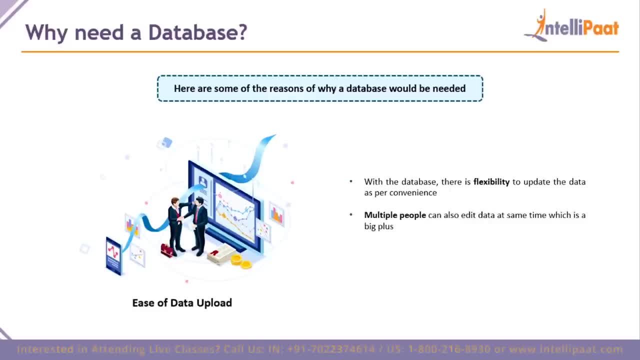 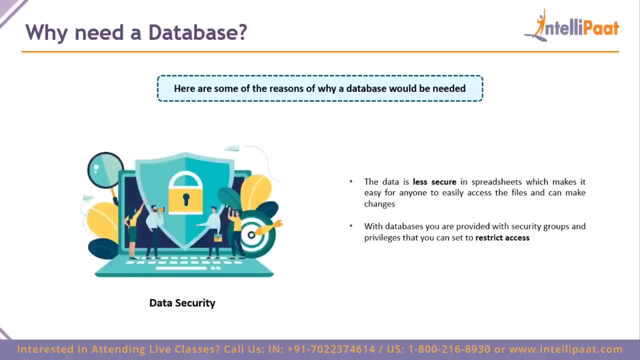 what do you think about the efficiency when it comes to the database technologies of today? head to the comment section and do let me know so. on that note, this brings us to the next reason why you should consider a database. it is pretty much because of data security, because you know, 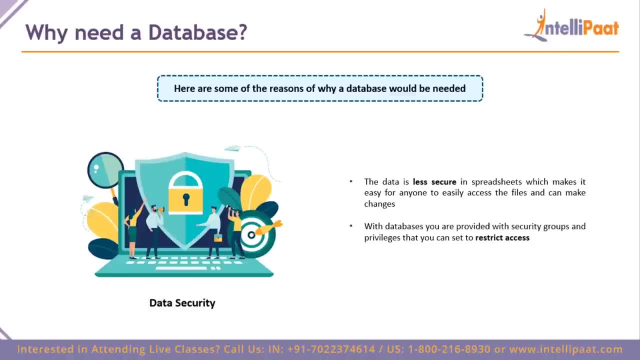 we do have passwords for spreadsheets and whatnot, but then the data is considered to be less secure and it makes it gullible because you know every gun can pretty much get access to all of these files. they can do some changes, remove whatever they want or, you know, add whatever unnecessary. 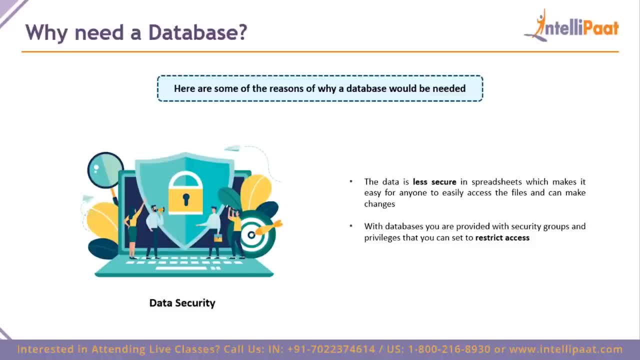 stuff and it hurts the data at the end of the day. but then with databases, pretty much you can have something called as security groups, privilege accesses and so much more. so at the end of the day, here you can pretty much, you know, restrict access to a certain number of people. 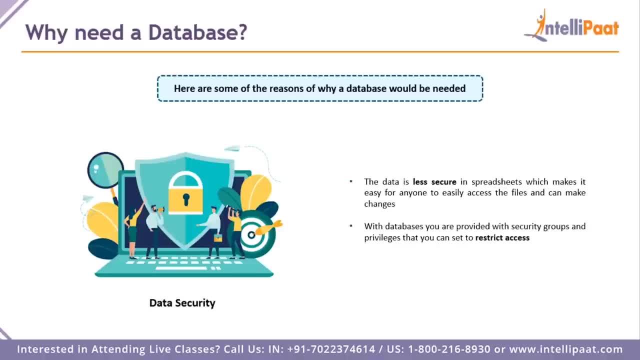 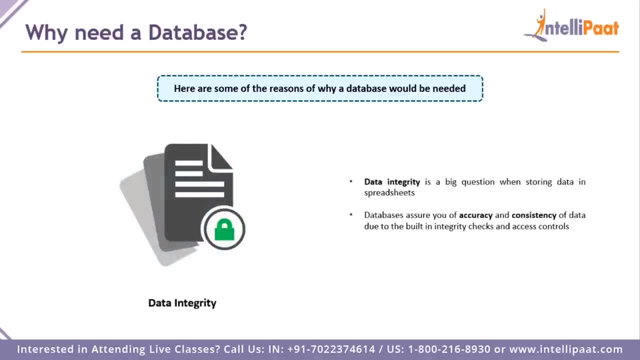 certain. you know people with the privilege to access the data, manipulate the data and whatnot. so your data will be in good hands at the end of the day. so what does that mean? well, adding on to that, this brings us to the next point, which is data integrity. data integrity is one of the big 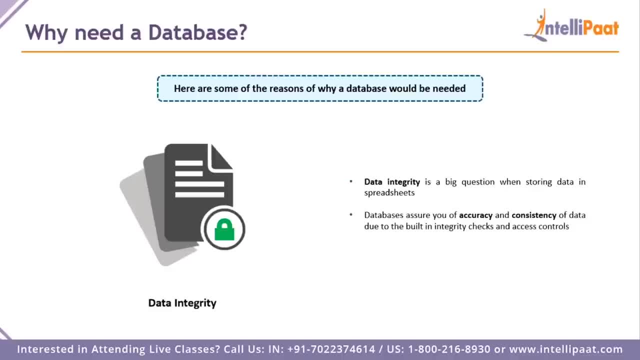 questions today. when we are storing, you know, data in spreadsheets as well as databases, because, again, we've already spoken about how data can be gullible when we've put it in spreadsheets, but then when you put it in a database, you know you are assured of accuracy, number one thing it is. 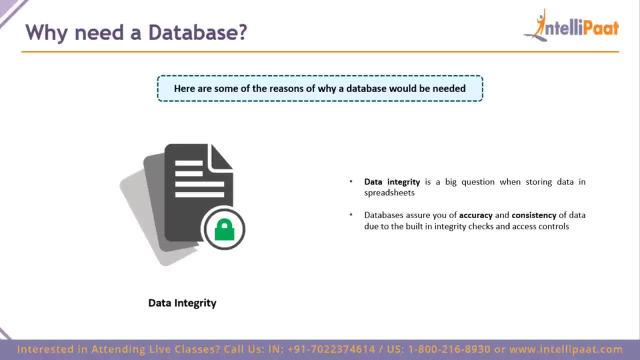 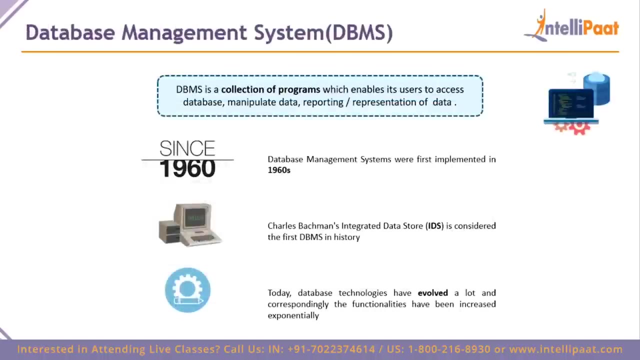 extremely efficient. number two and number three: your data is consistent, because databases, many multiple database service providers today, pretty much you know, go about giving you very good integrity checks, very good access controls, privilege accesses, member accesses and so much more. so this brings us to something, uh, you know, you might have heard of. 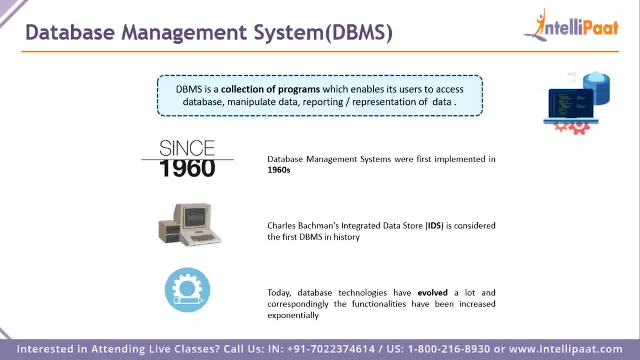 you might have used in college or you might not know as well, it's called as dbms. well, dbms pretty much means database management system, guys. so what is dbms? well, dbms, in the most simplest terms, is basically just a collection of programs which enables the user, whoever is using this particular 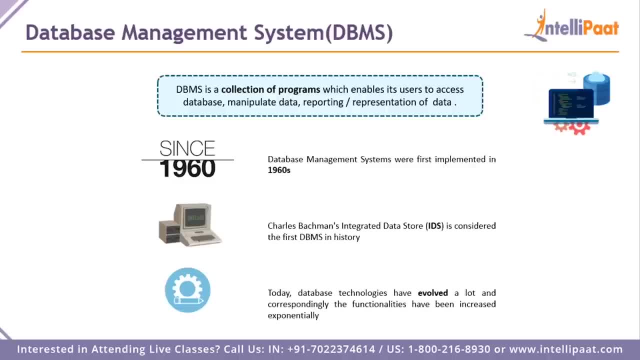 dbms softwares to go about accessing a database, creating a database, manipulating the data- uh, you know, deleting the data. so basically, this gives the user an interface where he can, where he or she can, you know, talk to the database and pretty much work with the database, edit the database, delete the database and do whatever the person wishes to. 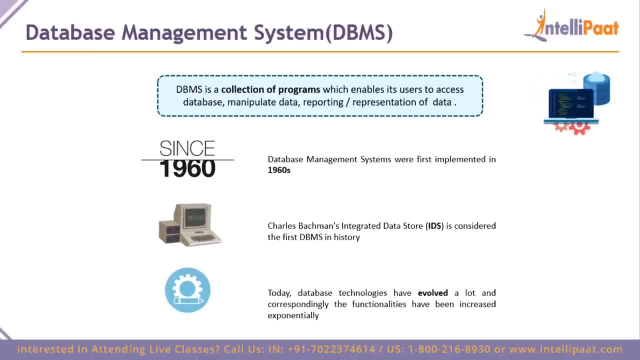 uh, if he has the right access, and this basically gives the person you know a very good interface. guys. so I have three facts for you, uh, with respect to the database management systems, and the first thing is that dbms is not a new concept. it was first implemented pretty much in 1960, so that is. 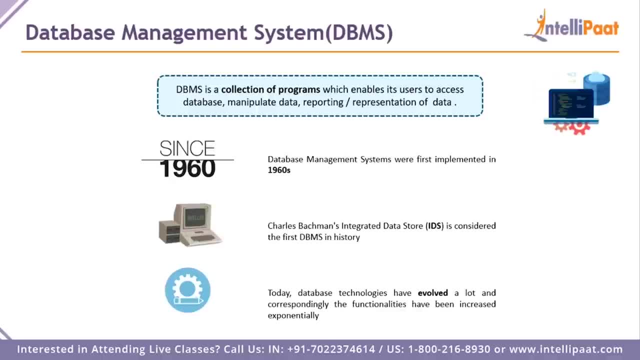 uh is, and then, when you can think about it, uh, the person who pretty much uh gave us the first dbms system, pretty much, is called as Charles Bachman, and his ideas is considered to be the first dbms. ideas is basically integrated data store is what Mr Charles chose to cause, call his first dbms. 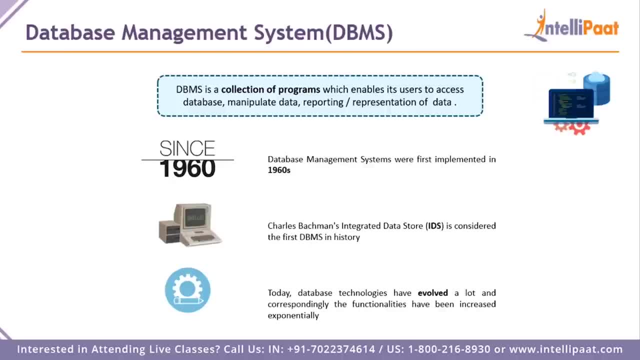 machine, guys. and then the third important fact is that today we know that the database technologies have evolved so much and all of the functionalities have been given, and these functionalities increase. the database systems today are so powerful. it drives, you know, millions and millions of gigabytes of data every single day. yes, millions and millions every single day, guys. I can say millions of. 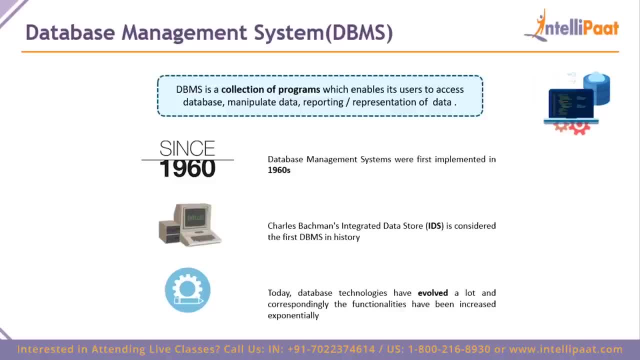 millions as well, because the world, you know, the entire world- is basically a big data problem. so, uh, having a place where we can handle all of these, store all of these and manipulate all of these is always a blessing, guys. so this brings us quickly to, uh, the introduction to SQL. well, so what is? 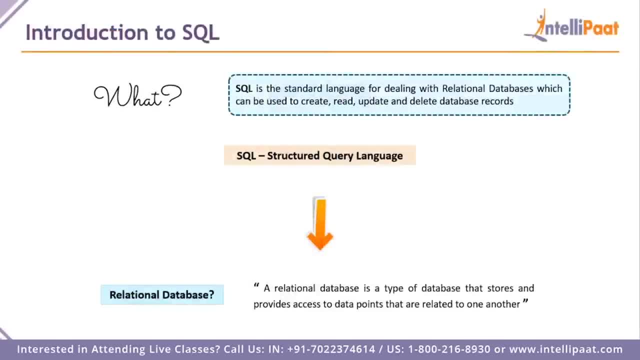 a SQL? well, SQL is one of the standard languages we use when we go on about dealing with relational databases which can be used to create, read, update and delete database records, guys. so these are some of the operations we can perform. so what does SQL stands for? well, SQL is simple. it stands for: 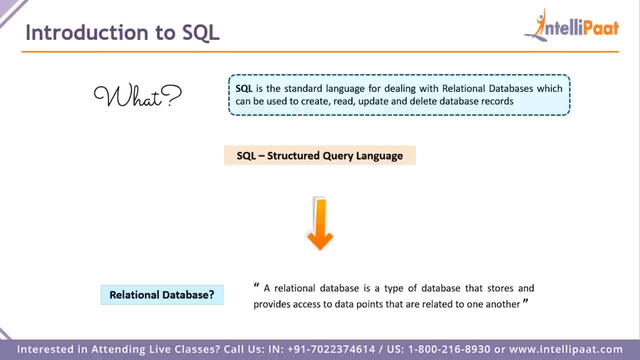 structured query language. guys, are you going to find out why we call it the query language in just a moment? but then you read the term relational databases. so what is a relational database? well, a relational database is basically just a type of database that stores and provides accesses to all. 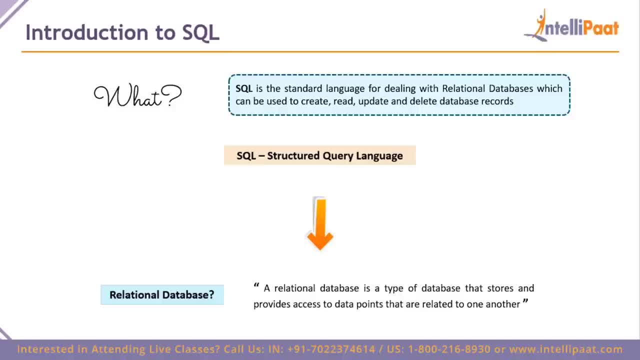 the data points which are related to one another. well, how are these data related to one another, guys? so, basically, when we call it a relational database, there has to be some relation with respect to the data, uh, using SQL and uh, the you know all the DBMS we call the rdbms because it's relational. 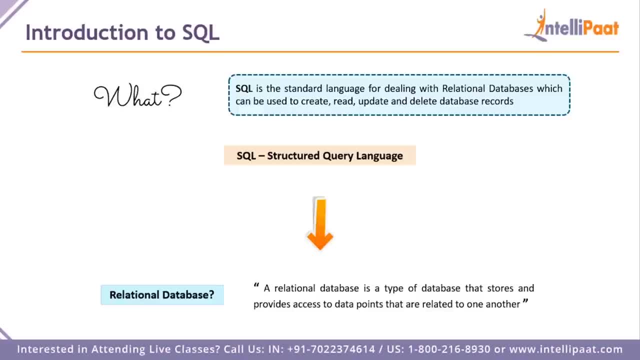 database management systems. here we have the data organized in tables, which you will see in just a second, and then we map the data so that the database knows what's important and what's not, and we do this using something called as keys- well, keys such as primary keys, candidate keys, secondary keys. 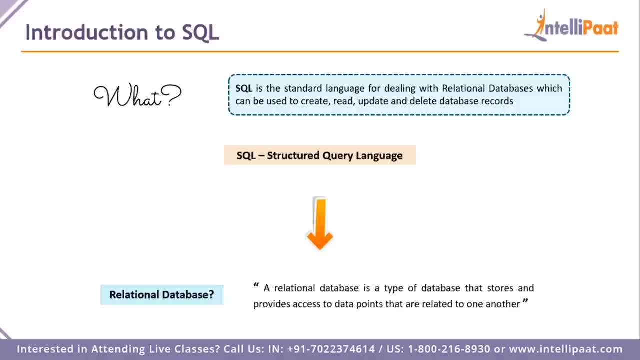 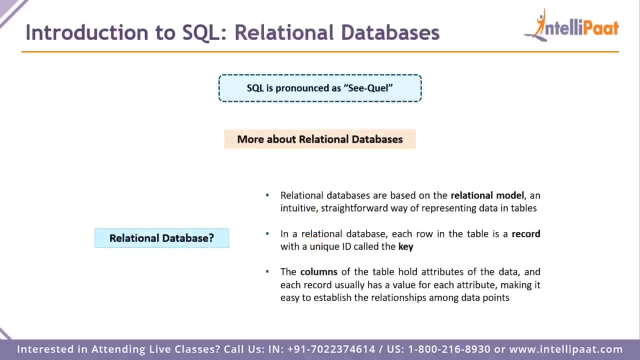 all of these provide relation between one column of the data to the other column of the data. guys, you'll see all of this in a couple of moments. but then coming to a little bit more about, uh uh, you know relational databases well, relational databases are pretty much. 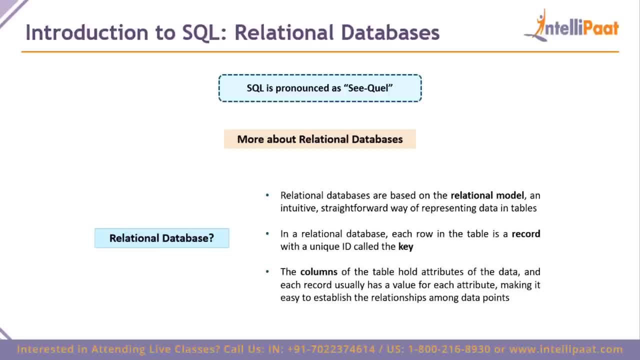 based on what we call as a relational model, where we pretty much map one concept to another, the other concept is mapped to another and we have this interdependency, interrelationships which are built throughout the data guys, and then this makes it very intuitive and extremely straightforward. uh, you know pretty much, it gives us a very straightforward way of representing the data. 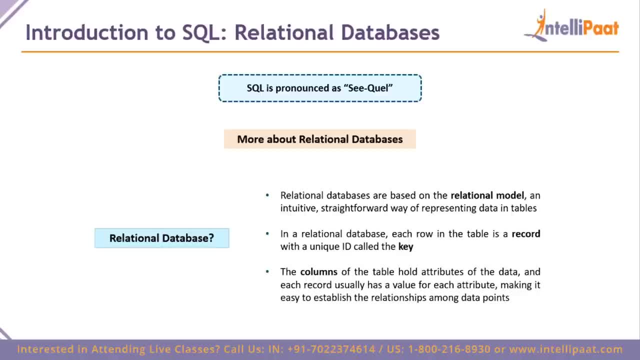 in the form of tables, as I just mentioned. and then the other good thing about the relational database as a, as I already told you, is that each row has something called as a record and there is some unique ID, called a scheme as well. again, we're going to check all of these in the upcoming slides, and then we have something. 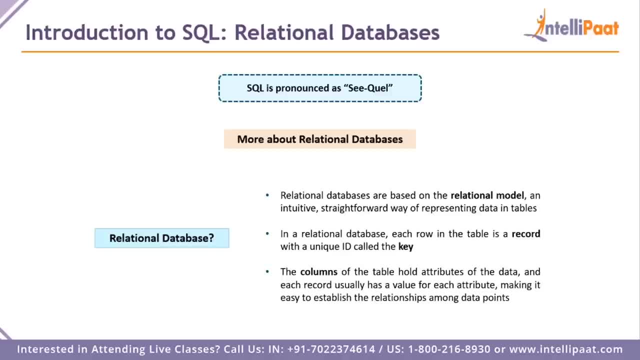 called as columns, which any data table will have, and then these columns basically hold all of the data, and each record in this column basically is uh mapped onto a unique thing, and then, you know, we go on about establishing something called as interdependency relationships and much more among 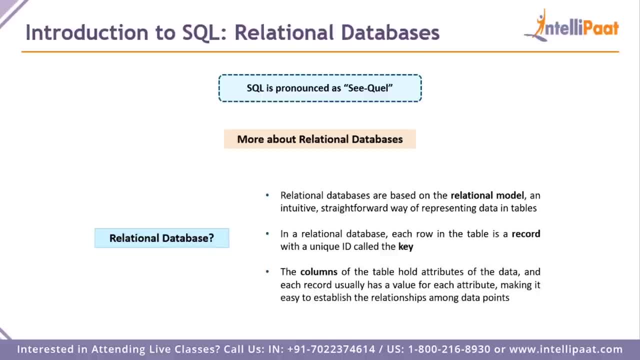 all of the data present, guys, and if you're wondering how SQL is pronounced, it is pronounced as either SQL or it's called sequel. guys, pretty much you will find developers, enthusiasts and many other developers either calling it SQL or sequel. so whenever you heard of the term, you know whenever 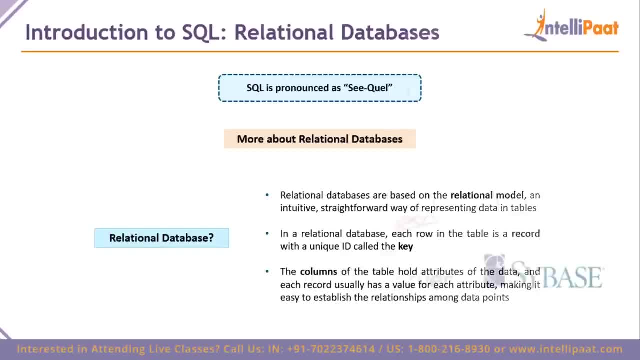 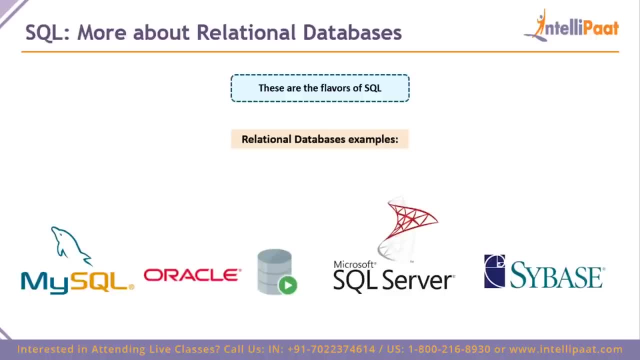 you hear the top sequel, uh, make sure to map it into SQL, guys. it's. it's pretty much simple and straightforward. so, uh, coming to you know a little bit more about relational databases. there are some flavors of SQL that I thought I should tell you guys. well, here are some of the examples of relational 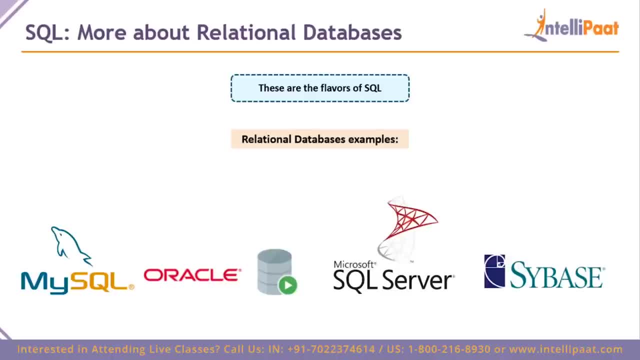 databases. we have my SQL, we have Oracle SQL, we have Microsoft SQL. uh, we have Sybase and we have. but the differences in between all of these providers are pretty much, you know, in in the shape of syntaxes, of how we pretty much talk to the database, and you know there are some proprietary 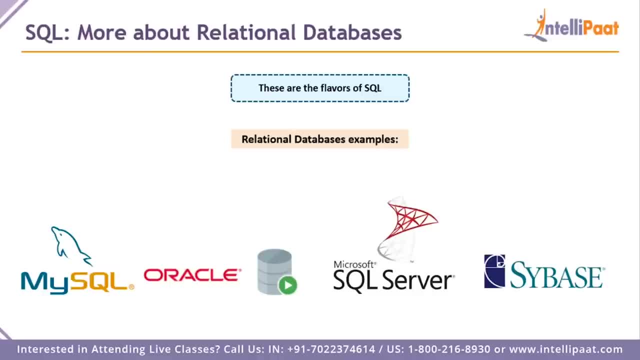 syntaxes as well, where you know those syntax only works with, you know, Microsoft SQL Server, and it might not work with my SQL and so on. but then it is recommended for all the beginners to pretty much go on to start with MySQL and then pretty much you know, jumping to any 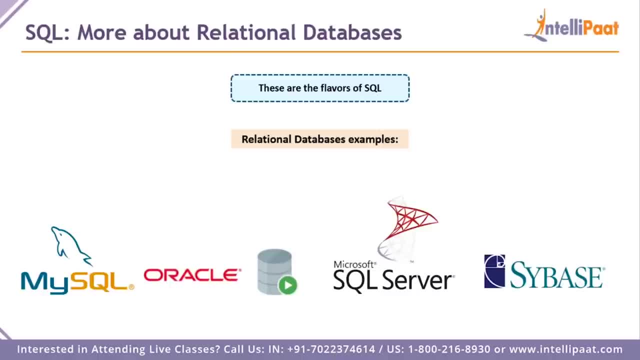 of these other providers, other flavors of SQL. it becomes very easy if you're a master of my SQL- guys note, make sure you stick till the end of the video, whereas, as usual, i'm going to give you a very attractive offer just for the viewers of this particular video, where you can fast track your 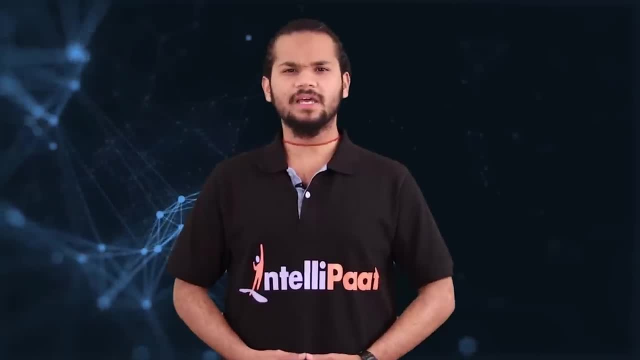 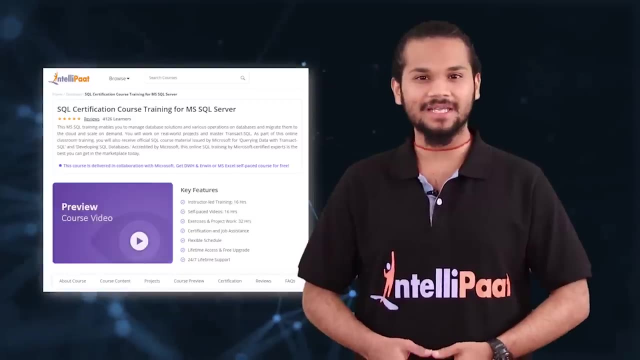 way to becoming a mysql expert. guys, just a quick info. if you guys are looking for end-to-end core certification in sql, intellipaat provides the sql core certification training program where you can learn all of these concepts in depth and earn a certificate at the same time. the link is given. 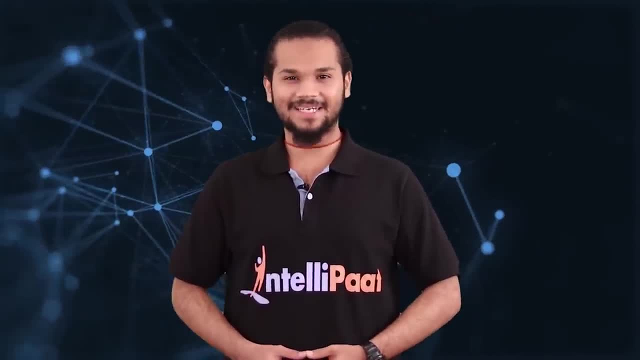 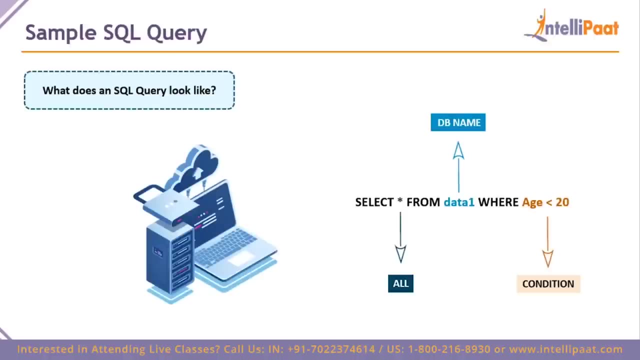 in the description box below. so make sure to check it out and, on that note, let's get back to the class. so, on that note, uh, we need to quickly check out, uh, what a query looks like. so a query is something very simple. it is the actual, let's say, the code we write, guys, in terms of sql. well, a. 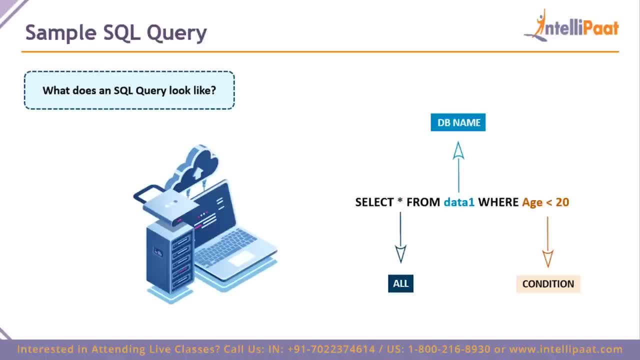 query will look something like this: think about you entering this in a shell or in a particular workbench, guys. so we have something called a select star from data, one where age is less than 20.. if you know a little bit of s sql, i'm sorry. so if you know a little, 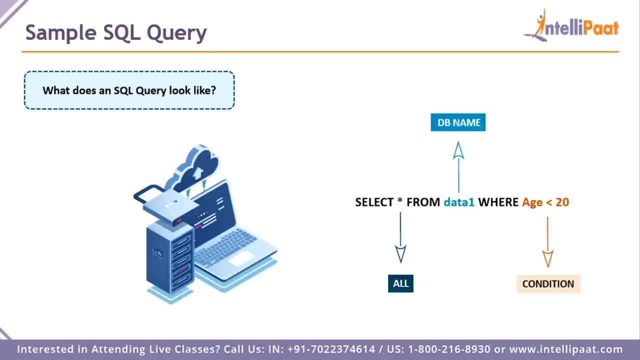 bit of sql, i'm sorry. so if you know a little bit of sql, i'm sorry. so if you know a little bit of bit of sql, then pretty much you can make sense out of this. but then if you do not, do not worry, because i'm going to walk you through what each of these mean. well, so basically we're going to be. 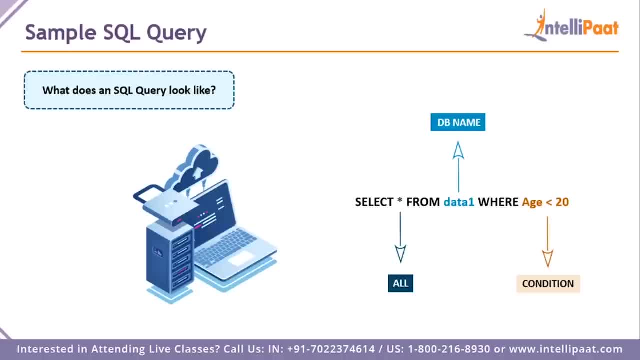 viewing a lot of data present in the database, right? so select statement is pretty much used to pick data from those actual servers and then show it to us. star pretty much means that you know, show everything that is present. everything from where? well, everything from a particular database. that. 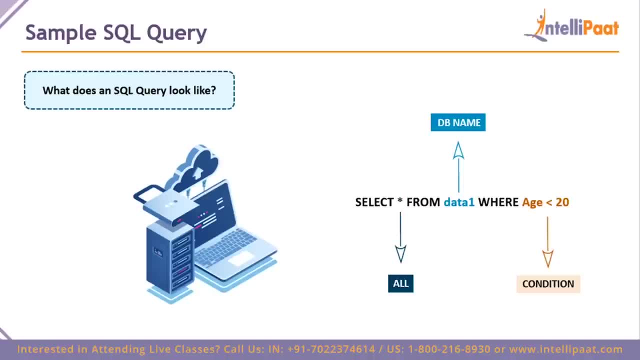 we have, and that database in this particular name is called as data one. and so do you want to see, just see everything from data one? well, no, i want to see some stuff from data one where the age of a person, let's say. we have talking, we are talking about a table which contains details about a lot. 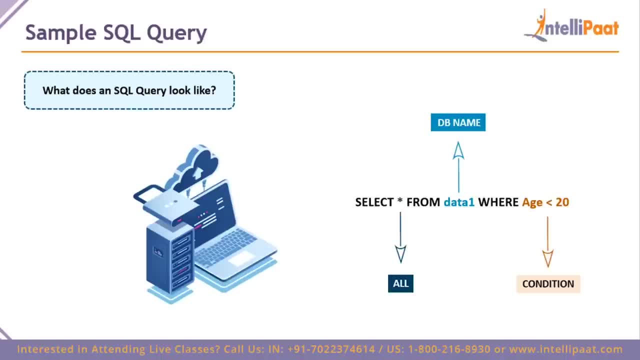 of human beings or college, you know, college people, school people and whatnot. so we just want to find out who all are less than the age of 20. so, when you think about it, uh, instead of just seeing millions or thousands of entries of students who are, you know, aged, 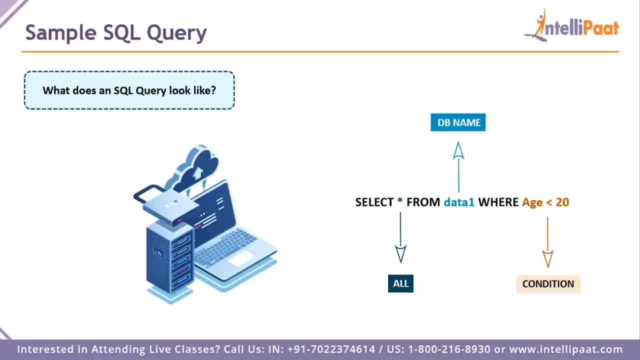 various from i don't know three to hundred uh. but then when you're thinking about uh efficiency, then we need to bring it down to a certain condition where we go on checking it right. so instead of just seeing thousands of entries, let us say we only require 11 and we're going to see 11 entries. 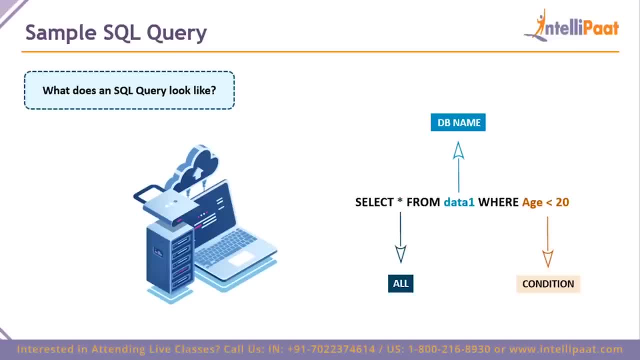 when we put the condition saying age is less than 20, because there are only 11 people who are less than 20 years old guys. so pretty much this is what a sample sql query would look like, and we're going to see 11 entries when we put the condition saying age is less than. 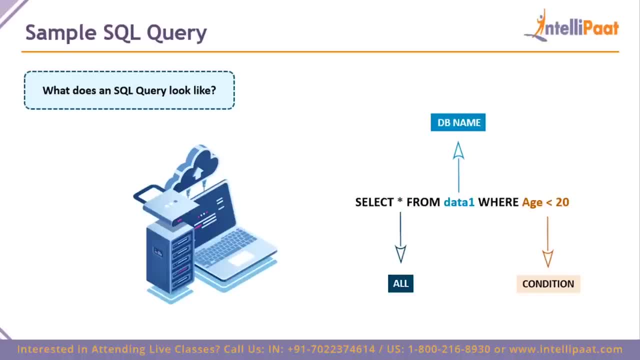 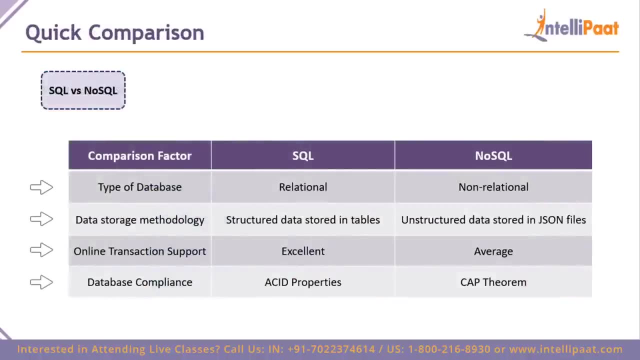 20 years old guys. so pretty much this is what a sample sql query will look like and, uh, we'll just be doing very simple operations at the end. you can follow along, in fact, and pretty much we can check out a little bit more about queries then, guys. but then when you think about it, i'm sure you guys are. 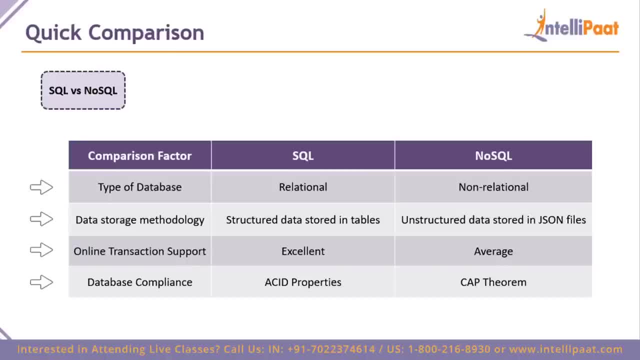 also curious as well. so there is something called as no sql as well. so how can we go on juxtaposing and comparing sql and, no excuse, no sql? well, uh, when you think about it, uh, the types of databases in sql, as i just told you, our relational database, where each of uh the data is mapped to, the 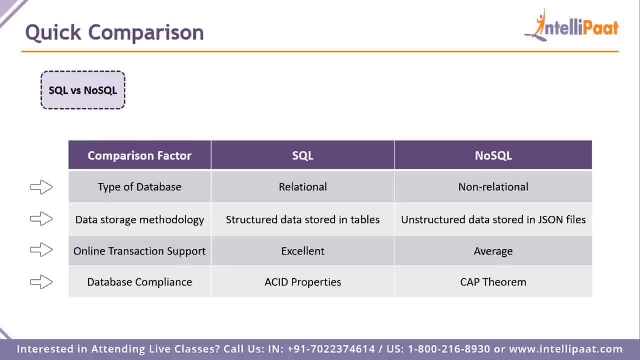 other by using keys in terms of no sql. we do not have relational. that's why it's called as no sql, guys. and then how is the data stored in sql versus no sql? again, structured data is stored in tables in terms of sql and in terms of no sql, unstructured data is stored in something what we called as json. 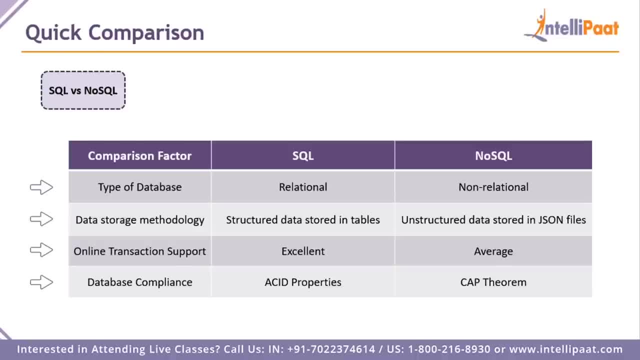 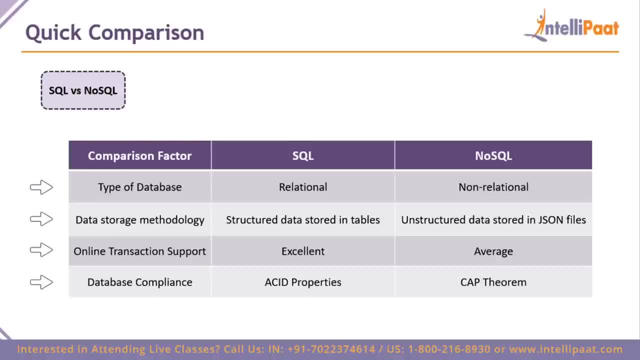 sql has excellent support when it comes to, you know, online transactions and no, sql pretty much just has about average uh online transaction support guys, when you can think about it. no, sql sure has its amazing advantages but then uh, pretty much sql stumps it in terms of online transaction. 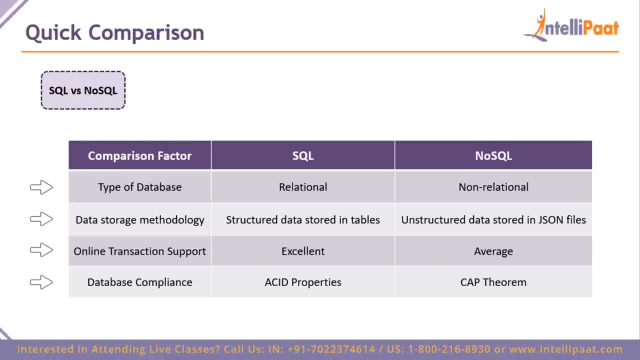 support and then, coming to database compliance, we have something called as the asset properties in terms of sql and we have something called as a cap theorem in terms of no sql guys. so we pretty much have an entire in-depth video of mysql, where we have a lot of data and we have a lot of data. 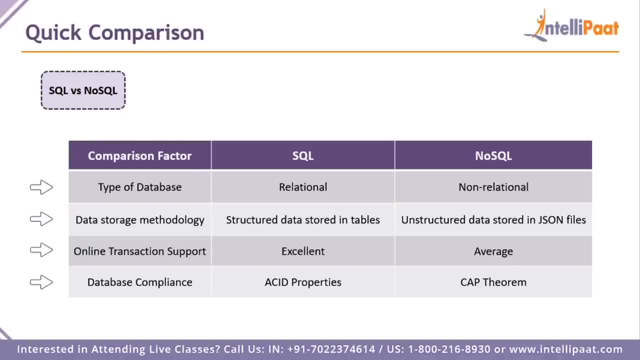 sql, where we train you on everything from the basics all the way uh, uh to a level of uh to an advanced level, and it's about uh. it's. it's on our youtube channel, so make sure to check it out if you want to know more about all of these data, data storage techniques, asset properties and much more. 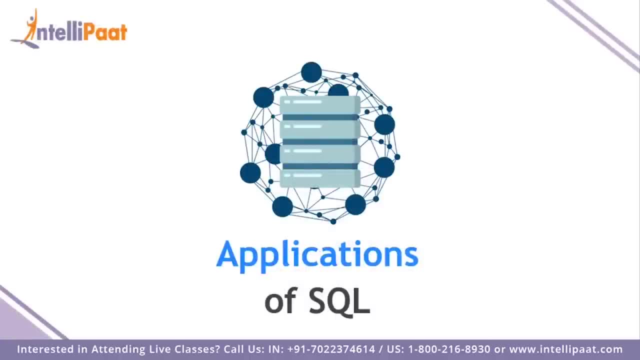 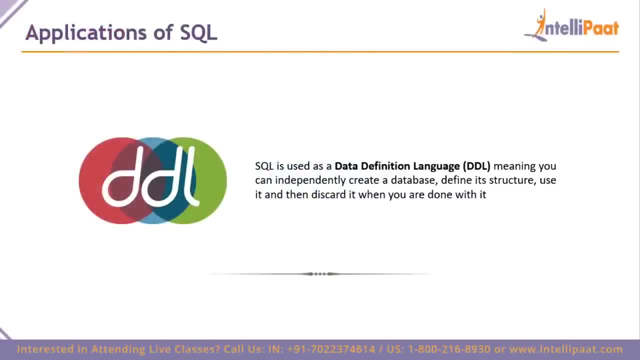 guys. so, on that note, this brings us to. this brings us to the applications of sql. so sql has a couple of applications, and let me tell you one by one. sql can be used as a data definition language- ddl for short. uh, what this basically means is that you can pretty much, you know, create a database on. 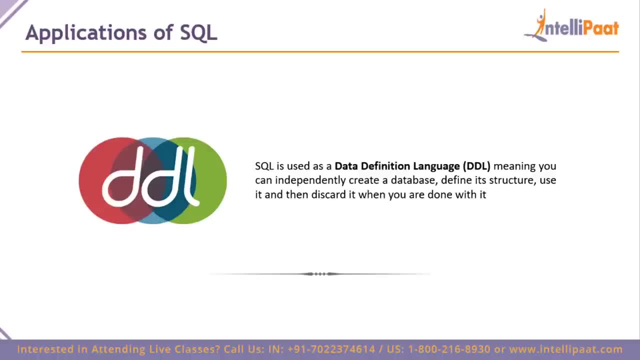 your own, define its structure on your own, use it on your own and, just you know, discard it when you're done with it. so this, this doesn't have to be just you. this can be among hundreds and thousands of people. you can scale it, obviously, but then know that, with respect to data definition, language, you 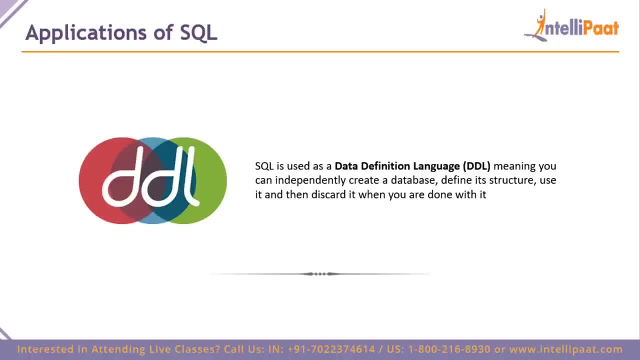 have all the right where you can individually create a database, define the structure and delete it when you're done with it as well, guys. and this brings us to the next application, which is data manipulation language, because sql can be used as dml as well. so what it basically means is that 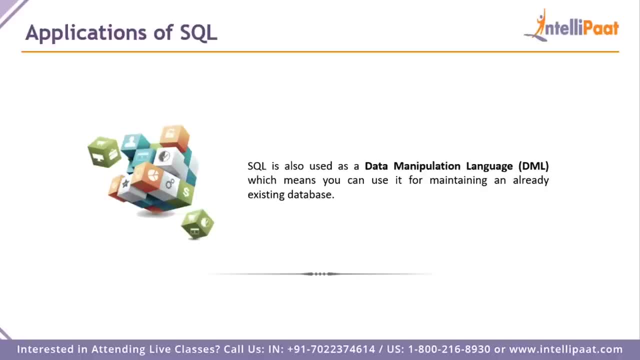 uh that you know, when we have something already in establishment, like uh data, which is already present in our database, we need to go on changing something in that database. we need to update a database, we need to delete a row, we need to update a column, and so much more so in that particular. 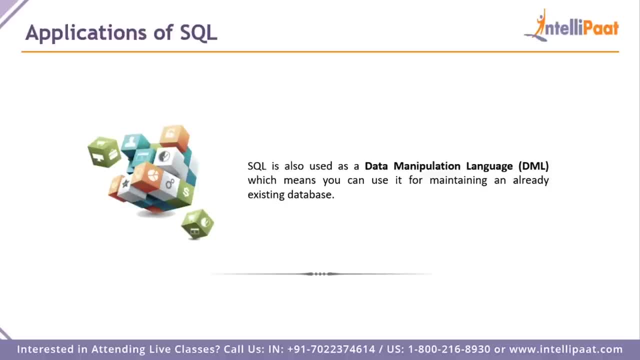 case we can use sql as a data manipulation language where you can pretty much alter stuff in the table. you can go on adding, removing and whatnot. so this brings us to the next application, which is the dcl guys data control language. so data control language is mainly. 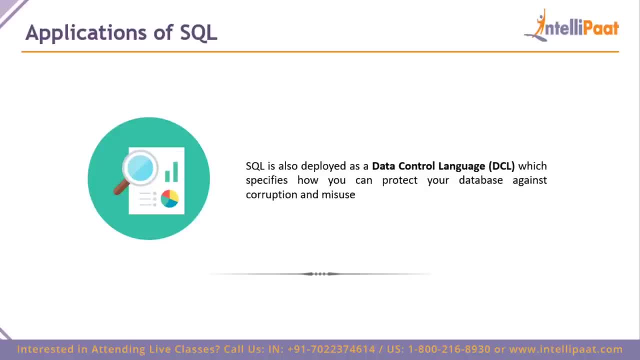 concerned with your data in terms of how you can avoid corruption and how you can avoid misuse as well. so, pretty much as you know, data has to be protected and, uh, misusing data is extremely easy, uh, even though with all the security measures, these tests. so, uh, you know, sql can pretty much. 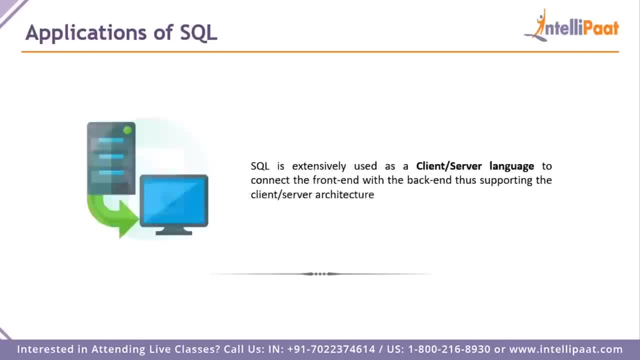 be used in terms of dcl, where we can, you know, protect the databases against corruption and misuse in a very good way as well, guys, and the next application of sql is pretty much that. uh, it can go on to be used as a very good client server language. you can, uh, pretty much so, program on the client side and the server side. 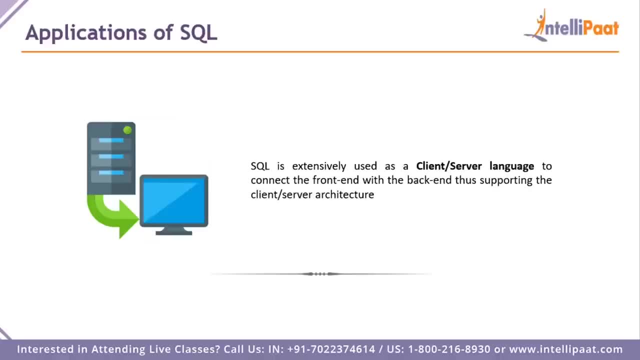 where you can, you know, connect front ends and back ends together, where we have an entire architecture which is set up. what we call is the client server architecture, where there is one server and then, I know, there are lots of clients. I'm sorry about that, there's lots of clients you. 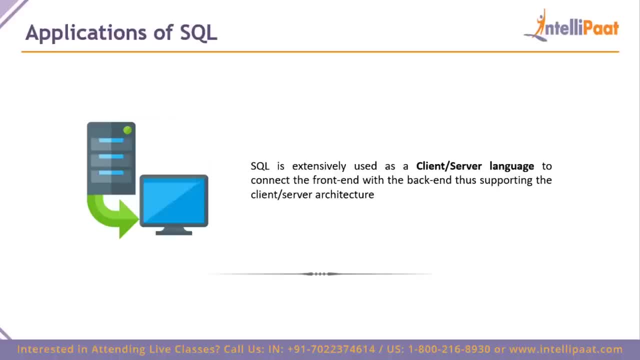 know connected to that particular server and then we pretty much, you know, go on hiring and talking to the server, getting the details from the server for each individual client and more guys. so the next application pretty much is what we call as the three-tier architecture. the three-tier architecture is something very similar to the client, uh server client architecture, where 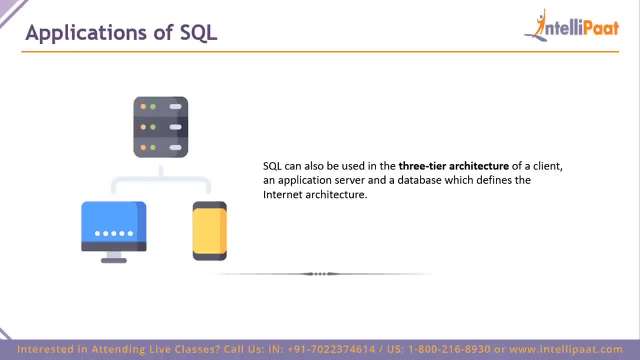 you know pretty much, we have something called as an application server, we have a database and all of these together in terms of the server, the client and the database form, uh, the three basic tier architectures, guys. so it's the client, it's the server database, where you know the data is uh present and it can be, it can go through the server, where 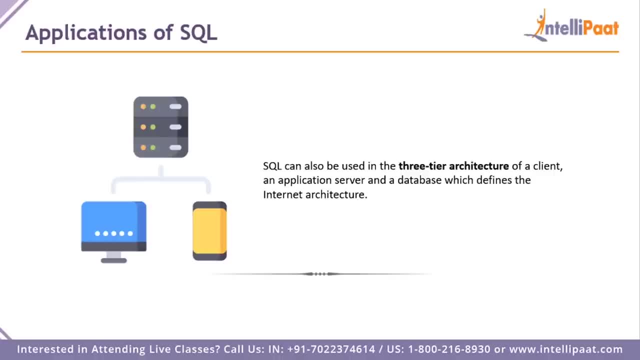 it can go to multiple machines or pretty much. you can have it come to the server and talk to the client directly as well, guys. so on that note, what do you guys think about the applications of SQL? can you think about any direct uh applications of SQL? if you can think of it, make sure to head. 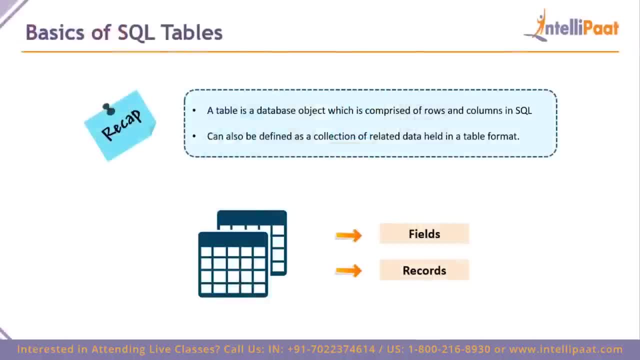 to the comment section. right now we can check out the basics of SQL tables really quickly, guys. well, uh, as I've already told you, let's have a quick recap. a table is basically a database object which is comprised of rows and columns. in SQL, we already saw that it is the structured way. 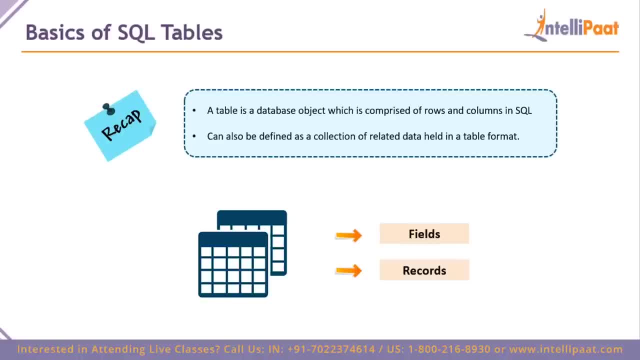 of going about, uh, using data, a table, and then it can also be defined as the collection of, you know, related data held in a table. it is related by the forms of keys, uh, which I told you, but then there are two things that I'd really want you guys to visualize, which is basically fields and records. 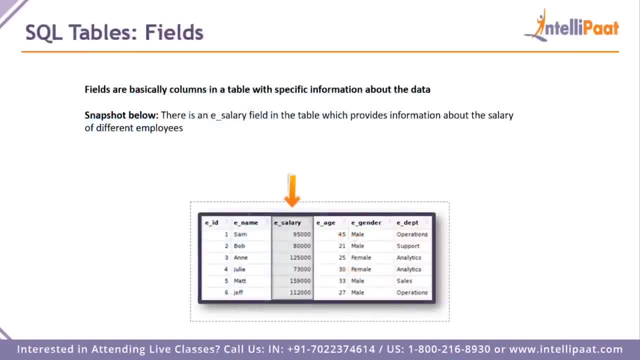 well, fields are very simple, guys. fields are the column where you know we have specific data, under which some we have a field called as e underscore salary. let's say it's employee salary, and this salary, pretty much you know, uh, is is the information which we provide. but then we have one header under: 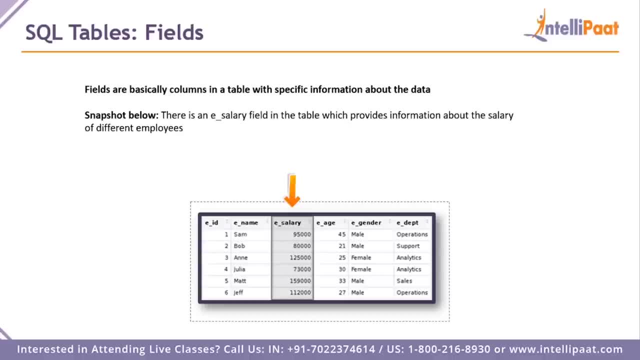 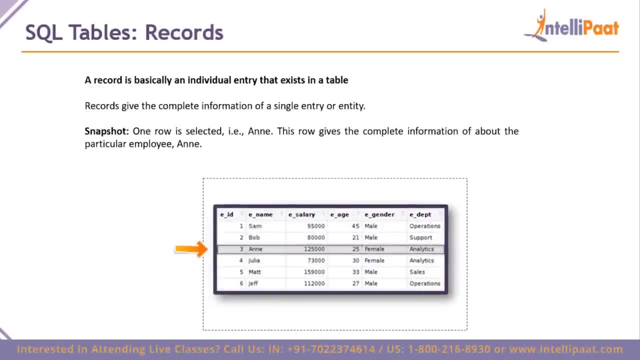 which the salaries are all coded right. so this, basically, is: this is the salary field. this entire column is what we call as a field. and then when we come to records, records is something very simple, because what is the record corresponding to a particular field? uh, well, let's say we want, uh, the 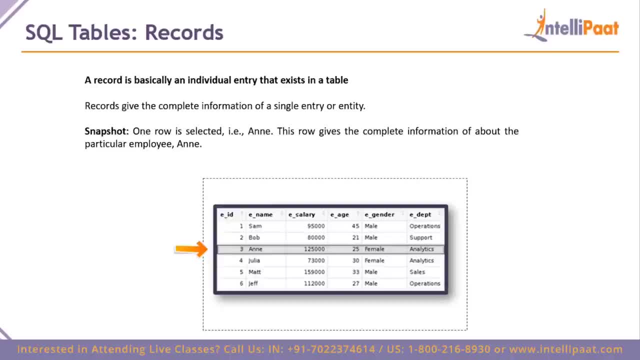 uh, here Annie pretty much goes on to, uh, you know be the employee ID 3.. uh, it's under the employee name. we searched it through the employee name, right? so we said we want to find out Annie. so Annie is pretty much the employee's name and the employee's name was the field and the record was 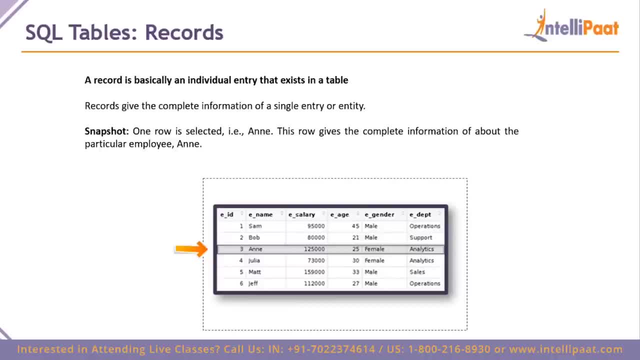 number three, right, so it's pretty simple. uh records give us an entire description, a complete information of all the entities present in that particular uh data set, guys. so you know we already have of data on the screen. but then when we highlight one row- uh, the annie's row, pretty much this row. 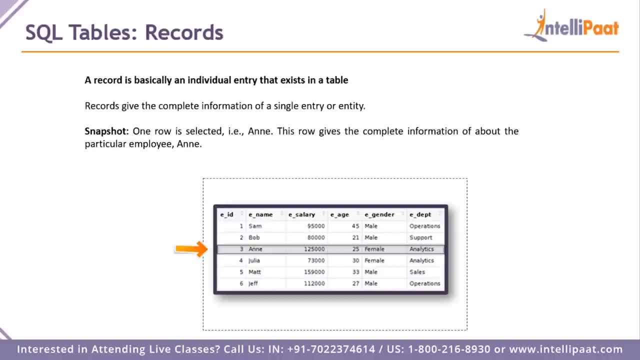 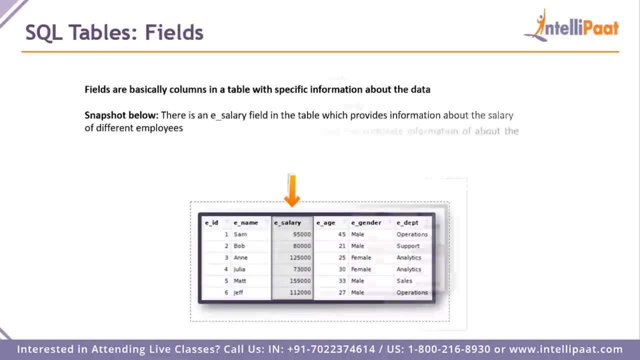 gives us the complete information about that particular employee guys. so this is what we call as a record. let me quickly step back, where you can see fields again. so this is the field, guys. the field is the column. the record is a single entity which gives us complete information. 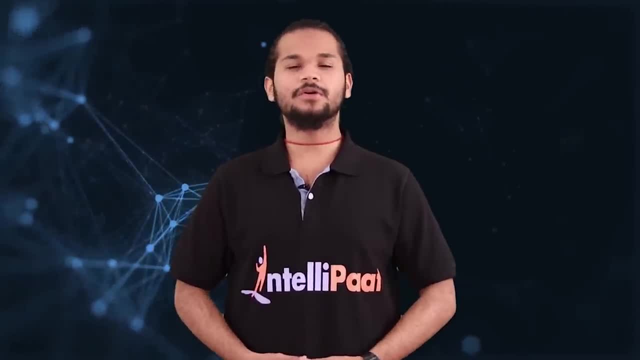 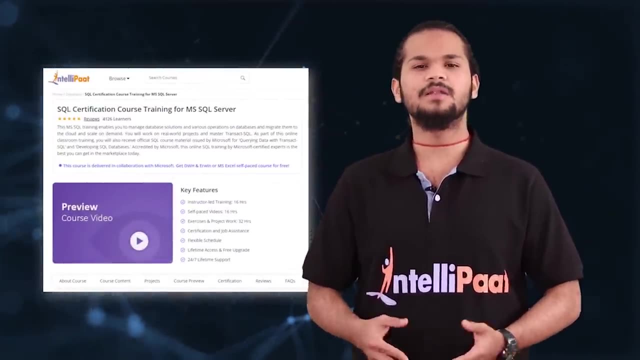 i hope i was clear with that. just a quick info. if you guys are looking for end-to-end core certification in sql, intellipaat provides the sql core certification training program where you can learn all of these concepts in depth and earn a certificate at the same time. the link is given. 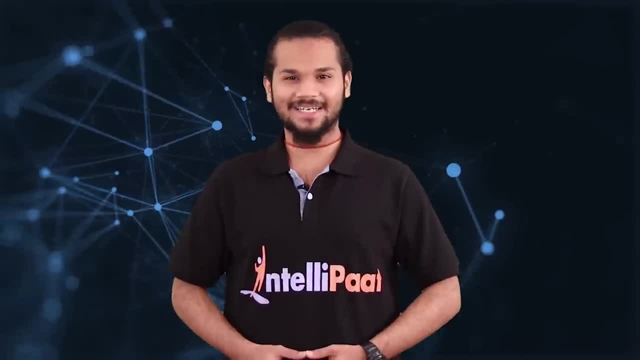 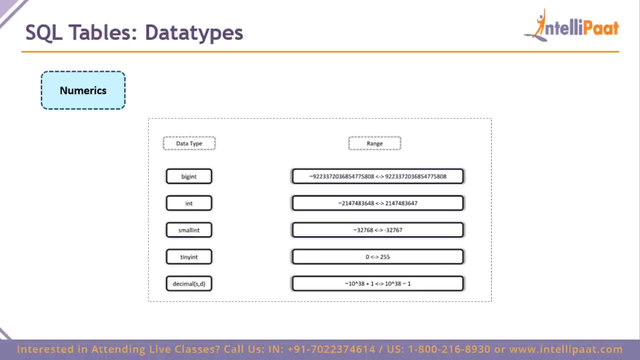 in the description box below. so make sure to check it out. and on that note, let's get back to the class. so this brings us quickly to the data types which are present in sql guys, so i will not go in depth, uh, because we need to keep this tutorial to the scope of all. the viewers are present tonight with 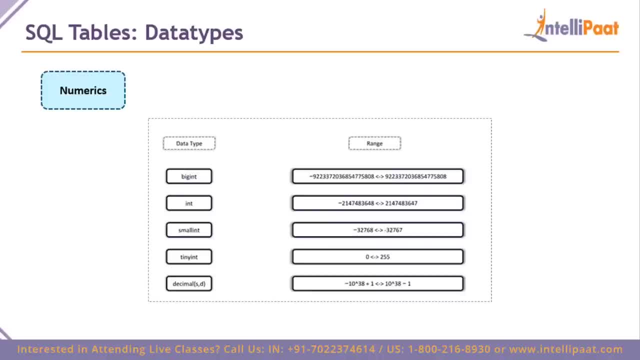 our session. so, basically, uh know that you can have numerical data, character data, date and time data and much more. with respect to numeric data, we can have integer data, decimal data and all of these as well. so, basically, what you have on your screen is the data type, but with the corresponding range of the numbers that you can use, so you can see a. 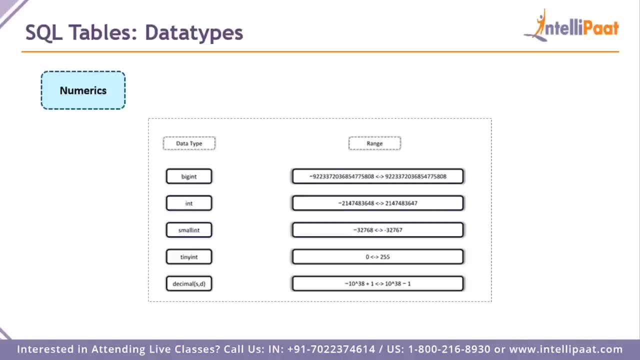 big number there, which is nine, two, two, three, three, seven, two zero, three, six, five, four, double, seven, five, double. you know, five, eight, zero, eight, right, so this one particular number, if in case you want to put in a number, uh, you know, say you want to put a phone number, you want to put an address. 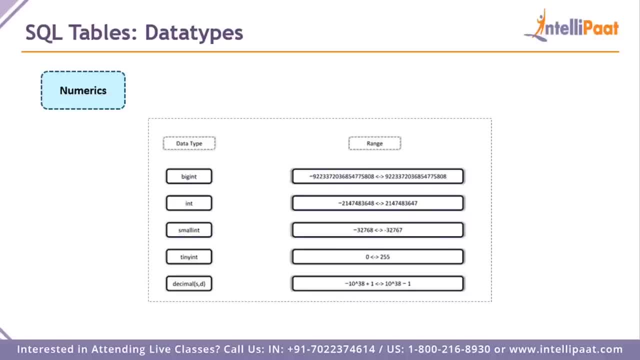 or whatever it is, and you need this amount of number, the huge number, then you've got to use uh, the data type, what we call as the big int guys. then the normal integer supports pretty much uh in the data range that you can see on the screen. a small end is a fairly smaller number somewhere. 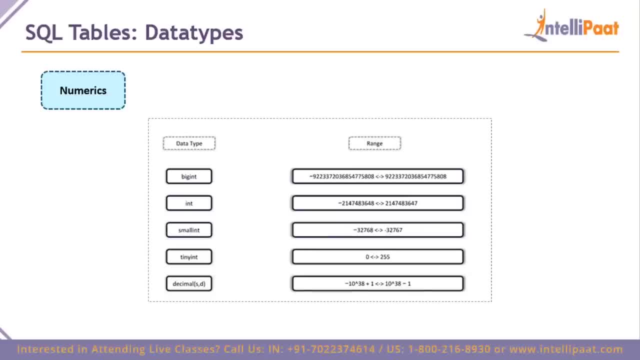 around 32 000, and tiny int is even smaller, where it only supports positive numbers- between 0 and 255 guys, and then with decimals as usual, you have a huge number. i access to huge numbers on the negative side and on the positive side as well, guys. so this brings us to characters. 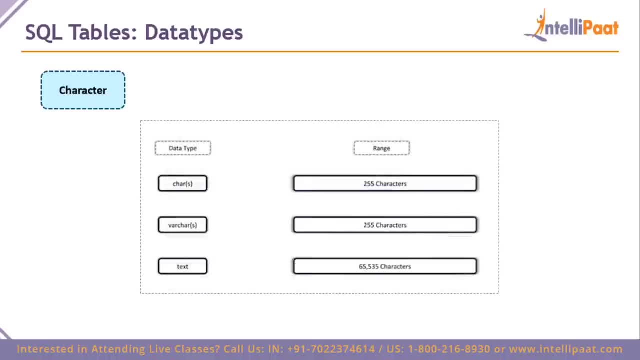 there are three main data types. one is the car, one is the varchar and the text again. pretty much, it is as simple at this point of time. you need to know that you can have 255 characters at once when you're declaring something, when you're declaring the name of a data type, or when you're 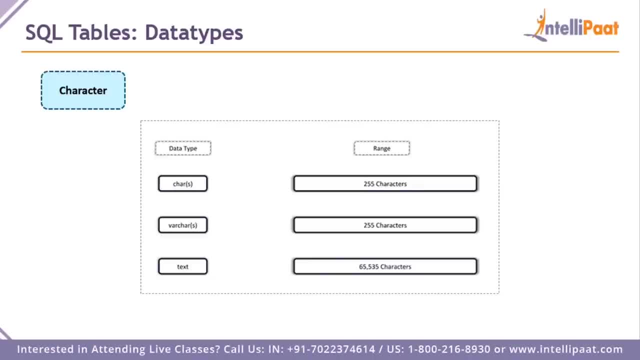 putting in the actual data for the data type as well, guys. so, but then we have something called as text, where let's say, you want to put in a description of something, so this, it will be a limit if we actually uh say 255 characters. right, so for that particular case, uh, you know the. 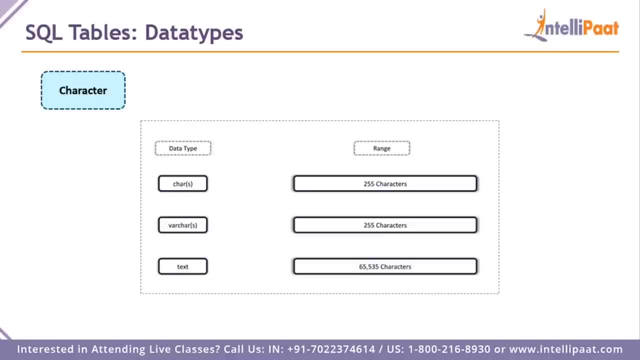 standard sql manufacturers pretty much have given us a range of 65 535 characters where you can pretty much i think that should suffice. uh, you know most of the applications where we're using the data type text, where we are actually putting out some sort of description guys, and then this: 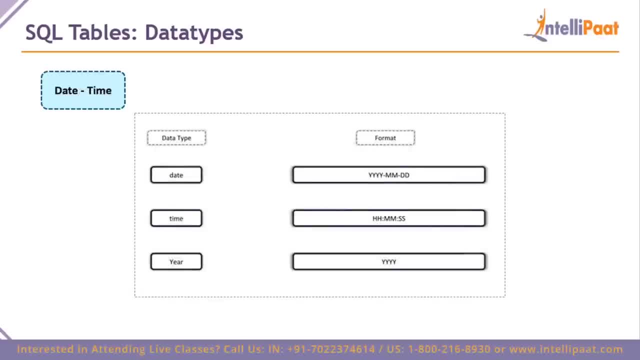 brings us to the date time data type. well, basically, you can go on to using date format in the format, your month, day, and then you can go on to use the time as well- time in terms of hours, minutes and seconds as shown on your screen- and we can just use the uh data type here: uh, by showing 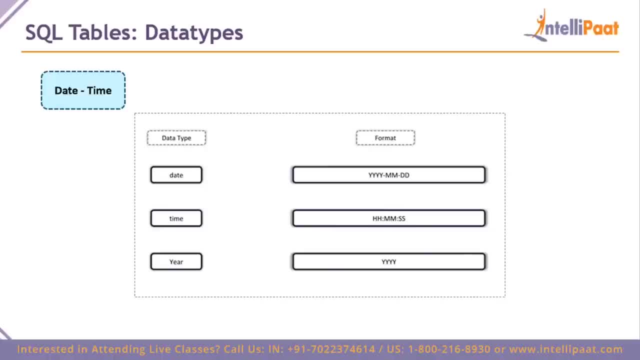 uh, you know by seeing the uh format on your screen as well, guys. so why, why? why pretty much means four numbers. uh, if you have to put it down right now, it's 2019, it's 2019, so that'll be, uh, the format of the year for now, guys. so this brings us to something what we call as crud. 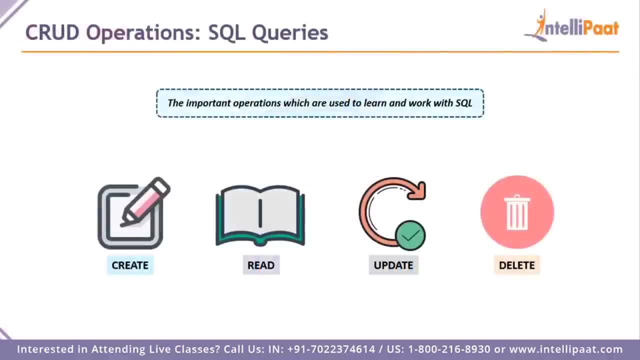 operations. crud operations is where we'll actually check out some quick sql queries where, uh, but first you need to know what crud stands for guys. so every time you begin to learn sql, or you're revising sql, or you need to understand what sql is, you will begin with crud operations as your first. 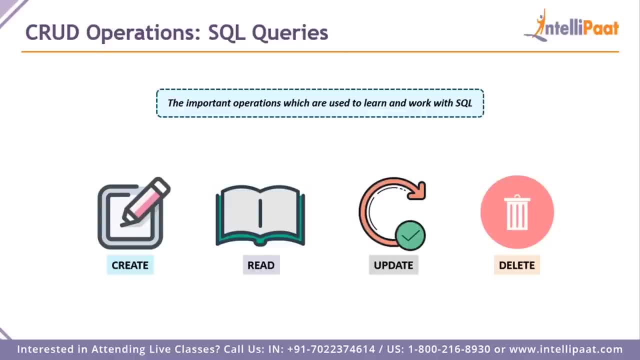 way of measuring utungs as it stands on the real world, right? so if you want to unbuild a single object, you can load multiple nous product, for example, you know, on youtube or endcom or for example just really normal, very něch adjust them. usually they're so easyvos it's like a static module. so basically, you see, once we create the table part audit. customer. célось allcareen here, so let us just give a quick space. i've chosen this particular thing to show it to you guys see in crud stands for create, our stands for read, u stands for update and d stands for delete guys. so these are some of the operations we can perform. 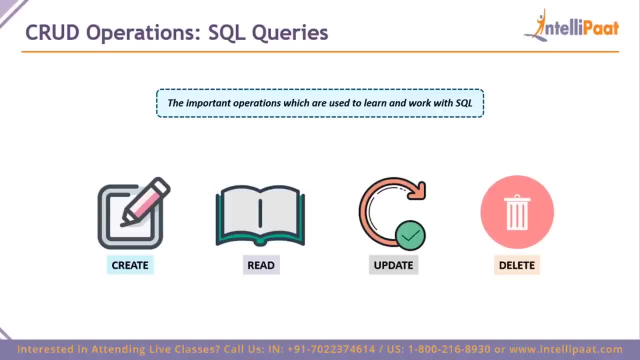 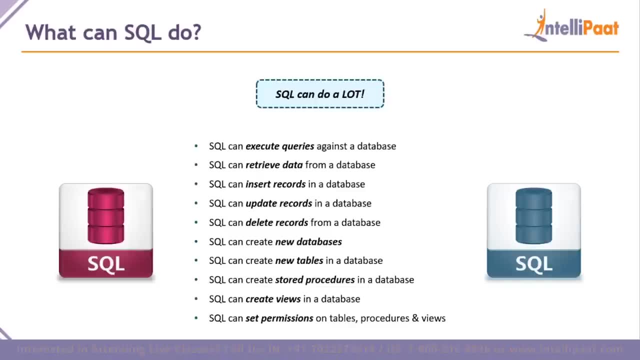 on a database so we can perform a create operation, we can create something on the database, we can read stuff from the database tables, update tables and so much more as well, guys. so on that note, what can sql do? we talk? we're talking a lot about. you know, sql can do this, sql can do that. but then if you have to put everything, 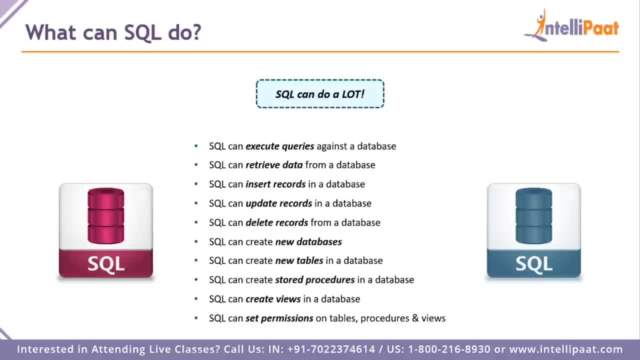 under one header. this is what i would say, guys. sql can execute queries in a database. it can retrieve data, it can insert the record into a database, update the records, delete basically the crowd operations. it can create new databases, create new tables, and then you have something called a stored procedure, which is basically like a ready set of commands. all you have to do is you. 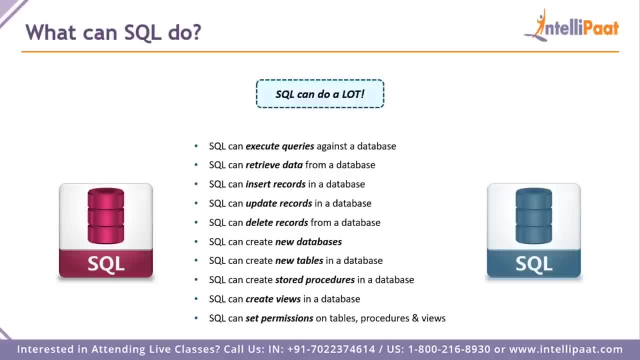 know pretty much, just run that stored procedure and it will run lots and lots of commands for you at once. and you know, let's say, let's say you're a huge organization, you do not want to type queries every single time and there are thousands and thousands of lines of queries. 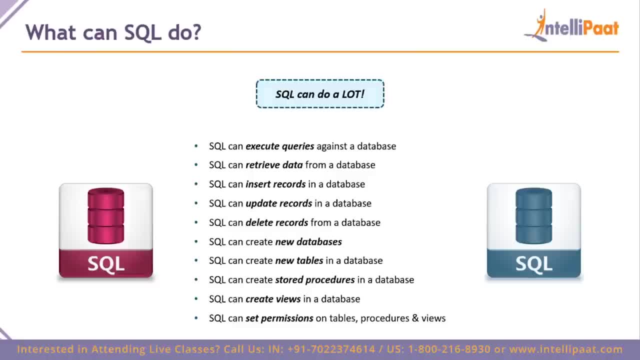 so a stored procedure is basically a saved file where you just run it and it runs all of these thousands of lines of queries for you to pick whatever data you're looking for in a database. so it's basically like a shortcut, and then sql can create views as well. views are these temporary entities where you know, let's say, 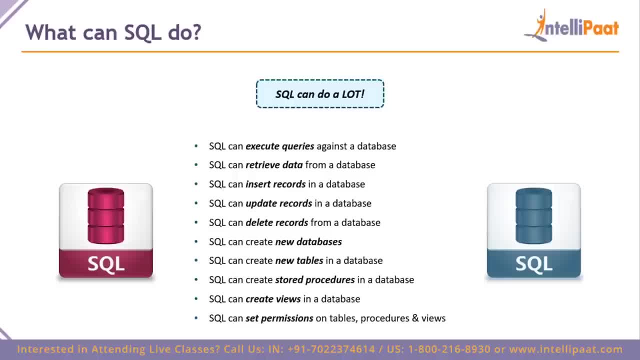 our data. our table contains thousand rows where we don't want to see thousand rows, or thousand columns in fact, so we just want to see three columns and three entries. so in that case we create something called as a view, where we only pick these stuff that we want to see, and 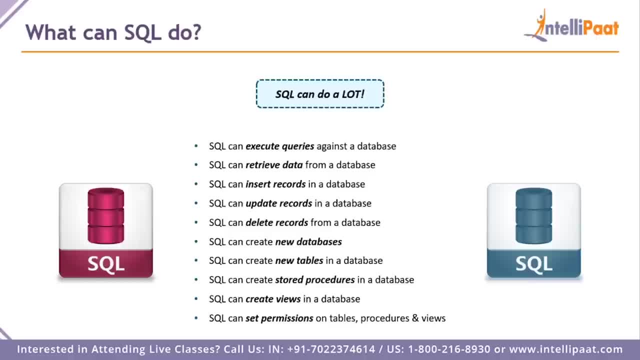 then we show it on the screen. it's as simple as that, guys. and then, coming to permissions, as we already told you, it offers very good security measures and we can set any permission for any person accessing the. you know, any client accessing the database, and then we can set. 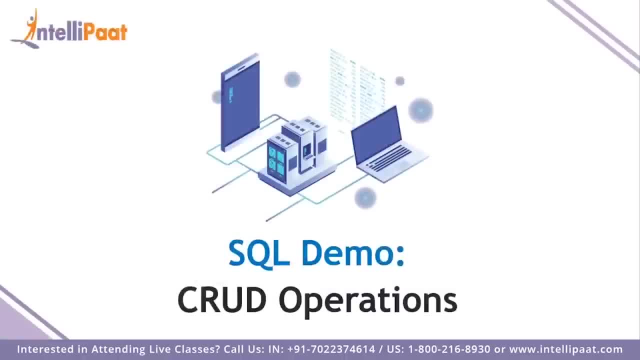 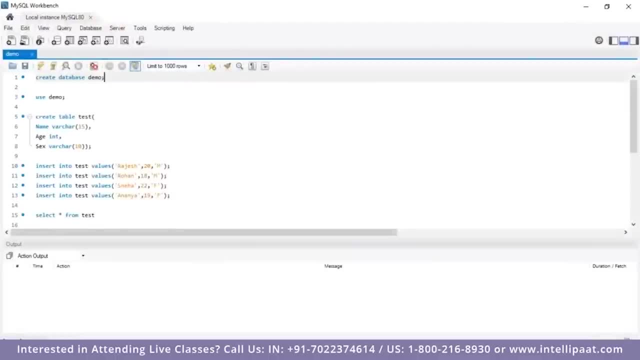 a database on tables, procedures, views and so much more, guys. so this quickly brings us to our crud operations demo. well, let me quickly jump into. uh, mysql workbench. so mysql workbench. again, this comes completely with the sql server installed. uh, it gives you a workbench, it gives you a, a platform. 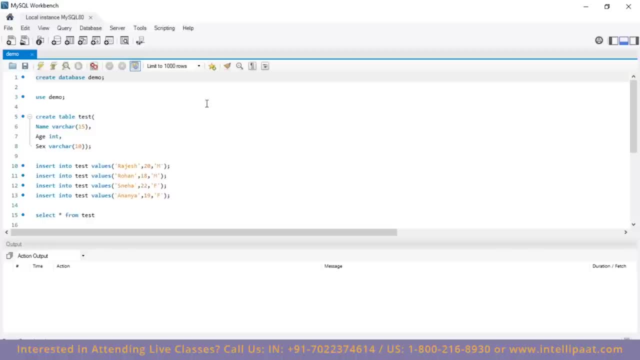 to basically write your queries guys. so i have pretty much written down a couple of sample queries for you guys to just take a look at and work with and let me work with you on every single line of query that we've pretty much written. so the first query says create- 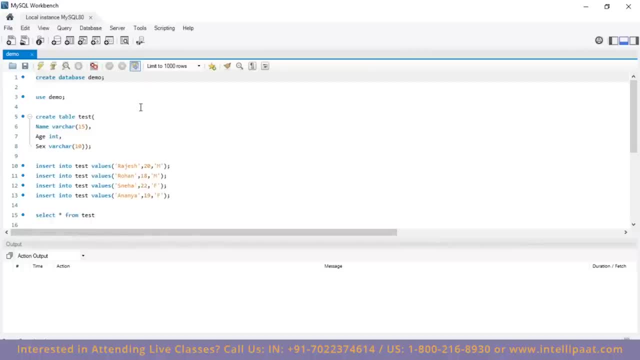 database demo. this line is fairly simple because you can pretty much. it's it's a very high level language, right? so we're creating a database entity and we're calling our database as demo. this particular name is extremely important because you're going to be using it a lot, guys. so 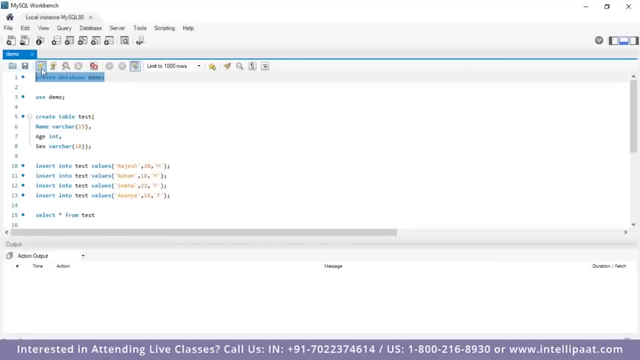 the first step is to create a database, and let me quickly run this query. as you can see, our database is created now. so, uh, we just created one database and we left it there. so think of it as a box, where you just close something in a box and put it next to you. so unless you actually open that box and 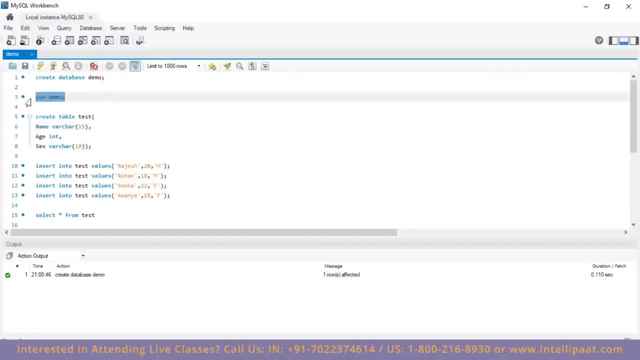 you know, start using stuff, it won't make sense, right? so then we actually use the query, which is use demo. demo is again it's basically used, followed by the name of the database. so use demo will pretty much uh open that uh database box for us where we can work with it on the inside guys. 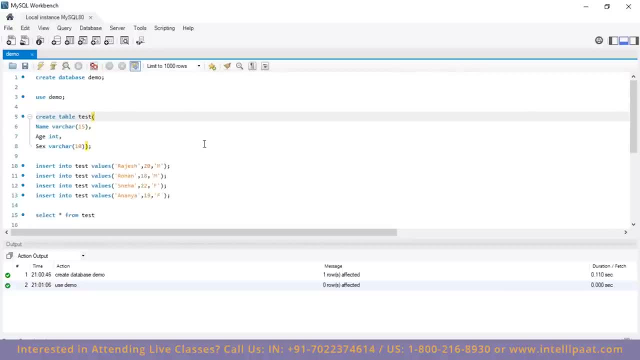 and the next query is, uh, something very simple, where we're going to create a database and we're going to create a table where, you know, our database is again a plain entity, right? so we need to create some tables there. so, in this particular demo, i'm going to create one table for you guys. 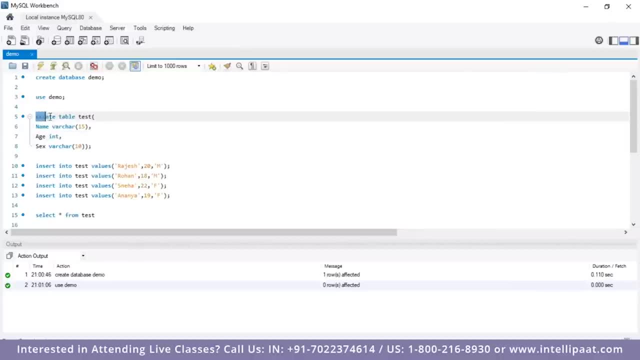 using this very simple syntax. so the actual syntax to begin with creating a table is create table. uh, the table name in my particular case is test. well, you can have it anything that you want, and we're going to open a bracket where, uh, whatever command we put in this particular uh, uh, you know. 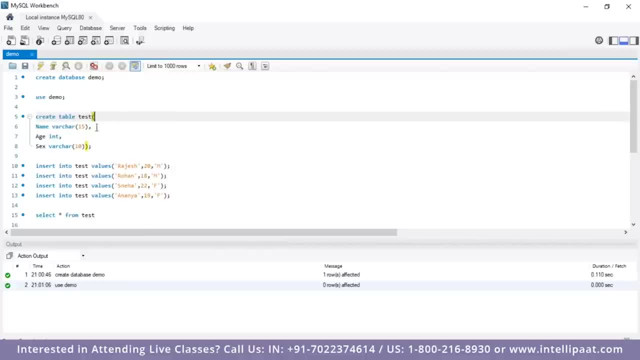 as a parameter needs to be under this parenthesis, guys. so, as you can see, we have highlighted one and one for me. so whatever from here till here pretty much goes on. uh, it goes on under the create table header, guys. so i've created three columns for my database. one is the name. it's a varchar. it means 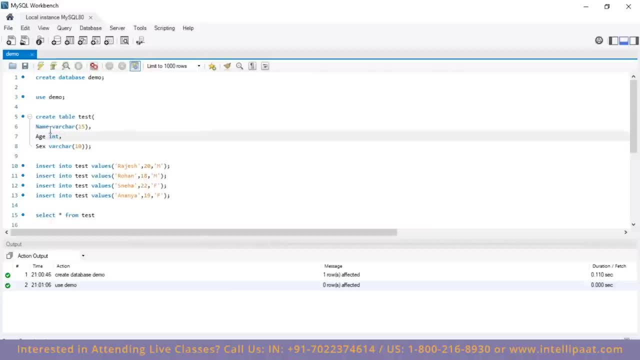 it's a character, name is a character, right, i cannot have name as two and three and whatnot. and then we have age. age is pretty much the integer as we uh, pretty much can use, go on using. we don't have to use short end, long end, uh, you know, tiny int. and all of that because, again, 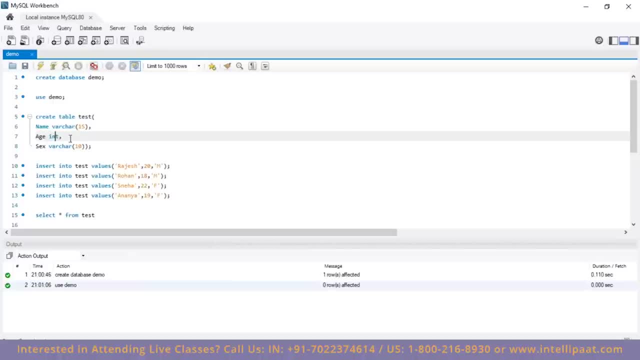 uh, we know pretty much, if you're going to work with a human age, it's going to be somewhere between zero and maximum 100 or something right. so int will suffice. and then we have the uh pretty much if the person is the male or a female, and more so pretty. 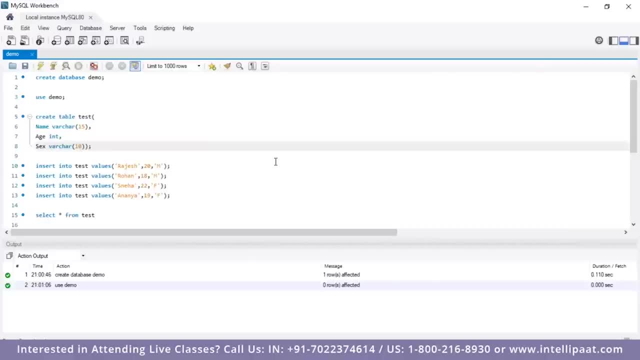 much that. that again is a single character, so we're gonna use car varchar and we can go on using text as well if we want, but then that's a waste of memory, guys. so as soon as i run this particular query, i'm going to select this query. i'm going to run it as soon as i run this. what it does is: 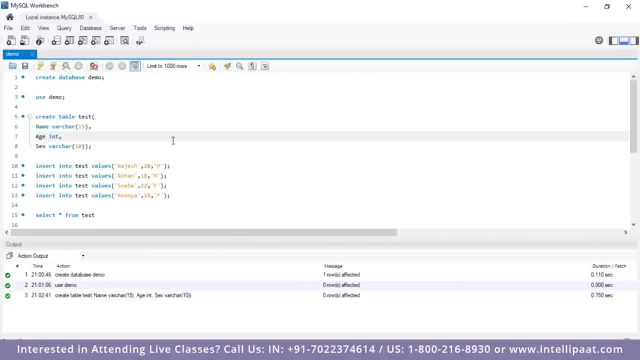 our database is now created, our table is now created, and then we just created an empty table, so we do not have any data in our table as of now. so to quickly change that, we're going to put in some data into the table. so the command we use: 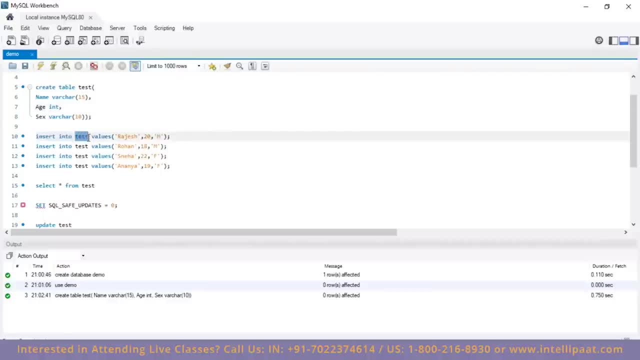 to put data into the table is insert into, followed by table name and values, and this is the most simple way you can go on to insert a test, insert a value to your table, guys. so, uh, we're gonna have to map it in the way that we have created. so i've created it as name, age and sex. so 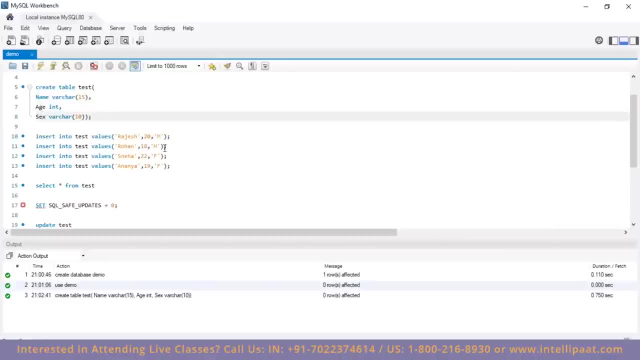 i need to go on to define name, define age and define the sex guys. so, uh, the name is name of this particular entry is rajesh. his age is 20 and rajesh is male. and then we have rohan, who's 18 years old. he's a male as well. then we have sneha, who's 22 years old, and she's a female. we have 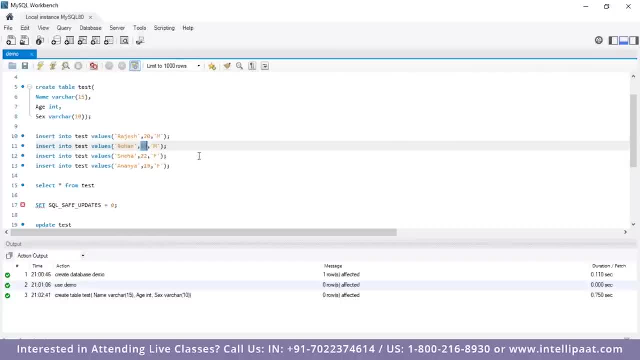 ananyam, who's 19 years old, and she's a female as well, guys, so we can run this query individually. where we know, we go on adding one by one, one by one, in fact, i'm going to show you that right now. so, if i go on to run this query, 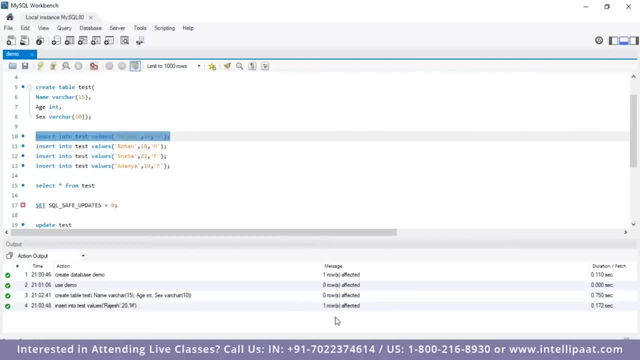 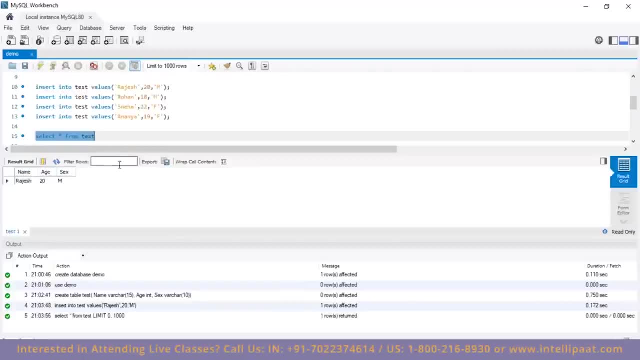 it says that you know one row has been affected. it means that you've changed something in one row of your database. so give me one second. let me run this for you, guys. you can see here, right? so this is the output. basically, this is what we call, as a result, grid guys. so here we can see that. 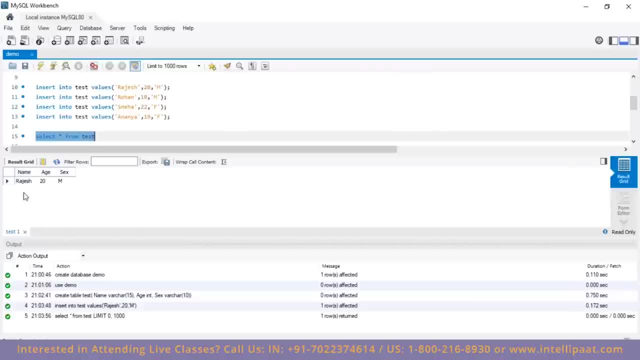 there is a date table created, basically, there's a database created. there's a table inside the database where the name is rajesh. he's 20 years old and his male, so we just used one of these, right? so let me run all of these and then we're going to run this command. select star from test. 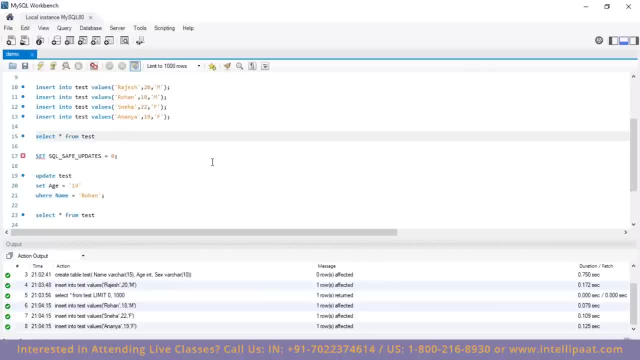 you might have seen the- uh, you know pretty much the basic sql query command that i showed you at the start of the session, where we had something more like a where clause and whatnot. right, so we can use that as well, but then this will give us the entire entry present in our date. 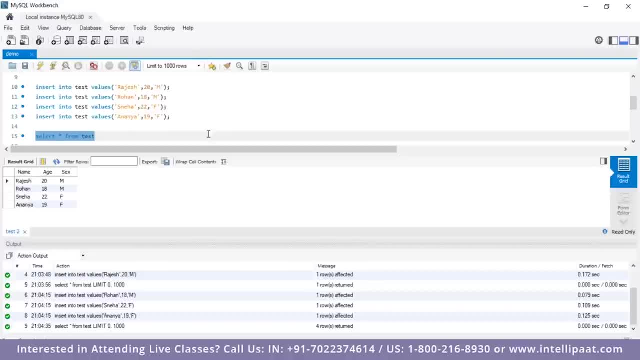 uh, present in our table. so as soon as i run this, instead of just rajesh, all of the all the four entities are present for us: rajesh, rohan, sneha, ananya and more guys. so it is pretty much, you know, as simple as. let me quickly bring this down a little. 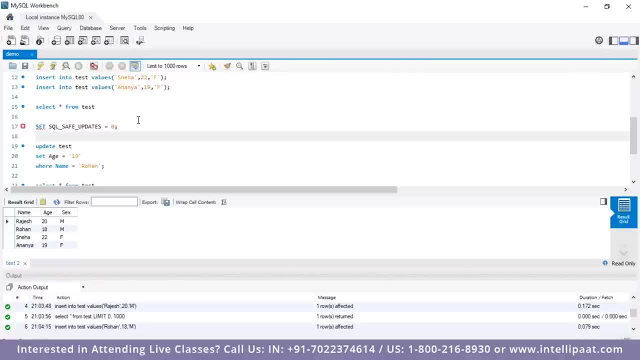 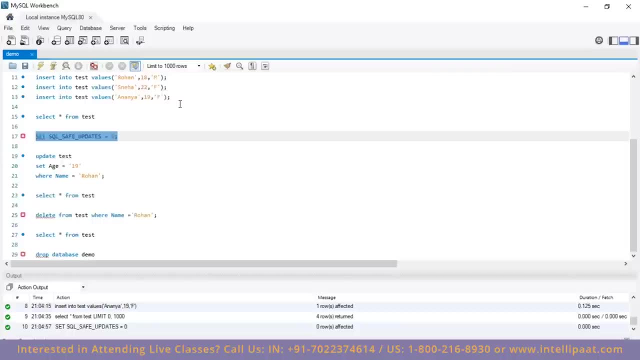 let me bring this down a little. yeah, perfect, so, uh, then, this command is particularly for mysql workbench, where we have something called as a safe mode and we, uh, you know, take away the safe mode to work with the data without having to worry too much about keys, guys. so this is: 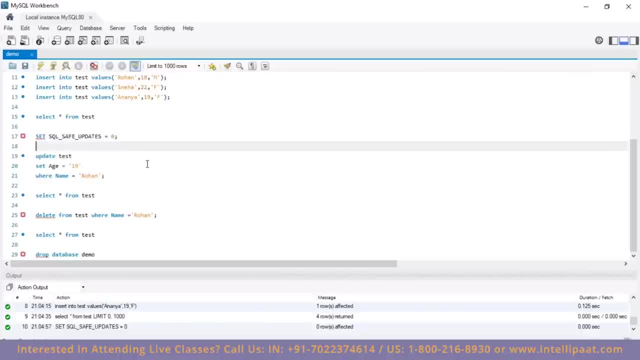 something that you might not have to use all the time, and i just quickly run it to make sure i do not get any uh warnings or errors up front guys. so the next command is: uh, so we've created uh, since we're doing the crud demo, so we're done with the c part, where you've 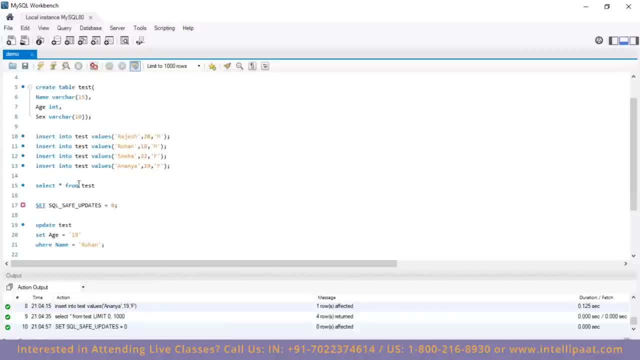 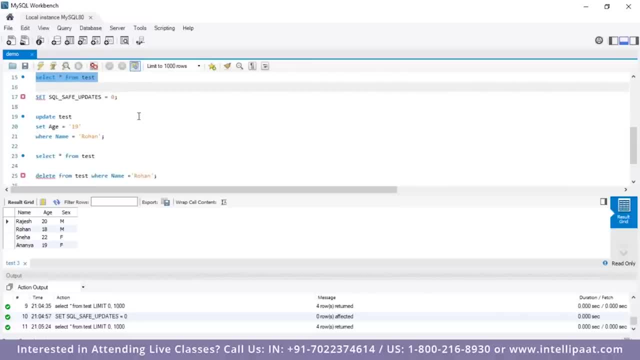 u and d. where u is for update, d is for delete, right, so now we're going to update some entry in this table. it's not as easy as double clicking and editing guys, so you need to put in queries and that's why we call it a structured query language and then, as you guys can see, it is extremely. 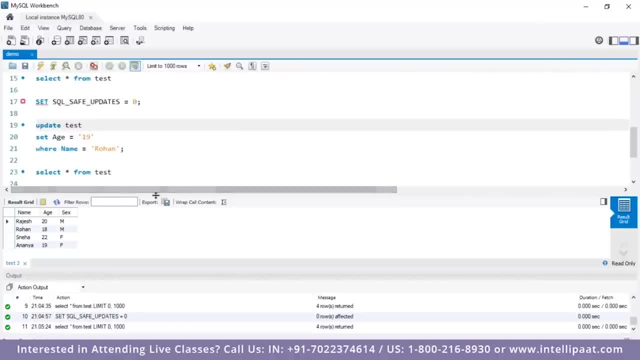 simple, so let me quickly zoom in a little, in case, uh, you guys are watching this on your mobile or something. so, uh, here is the query for updating it. so update the table name. so up it's basically: test is our table name, if you can see here, right? so test is our table name. this is the creation. 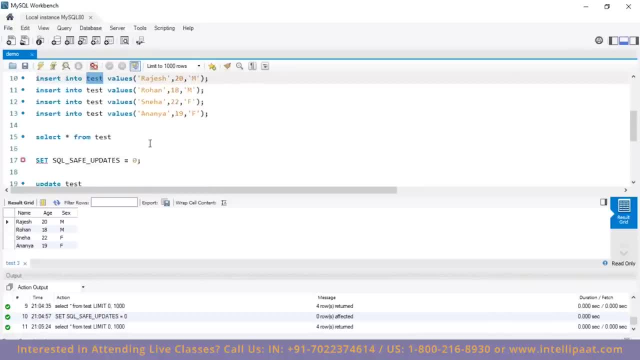 command test again, where we are inserting the data to which we're already done with. we're printing all of the things that we've already done and now we're going to update this particular table and we're going to set age equal to 19.. okay, but whose age are we going to? 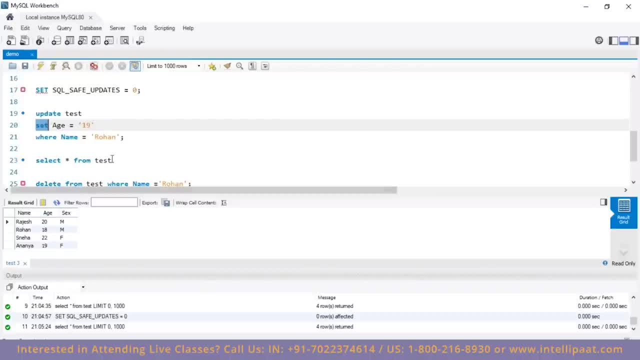 set to be 19, right? so there are four people right now. we need to tell our database who is age i want to change to 19.. uh, so basically that is where the where class comes into case. so the where class says hey, uh, hey, database, update my date. uh, you know, update my table. set age equal. 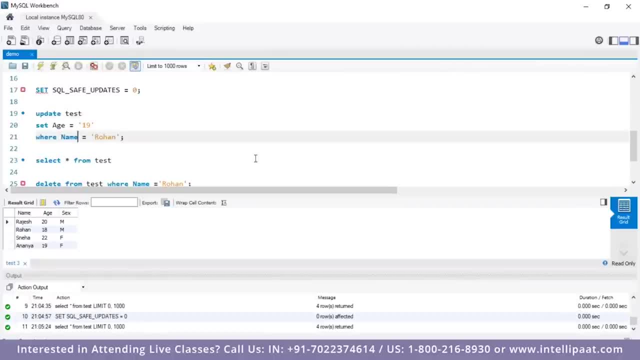 to 19, where name equal to rohan. so just find this person called rohan under the uh, under the name column and change his particular age, whatever it is, to 19.. so rohan, as you can see in this particular mouse highlight that i have done for you guys, currently is 18 years old. so let's say manually: 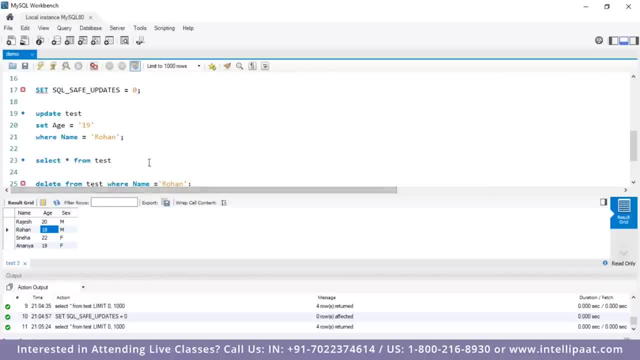 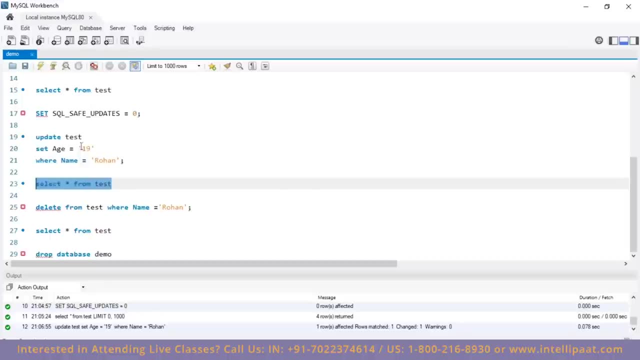 change ages at the end of the year or for his birthday or whatnot. so as soon as i go ahead and run this command, rohan will not be 18 years anymore. rohan will be 19 years old. so let me use the select star from test to print the database out and, as you can see, right. so rohan is not 18, he's 19.. so 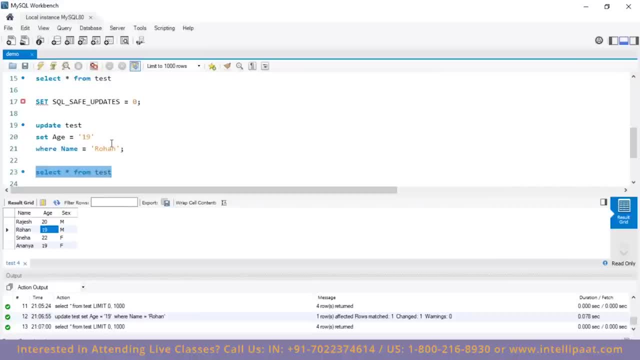 you can change all as well. so you you can change rohan's name uh, you can change uh his sex if you want, and you can have a lot more. this is a very simple database. example, guys. you can have a lot thousands of entries where you can run complex queries once you are trained to work with sql. as 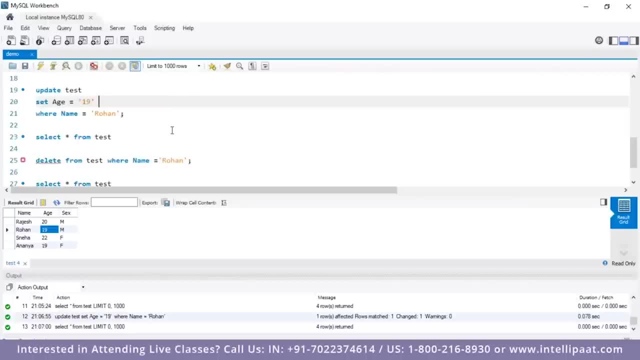 well, guys. so again, as i've said, uh, pretty much, my intention here is to just show you the basics and make you guys uh clear with the fundamentals of the crud operations. so now we have updated rohan's age. rohan is not 18 anymore, rohan is 19.. uh, and pretty much, uh, this brings us to the d operation. 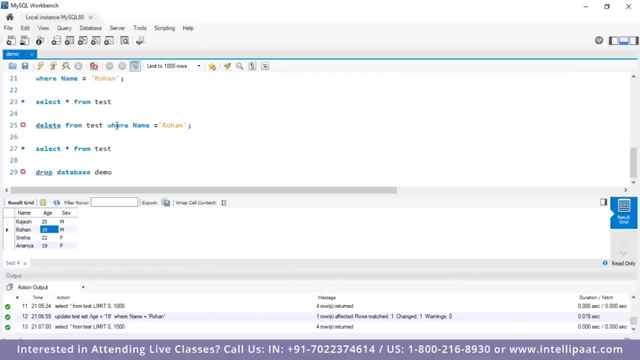 which is the delete operation again. so let's say: uh, you know, probably rohan, just uh, uh, you know, cleared out of college and they decided to drop his name from the database and they do not want his name anymore. so delete from the table name or table name is test, where name equal to ron. so 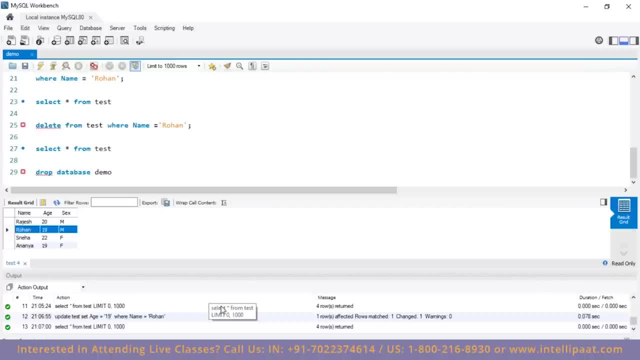 basically it's. i am telling you to wipe this so as you can see the mouse highlight and the blue color. i'm just telling my database. you know what. i don't want rohan or any particular uh thing associated with rohan anymore. so as soon as i run this command, uh, you can pretty much see uh, that uh. 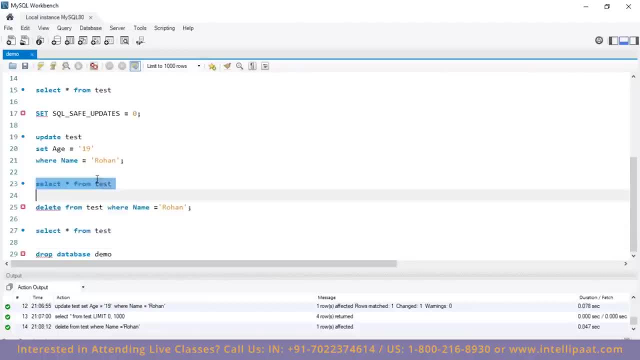 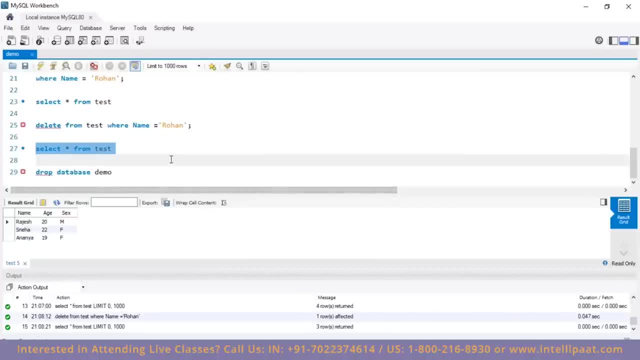 every time you run the command you have to view it right. so again, as you can see, i have a lot of tests everywhere present. so as soon as i run this, as you can see, rohan is not there anymore. we just have rajesh, sneha and ananya guys. so this, pretty much, is the most simple way you can go on to. 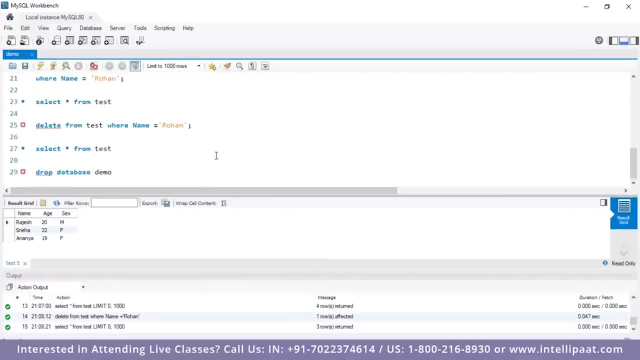 performing uh crud operations, in my particular opinion, guys. but then if you have to reuse the same thing, you will come up with one particular error case, which i'll just show you right now. so we are this. this is a server architecture, right? so our database, which is called demo, and our table. 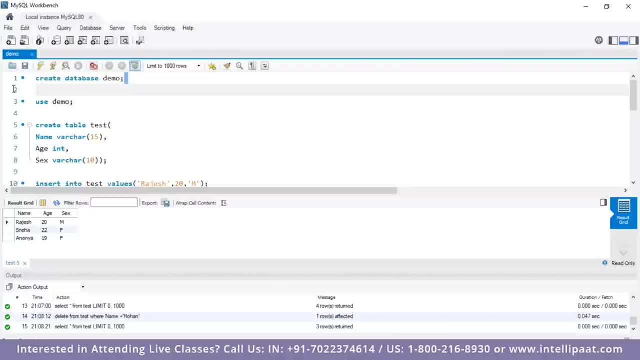 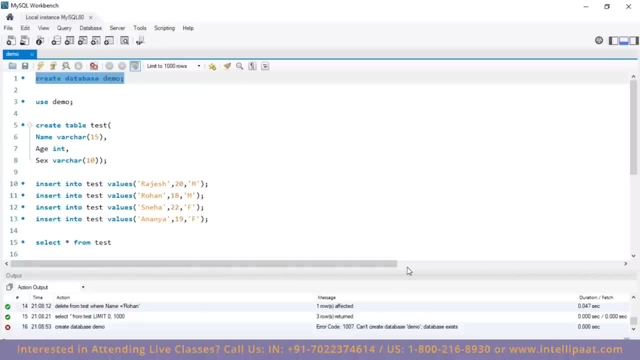 test inside this demo is already present. so if i go ahead and just run this query again to see what happens, it's going to give me an error. it says, hey, i cannot create another database with the name demo because something called as demo already exists. so you're gonna have to, you know. 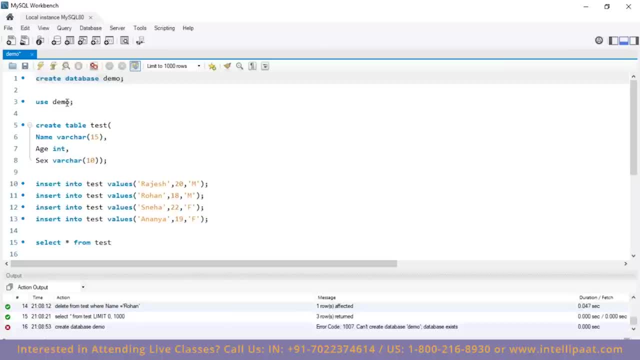 change this to demo one. demo one or two, whatever you're gonna have to get into that database. demo one or two, and then you can use the same table name, because you're using a different database. now, guys. so it's as simple as that. so, and after you have done everything, if you want to delete an, 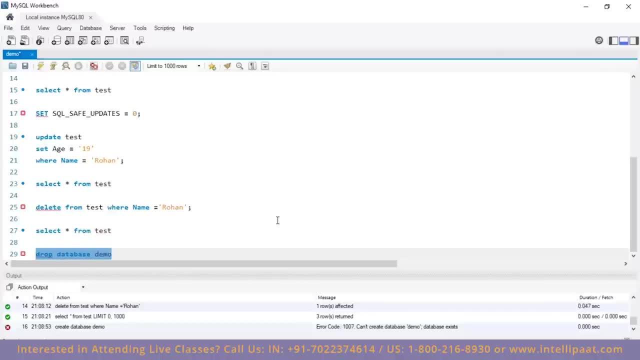 uh. you know a database can have n number of tables. so if you choose to delete all of them, you can pretty much hit drop uh database and followed by the database name and done. it says one row affected. your database has been dropped. so whatever we have done until line 26 from now, pretty much is deleted. 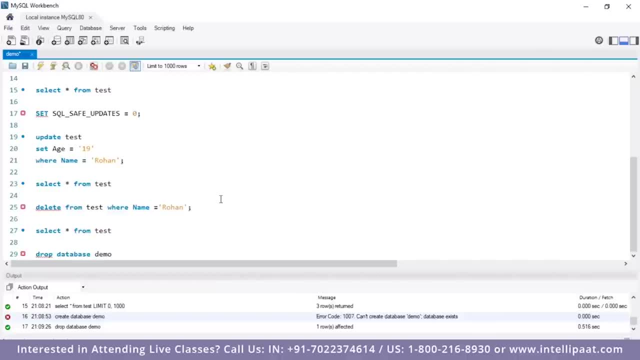 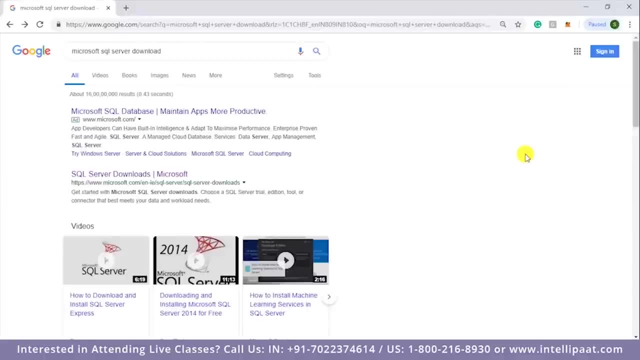 guys, you know it is as simple as this and you can understand the query because it is in such a high uh level syntax that it makes it very simple for beginners to learn. guys, we'll be installing the database as a demo, so now let's go to the database to see if we can use it. so the first: 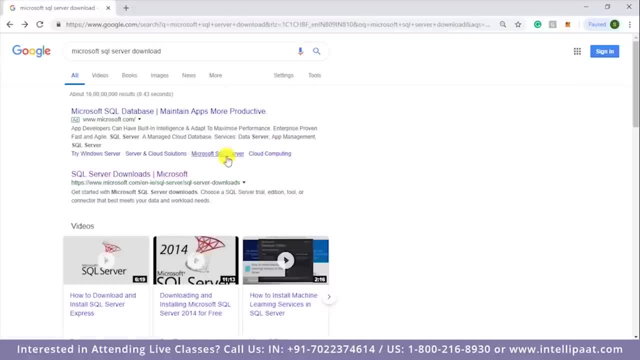 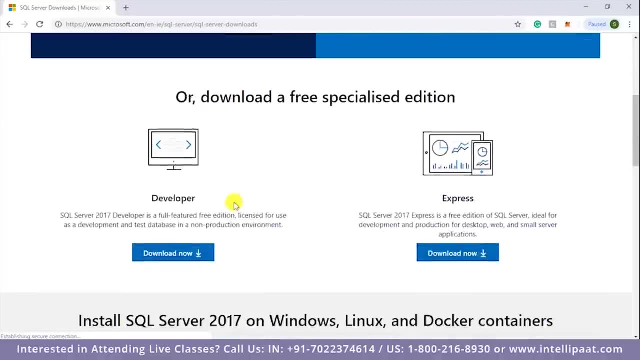 thing you're going to see is the database you had created, just like the previous below data. so i'm going to download an empty database, just like that, and then i'm going to go ahead and create just one more database and i'm going to add a new database and i'll choose a new one. 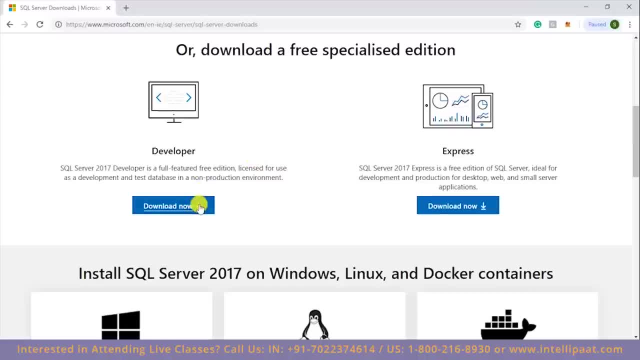 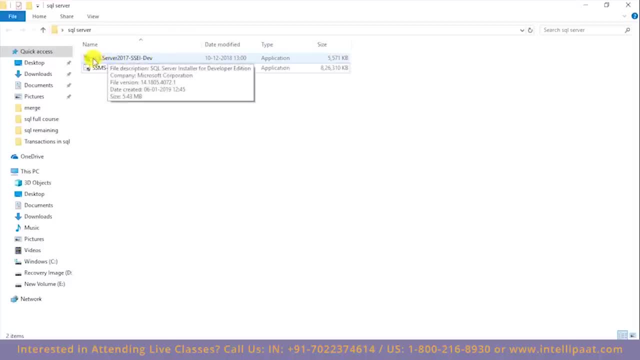 so in this case it is mp4, and i'm going to click on download and if you click on download you're able to see the number of downloads that's already created, and you can see on this page a lot of software and things like that. so it's working perfectly fine. i'm going to go ahead and start by. 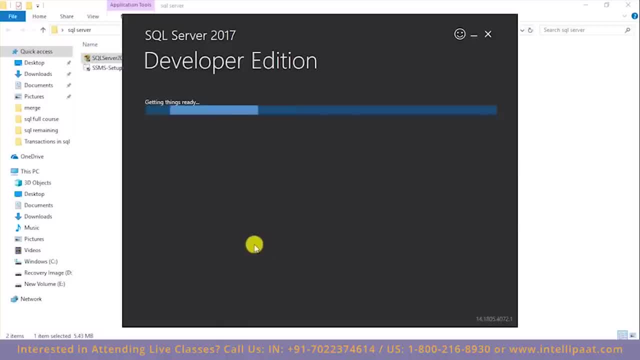 server 2017, SSEI development. so we get this window over here and we have three options: basic, custom and download media. so I'll click on custom. now we see that we have a media location where the sequel server will be downloaded and I will click on install. 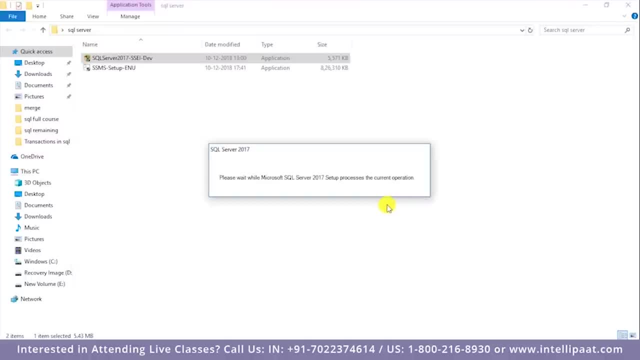 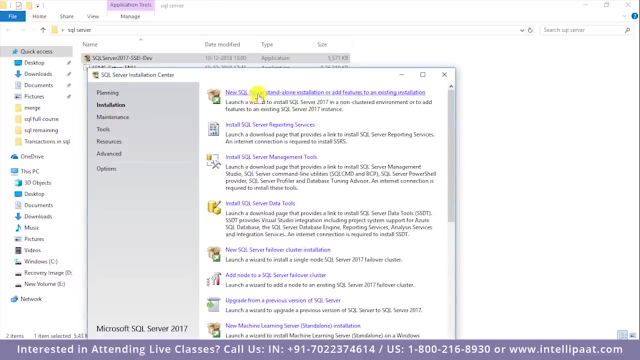 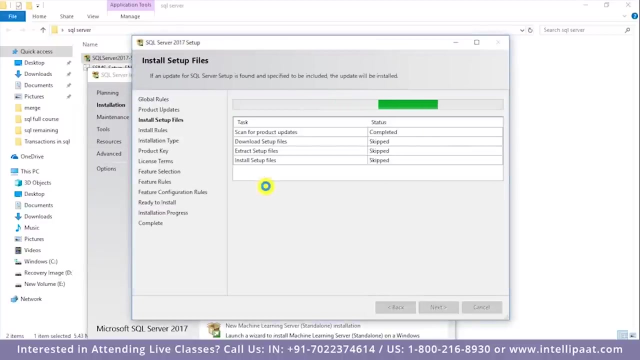 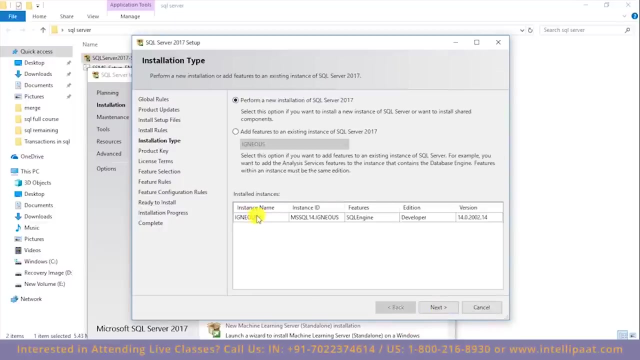 you see that the download is successful and our installation will begin shortly. you here, I'll click on installation and I'll select this one, so I'll be installing standalone installation of the sequel. so so let us wait for this to open. right, so hear I click on next. now I only have one instance of SQL. 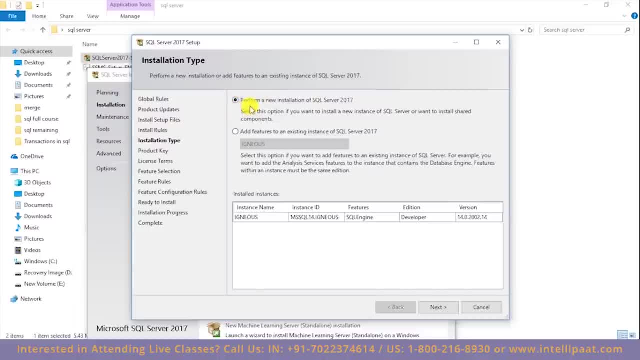 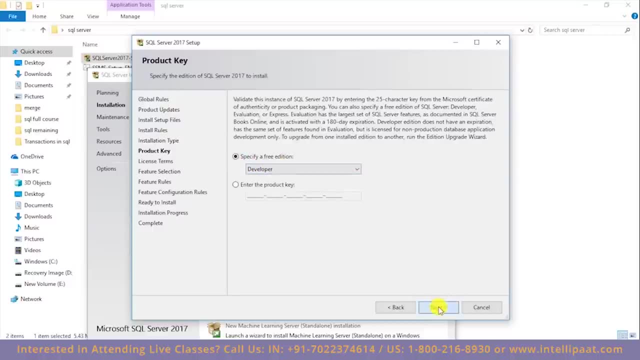 so. so I'll be installing a new one, so I'll uh uh uh, Select this: perform a new installation of SQL Server 2017, and then I'll select this free edition. I'll click on next. after that, I'll accept this license agreement and again, I'll click. 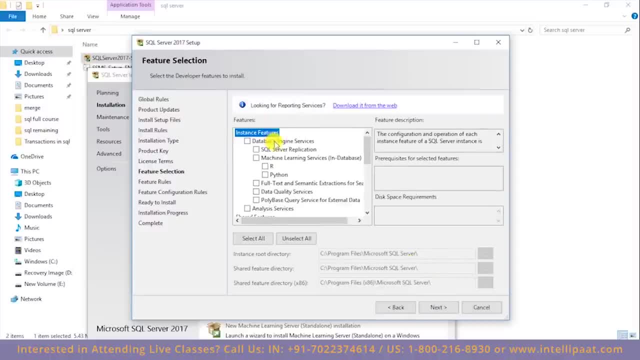 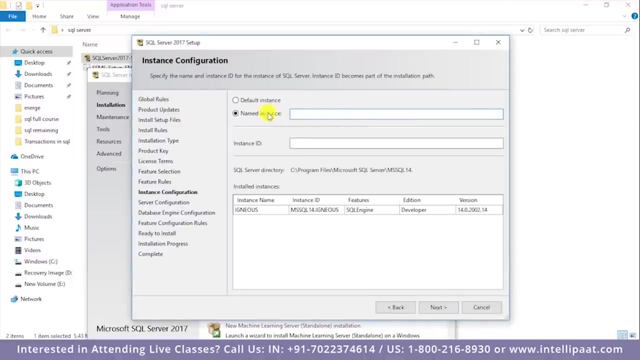 on next. So we have all of these features over here. So I would just need the database engine services. So I'll select this and again, I'll click on next. So I'd have to name the instance for the server which I'm installing. 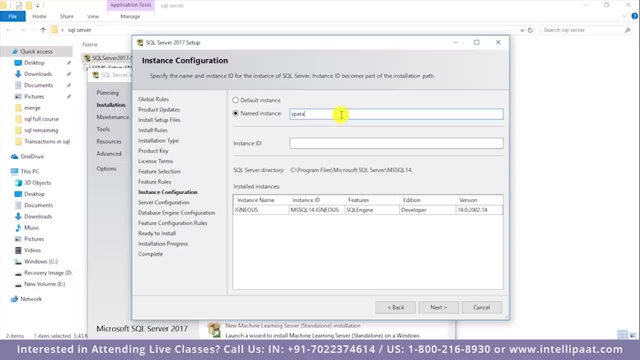 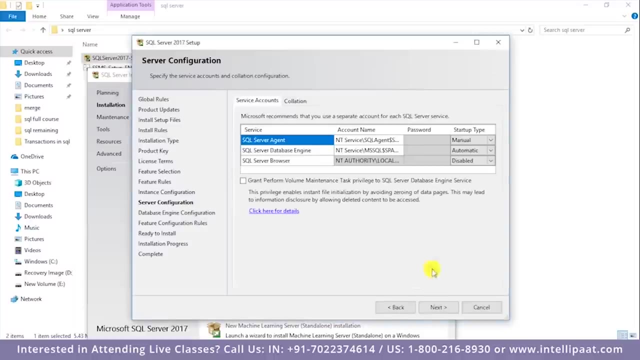 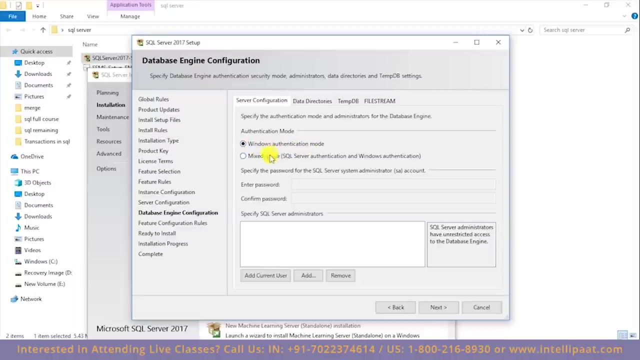 So I'll name this server as, let's say, Sparta. Similarly, I'll give the same instance ID over here. I'll click on next. So again, I'll click on next over here. So we see that we have two authentication modes: Windows authentication mode and mixed. 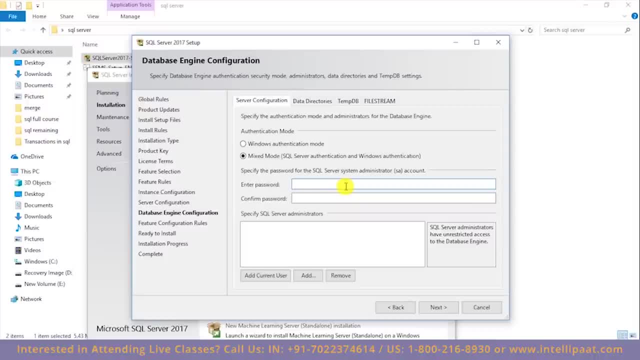 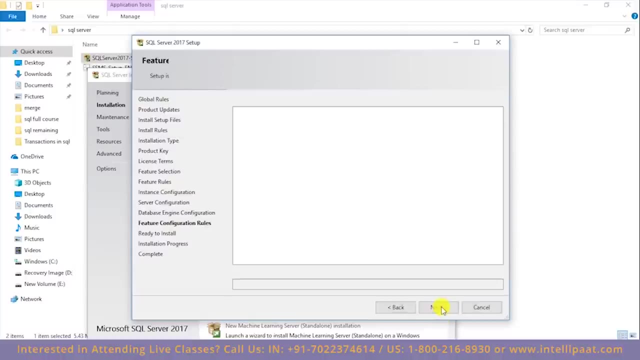 mode. So I'll select the mixed mode and then enter the desired password. Let me put in my password over here. I'll add the current user. so the current user has been added. Now I'll click on next again. Right, so we are finally ready to install SQL Server. 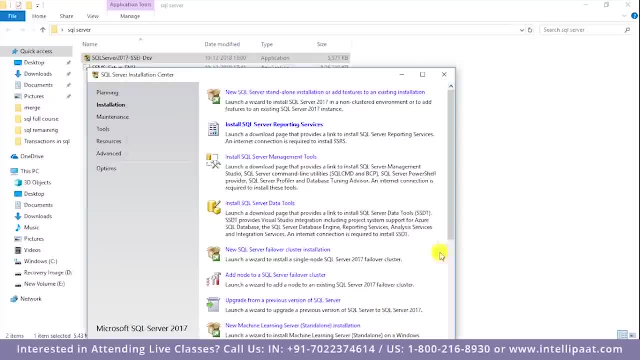 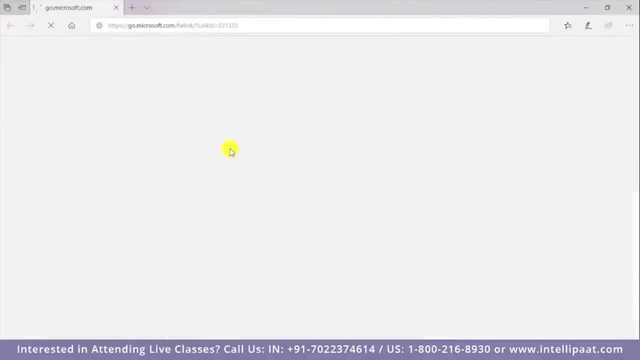 I'll click on install Right. so once the installation is done, I would also have to install the SQL Server. So the SQL Server management tools basically help us to connect with the database. I'll click on this and this will redirect us to the Microsoft web page and over here. I'd have to download the SQL Server management studio, and I'll be downloading the latest version And this is the downloaded file over here: SSMS setup enu. I'll click on this. So here we have these three options: repair, uninstall and close. 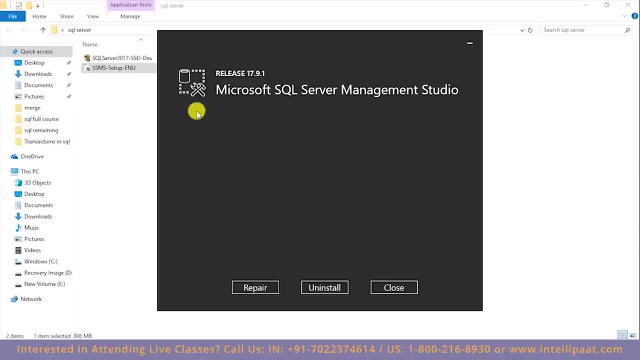 Now I have to install this, these three options, because I've already installed Microsoft SQL Server Management Studio in my system and if you are installing this for the first time, you will have the install button over here, so you would have to click on install and the install would be done automatically, right? so once you install, 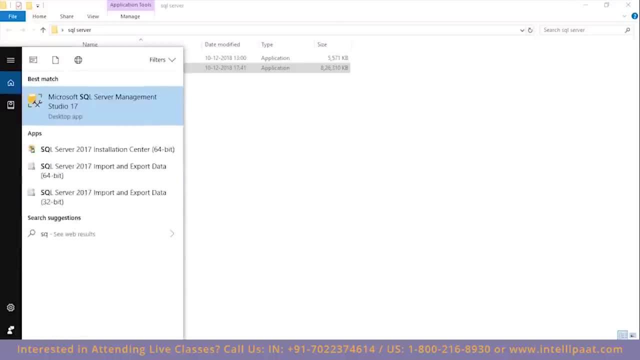 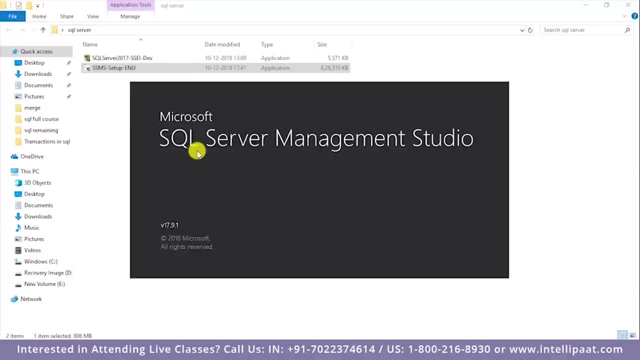 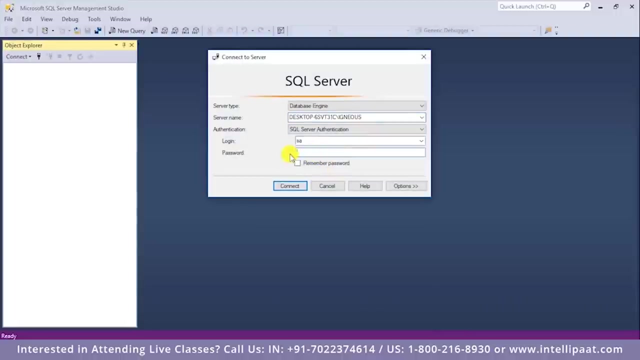 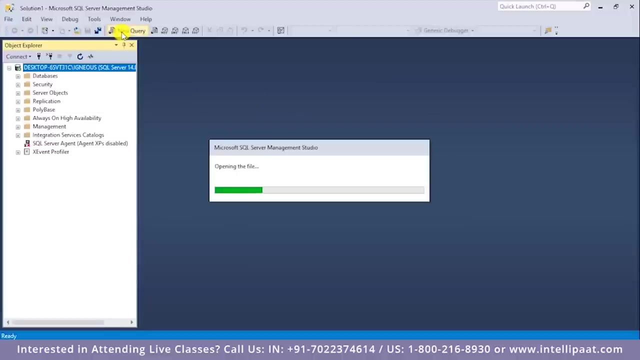 the SQL Server Management tools. go to the search tool and type Microsoft SQL Server Management Studio. click on this and Microsoft SQL Server Management Studio will start. so, over here, you would have to specify the password which you gave while creating the instance and then click on connect. and to start writing your SQL commands, click on new query over here. 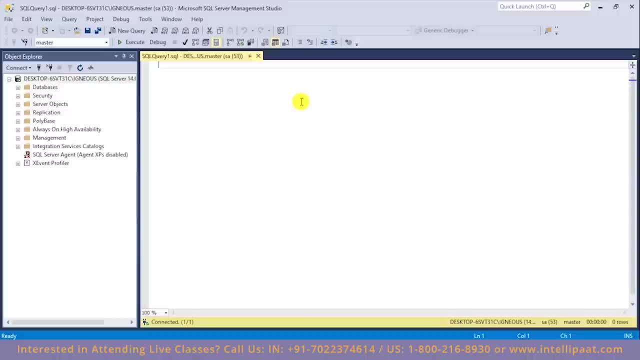 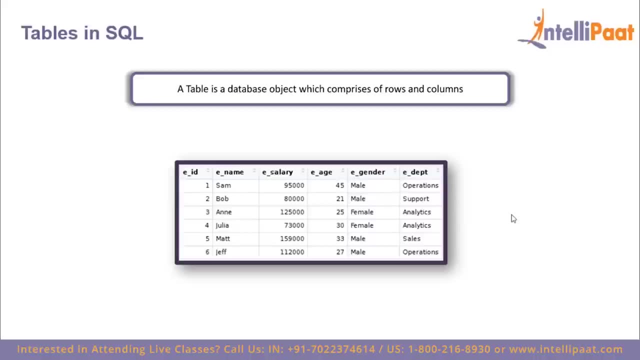 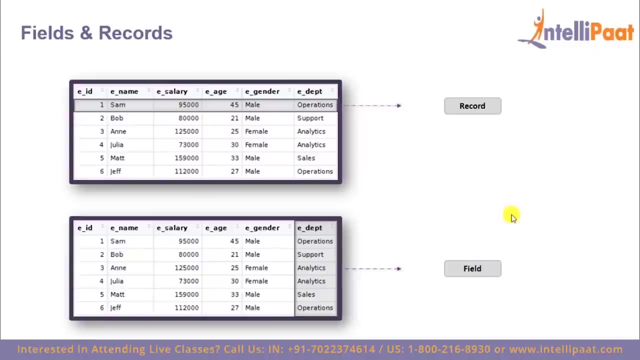 and then you can happily implement all of your SQL commands. right? so this was the installation of Microsoft SQL Server tables in SQL. so simply put, a table is a database object which comprises of rows and columns, and in SQL, the rows are known as records and the columns are known as fields, so the fields are basically columns, which 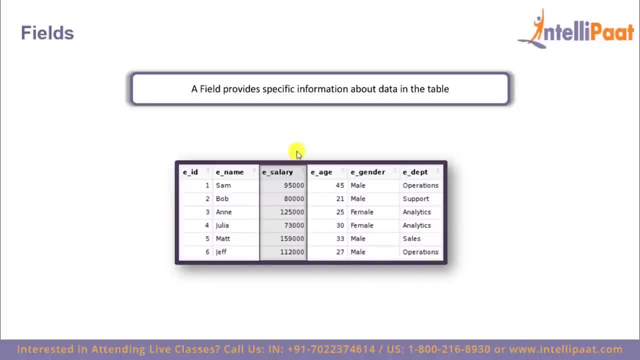 provide specific information about data in the table. for example, we have this esalary field in the table which provides information about the salary of different employees. similarly, we have this eh field which provides information about the age of different employees and a record as basically each individual entry that. 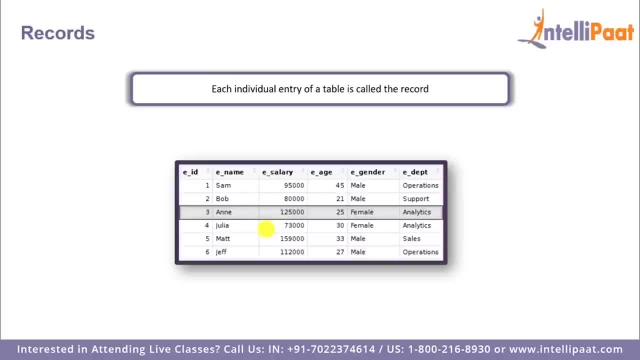 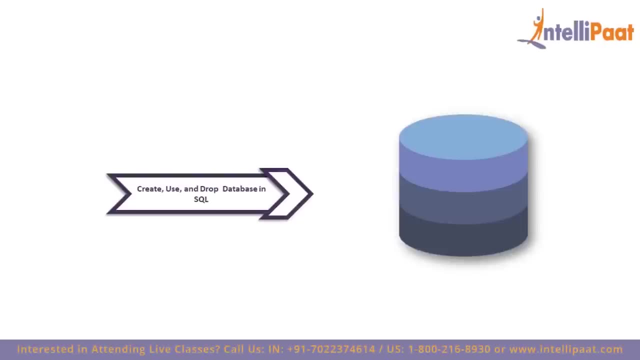 exists in the table. so record gives you complete information of one single entity. for example, if we take this record over here, this will give us complete information of this particular employee. so this was all about tables, how to create, use and drop a database. so this is the. 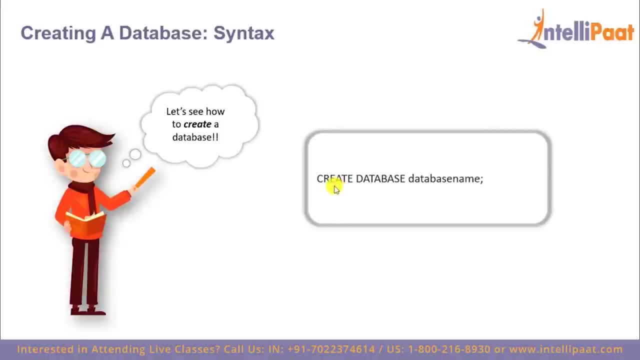 syntax to create a database in SQL. we will, given the keywords, create data table, table form and data sample table type, data data per, say, een, and then give the name of the database which you want to create. So let's go ahead and create a database in SQL. So let's create a first database, guys. So I 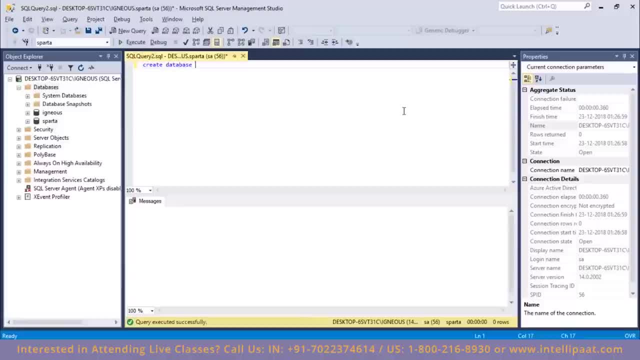 will give in the keywords create database, and let's say I want to name the database as happy, right? So I'll put a semicolon over here. I'll hit execute So see that commands have been completed successfully. Now let me hit refresh over. 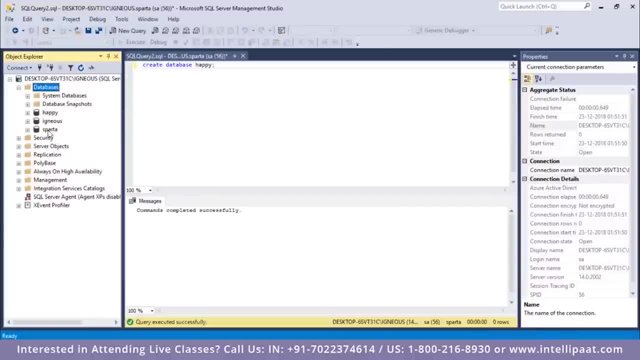 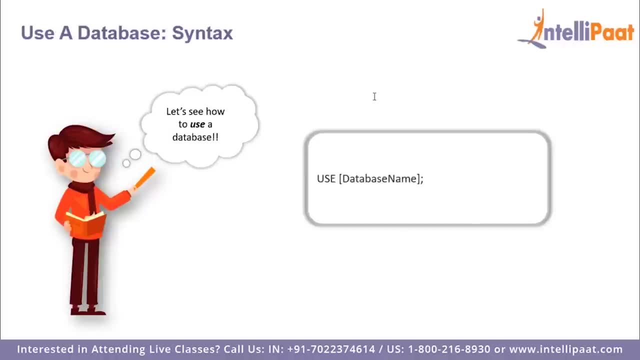 here. So initially we just had two databases: igneous and Sparta. After implementing this command, create database happy. we have successfully created a new database, happy. Now, after we have created a database, we need to know how to select a database from our existing list of databases. So we have. 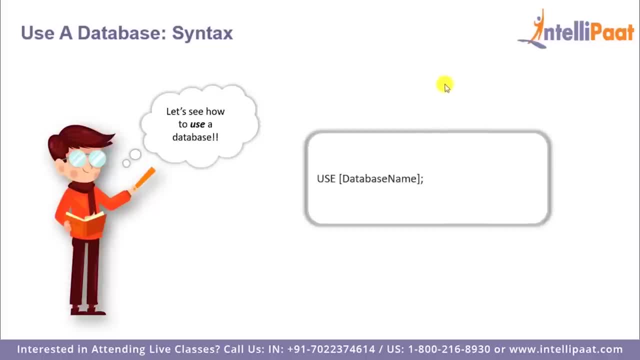 the use database statement. for this, All we have to do is give the keyword use and then state the name of the database. Now, this database which you selected remains default until the end of the session or execution of another use statement with some other database. So if 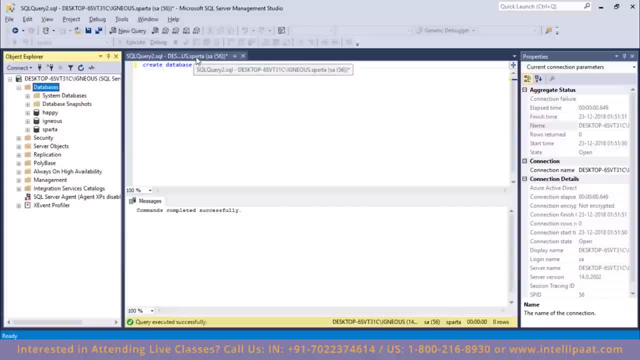 I put my mouse pointer over here So you see that currently we are using the Sparta database. So now I want to use the happy database instead of the Sparta database. So I will write the command for that use and then after that I need to. 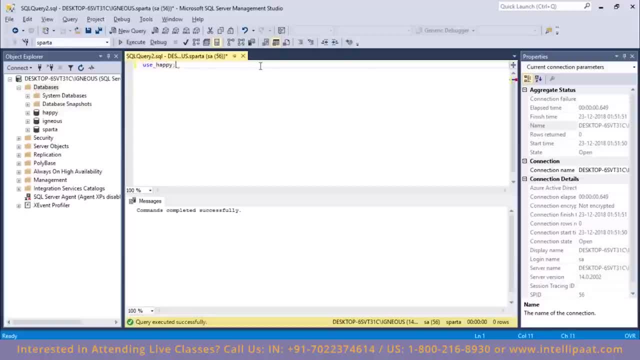 give in the database, which would be happy. I'll put a semicolon, I'll hit execute. So again, commands have been completed successfully. So now we see that the database has changed. So let's go ahead and create a new database. So 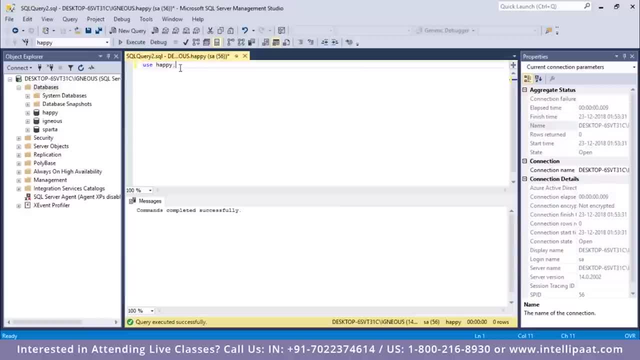 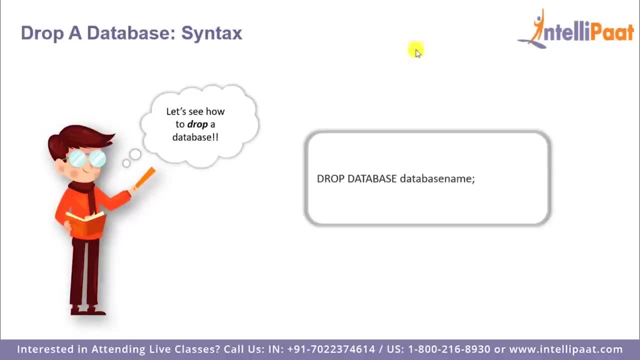 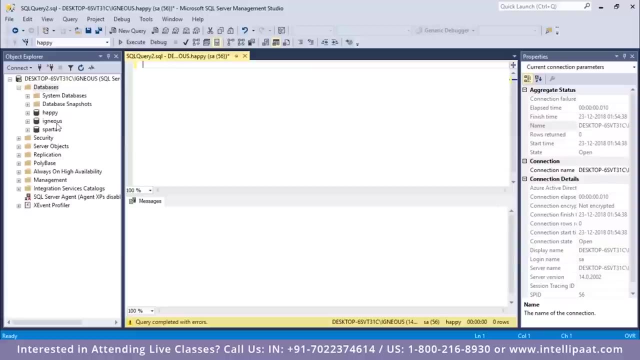 we have changed from Sparta to happy, So currently we are inside the happy database. Now we'll see how to delete a database, or in other words how to drop a database. So we have to give in the keywords drop database and then specify the name of the database which you want to drop. So now I do want to drop this. 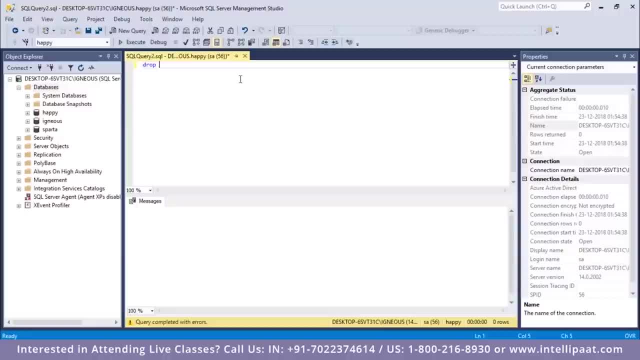 igneous database. So let me write the command for that Drop database, and then the name of the database is igneous, So I'll put a semicolon over here as a hit execute. so again, commands have been completed successfully. now I'll hit refresh. so we have only two databases: happy and Sparta. so database igneous has. 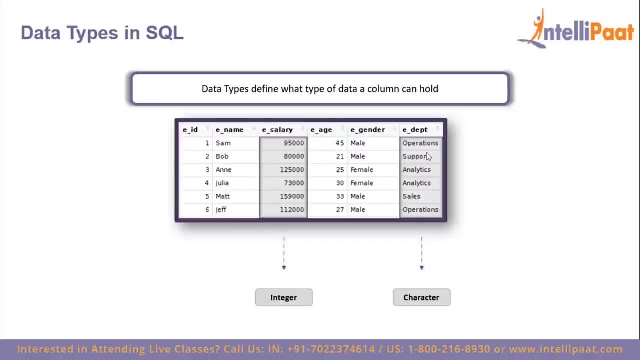 been dropped data types in SQL, so our data type basically defines the kind of data that I'll go into a particular column now. it needs to be kept in mind that all the entries of one particular column but are the same data type. so well, let's take this e salary column, for example. we see that the first entry is: 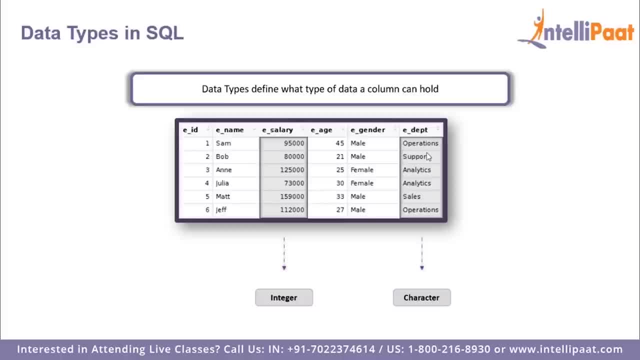 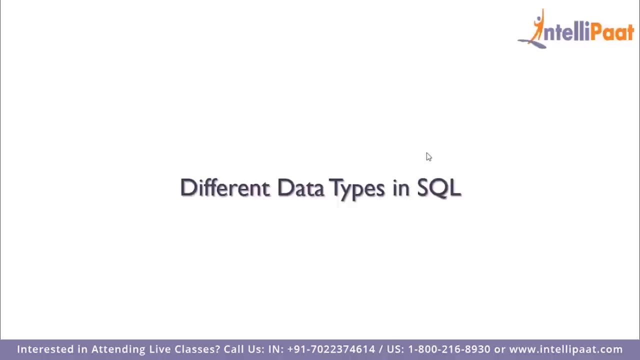 of integer type. the second entry is also of integer type. similarly, all the entries of this e salary column are of integer type. now let's take this department column. here we see that all the entries of this particular column are of character type. now that we've understood what exactly are data types. 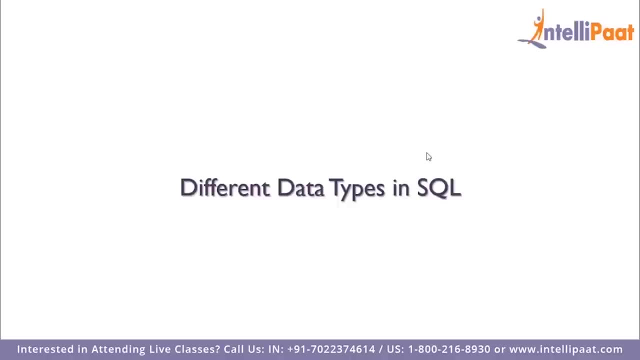 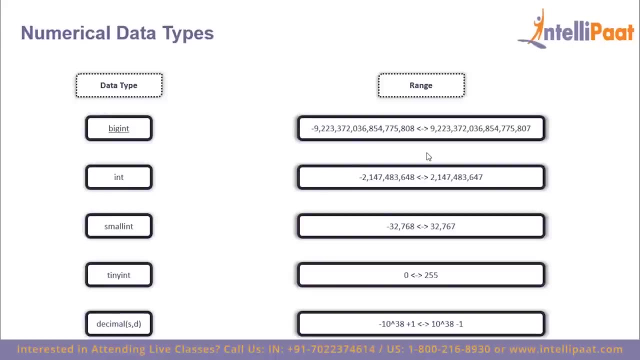 let's have a look at the different data types available in SQL. let's start with the numerical data types. so we have the big in data type, which helps us to store really, really big values. you so you can see the range of big int over here. then we have the int data type. 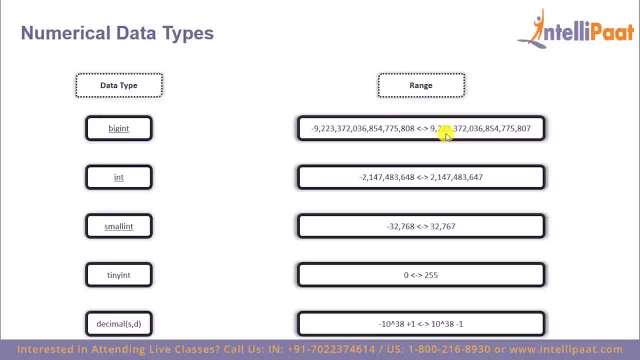 which helps us to store reasonably big values. after that we have the small int data type, and the range of small int is from minus 32,768 to 32,767. then there's tiny int, and the range is only between 0 to 255. after that we have 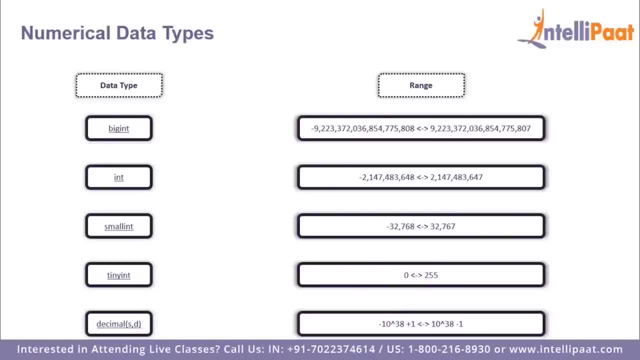 the decimal data type and it is used to store fractional values. so the decimal data type takes in two arguments. first is the size of the value, that is, the total number of digits. then we need to specify the number of digits after the decimal point. let's say we want to store the decimal value 12.50 here the size. 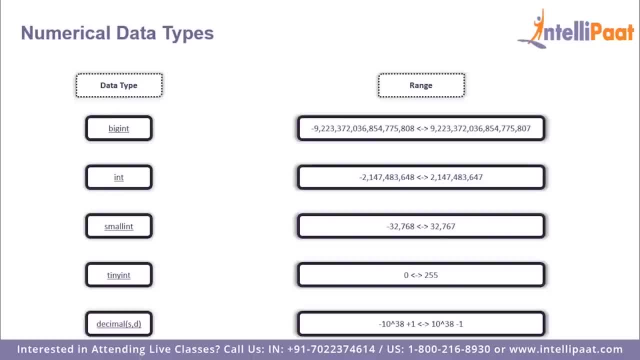 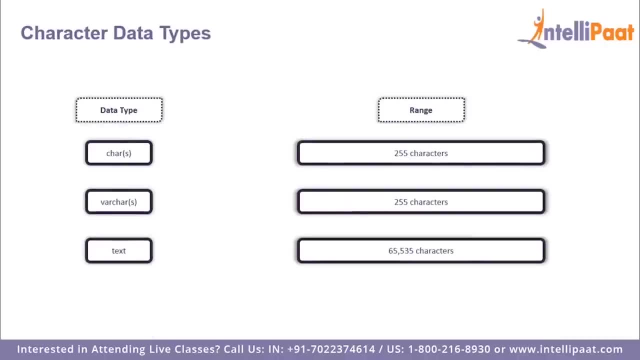 would be 4 because the total number of digits are 4, and value of d would be 2 because there are two digits after the decimal point. now let's have a look at the character data types. so first we have the char data type. this takes in one argument. 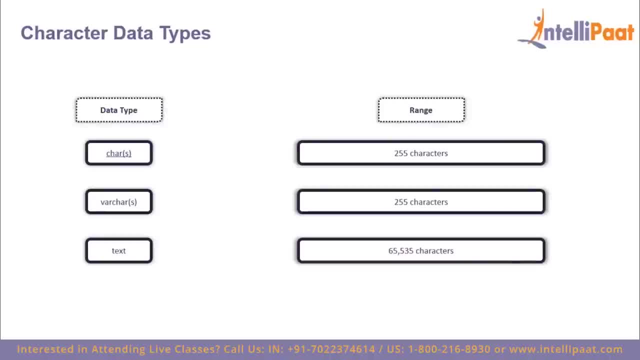 which is the size of the value. let's say you set the size to be 20. this would mean you cannot give in a value which would have more than 20 characters. now you need to keep in mind that char is a fixed length data type, that is, if you 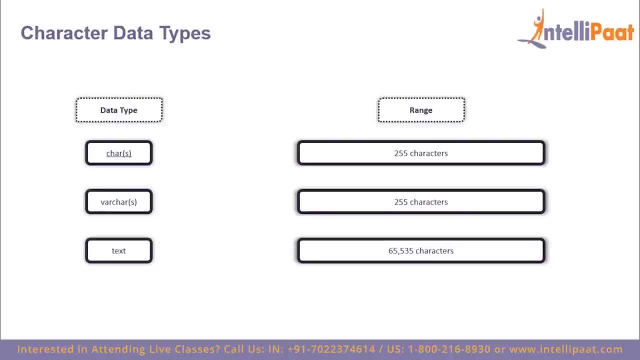 set the size to be 30, but you give it only three characters, then the memory which would be consumed is of 30 characters. so you are basically wasting the memory over here. then we have the var char data type. this again takes in size as the argument. now, var char is a variable length data type, unlike char. so here, if 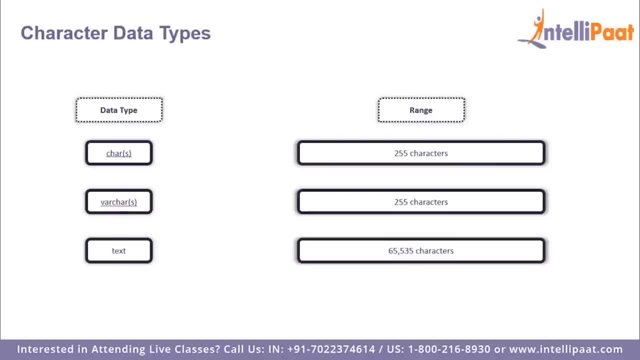 you set the size to be 30 and given only three characters, the memory consumed would be only 3. then we have the text data type, so this data type can take in a string with a maximum length of 65,535 characters. then we have the 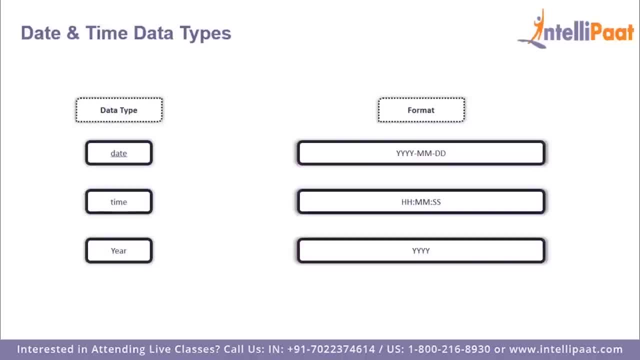 date and time data types. well, start with the date data type. so this data type helps us to specify the date in this format over here. let's say we want to store the date 2nd January 2019, then first we will give in the year, which would be 2019, then we'll specify. 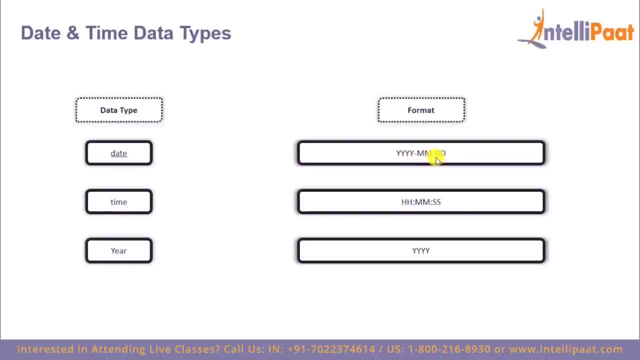 the month, which would be 01, and finally we'll specify the day, which is 02. after that we have the time data type and this helps us to specify the time represented in the format over here. now let's say, I want to store the time 830. 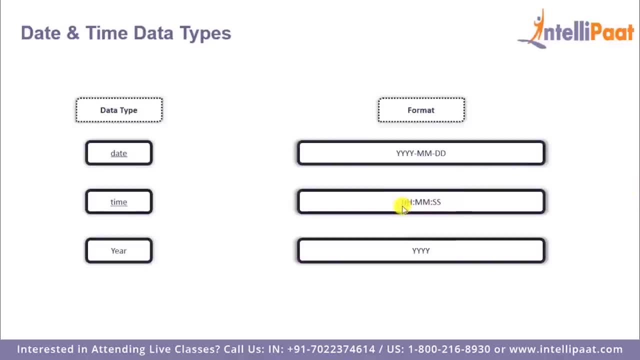 am 23 seconds. so first I will specify the hour, which would be 08, then I'll specify the minutes, which is 30, and finally specify the seconds, which would be 23. then we have the year data type, which just holds the year value, such as 1995 or 2011. so constraints are basically used to. 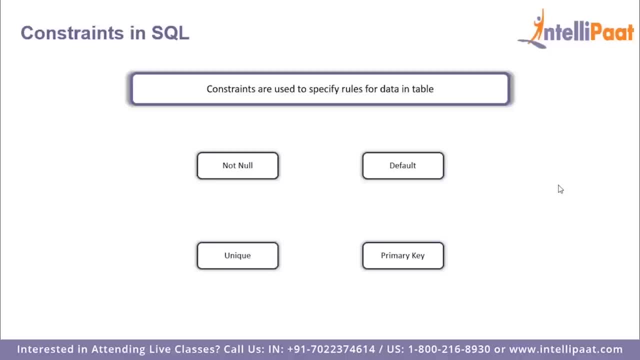 specify some rules on the data and limit the type of data that can go into a table. we will look at these four constraints: not nil, default, unique and primary key. let's start with the not nil constraint. let's start with the not nil constraint. let's start with the not nil. 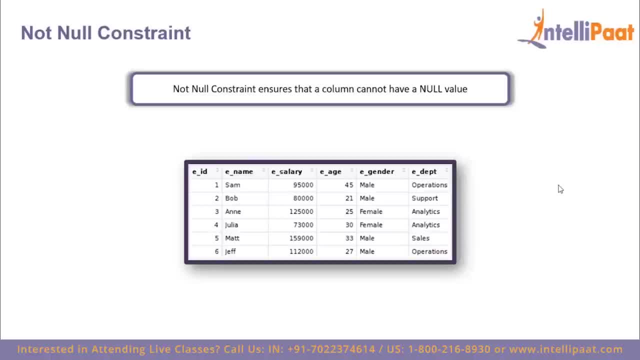 constraint. so by default, a column can hold null values and with the help of the not nil constraint we can ensure that a column does not have null values. so the not nil constraint basically ensures that a field always contains a value. for example, if we assign the not nil constraint to this e salary column. 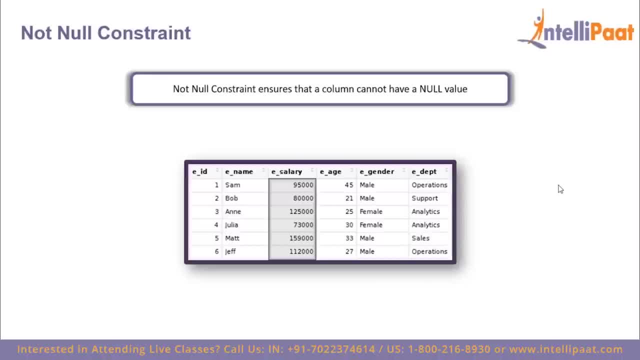 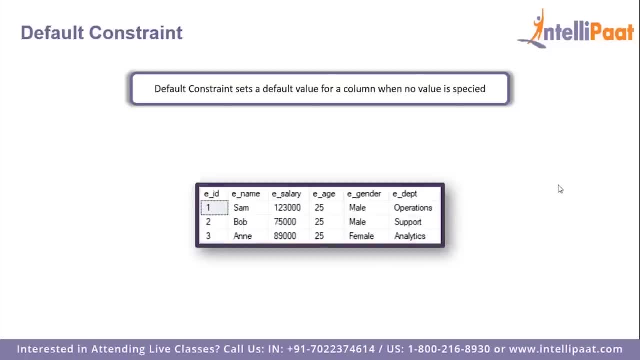 over here, then every single entry of this column should have a value. then we have the default constraint. so the default constraint is used to provide a default value for a column. so the default value will be added to all the new records if no other value is specified. for example, if we assign the 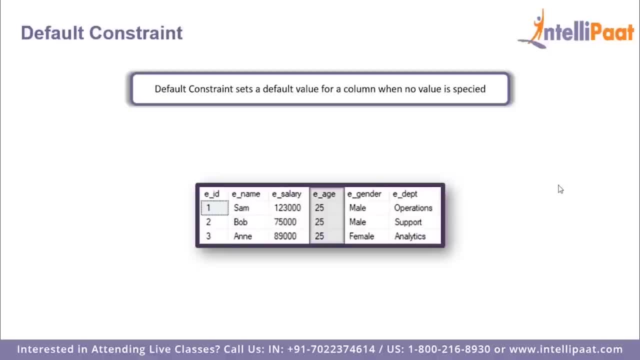 default constraint to the e each column and set a default value of 25, then all the entries of this column will have the default value of 25. if no other value is specified during insertion, then we have the unique constraint which ensures that all the values in a column are different. 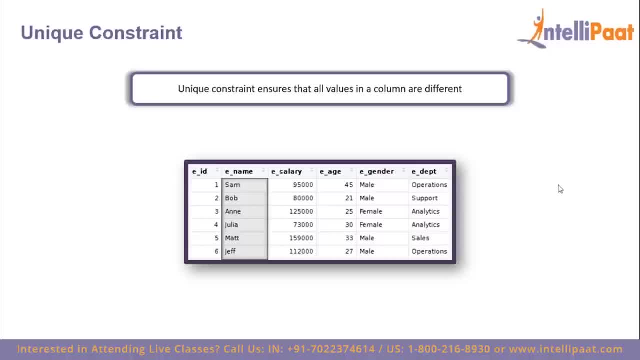 for example, if we assign the unique constraint for this column, then every entry of this column should have a unique value. And finally we have the primary key constraint. So the primary key constraint uniquely identifies each record in a table. or, simply put, it is just a combination of 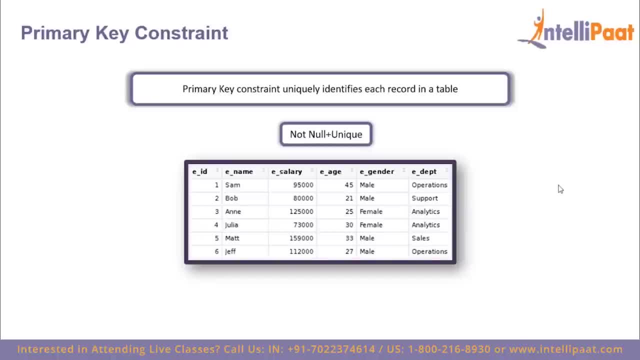 the not null constraint and the unique constraint. So when we assign the primary key constraint to a column, then that column shouldn't have any null values and all the entries should also be unique. For example, if we assign the primary key constraint to the employee ID column, then there should be no null. 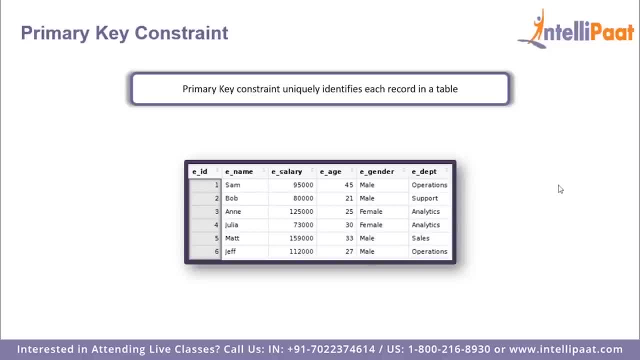 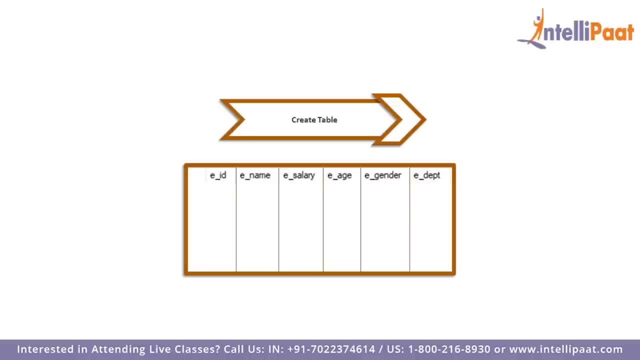 values in this column and all the entries should also be unique. How to create a table in SQL. So we'll be creating an employee table which would comprise of employee ID, employee name, the employee's salary, age and gender and the department in which the employee works. So let's have a look at the steps to. 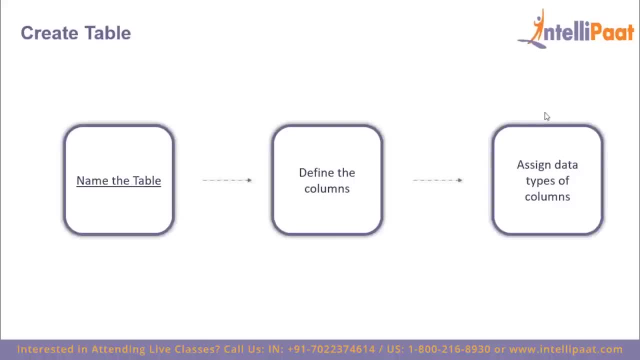 create a table in SQL. So first we have to start off by giving a name to the table. After that we have to create a table in SQL. After naming the table, we'd have to define the columns which would be a part of a table and finally, we'd have to assign a data type to each of the column which we 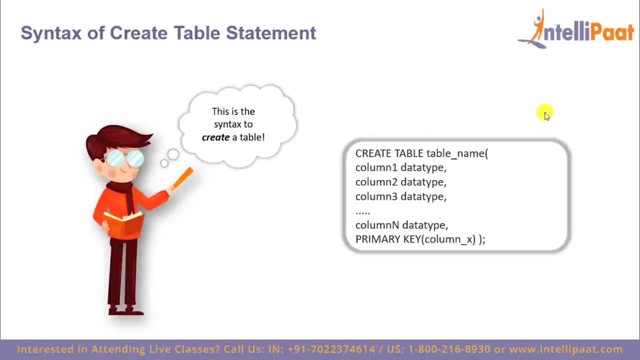 have defined. Now let's have a look at the create table syntax. So first we'd have to specify the two keywords, which are create, table, and then we'll give a space and then give a name to the table and inside the parenthesis, we will define all of our columns and assign them their respective data types. Now 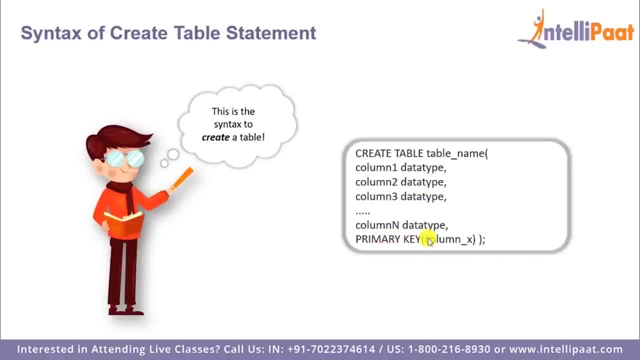 finally, if you want to give a primary key constraint, we can do it over here. So we will give in the keywords primary key and then give in the name of the column, which would be a primary key. So, as we have already learned in a previous 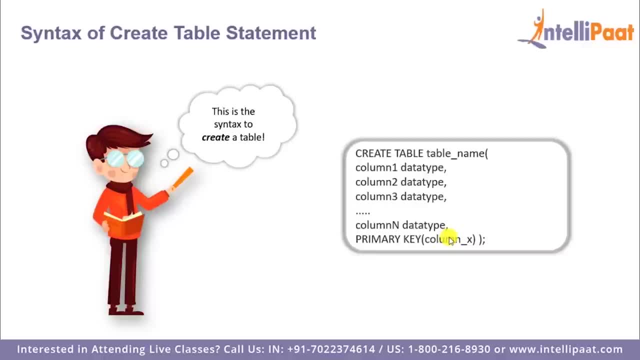 session. a primary key basically helps us to uniquely identify all of the records in our table, and guys also keep this in mind. A table cannot have more than one primary key. So now that you understand the syntax of create table command, let's go to MS SQL Server and create our employee table, Right? so this is MS SQL Server. 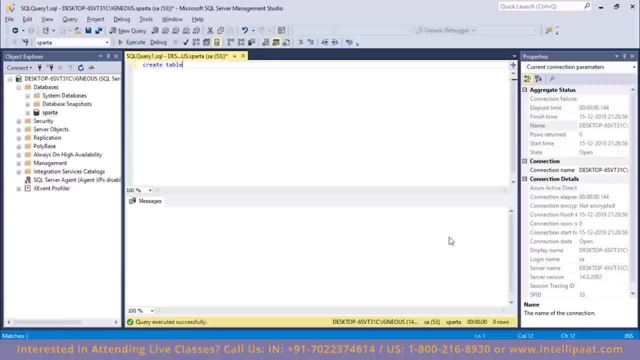 So I'll start with the command. I will give in the keywords create table, Then I will give in the name of the table, which would be employee, And inside the parenthesis I will give all of the columns. So the first column would be employee ID. So I will type E ID. 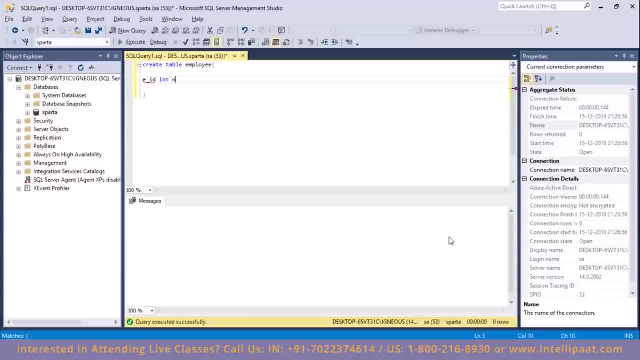 which is the name of the first column, And this is of type integer. So after this I will also put in the not null constraint. So this not null constraint means that all of the cells in this column should definitely have a value, And then I will give in the second column. So the second column is employee name. 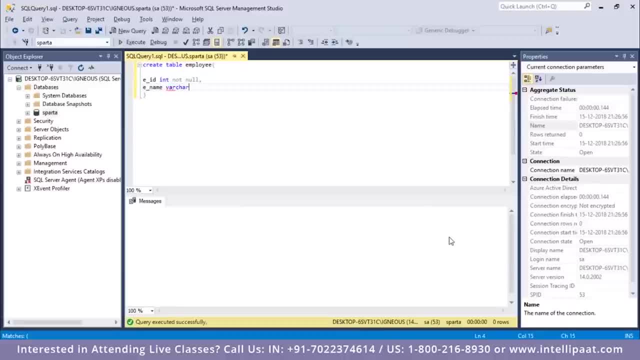 So E name, and this is of type varchar. So varchar stands for variable length character, and the maximum length would be 20.. Then I'll give in the third column. So the third column would be employee salary. So I will name the column to be E salary. 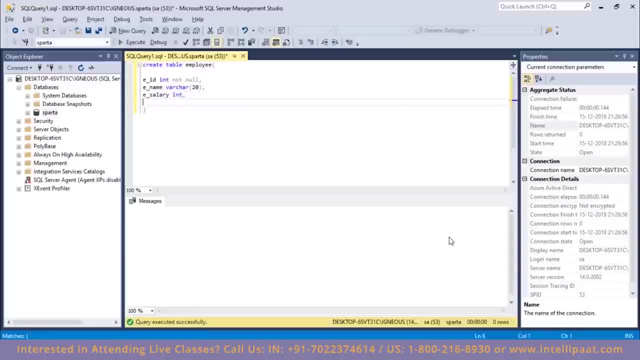 And this would be of type integer again. After this we have the employees age, So the column name would be E age And this is of type integer two. Then we have the employee's gender, So I will name the column to be E gender. 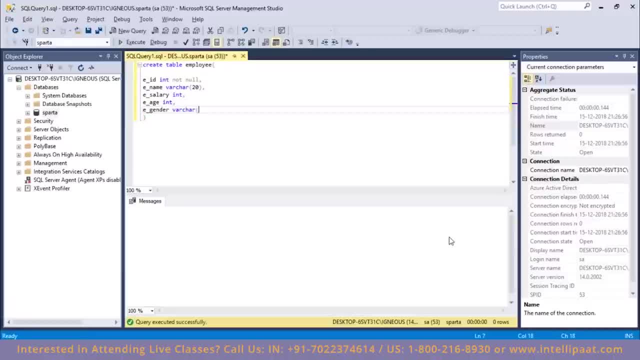 And this would be of type varchar. So this is of variable length character and the maximum length is 20.. And then we will give in the final column. So the final column would be the department in which the employee works. So let me name it to be E, D, E, E, T. 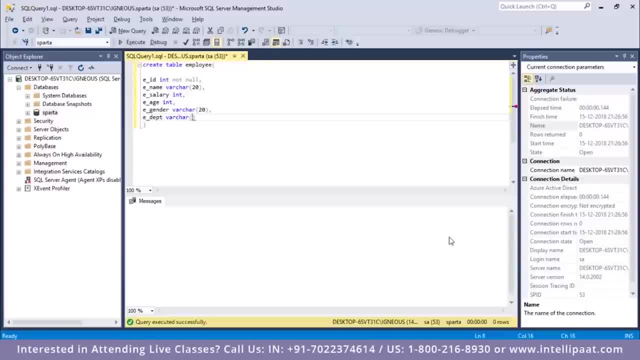 And this would be of type varchar two and a maximum length of 20.. Now, after this, I can set in the primary key. So I want this employee ID column to be the primary key. I will type primary key and inside the parenthesis I will give in E ID. 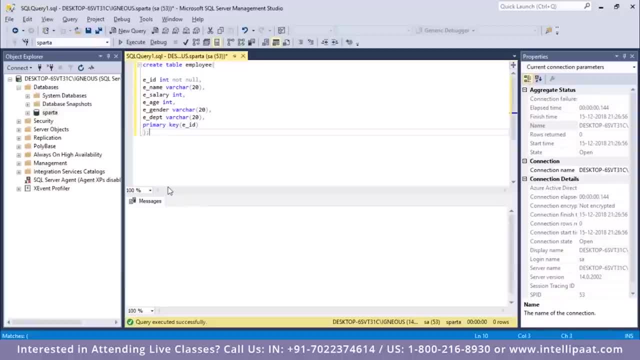 Right now. I will put in semi-colon over here to indicate that this is the end of the syntax. Now I will select all of this and click on execute Right. So we have successfully created the employee table. How do insert regards into a table? 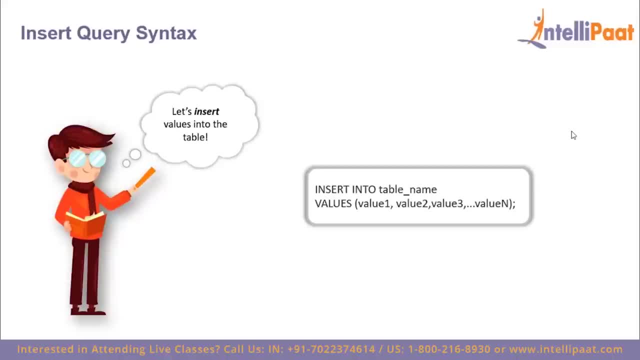 We can insert regards for this. insert into statement. Now let's understand this command properly. So first we'd have to type in the keywords, insert into, then we'll give in the table name, following which we'll give in the keyword values and, inside the parenthesis, we'd have to give in the values for each of the column respectively. 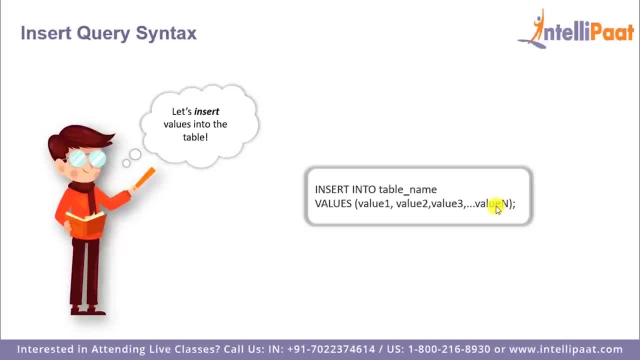 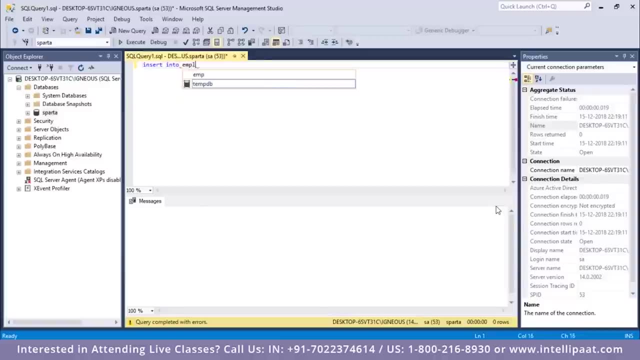 Now let's go to MS SQL server and insert regards into our employee table. So let me start with the command, So I will type in: insert into. then I'd have to give in the name of the employee. So I will type in the name of the table, which would be employee, after which I will give in the keyword values and inside the parenthesis I can give in all of the records. 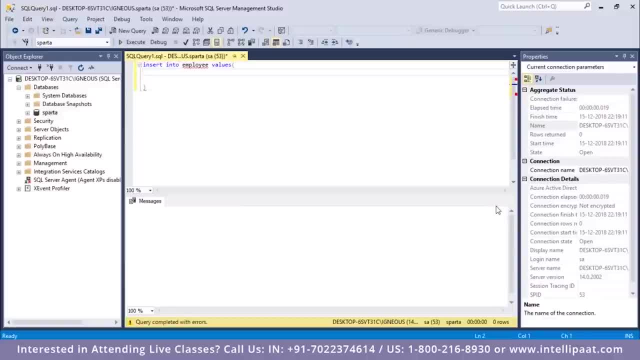 So let me start with the first record, Right. So we'll have to start off with the employee ID. So the employee ID is, let's say, one. Then the second column is the employee's name, and this is of type wire care. That is why I will give in the value inside these single quotes. 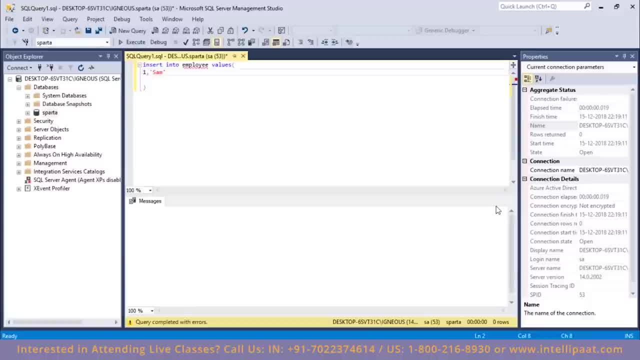 So the employee's name is Sam. After this we would have to give in the employee salary, So Sam earns Ninety five thousand dollars per annum. I will give in ninety five thousand over here. Then we have the employee's age, So Sam's age is forty five. 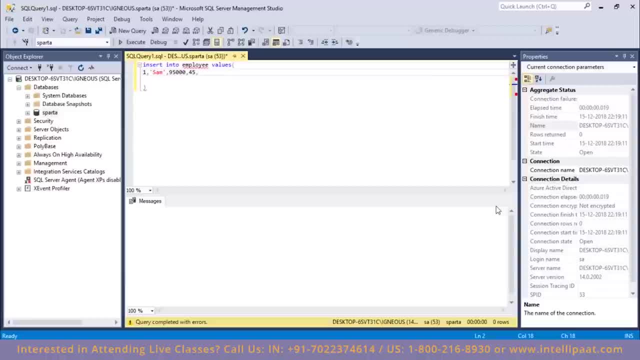 After which we have the employee's gender Again, since this is a variable character. So I will use the single quotes over here, and Sam is male, obviously, After which we'd have to give in the department in which the employee works. So again, this is variable length character. I will give in single quotes and Sam works in operations. 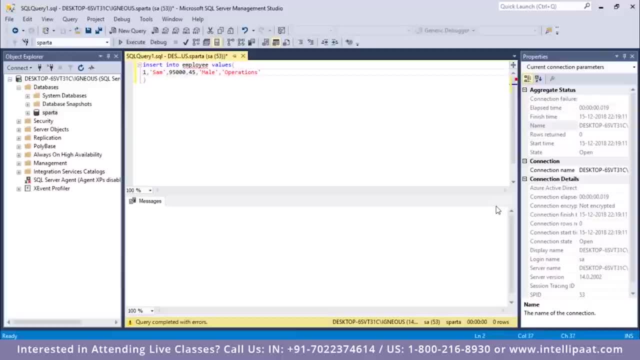 So let me type in operations over here Right Now. I will put in semi colon over here, I will select all of this and I will click on execute. So we have successfully inserted one record into our table. Now let me follow the same procedure and insert another record. 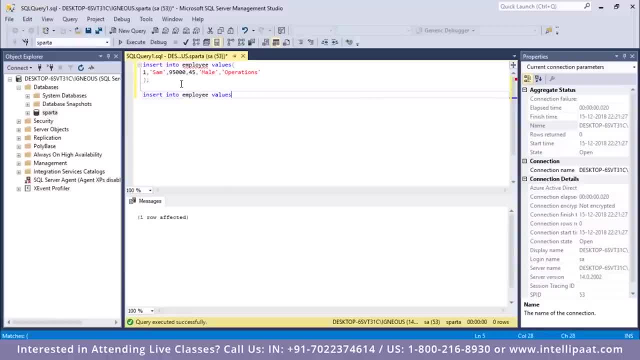 So insert into employee values, and inside the parenthesis, the first column is employee ID, which would be two. After this I'd have to give in the name of the employee. So the name of the employee is Bob, And Bob earns eighty thousand dollars, which is his salary. 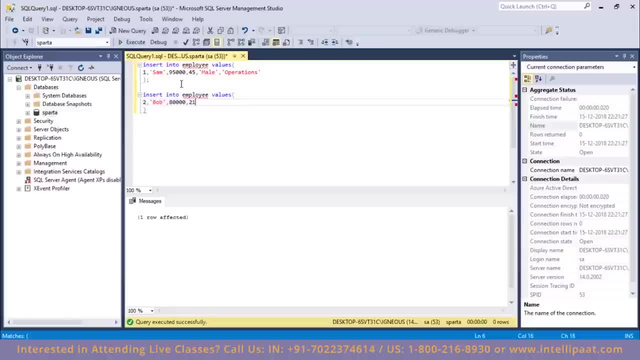 So let me put in eighty thousand over here. Then we have the employee's age, So Bob's age is twenty one. Then we have the gender of the employee, So Bob is male, obviously. again, Then we'd have to give in the department in which the employee works. 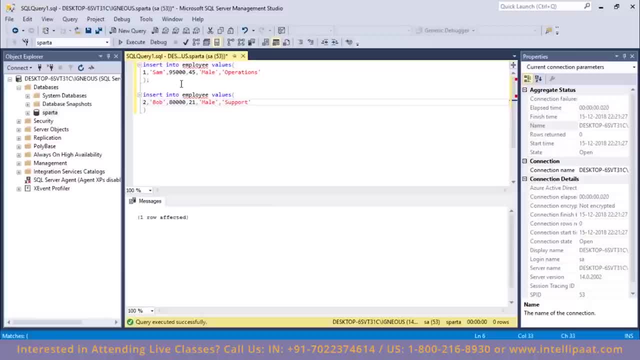 So Bob works in support. Again, I will put in semi colon. I'd have to select all of these. Let me click on execute Right. So we have also inserted the second record. Now let me insert the third record. So again it would be the same command: insert into employee values inside the brackets. 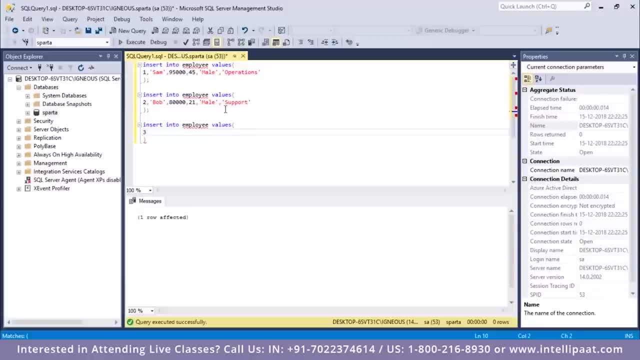 Let me give all of the values for the columns. So employee ID is three, The name is Ann, and Ann's salary is one hundred and twenty five thousand dollars per annum. She's quite rich, isn't she? And her age is twenty five. 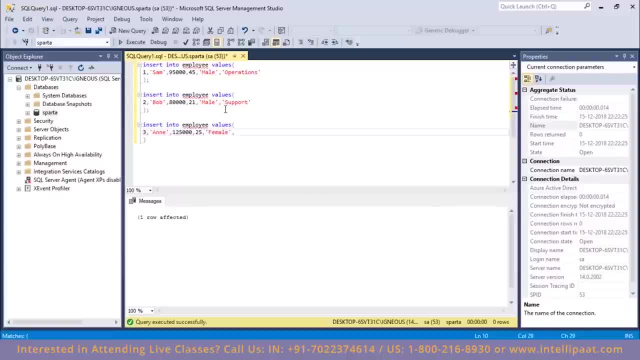 And she's obviously Female. Now we'd have to give in the department in which the employee works. So Ann works in analytics. Let me type in analytics over here. So it seems like people who work in analytics earn quite a lot, doesn't it? 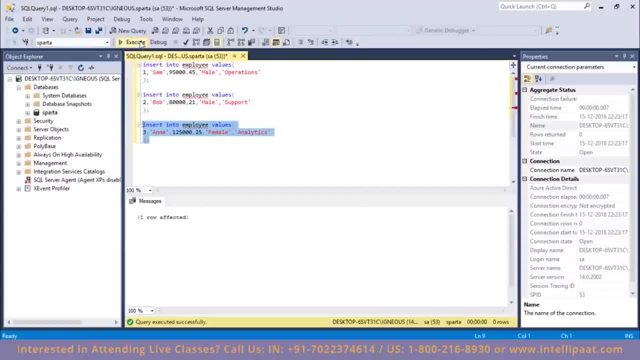 Let me put in semi colon over here, I'll select all of these and let me click execute. So, similarly, I will insert three more records into the same table. Right, so we have successfully inserted six records into a table. So, guys, this is how we can insert records into a table. 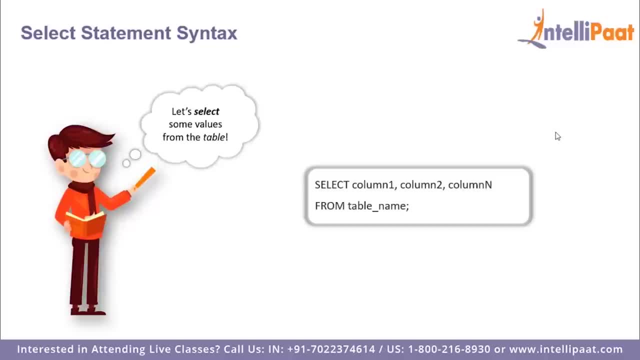 How to select data from a table. So first we will work with the select statement and learn how to extract individual columns. Then we will work with the select distinct statement to select only distinct values. So the select query is one of the most important commands in SQL and it is used to get data from a table. 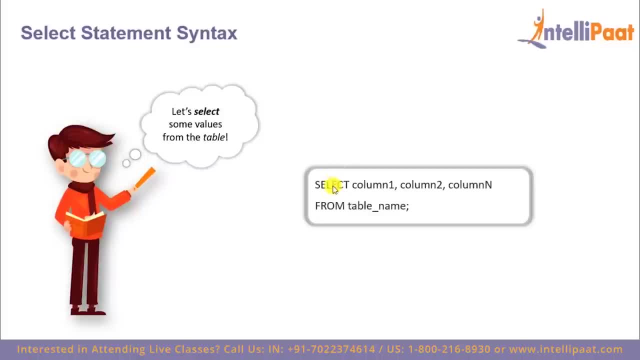 So let's have a look at the syntax. So first we give the keyword select And then list down all of the column names that you want to select, Following which we will give the keyword from And then finally give the table name from which we are supposed to select these columns. 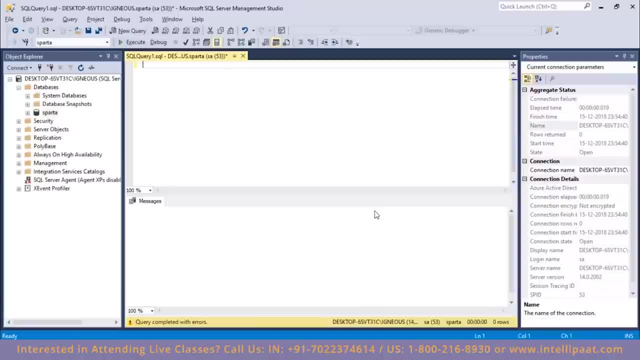 So let's select some data from our employee table. So let's say I want to extract only the employee name column from the employee table, So for that I would have to give in select and then I would have to give in the name of the column. 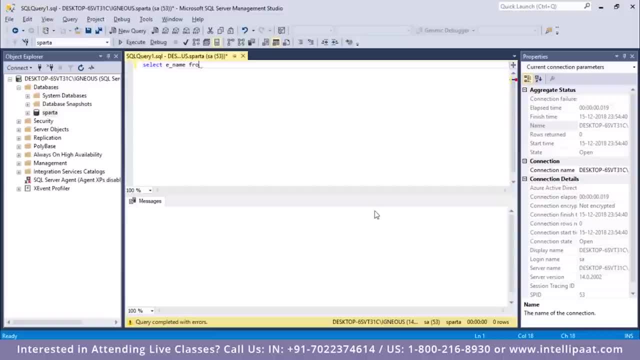 So the name of the column is ename, and then I will give in the from keyword, After which I will give in the name of the table, which is employee. Let me put in semicolon and let me hit execute Right. So I have successfully extracted only the name column from the entire employee table. 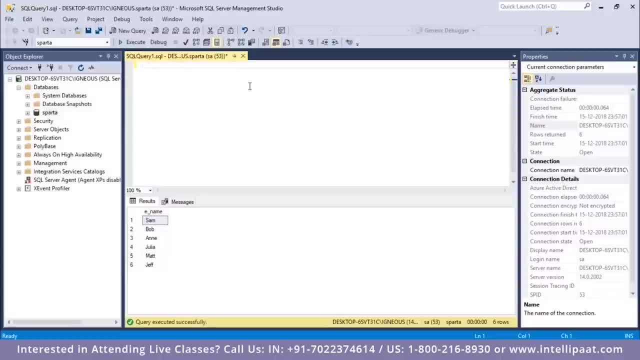 So, similarly, if I wanted to extract only the age column from the employee table, we would have to put in a similar syntax, So it would be select employee age from, and the name of the table is employee Execute Right. So we have extracted the age column from the entire employee table. 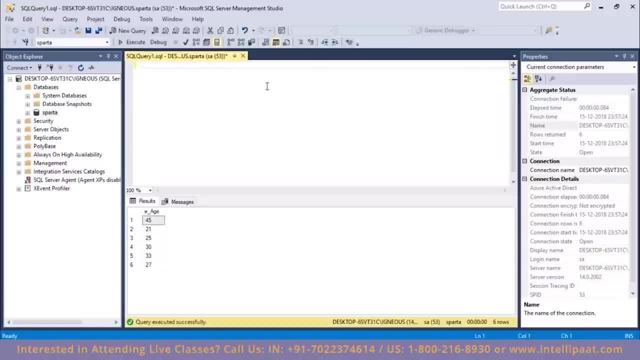 Now we can also extract multiple columns from our table, So for that we would have to separate each of the columns with a comma. So let's say I want to extract the name column, the gender column and the salary column from the entire employee table. 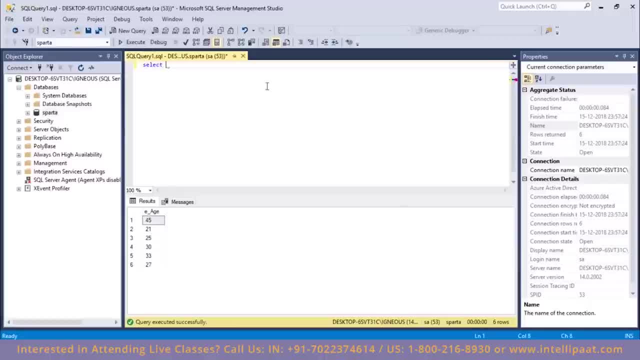 So let me write the syntax for that. So it would be select. So I will give in the first column, which would be ename. Now I would also want the gender. So I will put in the first column, I will put in e-gender, I'll put in a comma, and then I would also want the salary column. 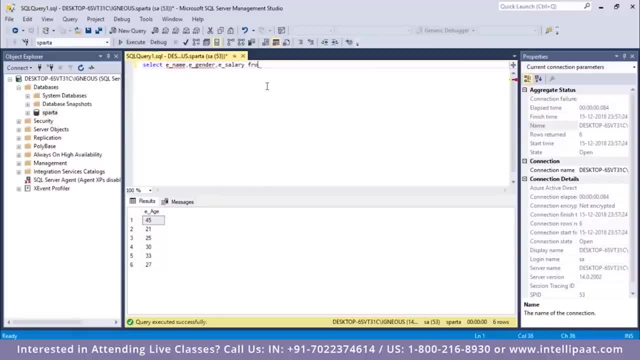 So I will put in e-salary, after which I will use the from keyword and then I will give in the name of the table, which would be employee semicolon, and let me hit execute Right. So I have extracted three columns from the employee table, and those three columns are ename, e-gender and e-salary. 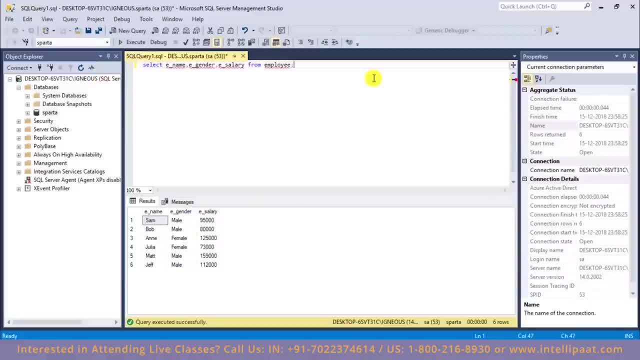 So this is how we can extract multiple columns from the same table. We can also extract the entire data from our table, And to extract the entire data from our table, we'd have to use the asterisk operator. So let me show you, guys, how it's done. 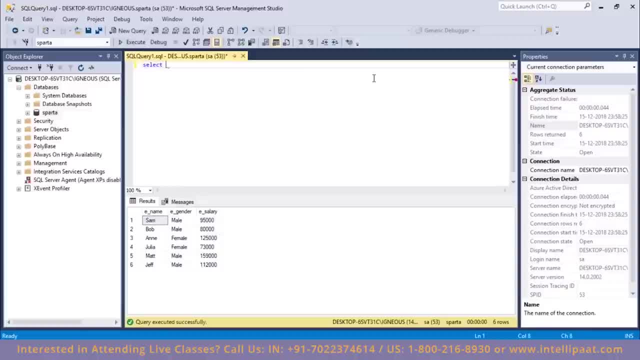 So the command would be select, and then I will put in star, after which it will be from employee. So as simple as that guy: select star from employee. So whatever table it is, all you have to do is select star from, and then you'd have to give in the table name. 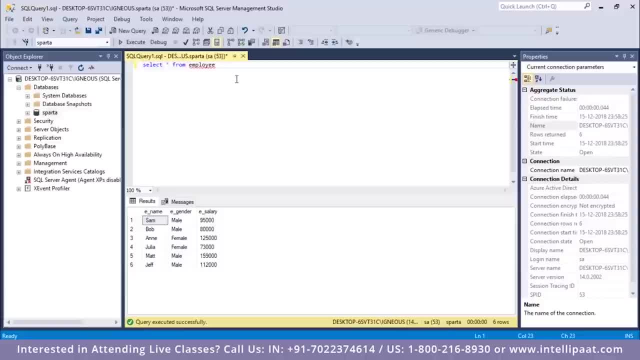 So this is how you can extract all of the data from a particular table. So I will give in semicolon and let me execute Right. So when I gave the command select star from employee, I was able to extract all of the data from the employee table. 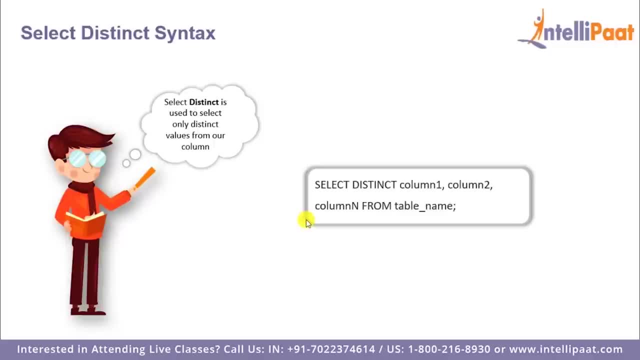 Now let's look at the select distinct statement. So a column often contains many duplicate values, and sometimes we'd want to extract only the distinct values from the column. So this is where select distinct comes in. So the syntax of select and select distinct is pretty much the same. 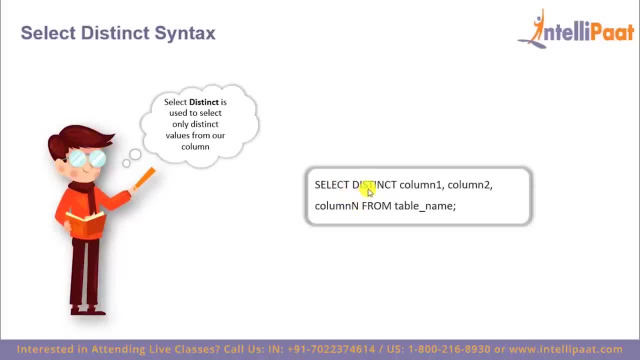 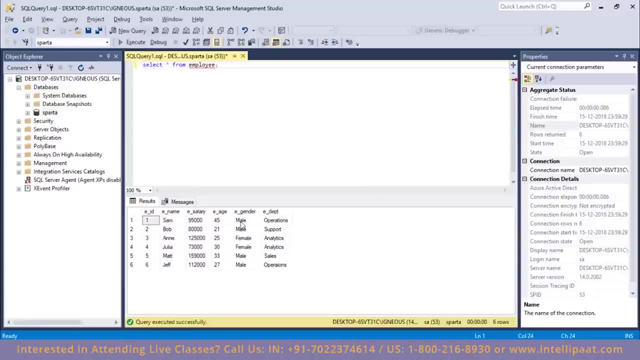 The only difference is we follow up the select keyword with the distinct keyword. Now let's select some distinct. So we have the distinct values from our employee table. If we have a glance at this gender column, we see that these two values are being repeated. 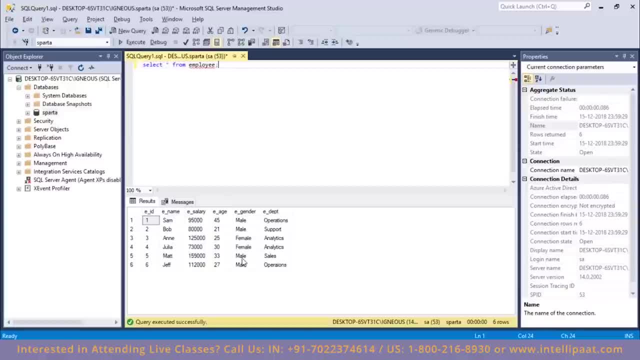 So we just have two values, male and female, and these two values are being repeated. So now, if I wanted to extract only the distinct values, so this would be the command for that. So I will type in select and I'll follow up the select keyword with the distinct keyword. 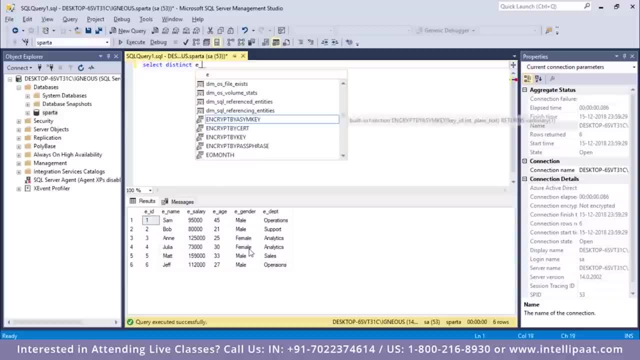 After which I'll give in the column name whose distinct values I'd want. So the column name would be: And then it will be from the name of the table, which is employee. So let's see what do we get. Select distinct e-gender from employee. 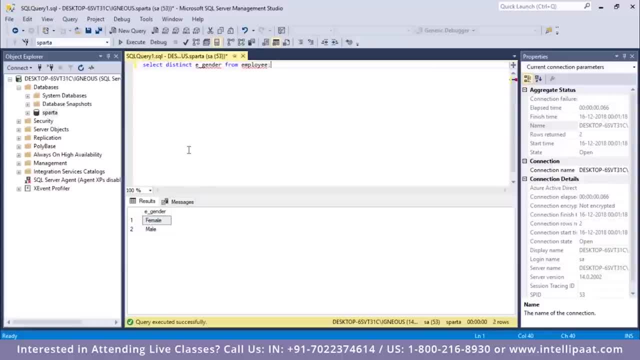 Right, So we see that we only get the distinct values, which are female and male. Now let me actually remove this distinct keyword and let me execute. So let's see what is the difference. right? So if I remove the distinct keyword, we get all of the values. 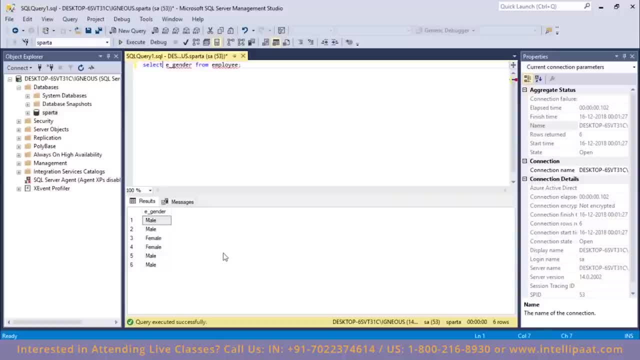 So male, male, female, female, male and female. Now. so if we use a distinct keyword, we'll only get the values which are different. So these are the cases where select distinct can be used. So the where clause is used to extract only those records that fulfill a specified condition. 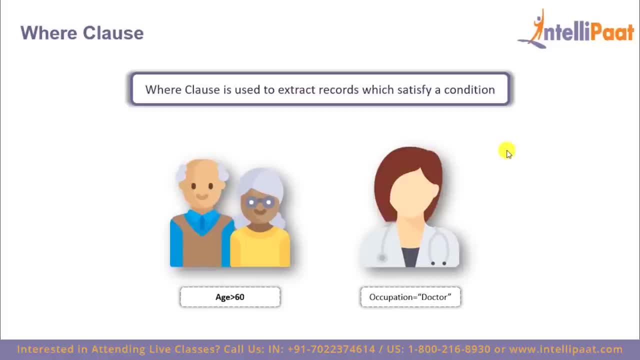 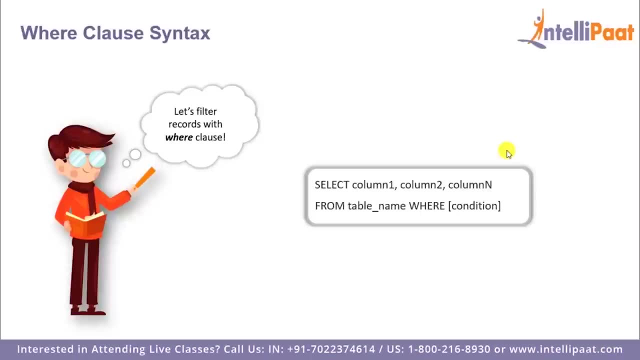 For example, we'd want to extract those records where the age of the person is more than 60, or filter out those records where the occupation of the person is doctor. Now let's have a look at the syntax of where clause. So we'll start with the select keyword. 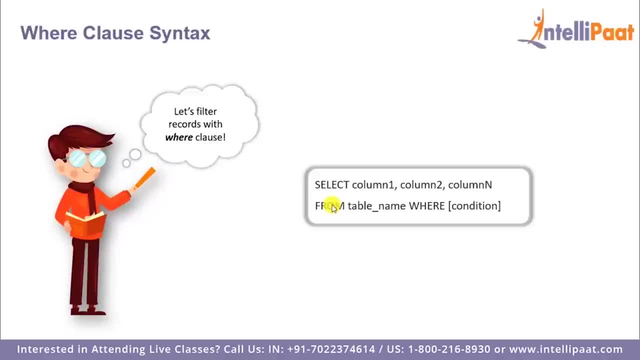 Then we will give in the list of all of the columns which we want to select, following which we'll use the from keyword And give the table name and finally use the where keyword and follow it up with a condition that would determine which records are to be extracted. 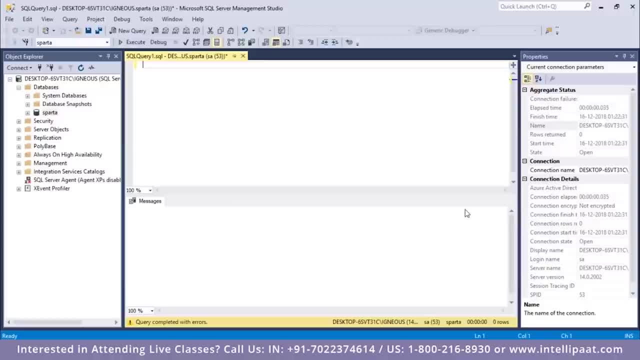 So let's filter out some records from our employee table. Now let's say we'd want to find out all of the female employees of our company, So for this I'd have to extract those records where the gender equals female. So let me go ahead and write the command for that. 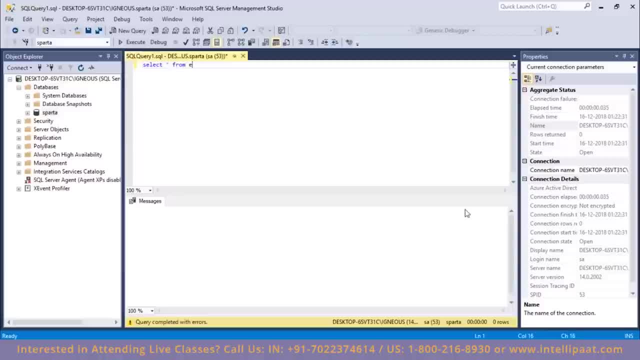 So that would be select star from. I will give in the table name Which is employee and then I will use the where keyword and follow it up with the condition. So the condition would be: E- gender is equal to female Right. So what I'm basically doing is I am extracting all of the female employees from this employee table. 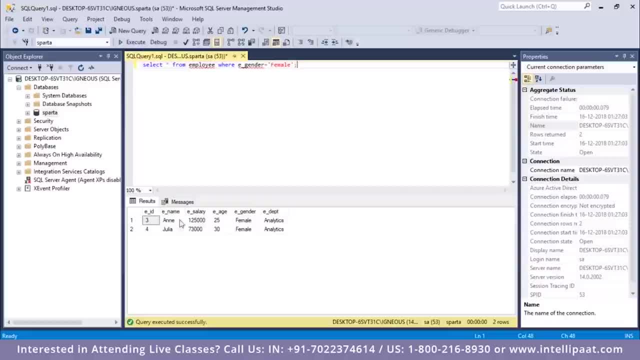 Let me hit execute Right. So Ann and Julia are the only female employees. Now I'd want to find out those employees whose age is less than 30. So let me write the command for that select star from employee where I will give in the condition. 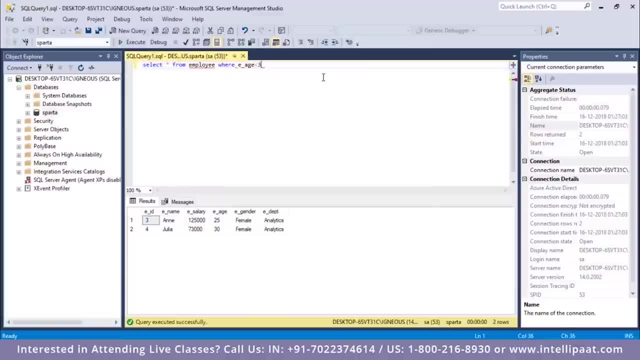 So this time the condition would be: E age is less than 30.. Right, So the age needs to be less than 30.. I'll give a semicolon, Let me hit, execute. Right, So these are the three employees, or these are the three records, where the value of E age is less than 30. 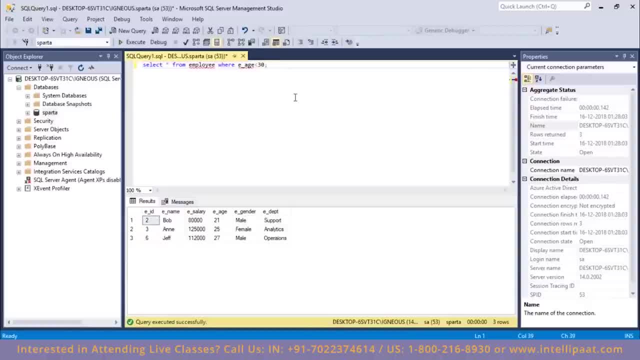 So Bob, Ann and Jeff, these are the three employees whose age is less than 30.. Now, similarly, let's say, I want to find out all of those employees whose salary is greater than $100,000.. So let me write the command for that. 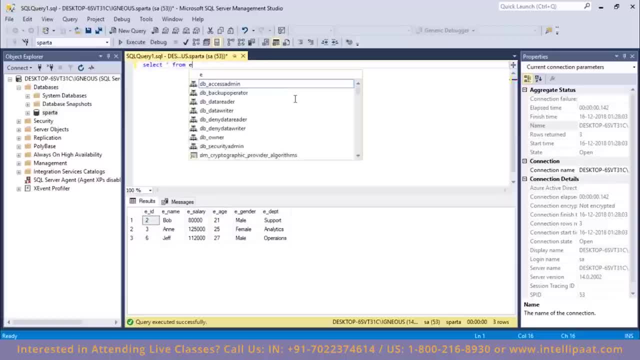 So this time the command would be: select star from employee, where so the condition would be: E salary is greater than $100,000.. Semicolon and execute. So Ann, Matt and Jeff are the three employees whose salary is greater than $100,000. 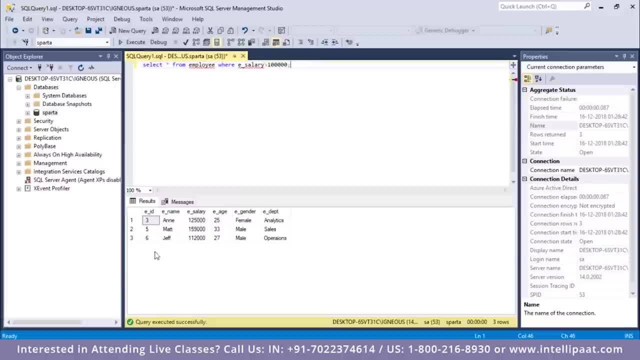 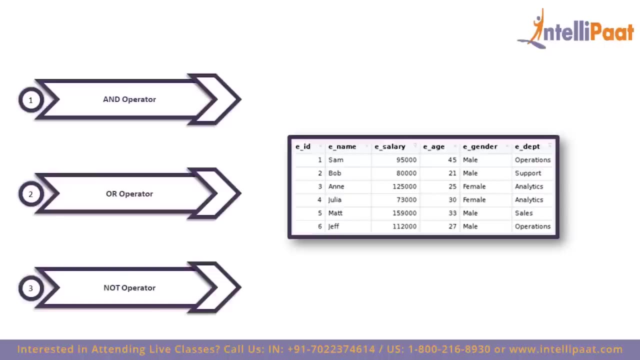 So Ann's salary is $125,000.. Matt's salary is $159,000 and Jeff's salary is $112,000.. So, guys, this is how we can filter out records with the WHERE clause, How to extract records on the basis of multiple conditions using the AND OR and NOT operators. 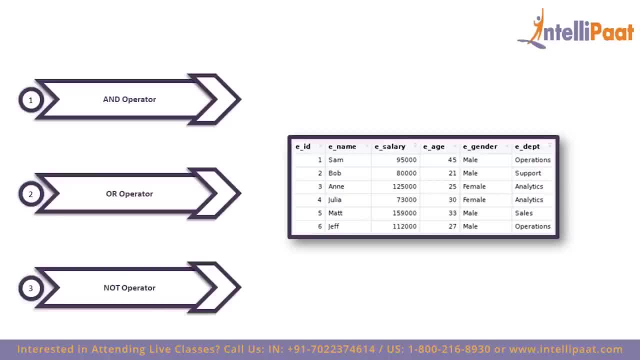 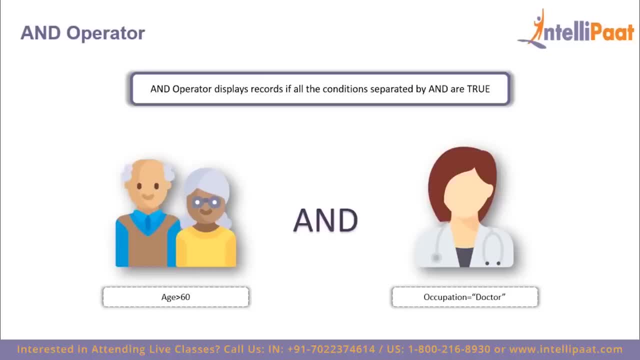 So we'll start with the AND operators First, then we'll filter records with the OR operator And finally we'll work with the NOT operator. So with the AND operator we can basically fetch those records which satisfy all of the conditions, separated by AND. 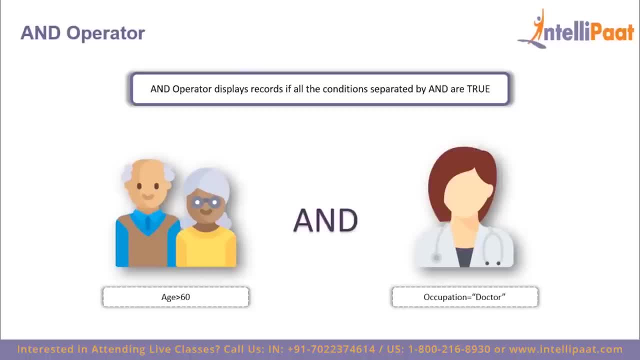 For example, we want to find out all the doctors whose age is greater than 60. So there are two conditions over here. First, the age needs to be greater than 60.. Second, the occupation needs to be doctor. So we'll get only those records. 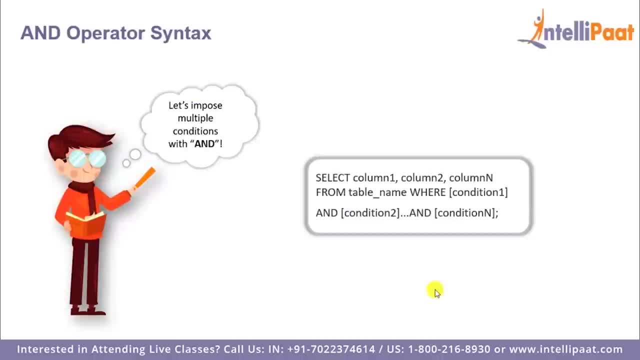 So we'll get only those records. So here both the conditions are being satisfied. Now let's have a look at the syntax. So here, after we give the first condition of the WHERE clause, we follow it up with the AND operator and give the second condition. 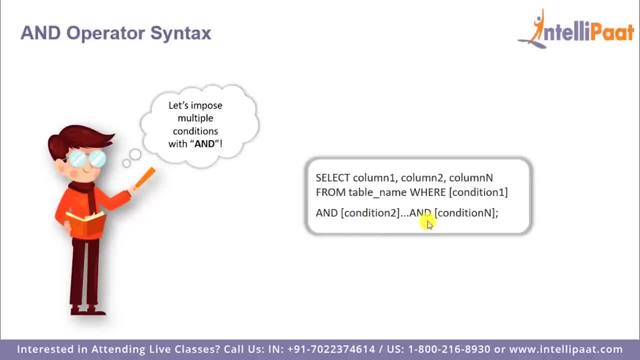 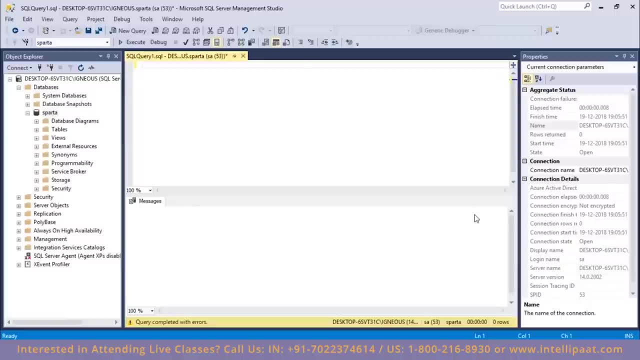 And similarly, if we have another condition to be satisfied, we'll again give the AND operator and then give the next condition. So let's fetch some records using the AND operator. So I'd want to extract all of those employees whose gender is male and age is less than 30.. 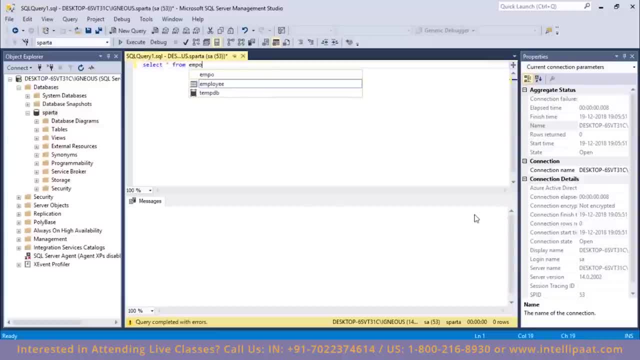 So the command would be select: Start from employee. I'll use the WHERE clause and then give it the first condition. So the first condition is: gender needs to be equal to male. So eGender is equal to male. I'll use the AND operator and then give it the second condition. 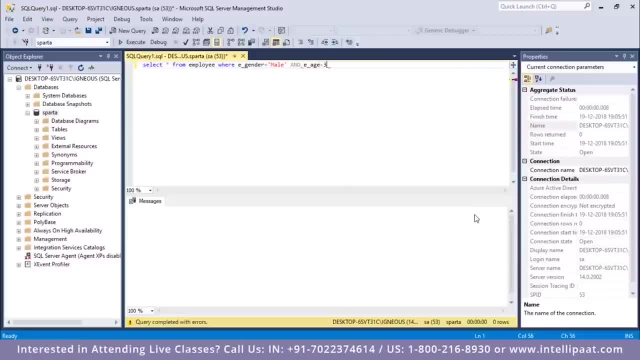 So the second condition is the age needs to be less than 30. Let me hit, execute. So Bob and Jeff are the two employees Who's gender is male and age is less than 30. Now, similarly, I'd want to extract all of those employees who work in the operations department. 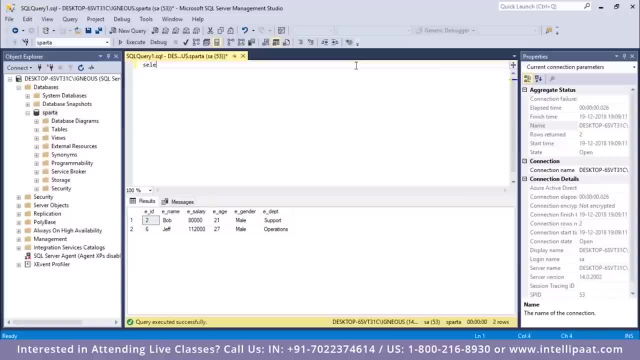 and their salary is greater than $100,000.. So the command would be select: Start from employee WHERE I have to give the first condition. So the first condition is: the department needs to be equal to operations. I'll use the AND operator again. 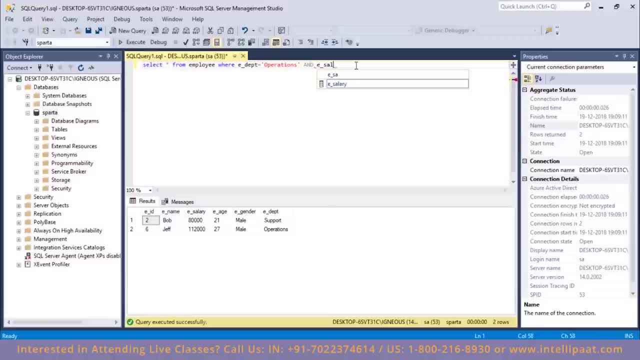 And then I'll give the second condition. So the second condition is the salary needs to be greater than $100,000.. Right Execute. So Jeff is the only employee who works in operations and his salary is greater than $100,000. 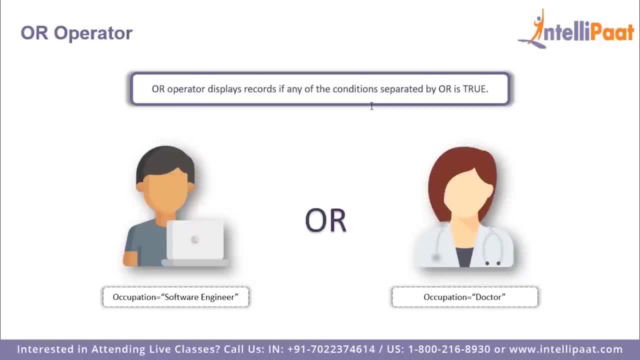 Then we have the OR operator. So the OR operator displays those records where at least one of the conditions is satisfied. For example, if we want to filter out either a software engineer or a software engineer, we can use the OR operator Or a doctor. 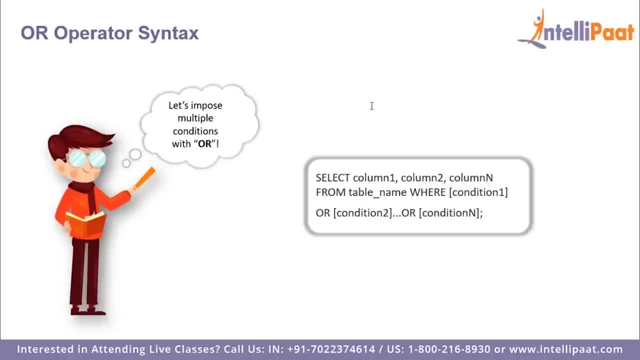 Then we can use the OR operator- And this is the syntax for the OR operator, So similar to AND operator. after we give the first condition, we follow it up with the OR operator and then give the second condition. Now we'll fetch some records from the employee table using the OR operator. 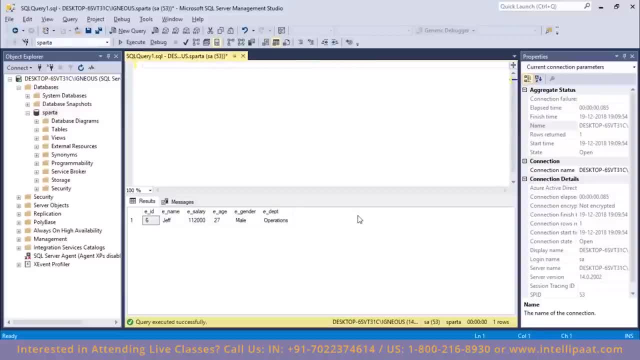 So I want to extract all of those records where the employee works, either in operations or in analytics. So the command would be: select: Start from employee WHERE. Start from employee WHERE. Start from employee WHERE. I need to get the first condition. So the first condition is: department should be equal to operations. 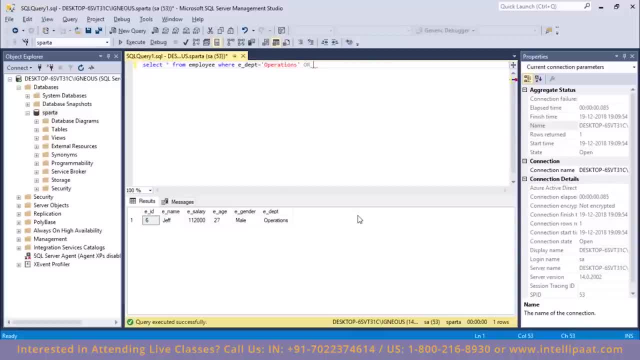 I'll use the OR operator now and then give the second condition. So the second condition is: the department needs to be equal to analytics, Right? So we have four records over here. So Sam works in operations and works in analytics, Julia works in analytics and Jeff works in operations. 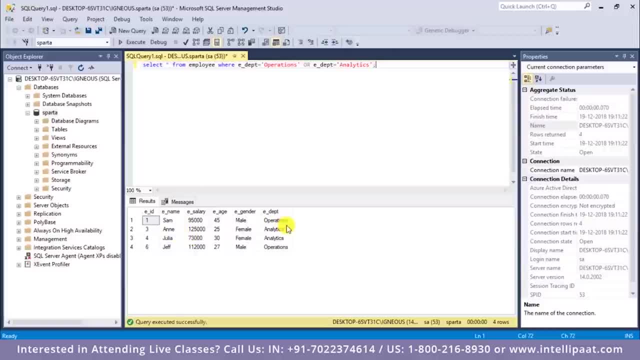 So there are four results, all of which two people work in operations and two people work in analytics. Now, similarly, I'd want to extract those records where either the salary is greater than $100,000 or the age is greater than 30.. 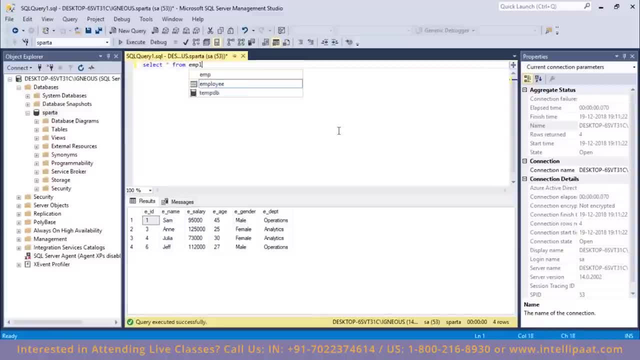 So this would be the command Select: Start from employee WHERE Salary is Greater than $100,000.. I'd have to use the OR operator and then give the second condition. So the second condition is age needs to be greater than 30.. 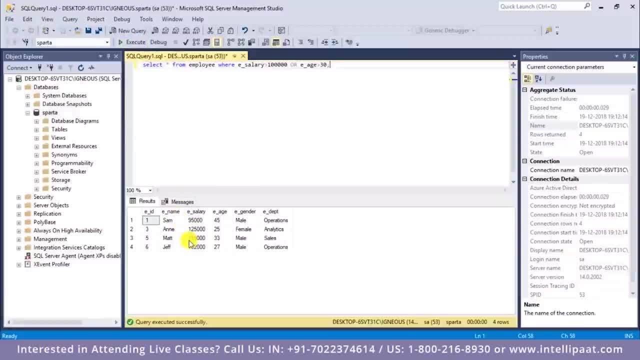 Execute. So again, we have four records over here. So the first record is Sam, whose age is greater than 45.. Then we have Anne, whose salary is greater than $100,000.. Then we have Matt, which satisfy both the conditions. 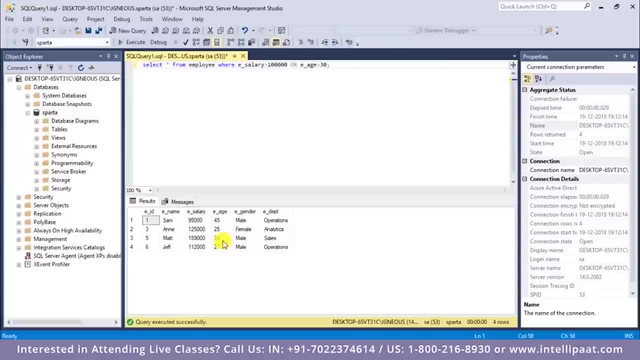 Actually, his salary is greater than $100,000.. And his age is also greater than 30. Then we have Jeff, whose salary is greater than $100,000.. So these four records. we see that at least one of these conditions is being satisfied. 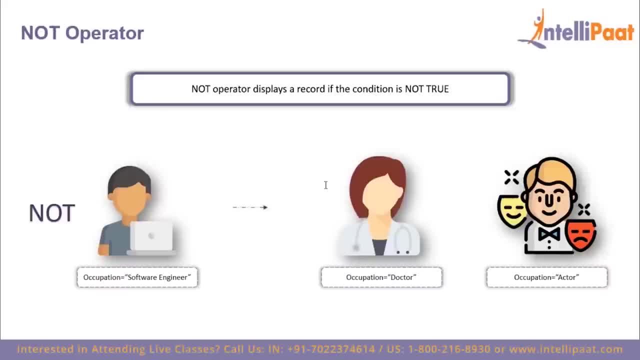 And finally we have the NOT operator. So with the NOT operator we can extract those records where the condition is NOT true. For example, if I wanted to extract all those records where the occupation of the person is NOT equal to software engineer, 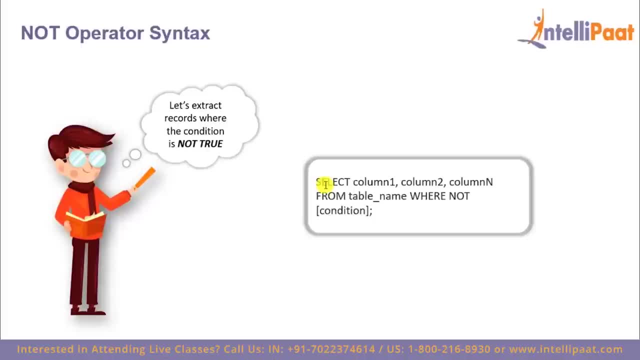 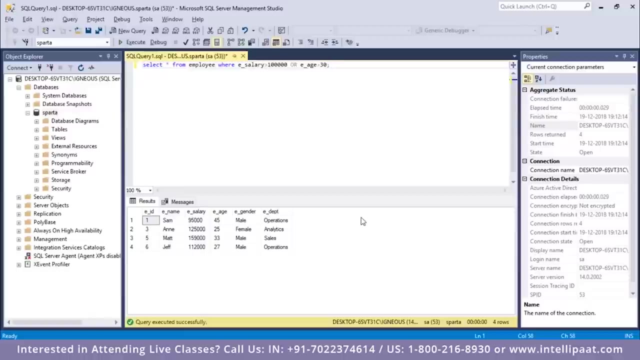 then I'll use the NOT operator operator. so let's have a look at the syntax of not operator. so here we follow up the var clause with the not operator and then give the condition: now let's work with this not operator. so I want to extract all of those records where the 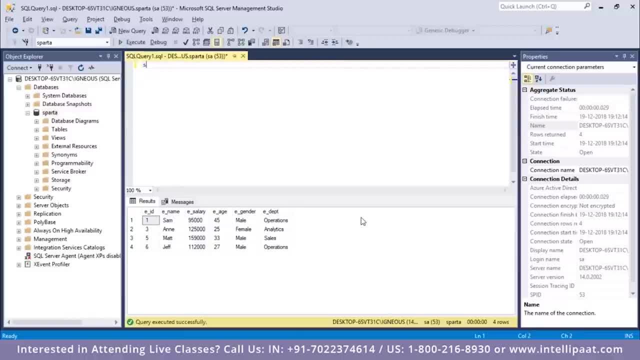 gender is not equal to female. so the command would be select star from employee var. after var clause I need to use the not operator and then give the condition. so gender is equal to female, right. so before the condition I use the not operator. so this would basically give me all of the records where gender 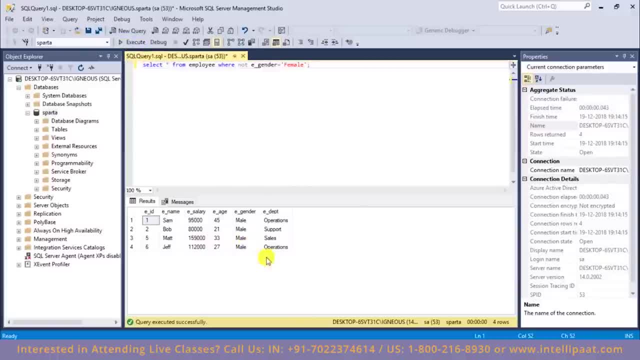 is not equal to female, so I'll hit execute. so you see that I get four records in total and all of those four records the gender value is male. now, similarly, I'll extract all of those records where the age is not less than 30. right, so select star from employee var. I need to follow it up with. 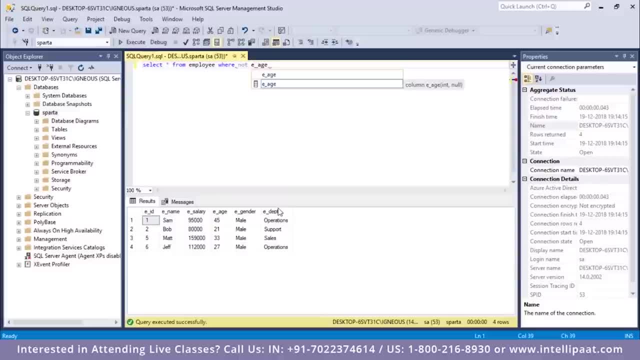 the not operator and then give the condition, which would be: e of age is less than 30. so this is the actual condition: e of age is less than 30. and since I preceded with the not operator, I will get all of the records where age is actually not less than 30. I'll hit. 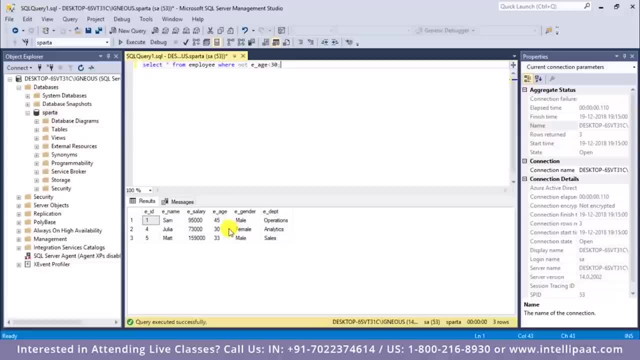 execute. so these are the three employees whose age is not less than 30. we have Sam, whose age is 45, we have Julia, whose age is exactly 30, and then we have Matt, whose age is 33. so, guys, this is how we can work with and or and, not operators. 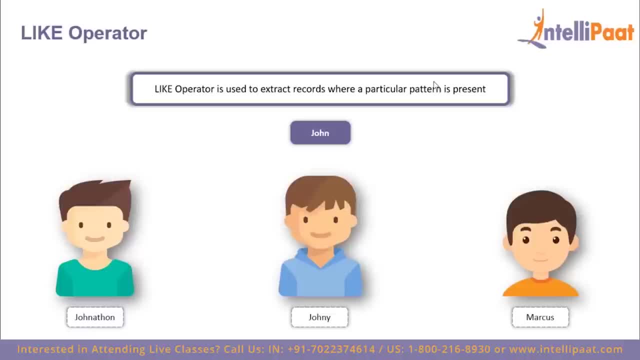 how to extract records with a like and between operators. we'll start with a like operator, for the like operator is used to extract those records from a table where a particular pattern is present. for example, we do want to extract all those records where the person's name includes John. so if we 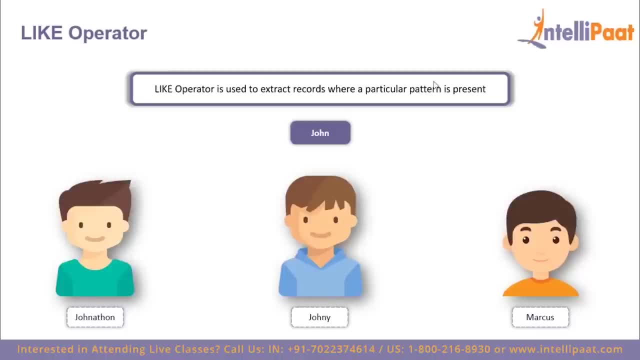 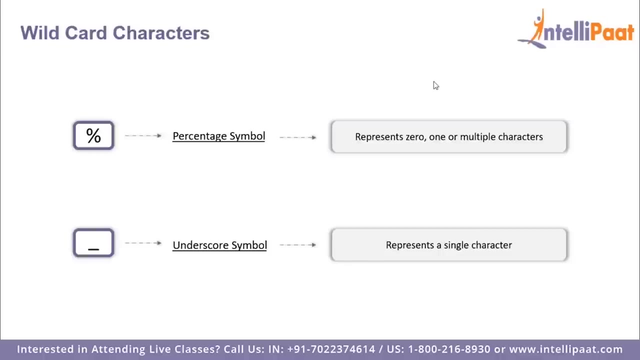 have records of three people in our table with the names Jonathan, Johnny and Marcus, then with the help of like operator, we can extract records where the names are Jonathan and Johnny, since they have the required pattern present in them now. the like operator is used in conjunction with the wild-card characters. 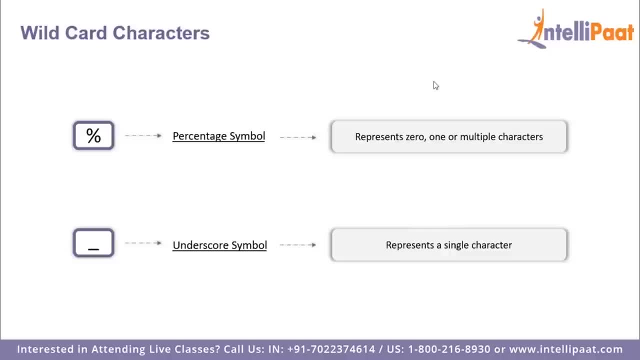 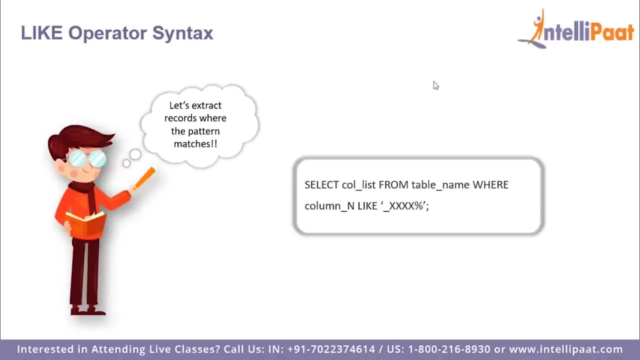 and there are two wild-card characters. first one is the percentage symbol and the second one is the underscore character. so the percentage symbol is substitution for zero, one or more characters, while the percentage symbol is substitution for a single character. and this is the syntax for the like operator after giving the where clause be. 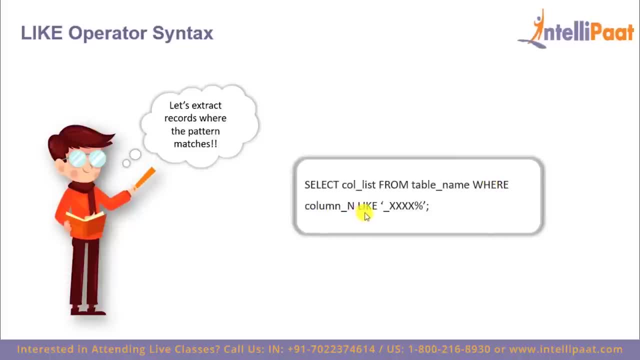 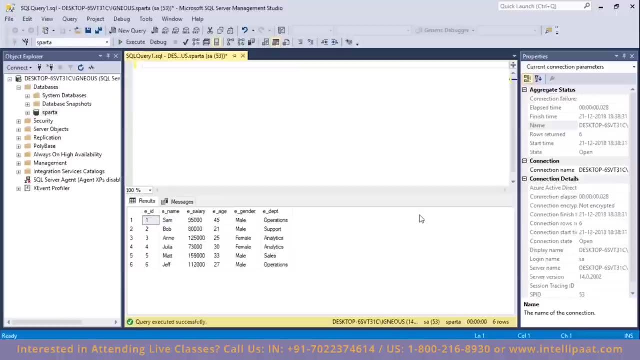 given the column name followed by the like operator and then the pattern which you want to extract. and keep this in mind, guys: the pattern should be inside single quotes. now let's do some operations with a like operator, so let's add what we extract: all of those records where the employees name starts with the letter J, so the 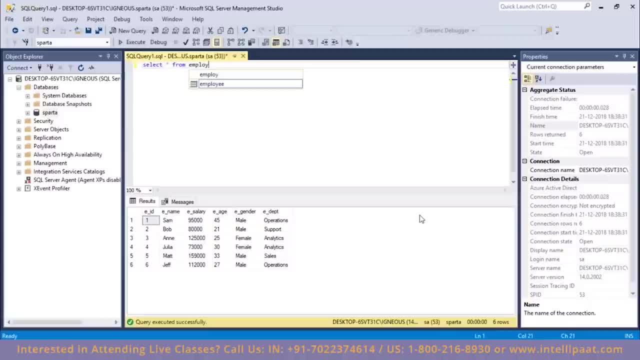 command would be select star from employee, where I will give in the condition, which would be E name, following which I will give in the like operator and inside single quotes, since the name should start with J, I will type J, after which I will use the percentage wild-card. 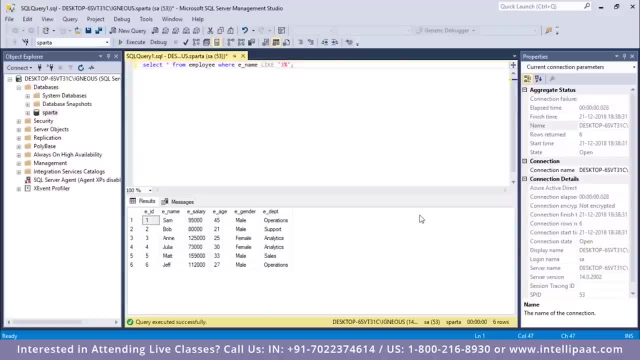 so all of those names with start with J would be extracted with this command. so let me hit, execute. so Julia and Jeff are the two employees whose name starts with G. now, similarly, I want to extract all of those employees whose age is in the thirties, right. 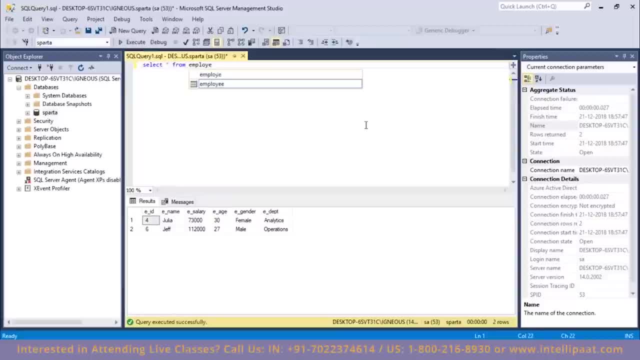 select star from employee where I need to keep the condition. so E age, following which i'll give the like operator and then single quotes. The age needs to be in 30s. So after 3, I will use the underscore wildcard character and then put in the semicolon. Let me execute. So we have Julia and Matt over here. So 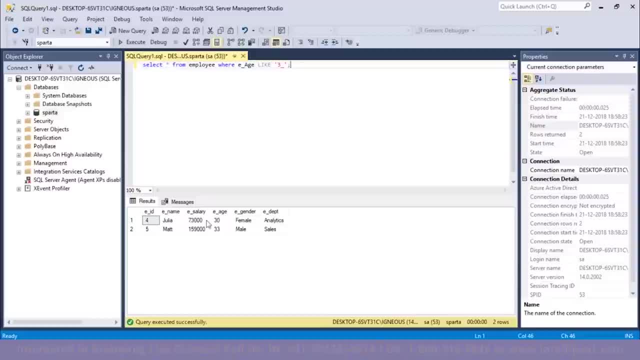 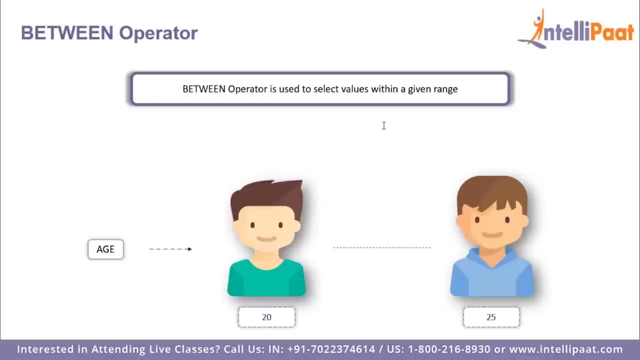 Julia's age is 30 and Matt's age is 33.. So they are the two employees whose age is in the 30s. Now let's look at the between operator. So the between operator is used to select values between a given range. For example, we can extract only those records where the age of the person is. 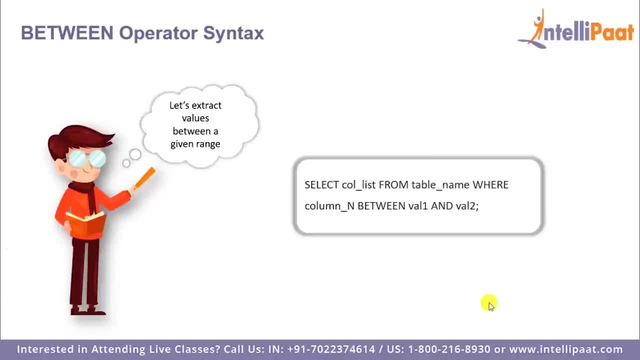 between 20 and 25.. And this is the syntax, After where clause we give in the name of the column, then we give the between keyword, after which we give in the lower value of the range, then use the end operator and then give the maximum value of the range. So I want to extract. 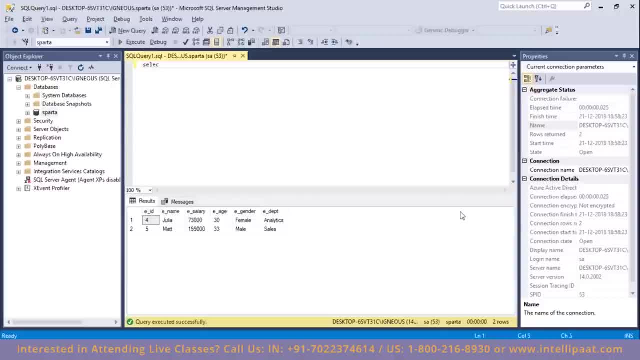 all of those employees whose age is between 25 and 35. So the command is: command would be: select star from employee where the condition would be: e age should be between 25 and 35.. Execute. So Ann, Julia, Matt and Jeff are the four employees whose age is between 25. 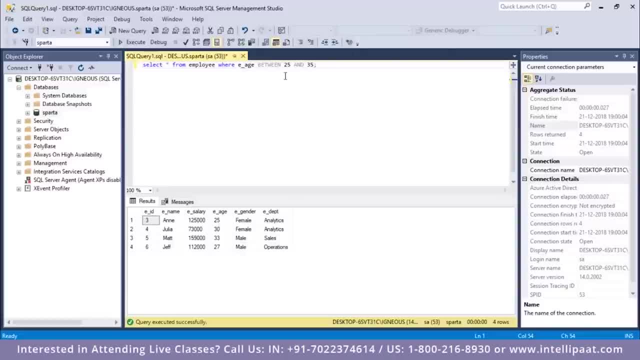 and 35.. So, as you see over here, this value is inclusive, right, 25 is inclusive. So Ann's age is 25.. Julia's age is 30.. Matt's age is 33.. And Jeff's age is 27.. And these are the four employees whose age is between 25. 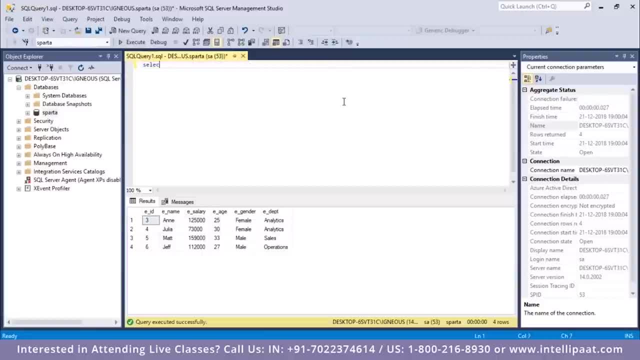 and 35.. Now, similarly, I'd want to extract all of those employees whose salary is between $90,000 and $120,000.. So the command would be: select star from need to give in the name of the table which is employee. Then I'll use the where clause and then give the condition. So the condition. 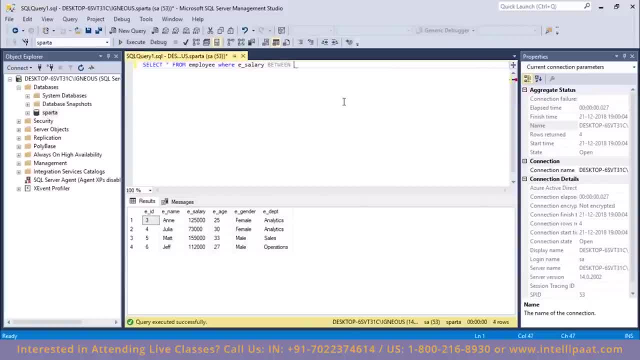 would be e salary between 25 and 35.. So I'll use the where clause and then give the condition. So the salary needs to be between $90,000 and $120,000.. I'll put a semicolon, Let me hit, execute. So, Sam. 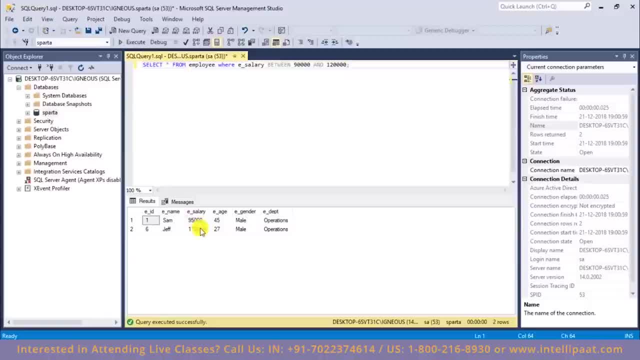 and Jeff are the two employees whose salary is between $90,000 and $120,000.. So Sam's salary is $95,000 and Jeff's salary is $112,000.. Some basic functions in SQL. So we'll look at the min function. 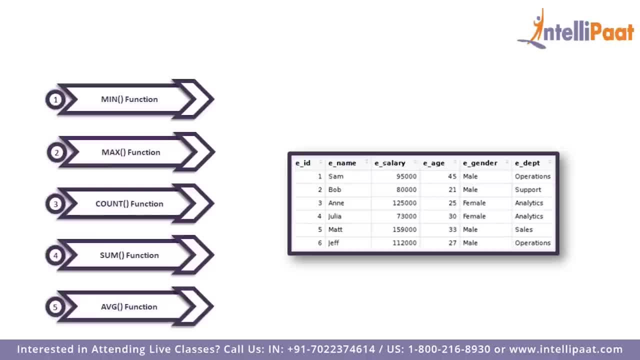 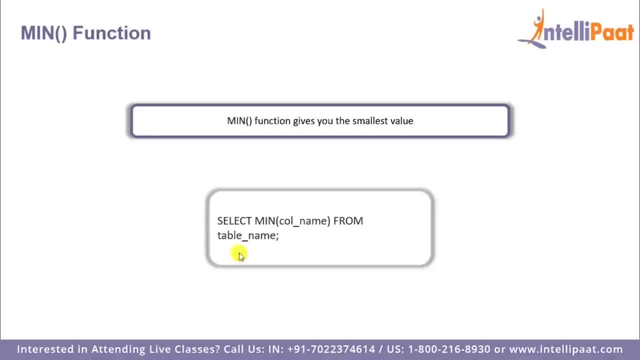 max function, count function, sum function and average function. Let's start with the min function. The min function gives the smallest value in a column. Let's look at the syntax. First we give in the select keyword, Then we give the min function And inside the parenthesis we specify the name of that column from which we 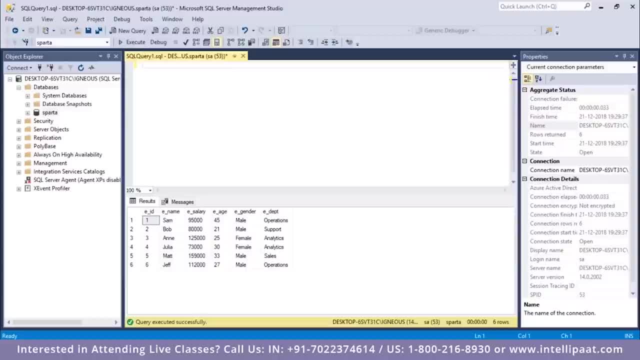 are supposed to find the minimum value. So I want to extract the age of the youngest employee of the company. So this would be the command for that Select, And then I'll use the min function and then pass in the column which would be e age. 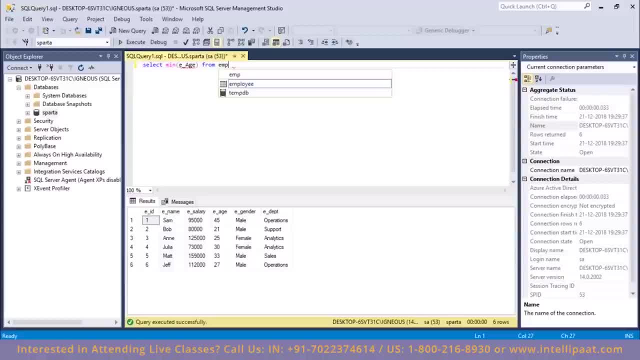 I'll use the from keyword and then, given the name of the table, which would be employee. So the total command is select minimum of e age from employee, I'll hit execute. So you see that the minimum age in the table is 21.. Similarly, if I wanted to extract the salary, 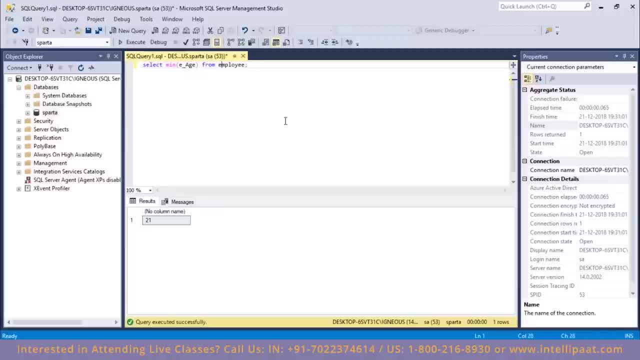 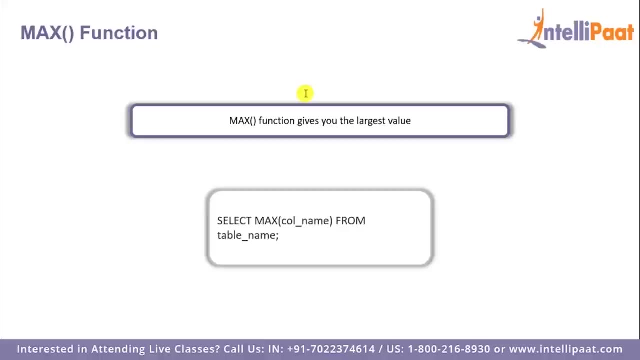 of that employee who would get the least salary. So the command would be select min and instead of e age it would be e salary from employee. So the salary of the employee who earns the least the least is $73,000.. Then we have the max function. The max function gives the 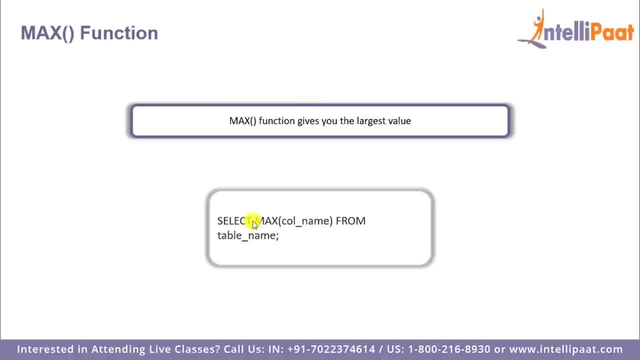 largest value in a column. Here again, we give in the select keyword, following which we give the max function, and inside the function we specify the name of the column from which we're supposed to get the maximum value. Now I'd want to extract the maximum age and maximum salary from this table, So this would be: 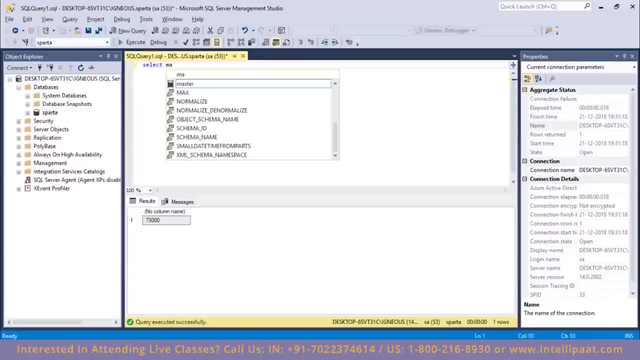 the command for that Select and I will start off by extracting the maximum age Inside the max function. I will pass in the column which is E of age and then I'll use the from keyword and then give in the name of the table, which is employee. 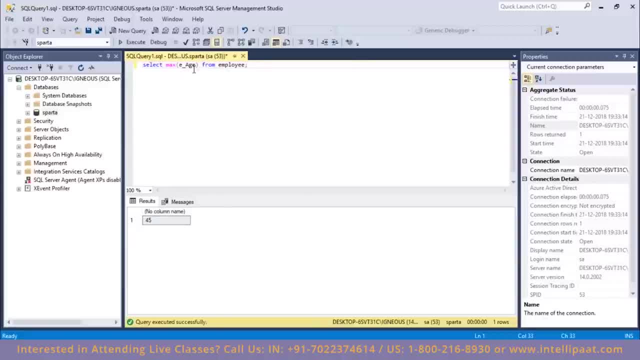 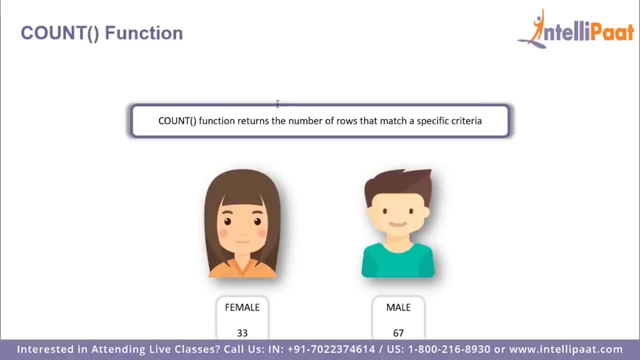 So the maximum age of an employee is 45.. Similarly, I want to find out the maximum salary, So that would be E salary from employee Execute. So the maximum salary is $159,000.. Then there's a count function, So the count function returns. 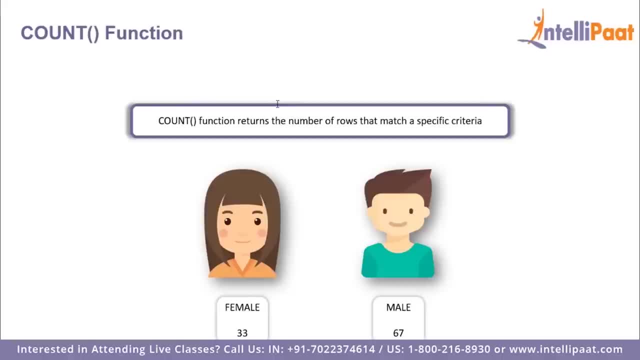 the number of rows that matches specified criteria. That is, if we wanted to find out the number of male and female employees in a company, then we can use the count function. Let's look at the syntax. So, after the select keyword, you will use the count function and give in an asterisk inside the parenthesis. 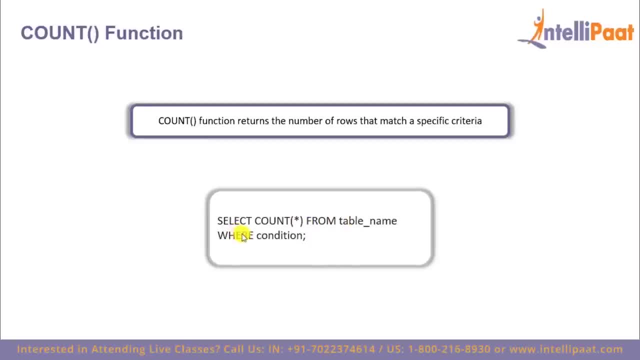 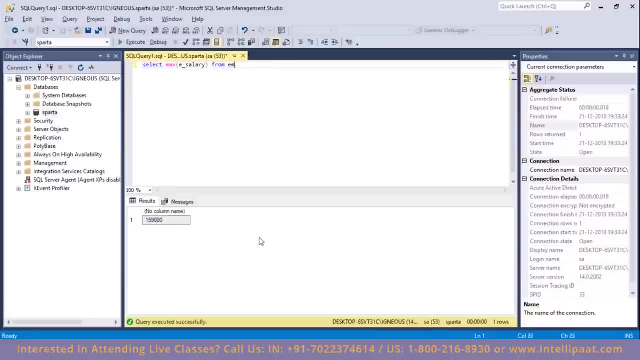 Then you will give the table name and finally, you will use the where clause to give the condition. So let's use this count function to get the count of number of male and female employees. So I'll start out by getting the count of number of male employees, So select I will. 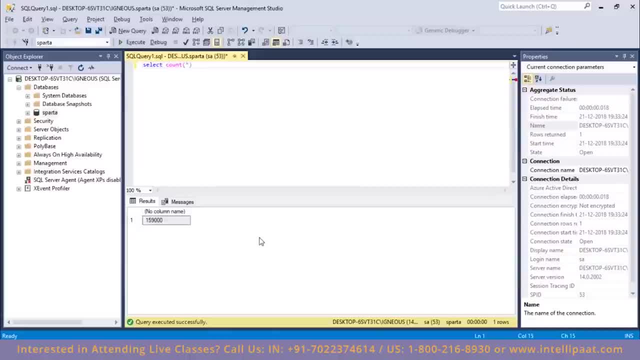 use the count function and inside the count function I will pass in the asterisk symbol, After which I'll use the from keyword and then give in the name of the table, which would be employee. Then, using the where clause, I will give in the condition. So I'd want the count of all of the male employees. So E of 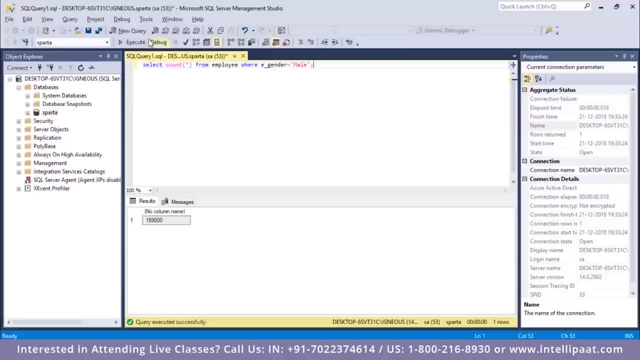 gender should be equal to male. Let me see what do we get. So there are 4 male employees in total. Similarly, if I wanted to get the count of all the female employees, the command would be: select count of stars from employee where egender equals female Right. so this would be the only. 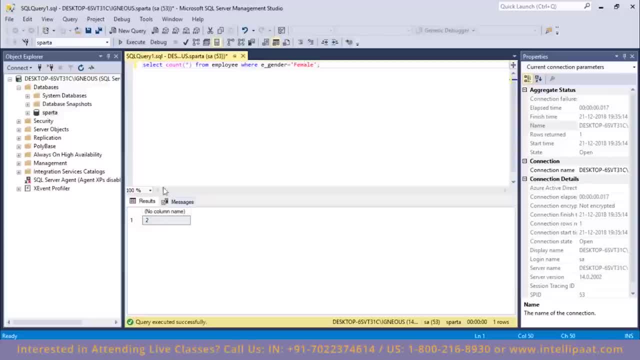 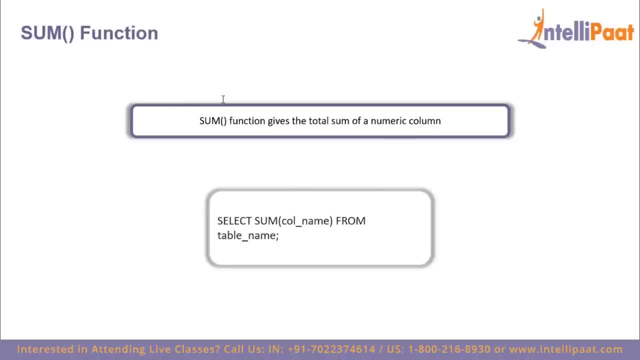 difference. I'll hit execute, So I get 2.. So there are 2 female employees in the entire organization. Then we have the sum function. So the sum function would give you the total sum of a numeric column, and this is the syntax. So here, 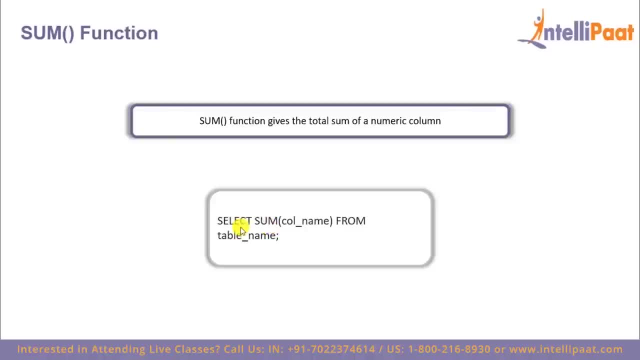 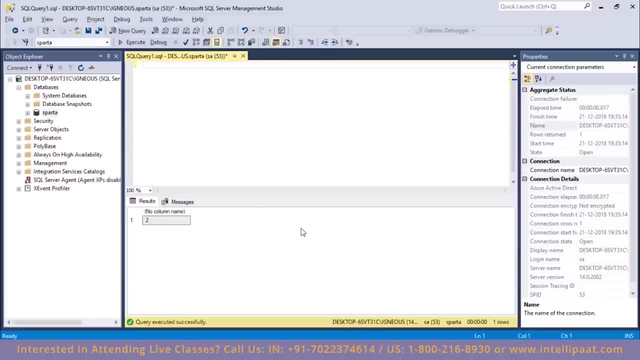 we will give in the sum function after the select keyword and give the column name inside the parenthesis. so I want to get the total sum of salaries of all of the employees, right. so the sum of salaries of all of the employees select, and then I'll use the sum function and then I'll pass in the column which would: 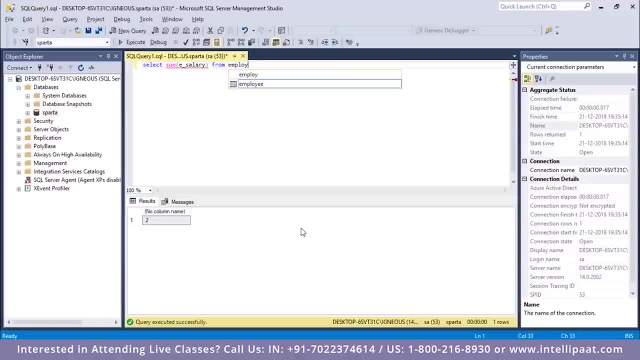 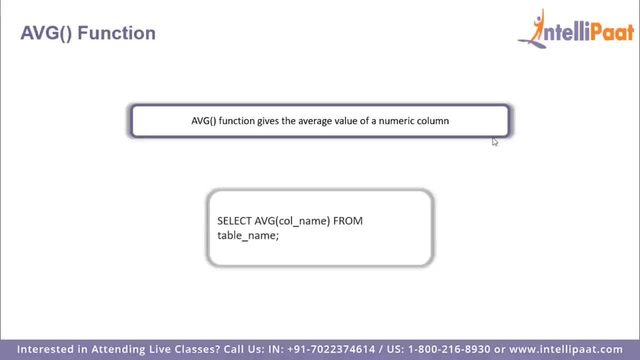 be e salary from the name of the table, which is employee. so the total salary of all of the employees included is six hundred and forty four thousand dollars per annum. and finally, we have the average function. so the average function gives us the average value of our numeric column and 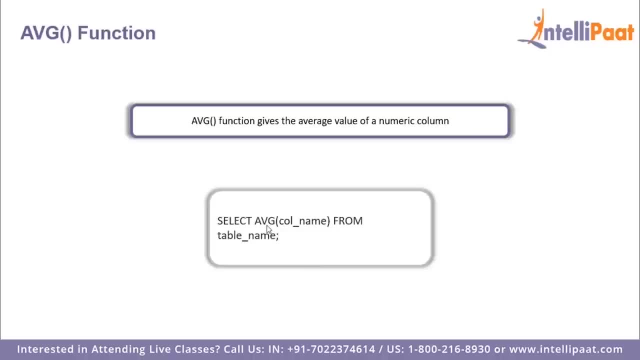 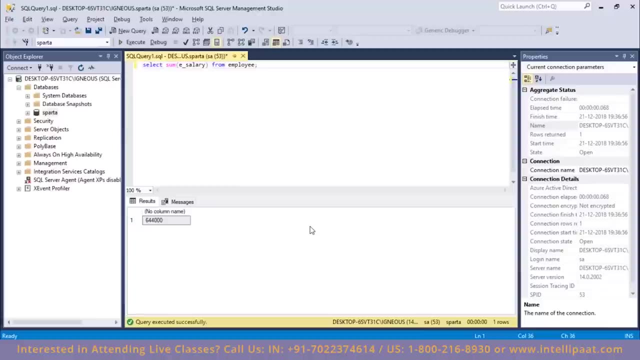 the syntax is same as the rest, so we'll give in the average function after the select keyword and give the column name inside the parenthesis. so this time I don't want to get the average age of all of the employees, so select, select, select, and then I will use the AVG function and then given the column which would be: 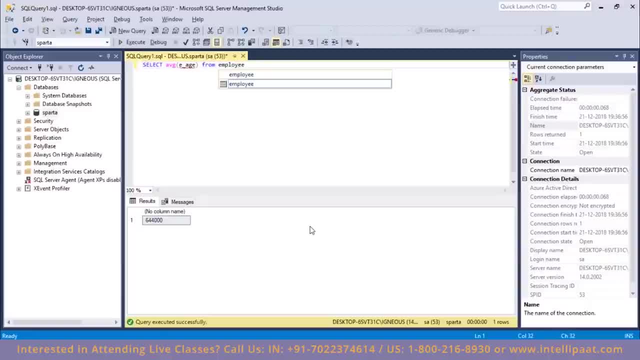 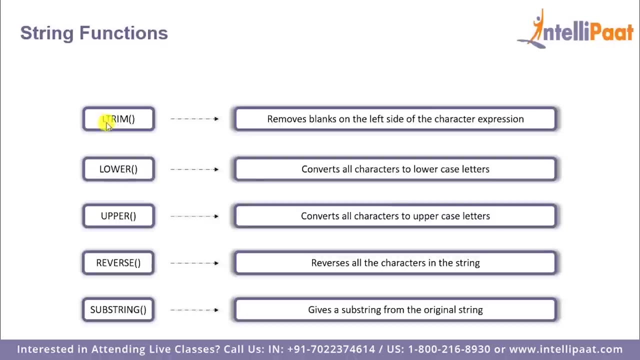 e age from the name of the table, which is employee. so the average age of all of the employees is 30. so, guys, these were some of the aggregate functions in SQL, some string functions. so first we have the L trim function, which helps in removing the blank spaces on the left side of the character expression. let's 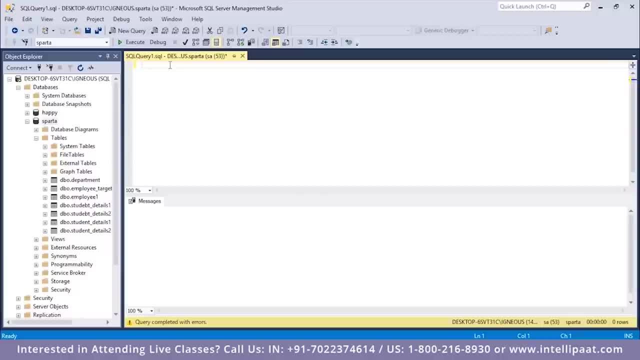 implement this function in SQL server. so let me first create a string with some blank spaces on the left side, so I'll type select and then I will give some blank spaces on the left side. now let me pass in a string and I'll name the string to be sparta. I'll hit execute. 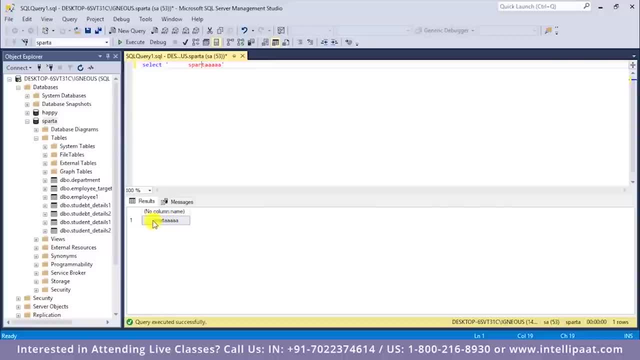 right. so this is the string which has some leading spaces on the left side. now, if I want to remove all of these blank spaces on the left side, all I need to do is use the L trim function. so I will type select l trim and inside this I will pass in the string with the leading spaces. so 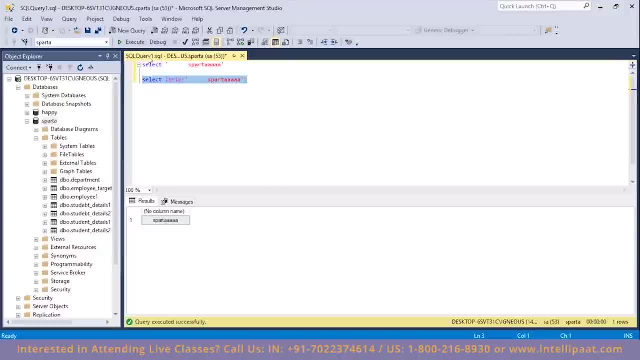 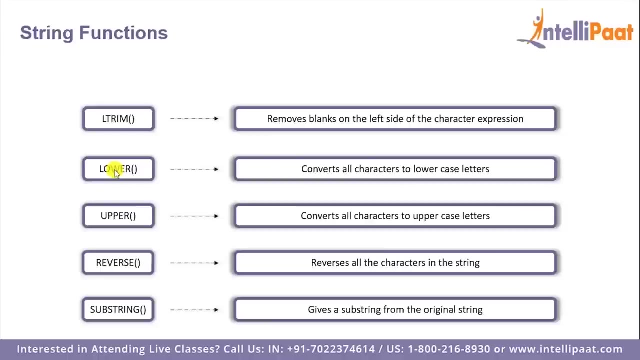 I'll copy this and I will paste it over here now. let me execute both of this simultaneously. right? so this is the string with the leading spaces, and when we use the l trim function, all of those blank spaces on the left side were removed. then we have the lower function, which basically converts all the 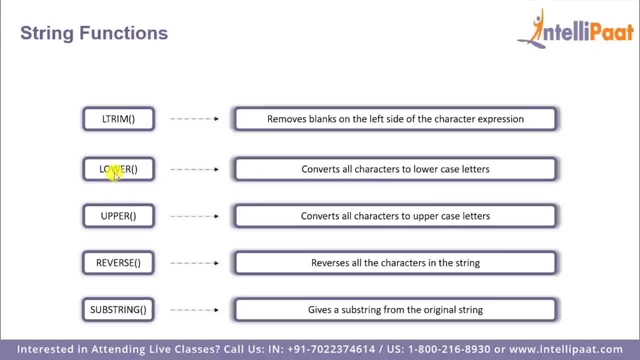 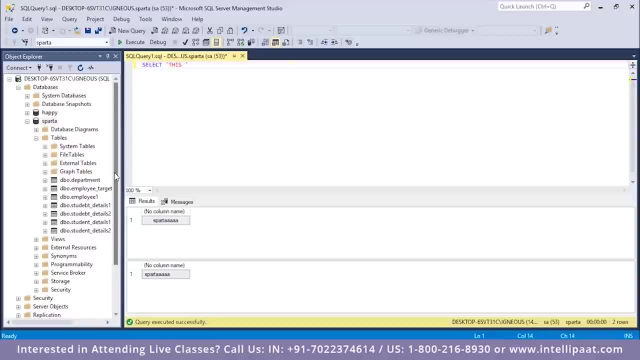 characters to the lower case. so let's look at an example. this time, let me actually print a string which has all the characters in capitals. so this is Pata. so here we see that all of the characters in the string are in capitals. I'll execute this and this is what we get now. if I want to convert all, 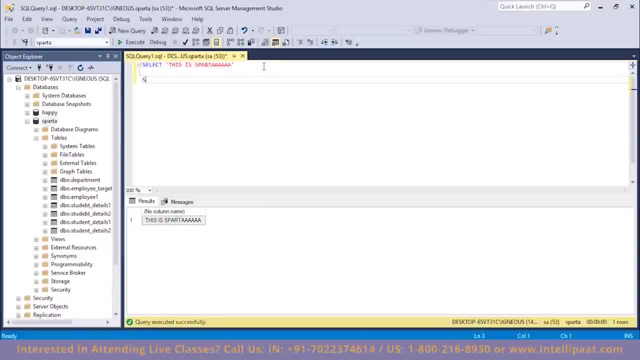 of the characters into lower case. I can just use a lower function, so I will type select lower and then pass in the string inside the function. I'll copy the string, I will paste it inside this. I'll hit execute. So this is the string where all the characters were in capitals and 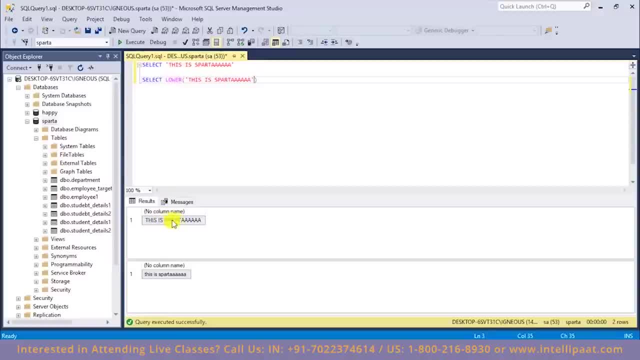 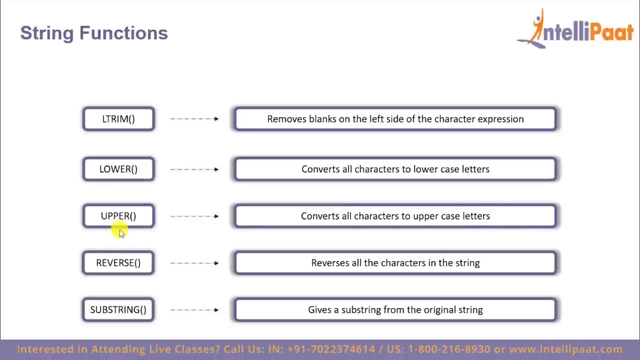 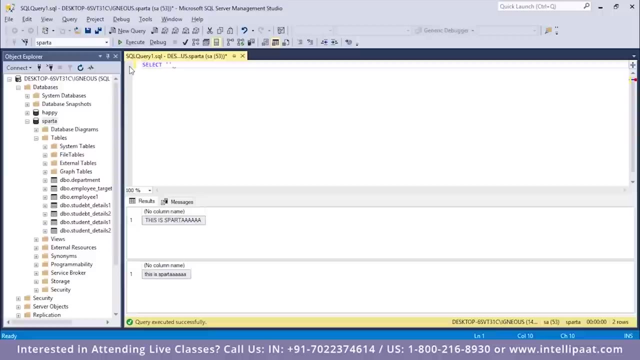 after using the lower function, this string, where all the characters were in capitals, have been turned to lowercase. Similarly, we have the upper function, which basically converts all the characters to uppercase. So this time I will take in a string which has all the characters in lowercase, So select. 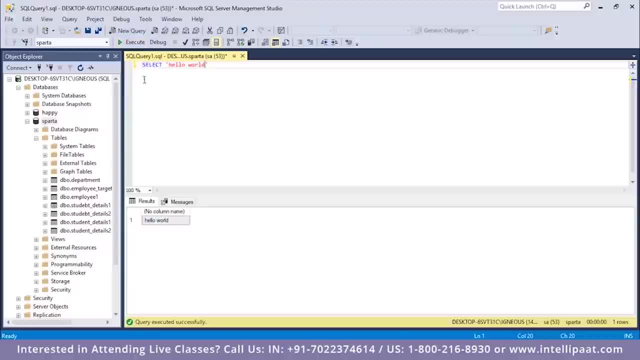 I will type hello world. Let me print this right. So here we see that initially, all of the characters are in lowercase. Now, after this, I will type select upper and then pass in the string inside the function. I'll copy this. I will paste it. 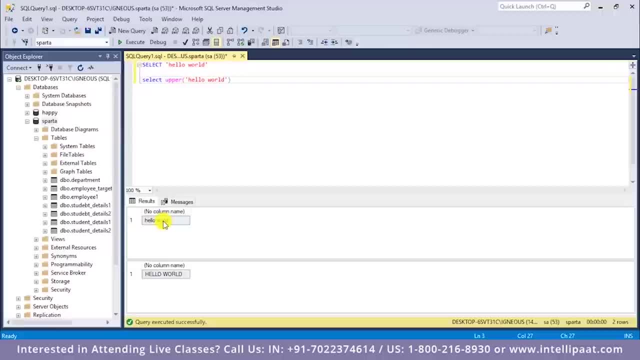 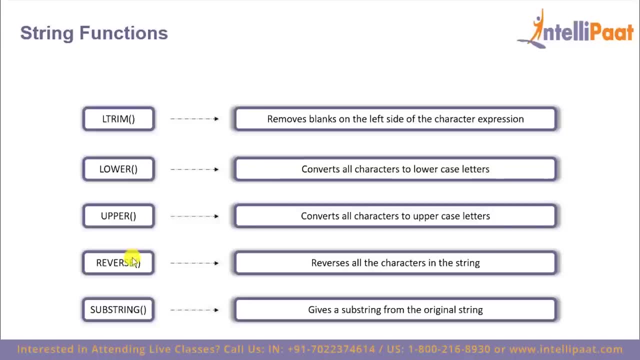 over here. I'll hit execute. So this was our initial string and after using the upper function, we have converted the string into capital case. After that we have the reverse function, which basically reverses all the characters. So this is the string where all the characters are in lowercase. 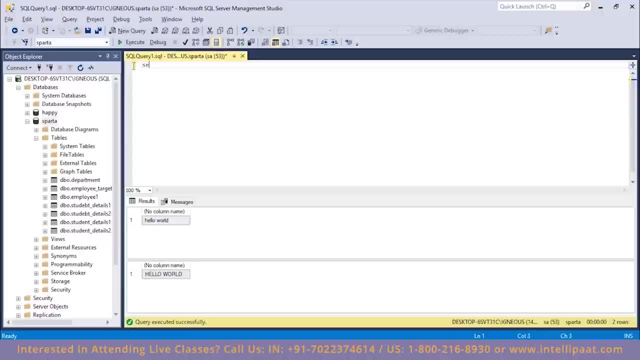 So let's implement this too. So let me take in a random string again Select, and I will type: I love ice cream. I'll hit execute. So this is what we get initially Now. after this, I will use the reverse function- Select, reverse and I 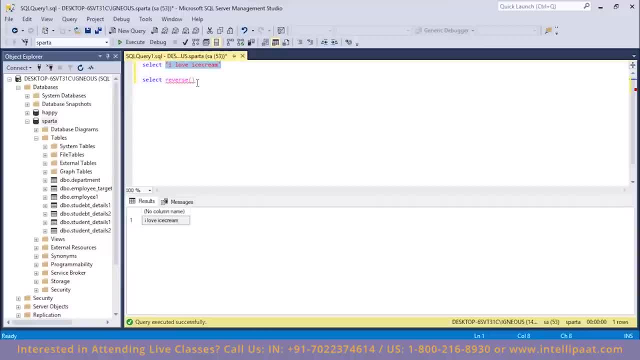 will pass in the string inside the reverse function. I'll copy it and I will paste it inside this function over here. Now let me execute. So this is the initial string and after using the reverse function, we have reversed all of the characters in the string, right? So you see that this is the 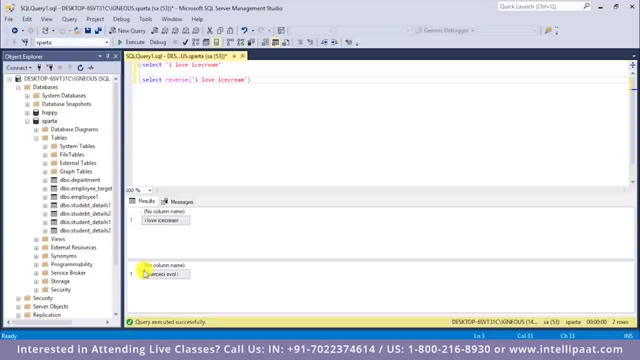 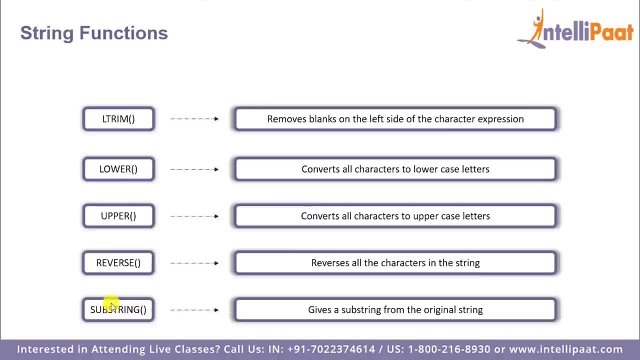 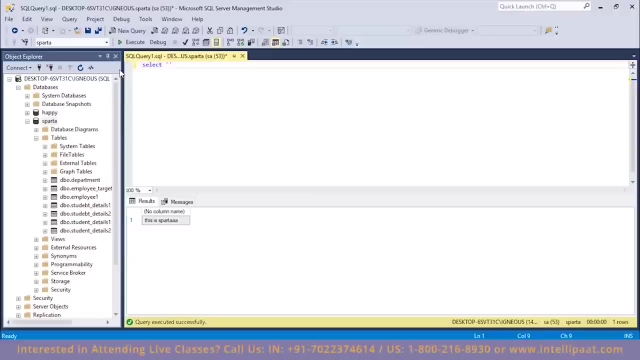 starting and this is the ending. over here, and after reversing it we get this final string and finally we have the substring function, which gives us a substring or part of the string from the original string. Now let me give in the original string first, So I will type select and then the string would be this: 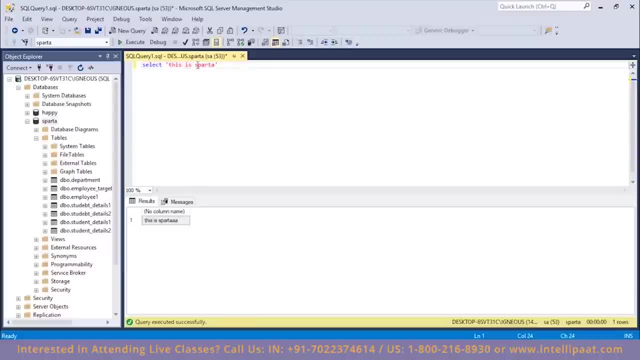 is part of the string. Now, let's say I would want the substring Sparta from this entire string. So this is where we can use the substring function. So I will type select substring. Now the substring function takes in three parameters. First, as the original string. 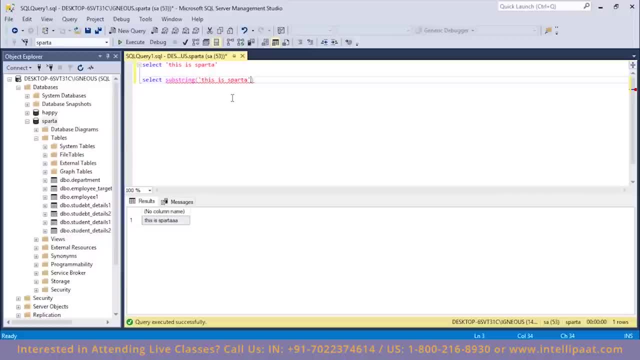 So I will copy the original string and I will pass it into this as the first parameter, and now, after that, I need to give in the index value from where the substring starts. So this is the first character of the substring which I want. So the index value would be 1,, 2,, 3,. 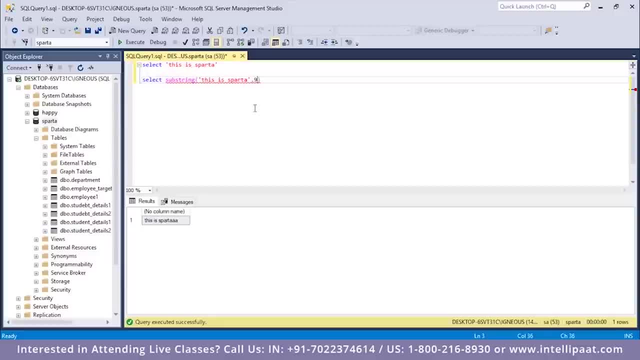 4,, 5,, 6,, 7,, 8 and 9.. So I'll type 9 over here, and then the third parameter would be the length of the substring. So the length of the substring is 1,, 2,, 3,, 4,, 5. 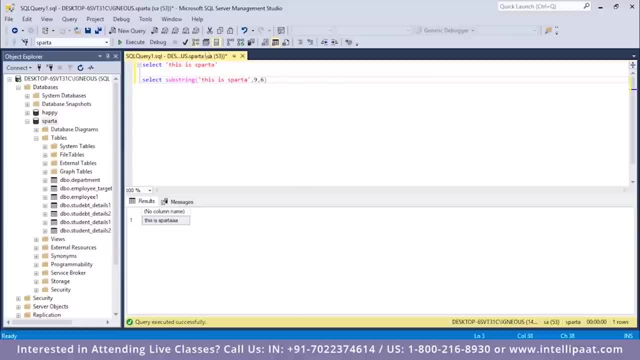 and 6.. So I will pass in 6 over here. Now let me execute all of these and let's see what do we get. So this is the original string, this is Sparta, and after using the substring function, we have extracted only this part from the. 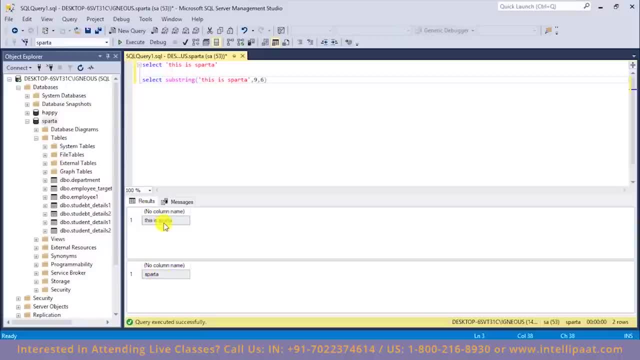 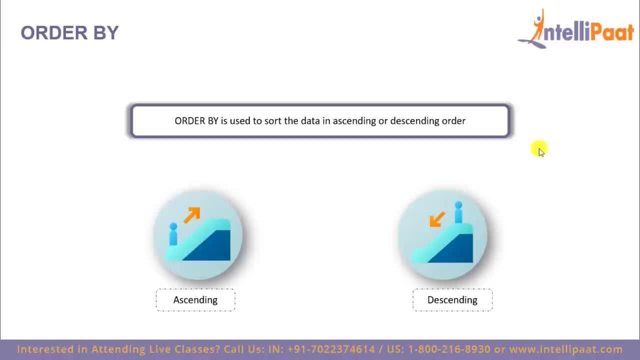 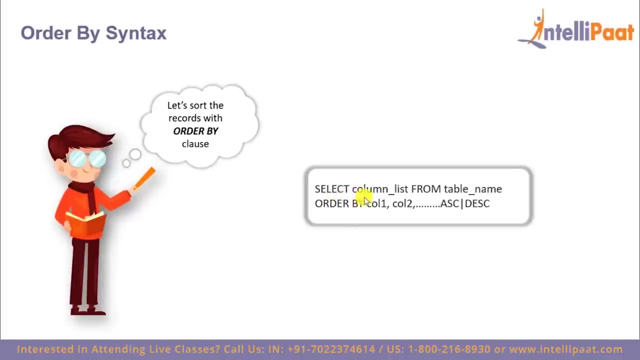 entire string. So these were some of the string functions in SQL Order by in the top clause. So order by is used to sort the data in ascending or descending order and, by default, order by sorts the records in ascending order. So let's have a look at the syntax. We'll start with select keyword and then given. 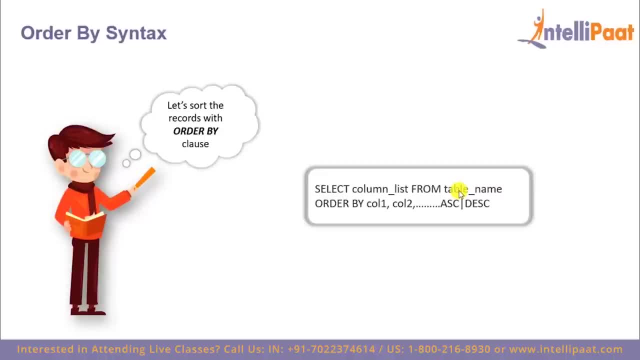 the column list, Then we'll use the from keyword and give the table name, Following which we'll type the keywords, order by and give the columns with respect to which you are to sort the data And, finally, we'll state whether the ordering should be in ascending or descending, and I've 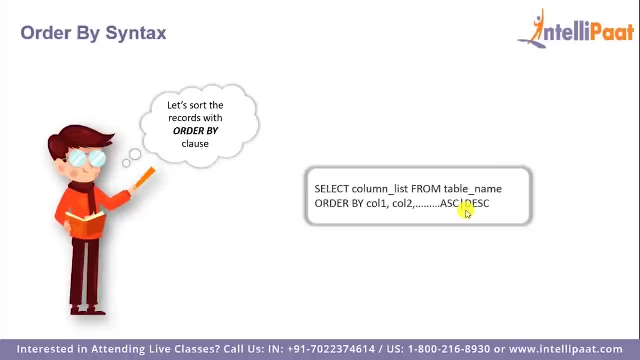 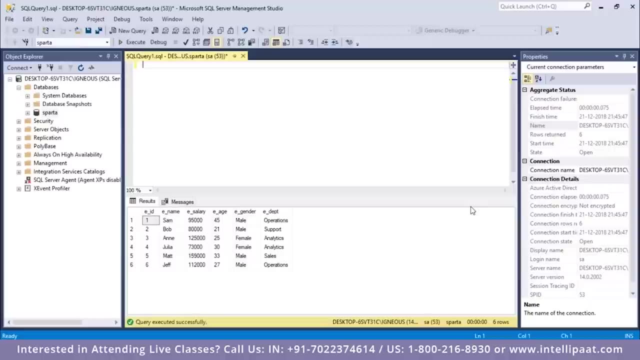 already told you guys that by default the sorting is done in ascending order and if you want the sorting to be done in descending order, we will use the DESC keyword. So I want to sort the table with respect to the salary column in ascending order. So this would be the command for that Select. start from the name of the. 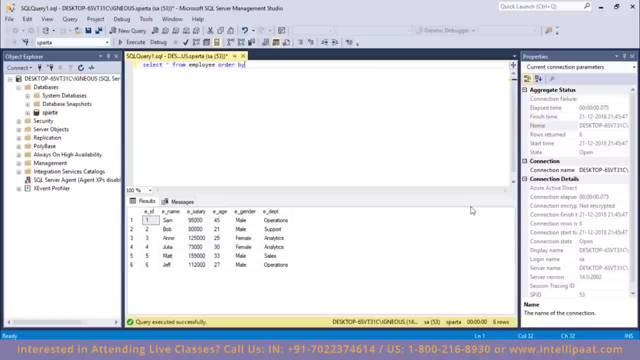 table as employee, After which I will use the keywords order by, and then given the name of the column, which would be salary, And since I want it with respect to ascending order, so I don't need to add anything else. So let me hit. execute Right. So we have successfully. 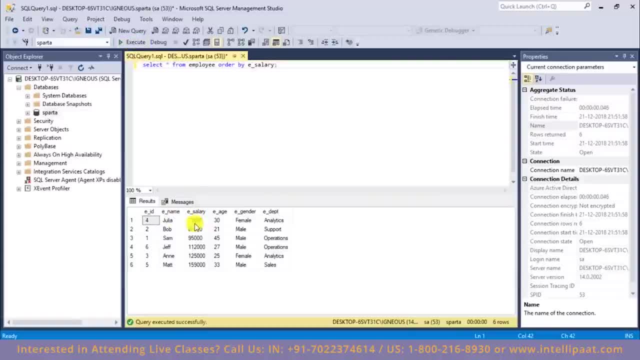 sorted this table in ascending order, right. So Julia has the lowest salary and Matt over here has the highest salary. So this is an ascending order: 73,000, 80,000, 95,000 and goes on till 159,000.. Now let's say I want to sort this table in descending order of the salary. 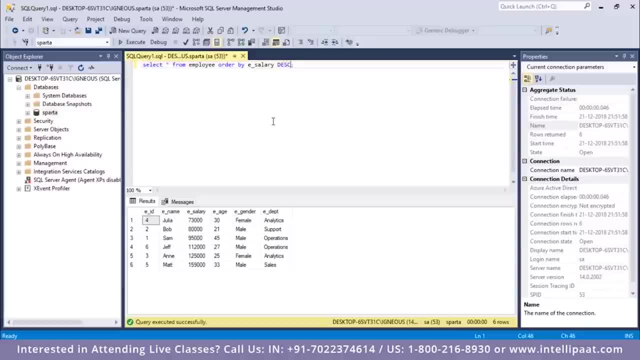 So for that all I need to do is add in the keyword DESC. Let me hit execute Right. So this time the table is sorted in descending order, Right. So over here, at the top we have the maximum salary, which is 159,000, and at the bottom we have the lowest salary, which 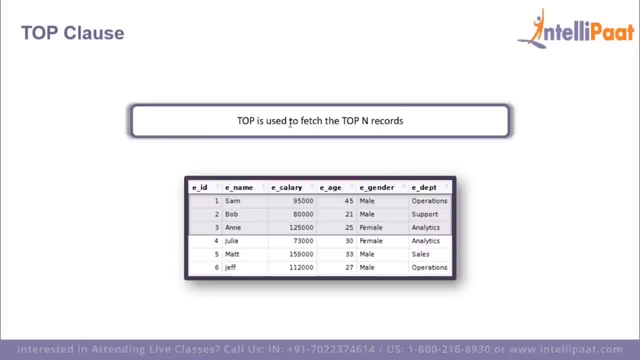 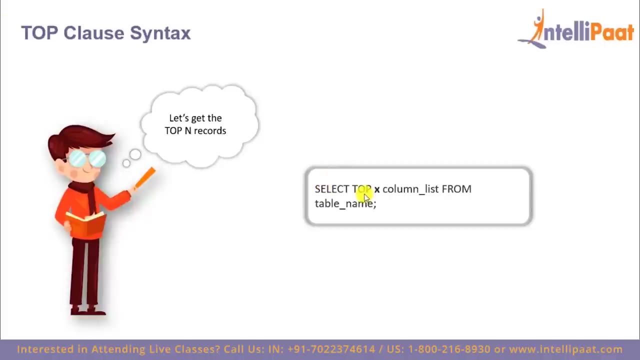 is 73,000.. Now let's look at the top clause. The top clause is used to fetch the top end records from a table. So top clause is useful on large tables with thousands of records. This is the syntax. We've got the select keyword first. Then we type in top and then the number. 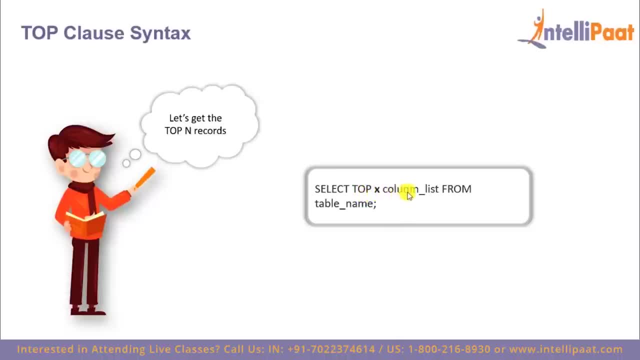 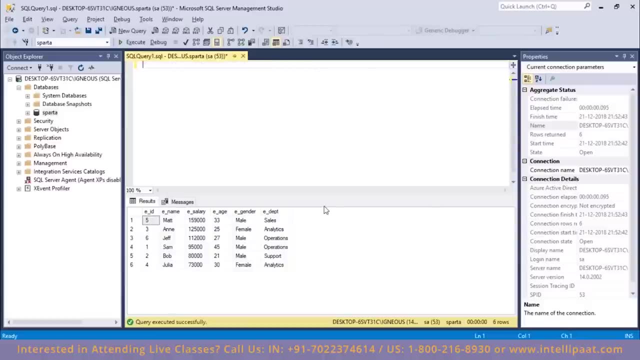 of records we want to see in our result, followed by the column list, And then we use the from keyword and given the name of the table. So I want to see only the top three records from the entire employee table. So this would be the command for that Select and then I will. 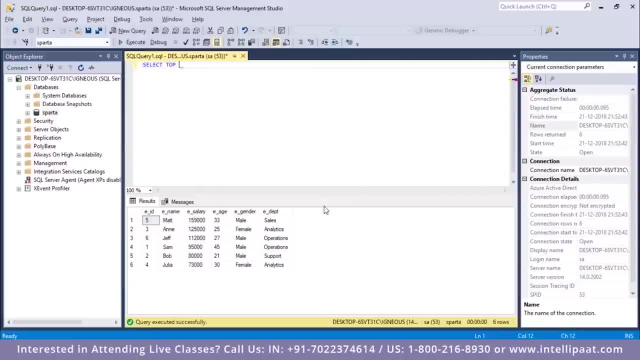 use the top keyword. And since I want three records, the number would be three. And since I want to see all of the columns, I will put in star over here. Then I want all of these records from the employee table. So this is the entire command: select top three star from employee. I'll hit execute Right. 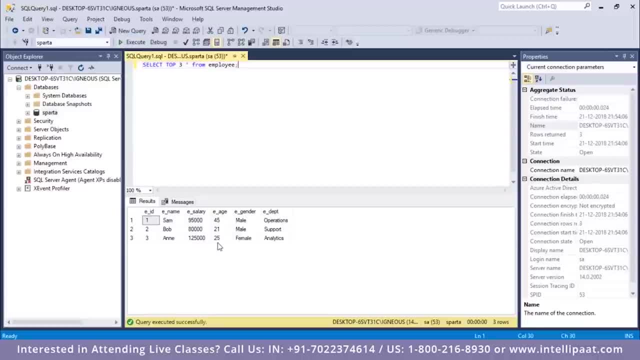 So I've got the top three records from the table. Now I will use the top clause and the order by clause and fetch the three oldest employees of this company. So let me write the command for that: Select top three records Star. So I've used the top clause to fetch the top three records. Now this would be from: 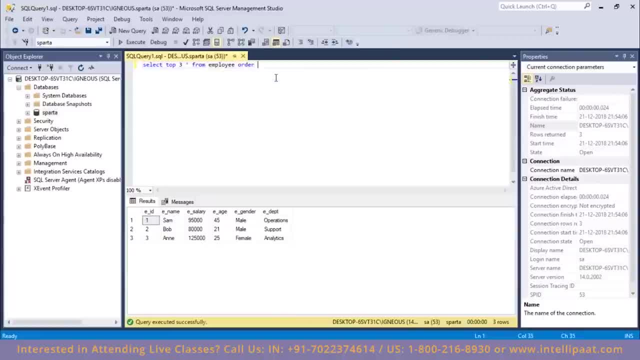 the employee table And then I will use the order by clause. So I want to order it with respect to the age of the employee And I want it in descending order, that is, the employee who has the maximum age should be at the top. Now let me hit execute. 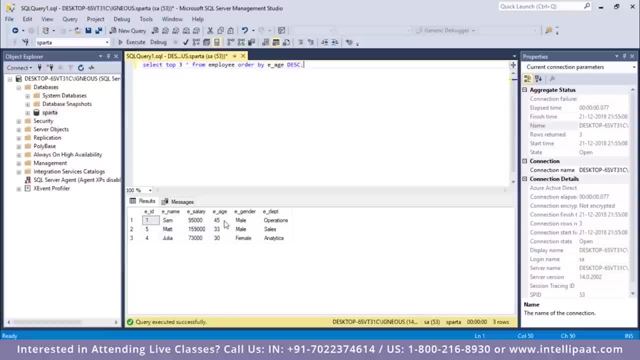 So I've got three records over here and the records are arranged in descending order of their age. So Sam has the highest age, 45, and Julia over here has the lowest age, 30, right? So Sam, Matt and Julia are the three senior, most employees of this company. And this is how we can work. 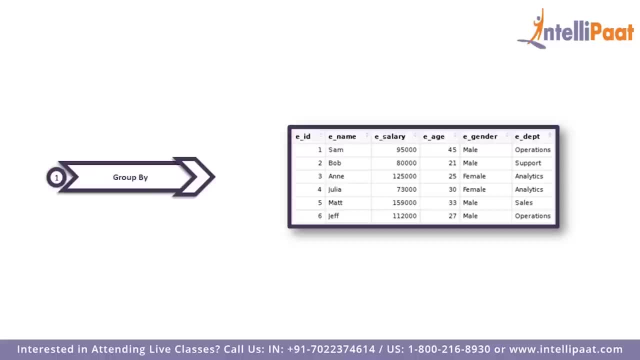 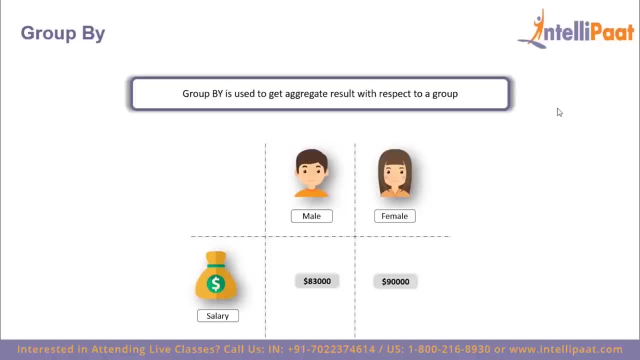 with the order by clause and the top clause With the group by statement. the group by statement does used to get aggregate result with respect to a group. For example, let's say we wanted to find out the average salary with respect to gender, that is, average salary of male employees separately and average salary. 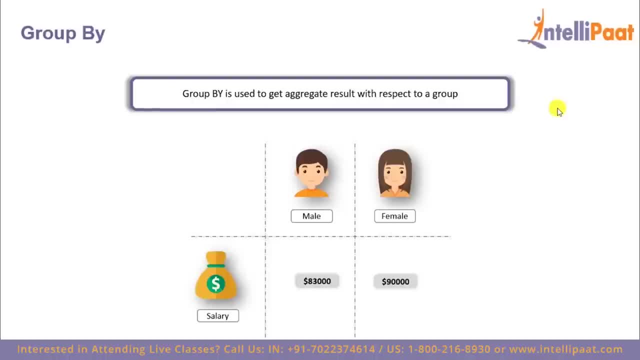 of female employees separately. And the average salary of male employees separately. and average salary of male employees separately. And the average salary of male employees separately and average salary of female employees separately. This is where we can use group by to divide the data into two groups- male and female- and find out the average salary of each group. 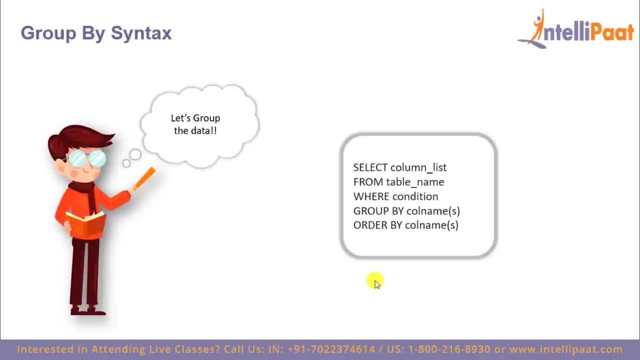 separately. Now let's have a look at the syntax. So here you'd have to be careful of the sequence. So the group by clause follows the where clause and receipts the order by clause. So if you mix up the sequence then you may not get the right result. 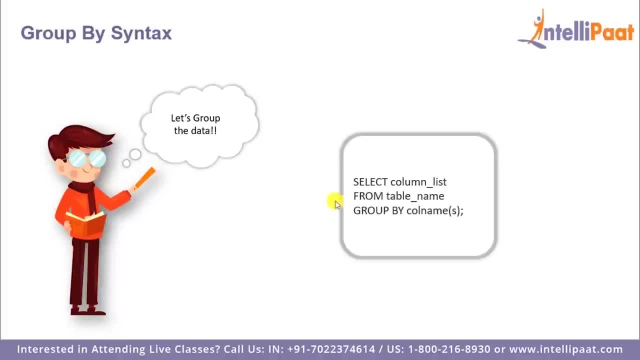 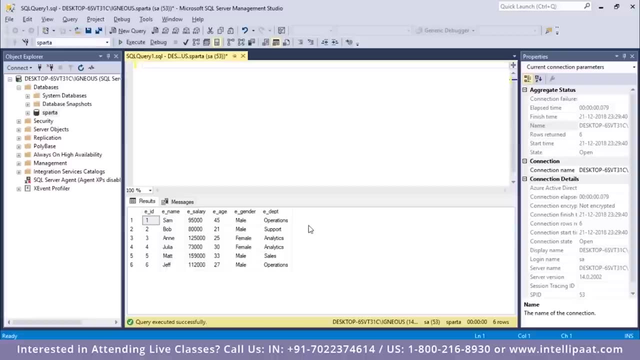 And if you're not using the where clause and the order by clause, you can directly follow up the group by statement after the table name. So I would want the average salary with respect to the gender. So this would be the syntax for that select. And since I want, 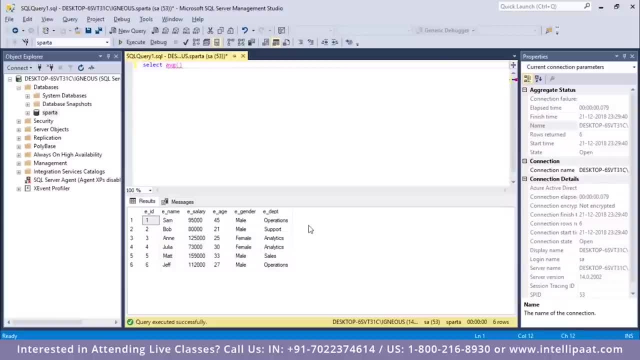 average salary, I will use the AVG aggregate function and then given the name of the column, which would be e salary, And since I also want to see the gender column, I will given each gender over here. And this is from the employee table. And since I have already given 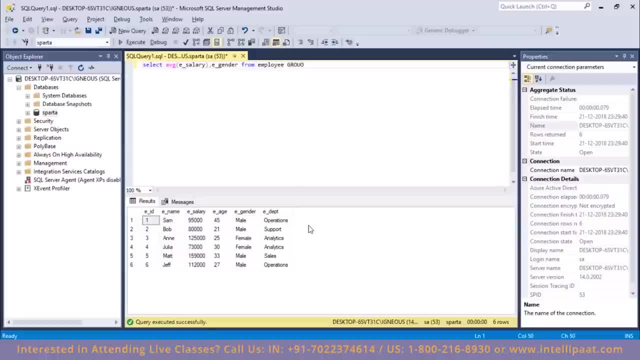 the name of the table. I can use the group by statement over here And after the group by statement, I need to give him the column with respect to which I have to group the data And I want to group the data with respect to the gender column. So this would be my total command. 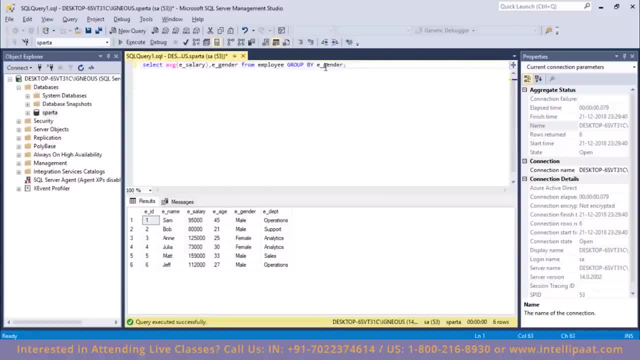 select average of E salary and E gender from employee group by E gender. So let me hit, execute Right. So this is the average salary with respect to the female employees And this is the average salary with respect to the male employees. So the average salary of female employees is around. 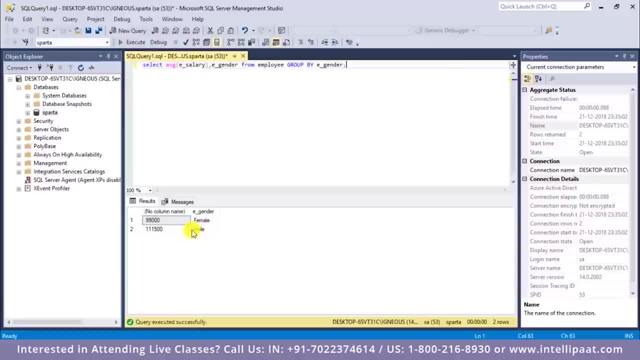 $99,000 per annum, And average salary of male employees is around $111,000 per annum. Now I want the average age with respect to the department, And I'll also use the order by keyword to sort the data in descending order with respect to the average age. So this is the syntax select Since. 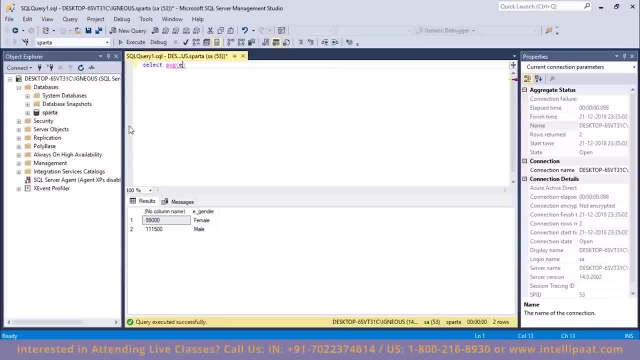 I want average age. I will use the average aggregate function and then pass in the column, which would be E age, And I would also want to have a glance at the departments E, D, E, P, D. I will give in the name of the table, which would be employee, After which I will give in the group by statement. 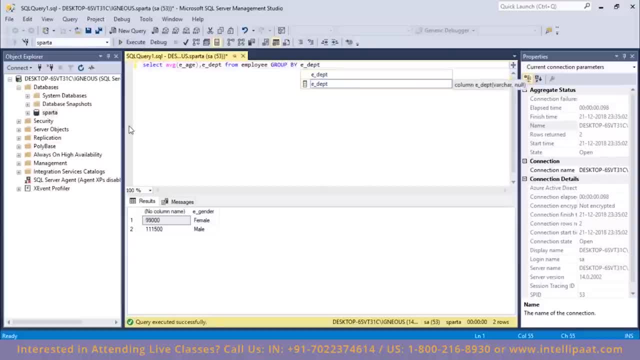 and I want to group this with respect to the department, So group by: E, D, E, P, D, And after the group by statement. I need to give the order by statement, So order by, and I want to order the result with respect to the average age. 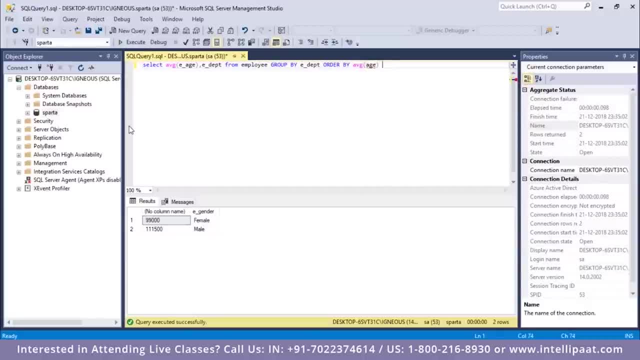 So again, this would be average age And I want the sorting to be in descending order. So D, E, S, C. So this is a total command, Select average E age in E department. So I'll be getting the average age. 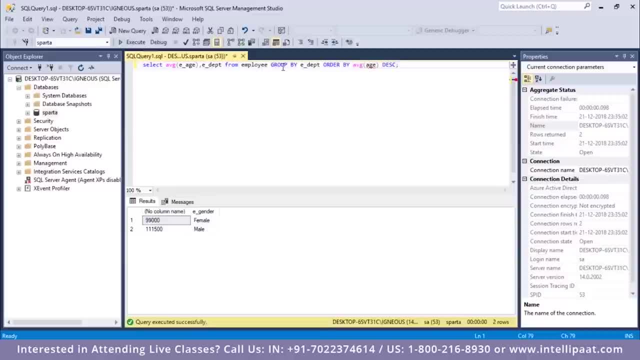 and the department column from the employee table And I'm grouping it with respect to the department column And I'm sorting it in descending order of the age. So this would be E age over here. So let me hit execute. We have the average age with respect to each department, ordered in descending order. So operations. 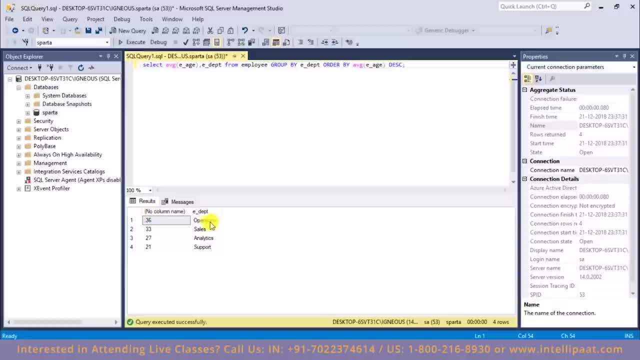 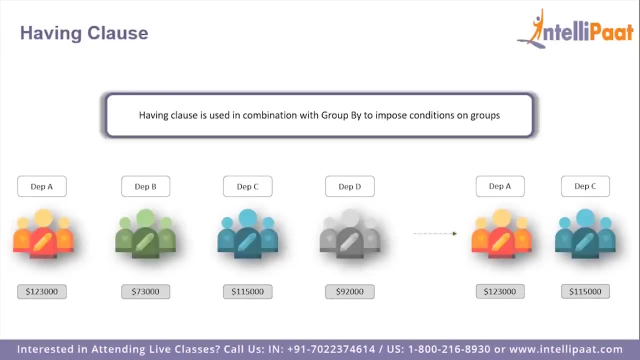 department has the maximum average age of 36.. Then sales has an average age of 33.. Analytics department has an average age of 27 and support has the youngest staff of age 21.. And this is how we can use a group by clause. The having clause is used in conjunction with the group by statement to. 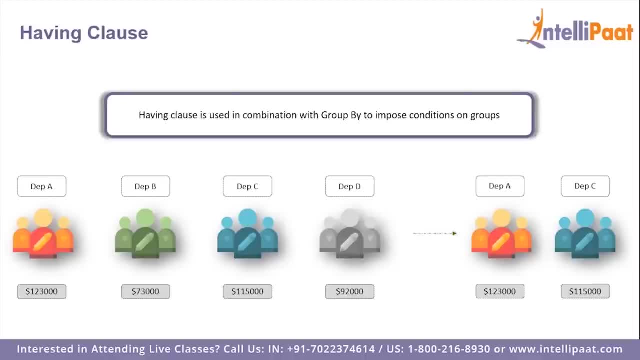 impose certain conditions on the groups which are to be displayed. So the having clause was added to SQL, because the where keyword could not be used with aggregate functions. For example, over here we have four departments, A, B, C and D, And we also have the corresponding average salary of the employees. 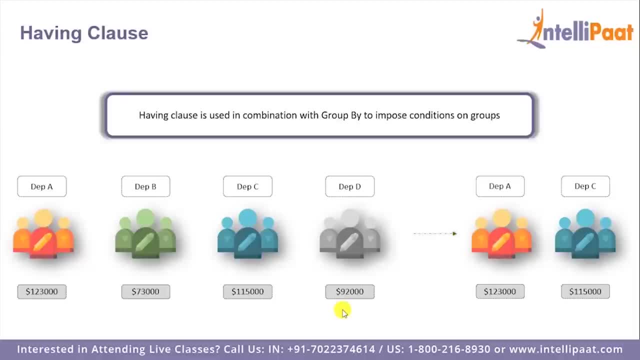 belonging to each department. Now, let's say we wanted to see only those departments where the average salary is greater than $100,000.. So this is where having clause can be used to impose the condition and get only those departments where the average salary is greater than $100,000. 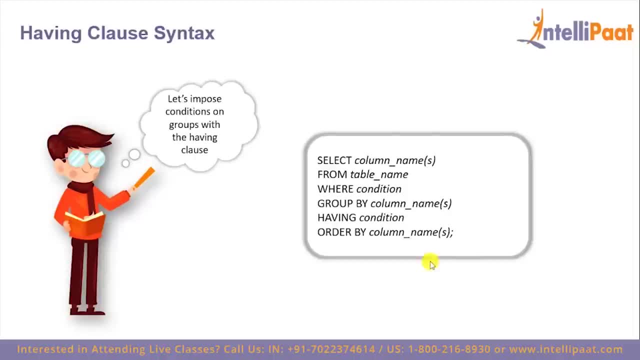 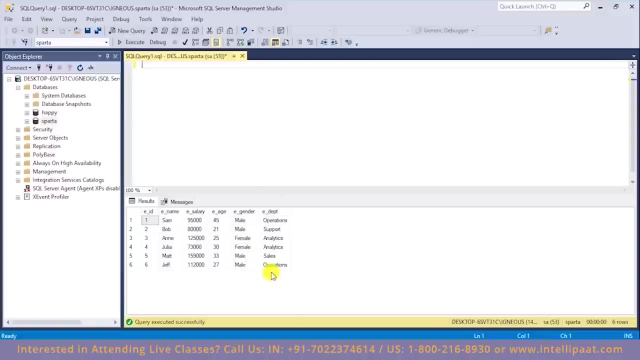 And this is the syntax for the having clause. Here you need to keep in mind that the having clause must follow the group by clause and must also precede the order by clause, if use. So let's go to SQL server and implement the having clause, So we'll group this table with respect to the 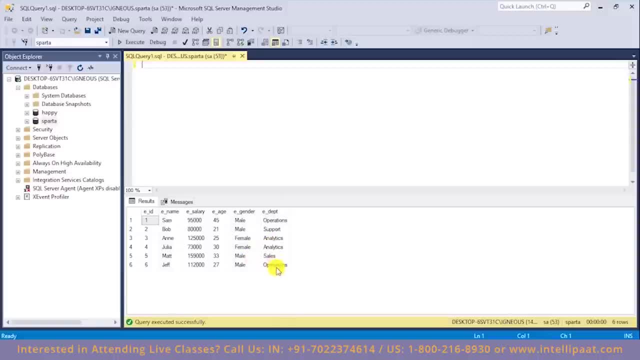 department column and then use the having clause to display only those departments where the average salary is greater than hundred thousand dollars. So let me go ahead and write the syntax for the having clause. I will type in the select keyword and then list down all of the columns which I want. 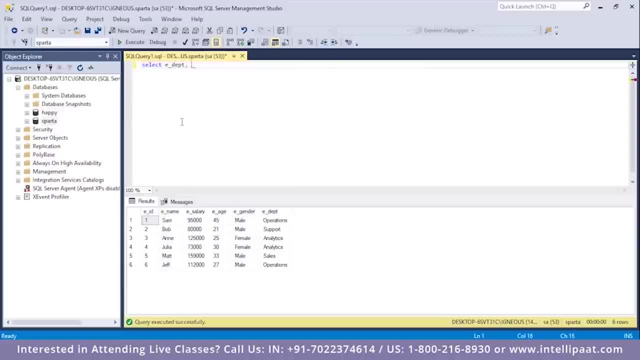 from this employee table, So I need the department column. I would also need the average salary, So I'll use the aggregate function AVG and then pass in the column which is e salary And I will name this column as average salary. Now I would want this from the employee table, So I'll use the. 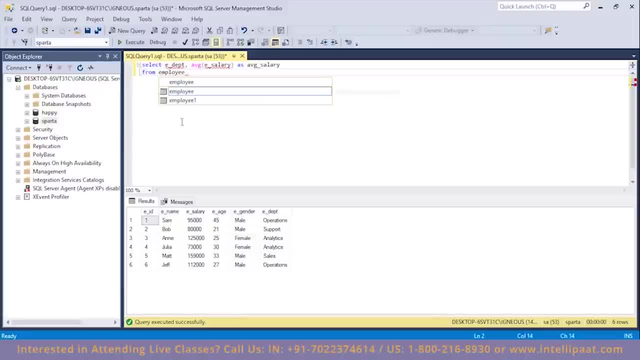 from keyword and then give the name of the table which is employee. After this I'll give the group by keyword to group this table with respect to the department column. So I will give in the name of the column which is E, D, E, P, T. Now, before I go ahead and use the having clause, let me actually 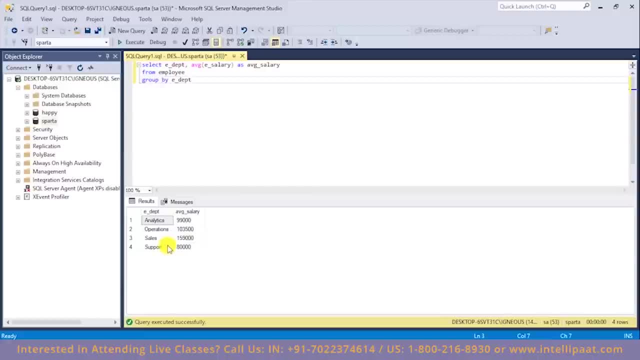 execute just these three lines of code, Right? So what I've basically done is I have grouped this employee table with respect to the department column And we have the average salary with respect to each of these departments, right? So this is the average salary of analytics. 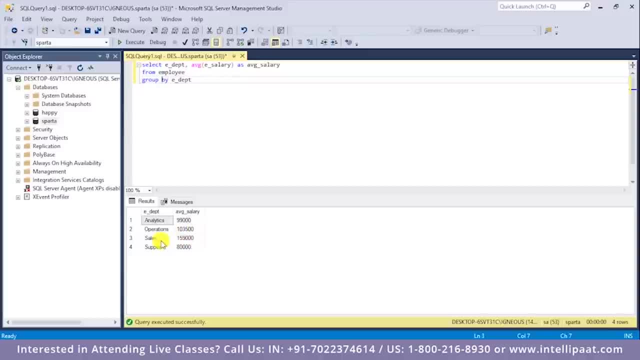 department, average salary of operations department and average salary of employees department. Now I will use the having clause to display only those records where the average salary is greater than $100,000.. So the average salary needs to be greater than $100,000.. Now I'll select all of this. 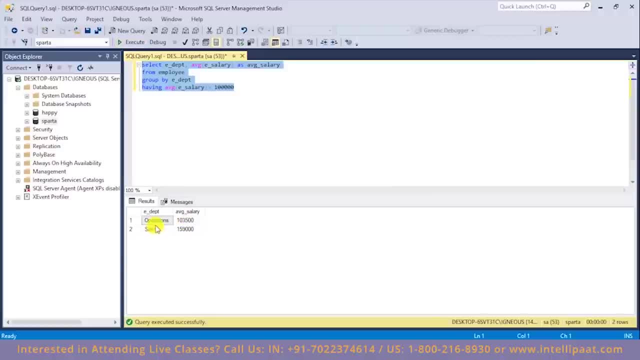 I'll hit Execute right. So we see that out of the four departments, only operations and sales department have the average salary of the employees to be greater than $100,000.. So the The average salary of employees in operations department is $103,000 and the average salary 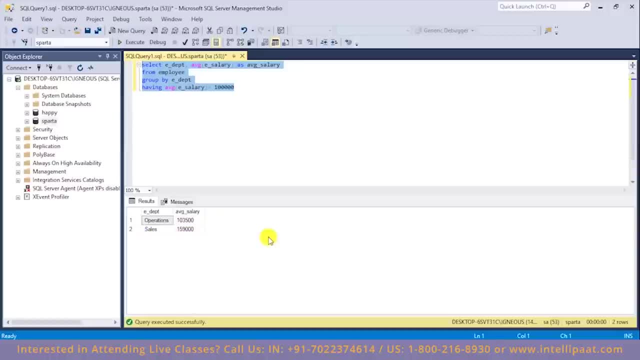 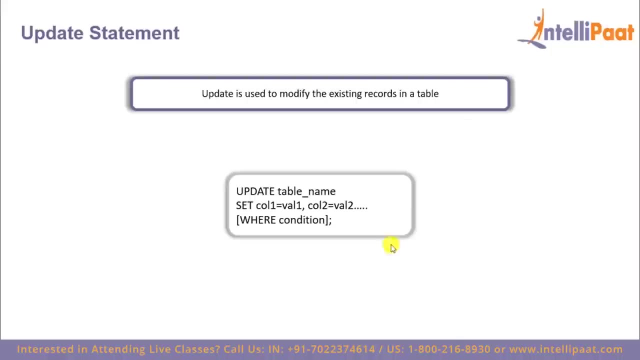 in the sales department is $159,000.. This is how we can work with the halving clause in SQL. So the update statement is used to modify or change the existing records in a table, And this is the syntax for the update statement. 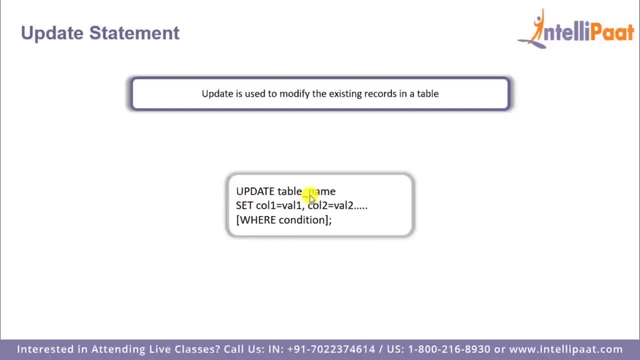 So we'll start with the update keyword and then given the name of the table, Then we'll use the set keyword and assign new values to the columns which you want to update. We'll use the where clause to give in the condition which should determine where the 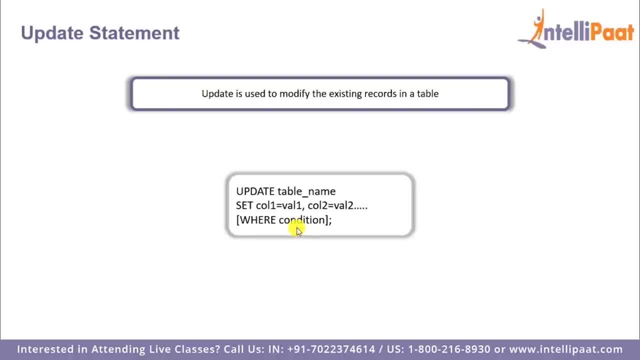 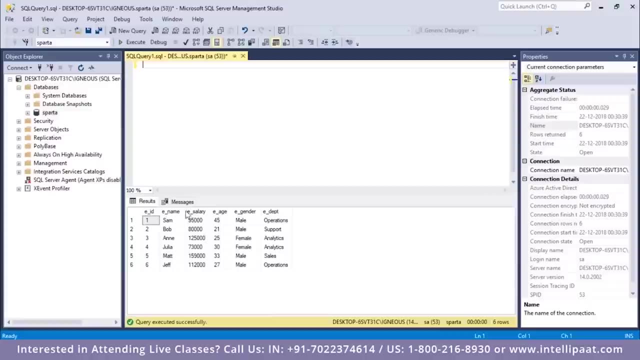 columns are to be updated. So why we are putting the where clause over here in square brackets? because it is optional. Now let's update some records of our employee table. So this is our employee table and I want to set this age value to 42, where the name equals. 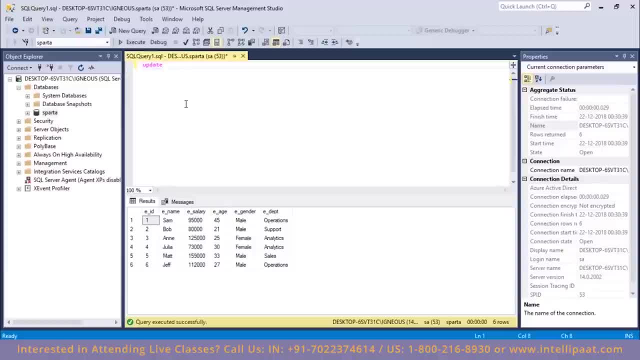 Sam, So this would be the command for that. So I will give in the update keyword and then, given the name of the table, which would be employee, and then use the set keyword And then set the age value- I want the value to be equal to 42- then use the where clause and then set the condition. 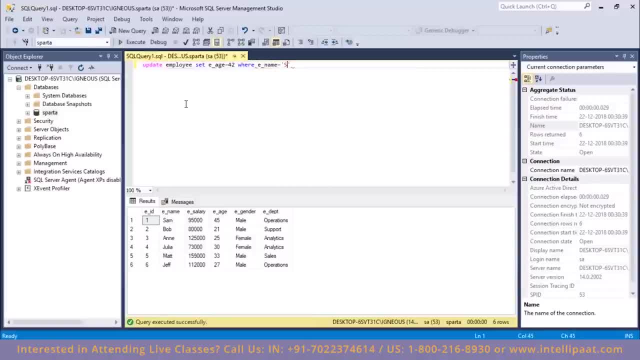 So the condition is the name should be equal to Sam. So where the name is equal to Sam, I am updating the value of age from 45 to 42.. Let me put a semicolon, Let me hit execute So you see that one row has been affected. 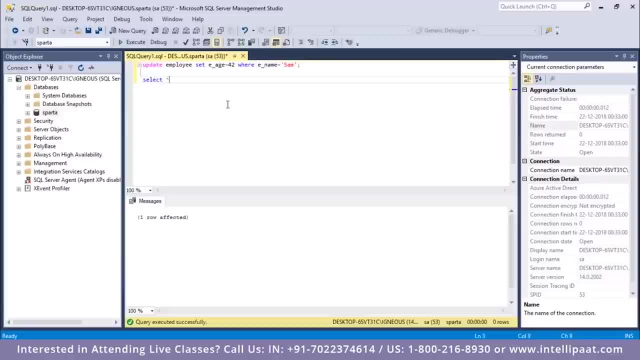 So now let me have a glance at the change table, Select star from Employee Right. So we see that initially the age value was 45, where the name was Sam. So the age value has been changed from 45 to 42.. 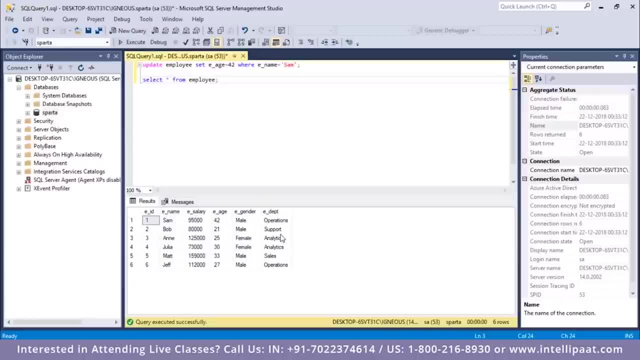 Now, similarly, I don't want to change the department to tech wherever the gender value is female, That is, I want to change the department of all of the female employees from analytics to tech. So this is how I can do it Again: update keyword and then I'll give in the name of the table. 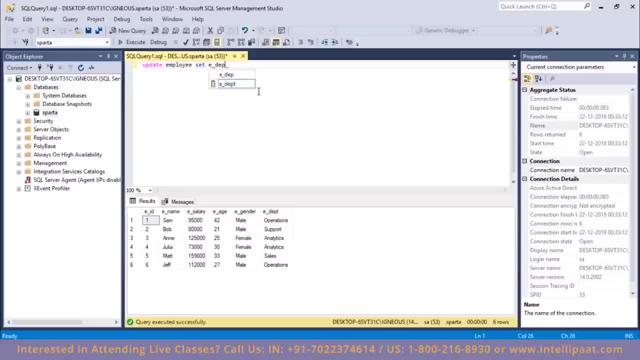 And then the set keyword. So over here I want to set the department to be equal to tech, where the gender is equal to female. So let me put in female over here, Right? So let me hit execute now and let's see what happens. 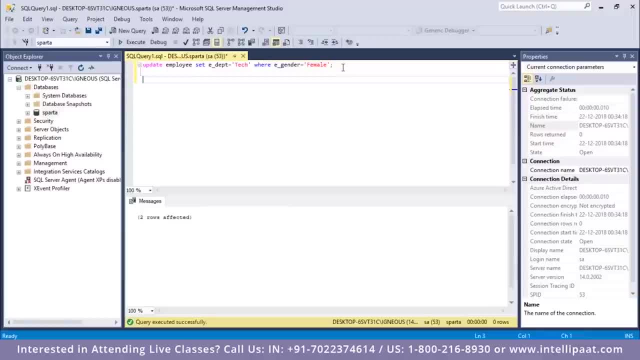 So we see that two rows have been affected. Now again, let me have a glance at the modified table. Select star from Name of the table is employee Right. So we see that initially the department of both of the female employees was analytics. 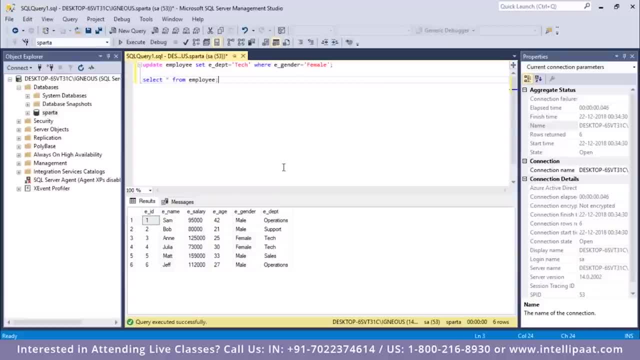 So that department has been changed from analytics to tech. Now I want all of the employees to have the same salary, So I will update this entire column to have the same value, which is $50,000.. So this command would be quite simple. 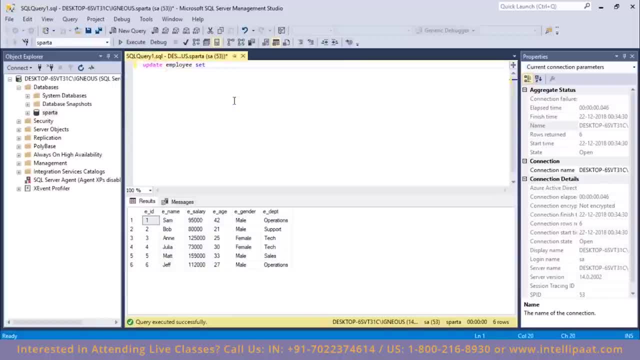 Update And then the name of the table, which is employee, And then I'd have to set the salary to be equal to $50,000.. That's it, Let me hit execute. So we see that six rows have been affected. 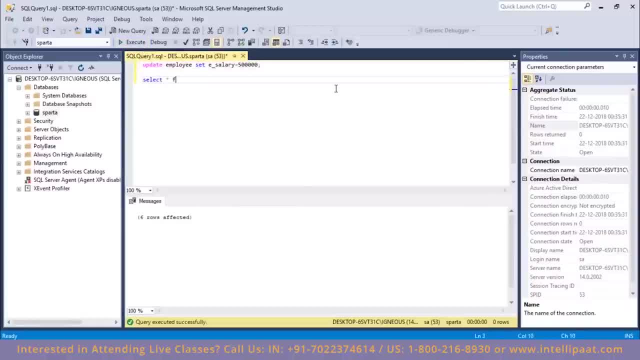 Again, let me have a glance at the modified table. Select star from The name of the table is employee Execute- again Right. So we see that the salary has been Right. So we see that the salary has been updated. So every employee's salary is same. 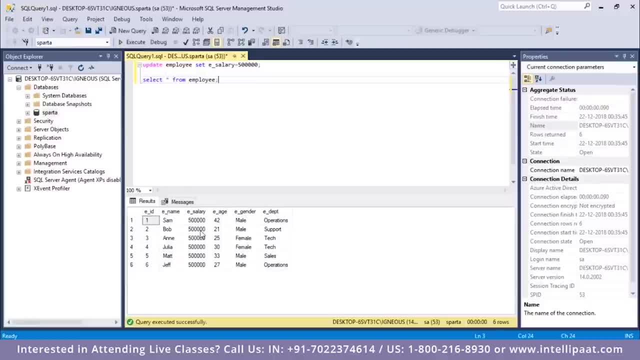 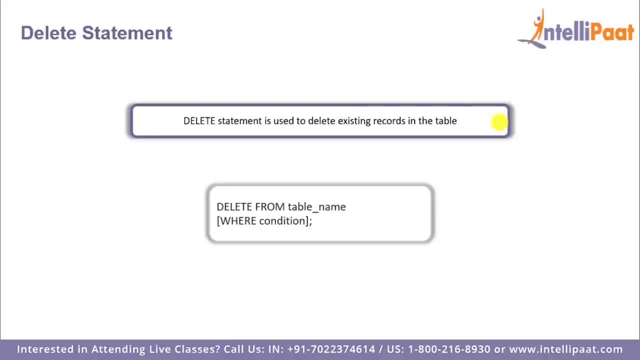 It is $50,000 per annum And this is how we can work with the update state. So the delete query is basically used to delete or remove one or more existing records in the table. So let's have a look at the syntax. 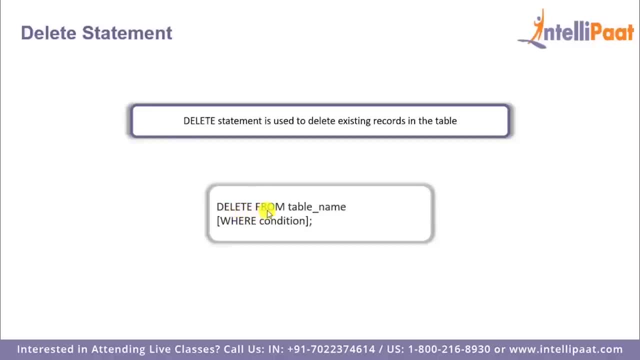 We'll start with the delete keyword and then put in the keyword. from Then we specify the name of a table. After that we'll specify the where condition, But that's optional. Now let's delete some records from our employee table. So we have our employee table right here. 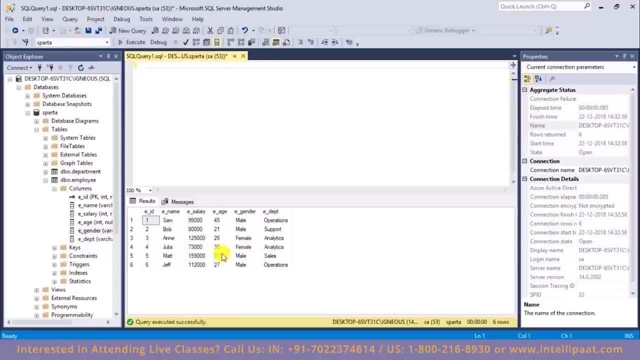 And I'd want to delete that record where the age of the employee is equal to 33.. So this would be the command for that. I will give in the delete keyword And then I'll type from And give in the name of the table which would be employee. 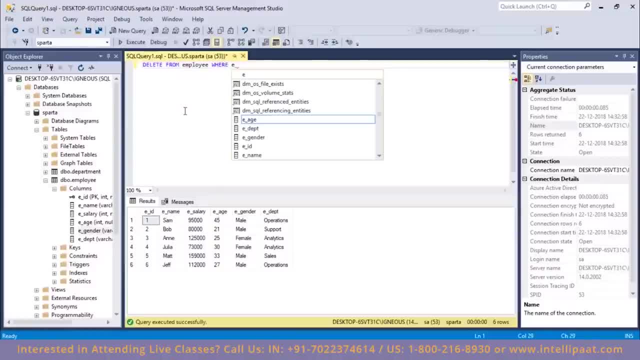 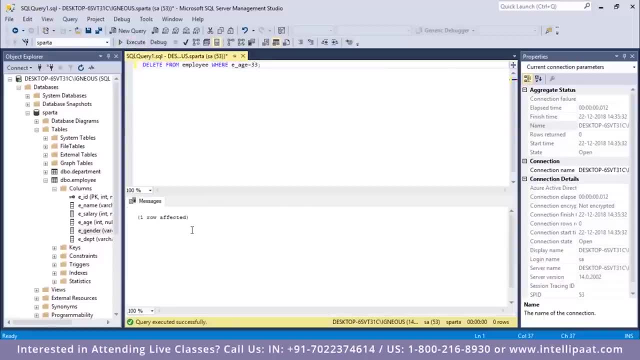 After that I'll use the where clause and give the condition. So the condition would be: eh is equal to 33.. I'll put in a semicolon over here and I'll hit execute. So you see that one row has been affected. 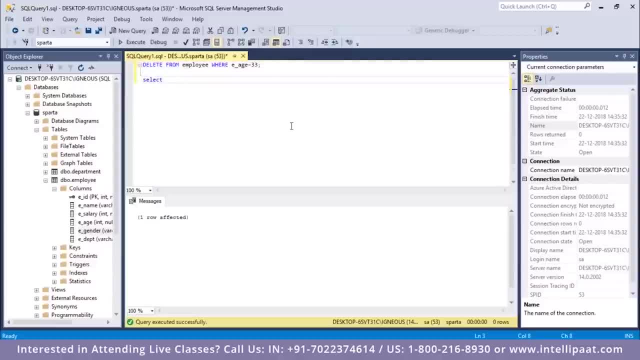 Now let me have a glance at the modified table. So I will type in select star from employee Execute again. So you see that that record where the age was equal to 33 has been removed. So initially we had six records. Now we only have five records in our table. 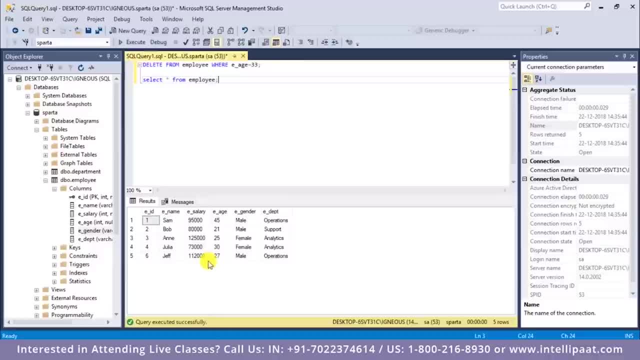 Now, similarly, I'd want to delete that record where the employee name is equal to Sam. So let me write the command for that. So I will give in the delete keyword first And then I'll give in the from keyword. After that I'll give the name of the table employee. 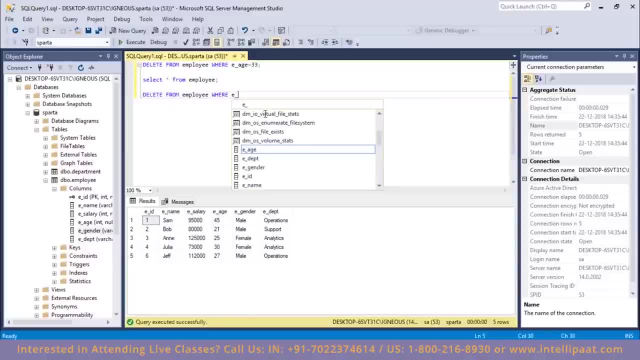 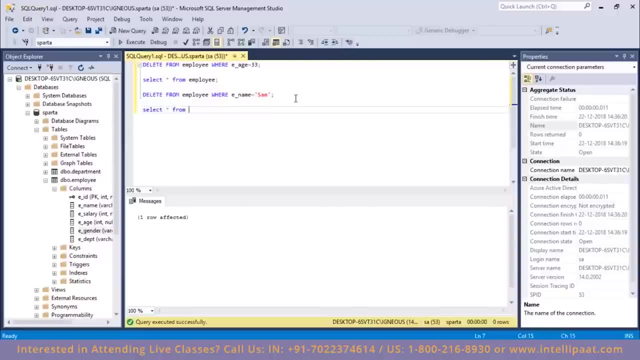 Then use the where clause and then give the condition. So this time the condition would be: ename is equal to Sam Right Execute. Again, we have one row which has been affected. Select star from employee. And let's see the modified table now. 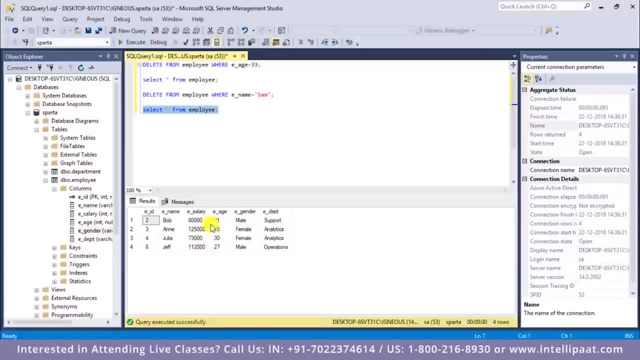 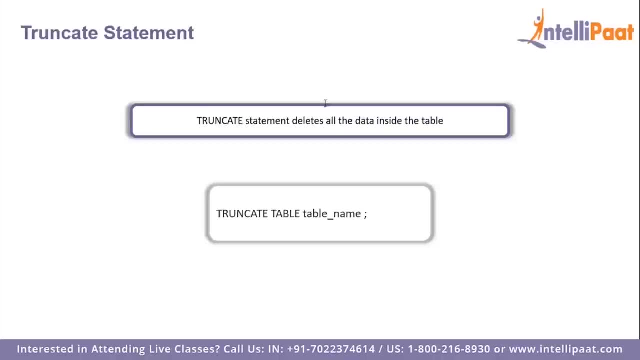 So see that another record has been deleted And that record where the name was equal to Sam is the record which has been deleted. Then we have the truncate statement. So the truncate statement deletes all of the data inside the table. So here we'll give in the keywords truncate, table and then give the name of the table. 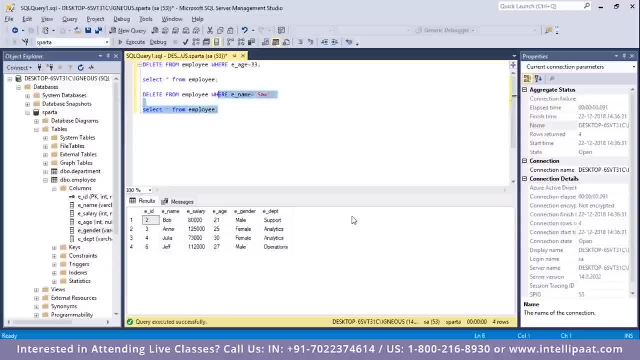 So let me go ahead and remove all of the records from this employee table using the truncate command. So I'll type truncate table And then I'll give in the name of the table which is employee Execute. So see that commands completed successfully. 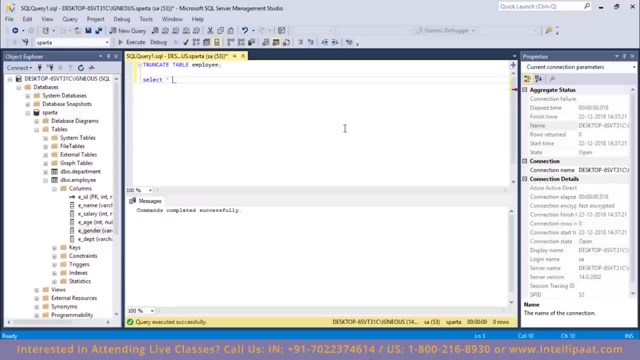 Now I will type select star from employee. Now let's see what do we get. So we see that all of the records are empty. This is because the truncate table command basically removes all of the data from the table. And the specialty of the truncate command is, even though it removes all of the records from the table, 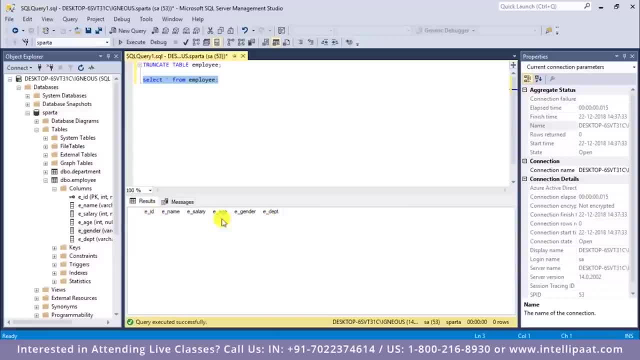 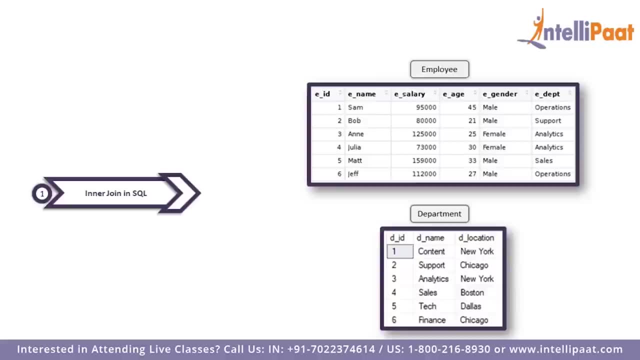 the structure of the table remains intact. So we see that the structure of this table over here employee table it is still intact. So this is how we can work with the delete and truncate statements: How to implement the inner join. We'll be implementing the inner join on these two tables. 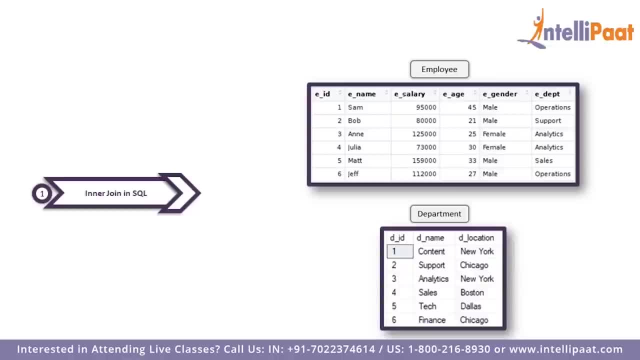 First is the employee table, which comprises of employee ID, employee name, employee salary, age and gender and the department in which the employee works. Then we have the department table, which comprises of department ID, department name and the location where the department is located. 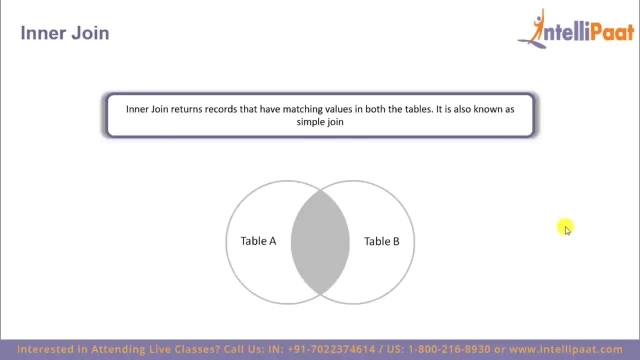 So the inner join basically gives us those records that have matching values in both the tables. So let's say we have two tables, table A and table B, And when we apply inner join on these two tables we'll get only those records which are common to both table A and table B. 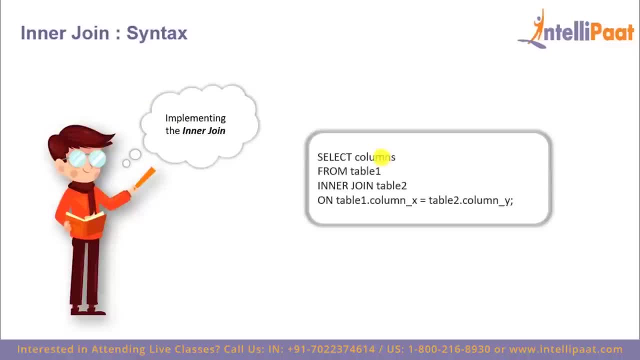 So let's have a look at the syntax. We'll give the select keyword first and then the list of the columns, Following which we'll give the from keyword and give the name of the first table. Now let's see what happens. Then we'll use the keywords inner, join and give the name of the second table. 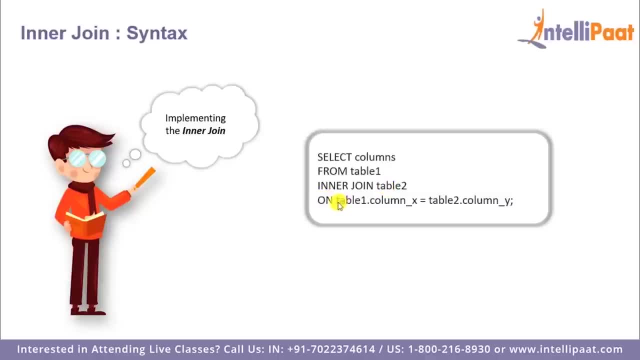 After which we'll use the on keyword. So this on keyword tells SQL that this inner join needs to be done on some condition, And that condition would be: values from column X of table 1 should be equal to the values of column Y from the table 2.. 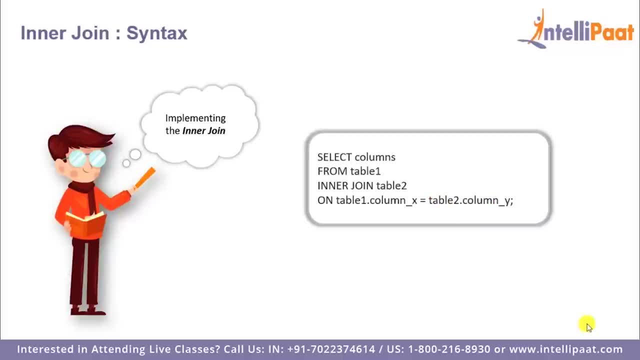 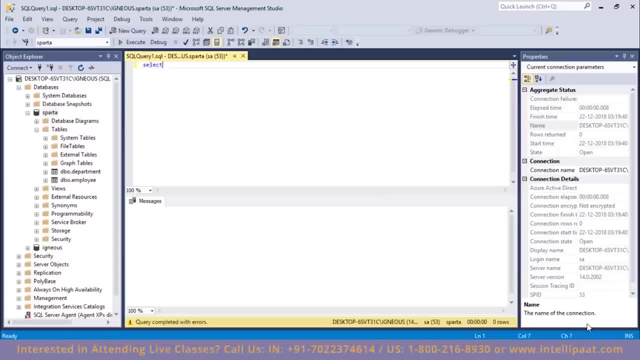 Now this might sound complicated, so let's just implement this inner join on the employee table and the department table. So before I go ahead and implement the inner join, let me have a glance at both of the tables. So I'll start with the employee table. 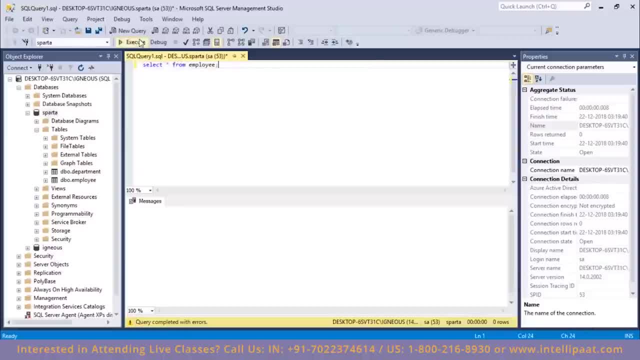 Select star from employee Right. so this is our employee table. So we see that we have this department column over here which tells us about all the departments in which the employees work in. Now, similarly, let me have a glance at the department table. 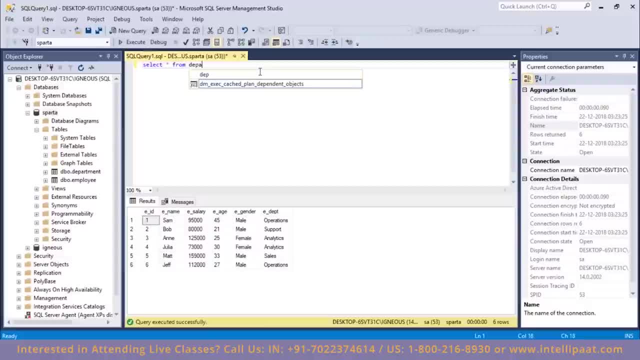 Select star from. I've given the name of the table, which would be department Right. So we have three columns over here And I have this dname column over here which gives me all of the names of the departments. So this is the common column between the employee table and the department table. 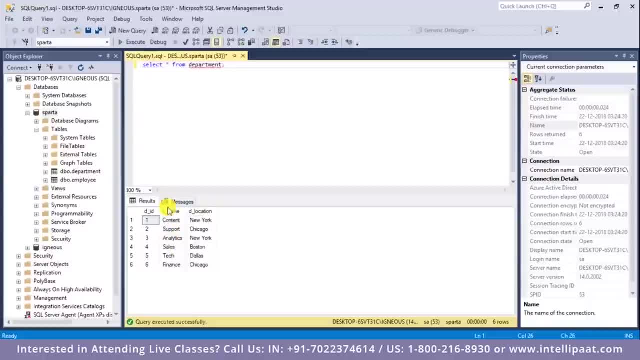 So we'll be applying the inner join condition on the dname column of the department table and the edept column of the employee table. So let me go ahead with the syntax of inner join. I will give in the select keyword and then give in all of the columns which I do want to select. 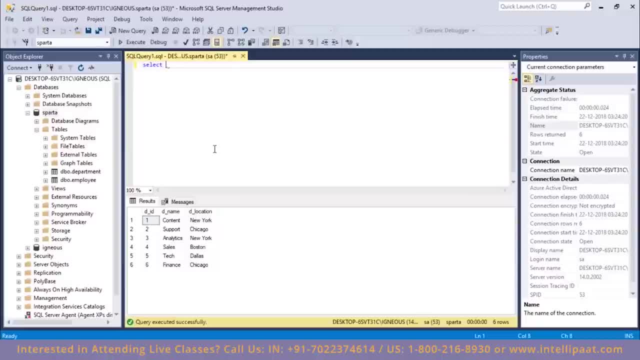 So I want to select the ename column and edept column from the employee table. So first I would have to give in the name of the table which is employee, Then I'll put dot over here and then give in the name of the column. 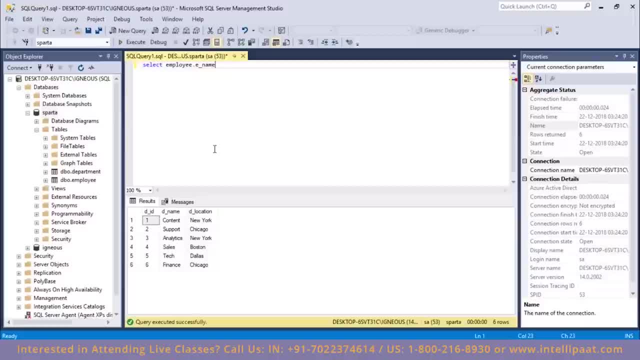 So I want the name column from the employee table And similarly I'd also want the department column from the employee table. First I will give in the name of the table, I'll put in dot over here and then give in the name of the column which is edept. 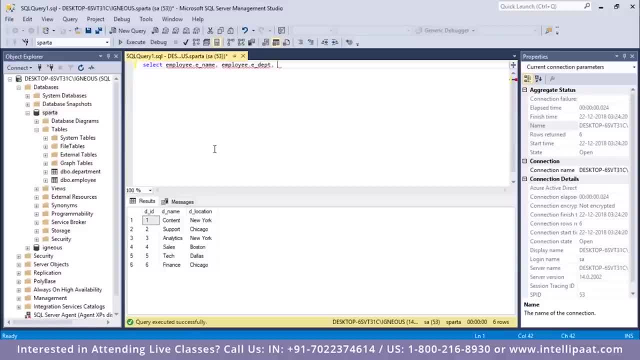 Right Now I'd also want the department name column and the department location column from the department table. So first I will give in the name of the table, which is department. I'll put in dot over here and then give the name of the column which is dname. 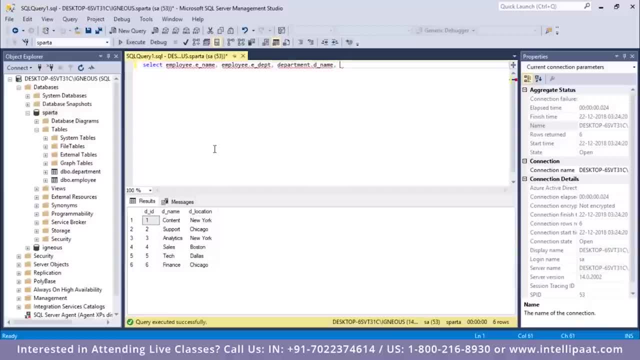 Similarly, I'd want to extract the department location column from the department table. First I will give in department over here, which is the name of the table, I'll put in dot And then I will give in the name of the column, which is d underscore location. 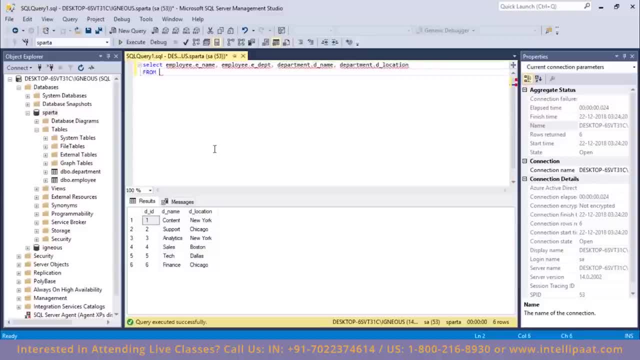 After this I will give in the from keyword and then give in the name of the first table, which would be employee. Then I will give in the keywords inner join and give in the name of the second table, which would be department Right. 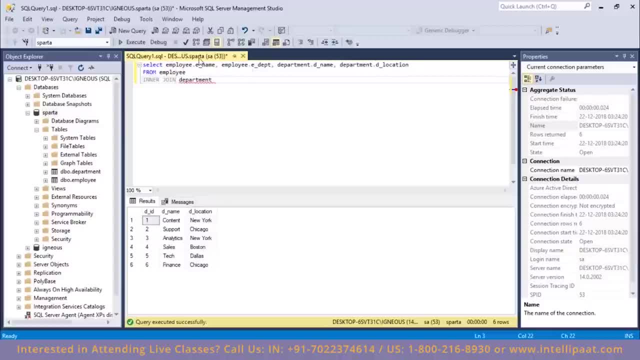 So I am selecting these four columns and the inner join would be on the employee table and the department table Right. So I will use the on keyword and give the condition. So the condition would be the values of the edept column of the employee table and the values of the dname column of the department table should be equal. 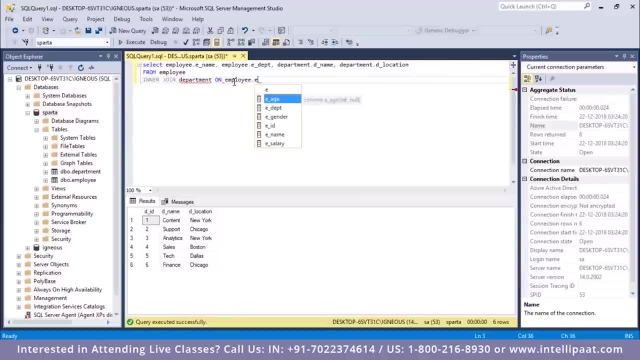 So employee dot edept should be equal to department dot dname, Right guys. So this is the complete syntax to implement inner join on these two columns of the employee table, And I am selecting the ename and edepartment columns from the employee table and dname and dlocation columns from the department table. 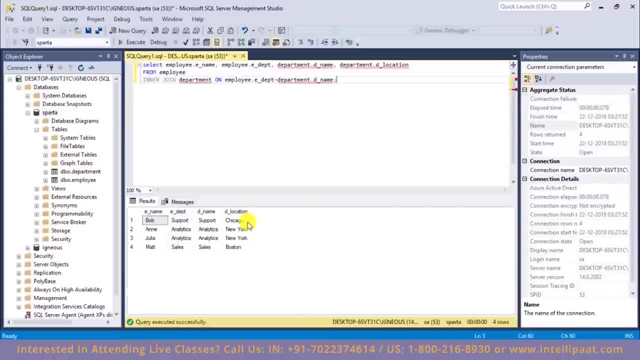 Let me hit, execute Right And this is what we get. So we have these four columns over here: Employee name, employee department, department name and department location. And since this is inner join, we have only those records where the values from edept have matched to those values of department. 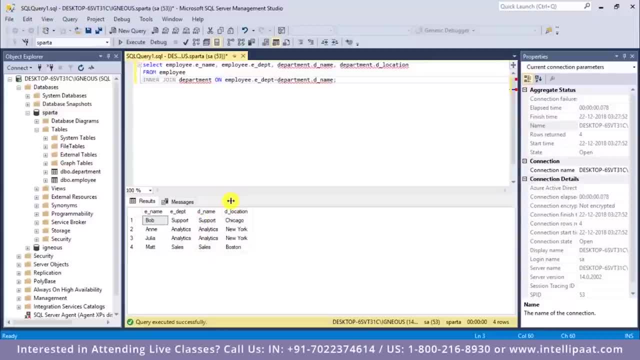 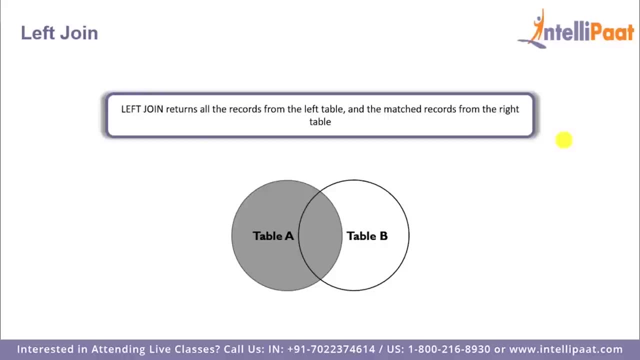 Those values of dname And this is how we can implement inner join. So the left join basically returns all the records from the left table and the matched records from the right table. So if we take table A and table B, then applying left join on these two tables would give us all the records from table A and only the matched records from the table B. 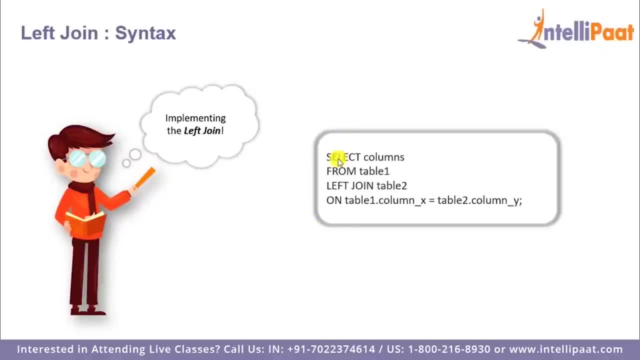 So let's have a look at the syntax. We will start with the select keyword and then give the list of the columns, Following which we will give the from keyword And give the name of the first table. Then we will use the keywords left- join- and then give the name of the second table. 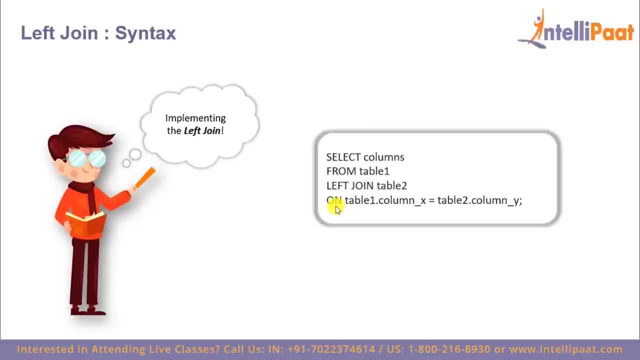 After which we will use the keyword on. So this on keyword tells SQL that this left join needs to be done on some condition, And that condition would be: values from column X of table 1 should be equal to values from column Y of table 2.. 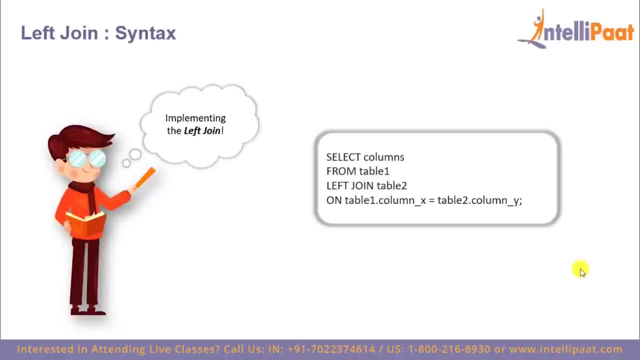 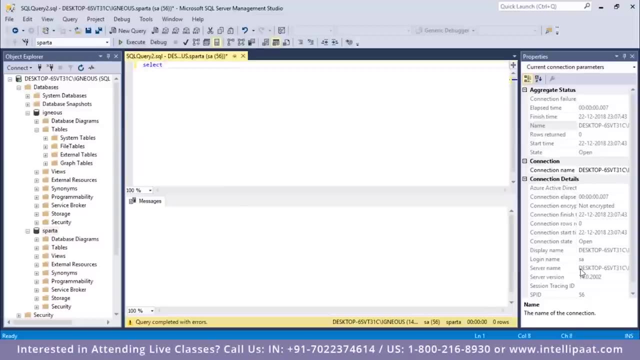 So let's implement this left join on the employee table and the department table. So before I implement the left join, let me actually have a glance at both of the tables. So I will start with the employee table. Select star from employee. And these are the columns present in the employee table. 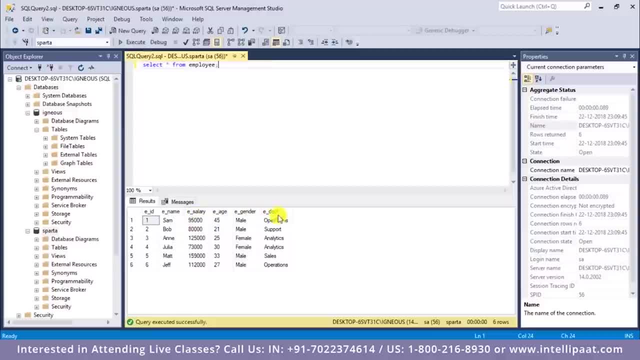 Employee ID, employee name, employee salary, employee age, employee gender and employee department. So I will be taking this employee department column from the employee table Now. similarly, let me have a glance at the department table. Select star from The name of the table is department. 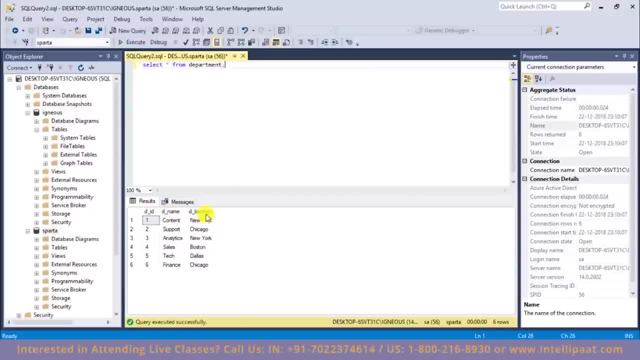 So we have the department ID department, The department name and the department location And from this department table we will be selecting this D name column. So we will be applying the left join on the E, D, E, P, T column of the employee table. 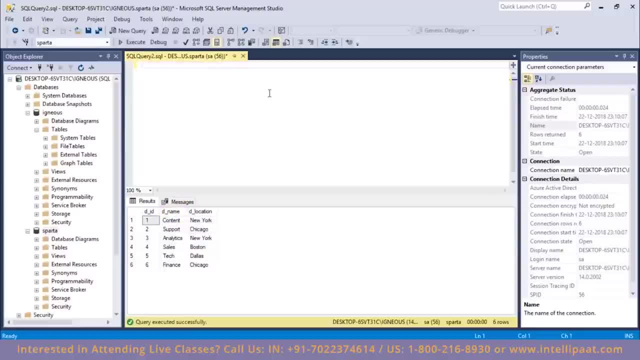 And the D name column from the department table. So let me start with the syntax to implement the left join. So I will give in the select keyword first And then I will give all of the columns which I want to select. So I want to select the employee name column from the employee table. 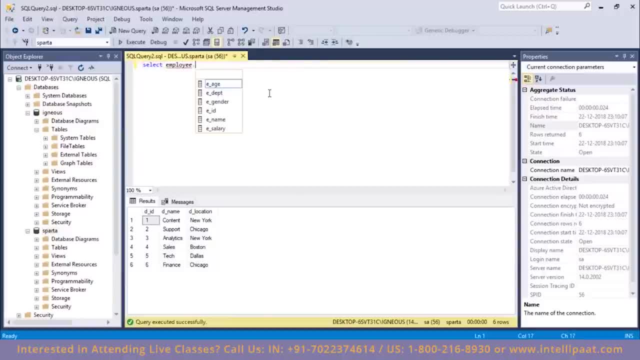 So first I will give in the name of the table which is employee, Then I will put dot over here Type: employee name. Now I'd also want the employee department column. So first I will give in the name of the table which is employee. 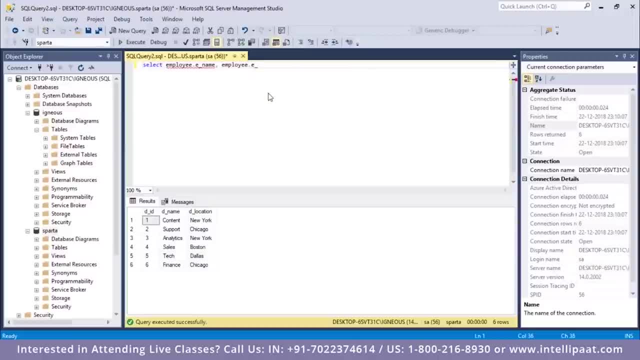 I will put dot over here And then I will give in E, D, E, P T over here. Then I'd want the department name column and the department location column from the department table. So I will give in the name of the table first, which is department. 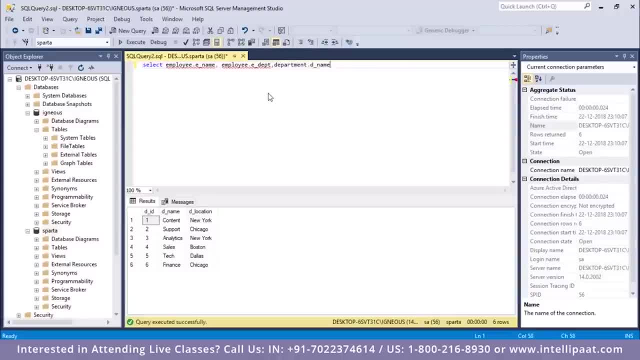 I will put a dot over here And I will select the department name column from the department table. Similarly, again, I will type in the table name, which is department, And I will put a dot over here And then I will also select the department location column. 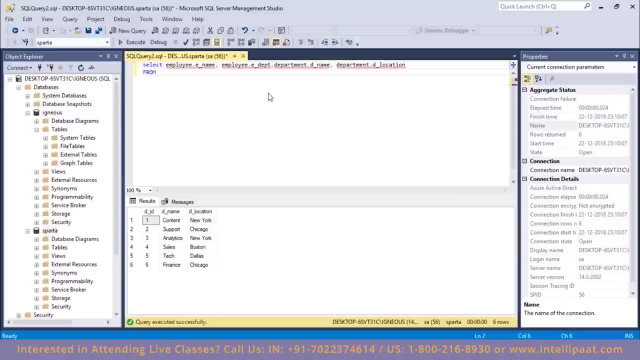 So, now that I have selected all of the columns, let me give in the keyword from And then give the name of the first table, which is employee. Then I will give the keywords left, join, And then give the name of the second table, which is department. 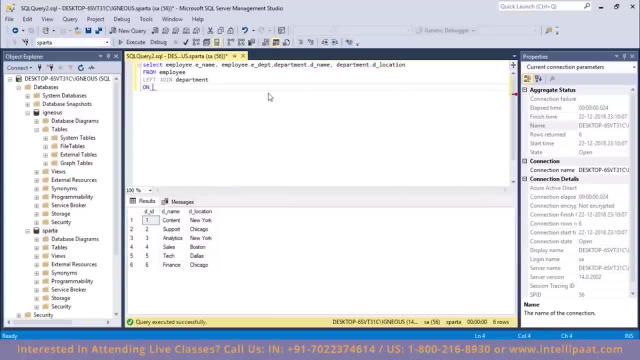 Now I will give the on keyword and then give the condition. And the condition would be: the values from the employee department column from the employee table Should be equal to the values of the department name column from the department table. So employee dot E, D, E, P, T, these values should be equal to department dot T name. 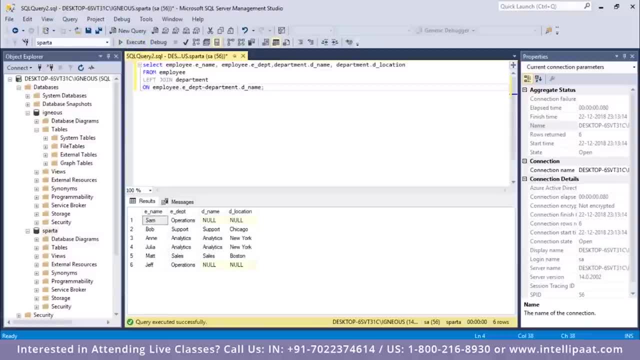 I will put a semicolon over here. Now let me hit execute- Right. so this is the result when we apply the left join operation on the employee table and the department table. So we've got all of the records from the left table, which is the employee table. 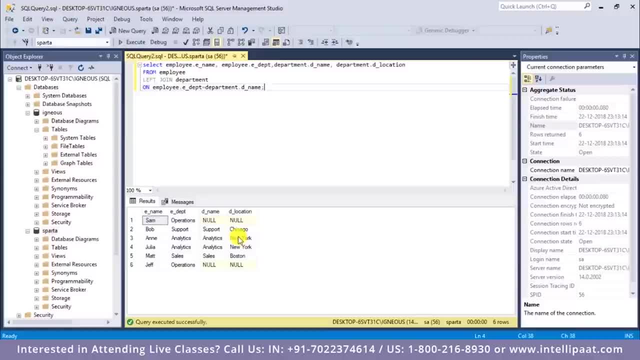 And we see that we get only the match records from the department table, which is the right table, And wherever the records haven't matched, we get null values. So we see that the operations department is not present in the department table. So that is why we have null values over here. 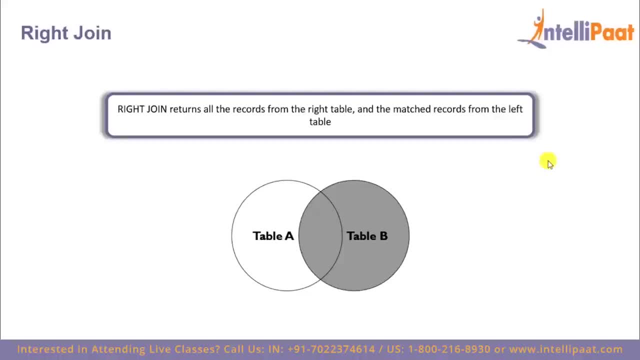 And this is how we can implement the left join. So the right join basically returns all the records from the right table And only the match records from the left table. So if we take table A and table B, Then applying right join on these two tables would give us all the records from table B. 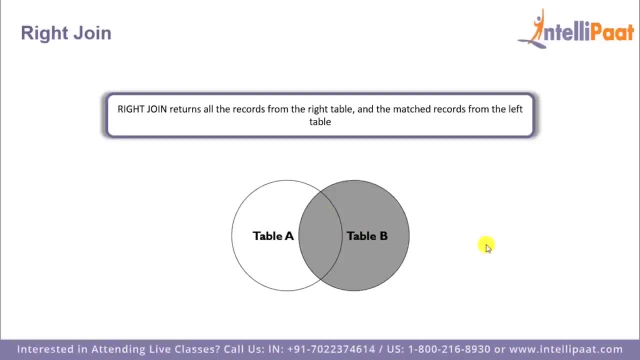 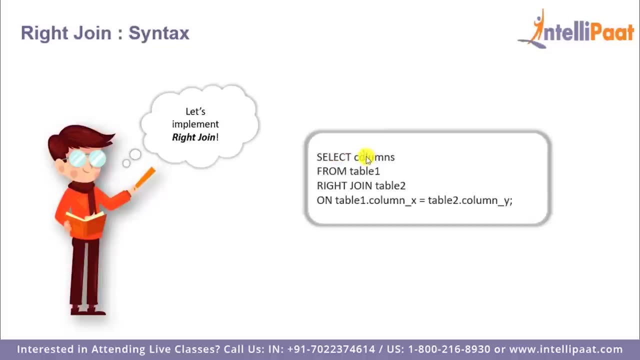 And only the match records from table A. So let's have a look at the syntax. We'll start with the select keyword first And then give them the list of the columns, Following which we'll give the from keyword And then give the name of the first table. 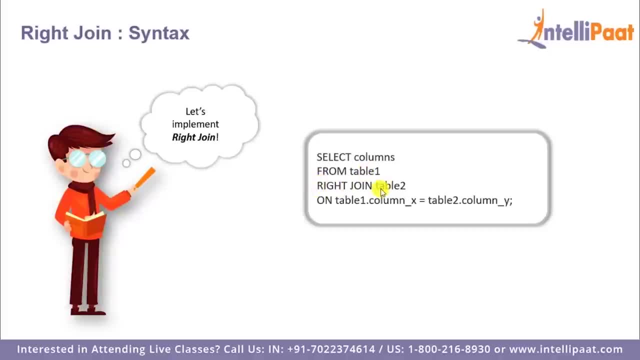 Then we'll use the keywords, write join and then give the name of the second table, After which we'll use the keyword on. So this on keyword tells SQL that this right join needs to be done on some condition, And that condition would be: values from column X of table 1 should be equal to values from column Y of table 2.. 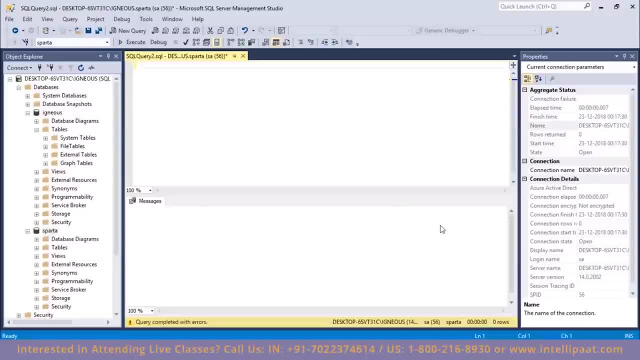 So before I go ahead and implement the right join, Let me actually have a glance at the employee table and the department table. So I'll start with the employee table. Select start from employee. So this is our employee table, which comprises of these columns: 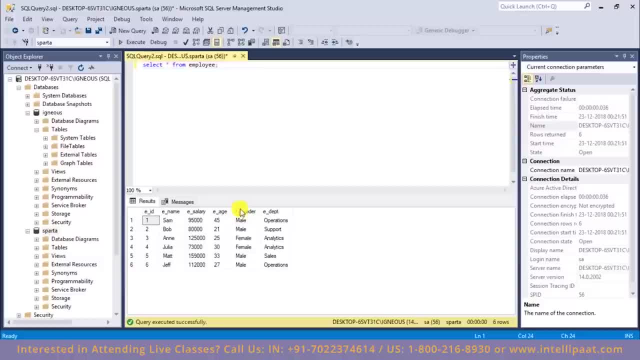 Employee ID, Employee Name, Employee Salary, Employee Age, Employee Gender and Employee Department, And we'll be implementing the right join with respect to this column: Employee Department. Now let me also have a glance at the department table Select. Start from the name of the table as department. 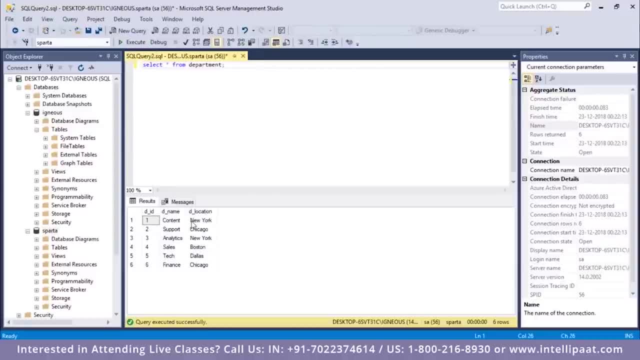 I'll hit execute. So the department table comprises these three columns: Department ID, Department Name and Department Location, And we'll be implementing the right join with respect to this D name column. So now let me go ahead and write the syntax for the right join. 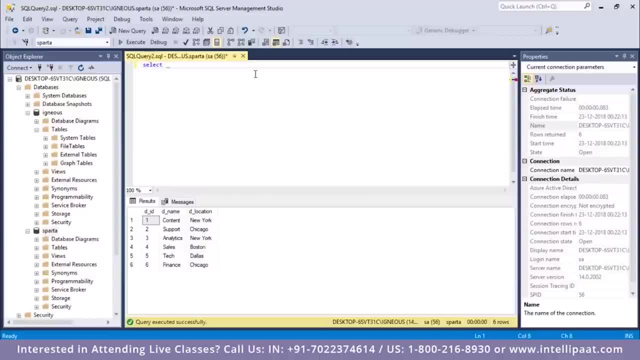 So I will put in the select keyword first And then I'll give in all of the columns which I want to select. So from the employee table I want to select the employee name and the employee department columns. So for that I'd have to give in the name of the table first. 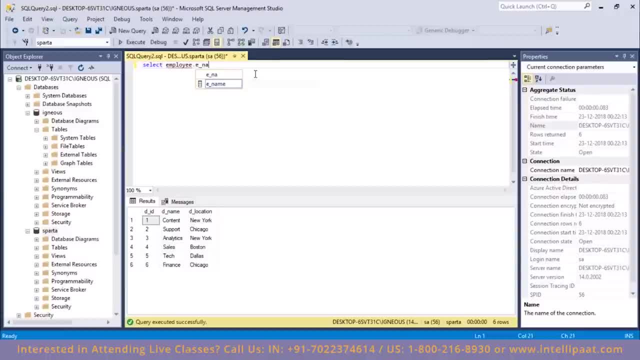 Then I'll put dot And then I will give in the name of the column which I want to select, So employee name. Similarly I also want the employee department column. So first I will give in the name of the table which is employee. 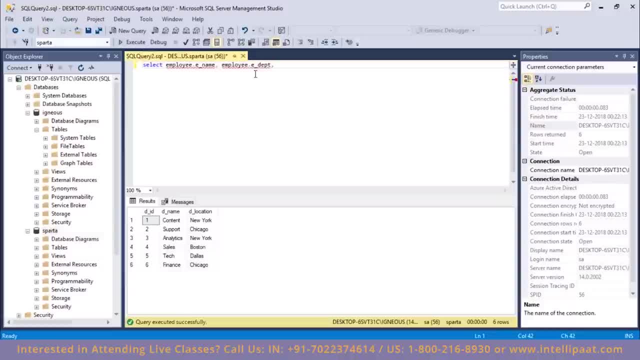 And then I'll select the EDPT column And then I want the department name and department location columns in the department table. So I'd have to give in the name of the table which is department. I'll put in dot over here And then give in the name of the column which is D name. 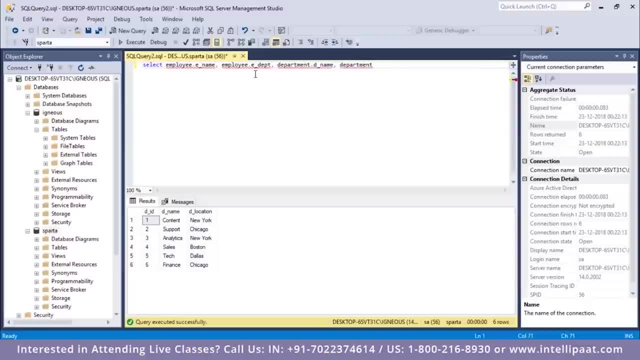 Similarly I'd also want the department location, So I'll put dot and then select department location. Now I will give in the from keyword and then give in the name of the first table, which would be employee. After that I will type the keywords right- join- and then give the name of the second table, which is department. 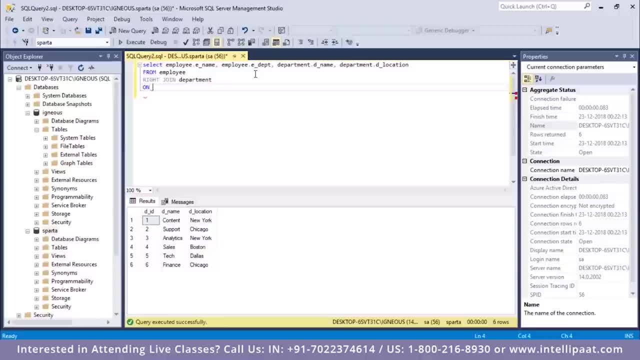 Then I'll use the on keyword and then give the condition. So the condition would be: values of EDPT column from employee should be equal to values of EDPT column from employee. I'll use of D name column from the department table. So employee dot E D E P T should be equal to department dot D name. 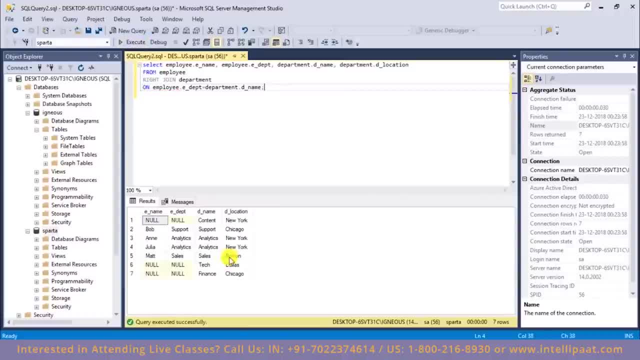 I'll put semicolon over here. Let me hit execute. And this is the result which we get when we apply right join on the employee table and the department table. And since this is the right join, we see that we have all the records from the department table. 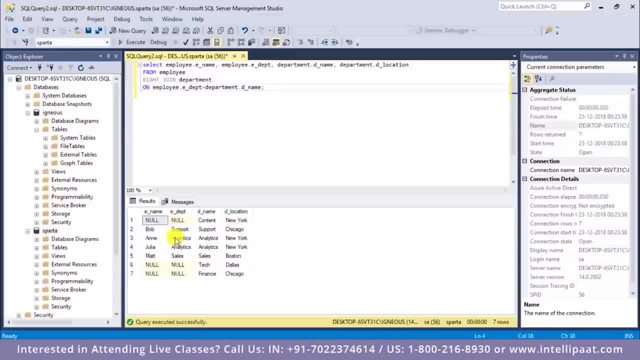 And we have only the match records from the employee table. So we see that there is no content, tech and finance departments in the employee table. So that is why we have null values over there And this is how we can implement the right join. 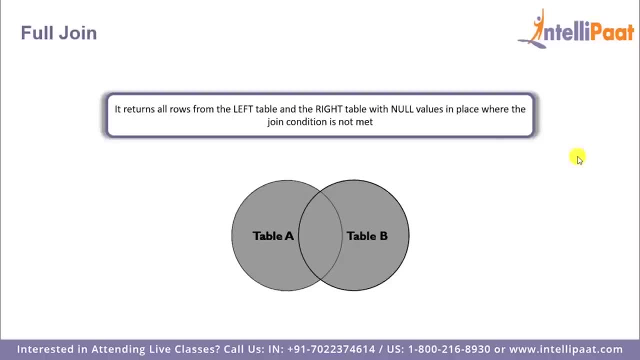 So the full join basically returns all the records from the left table and also all the records from the right table. So if we take table A and table B, then applying full join on these two tables would give us all the records from table A and also all the records from table B. 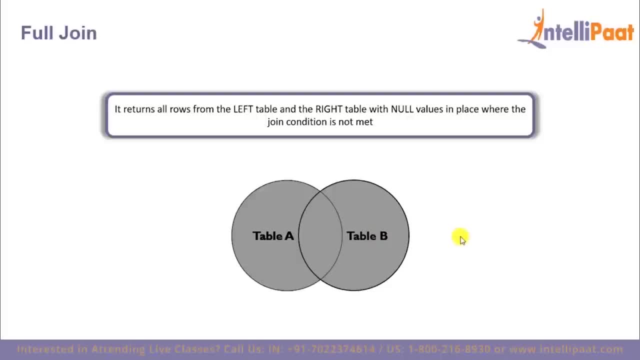 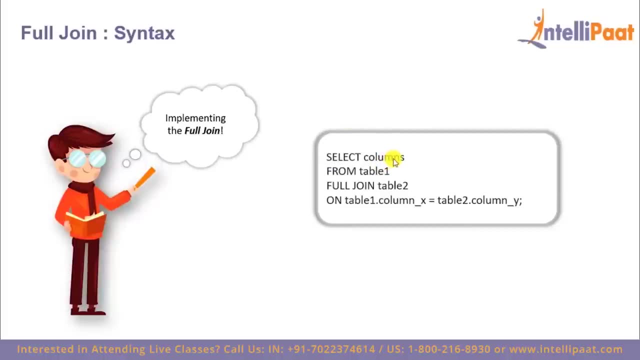 And wherever the join condition is not met, we'll get null values in that place. So let's have a look at the syntax. We'll start with the select keyword first and then give in the list of the columns, Following which we'll give the from keyword and then give the name of the first table. 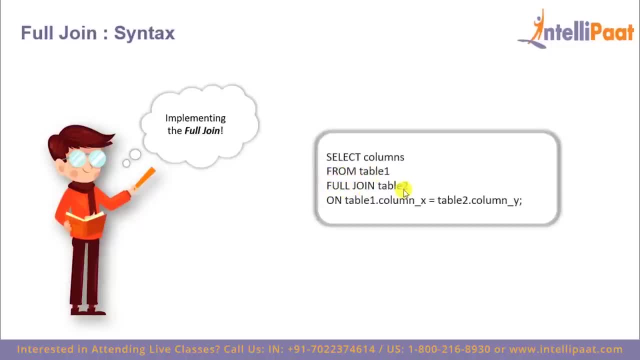 Then we'll use the keywords full join and then give the name of the second table, After which we'll use the keyword on. So this on keyword tells SQL that this full join needs to be done on some condition, And that condition would be: values from column X of table 1 should be equal to values of column Y from table 2.. 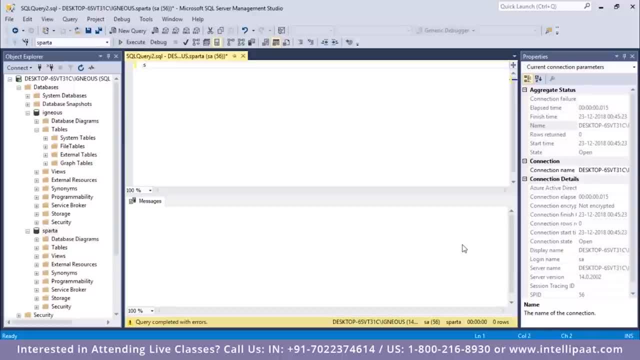 So before I go ahead and implement the full join, let me actually have a glance at the employee table and the department table. So I'll start with the employee table first. So select start from the name of the table is employee. So we have these columns in the employee table. 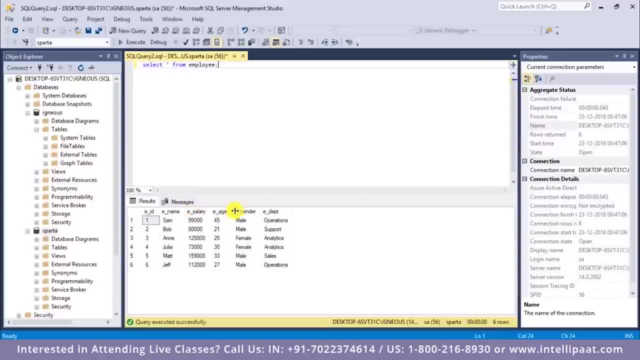 Employee ID, Employee Name, Employee Salary, Employee Age, Employee Gender and Employee Department And we'll be applying the full join on the employee department column. Now let me also have a glance at the department table. Select- start from the name of the table is department. 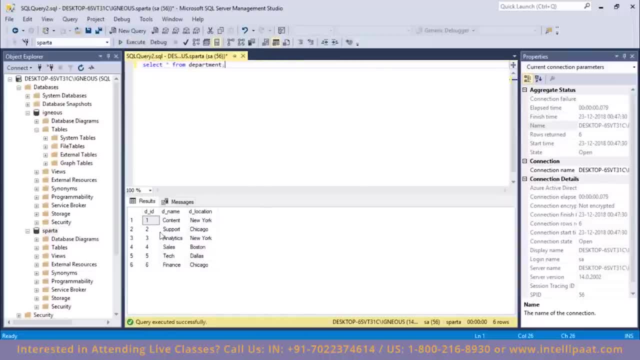 I'll hit execute. So the department table has these three columns: Department ID, Department Name and Department Location- And we'll be applying the full join condition on this department name column. So let me start with the syntax for the full join. So I will give in the select keyword first and then I'll give in the list of all of the columns which I want to select. 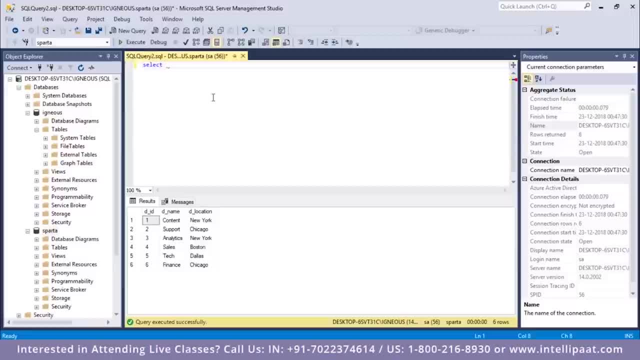 So I want to select the employee name and the employee age And I'll know the order of the column number for the column. First I'll name the person and name the table And I'll say employee name. So I'll give in the name of the table Employee and I'll put a calc over here. 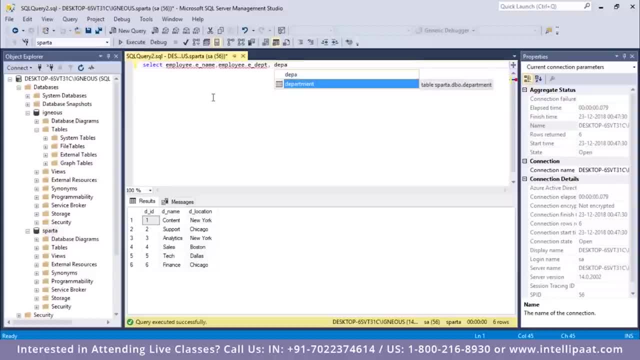 Now that I have entered the teller left, BER ebenfalls checked here and then I'll select department name. Similarly, I'll also select the department location column. So I will give in the name of the table, I'll put dot and then I'll select the department location column. After this I will use: 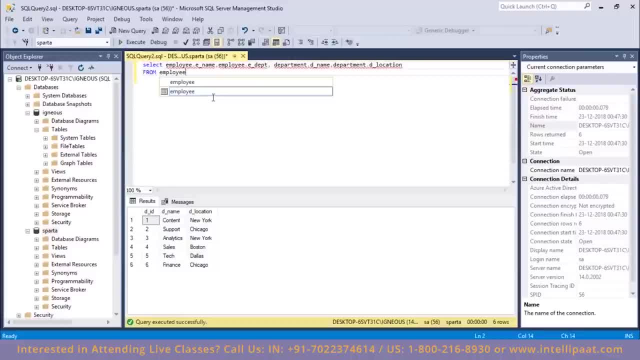 the from keyword and then give in the name of the first table which is employed. Then I will use the keywords pull, join and then give in the name of the second table which is department. After that I will give the keyword on and then specify the condition on the basis of which the full join is to be done. So the 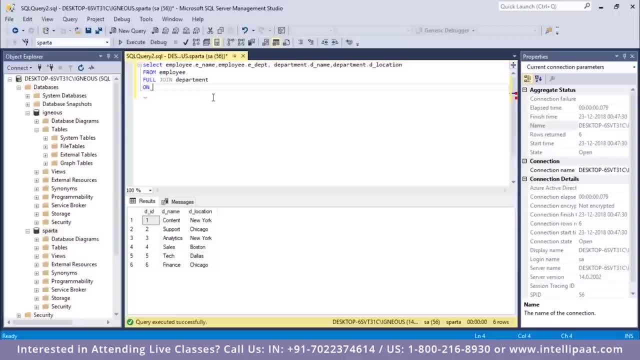 condition is: the values of edept column from the employee table should match with the values of the dname column from the department table. So that could be: employee dot edept is equal to department dot dname. I'll put semicolon over here. let me hit execute. So this is the result of the full join. 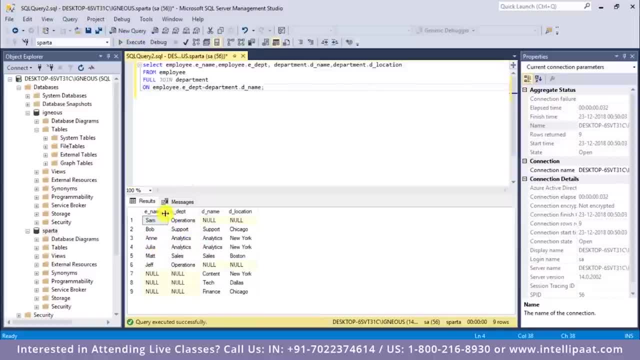 on the employee table and the department table. So wherever we see null values, that means that the records have not matched over here. So operations is present in the employee table but it is not present in the department table. So that is why we have null values in the columns extracted. 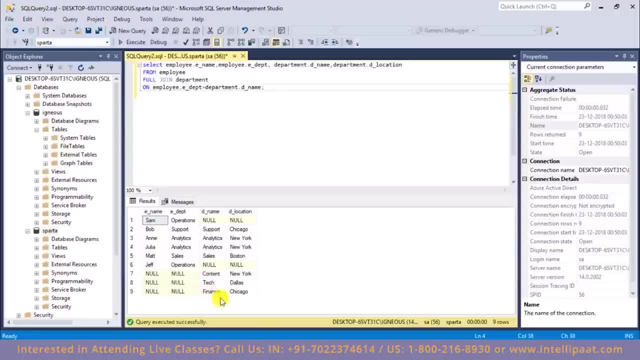 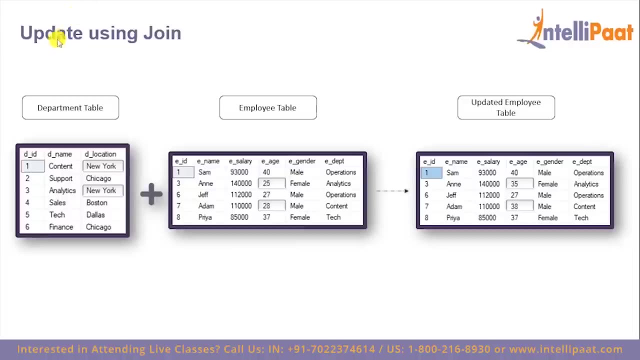 from the department table. Similarly, we have content tech and finance departments only in the department table and that is why we have null values in the columns extracted from the employee table. And this is how we can implement the full join. So let's understand: how can we use update with join Here we have 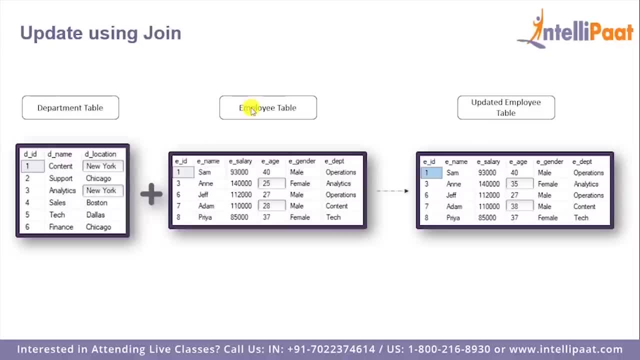 two tables: The department table and the employee table. Now I'd want to update the age value in the employee table Wherever the department location is brought in for nutrients. So from the department table we can find out that content and analytics departments are based in New York. So in the employee table will 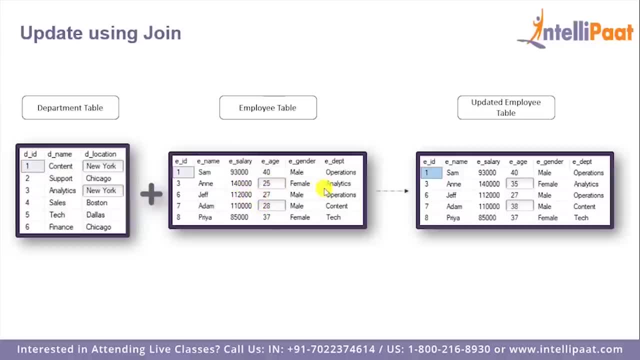 update those. each values for the department is either analytics or content, And after updating the table using the join statement, you see that these two values have been modified. So we have the department and employee tables right in front of us and we'll be implementing the same task. so, from this, 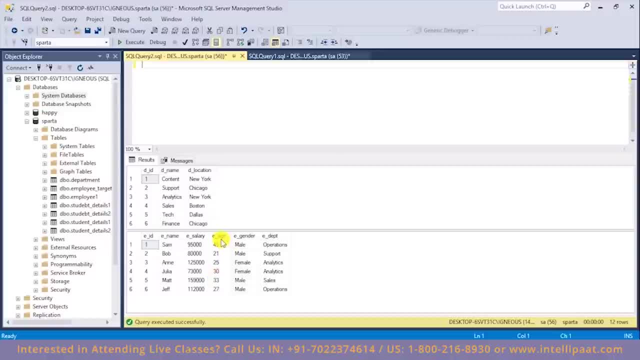 employee table. we'll add 10 more to the age values wherever the department location is equal to New York and since we've already seen that content and analytics are based in New York, so basically these two records where the EDPT value is equal to analytics, we'll be adding 10 more to these two age. 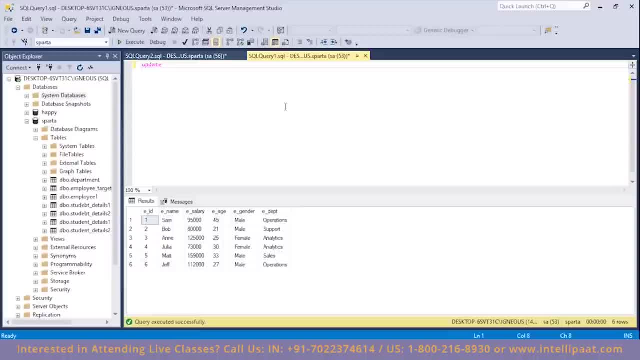 values. so let me write the syntax for that. I'll type update and then give the name of the table which I want to update, so that would be employee. after that I'll use the set keyword and then update the age value. so eh, and I'm adding 10 more to the eh value. after that I'll use the from keyword and give. 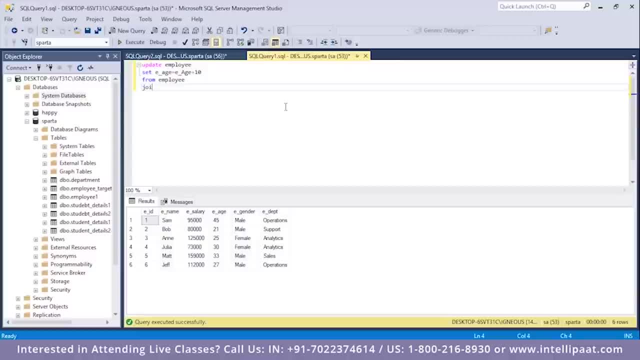 the name of the first table, which would be employee, then I'll type join and then give the name of the second table, which would be department. then I'll type on and then state the join condition. so the join condition is you. the values of the EDPT column from the employee table should be equal to the 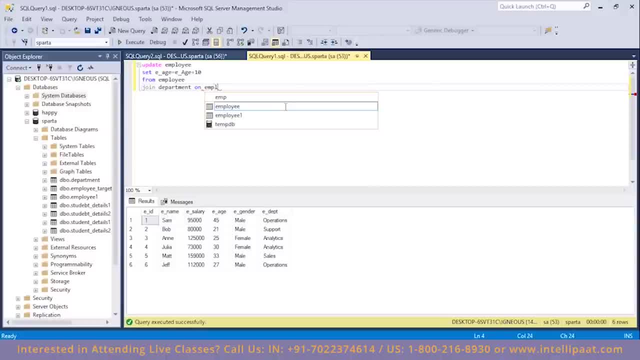 values of D name column from the department table. so employee dot EDPT should be equal to department dot D name. and finally we'll specify the where condition, which would be the location should be equal to New York. so I'll select all of this, I'll click on execute so you see that two rows have. 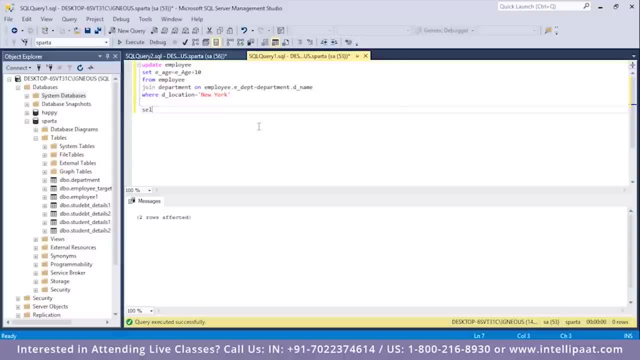 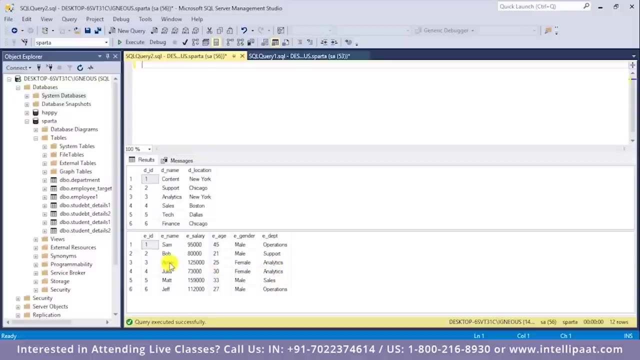 been affected. now let me have a glance at the modified employee table select. start from. I'll type the name of the table which would be employee. now I'll execute this. so let me see the original age values. so over here the department is analytics and we see that the initial age of Ann and Julia is twenty-five and 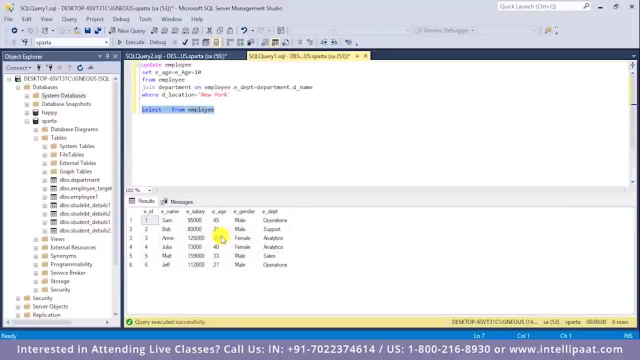 thirty. and after applying the update command, we see that the age has been been modified to 35 and 40. So Ann's initial age was 25. after updating it became 35.. Similarly, Julia's initial age was 30. after updating it became 40. So 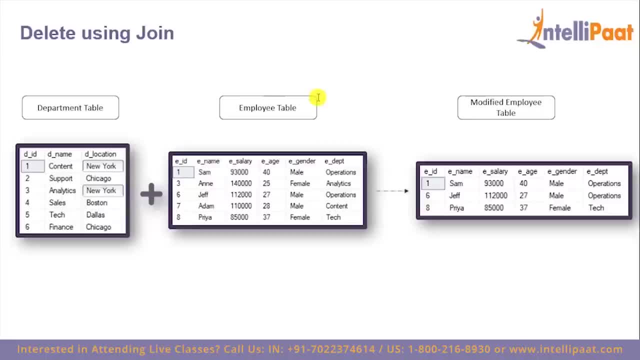 this is how we can use update with a join condition. Now let's understand how can we use delete with join. So this time, from the employee table, I'll be deleting those records where the department location is equal to New York and since content and analytics are based in New York, we will go ahead and delete those. 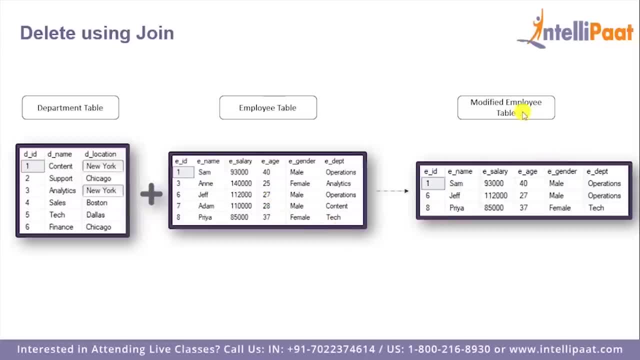 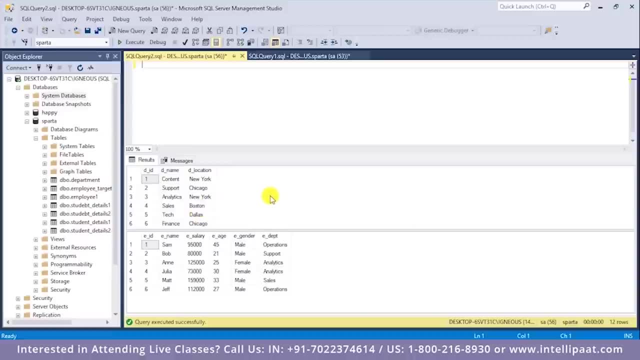 two records from the employee table. So in the final modified employee table we see that there are no records for the department is either content or analytics. So again, we'll be implementing the same task from this employee table. I'll be deleting those records where the department location is in New York. So 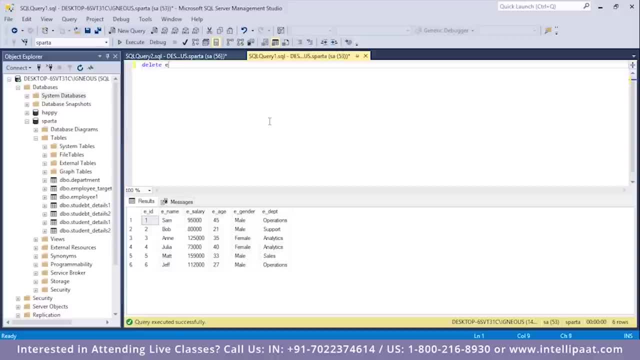 let me write the syntax for that. so I'll type delete and then give the name of the table from which I'd want to delete the records, so that would be employee or shin. After that I will give the from keyword and then give the name of the first table which. 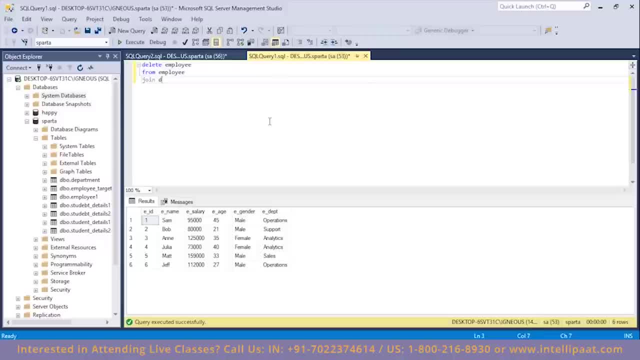 would be employee again. Then I'll type join and then give the name of the second table, which would be department. Now I will give on and give the join condition, which is same again. So the values of E DEPT column from the employee table should be equal to the values of D name. 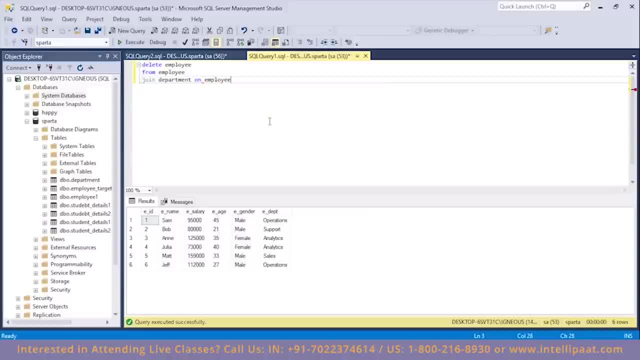 column from the department table. So employee dot E DEPT should be equal to department dot D name and finally, I'll use the where condition, which would be D location should be equal to New York. So I'll select all of this, I'll click on execute. 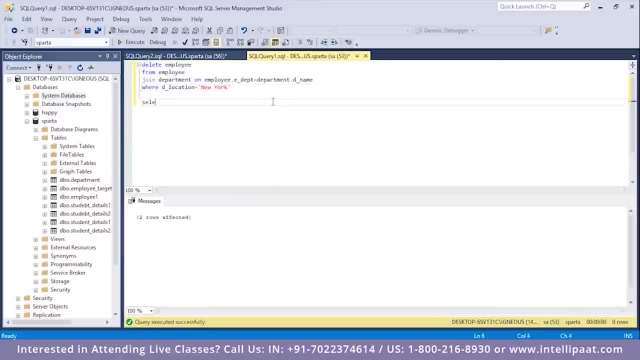 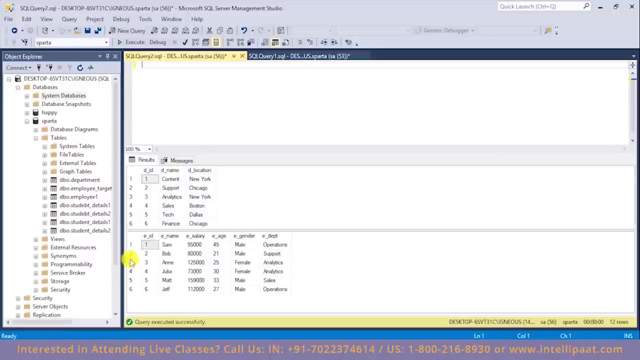 So again we see that two rows have been affected. Now let me have a glance at the modified table. Select start from employee. so see that there are no records for the department is analytics. So if you have a look at the original table, we see that there are two records where the 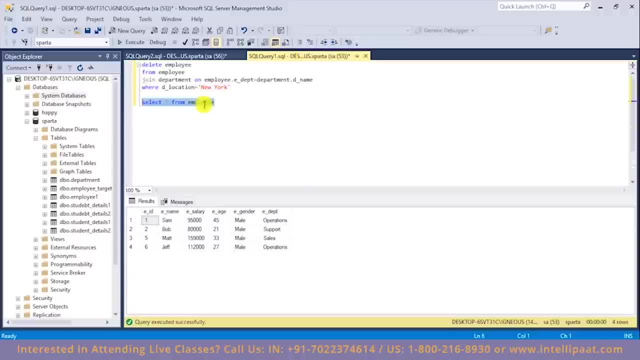 employees were present in the analytics department and after deleting those two records, we just have four records present in the employee table, And this is how we can work with: update and delete statements using join. So the union operators used to combine. the results set off to almost three. 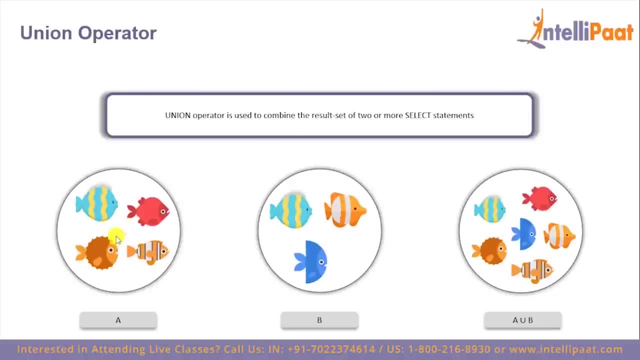 For example, if the first select statement returns these four fish and the second select statement returns these three fish, then the union operator would return the results set of these two select statements, And if there is a record which is present in both the tables, we'll get only one of. 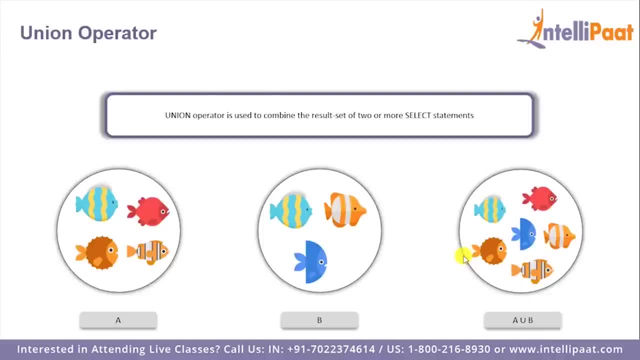 them in the final result. That is, there would be no duplicates in the final result. So here we see that this blue fish is present in both the tables A and B, but in the final result of A union B We'll get only one of the value. 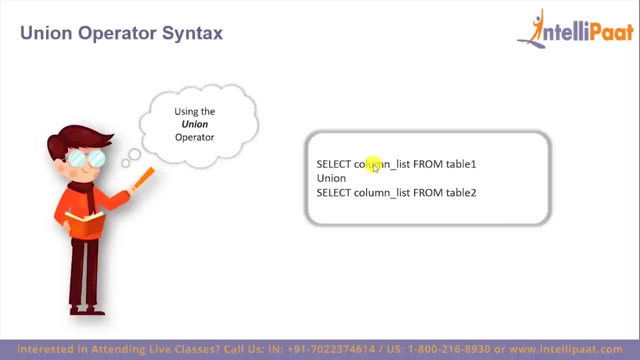 And this is the syntax for the union operator- We'll give the first select statement. After that, we'll give the union operator, following which we'll give the second select statement. Now you also need to keep in mind that the number and order of columns must be same in. 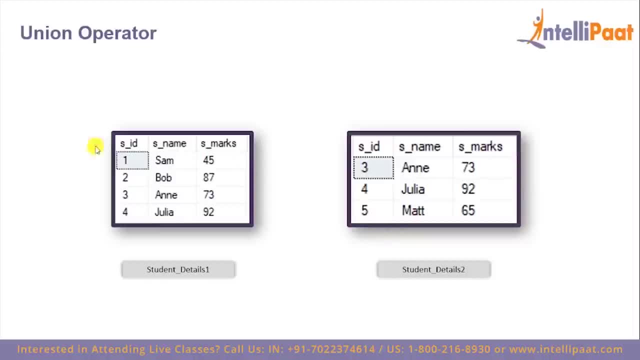 both the select queries And we'll be implementing the union operator on these two tables. So we have the student details: one table which has the columns SID, S name and S marks and has these four records. The other table is student details two, which has the same columns and comprises of these: 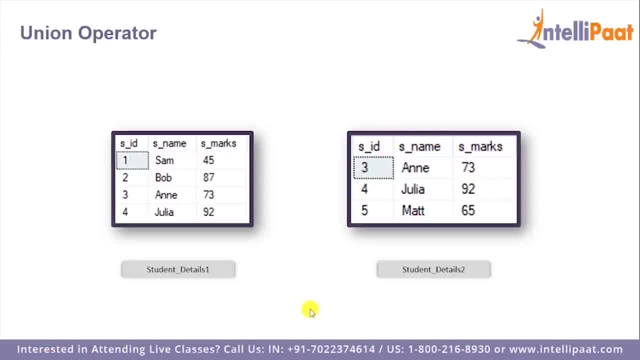 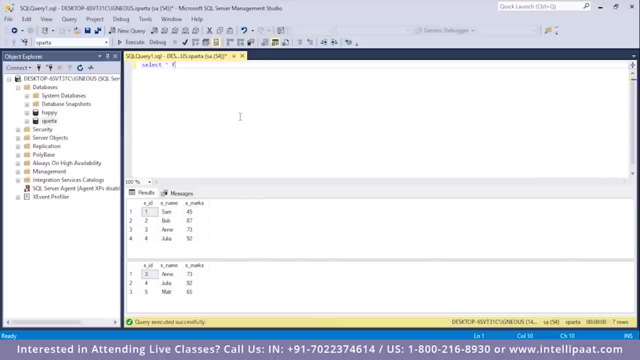 three records. So let's go to SQL server and work with the union operator. So we have our two tables right in front of us. So let me start with the syntax. I'll get the first select query, Select, start from, and then I'll give the name of the table, which is student details one. 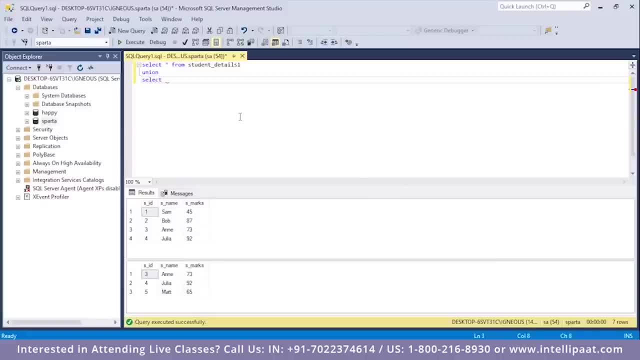 After that I'll give the union operator and then give the next select statement, Select start from, And then the name of the table is student details one. I'll select all of this and I'll hit execute. So the union operator has given us the result set of both of the select statements. 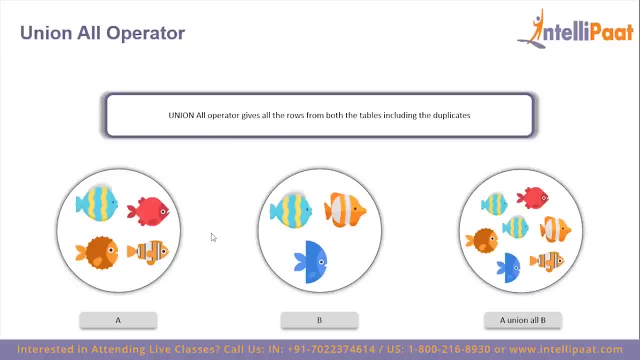 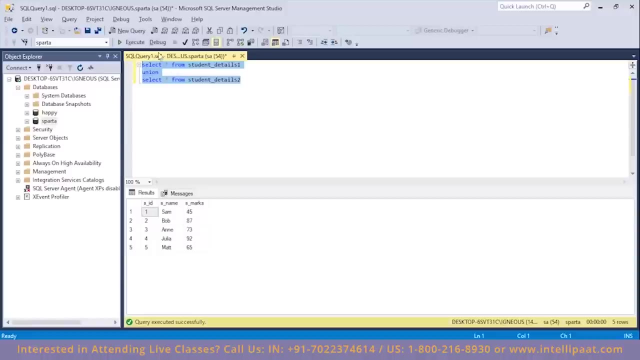 Then we have the union all operator. The union all operator gives all the rows from both the tables, including the duplicates as well. So here, since the blue fish is present in both the tables A and B, the final result of A union all B will also have the duplicate value. 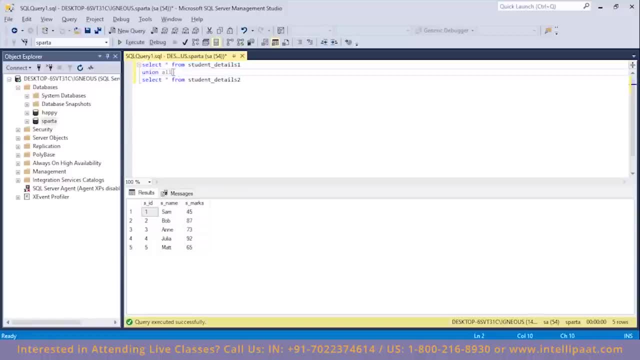 So now Let's add the all keyword over here. So I am using the union all operator between these two tables. Now I'll hit execute So we see that we also have the duplicate values. So here these records where Ann and Julia are present. 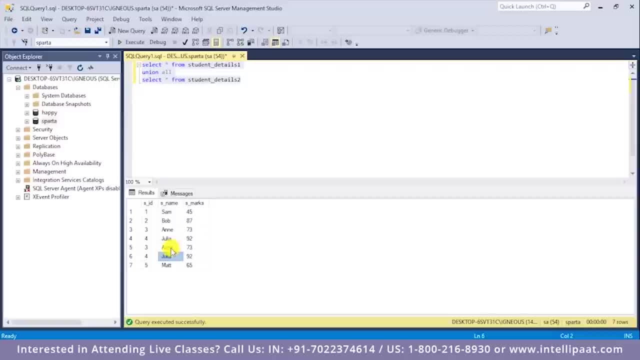 These are from the first table, And again here, Ann and Julia. So these records are from the second table. So we have also got the duplicate records this time because we've used the union all operator. Now again, let me remove this all keyword. 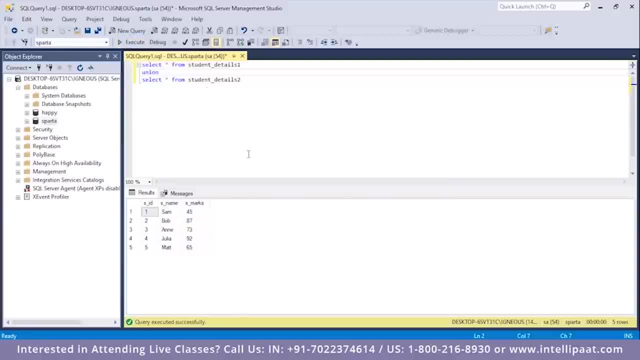 Let me hit execute So you see that there are no duplicates this time. So this is a difference between union and union all operators. So this is how we can work with the union and union all operators. So the except operator combines two select statements and returns unique records from: 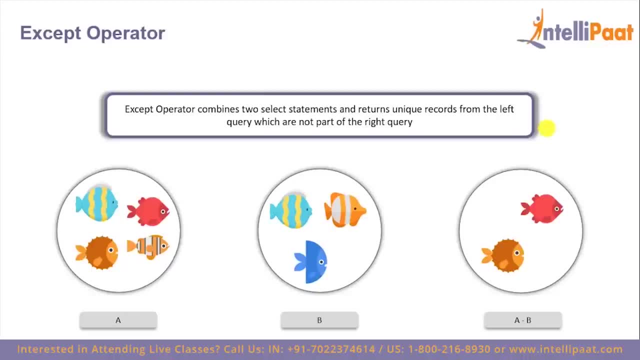 the left query which are not part of the right query. For example, if the first select statement returns these four fish and the second select statement returns these three fish, then the except operator would return us these two fish. So we will call the except operators instead of the select s which were part of the first. 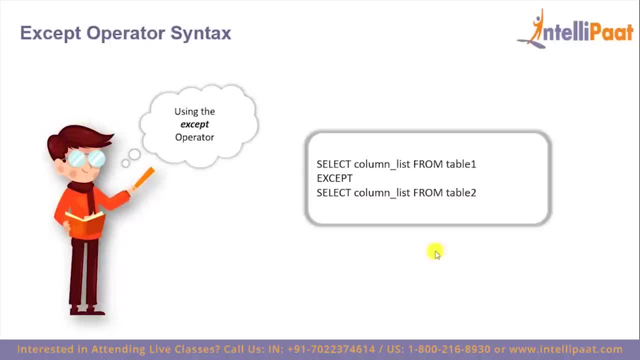 select statement, but not the second select statement, And this is the syntax of the except operator. We'll get the first select statement. After that we'll get the except operator, following which will get the second select statement. Now you also need to keep in mind that the number and order of columns must be same in 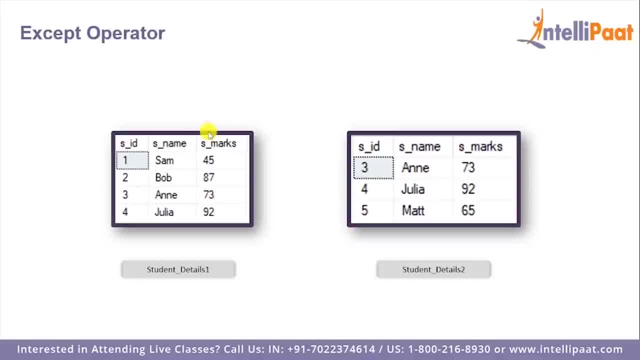 both the select queries And we'll be implementing, except operator, on these two tables. So we have the student details, one table which has the columns s, I, D s name and f, h, And this is what we get marks and as these four records, and the other table is student details 2, which 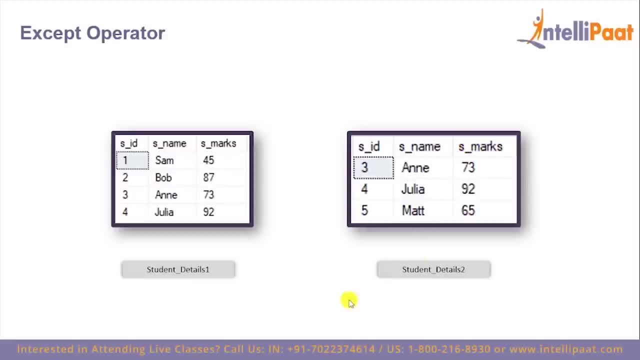 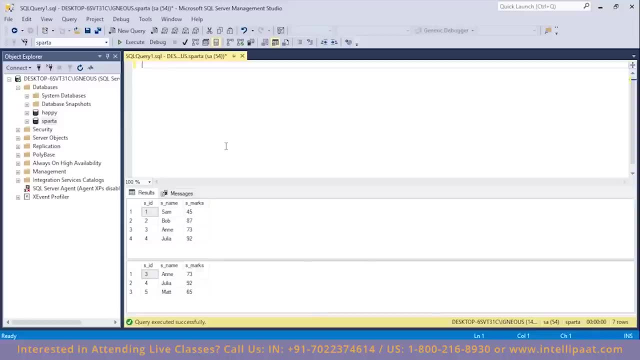 has the same columns and comprises of these three records. so let's go to SQL server and work with the except operator, right, so we have our two tables right in front of us. so let me type in the syntax. I will give the first select query, which is select star from, and then I'll given the name of the table, which is student. 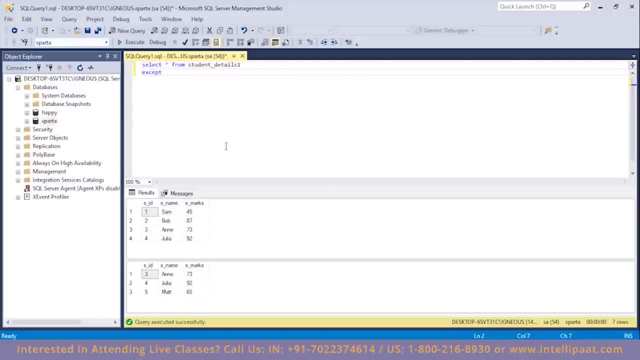 details 1. after that I will use the except operator and then, given the second select statement- select star from the name of the table is student details 2. I'll select all of this again, I'll hit execute. so this is the result of the except operator. so these are the two records which were part of the first. 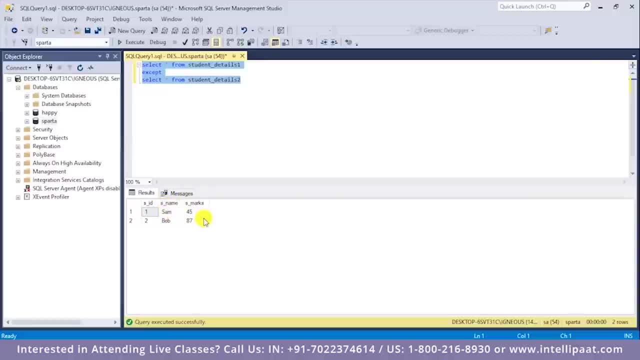 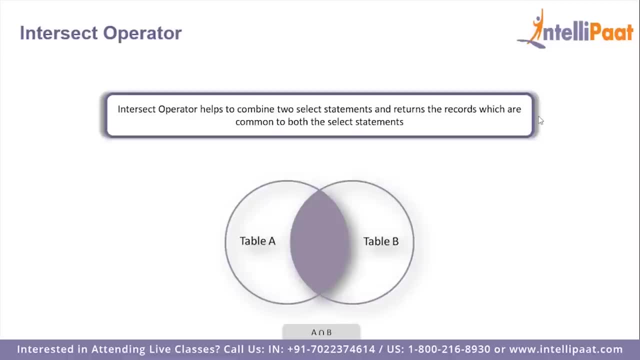 select statement but not the second select statement, and this is how we can work with except operator. so with the intersection method, which is select, in a lot of these cases it is important to Intersect. operator helps to combine two SELECT statements and returns only those records which are common to both the SELECT statements. 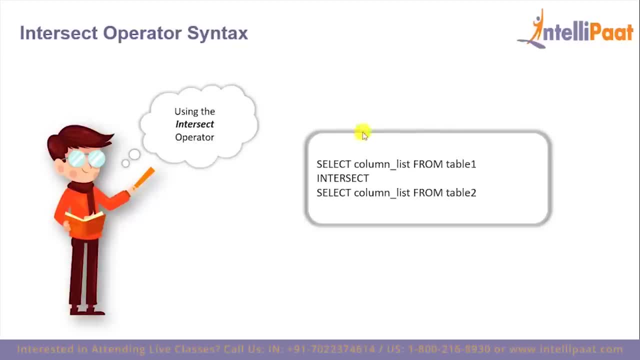 And this is the syntax for the intersect operator: We'll give the first SELECT statement, after which we'll give the intersect operator, following which we'll give the second SELECT statement. So this intersect operator basically retrieves the common records from both the left and 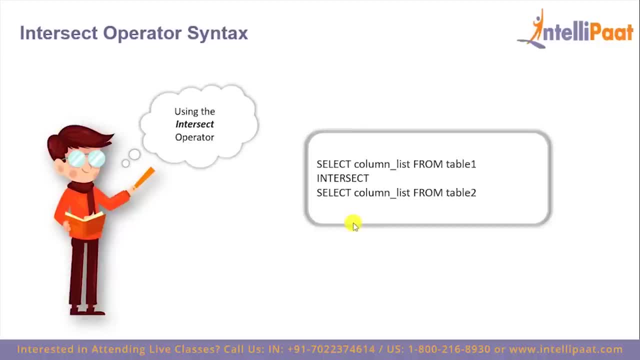 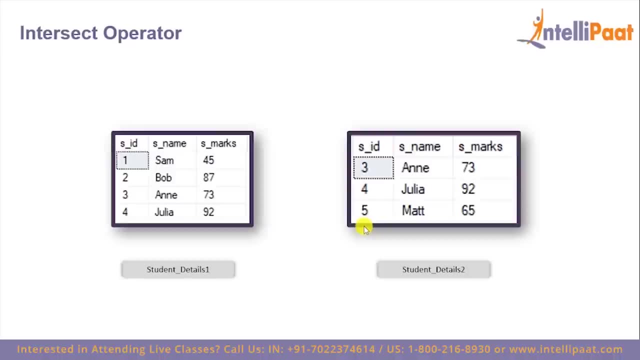 right side of the intersect operator. Now you also need to keep in mind that the number and the order of the columns must be same in both the SELECT queries, And we'll be implementing the intersect operator on these two tables. So we have the student details, one table which has the columns SID, SNAME and SMARKS. 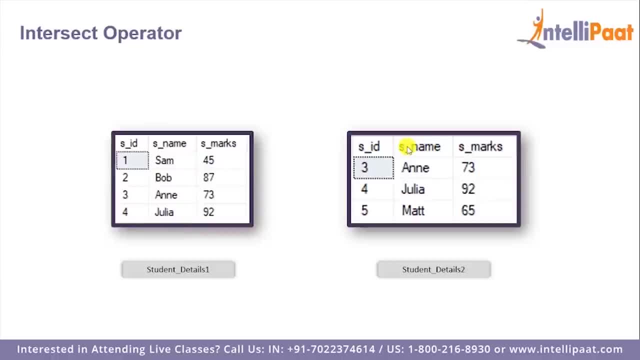 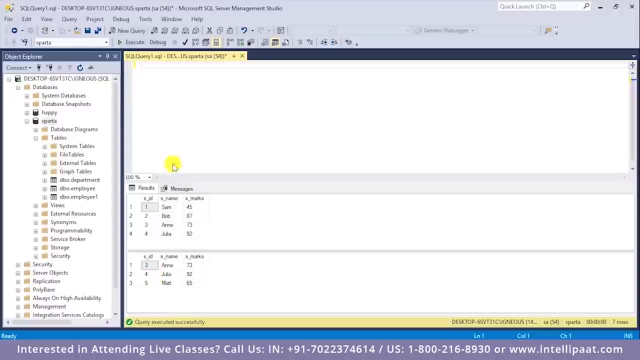 and has four records. The other table is student details two, which has the same columns and comprises of three records. So let's go to SQL Server and work with intersect operator. So these are our results. There are two tables over here. This is the student details one table and this is the student details two table. 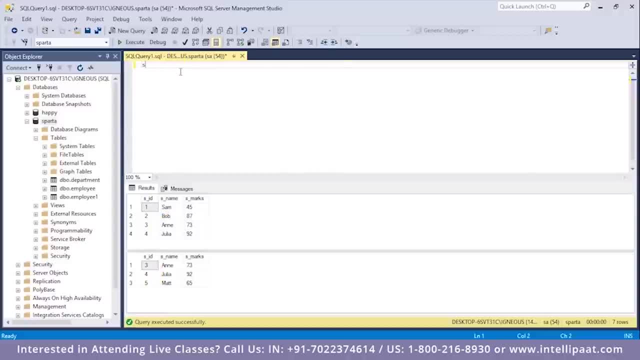 Now let me implement the intersect operator on these two tables. So I will, given the keyword SELECT, START FROM, and then give the name of the table, which would be student details, one After that I will give the intersect operator, INTERSECT- and then give the second SELECT statement. 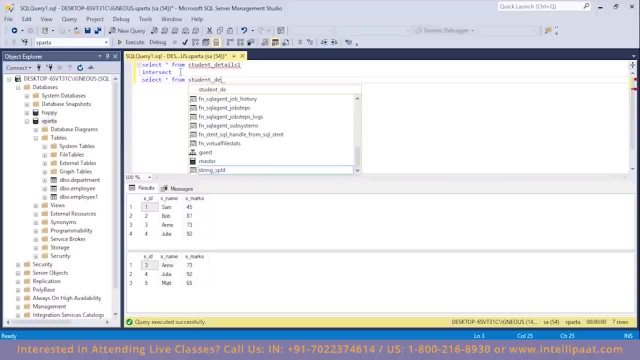 Okay, START FROM student details. two right guys. So this is pretty much the syntax. So we'll give the first SELECT statement, After that we'll give the intersect operator and then we'll give the second SELECT statement. Now let me select all of this. 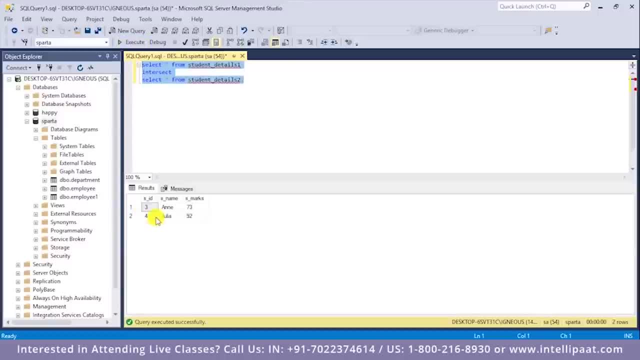 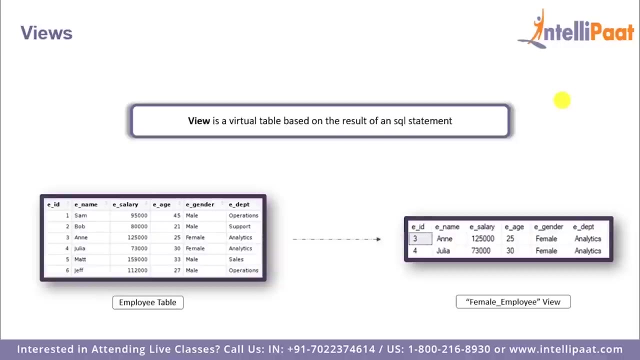 Let me hit execute. So these are the two records which are common to both the student details- one table- and also the student details- two table. And this is how we can work with the intersect operator. So views are virtual tables which I use to limit the information that you want to display. 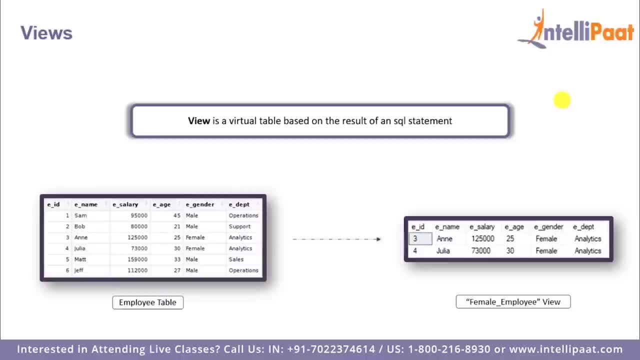 And these are actually nothing but the result of an SQL statement, which have a name associated with them. For example, from this employee table. let's say we wanted to perform multiple operations on the records where the gender is female, So we can create a view for only the female employees from the entire employee table. 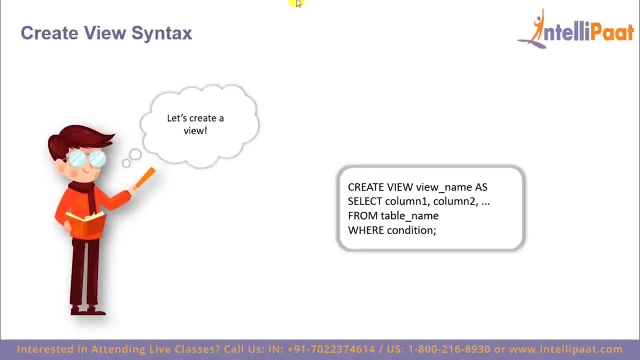 So let's have a look at the syntax to create a view. We'll start off Using the keywords create view, then give the name of the view, after which we'll give the keyword as and then give the list of the columns which you want to select from. 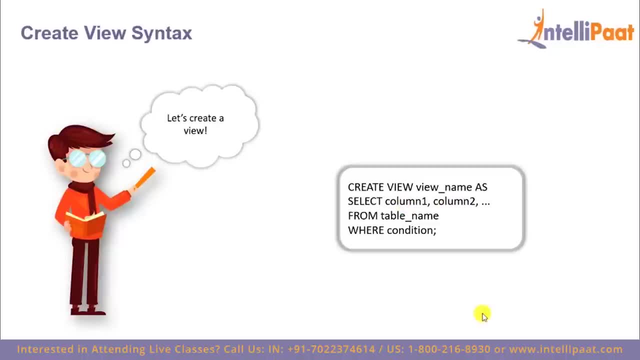 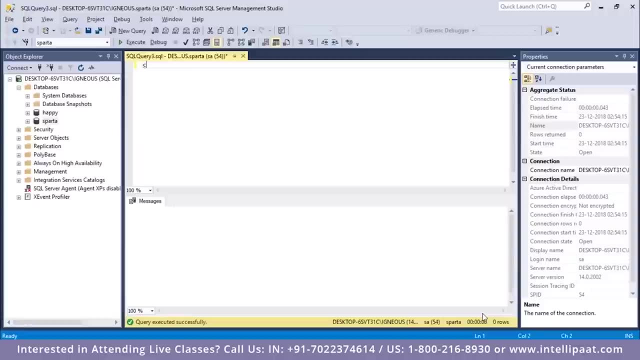 the table. So let's actually create a view from our employee table. So I don't create a view which would comprise of only the female employees from the entire employee table. So this would be the command for that: Create view. then I'll give the name of the view, which would be female employees. 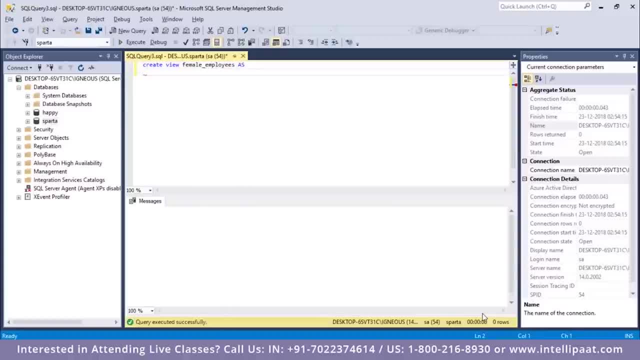 After that I will give in the keyword as and I will select all of the columns from the employee table. So select star from employee. then, using the where clause, I will give in the condition. So the condition would be: each gender is equal to female. 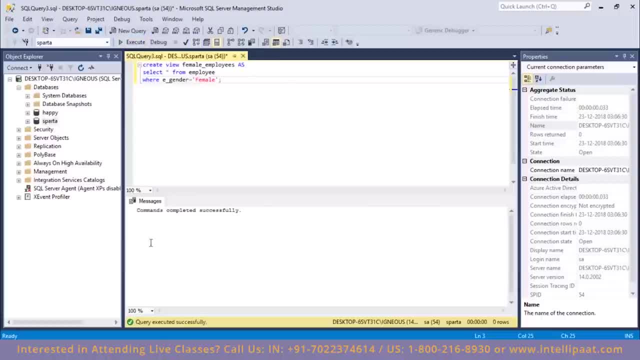 So I'll put a semicolon over here, I'll hit execute. So you see that commands have been completed successfully. So now let me have a glance. The female Employees view Select star from- I'll give the name of the view which would be female employees. 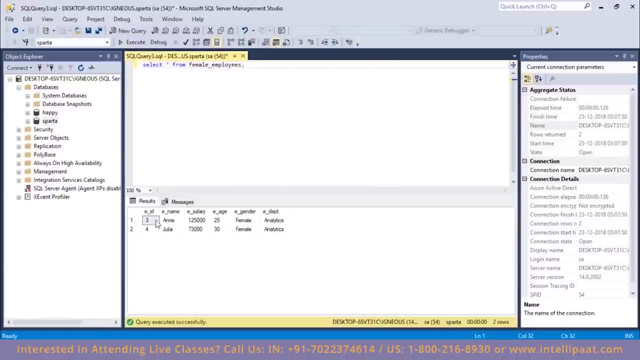 I'll put a semicolon: hit, execute right. So we see that we have successfully created a view from the employee table And in this view we have only two records which comprise of the employees Ann and Julia, and both of them are obviously female. 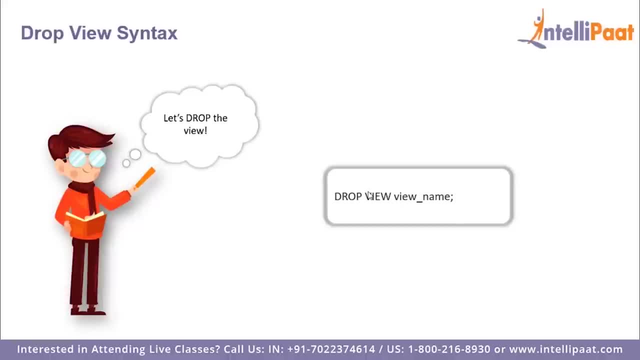 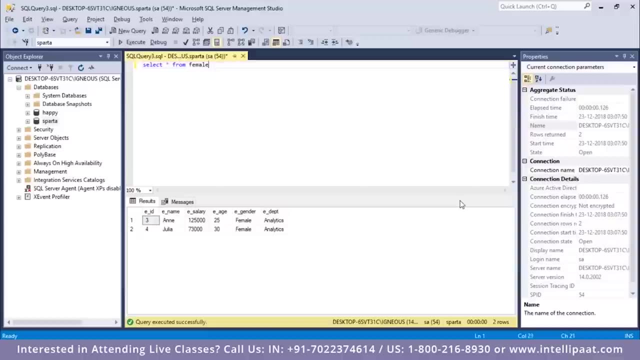 Now let's see how can we drop a view. So the syntax for dropping a view is pretty simple. All we have to do is give the keywords drop view and then give the name of the view. So let me drop this. female employees view. 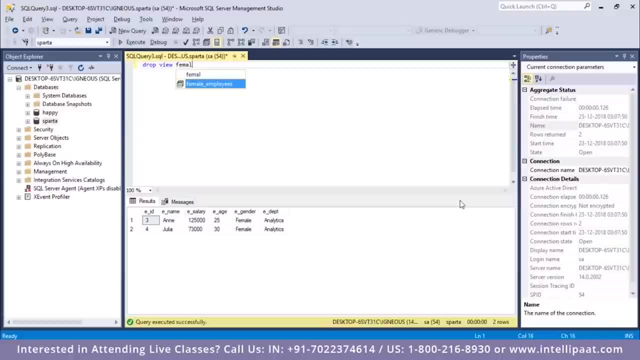 I will type in drop view and then I will give in the name of the view, which is female employees. I'll put a semicolon: execute. So again, commands have been completed successfully. So now let me see if the view exists or not. 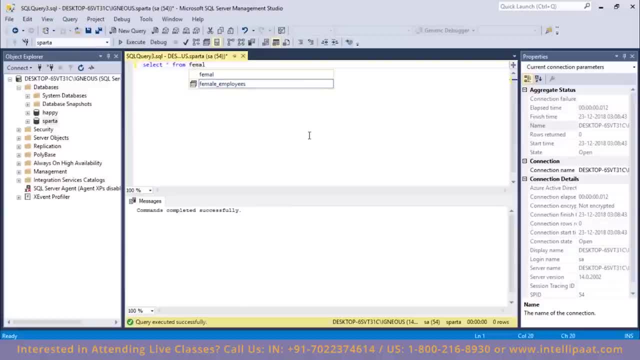 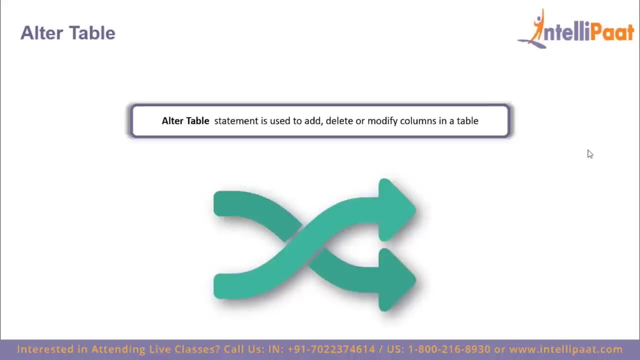 Select star from female employees, Execute. And this is the result which we get: invalid object named female employees. And we get this because the view female employees has been dropped. So this is how we can work with views. So the alter table statement is used to add, delete and modify columns in an existing table. 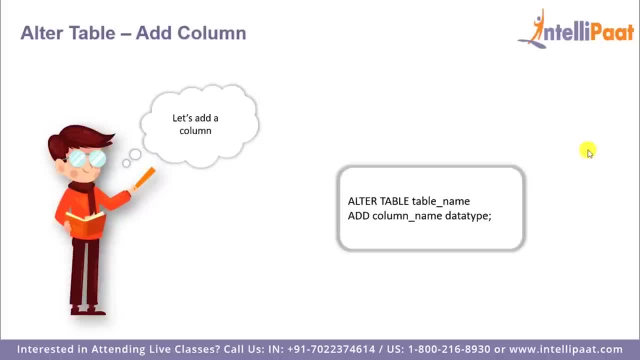 Now let's have a look at the syntax to add a column to an existing table. So we'll start off by giving the keywords alter table, then we'll give the name of the table. After that we'll give the add keyword And then we'll give the name of the table. 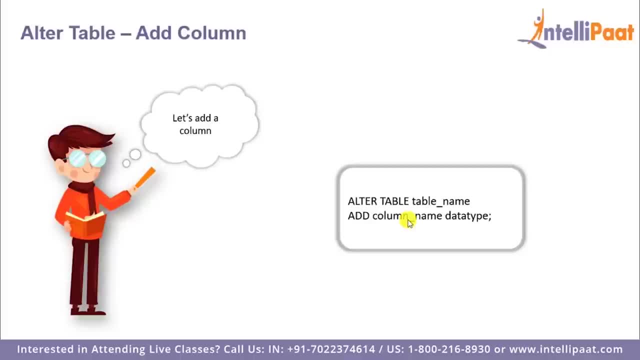 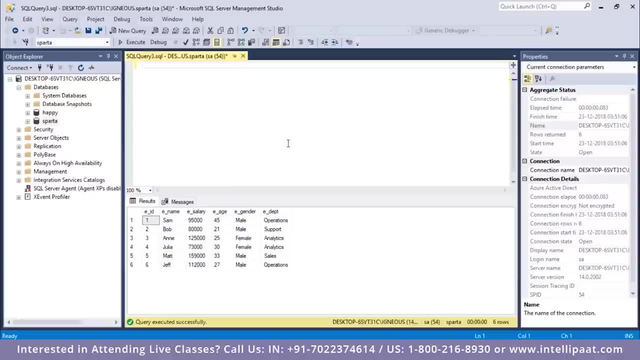 And the name of the column which you want to add to our table. And finally, we'll have to assign a data type to this new column. So to our existing employee table I'll add a new column, date of birth, using the alter. 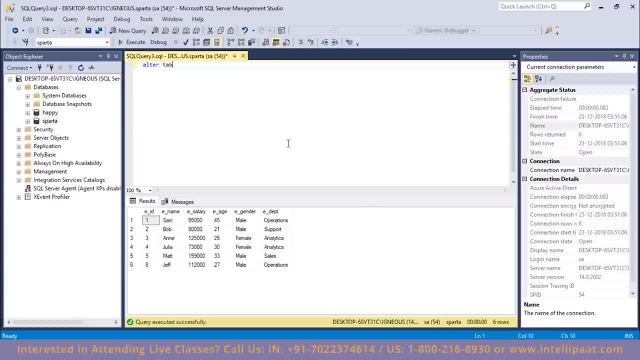 table statement. So let me start with the syntax alter table. then I'll give the name of the table, which would be employee. After that I will give in the add keyword and then, given the name of the column, So I'll name the new column to be E-D-O-B. 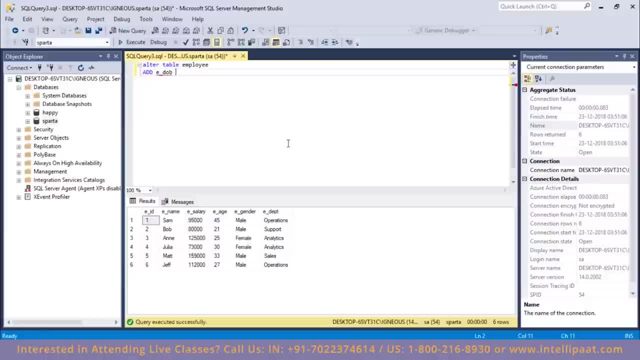 E-D-O-B, which would stand for employee date of birth, And then I'll finally give the data type of this new column, So the data type would be date. So I'll put a semicolon, I'll hit execute. So commands have been completed successfully. 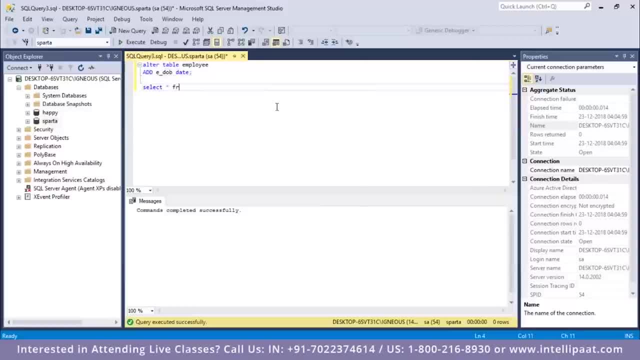 Now let me have a glance at the modified table Select star from employee Right Right. So we see that this new column, employee date of birth, And then I'll give the new column E-D-O-B. E-D-O-B has been added. 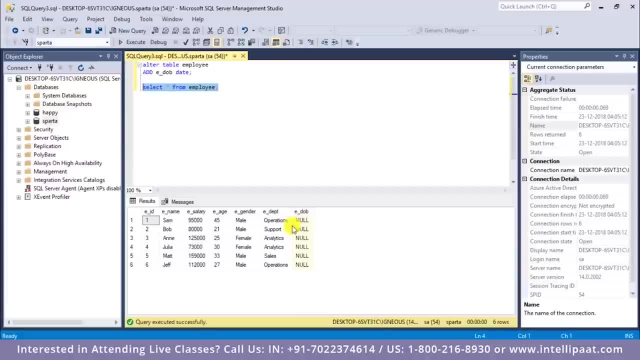 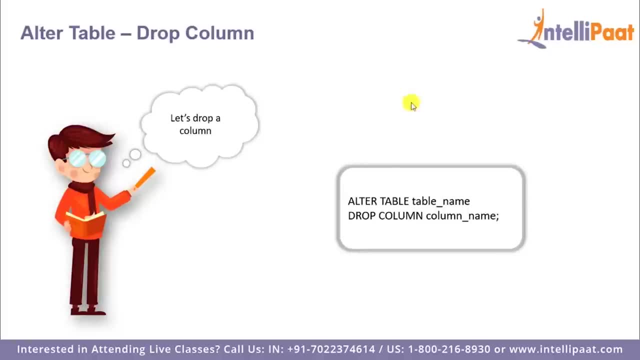 So you see that this new column, employee date of birth, has been added to our employee table. Now let's see how can we drop a column from a table Again. we'll start off by giving the keywords alter table and then we'll give the table. 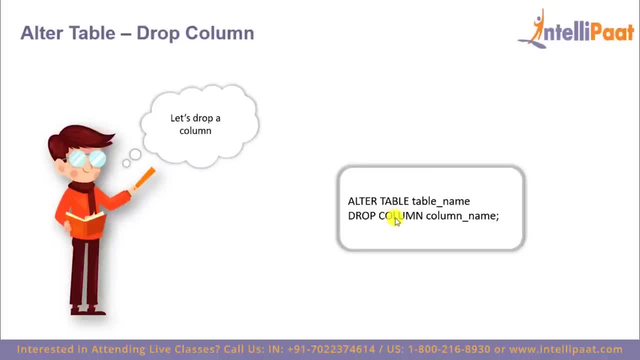 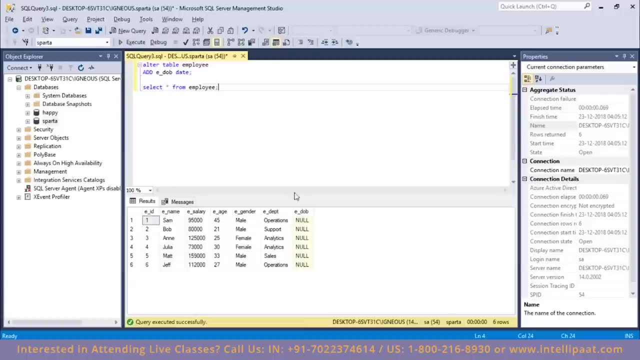 name. After that we'll give the keywords drop column and specify the name of the column which is to be dropped. So I want to drop this new column which I have just added to this employee table, So let me write the command for that. 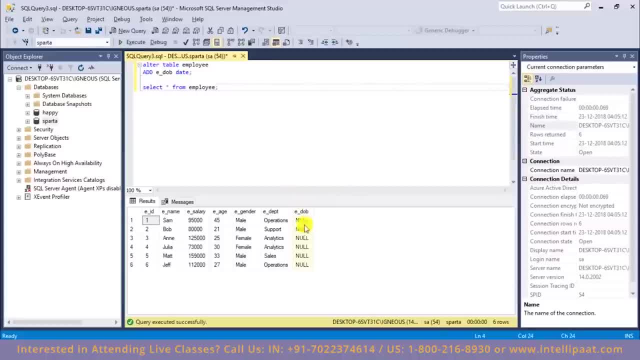 So I want to drop this new column E-D-O-B which I have just added to this employee table. So let me write the command for that alter table and then the name of the table is employee- Alter table and then the name of the table is employee. 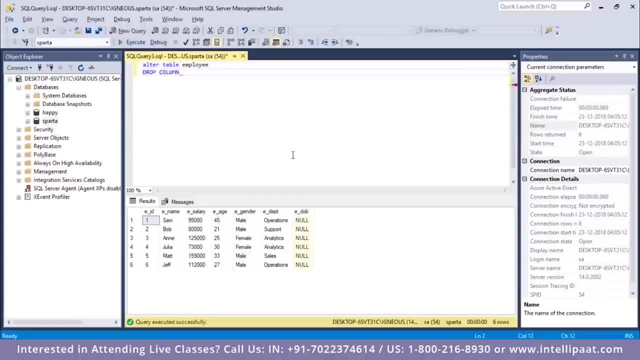 After that I will give in the keywords drop column. and I want to drop the E-D-O-B column from this employee database. I'll put a semicolon, hit execute. So again, the commands have been successfully executed. Let me have a glance at the modified table. 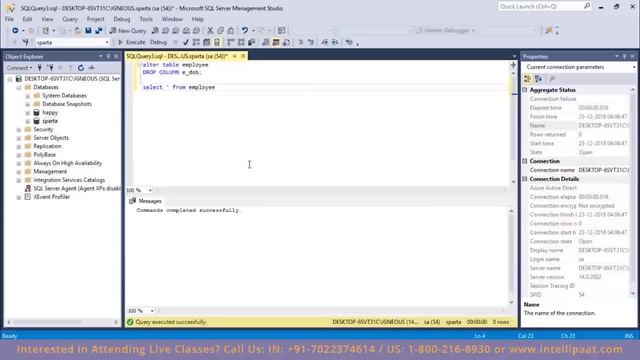 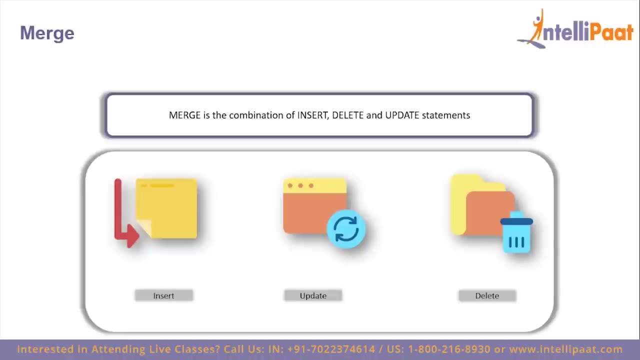 Select star from employee. I'll put a semicolon: execute. So again, the new column which we had just added has been dropped. So this is how we can do this. Now we can work with the alter table statement, So the merge statement helps us to perform insert, update and delete in just one statement. 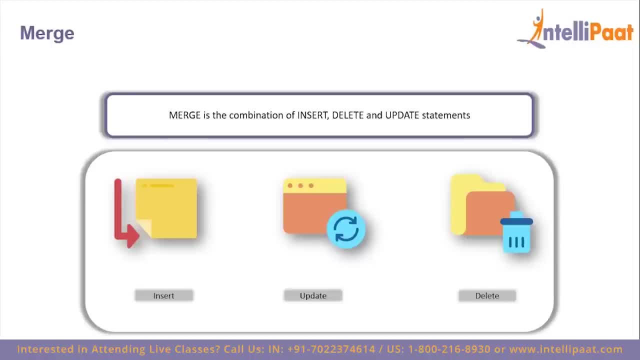 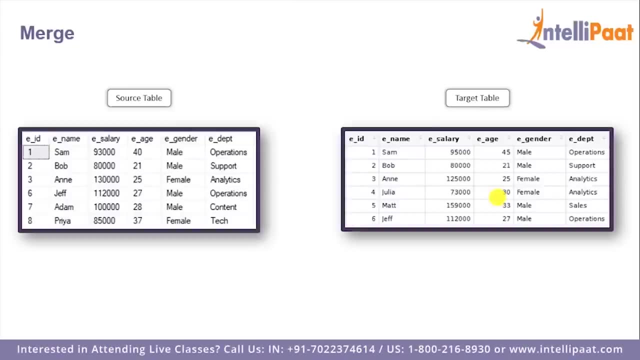 This means we no longer require multiple statements to perform insert, update and delete, And for the merge statement we require two tables: a source table and a target table. So the source table basically contains all the changes which are to be applied to the. 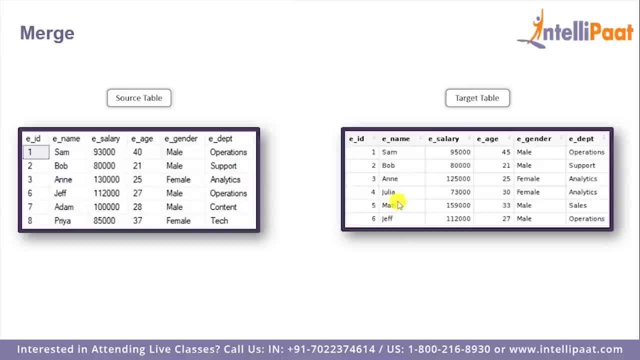 target table And the target table is that table upon which we'll be implementing all the changes Now. the merge statement Basically joins the target table to the source table using a common column. in both the tables, And based on how the rows match up, we can perform insert, delete and update operations. 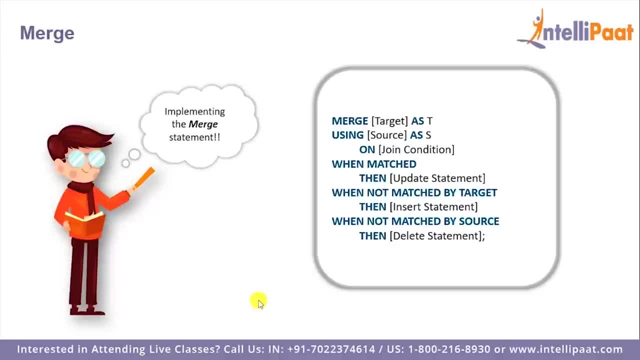 on the target table. Now let's have a look at the syntax of the merge statement. So we'll start with the merge keyword and then give the name of the target table and assign it an alias using the as keyword. Then we'll type, using and give the name of the source table and also assign it an alias. 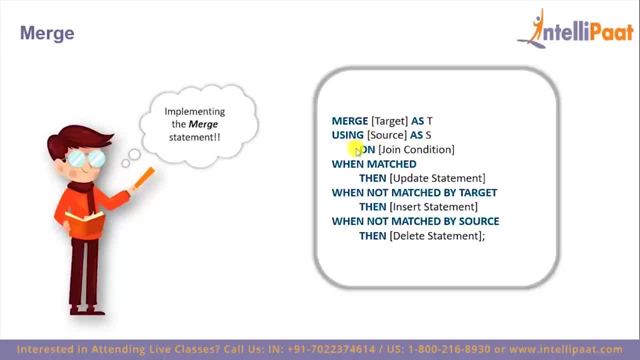 using the as keyword again. After that we'll type on and then set the join condition. Then we'll type when matched. So if the rows match up based on the join condition, then we'll go ahead and update the target table. After that we check when not matched by target. 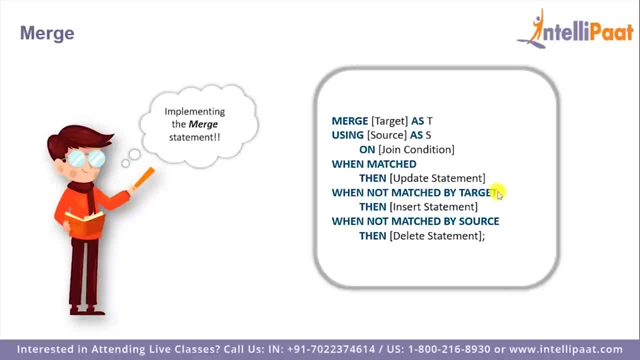 So this basically means that if there are some rows which are present in the source table but not in the target table, then we'll go ahead and insert those rows from the target table And finally, we check when not matched by source. So here we are checking if there are some rows which are present in the target table. 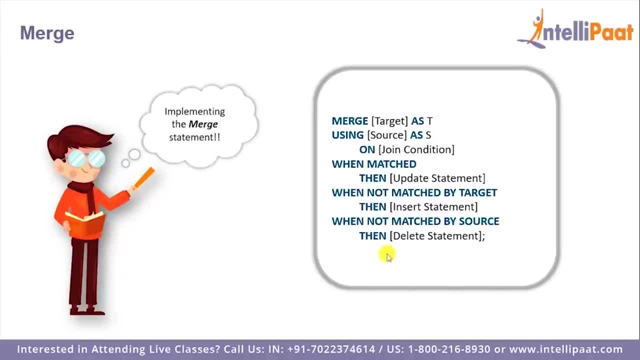 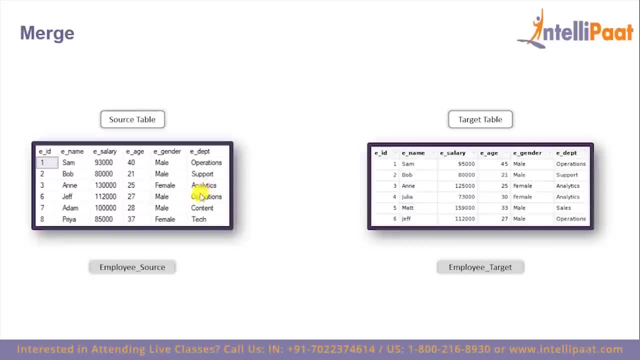 but not in the source table, then we'll go ahead and delete those rows from the target table And for the practical purpose we'll be using these two tables. So this is our source table with the name employee source and this is our target table. 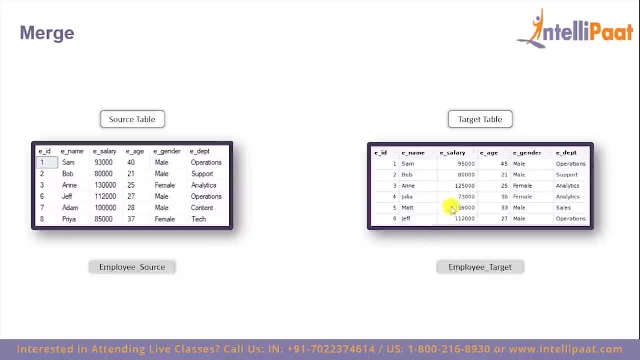 with the name employee target. So, using the merge statement, we'll be updating the esalary index. So we'll be updating the eSalary index. However, you guys can use complete and topping- Let's first nothing here- for slight sort of randomness, because we also have some. 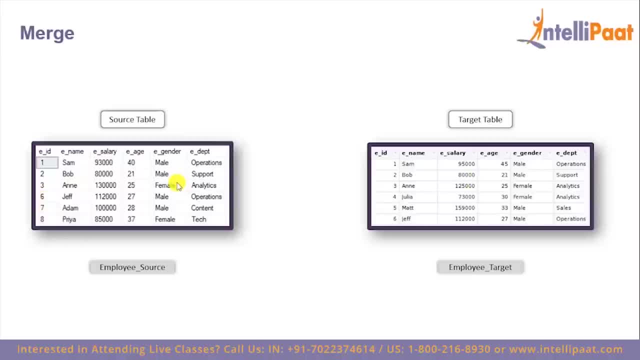 SQL: endless studies. now, Before that, we will just go ahead and hit complete, Obviously all reiterate steps. So let's go ahead and make a combination of the equals statement, So we'll add equals statement. All right, so you'll see that here we have multiple products and let's right click on. 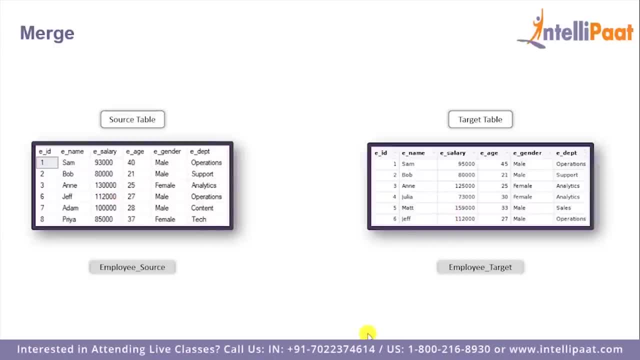 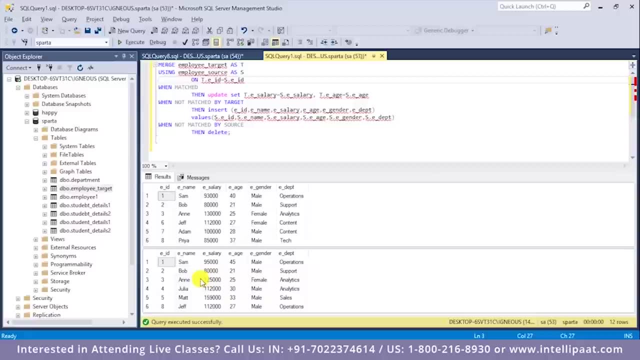 this one, And here we'll sayそれでは, And we can also just use the addition result instead. So we can just to size this out. For example, for this example, here we're going to say: we want one-alert AndroidOS and 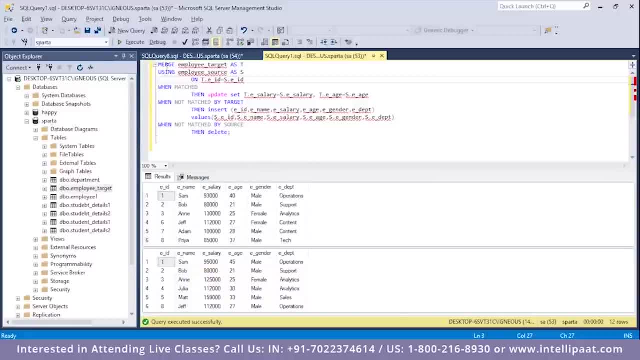 have the merge syntax to apply on these two tables. So we'll type merge and then give the name of the target table- employee target- we'll assign it an alias t. Similarly, we'll give the employee source table and then assign it an alias. 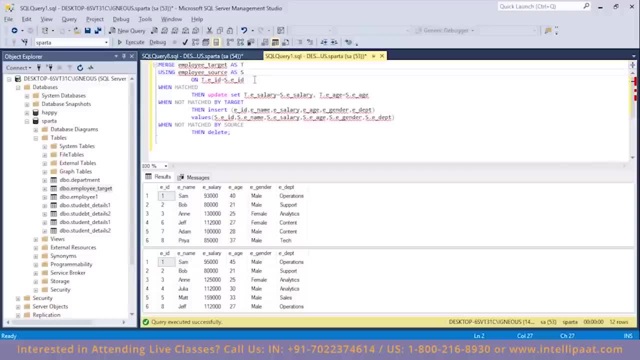 s. After that we'll type on and then set the join condition. So join condition is t dot eid is equal to s dot eid. So we've basically set the join condition on the employee ID columns of the source table and the target table. Then we have when. 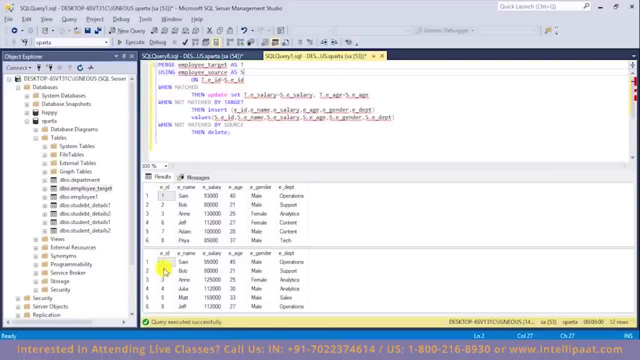 matched. So if there is a match between the rows of these two tables, then we'll go ahead and update the target table. So here in the update statement we have: t dot e salary equals s dot e salary and t dot eh is equal to s dot eh. So if the 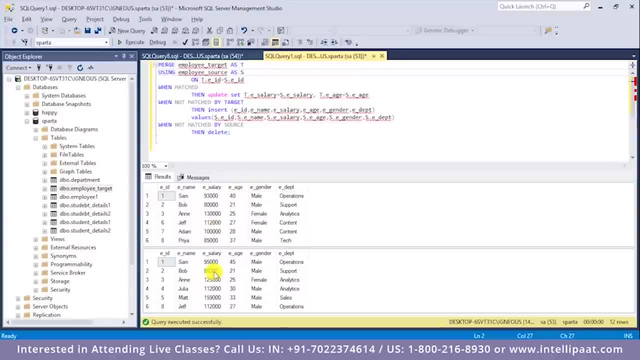 records match, then I'll be setting the value of the salary column of the target table to be equal to the values of the salary column of the source table. Similarly, I'll also set the values of the age column of the target table to be equal to the values of the age column of the. 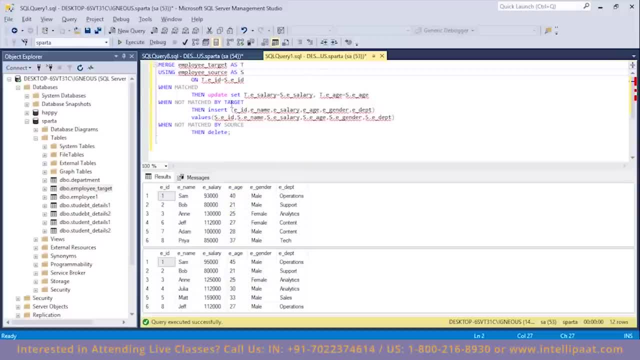 source table And then we have when not matched by target. So here we are checking if there are some rows which are present in the source table but not in the target table, And if that is the case, we'll go ahead and insert all of those into these columns of the target table and the values would be. 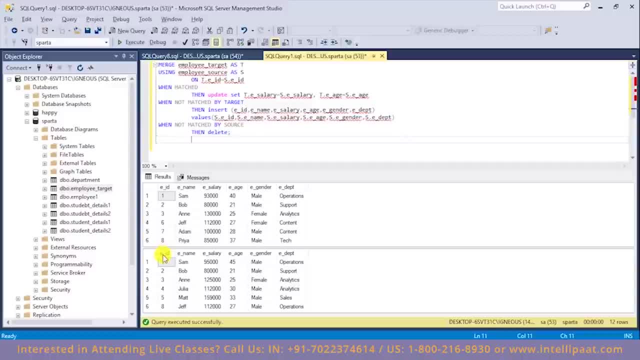 coming from the source table. So this employee ID column from the target table would be getting the values from the employee ID column of the source table. Similarly, this employee name column of the target table would be getting its values from the employee name column of this source table. And finally we'll 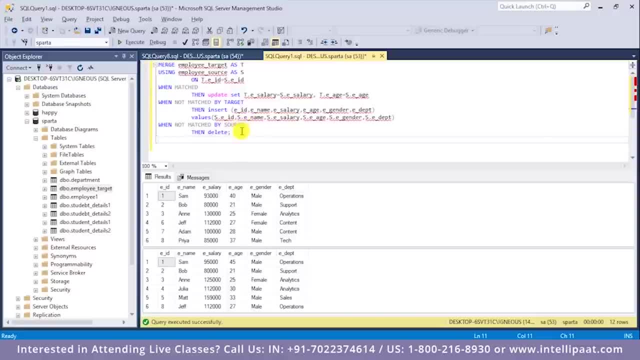 check when not matched by source. So if there are some rows which are present in the target table but not present in the source table, then we will just delete all of those rows. So I'll select all of this and I'll click on execute. So 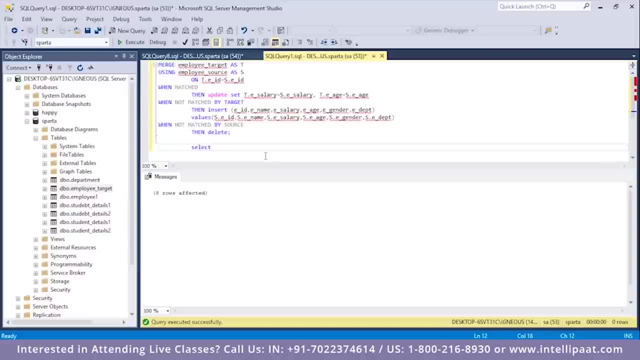 you see that eight rows have been affected. Now let me type the select statement and have a glance at the modified employee target table. Select star from employee target. I'll select this. I'll click on execute Right. so this is our modified employee target table. So we 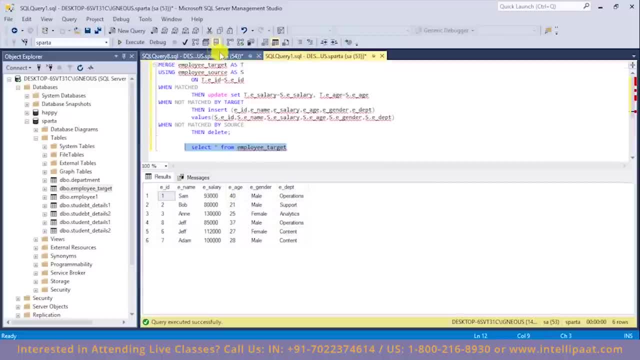 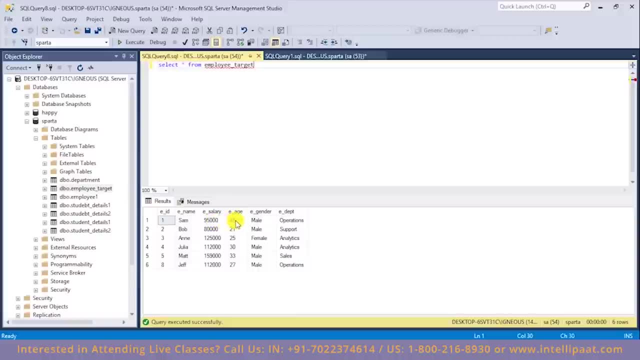 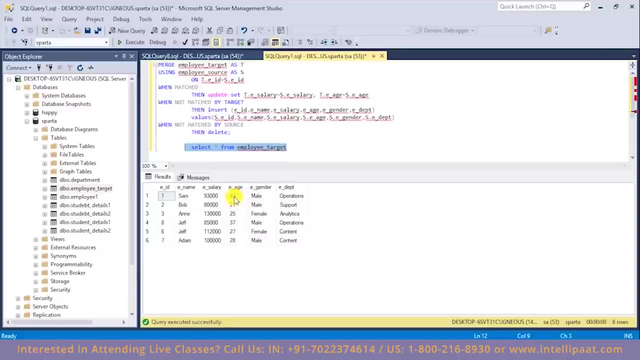 have our original employee target table over here, So let me compare these two tables. So we see that initially Sam's salary was $95,000 and his age was 45, and after applying the merge statement his salary changed to $93,000 and his 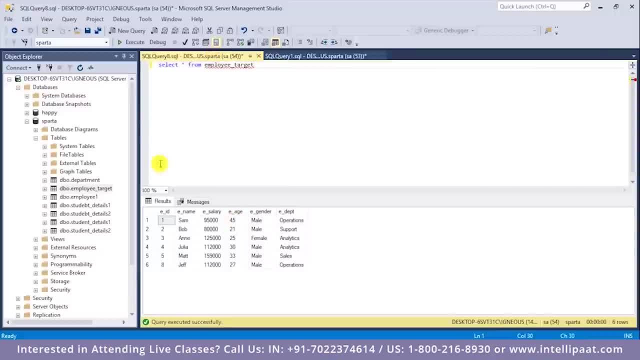 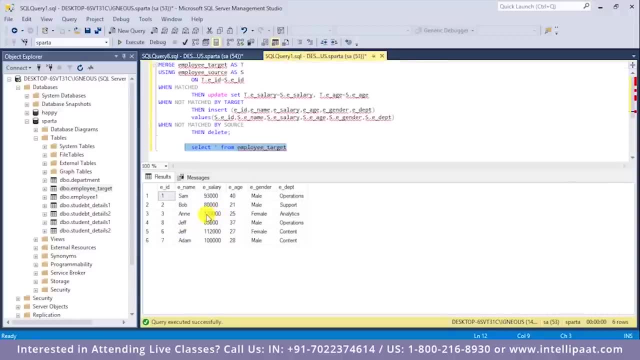 age changed from 45 to 40. Similarly, Ann's initial salary was $125,000 and after applying the merge statement, her salary changed to $130,000 and then, with the merge statement, we have also inserted the records with employee ID 7 and employee ID 8 and deleted these two records from the 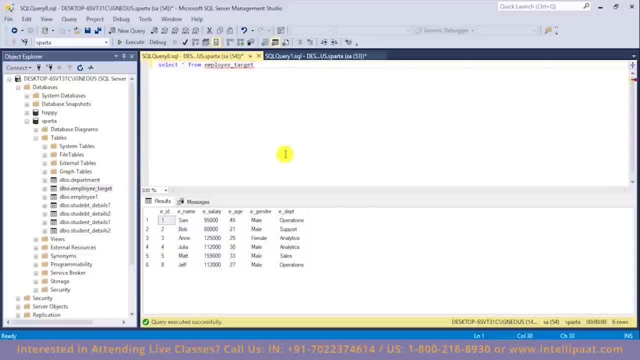 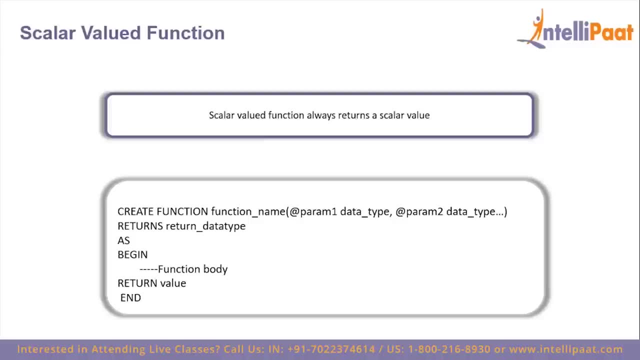 employee target table. So this is how we can work with the merge statement. So these are the two types of user-defined functions. in SQL We have scalar valued functions and table valued functions. We'll start with the scalar valued functions. So, as the name states, a scalar valued function always returns a scalar value. 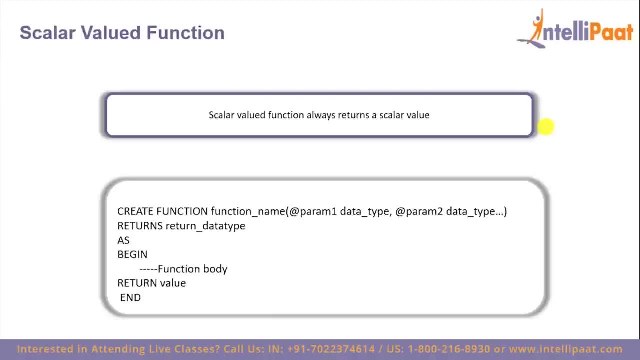 So a scalar value could be int, varcat, date and so on, and this is the syntax for a scalar valued function. So we'll type create function and then we'll give the function name and inside the parenthesis we'll specify the names of the. 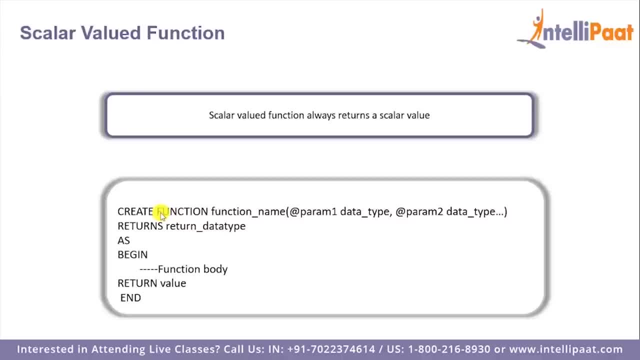 parameters and their data types. And since the function is going to return a value, we'll type the returns keyword and specify the type of data which will be returned. After that, we'll type as begin and then give the function body and then return the final scalar value. Finally, we'll use the end keyword. 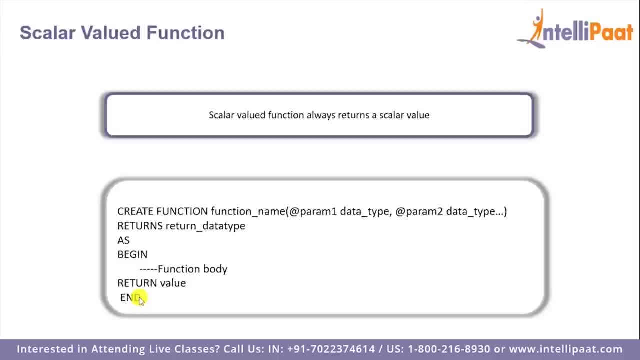 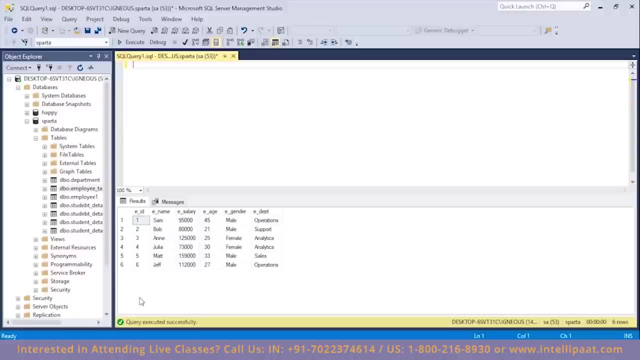 to end the function. So let's go to SQL server and create our first scalar valued function. So I'm going to create a scalar valued function which will take one integer value, add five more to the original value and return the updated value. So let me type the syntax for that Create. 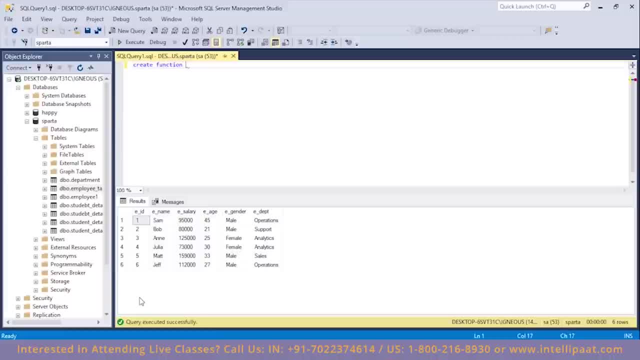 function. then I'll give the function name, which would be add phi, and inside the parenthesis I'll pass the first parameter. so I'll name the parameter to be num, and this would be of integer type. after that I'll type the returns keyword, and then the type of data which will be returning is also of integer type. after, 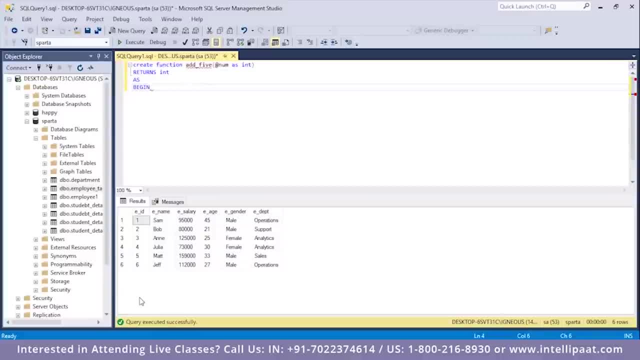 that I'll type as begin, and since all we have to do is, and since all we have to do is add 5 more to the original value, so I'll not write anything inside this. so I'll directly type the return keyword and inside this return keyword, I will. 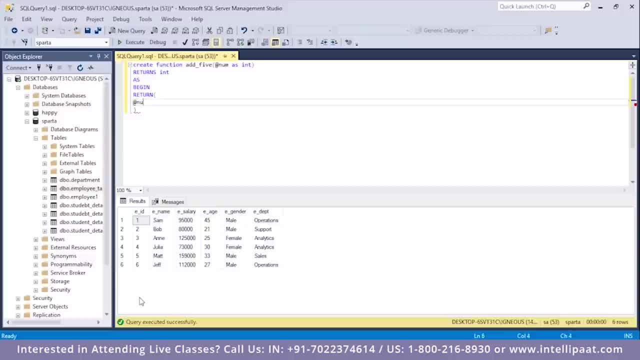 add 5 more to the parameter value. so that would be at the rate num plus 5. so what we are basically doing over here is the value which is sent as parameter inside. this function will take it and add 5 more to that value and then return. 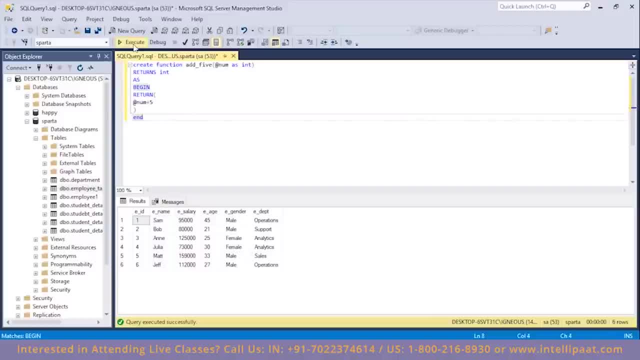 also add 5 from the new function in version 2. those who actually runs're created and it does. now is quote: is that where I have entered the default value, I'll type it in front hereướ Ctrl M to failed. I have to shaking to. 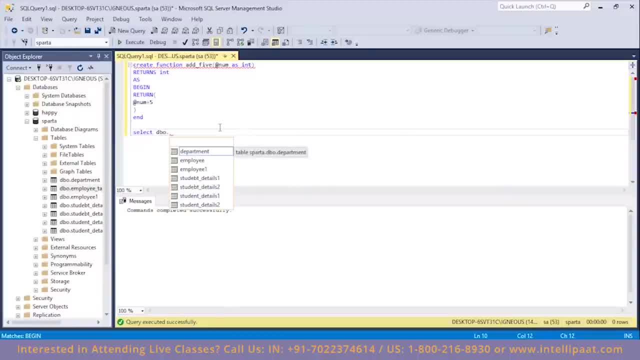 pass to what I called the error run and I can say: got little turned off, but that is all OK. so then now I'm going to have to specify as Bardingatri here, because it has right, so that every time this gets removed. so since I've got, 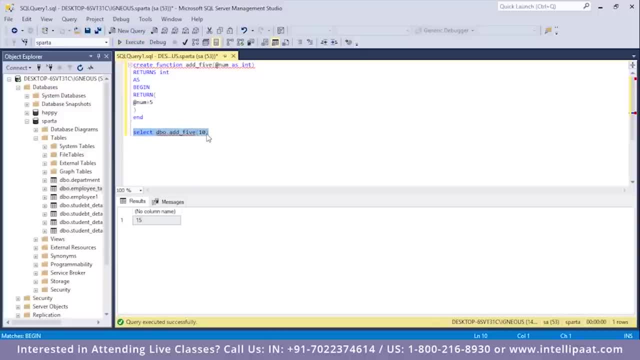 right. so we see that this function works properly. so I've sent 10 and the result which you've got is 15. similarly, let me send 100 as the parameter. now I'll select, I'll hit execute right. so the value which is returned is 105. so this: 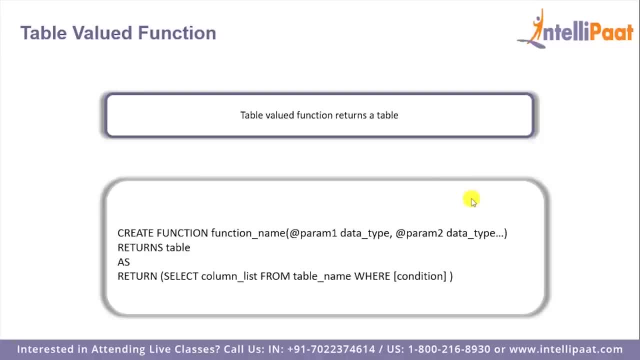 is how we can create a scalar valued function. then we have table valued functions. so these table valued functions return a table instead of a scalar, and this is the syntax for a table valued function. so here the return type is table. so after the returns keyword we'll type in table, because we 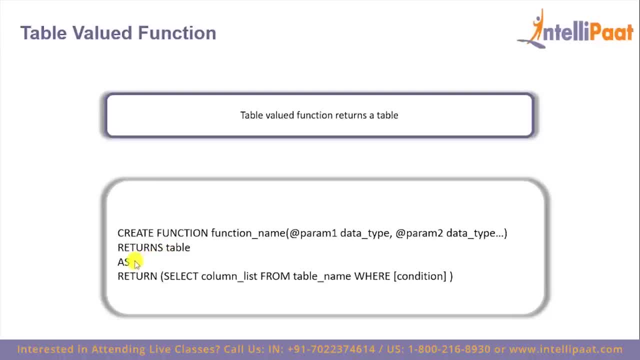 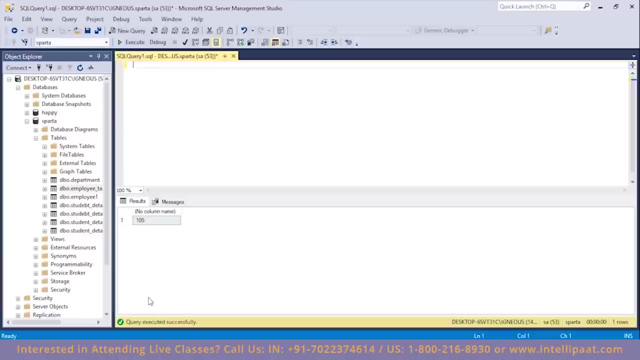 are supposed to return a table. after that, we'll give the keywords as return and then given the select statement. now you need to keep in mind that there are no begin and end keywords for the table valued function. so let's go to SQL server and create a first table valued function. now I'll be creating a function. 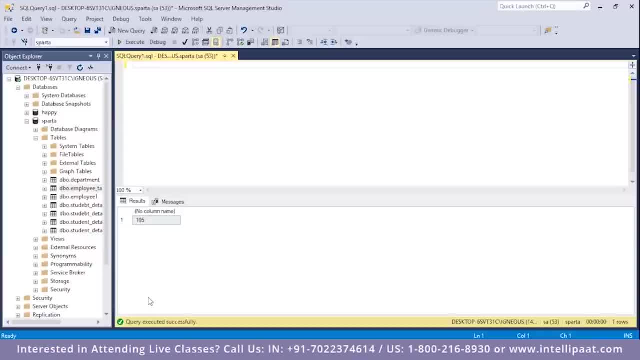 which would help me to individually extract the male employees and the female employees from the employee table. so before I do that, I'm going to create a function which would help me to individually extract the male employees and the female employees from the employee table. so before I do, 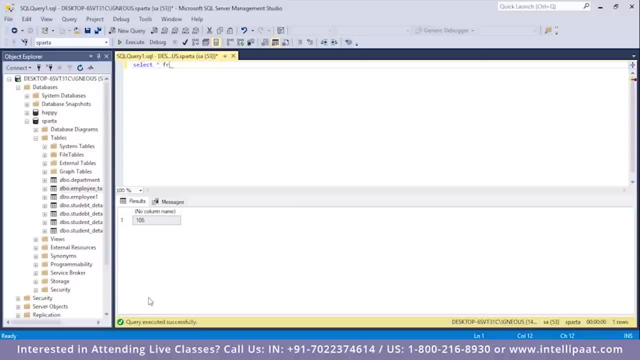 that let me actually have a glance at the employee table first. so I'll type select star from employee right. so we have this employee table right in front of us. now let me go ahead and create the command. so again, I'll type create function and then I'll give the name of. 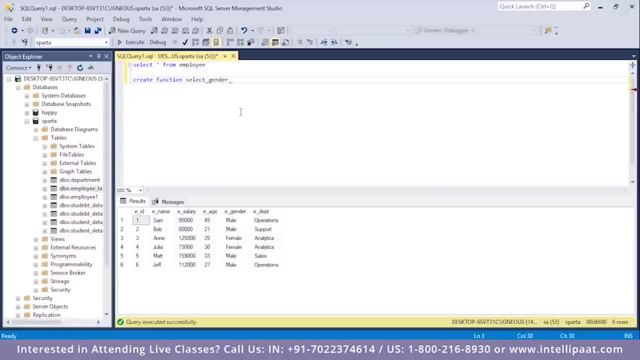 the function, which would be select gender. now, inside the parenthesis, I will pass in the parameter. so I'll name the parameter to be gender and this would be of varchar type, so as varchar, and the length would be 20. after that I'll give the returns keyword and, since this is a table valued function. 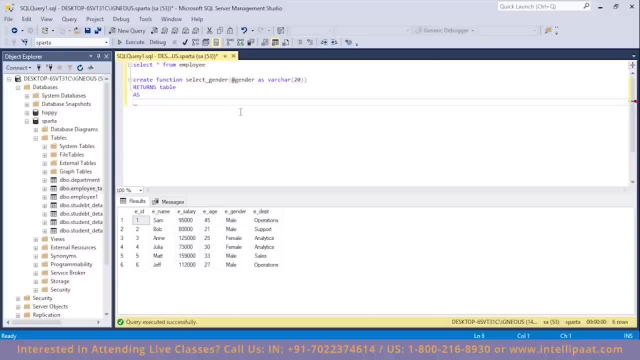 the return type would be table. so I'll type as return and then given parenthesis, and inside the parenthesis I will give my select statement. so the select statement would go something like this: select star from the employee where he gender is equal to, at the rate gender. so this e gender is basically the e gender column from the. 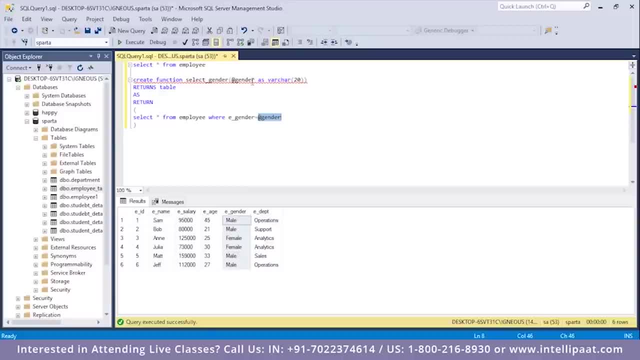 employee table. in this, at the rate, gender is the parameter which will be passing inside this function. so let's say, if the user passes the value male inside this function, then we'll be extracting all of the records where the gender value is male. similarly, if the user passes the value 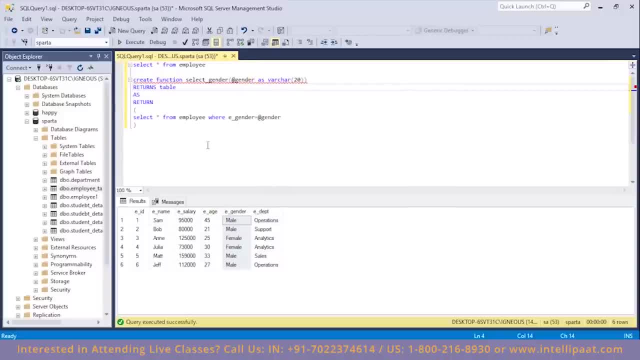 female inside this, then we'll be extracting all the female employees from this table. so let me select this, let me hit execute. right, so we have also created this select gender function. so now, using this function, let me extract all of the male employees from the employee table. so to do that, the syntax 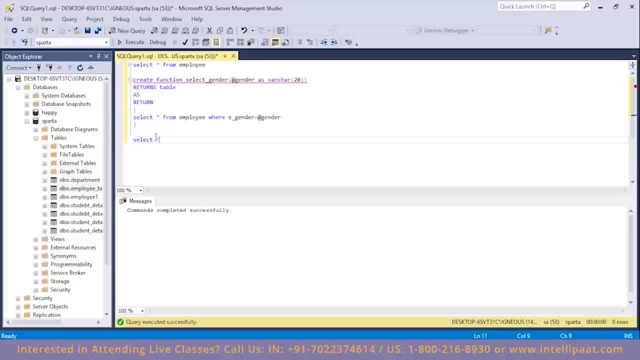 would be a bit different. select star from and then I'll type DBO dot and then give the name of the function, which would be select gender, and inside the parenthesis I will pass in the value and since I want all of the male employees, I'll type male over here, right? so I'm typing select star from this because 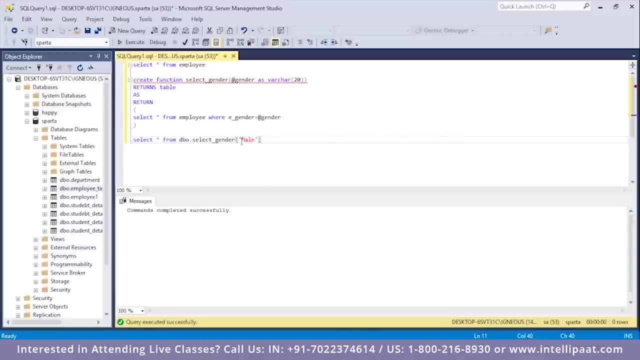 this will basically return a table, and from the table which is returned, I would want all of the records. so let me select this. I'll hit execute right. so we have successfully extracted all of the male employees from the employee table. similarly, if I'd have to extract all of the female, 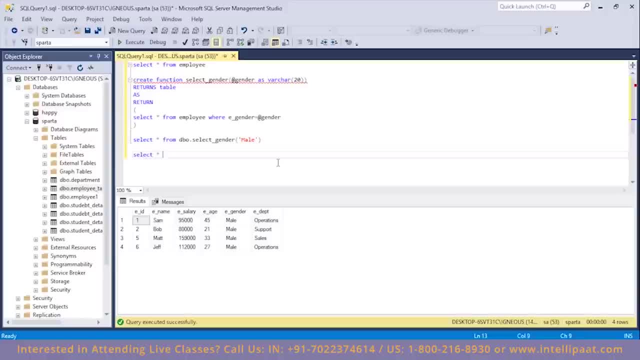 employees. the syntax would be similar, so I'll type select star from, and then I will type DBO dot select gender, and then I will pass in the value female, I will select this, I'll hit execute. so again, we have successfully extracted the female employees from the employee table. so this is how we can create table. 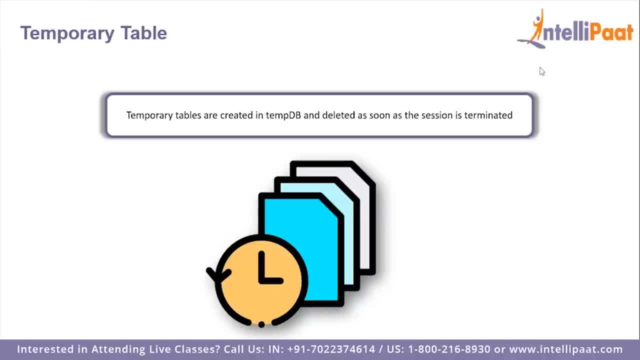 valued functions in SQL, so temporary tables basically help us to store and process intermediate results. now these temporary tables are created in the temp DB and are automatically deleted when they're no longer used. so the temporary tables could be very useful in cases wherever we need to store temporary data, and this is the syntax to create a. 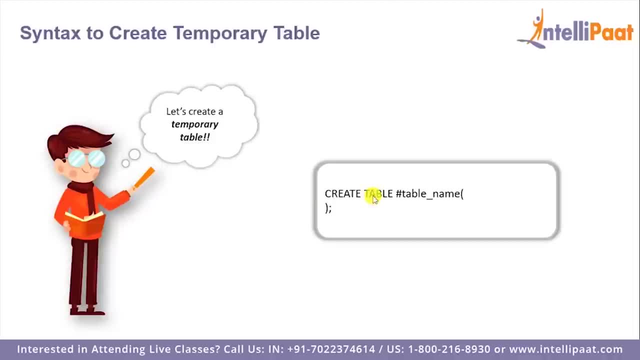 temporary table. so first we'll give the keywords create, table and before we give the name of the temporary table, we'll precede it with a hash. so this hash symbol will give us the name of the temporary table and then we'll give the hash symbol. basically signifies the table which we are creating is temporary. so 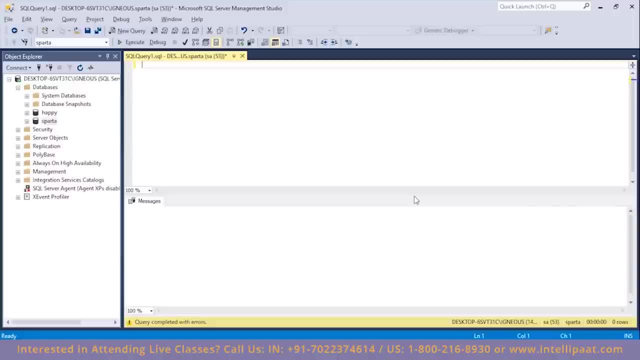 let's work with some temporary tables now. so let me create a temporary table with the name student, which has two columns: one is student ID, another is a student name. so I'll type create table, I'll put in the hash symbol and then give the name of the temporary table, which would be student. so now this would have just two. 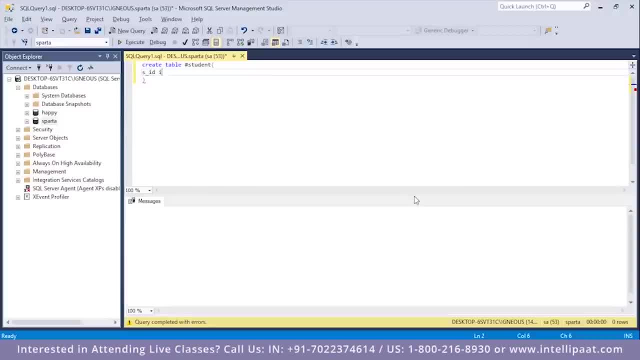 columns: first would be student ID, so s ID, and this is of integer type. then we have the student name, so I'll name the column as s name and this is of variable length character of max length: 20, so I'll put a semicolon over here and 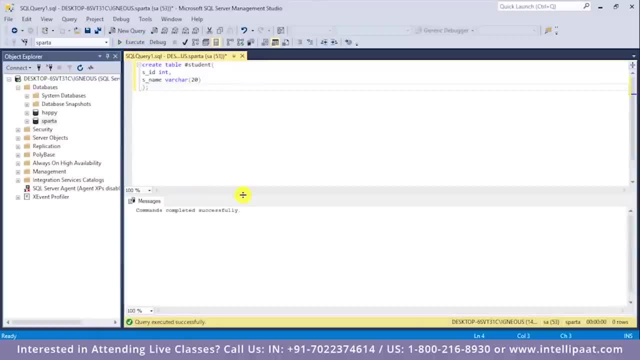 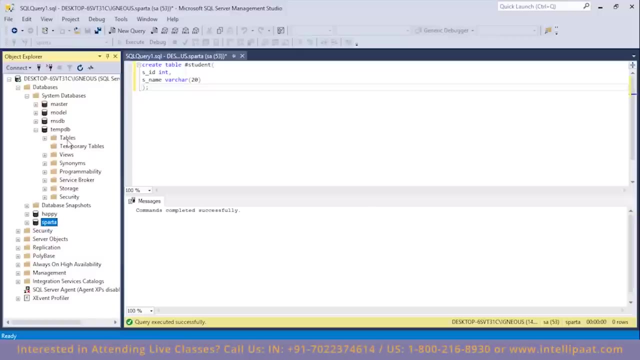 I'll hit execute right, so see that the commands have been completed successfully. now I've already stated that this temporary table is stored in the temp DB, so let me show you guys where the temp DB is actually. so you'd have to click on the system databases and over here you will see the temp DB and inside temp DB. 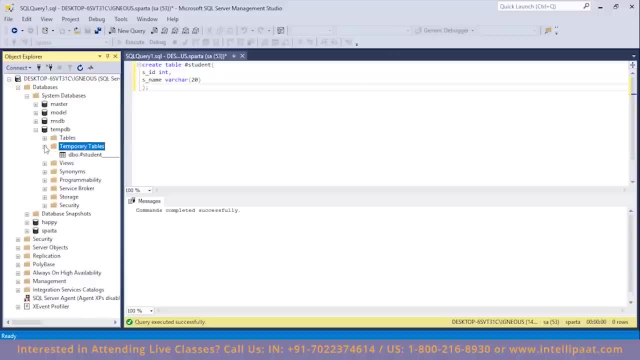 you have all of the temporary tables, so let me refresh this right so we see that we have this temporary table student inside our tempdb database now. similarly, i can also use the select statement with this temporary table which i've created. so i'll type select star from and before giving the. 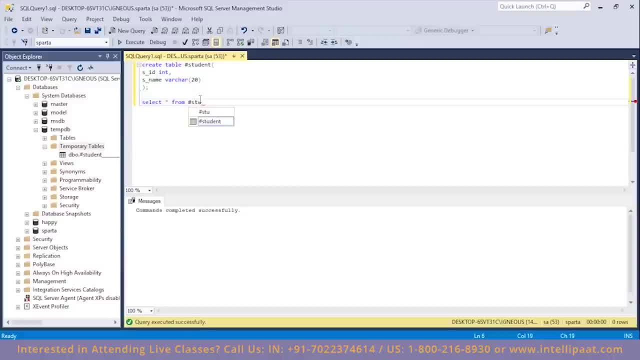 name of the table. i need to give the hash symbol and then give the table name, which would be student, right? so let me select this and i'll click on execute, right? so this is our table and we don't see any values because we haven't inserted any into this table. so, similarly, we can also use: 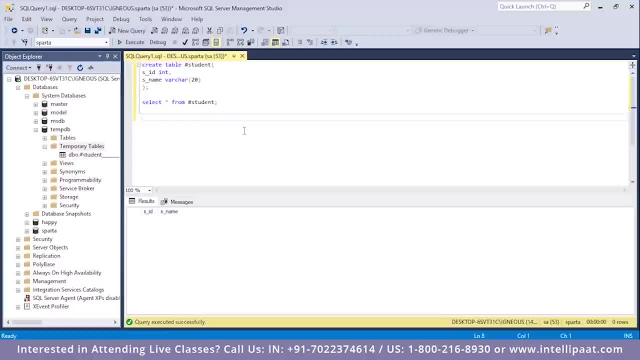 the insert command and insert some values into this temporary table. so i'll type insert into. after that i'll give the hash symbol and then give the name of the temporary table, which would be student. i'll follow it up with the values keyword and then give the values which are to. 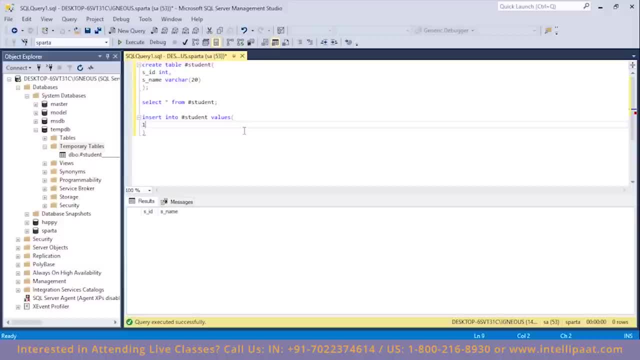 be inserted inside this. so, for example, if i want to insert some data, then i save it inside. the First is the student ID, which will be 1, then I'll give the name of the student. So name of the student is Sam. So again, I will select this and I'll click on execute. 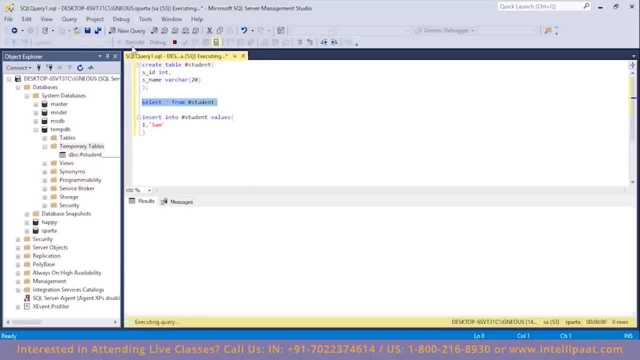 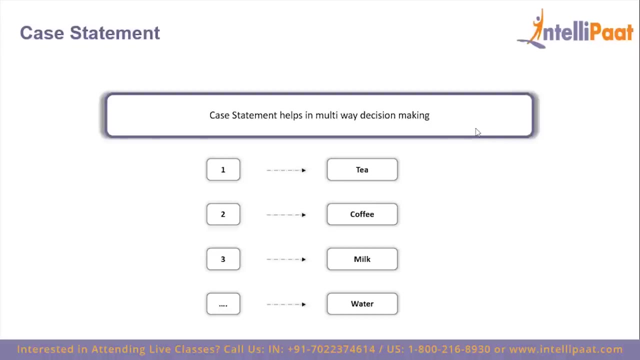 So one row has been affected. now I'll select this line again and I'll hit execute. So we have successfully inserted this record inside our temporary table student. So this is how we can work with temporary tables in SQL. So the SQL key statement helps us in multi-way decision making. 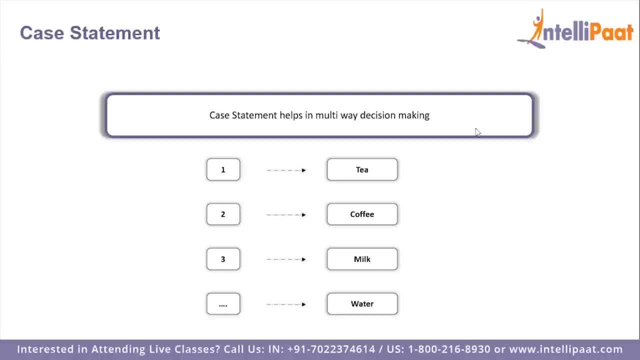 So let's take this example to understand key statement properly. Let's say there are 10 buttons, starting from 1 to 10.. So if the person selects 1,, then he wants tea. If he selects 2,, then he wants to order coffee. 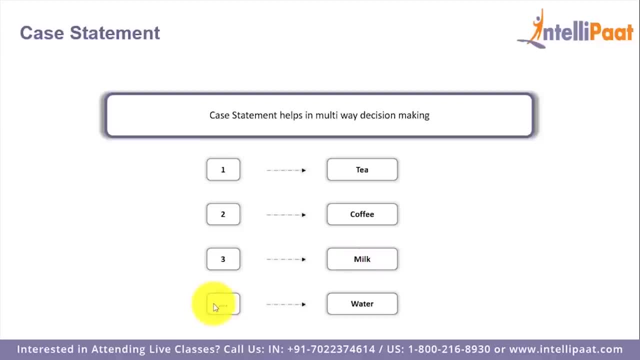 Similarly, if he selects 3,, then he wants milk, And for any other case the person will order water. So this is basically how the key statement works. So the key statement goes through conditions and returns a value when the first condition is met. 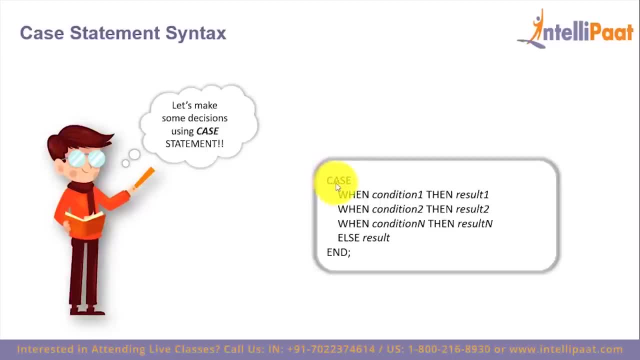 And this is the syntax for the key statement. So we'll type in case, following which we'll give the when keyword and give the first condition. After that we'll type then and specify what will happen if this condition is satisfied, And we'll do the same for the rest of the conditions. 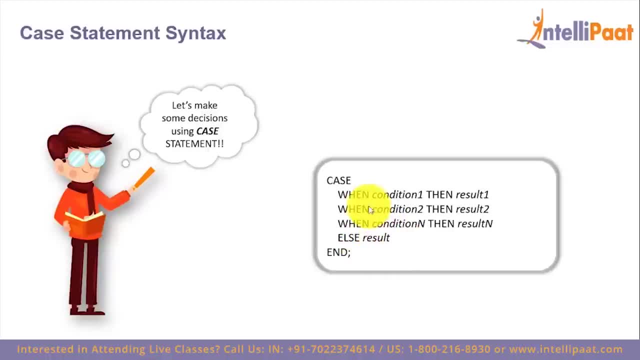 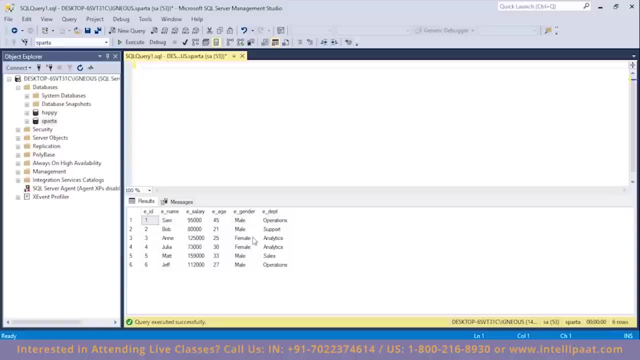 After that we'll type else and state what will happen if none of the above conditions are satisfied. Finally, we'll give the end keyword. Now let's go to SQL server and start working with the case statement. So I'll check some conditions using the case statement. 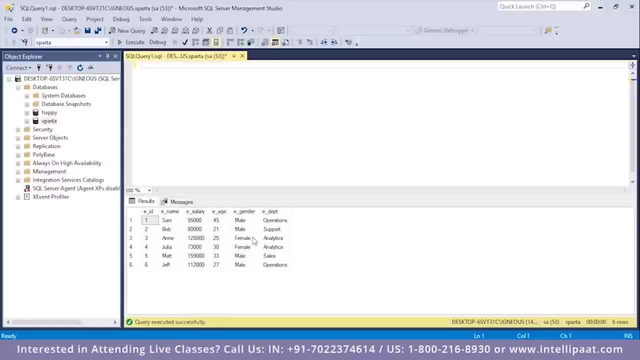 So first I'll check if 10 is greater than 20. And if this evaluates to true, I'll just print 10 is greater than 20.. After that I'll check if 10 is less than 20. And if this condition evaluates to true, I'll print 10 is less than 20.. 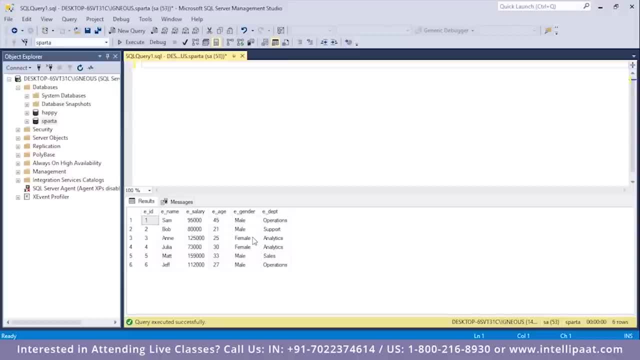 And if none of these two conditions evaluate to true, I'll just print: 10 is equal to 20.. So let me write the syntax for that Select, I'll give the case statement, Then type when and give the first condition, which would be 10 is greater than 20.. 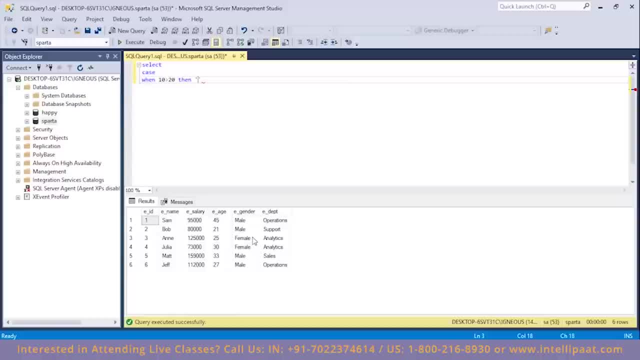 I'll type then And state what will happen If this condition is evaluated to true. So I'll just print 10 is greater than 20.. Then I'll type when And then state the second condition, which would be 10 is less than 20.. 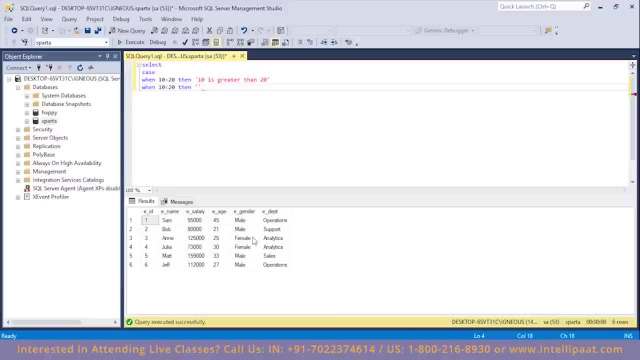 I'll type then. And if this condition evaluates to true, I have to print 10 is less than 20.. And if none of these conditions evaluate to true, I'll type else And just state 10 is equal to 20.. 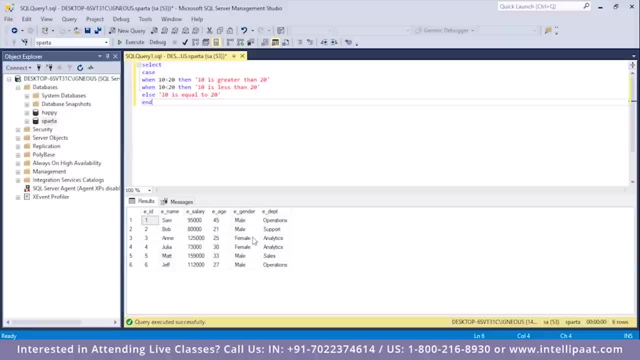 And I'll finish off the case statement with the end keyword. So let me hit execute So you get the result: 10 is less than 20.. So we get this result because the first condition has been evaluated to false, Because obviously 10 is not greater than 20.. 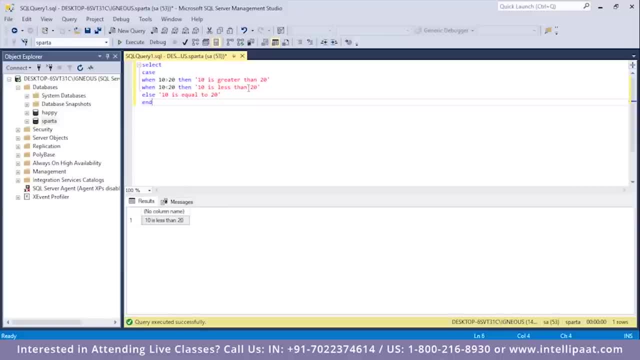 And since 10 is less than 20, this has been evaluated to true And we print: 10 is less than 20.. So now let's also implement this case statement on top of our employee table. So before we do that, let us actually have a glance at the employee table. 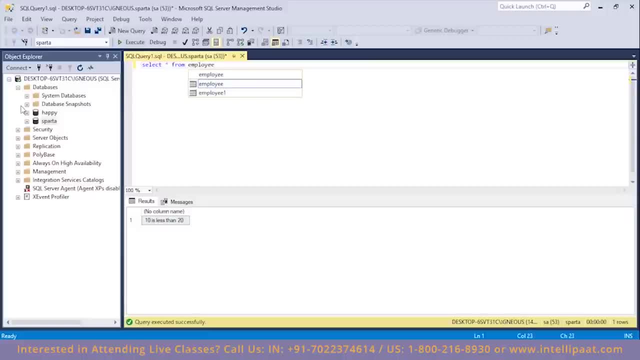 So I'll type select: start from employee Right. So this is our employee table. Now, using the case statement, I would want to add a new column grade which would be dependent on the salary column. So if the salary is less than $90,000, the grade would be C. 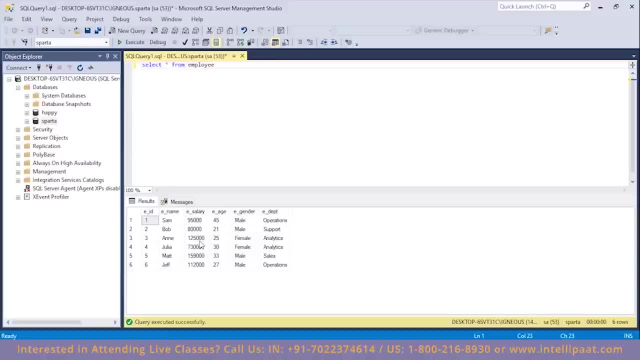 If the salary is between $90,000 and $120,000, the grade would be B, And if the salary is greater than $120,000. $90,000, the grade would be a. So let me write the syntax for that. So I'll type select and I want all of the columns from the employee table. 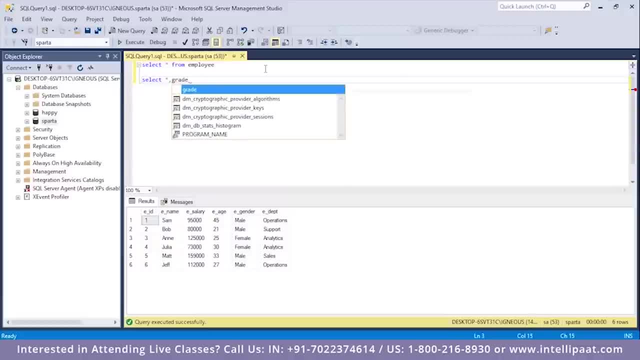 I'll type start and I'll add a new column, grade, and I'll be getting the values in this column with the help of the key Statement. so I'll type case and then type the when keyword and give the first condition. So the first condition would be: e salary is less than. 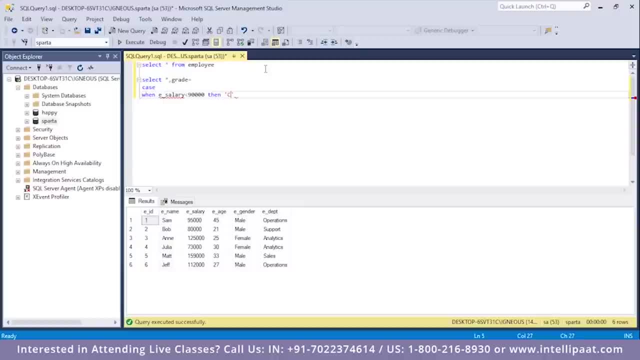 $90,000 and if this evaluates to true, The grade would be C. I'll type one and say the second condition. So the second condition would be if e salary is less than $120,000. so here, if the first condition is evaluated to false, then it would mean the salary is greater than. 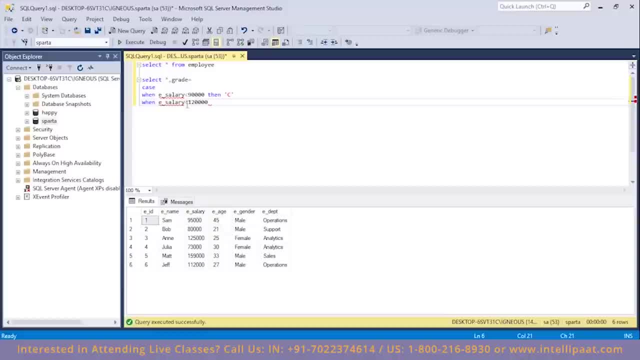 $90,000, and after that we'll check if the salary is between $90,000 and $120,000 and if that evaluates to true, The grade would be P, and if none of these conditions Evaluate to true, That would mean The salary is greater than hundred and twenty thousand dollars. 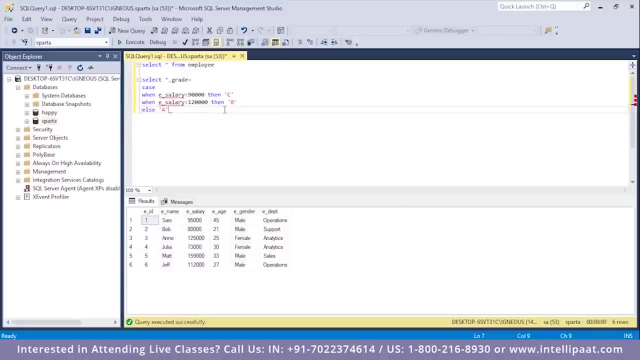 so I'll type else and then the grade which I want is E and I'll finish off this case statement with the end keyword: and I want all of this from the employee table. So I'll type from and then give the name of the table which would be employee. 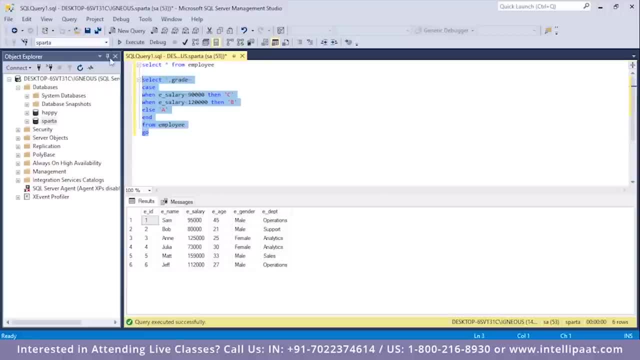 I'll type go, I'll select all of this and I'll hit execute Right. So we see that this new column grade has been added to the employee table and this grade column is dependent on the Salary column. So here we see that the salary is between ninety thousand dollars and hundred and twenty thousand dollars. 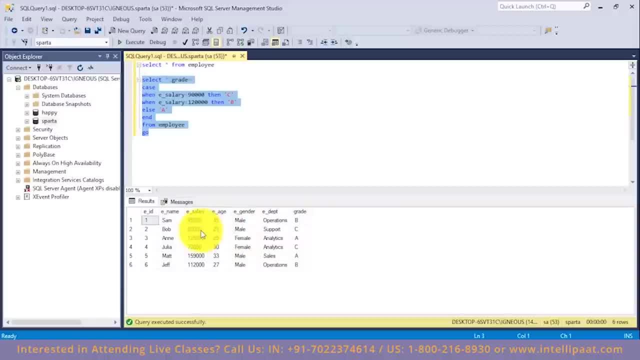 That is why the grade is B. here The salary is less than ninety thousand dollars. The grade is C and over. here The salary is greater than hundred and twenty thousand dollars. That is why the grade is a. so This is how we can work with a case statement in sequel server. 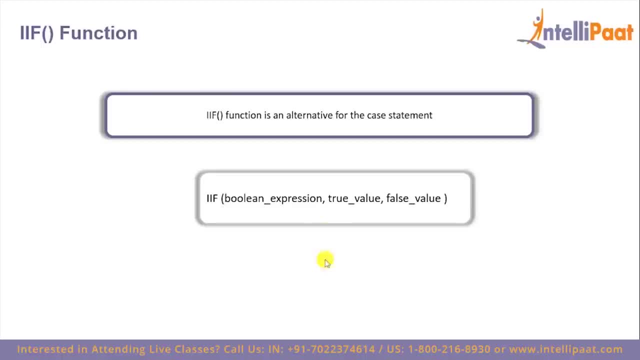 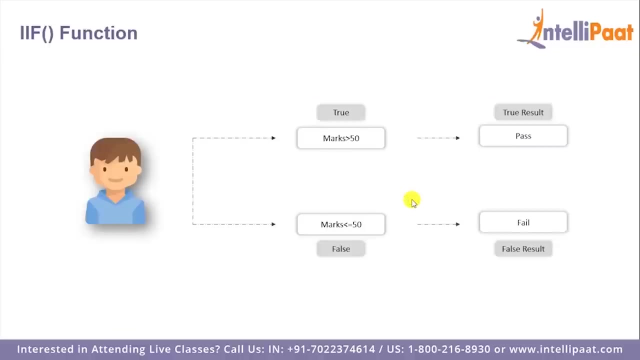 So the F function is an alternative to the case expression. This F function takes in a boolean expression as the first parameter and returns the true value If the boolean expression is evaluated to true. Similarly, returns the false value if the boolean expression is evaluated to false. For example, let's say, in the boolean expression: 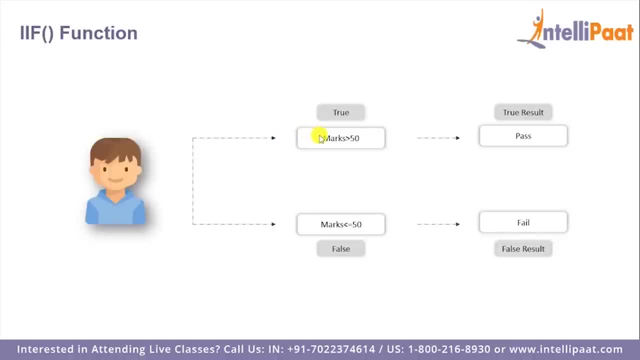 We are checking if the marks scored by a student are greater than 50, and if it evaluates to true, Will return pass, and if the boolean expression evaluates to false, will return fail. So this is how the F function works. Now let's implement this F function in sequel server. 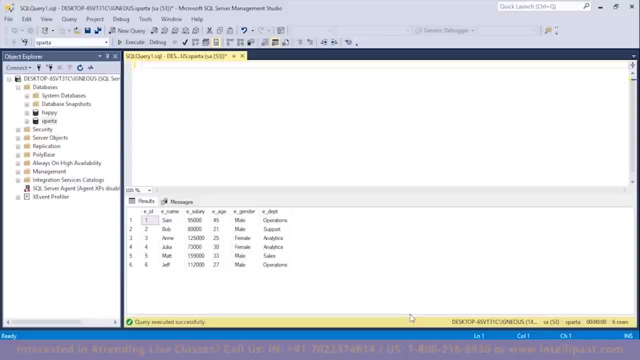 So, using the F function, I don't Check if 10 is greater than 20, and if it evaluates to true, I'll print 10 is greater than 20. on the other hand, if it evaluates to false, I'll print 10 is less than 20. 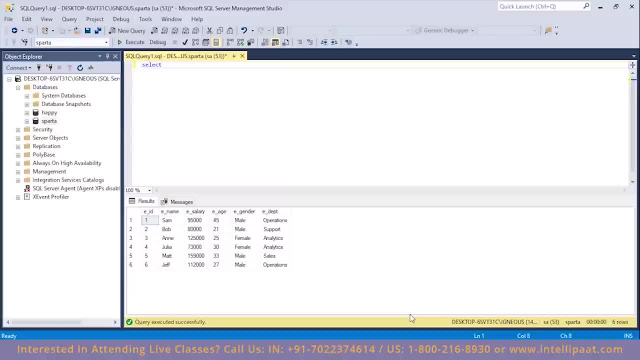 So let me write the syntax for that. I'll type select. after that I'll use the F function and pass in the first parameter, which is the boolean expression. So 10 is greater than 20, and if it evaluates to true, I would want to print. 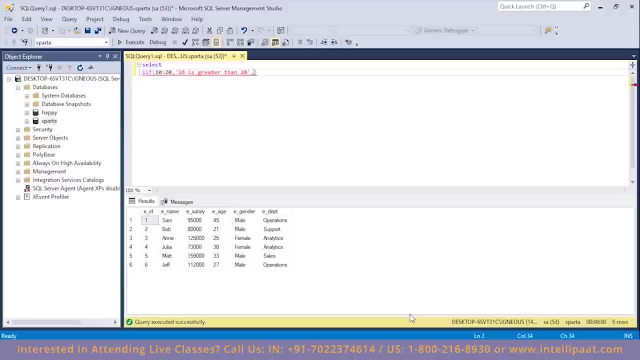 10 is greater than 20. On the other hand, if it evaluates to false, I would want to print: 10 is less than 20. I'll hit execute right. So what we get is 10 is less than 20. So we get this result because this boolean expression has been evaluated to false and it is redirected over here and we get the false result. 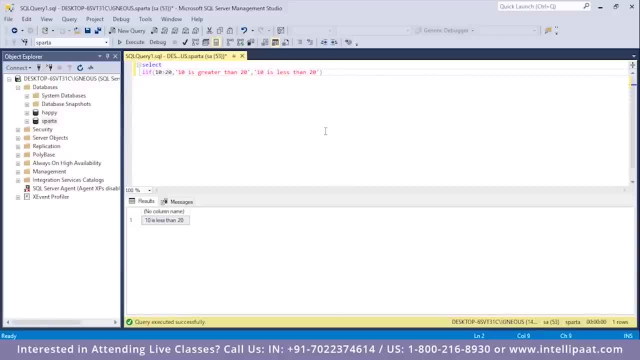 Which is 10, is less than 20. now I'll go ahead and also implement this F function on top of the employee table. so before I do that, Let me actually have a glance at the employee table first. So I will type select star from employee. 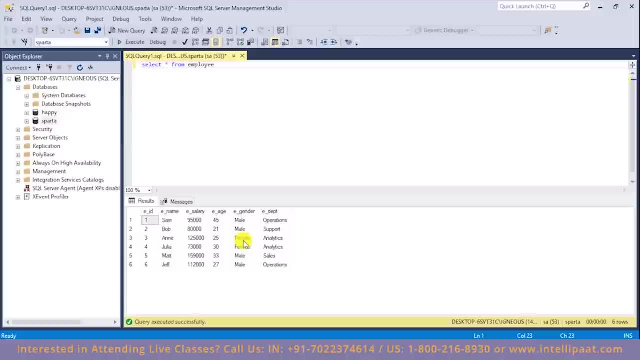 So we have our employee table right in front of us now. using the F function, I'd want to add a new column- employee generation, and that new column would be dependent on this age column. So if the age of the employee is greater than 30, Then the new column would have a value: old employee. 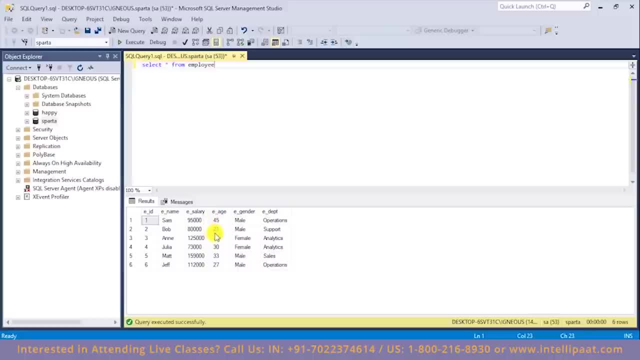 similarly, if the age of the employee is less than 30, then the value in the New column would be young employee. so let me write the syntax for this. I Will type, select and less down all of the columns which I want from the employee table. So I want the employee ID column. employee named column. 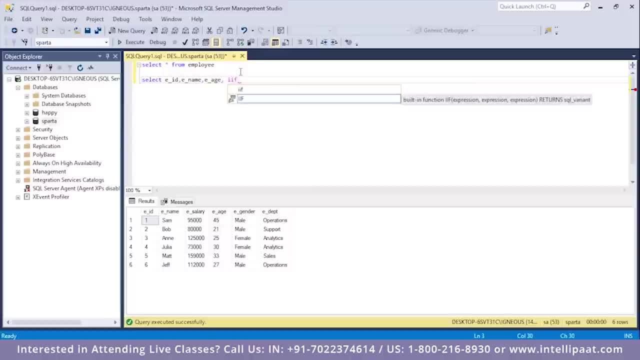 Employee each column now. after this I will use the F function to add the new column. So here the first parameter, which would be the boolean expression. so here I will check if E of age is greater than 30 and if the age is greater than 30, I. 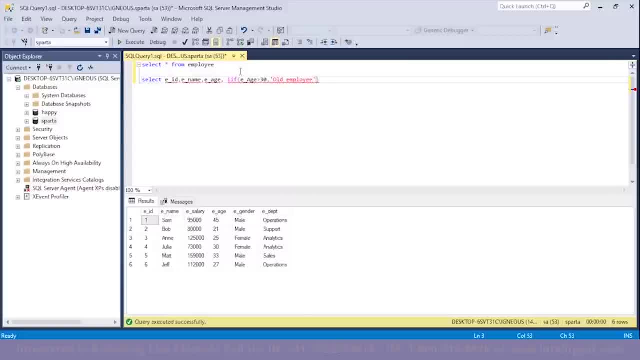 would want the value to be old employee. on the other hand, if the age is less than 30, I would want the value to be young employee. now I will name this new column as employee generation. so let me just type the name of the column employee generation over here. and I would want all of this from the table. 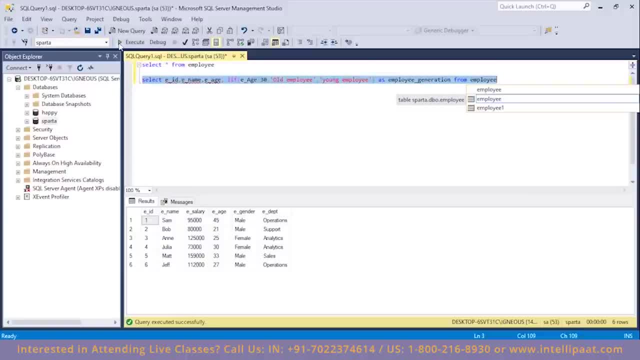 employee. now I'll select this. I'll hit execute right. so we see that a new column has been added to this and the name of this column is employee generation. so here, if you have a glance at this age value, it is 45 and the corresponding value in employee generation is old employee. similarly, 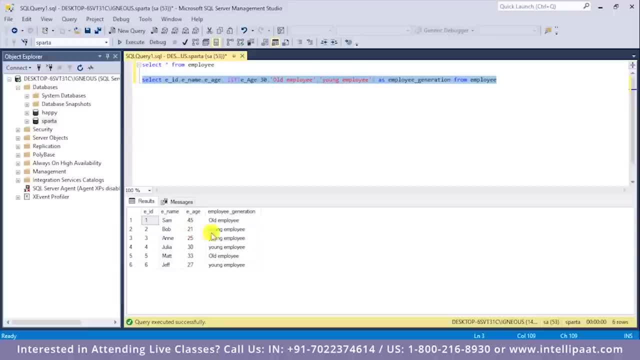 here, it is 21, and since the value is less than 30, we get young employee. and these two, it is 25 and 30, and since these two values are also not greater than 30, we have young employee over here, and Matt, whose age is 33, we have the. 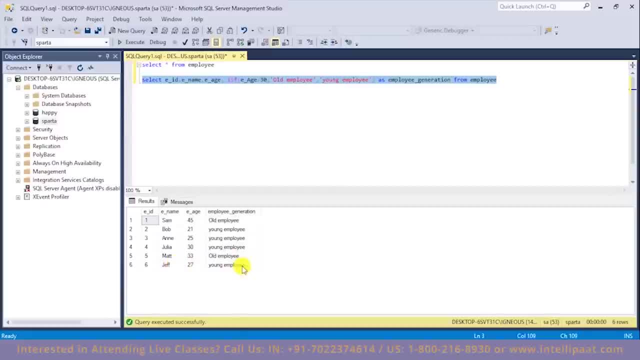 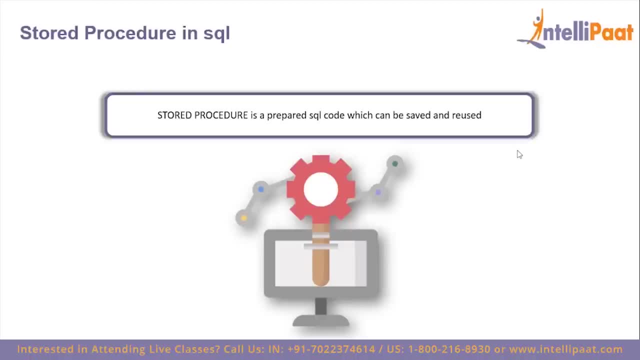 value old employee and we have Jeff whose age is 27, and these two values are also not greater than 30. we have young employee over here. he's a young employee too. So this is how we can work with the if function in SQL. So a stored procedure is basically a prepared SQL code which we can save. 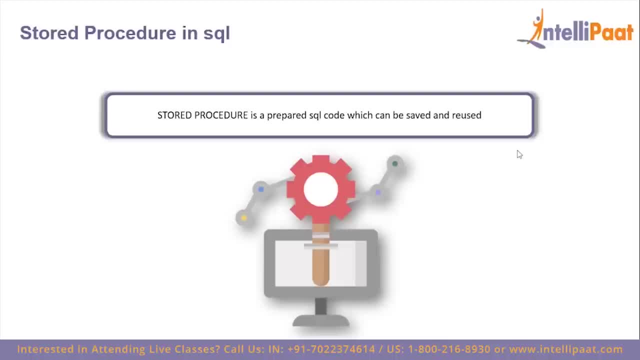 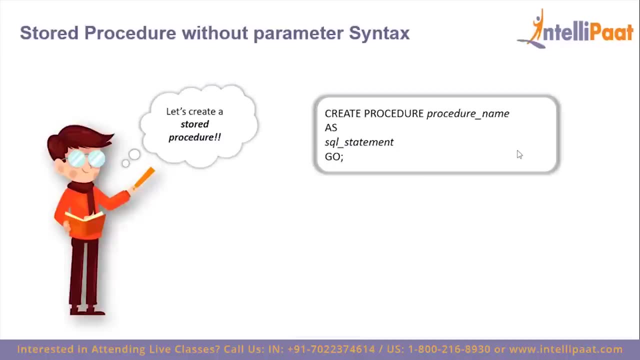 so that the code can be reused again. So if you have an SQL query that we write over and over again, we can save it as a stored procedure and then just call it whenever we want. Now let's have a look at the syntax of the stored procedure. So we'll give the keywords create. 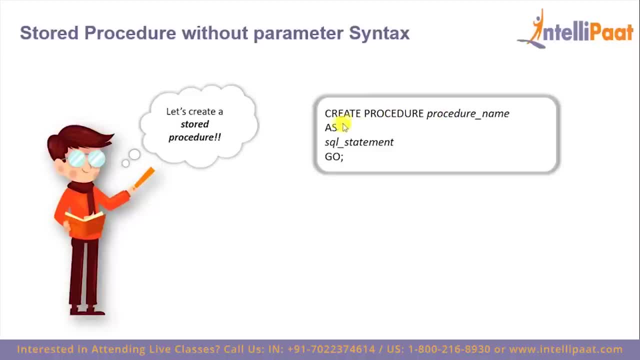 procedure and then give the procedure name. After that, we'll give the keyword as and then give the SQL statement for which we need to create the procedure, And we'll end the procedure with the go keyword. Now, after we create a procedure, we need to execute. 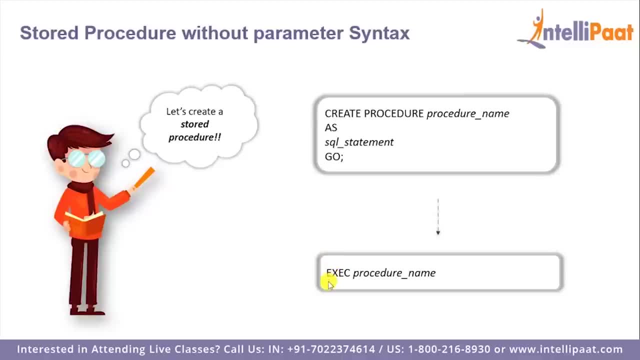 it. So this is the syntax to execute the procedure. We'll type exec and then give the name of the procedure which is to be executed. So let's go to SQL server and work with some procedures. So now I want to create a procedure which would help me to easily access this. eh. 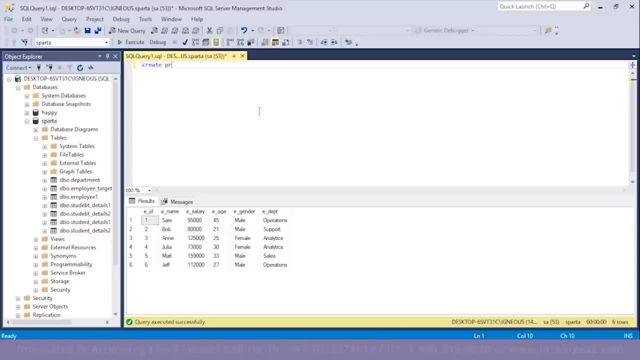 column from the employee table. So I'll type create procedure and then I'll give the name of the procedure, which would be employee age. I'll type as and then give the SQL statement which would help me to access this eh column, That would be: select eh from the name of the table is employee, and then I'll give the go. 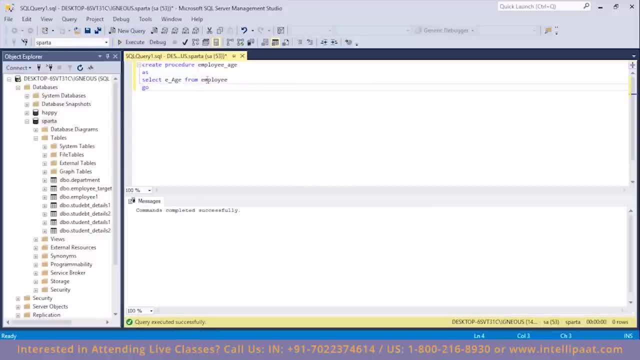 keyword. Now I'll hit execute Right. so we see that we have successfully created the employee age procedure. Now I will use the exec keyword and then call this procedure. So the name of the procedure is employee age. I'll select this line, I'll hit execute Right. so with this employee age procedure we can easily 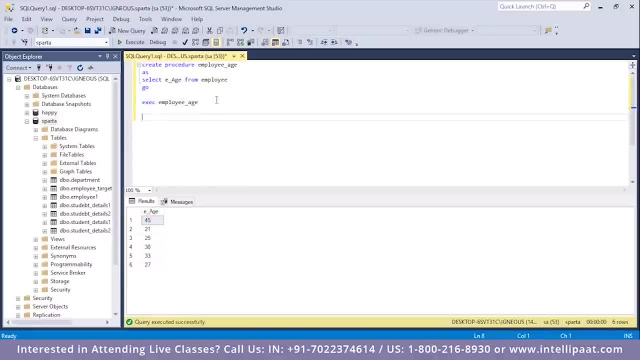 access the eh column from the employee table Now. similarly, I'll create another procedure which would help me to access all of the records from the employee table: create procedure and I'll name this procedure as employee details. I'll follow it. however, I want to. 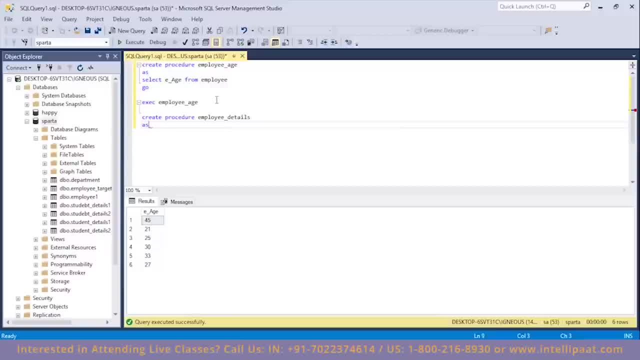 click on create procedure, follow it up with the as keyword and then give the SQL statement which would help me to access all of the records from the employee table: Select, start from employee and again I'll finish this procedure off with a go keyword. I'll. 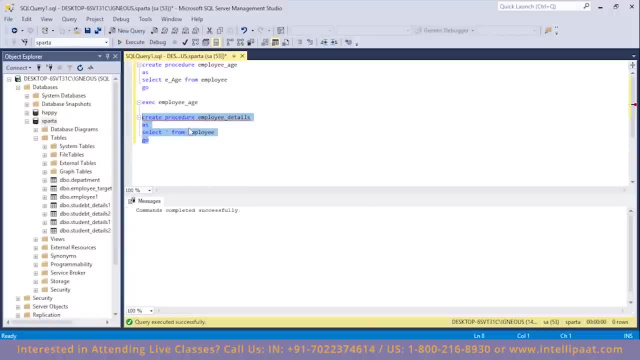 select all of this, I'll hit execute. So again, we have successfully created the employee details procedure. Now, to call this procedure, I'll use the exec command and then pass in the name of the procedure, which is employee details. So I'll select this and hit execute. So, with the help of employee details, 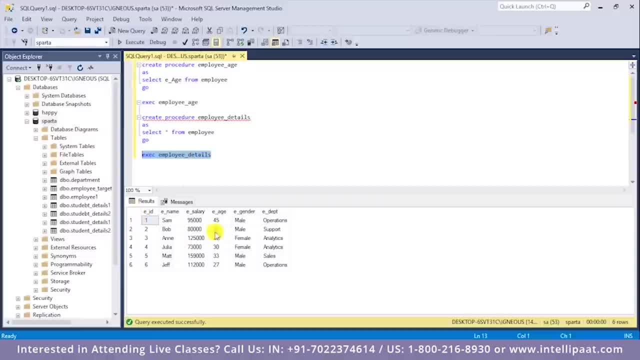 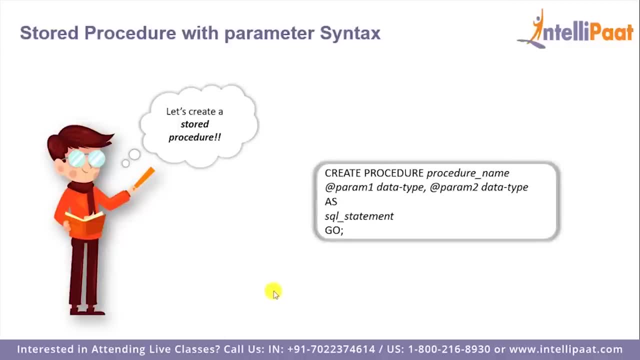 procedure. we can easily access all of the columns and all of the records from this employee table. Now we can also pass parameters to the procedure, So the syntax for this is just lightly different Here. after giving the procedure name, we follow it up with the list of parameters and their 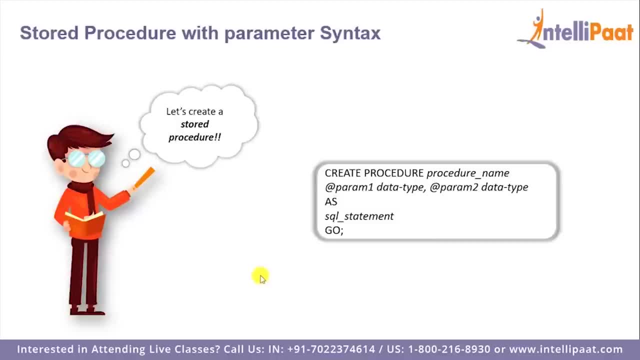 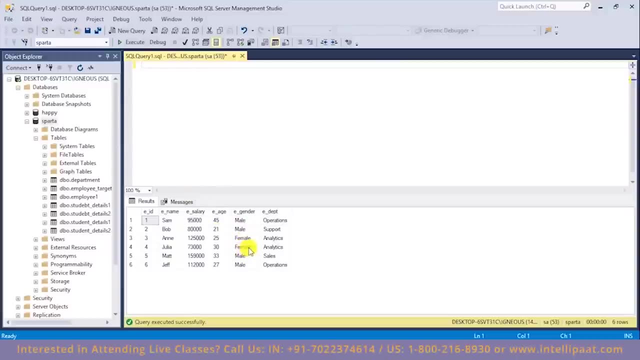 corresponding data types. So let's create a procedure with a parameter now. So now I'll create a procedure which would help me to access the male employees and the female employees separately from this employee table. Create procedure and I'll name this procedure to be employee gender. After this, I will pass in the parameter. 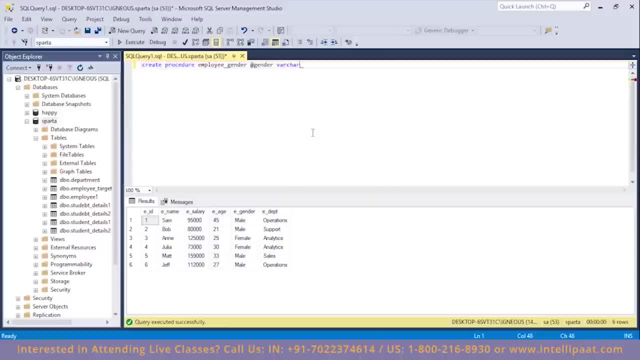 So the name of the parameter would be gender and that is of variable length character, with a maximum length of 20.. I will give the ask keyword after this and then pass in the statements which would help me to individually access the male employees and the female employees. 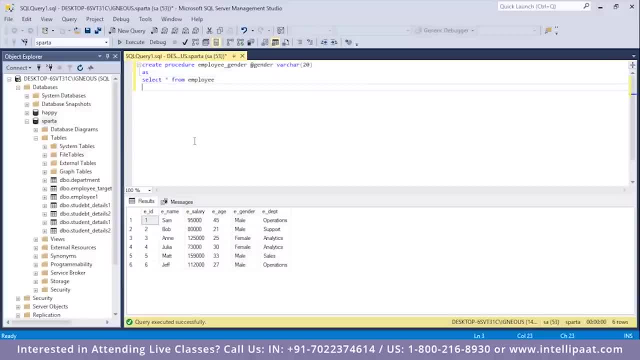 Select. start from the name of the table. as employee, I'll follow it up with the var clause and give the condition. So this time the condition would be: agenda is equal to the date gender. Let's understand this properly. So here eGender is basically this column and we are passing in the value of this parameter. 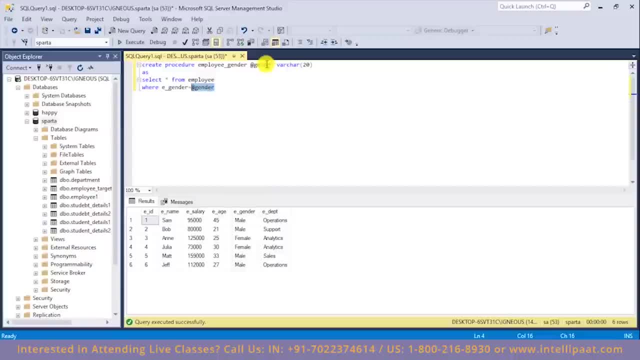 to this column. So let's say, when we call this procedure and the value is female, then we'll get all of the female employees And similarly, if the value is male, then we'll get all of the male employees. Now let me finish off this procedure with the go keyword. 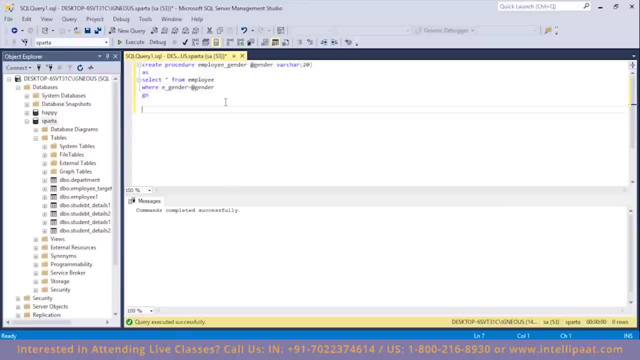 Right, so we have successfully created this employee gender procedure. Now let me go ahead and execute this procedure. So I'll type exec and then give the name of the procedure, which would be employee gender. Now let's say I want all of the male employees. 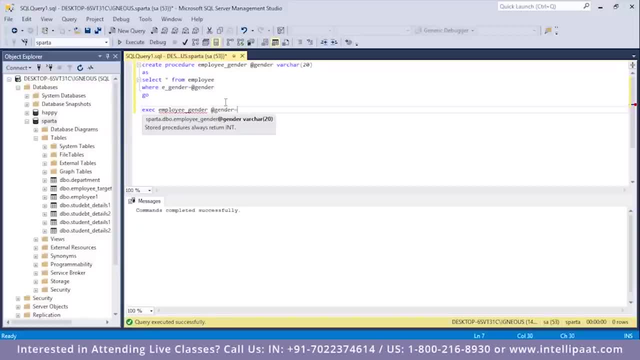 So I will give in the parameter name at the rate- gender- and I will give in the value, which would be equal to male. So let me execute this now. Right, so I've got all of the male employees from the employee table. Similarly, if I wanted all of the female employees from the employee table, 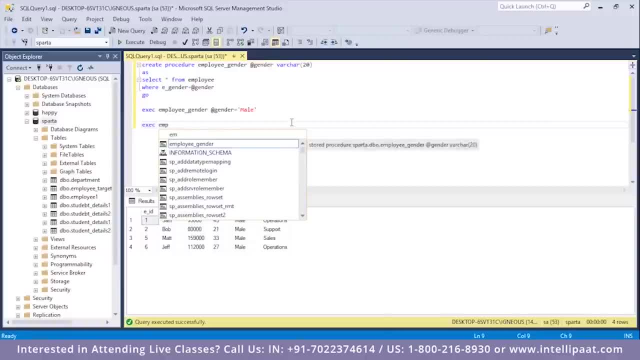 This would be the command for that Execute. I will give in the name of the procedure, which would be employee gender. I will give the name of the parameter, which would be, at the rate, gender, and then pass in the value. So this time I would want all of the female employees, so the value would be female. 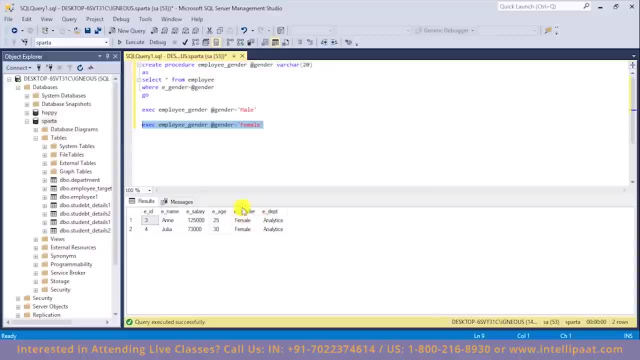 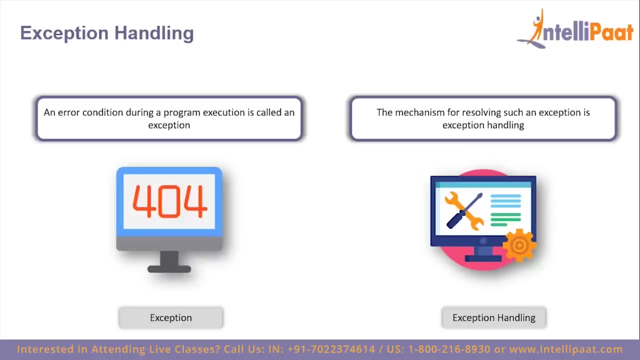 I'll select this, I'll hit execute Right. so this time we've got all of the female employees from the employee table. So this is how we can work with stored procedures, either with parameters or without parameters in SQL. So an error condition during a program execution is called as an exception. 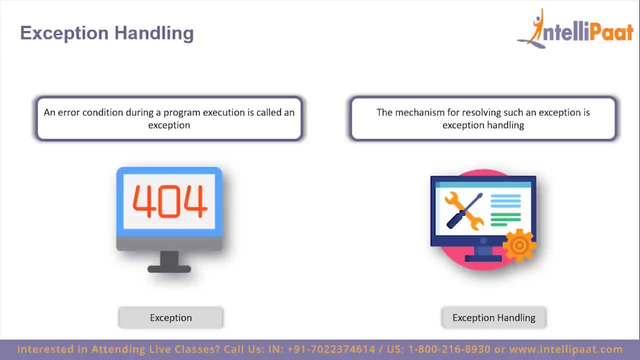 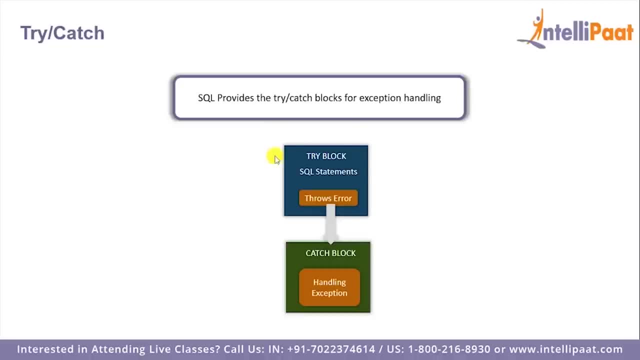 And the mechanism for resolving such an exception is known as exception handling, And we can do exception handling in SQL with the help of try-catch blocks. So the try statement allows us to test a block of statements while they're being executed And the catch block allows us to handle any exception which occurs in the try block. 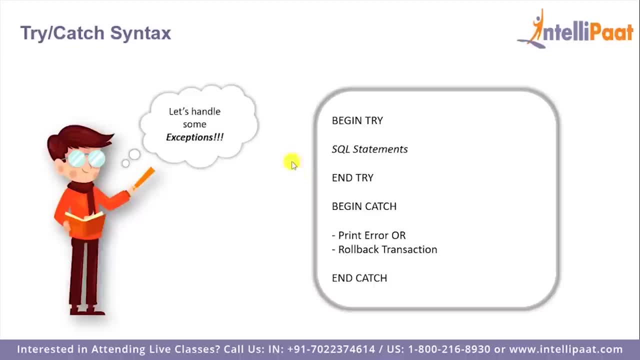 Now let's have a look at the syntax of the try-catch block. So we'll give the keywords Begin, Try And then give the statements which are to be tested. After that we'll end the try block and begin the catch block. 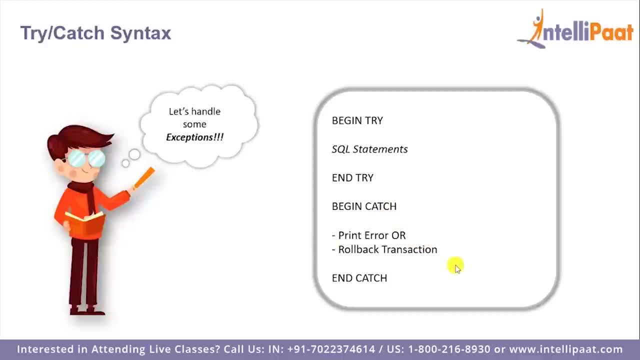 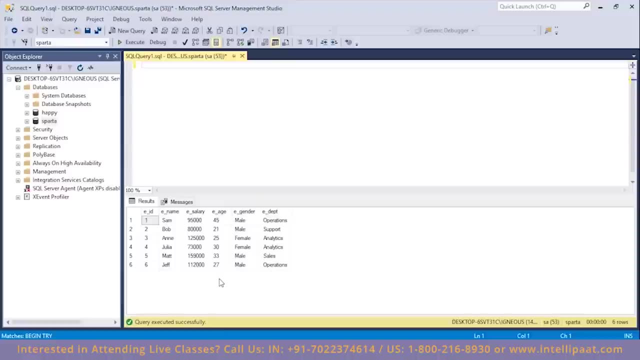 And inside the catch block we'll either print the error or roll back the transaction And we'll end the catch block as well. So let's go to SQL server and do some exception handling. So I'll be declaring two variables and divide one of the variables with zero. 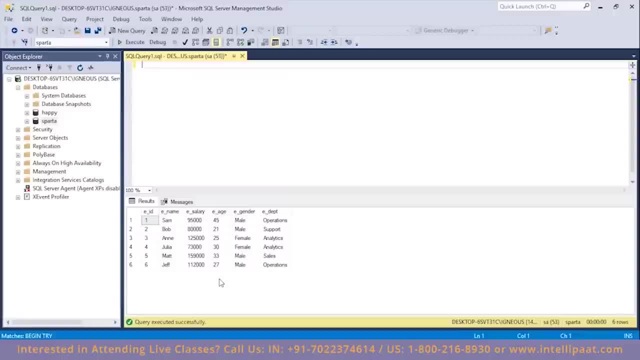 So this needs to give us divided by zero exception. So let's go ahead and handle this exception now So we can declare a variable in SQL By using the declare statement. So I'll type declare And then use the iterate symbol to declare a value. 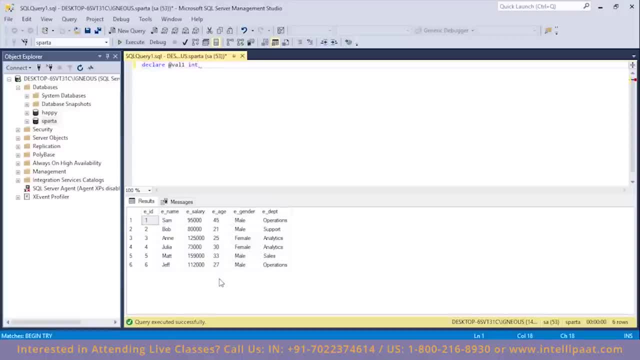 And I'll name this variable as val1.. And this is of integer type. Similarly, let me go ahead and declare the second variable. I'll type: declare iterate, And the name of this variable is val2.. And the data type is integer again. 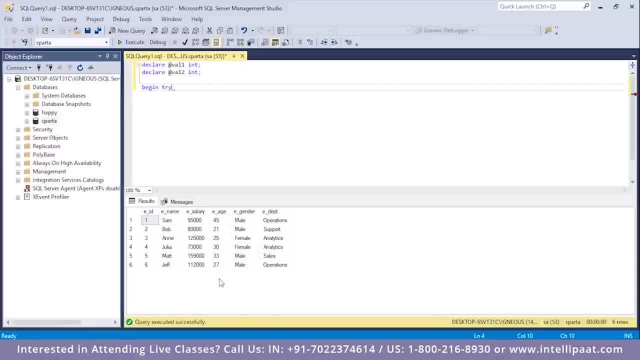 Now I'll begin the try block. I'll type begin try And then inside this I will set the values for both the value 1 and value 2.. So I'll use the set keyword. So I'll use the set keyword. 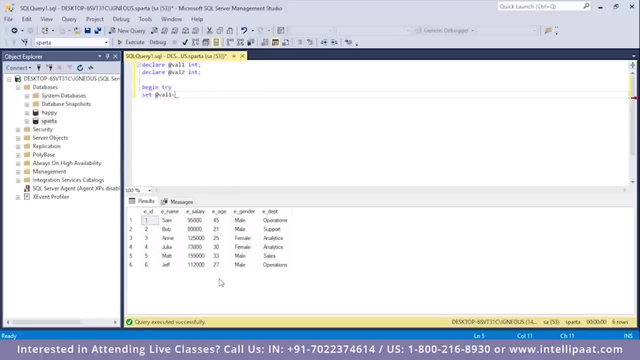 And then the value which I'll be assigning to val1 as 8, I'll put semi-colon. Similarly, let me assign something to val2 as well. So set at the rate val2.. Now, inside val2, what I'll basically do is divide val1 with zero. 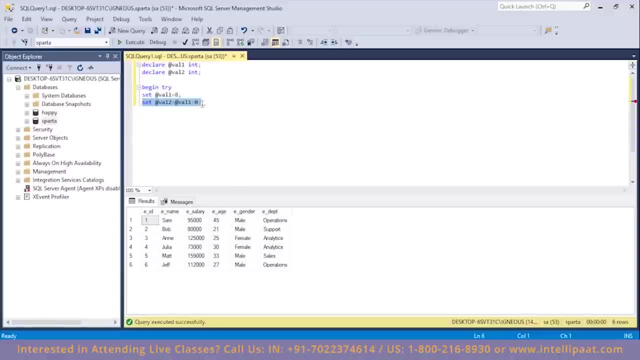 So now this statement should basically give us the error. So when we divide any integer value with a zero, we'll get an indefinite value. So this is the statement. So this is the statement which will be giving the error. Now I will end the try block and try right. 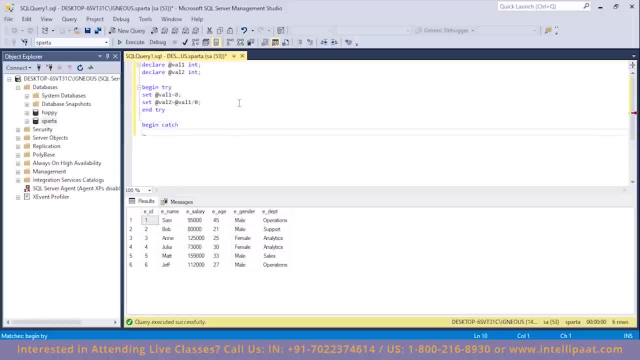 Now, after this, we'll begin the catch block, Begin catch And inside the catch block, I will just print out the error which occurred in the try block And I will display the default error message And I will end the catch block as well. 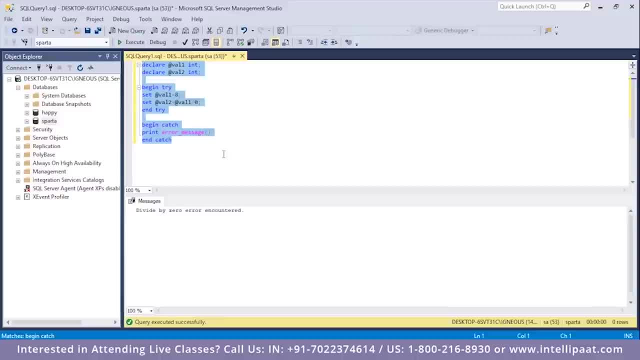 So let me hit execute now. So the default error message, The default error message which you get, is divide by zero error encountered. So what we basically did with this set of statements was: we encountered an error within the try block and we handle that error inside the catch block. 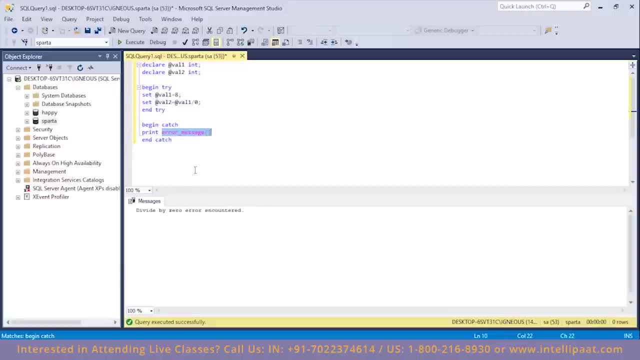 So inside the catch block we sent a default error message and the default error message was divide by zero error encountered. Now we can also create user defined messages. So let's go ahead and create some user defined messages And for that purpose I'll be doing exception handling on top of the employee table. 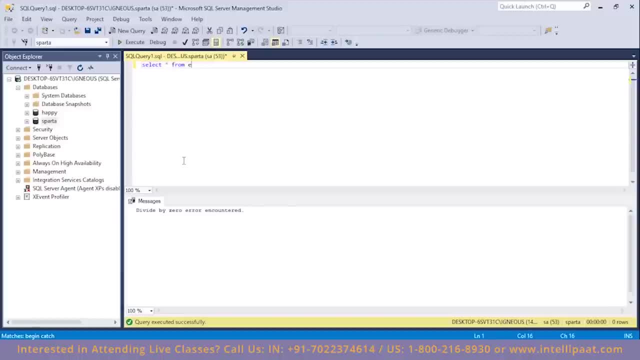 So let me actually have a glance at the employee table. first, Select- start from the name of the table- is employee right. So we have this employee table right in front of us. So now what I'll do is I'll try to add the salary column and the name column. 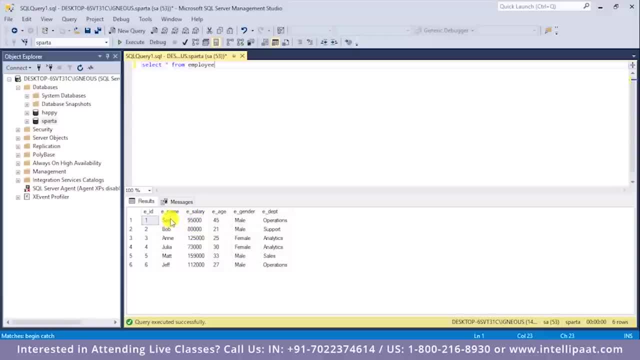 Now the problem with this is we cannot add a numerical column with a string value. So let's handle this exception. So I'll type begin, try And then try And then try. I will give the select keyword and I will try to add e salary column with the e name. 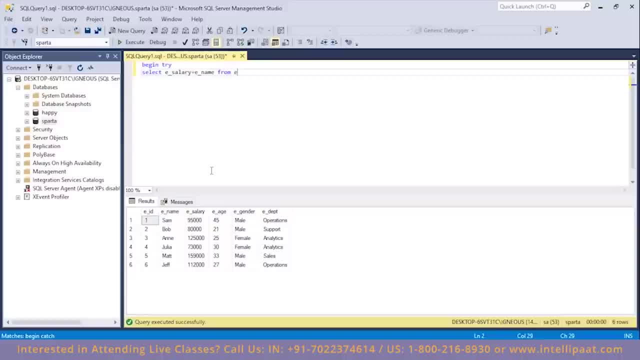 column And I want this from the employee table. I will end the try block after this. I need to begin the catch block, So begin catch inside this. I will print a user defined message, So print and I would want to print. 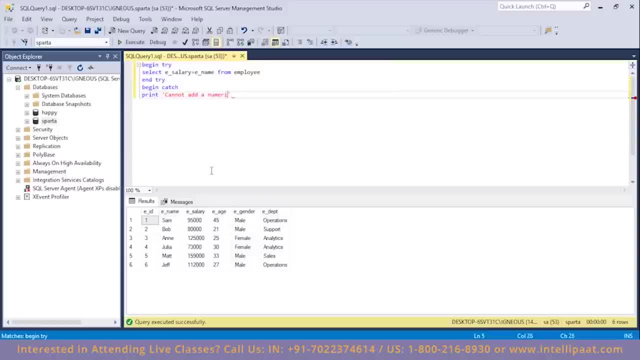 Cannot. Cannot add a numerical value with the string value. I will end the catch block as well. After this, I will give the go statement. Let me hit execute. So this is the message which we get: Cannot add a numerical value with the string value. 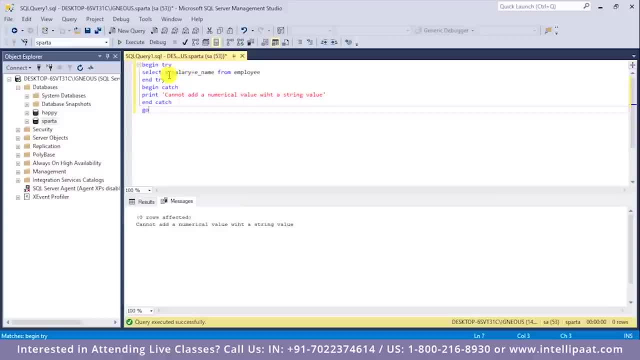 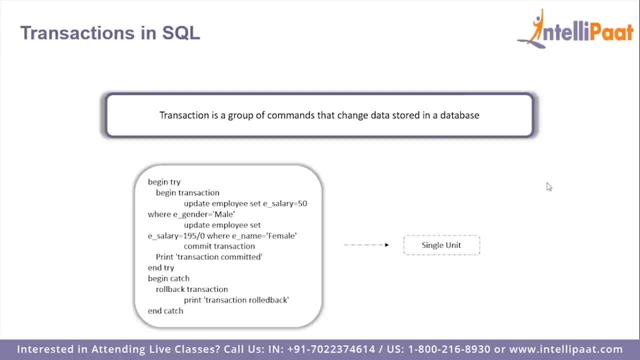 And we got this user defined message because we had encountered an error inside the try block. So this is how we can do exception handling in SQL. So let's try. So here we have a transaction. This is basically a group of commands, so we'll change data stored in a database. 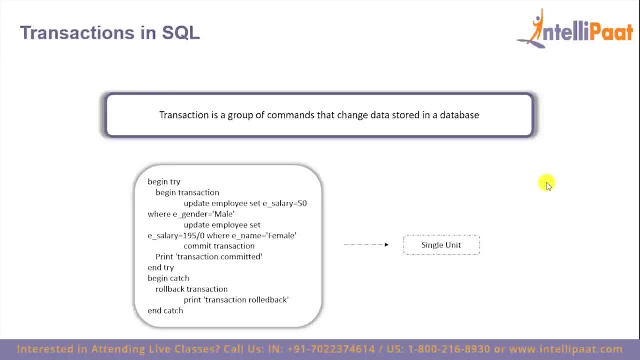 And the transaction is treated as one single unit. So this transaction basically ensures that either all of these commands are executed successfully or none of them is. So let's say, if one of the commands in the transaction fails, then all the commands will fail. 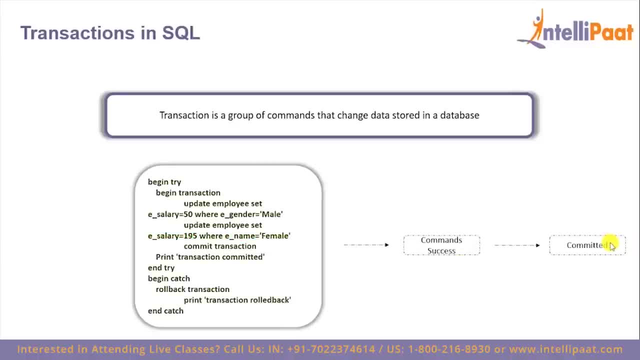 And any data which was modified in the database will be rolled back. Similarly, All the commands inside the transaction will be loaded back inside the transaction execute successfully. only then the transaction will be committed. So this is how transactions ensure integrity of data. So 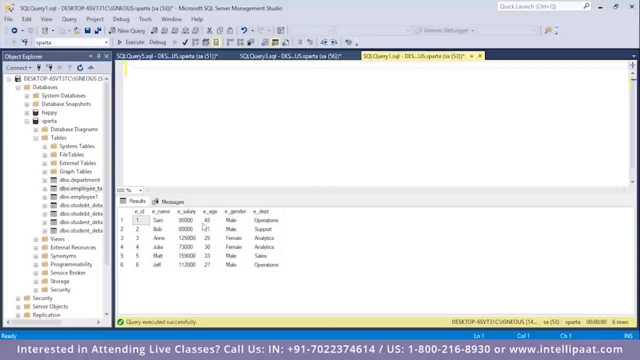 now I'll begin a transaction and inside that transaction I'll try to update this age value from 45 to 30. So let me write the syntax to begin a transaction, So I'll type begin and then type transaction and inside this I'll give all of those. 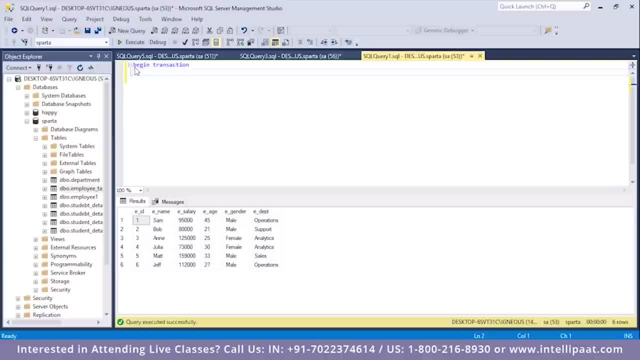 SQL statements which either have to be committed or rollback. So over here I'll give the update statement. I'll type update and then give the name of the table, which would be: employee Set eh to be equal to 30 where ename is equal to. 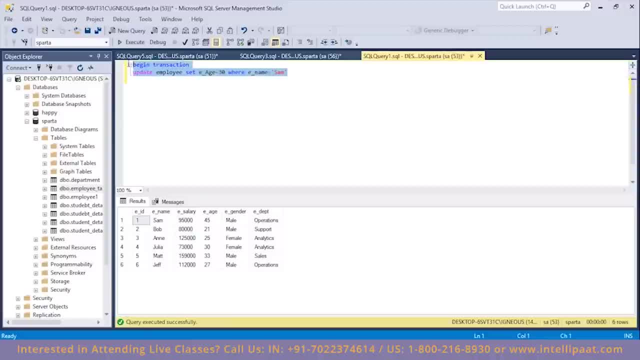 Sam. So I'll select these two statements and I'll execute them. So we see that one row has been affected. So now let me have a glance at the modified table. So I'll type select star from employee. I will select this command over here. I'll. 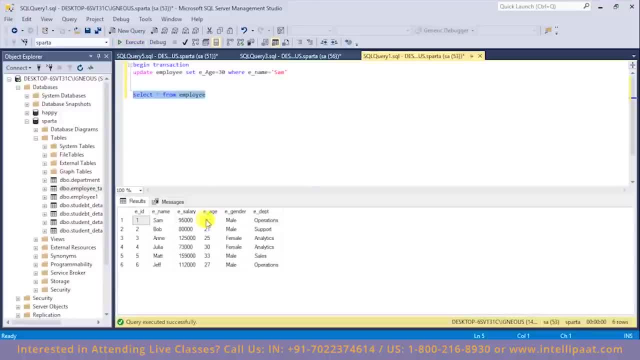 execute this right. so see that initially, the age value was 45 and after we applied this update command, the age has been changed from 45 to 30. now, since this command is inside a transaction, we have the option to either roll back this command or commit this command. so now let me go ahead and actually roll back. 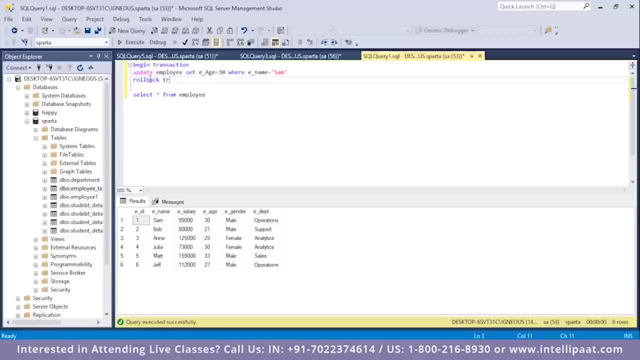 this transaction. so to do that, I'll type role back transaction. so now let me select this. I'll click on execute so we see that the commands have been completed successfully. now let me again have a glance at the employee table right. so since we have roll-back 2 transaction, we see that each value has 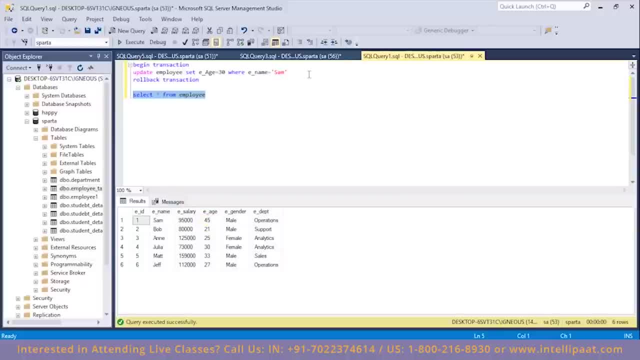 gone back to the original value, which is 45. so initially, using the update command, we had changed the age value from 45 to 30, and after that we had rolled back the transaction now. now, what I'll do is I'll execute these two statements again and let me have a glance at the table right. so 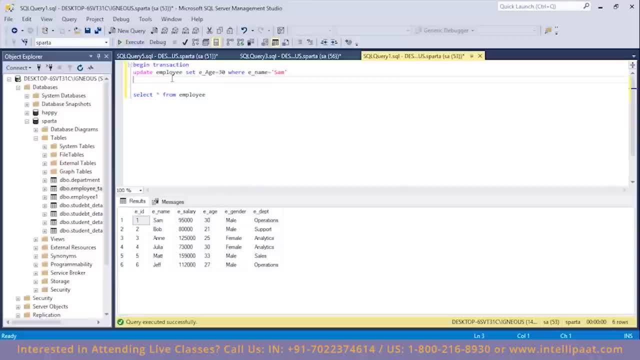 again we see that the age has been changed to 30. so this time, instead of rolling back the transaction, I will commit the transaction. so I'll type commit transaction, so I'll select this, I'll click execute. now let me have a glance at the table. so this time the transaction has been committed and the 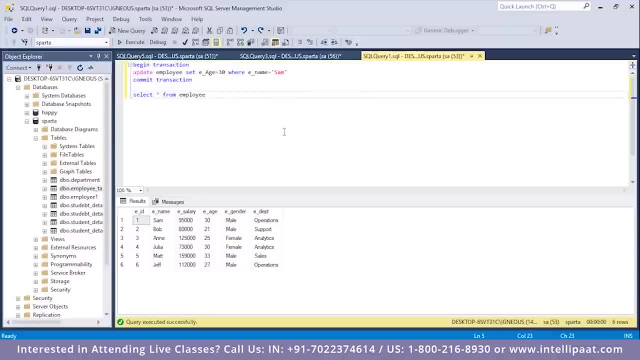 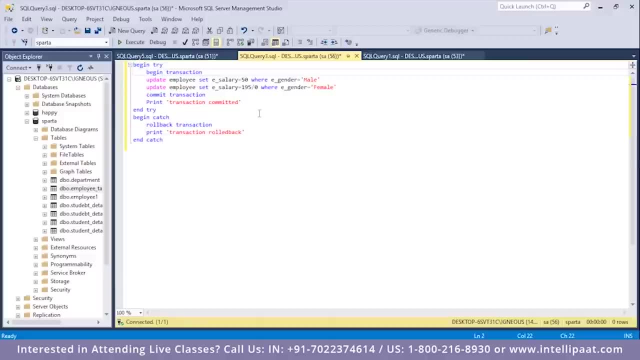 change is permanent. so this is how we can either come in our rollback, the commands using the transaction. now let's look at another example. so when this example, we are using transactions inside the try catch block, so over here we are beginning the try block and inside this we are beginning the transaction. and 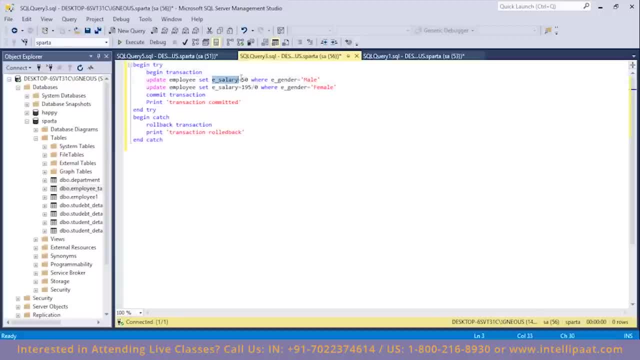 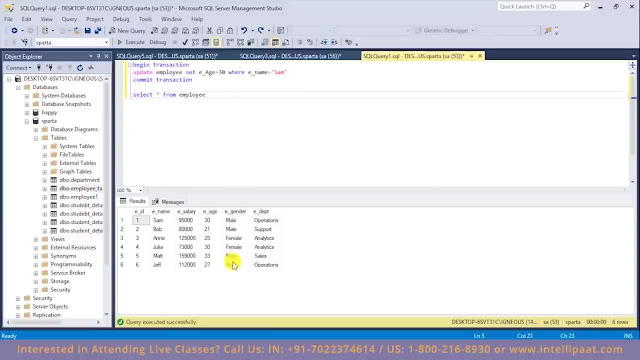 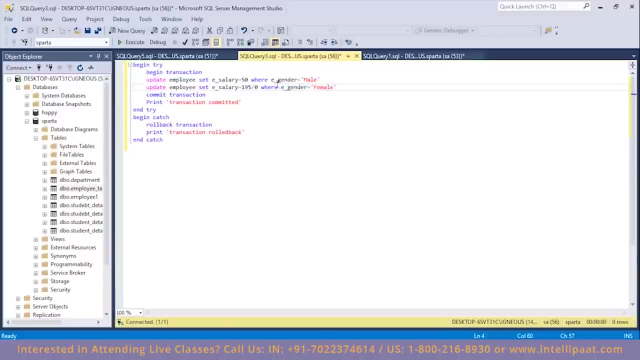 inside the transaction. we are trying to update the salary value to be equal to fifty. gender value is equal to male, So wherever the gender is equal to male, we'll update that salary value to be equal to 50.. Similarly, wherever the gender value is equal to female, I will change. 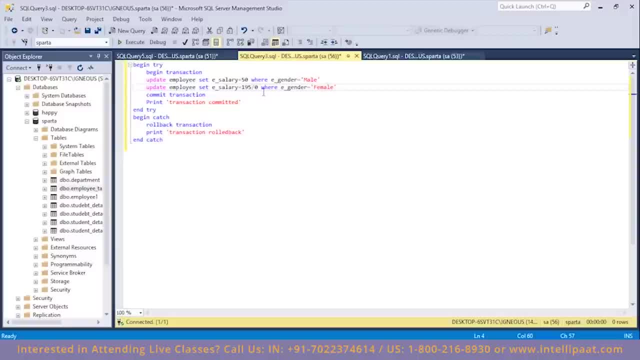 that salary value to be 195 divided by 0, which would give us an undefined value, and after that we'll commit this transaction and print transaction committed. Now, since we have put this transaction inside the try block, if any error occurs, that will be sent to the catch block and we will roll. 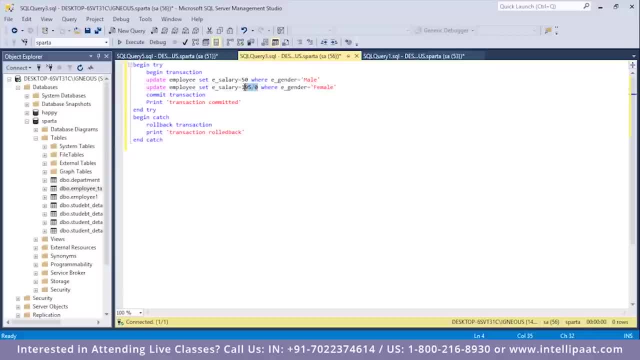 back the transaction. So over here we see that we are dividing 195 with 0 and since this gives us an undefined value, we will get an error and that error will be handled in this catch block and we will roll back the transaction. So let me execute this So you see that the transaction has been. 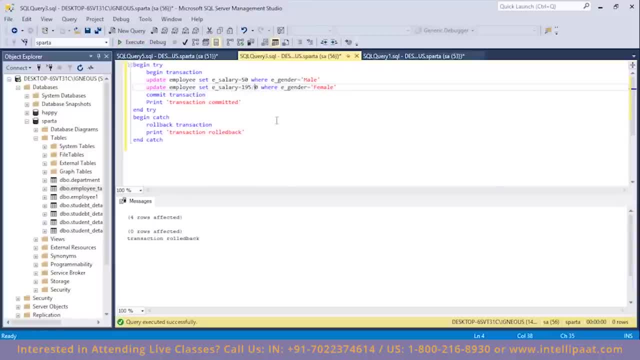 rolled back because we get an error inside the try block. Now what I'll do is I will remove this divided by 0 and run this command again. So this time we see that the transaction has been committed because there was no error inside the try block. So now, 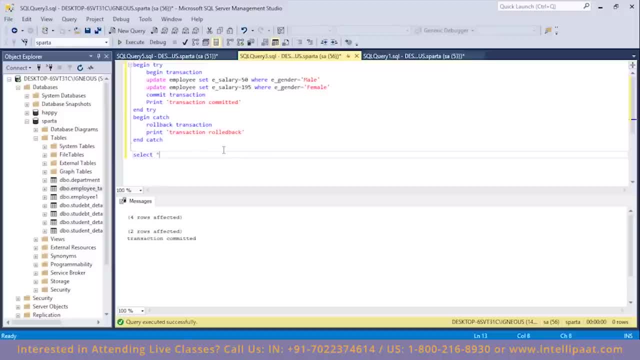 let me have a glance at the modified employee table. So I'll type select start from employee, I'll select this, I'll click on execute Right. So we see that we have changed the salary value to be 50 where gender is equal to male. Similarly, 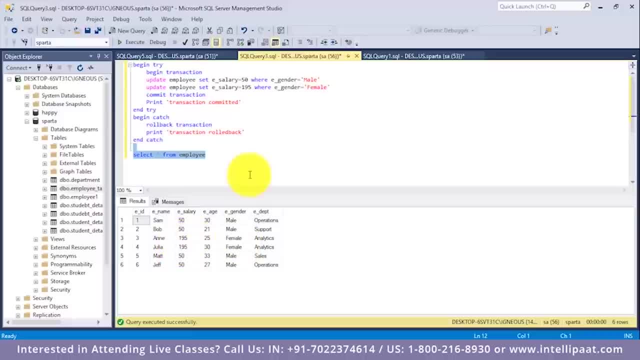 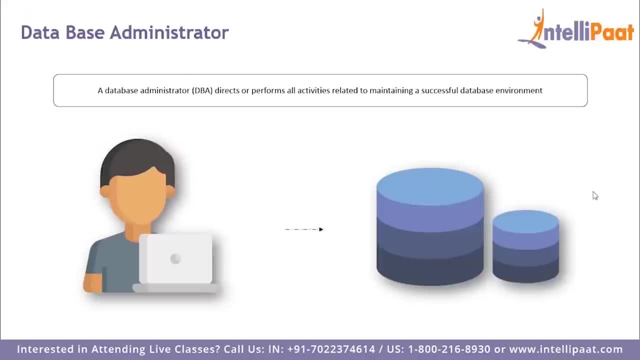 I have changed the salary value to be equal to 195, where the gender is equal to female. This is how we can work with transactions in SQL. So who is the database administrator? Well, a database administrator is someone who directs or performs all activities related to maintaining a successful database environment. So now that we 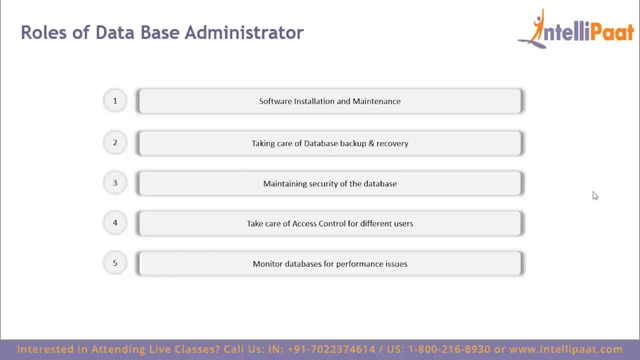 know who is a DBA, let's look at some of the roles of database administrator. So a DBA has to take care of the initial and configuration of a new Oracle or SQL server database. The system administrator sets up hardware and deploys the operating system for the database server. Then the DBA installs. 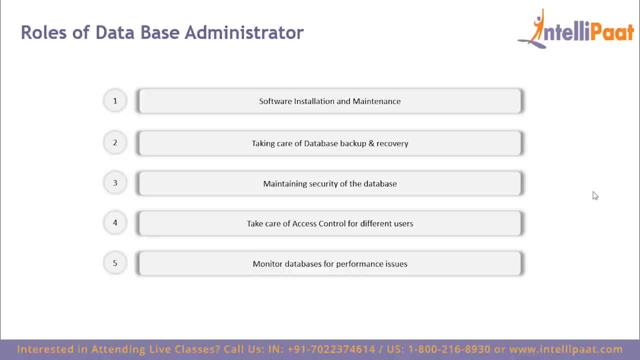 the database software and configures it for use. As updates and patches are required, the DBA has to handle this ongoing maintenance. A DBA has to also take care of backup and recovery of databases, So DBAs have to create backup and recovery plans and procedures based. 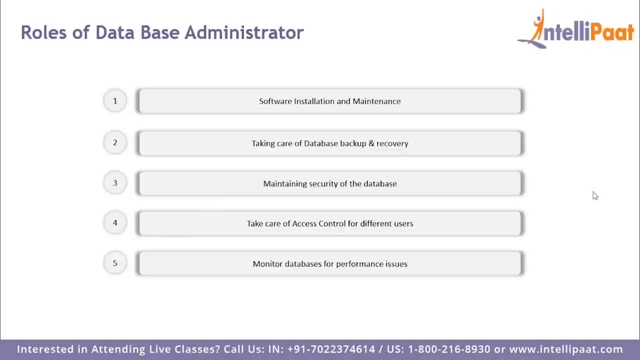 on industry best practices that make sure the necessary steps are followed. Another role of DBA is to maintain security of the database, So a DBA needs to know potential weaknesses of the database software and the company's overall system and work to minimize risks In case of a security. 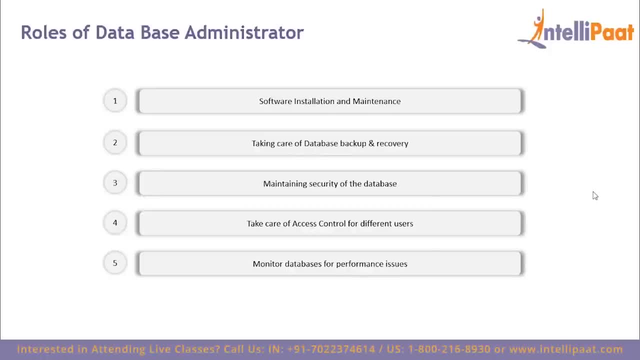 breach or irregularity. the DBA can consult audit logs to see who has the most potential issues. The DBA has to also take care of access control, That is, it has to verify which users can be granted access to the system and which users should be denied. Then a DBA has to also 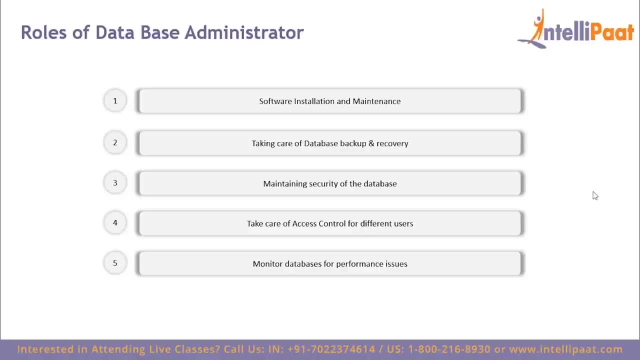 monitor databases for performance issues. So if some part of the system is slowing down the processing, the DBA may need to make configuration changes to the software or add additional hardware capacity. So now that we know what are the roles of a DBA, 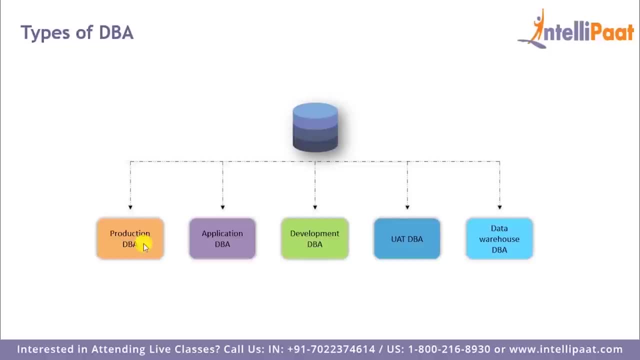 let's look at the types of DBA. Let's start with production DBA. So a production DBA is responsible for maintaining databases within an organization. The production DBA often gets involved when all the design decisions have been made and he or she has to keep things up and running. So the 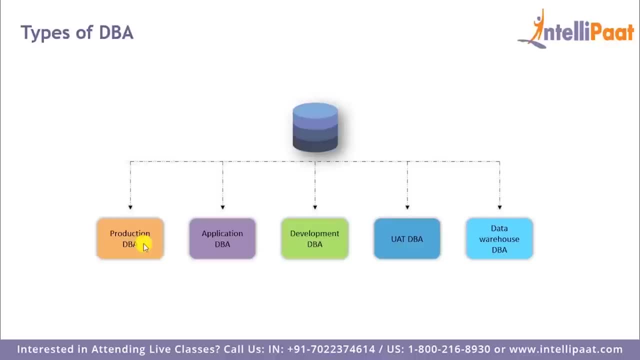 production DBAs basically take over after applications have been created, and they would have to keep the server running smoothly, back it up and plan for future capacity needs. Then we have application DBAs, So a production DBA is responsible for maintaining databases within an 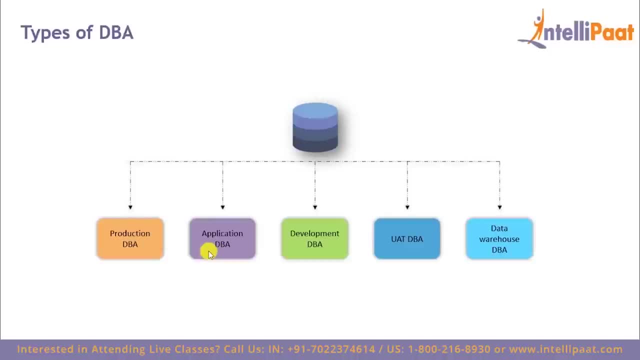 organization. So an application DBA focuses on a specific business application. He or she would be an expert in SQL and would implement the application business logic using SQL or any other query language. They would be also responsible for performance tuning of the database application. Next we have development DBA. So the development DBA focuses on tasks. 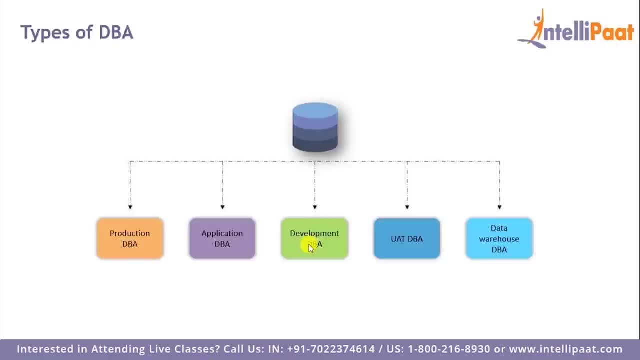 related to building an effective, usable database environment to support the creation and maintenance of applications Development. DBAs need to be skilled in the process of data modeling and normalization to ensure that databases are designed to promote data integrity. Then there's UAT DBA, So a UAT database actually stands for under application testing database. 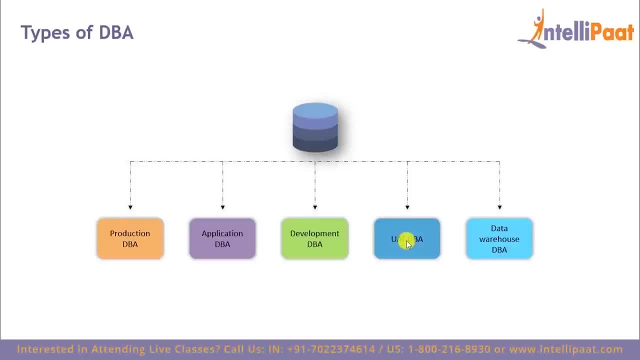 And the UAT DBA is completely responsible for the testing and development of UAT database. And finally, we have data warehouse DBA. So a warehouse DBA is responsible for analyzing and understanding the data provided. It is his responsibility to study and track patterns for analytics and business intelligence, Hence a 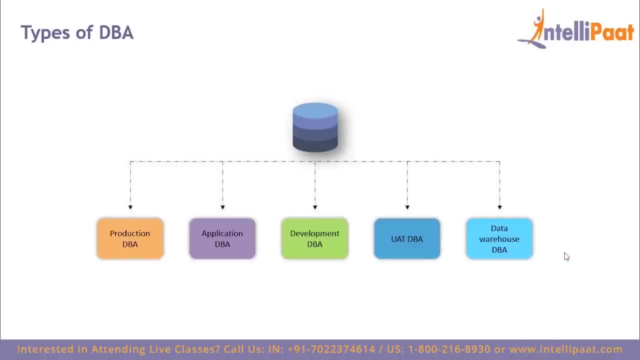 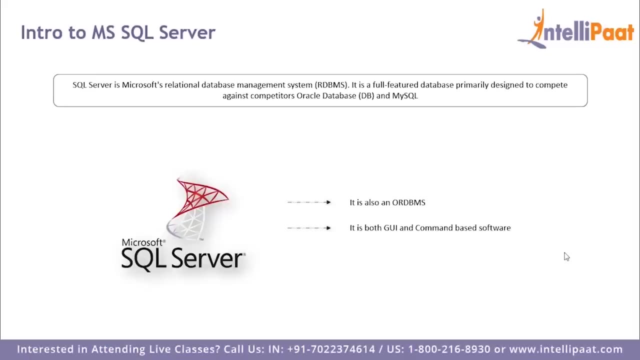 warehouse DBA handles a more significant amount of data for a more critical function. Now let's understand what is MS SQL Server. So Microsoft SQL Server is a relational database management system, or RDPMS, that supports a wide variety of transactions. So Microsoft SQL Server is built on top of SQL that is tied to TransactSQL or TSQL, which is an 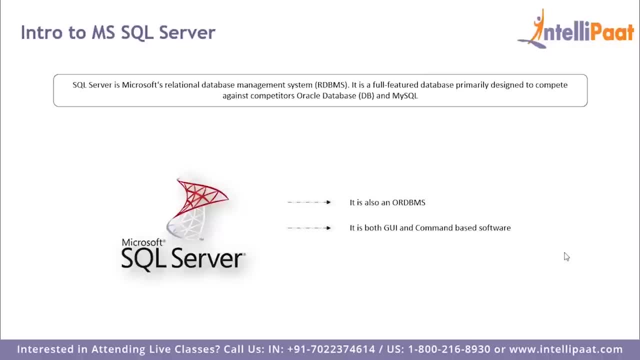 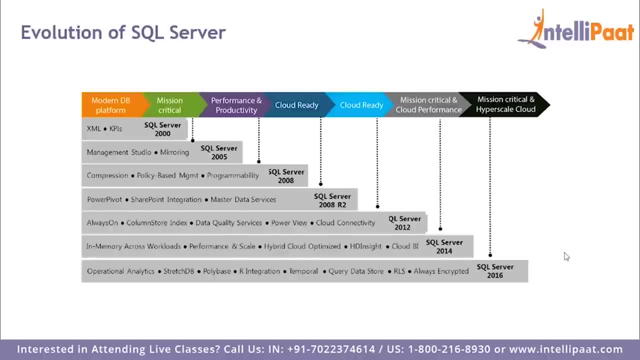 implementation of SQL from Microsoft that adds a set of proprietary programming extensions to the standard language. Now let's look at the evolution of SQL Server. So the SQL Server database platform that we know today began with the SQL Server 7.0 release in 1998.. So 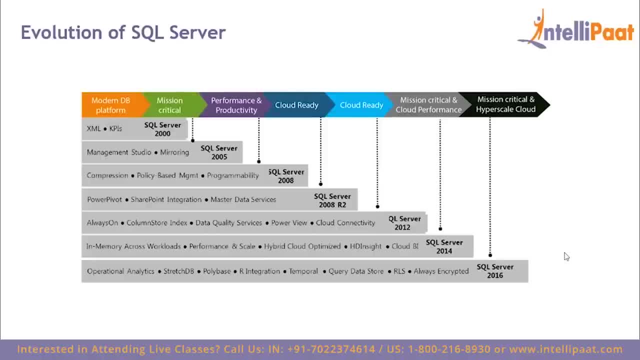 Microsoft re-architected the core database engine code in SQL Server 7.0 to address the database's scalability issues, transforming it from a departmental database into a true enterprise-level database. Perhaps even more important, Microsoft added OLAP services. 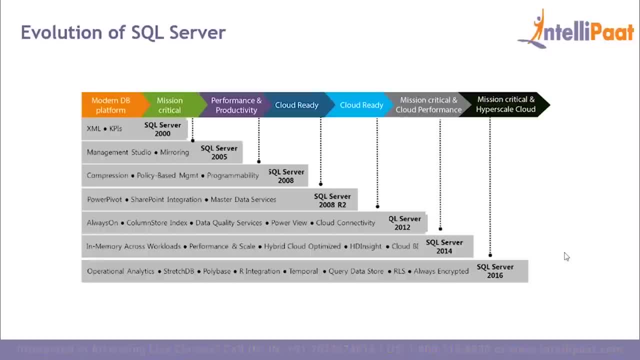 which would eventually become SQL Server analysis services. Then the SQL Server 2000 release saw Microsoft continuing to push the platform into enterprise. This boosted scalability through large memory and address windowing extension support. The company also expanded SQL Server's data handling capabilities with the new XML data type. 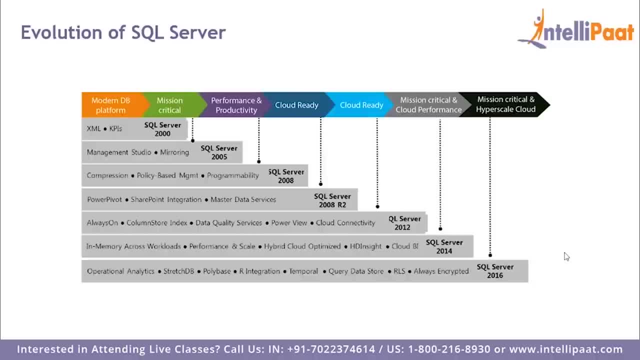 And then came SQL Server 2005,, which was a major milestone. Microsoft added CLR integration plus. this was the first release to include the popular SQL Server reporting services subsystem out of the box. Microsoft also had replaced data transformation services with the new SQL Server integration services in this release. 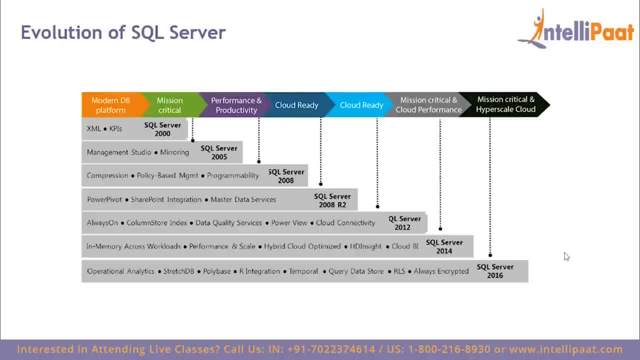 And then SQL Server 2008,. Microsoft refined SQL Server's enterprise capabilities, adding transparent data encryption as well as the file stream and geospatial data types. SQL Server 2008 was also the first release with built-in row and page compression for. 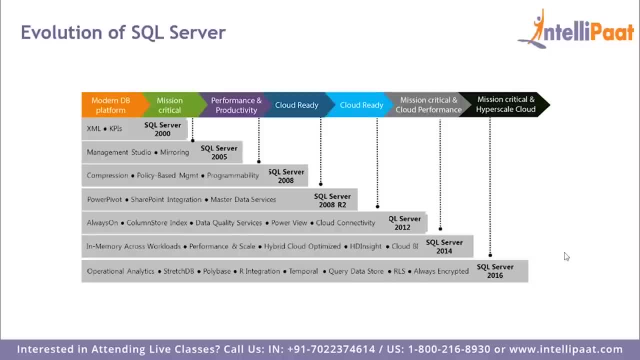 tables and indexes. Then came SQL Server 2012,, which expanded SQL Server's BI capabilities, with the addition of PowerView, which is a graphical data navigation and visualization tool. In this release, Microsoft also added Always-on availability groups, which extended SQL Server's high availability and disaster recovery options. 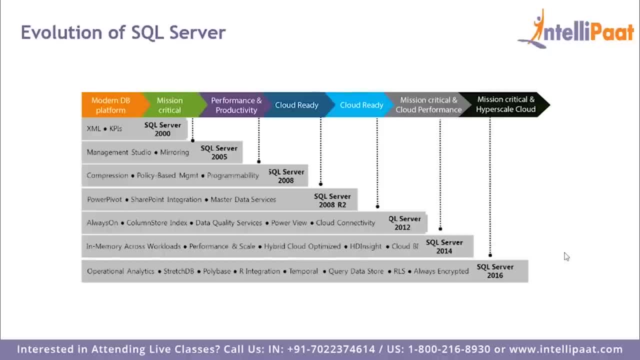 The next release was SQL Server 2014,, which provided a new in memory capability for tables that could fit entirely in memory. It also provided a new hybrid disaster recovery and backup solutions with more API andж Microsoft Azure, enabling customers to use existing skills with the on-premise version. 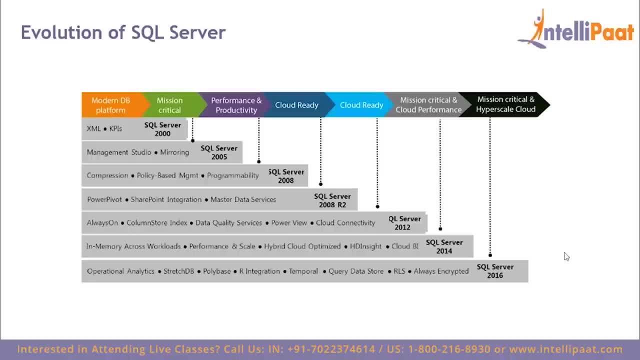 of SQL Server to take advantage of Microsoft's global data centers. Then SQL Server 2016 released, which added new built-in JSON support in SQL Server for JSON imports, exports, parsing and storing. A new poly-based query engine was also added to integrate SQL Server with external data. 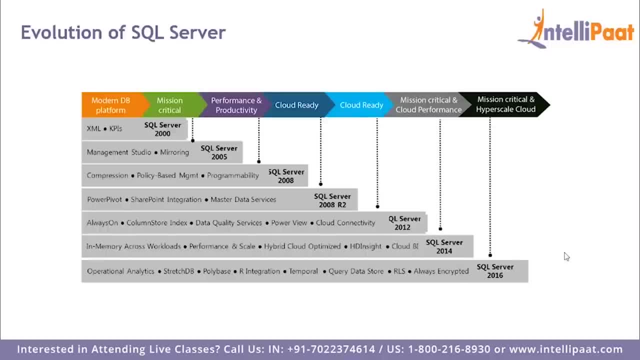 in Hadoop or Azure Blob storage, And the latest release is SQL Server 2017, and with this release, SQL Server is no longer just a Windows-based RDBMS. We can now develop applications with SQL Server on Linux, Windows, Ubuntu or Docker, and. 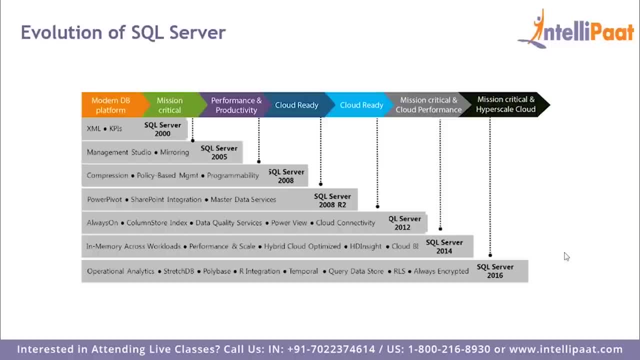 deploy them on these platforms. This release also has support for Python, So our data scientists can now more easily perform machine learning right inside of SQL Server. Now let's look at the different editions of SQL Server. So first we have the Enterprise. 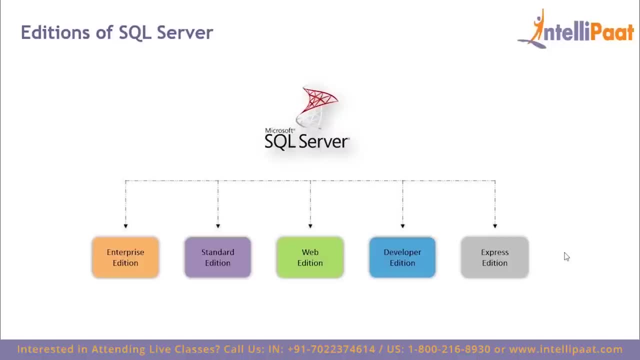 So SQL Server Enterprise Edition includes both the Core Database Engine and add-on services, and with a range of tools for creating and managing a SQL Server cluster, So it can manage databases as large as 524 petabytes and it supports 640 logical processors. 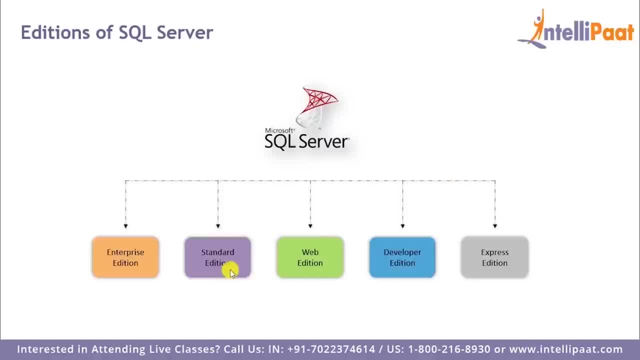 Then we have the Standard Edition. The SQL Server Standard Edition includes the Core Database Engine along with the standalone services, So it differs from the Enterprise Edition in that it supports fewer active instances, that is, fewer number of nodes in a cluster, and it also does not include some high availability. 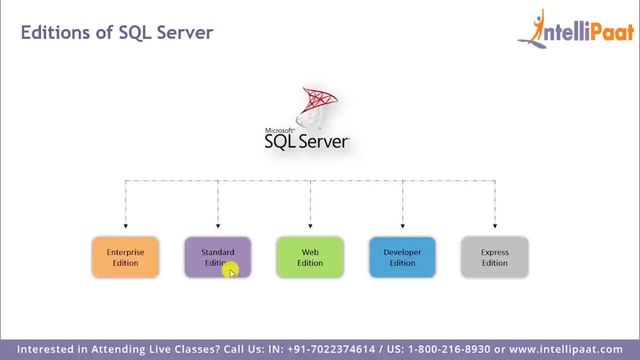 functions such as hot-add memory and parallel indexes. Then we have the Web Edition, which is just a low TCO option for web hosting, And then we have the Developer Edition. So this edition includes the same features as Enterprise Edition, but it is limited by. 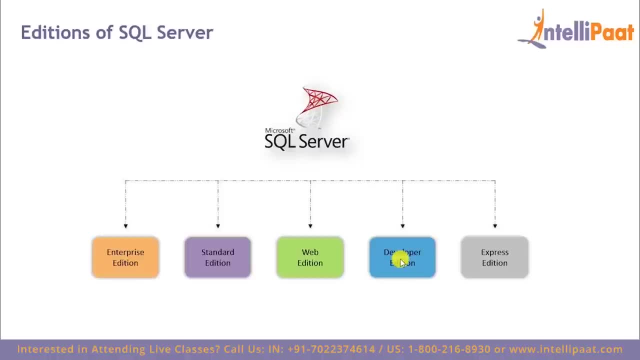 the license. It is only used as a development and test system and not as a production server. And finally, we have the Express Edition. So it is basically a scaled-down free edition of SQL Server, which includes the Core Database Engine. While there are no limitations on the number of databases or users supported, it is limited. 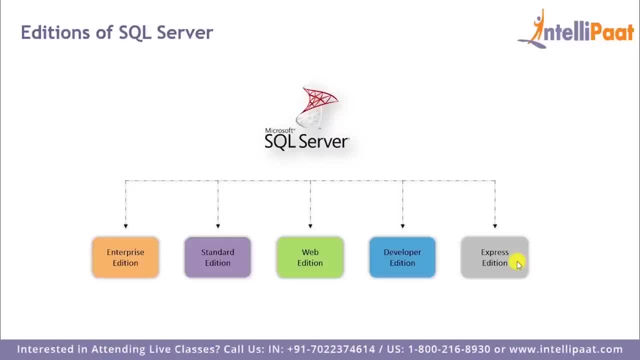 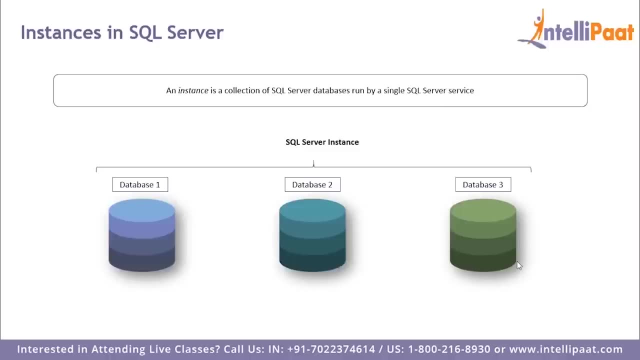 to using 1 processor, 1 GB memory and 10 GB database files. Now let's learn about Instances. So you can consider an instance to be one case: One complete installation of SQL Server, And each instance manages several system databases and one or more user databases. 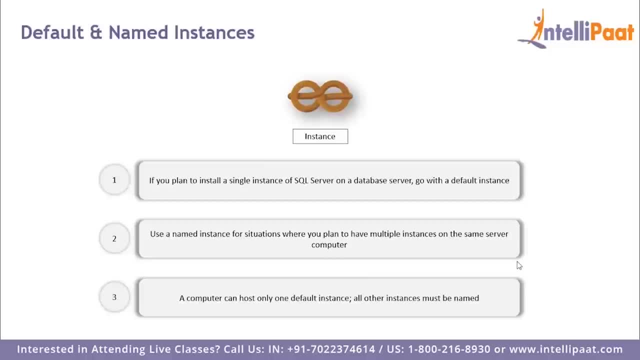 So an instance is either the default named instance or it is a named instance. A default instance does not require a client to specify the name of the instance to make a connection. But a named instance is identified by the network name of the computer plus the instance. 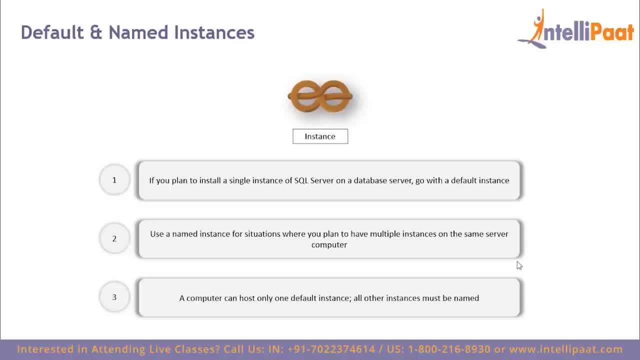 name that you specify during installation. So the client must specify both the server name and the instance name when connecting, And a computer can have only one default instance and all the others must be named. Now let's go ahead and install SQL Server into our systems. 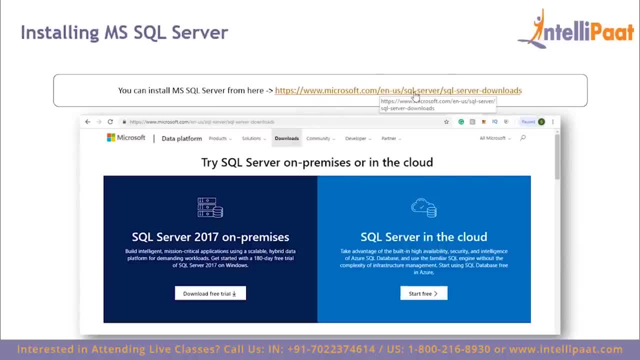 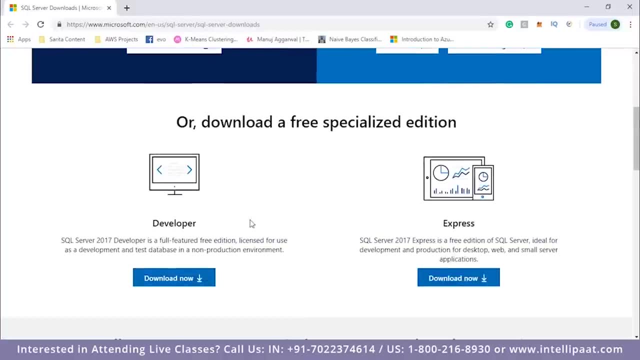 So we can install SQL Server from this site over here. Microsoft SQL Server, SQL Server Downloads. So I'll click on this link. So this is the website And for this course I'll be using the Developer Edition. So all I have to do is click on Download. 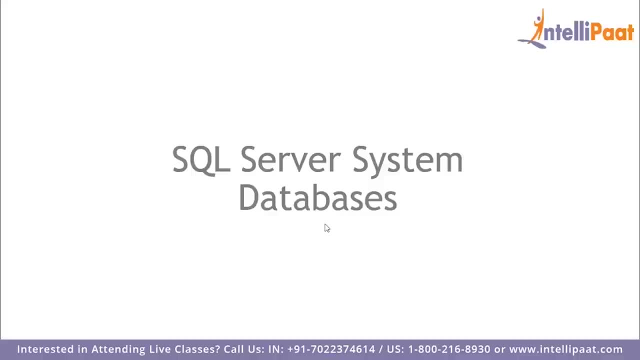 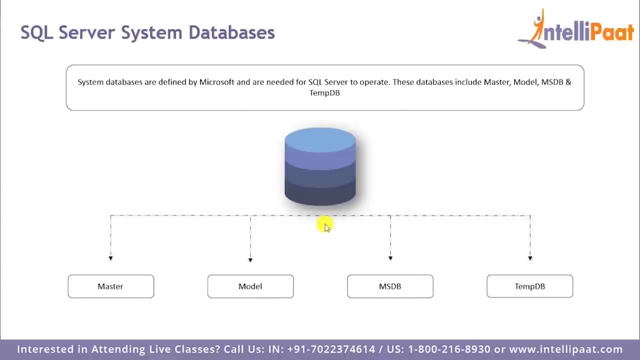 And it'll be downloaded. Now let's look at the different system databases in SQL Server. So when we install Microsoft SQL Server, the system databases are automatically created on every SQL Server instance. These system databases allow the database engine and administrative applications to properly manage the system. 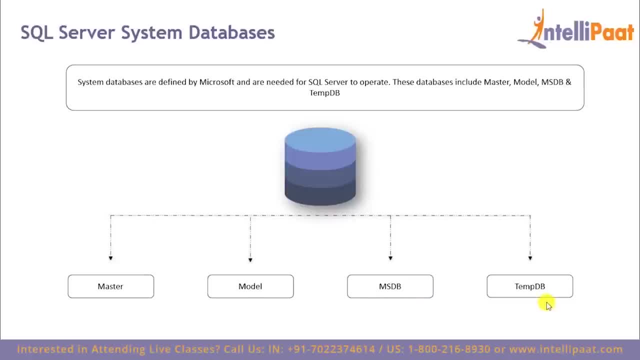 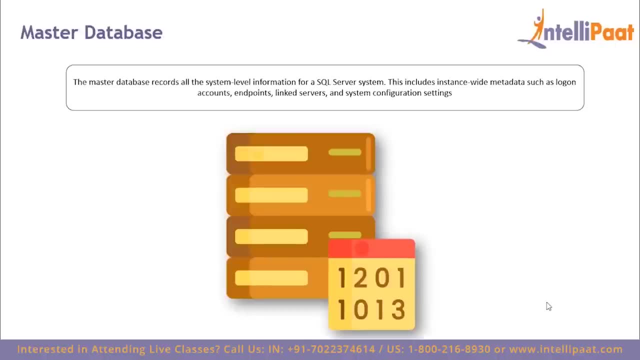 And these are the available system databases: master model, MSDB and tempdb. So let's start with master database. So master database contains all of the system level information for SQL Server, All of the logins, linked servers, endpoints and other system-wide configuration settings. 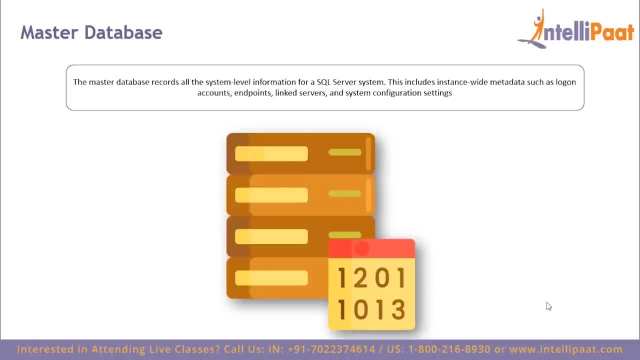 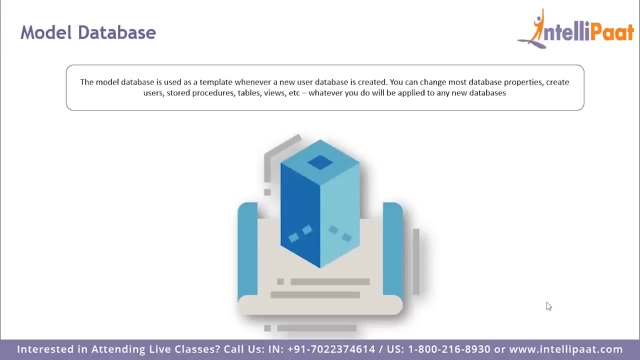 The master database is also where SQL Server stores information about the other databases on this instance and the location of their files. So if the master database is not present, SQL Server cannot start. Then we have the model database. So the model database. 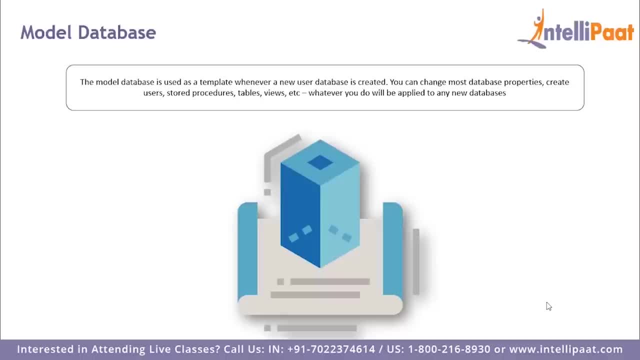 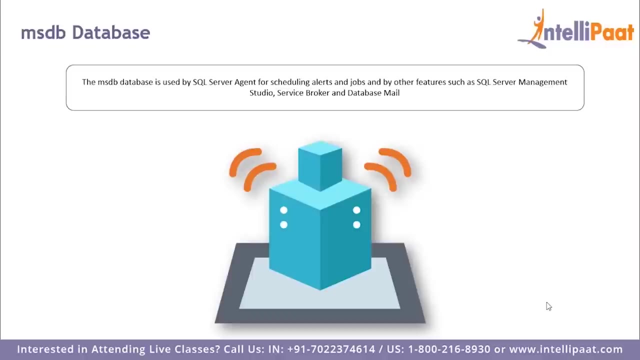 new user database is created, So modifications made to the model database, such as database size, collation, recovery model and other database options, are applied to any databases created afterward. Then we have MSDB, which is used by SQL Server agent for scheduling, alerts and jobs, So MSDB also holds. 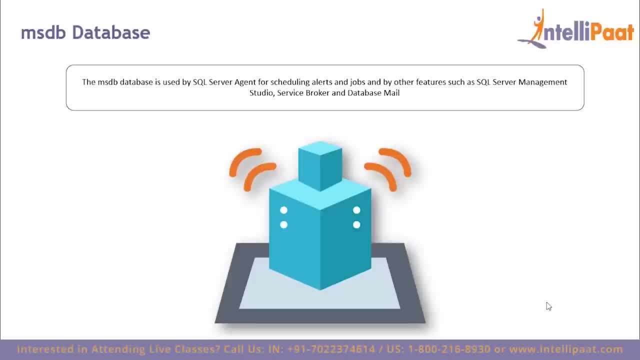 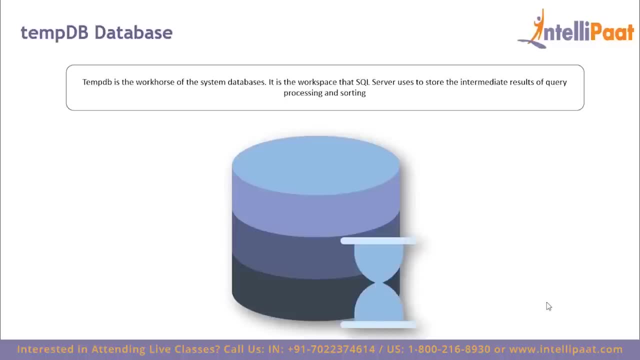 backup history. So using the MSDB tables, it's possible to determine when each database and file group was last backed up. Then we have tempDB, which is basically a workspace for holding temporary objects or intermediate results sets. One interesting thing about tempDB is that it is recreated every. 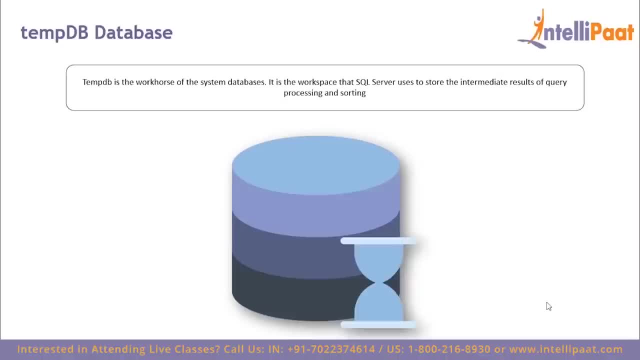 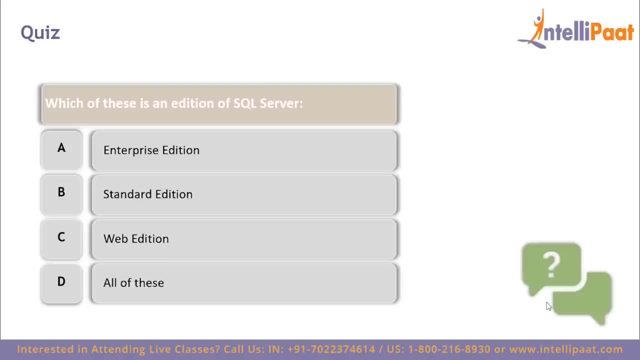 time the SQL Server service is started and any objects that we've created in tempDB will be gone once the server restarts. So now we'll head on to the pop course. So we have this first question: which of these is an edition of SQL Server? The answer is yes. 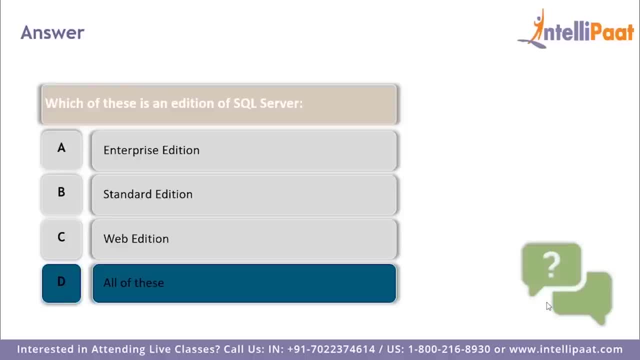 is obviously all of these. so enterprise edition, standard edition and web edition, all of these are different editions of sql server. so next question: which of these is not a sql server system database? so, guys, what do you think? what would be the answer? well, it's slave database. 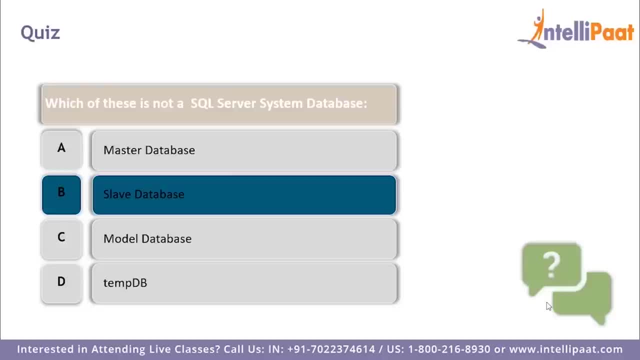 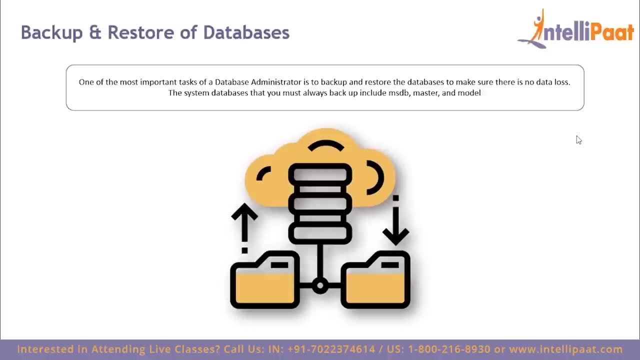 so master database, model database and demdb are system databases, but there is no such system database with the name slave database. so one of the most important tasks of a database administrator is to backup and restore the databases to ensure that there is no data loss and for this purpose. 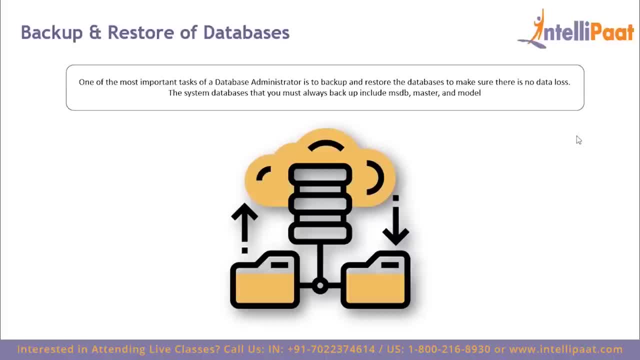 the sql server backup and restore component provides an essential safeguard for protecting critical data stored in our sql server databases. so, to minimize the risk of catastrophic data loss, we need to backup our databases to preserve modifications to our data on a regular basis, and this is where a well-planned backup and restore strategy helps in protecting our database. 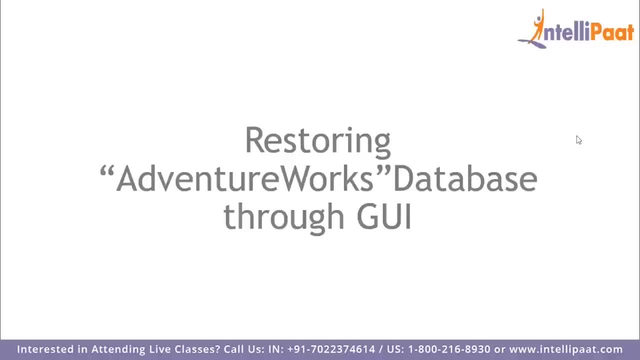 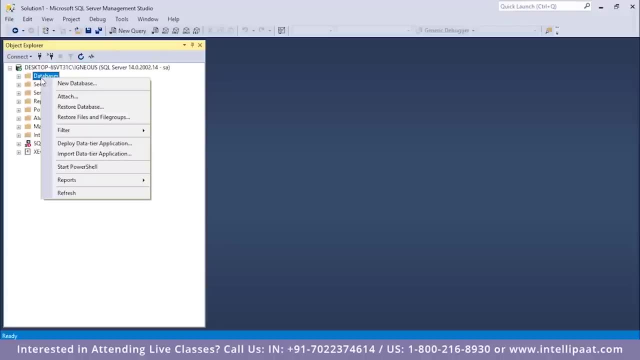 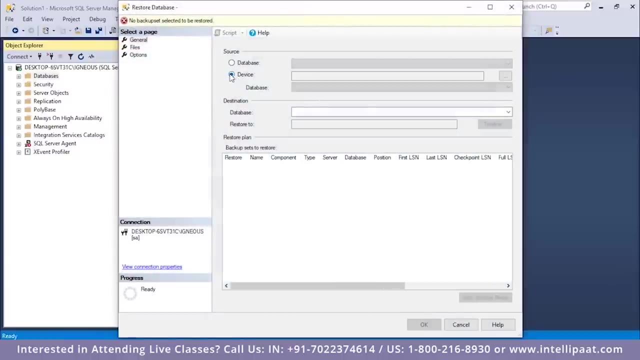 against data loss caused by a variety of failures. Now it's time to restore and backup the AdventureWorks database. So I will right click on this databases folder over here and, since I want to restore the AdventureWorks database, I will select this option- restore database- and I will set the source to be device. 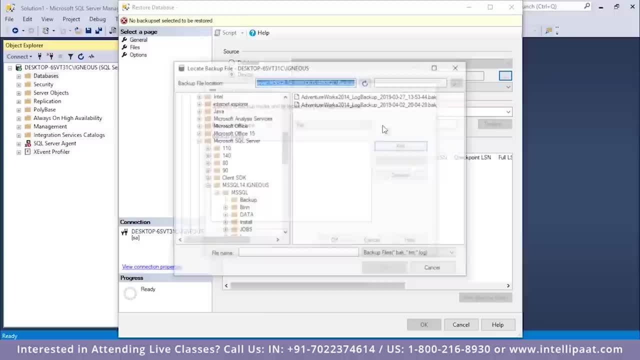 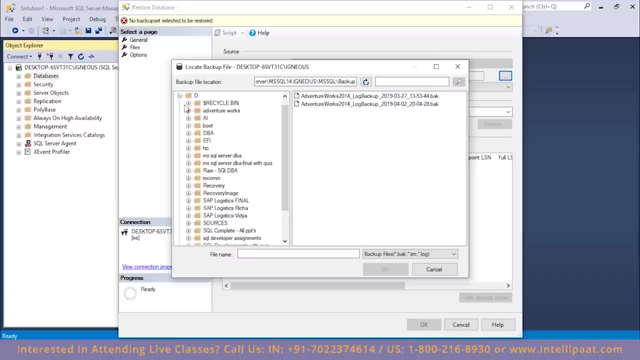 and I will add a device. So that would basically be the file which I have to add. So I will go to the D Drive and so inside D Drive I have this AdventureWorks folder and this is my database over here: AdventureWorks 2014.. I'll click on OK Again. I'll select this. 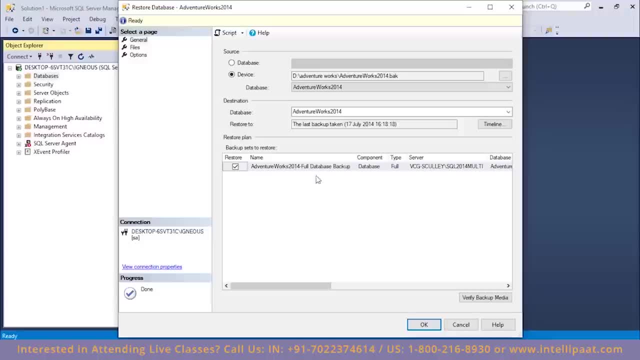 and I'll click on OK. So I have successfully added this AdventureWorks 2014 database. Now I'll click on OK and I'll just wait for the database to be restored. Right, so we get this message: that database AdventureWorks 2014 has been. 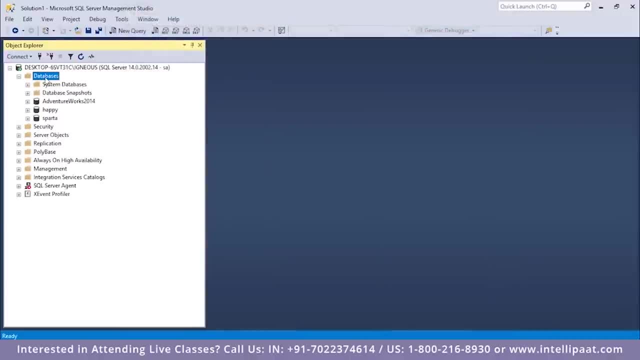 restored successfully. Now, if I open this databases folder, I will refresh this and we see that we have this AdventureWorks 2014 database over here. Now my next task would be to make a backup of this database, So for that purpose, I will right click on this. 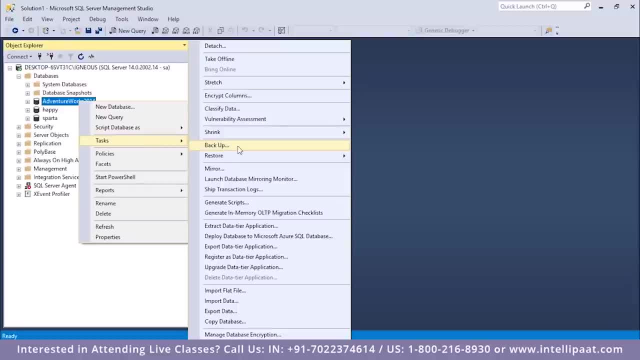 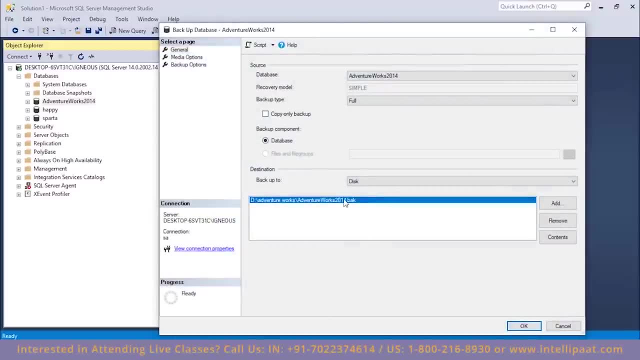 and then select tasks and I have this option of backup. I'll select this. Now I will remove all of the previous backup models which I had created, So I will select this. I'll click on remove Now. I will click add and add a new backup. Let me name that to be new backup. I'll. 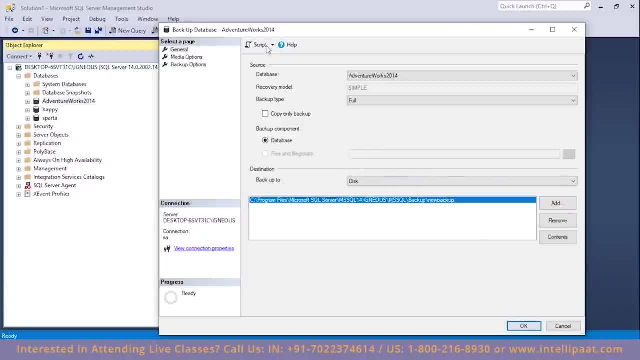 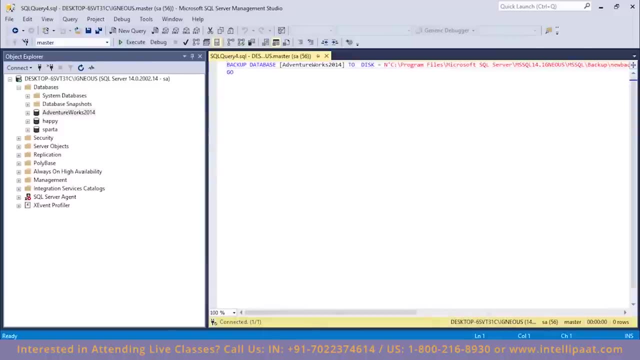 click on OK. Now again, if I want the TSQL code for this, all I have to do is select this script, and this would be the TSQL code to get a full backup of this AdventureWorks database. So now I'll select OK Again. let me wait till the. 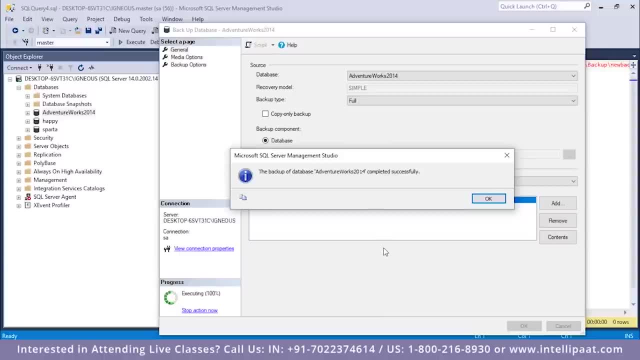 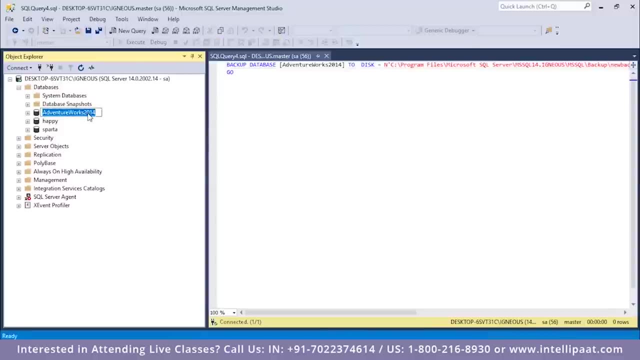 backup is completed. So we get this message that the backup of database AdventureWorks 2014 has been completed successfully. Right, so first we went ahead and restored this AdventureWorks 2014 database and after that, I made a full backup of this database. Now let's look. 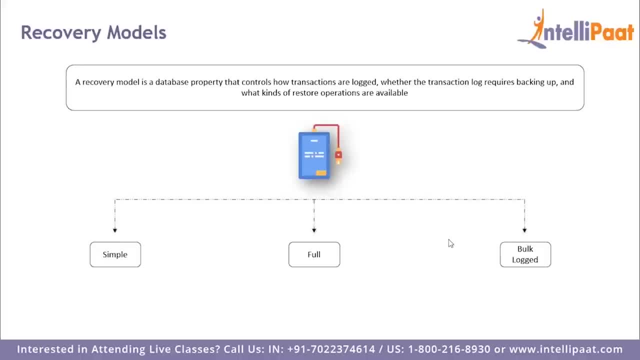 at recovery models. So recovery model is basically your database property that controls how transactions are logged, whether the transaction log requires backing up and what kinds of restore operations are available, and all of the backup, restore and recovery operations are based on one of these three available recovery models. 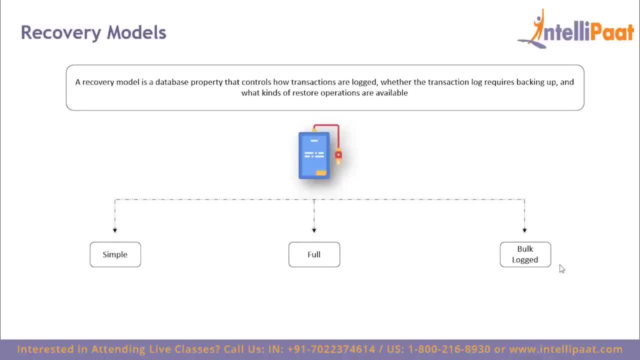 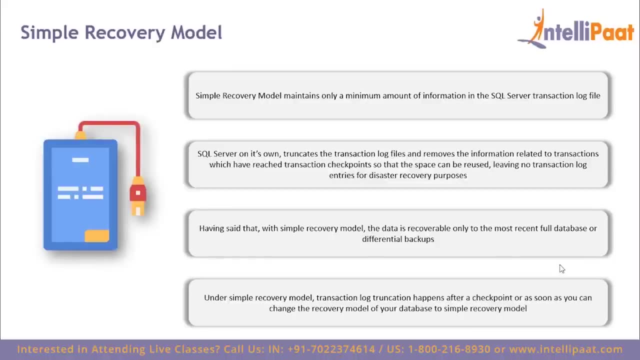 models which are simple, full and bulk logged recovery models. So let's start with simple recovery model. Well, as the name suggests, it is the simplest among the available models. So when we choose the simple recovery model, SQL Server maintains only a minimum amount of information in the transaction log and 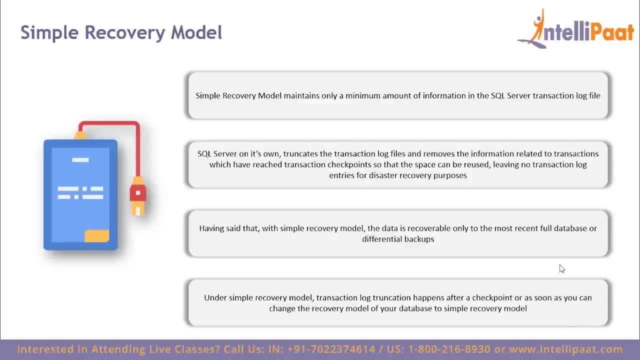 while using the simple recovery model, we may restore full or differential backups only. So it's not possible to restore such a database to a given point in time, and we may only restore it to the time when a full or differential backup occurred. Therefore, it will automatically lose any data modifications made between. 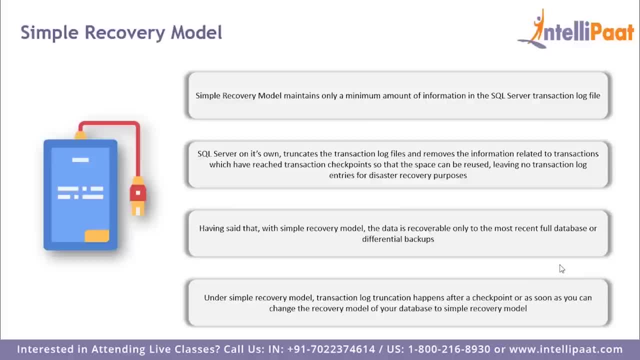 the time of the most recent full or differential backup and the time of the failure. So the simple recovery model requires very less administration and it is easier to manage in the full or bulk logged models. But there would be higher data loss if a data file is damaged. So next we 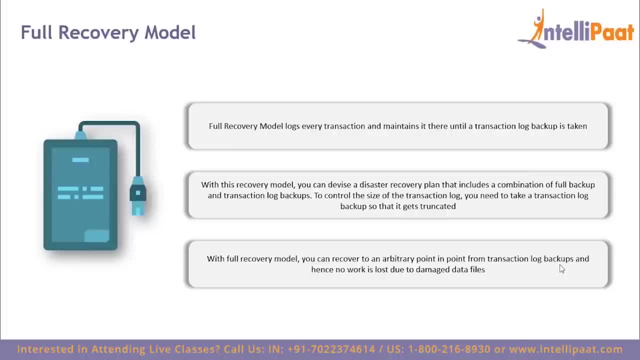 have full recovery model SQL Server, which is more straightforward. It has a recovery model. So with the full recovery model, all the transactions are fully recorded in the transaction log file, and this allows us to design a disaster recovery plan that includes a combination of full and differential. 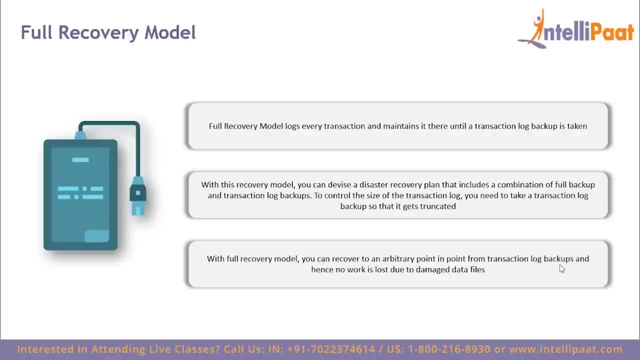 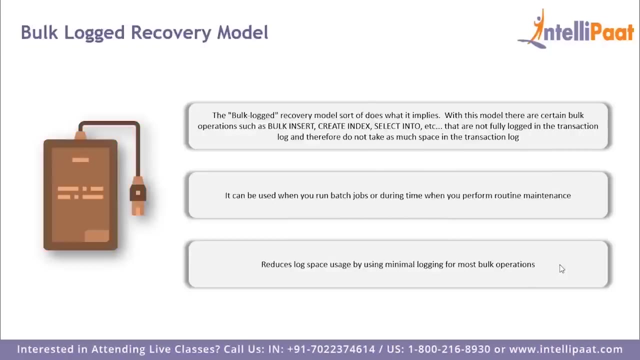 database backups in conjunction with transaction log backups, And in addition to preserving data modifications stored in the transaction log, the full recovery model also allows us to restore a database to a specific point in time, and hence no work is lost due to a damaged file. Next, we have bulk log model, The 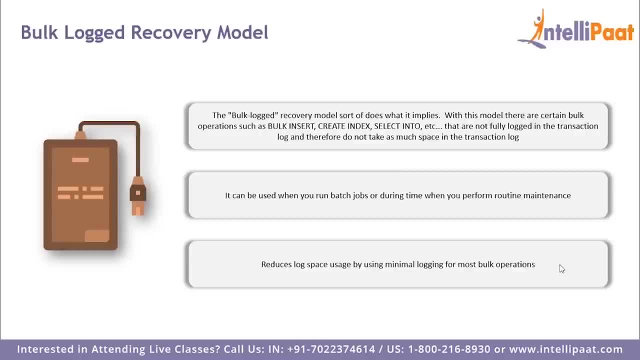 bulk log recovery model is a special purpose model that works in a similar manner to the full recovery model. The only difference is in the way it handles bulk data modification operations. So the bulk log model records these operations in the transaction log using the technique known as minimal logging. So 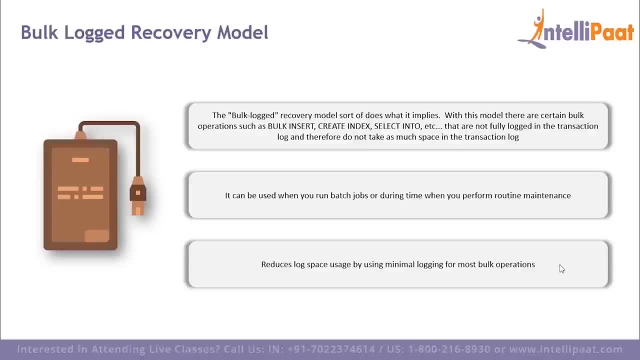 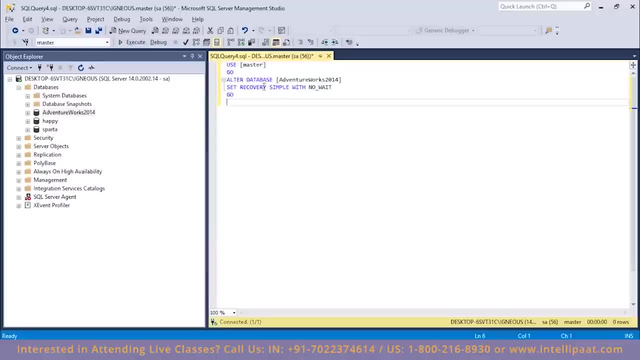 this saves significantly on processing time but prevents us from using the point in time restore option. So now let's change these recovery models in SSMS. So this would be the command to set the recovery model to be simple. So set recovery simple with no wait. go, Let me just execute it So see that commands have. 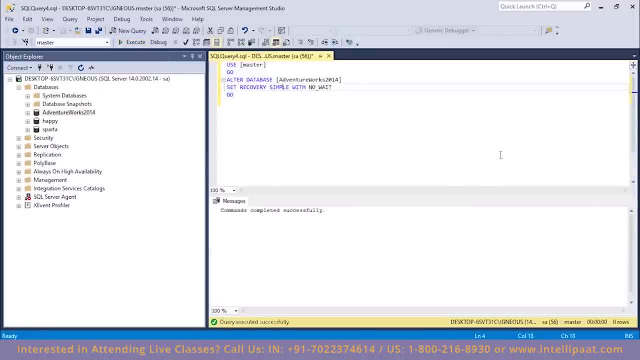 been completed successfully. Now, if I want to change this recovery model from simple to full, all I have to do is write full over here Now I'll click on execute. So this time we have changed the recovery model from simple to full. Now again, if I 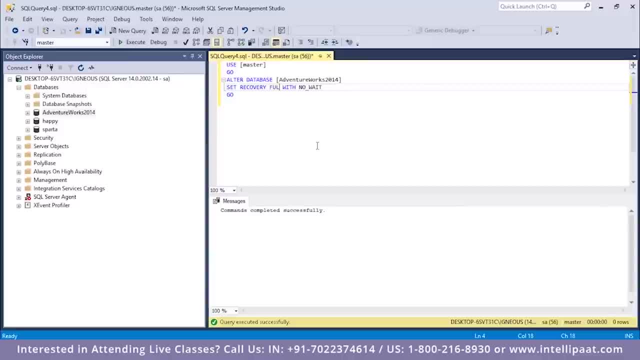 want to change this recovery model from full to bulk log. all I have to do is type in bulk underscore logged over here, I click on execute Right. so this time the recovery model which we are using is bulk log. Now let's see how can we plan. 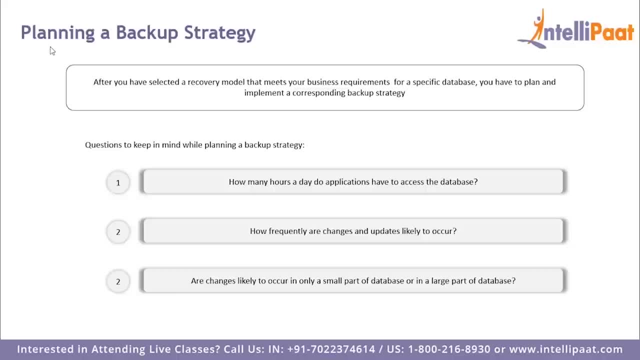 our backup strategy. So, after we have selected the recovery model that meets our business requirements for a specific database, we have to plan and implement a corresponding backup strategy. So these are some of the questions which we'd have to keep in mind while we are implementing our 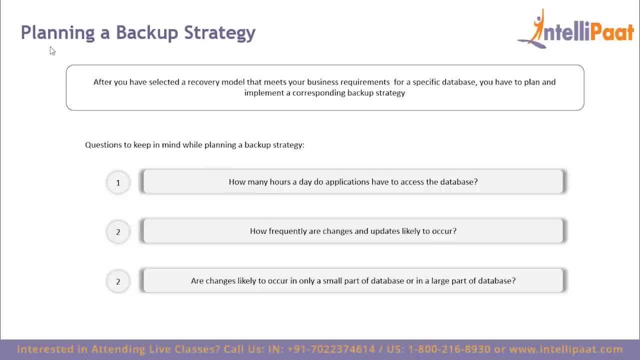 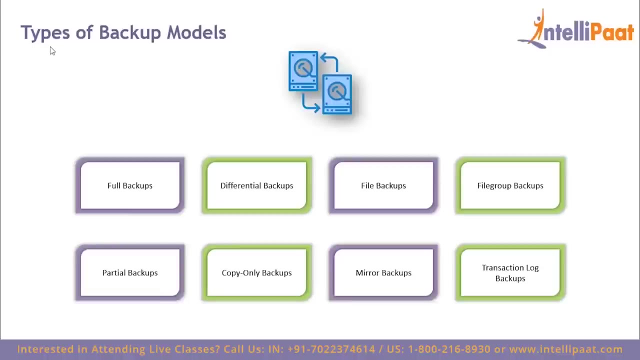 planning a backup strategy. How many hours a day do applications have to access the database And how frequently are changes and updates likely to occur? And are these changes likely to occur in only a small part of the database or in a large part of the database? And these are the different types of backup models. 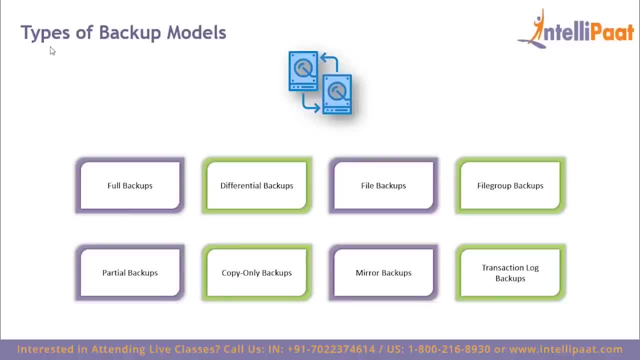 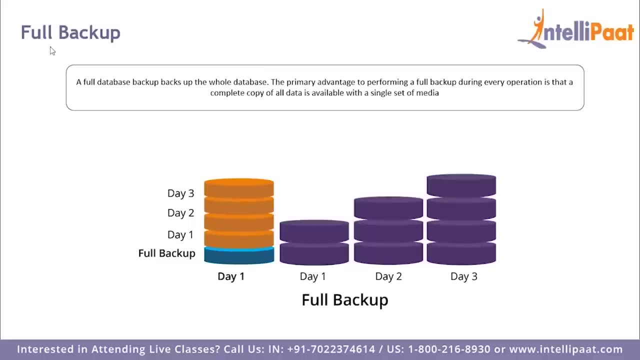 which we can use. So we have full backups, differential backups, file and file group backups, partial backups, copy only backups, mirror backups and transaction log backups. So a full backup, as the name implies, backs up everything. It is the 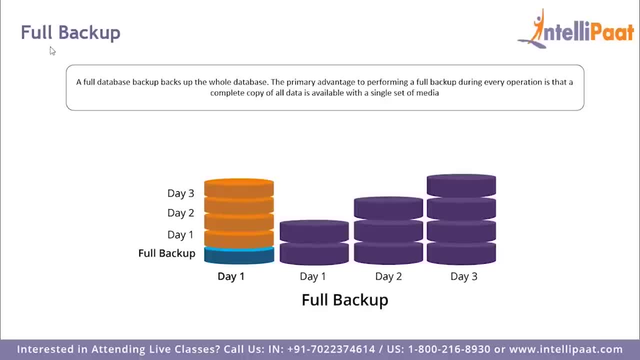 foundation of any kind of backup. So this is a complete copy which stores all the objects of the database, ie tables, procedures, functions, views, indexes, so basically everything. So the full backup will be able to easily restore a database in exactly the same form as it was at the time of the backup. Then we 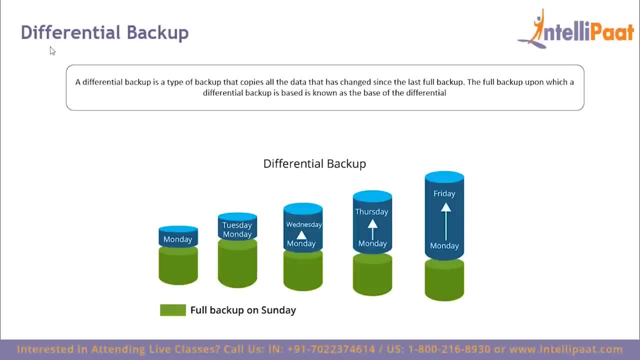 have differential backup. So you can consider a differential backup in the build-in 不通建柱 Type ID comenz活用 志 statement database backup to be the superset of the last full backup and it contains all changes that have been made since the last full backup. so if there are very 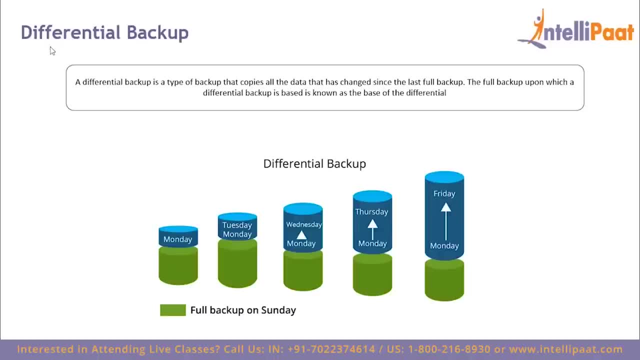 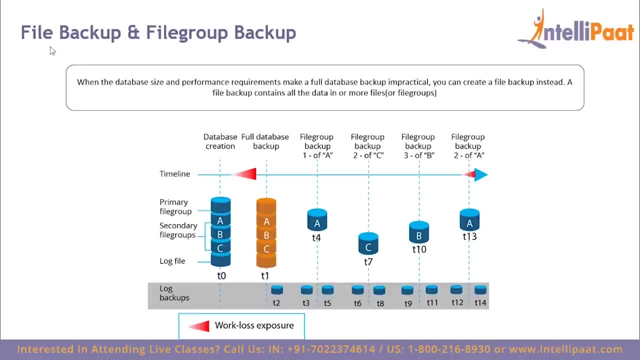 few transactions that have happened recently, a differential backup might be small in size, but if you made a large number of transactions the differential backup could be very large in size. then we have file and file group backup. so whenever the database size and performance requirements make a full 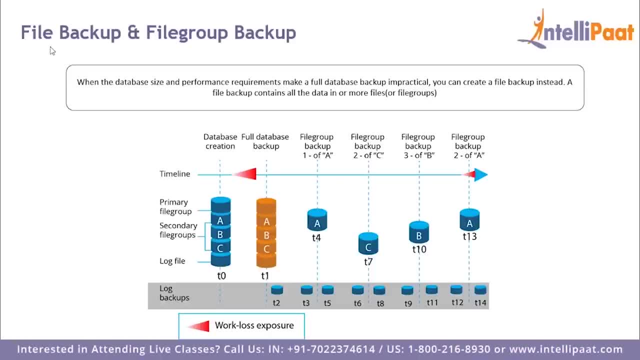 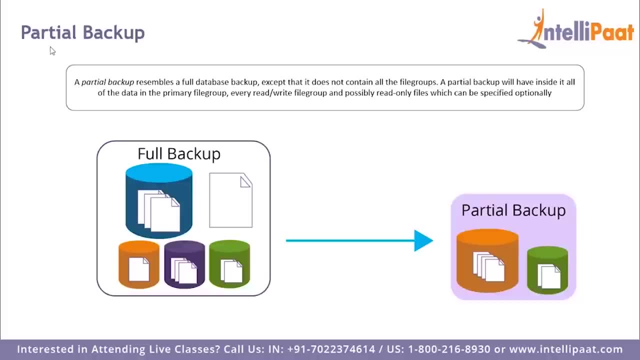 database backup impractical. we can create a file backup instead. so a file backup contains all the data in one or more files, which are known as file groups. then we have partial backup. so partial backups allow us to back up only a subset of the data files. so these partial backups will make a backup copy. 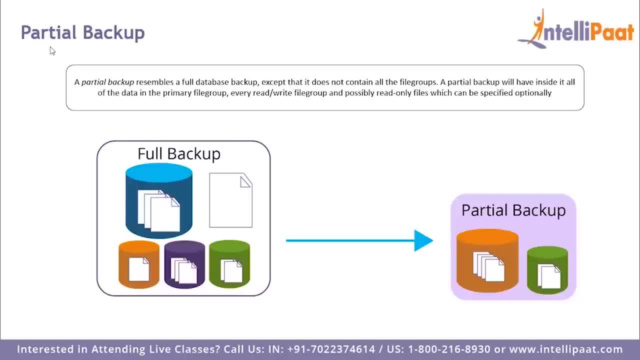 of the primary file group and all read write file groups and by default they will omit any file groups designated as all read-only. this means that partial backups are only relevant for databases that contain read-only file groups. otherwise, a partial backup will capture exactly the same data and objects as an equivalent full database backup. so next, 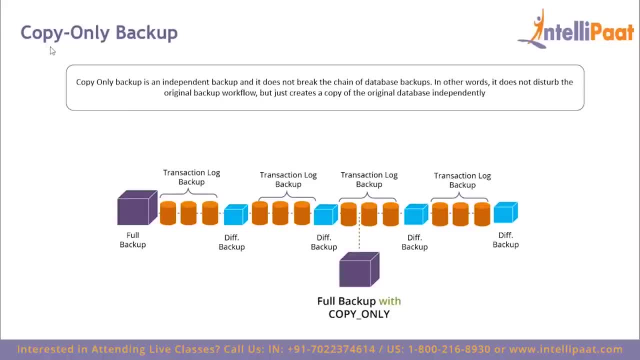 we have copy only backup. so a copy only backup is a sequel server backup that is independent of the sequence of conventional sequel server backups. usually taking a backup changes the database and affects how later backups are reached restored. however, occasionally it is useful to take a backup for a special 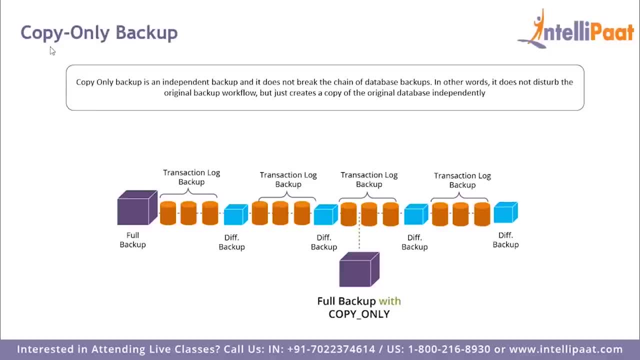 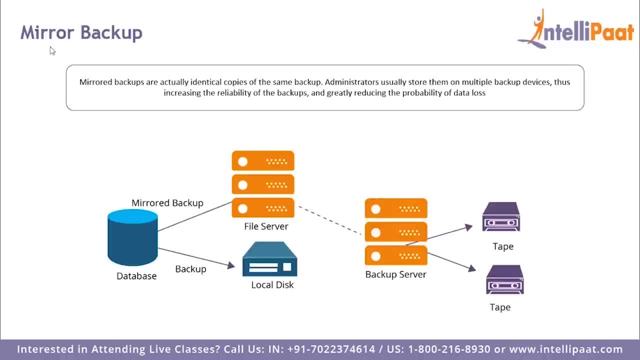 purpose, without affecting the overall backup and restore procedures for the database, and this is exactly where a copy only backup can be used. then we have mirror backup, so mirror backups are actually identical copies of the same backup, and these identical copies are stored on multiple locations. so this 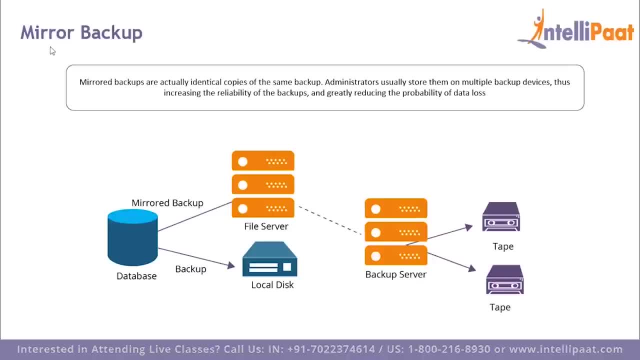 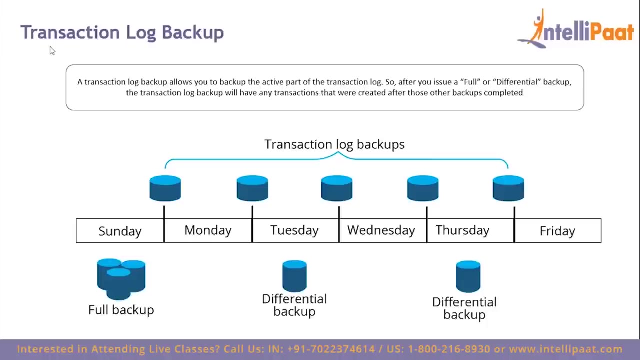 increases the protection level by having additional copies of the backup set and in case one of the copies gets lost or is corrupted, we can use the mirrored copy to perform a restore. so, finally, we have the transaction log backup. so our transaction log backup allows us to backup. 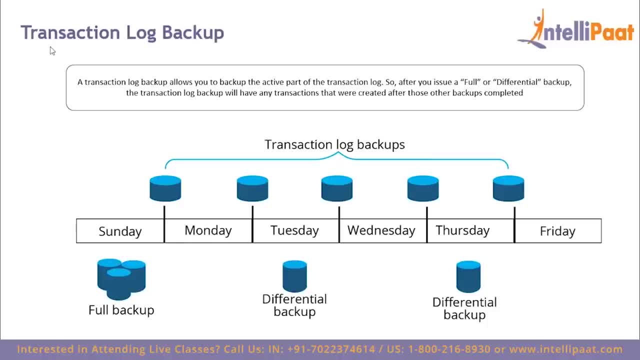 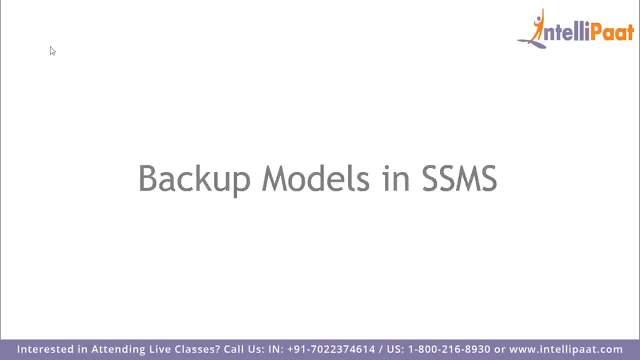 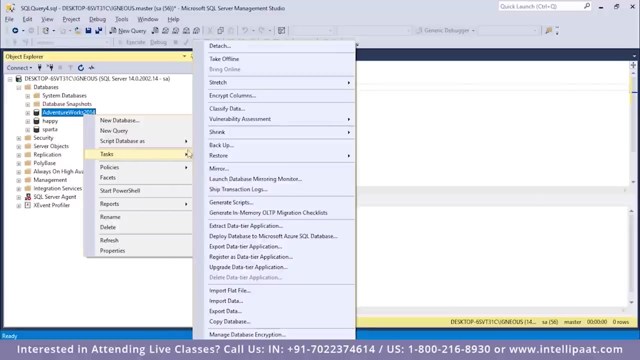 the active part of the transaction log. so after we issue a full or differential backup, the transaction log backup will have only those transactions that were created after those other backups had completed. so now let's implement backup models in SSMS. so now again, I will select this Adventure works database and right-click on it, I will select tasks and since I want to 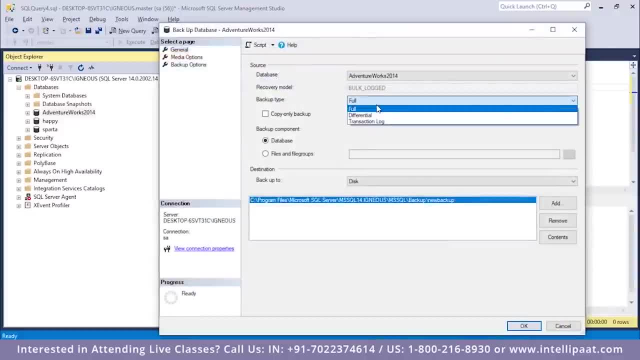 backup, I click on backup. so this time I want a differential backup, so I'll select differential and all I have to do is click on ok. and before that, if I also want the tsql code for this, all I have to do is click on script and this is the. 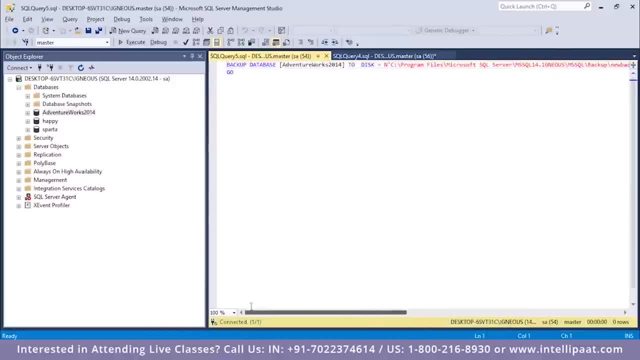 t-sql code. to get the differential backup of this database, I will click on entendang theydi AskPожд Bead core code. okay, So see that the backup of the database has been completed successfully Now. similarly, if I want to get a transaction log backup, I'll right click this: tasks backup. 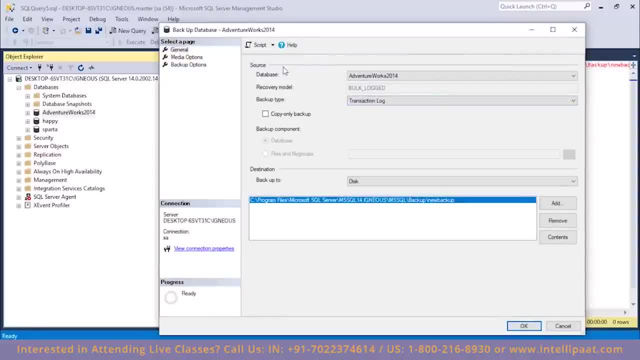 And this time, instead of choosing full, I'll select transaction log And again, if I want the TSQL code, I'll click on script. So I'll just click on OK. So this time we have a transaction log. backup of the adventureworks 2014 database. 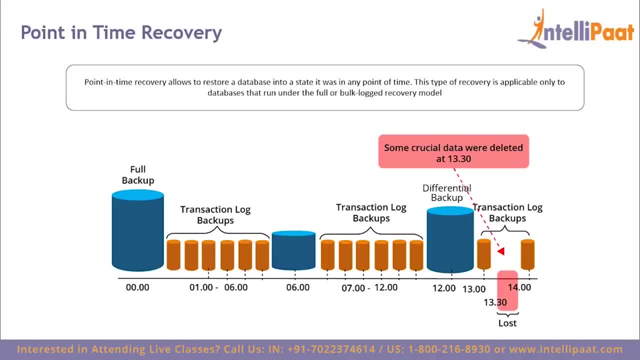 So now let's understand what is point in time recovery. So point in time recovery allows us to restore a database into a state it was in at any point of time. This type of recovery is applicable only to databases that run under the full or bulk. log recovery model. So now let's implement point in time recovery in SSMS. So I have this adventureworks 2014 database over here. I'll right click this, select tasks, I'll click on restore database And I have this timeline option over here. 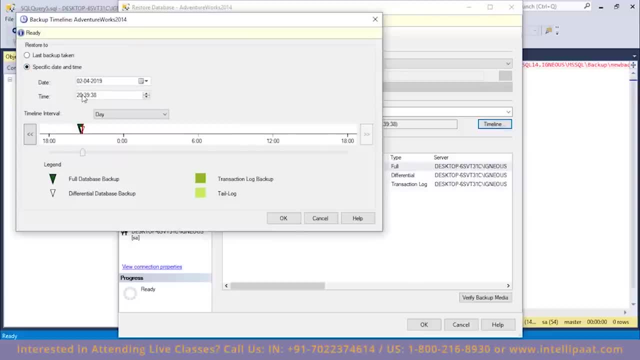 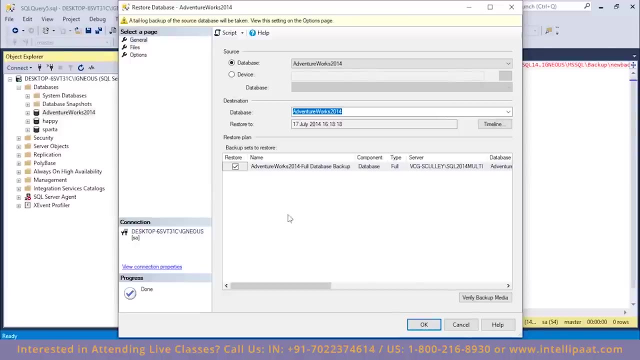 So I'll select timeline And I will set a specific date and time. So I want to recover this database from two hours back, So I'll set this to be 18. And I will click on OK, right. So this is how we can do point in time recovery. 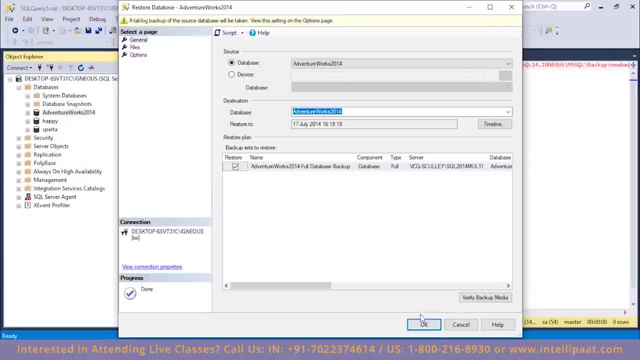 So again, if I want the TSQL code for this, all I have to do is click on script, But for now I'll click on OK. So we've successfully got the point in time recovery. So we've successfully got the point in time recovery. 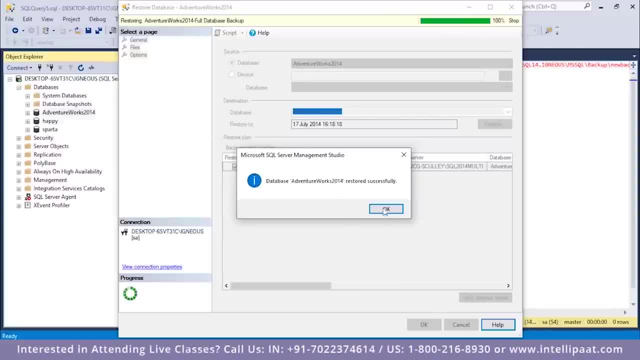 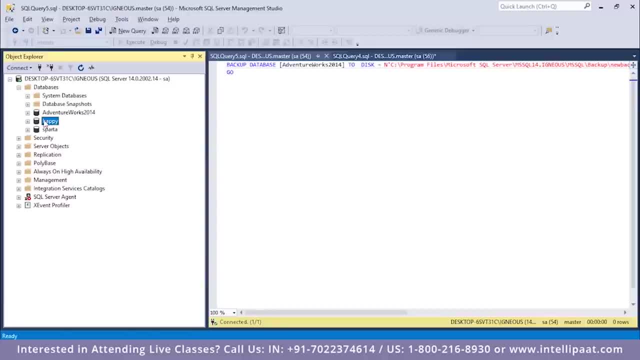 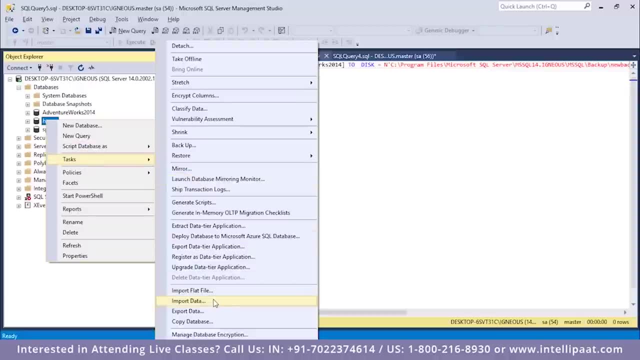 So I have this happy database over here And I want to import a flat file into this database. So for that I'll right click this. I have the option of tasks And over here I have to select import data. I have to set the data source. 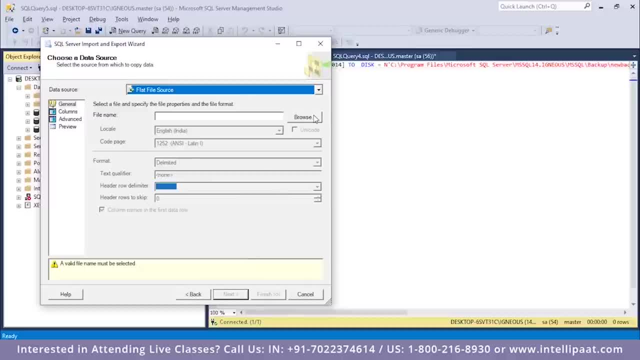 So the data source would be a flat file- flat file source. Now let me browse that flat file. So I have this new file over here. I can just reset it, So let me save this. I'll open this now. all I have to do is keep clicking on next. so this is the. 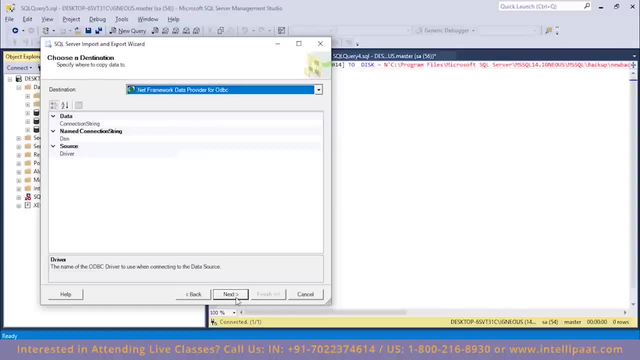 data which is present in this flat file. click on next and then I'd have to set the destination. so I want to store this into my database. so the database would be sequel server- native client. now this will be stored in this happy data face. I'll click on next next and I'll have to click on finish over here. so you see. 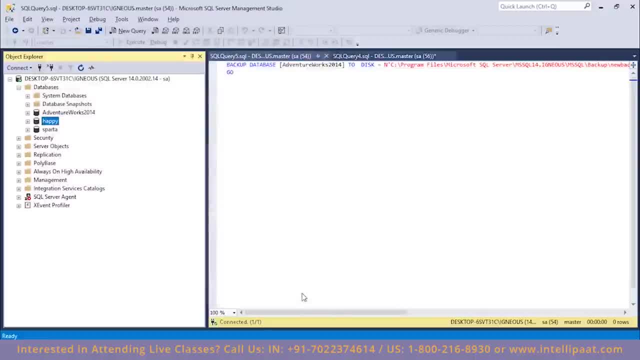 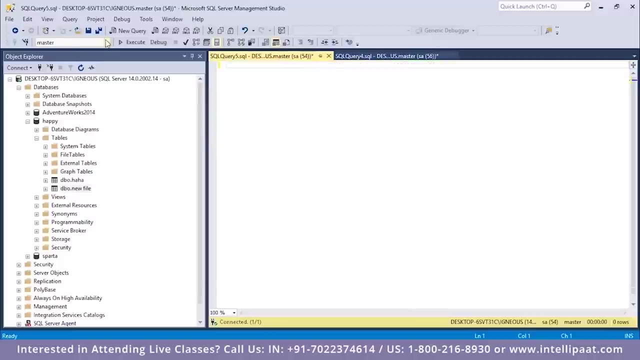 that we have successfully imported this flat file into our database. now let me refresh this. let me have a look at the tables over here. so we have imported this new file into this database now. let me go to this database first, which would be happy over here. so select star from. 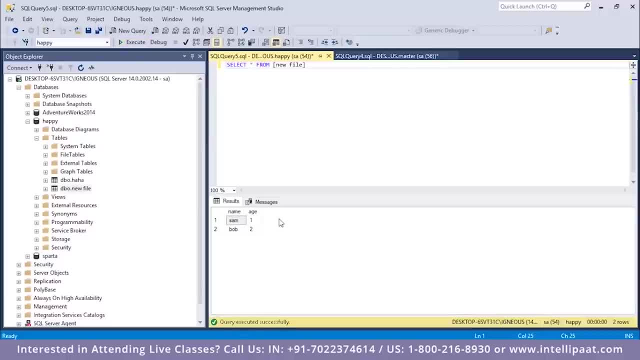 new file. I'll execute right. so we have successfully imported the data set. now what I'll do is add a new row to this file and export this into a new file. so insert into new file. it will be values. and then let's see the name is Anne and her age is three. I'll execute this. now. let me look at the. 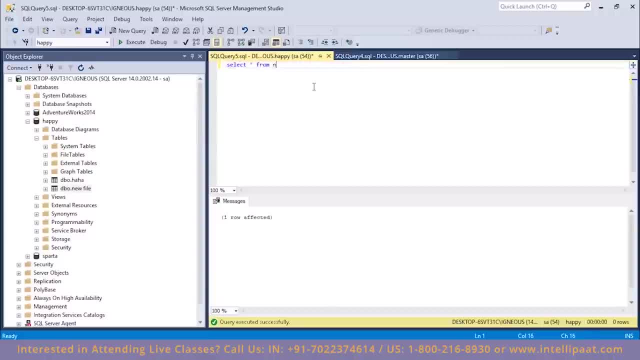 ody the do the modified data. that'll be select star from new file. so we have radically harder this new record now. I had wanted to export this data, so this time again I will right click the database and I will select tasks over. here I have the option of exporting data. now the source would be sequel, so a 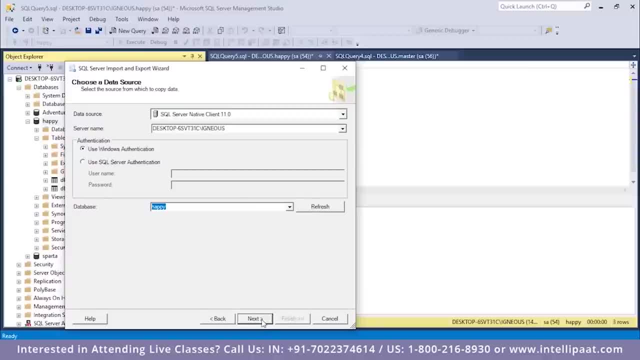 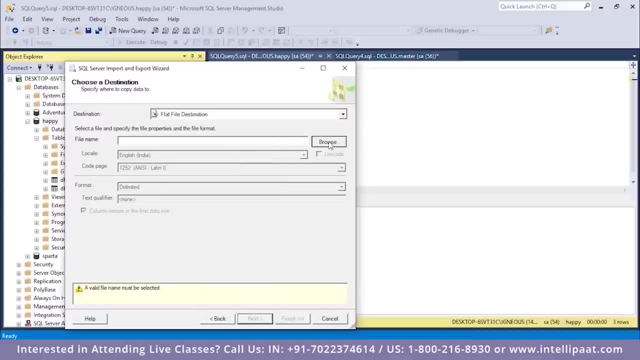 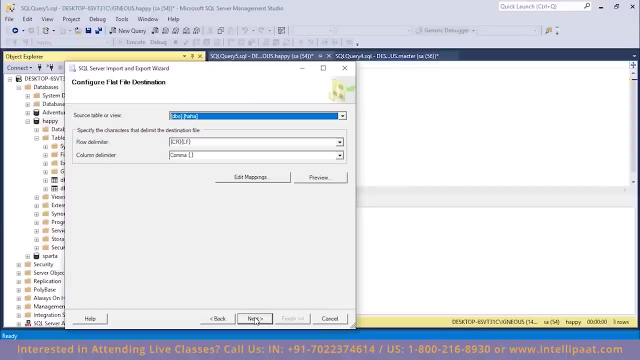 native client. now, this time the database, as again happy. so next I have to choose a destination. so the destination would be a flat file. i'd have to choose a file name over here. so i want to store this into new file too and i'll click on next next. so over here i'd have to choose. 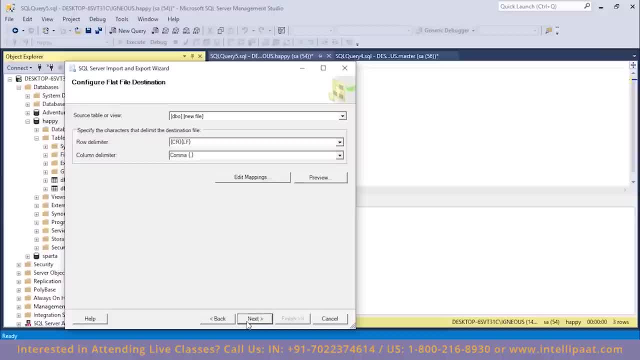 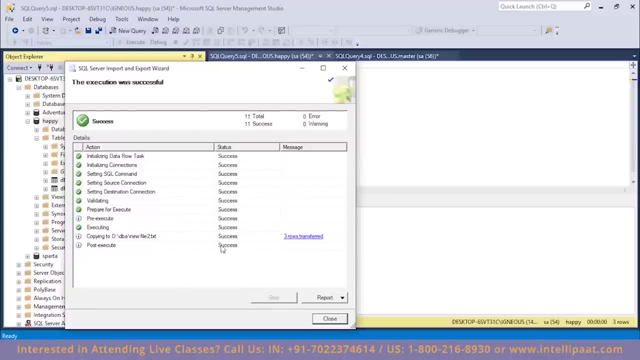 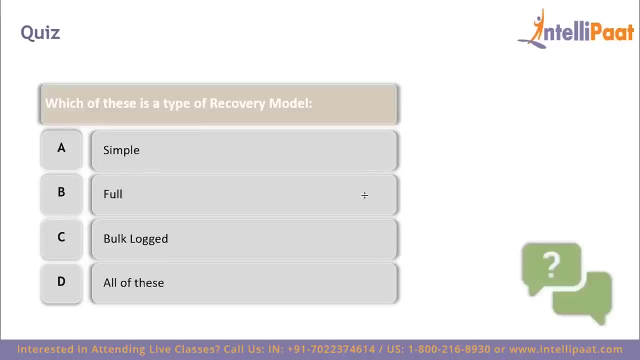 the table which i want to export. so i want to export this new file. i'll click on next now, next again and i'll click on finish. so this time we have successfully exported this data from ssms. so we have this pop quiz over here. so the first question is: which of these is a type of recovery? 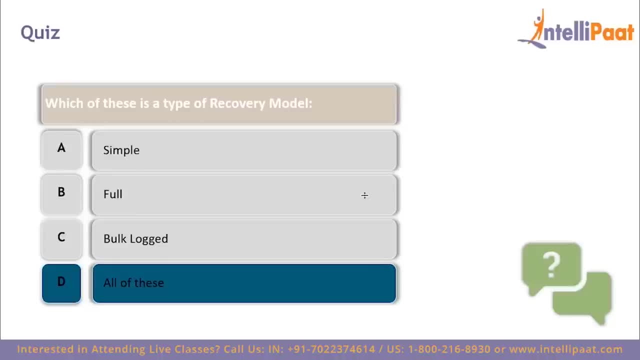 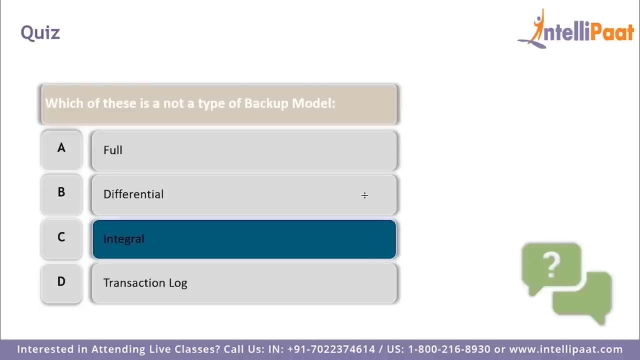 model. so, guys, what do you think? well, all of these, so simple, full and bulk log, all of these are types of recovery models. the next question: which of these is not a type of backup model? so we have full backup, differential backup and transaction log backup, but there is no backup by the name. 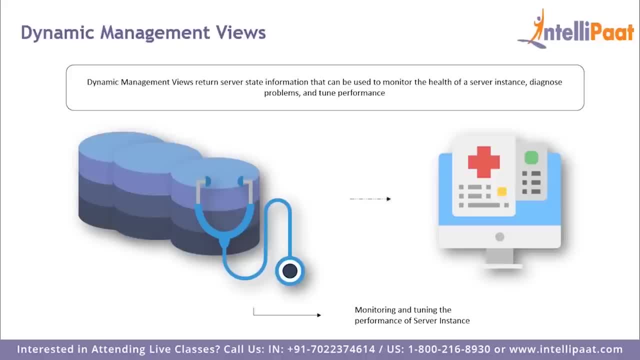 integral backup. so dynamic management views and dynamic management functions are system views, and system functions return metadata of the system state On querying the related system objects. database administrators can understand the internals of SQL Server. So these dynamic management views allow us to monitor the performance of SQL Server. 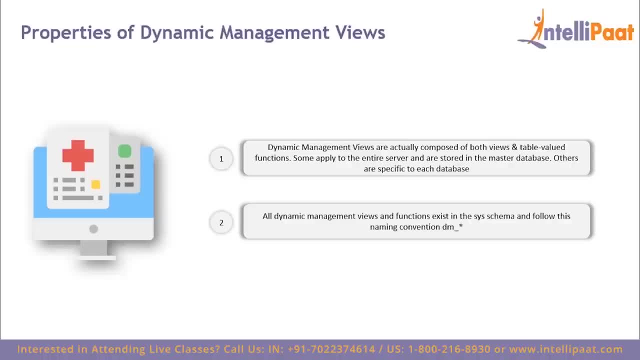 instance, and diagnose issues with it. Now let's look at some of the properties of dynamic management views. So dynamic management views are composed of both views and table-valued functions. Some of them apply to the entire server and are stored in the master database. others are specific to each individual database and 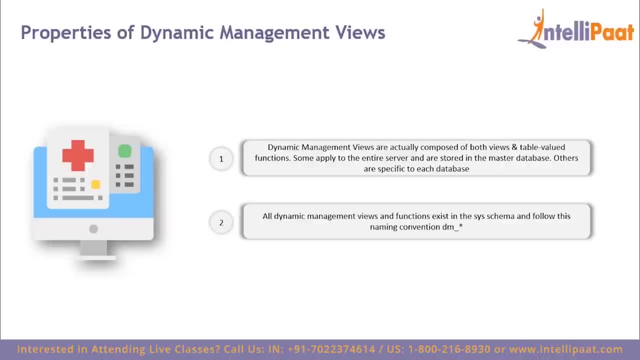 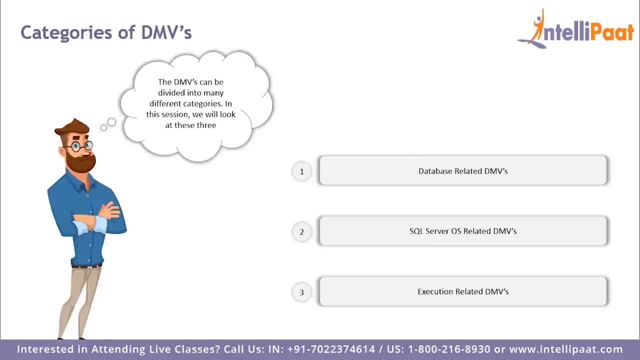 all of these DMVs start with the prefix dm underscore. Now let's look at some categories of DMVs. So DMVs can be divided into many different categories and in the session we'll be looking at three of those. So we'll be looking at 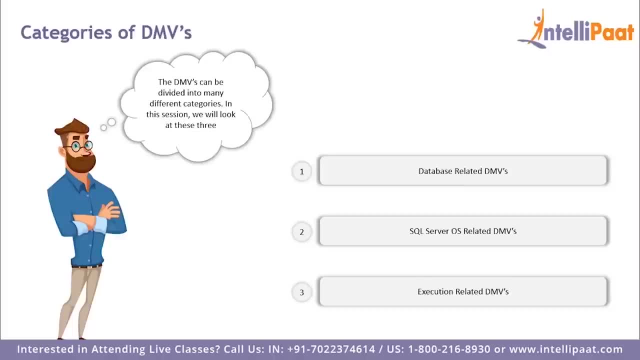 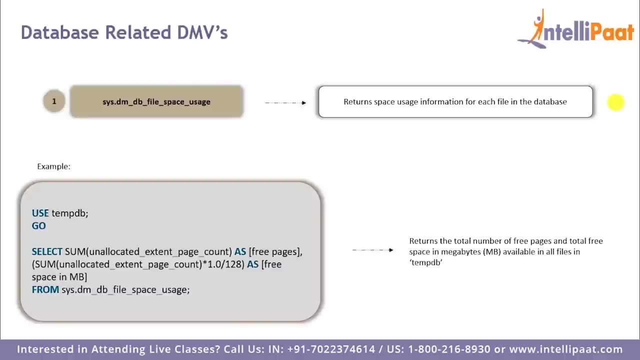 database related DMVs, SQL Server, OS related DMVs and execution related DMVs. So let's start with database related DMVs First. we have dm underscore, db underscore, file, underscore space usage, which returns the space usage information for each file in the database. Now we will use this DMV to get the total number of free pages and total. 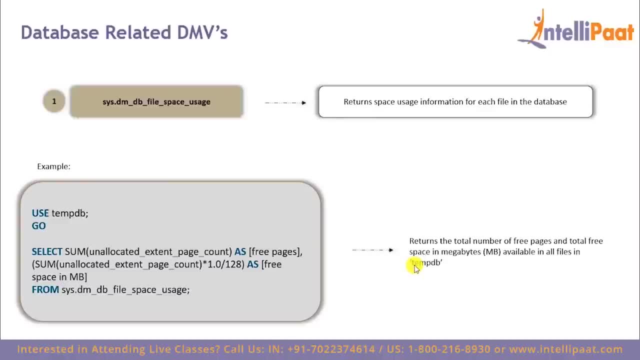 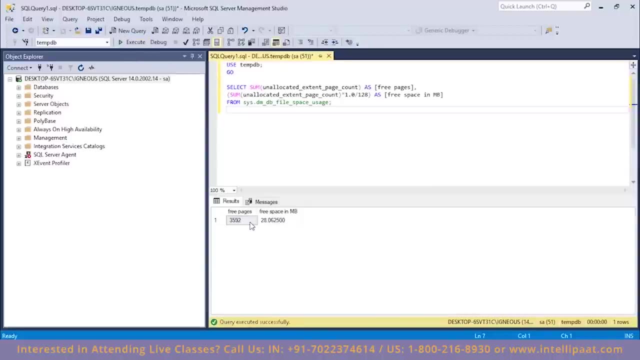 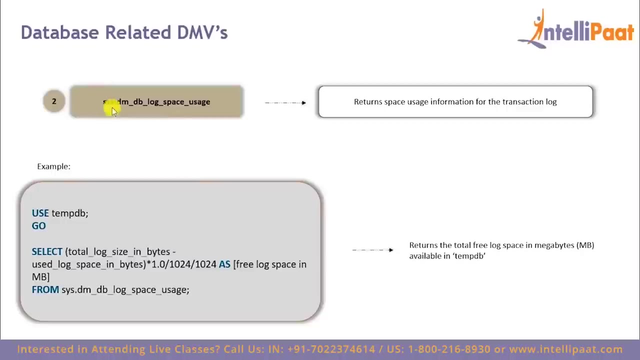 free space in megabytes available in all files in tempdb. So let me just run this command over here. I will click on execute. So the total number of free pages available in tempdb are three thousand five hundred and ninety two and the total free space is twenty eight MB. Next we have dm underscore db. 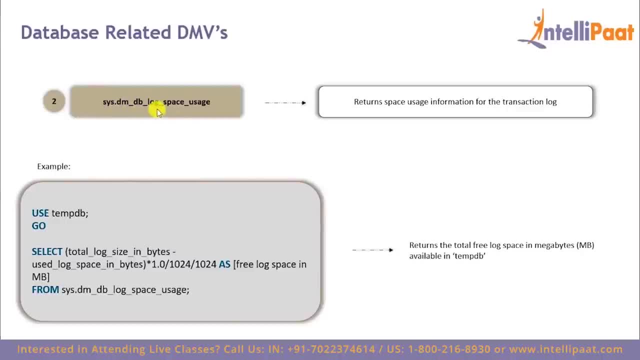 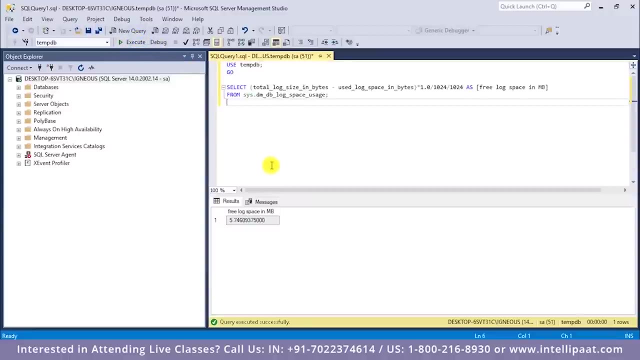 underscore log space usage, which returns space usage information for the transaction log, and we will use this DMV to get the total free log space in megabytes available in tempdb. Again, I will run this command in SSMS, I'll click on execute So see that the total free log space is five point seven, four MB. So 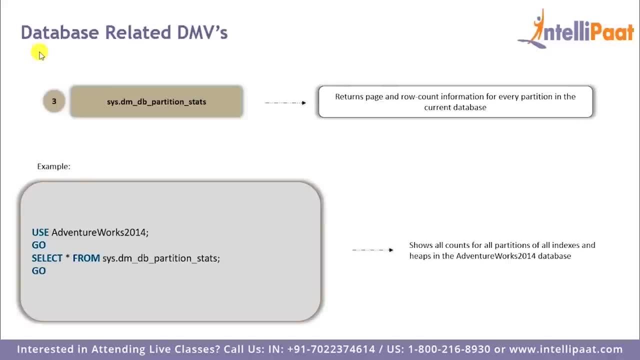 this is the total free log space in tempdb. Next, we have db underscore partition stats, which returns page and row count information for every partition in the current database and this time we will get the counts for all partitions of all indexes and heaps in the AdventureWorks 2014. 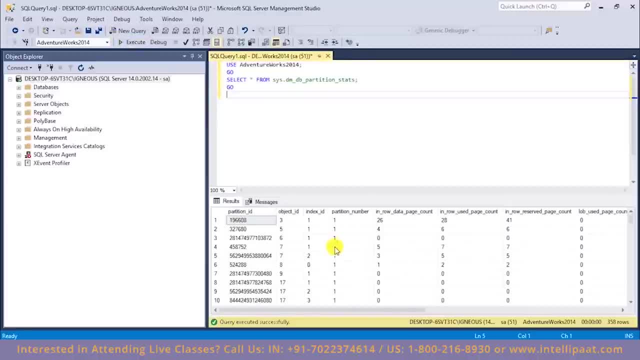 database. Let me click on execute. So these are all of the partition stats for all of the indexes and heaps in the AdventureWorks 2014 database. So here we have different statistics, such as index ID, partition number, data page count and so on and over. here we have the reserved page count, the used 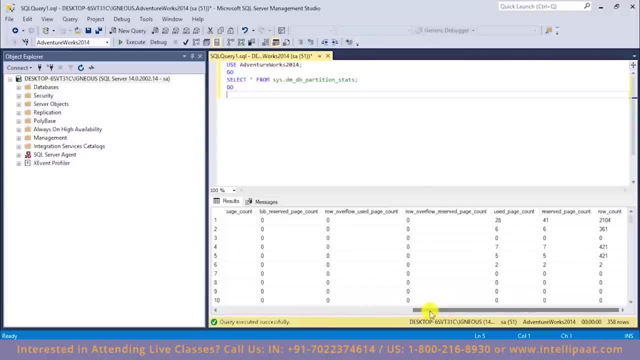 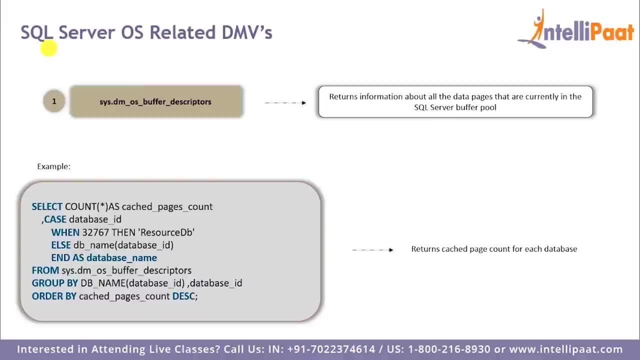 page count the row count Right. so these are all of the partition stats which we can get from this DMV. Next we'll head on to SQL Server OS related DMVs. So first we have the dm underscore OS buffer descriptors, which returns information. 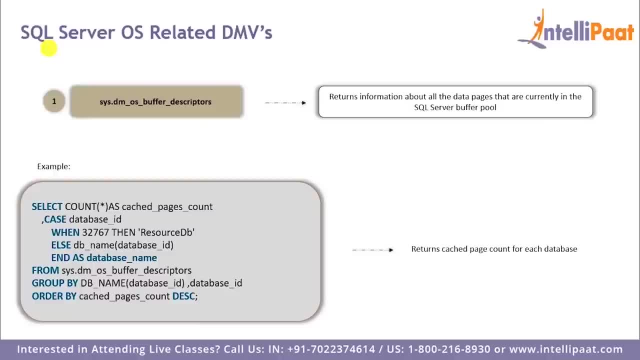 about all the data pages that are currently in the SQL Server buffer pool. So with this command over here we'll get the cached page count for each data base. Again, I'll run this command in SSMS, I'll click on execute. So these are. 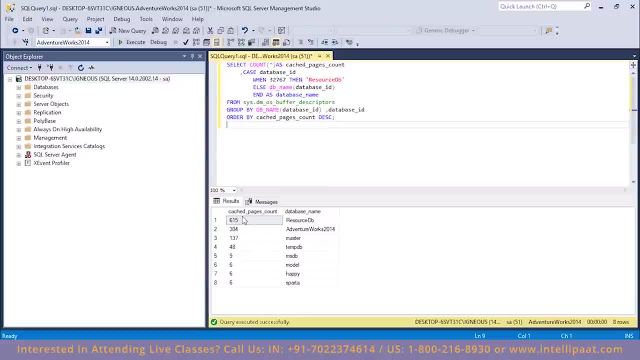 the different databases which I have in SQL Server and this is the cached page count. So in master DB I see that there are 137 cached pages, in MSDB there are nine, in Spada there are six and in AdventureWorks there are 304.. Next we 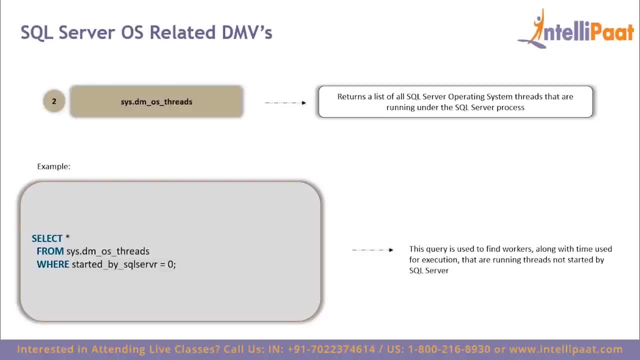 have dm underscore OS threads, which returns a list of all SQL Server operating system threads that are running under the SQL Server process. So this query over here is used to find workers, along with time used for execution and our running threads which are actually not started by SQL Server. 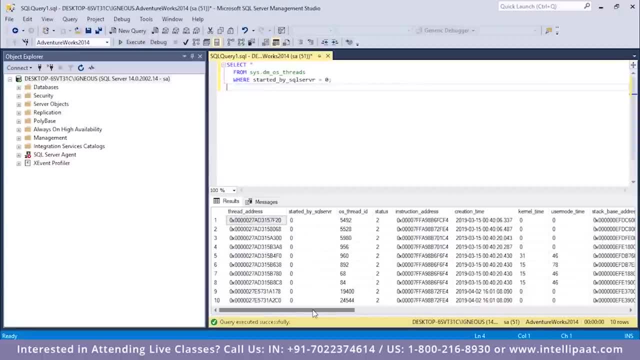 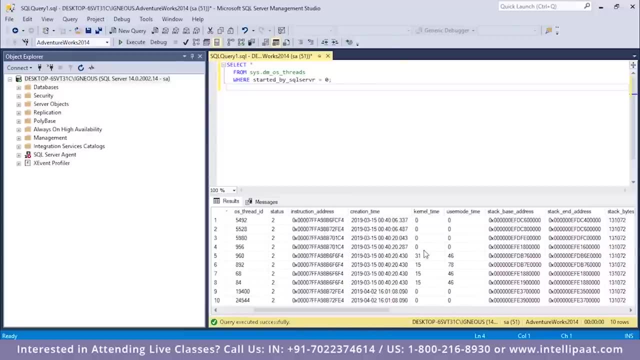 So this is all of the information about the threads which are not yet started by SQL Server. So we have different columns, we have the OS thread ID, the creation time over here, the kernel time, user mode time and over here at the back end of it. 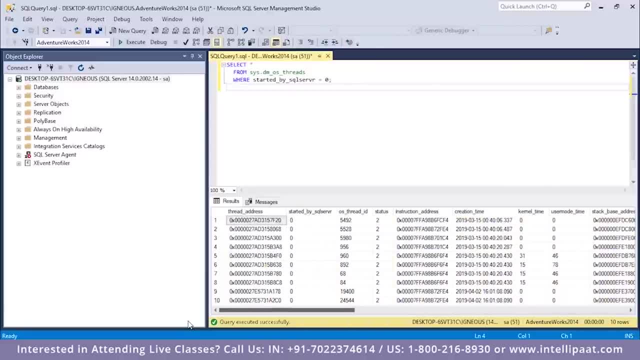 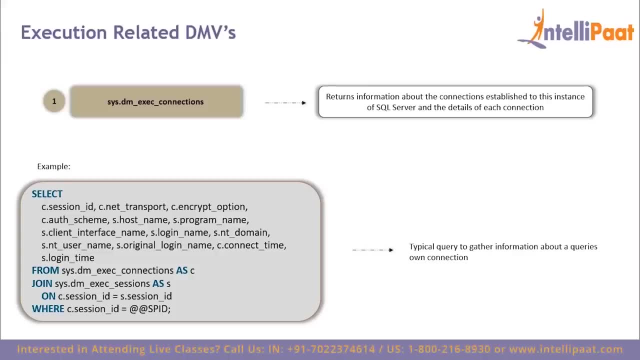 we've got the address associated with each of these threads over here. Now it's time for the third category of DMVs, which is execution related. So first we have dm underscore exec connections, which returns information about the connections established to this instance of SQL Server and the details of each. 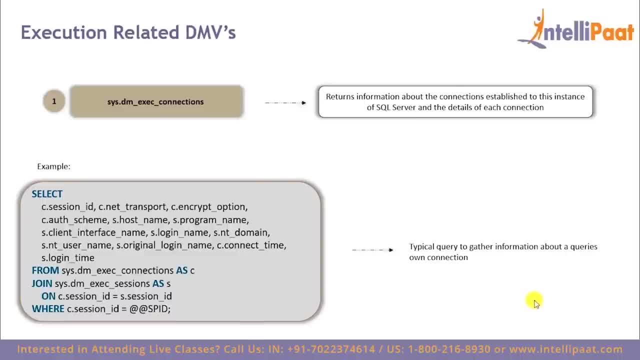 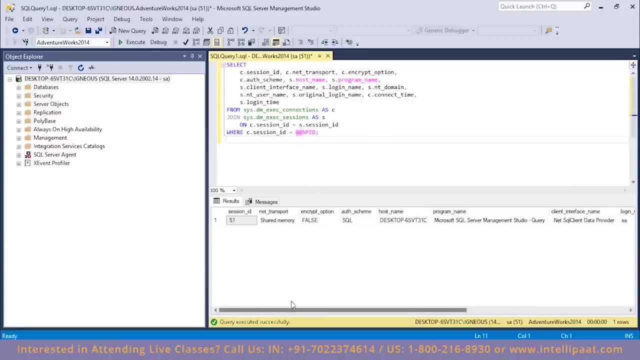 connection, And this command over here is used to gather information about a query's own connection. So for this query we see that the session ID is 51 and we have other columns as well, so we have the host name over here. this is the host name. 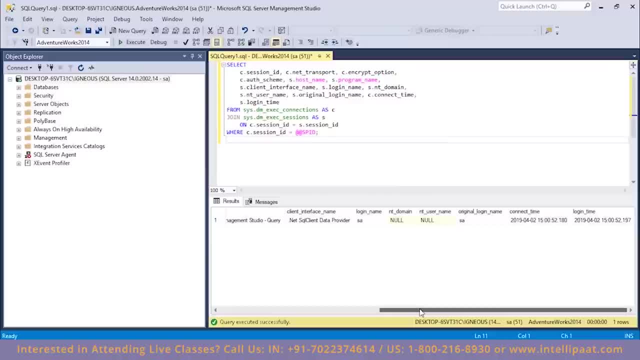 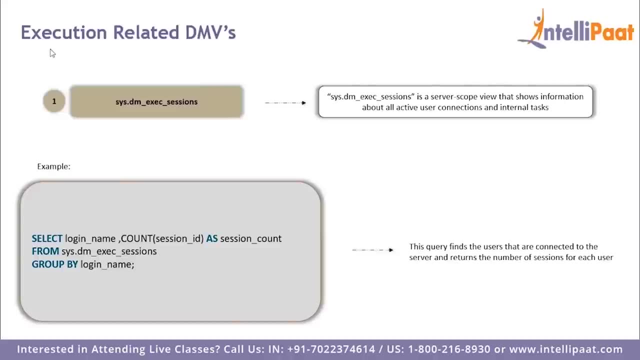 We have the program name over here, we have the login name and we have the original login name, the connection time and the login time. So next we have dm underscore, exec sessions, which shows information about all active user connections and internal tasks, and this command over here it finds the users that 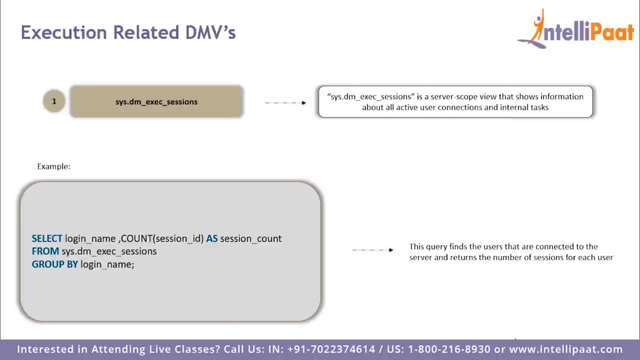 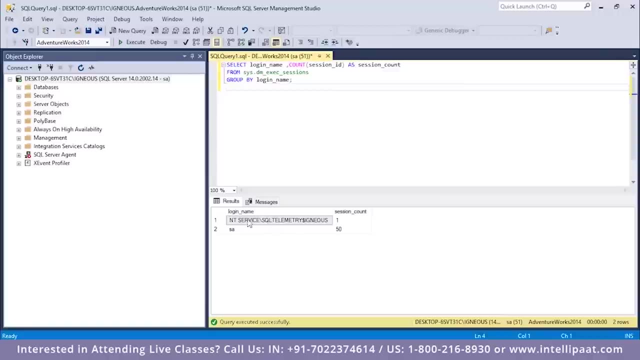 are connected to the server and returns the number of sessions for each such user. So we see that there are two users currently. One is NT SERVERS- IGNEOS. for the first user the session count is 1 and for the second user the session. 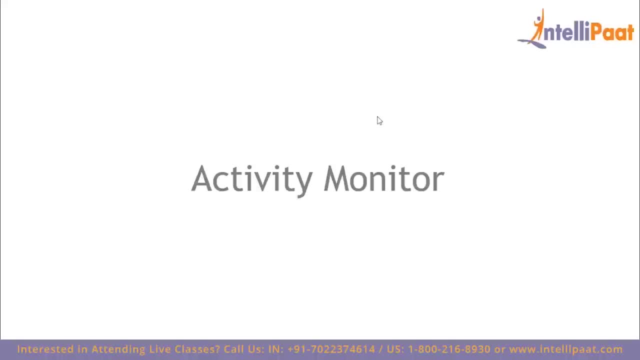 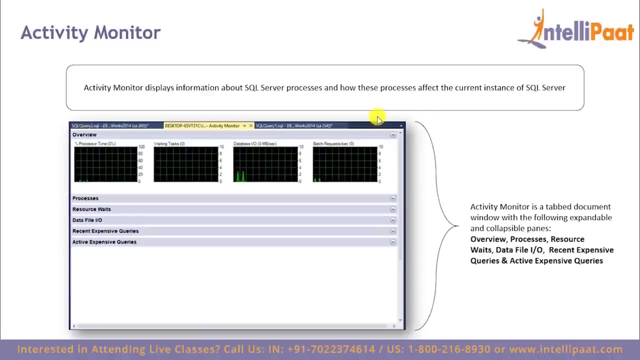 count is 50.. So those were some of the dynamic management views. Now we will work with Activity Monitor. So SQL Server Activity Monitor is a feature in SQL Server Management Studio that displays information about the SQL Server processes and their effect on SQL Server performance. So the Activity Monitor, 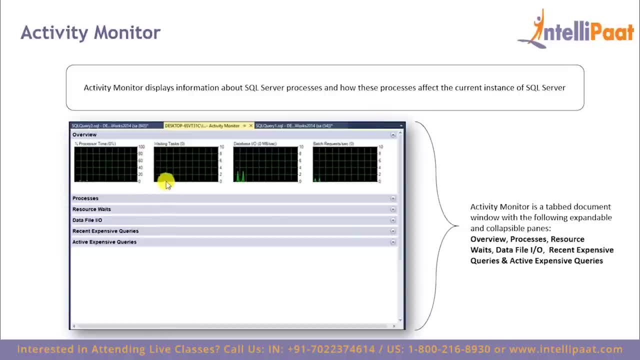 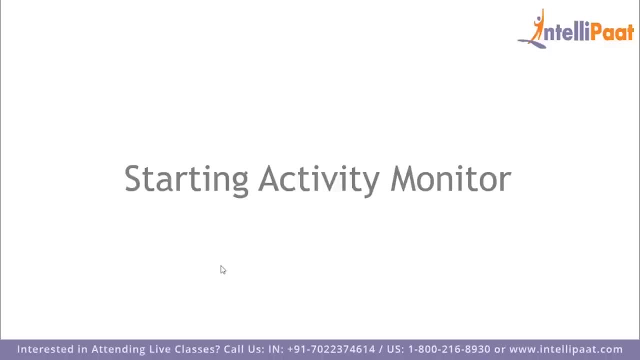 consists of these expandable panes. So we have overview, we have processes, resource weights, data file IO, recent expensive queries and active expensive queries. Now let's go ahead and start Activity Monitor in SSMS. So over here I would. 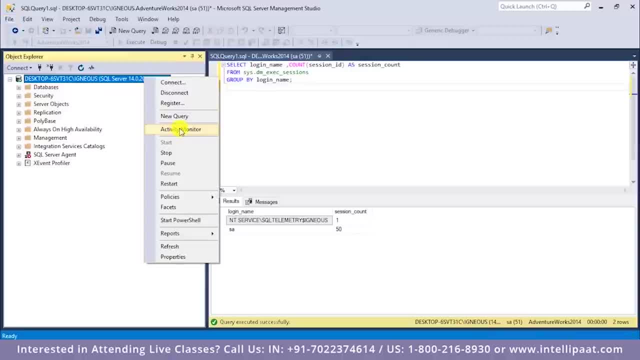 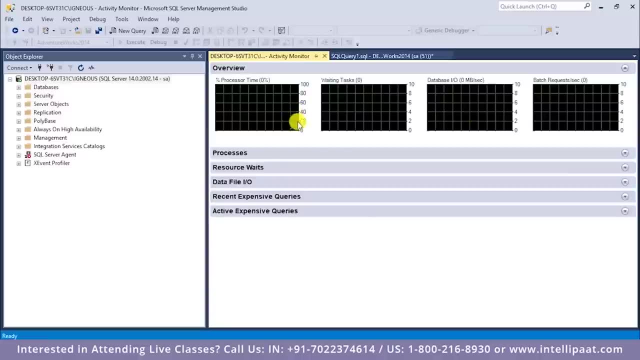 have to right click on this and then select Activity Monitor. So we have opened up Activity Monitor. So this overview pane over here it contains the graphs for the most important SQL Server instance information. So there's percent processor time. it tells us the percentage of. 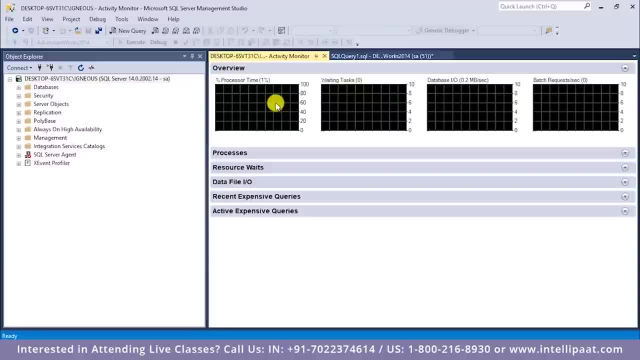 time the processors spend to execute threads that are not idle. and then we have waiting tasks. so this over here gives us the number of tasks that are waiting for processor IO or memory to be released so that tasks can be processed. then we have database IO, so this gives us the data transfer rate in megabyte. 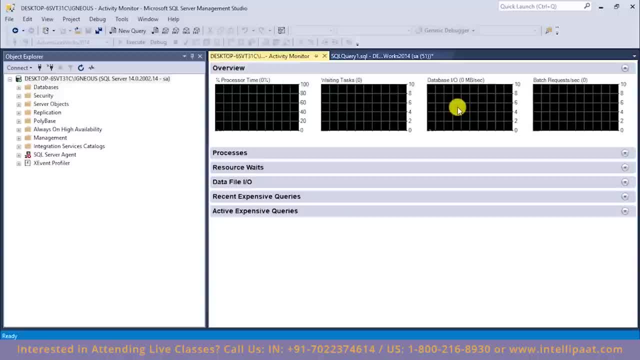 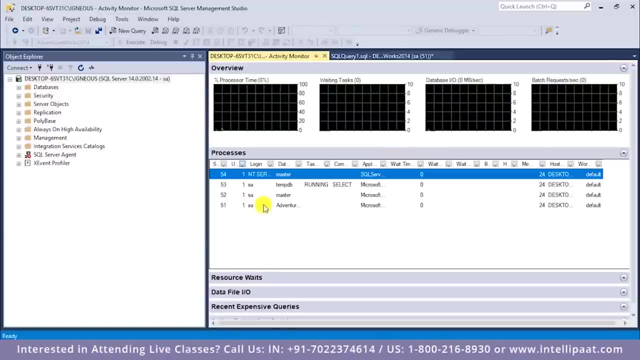 per second, and it could be either from memory to disk, disk to memory or disk to disk. and finally, we have batch requests per second, which gives us the number of sequel server batches received by the instance in a second. now let's look at the processes pane. so this process pane shows us the information about the 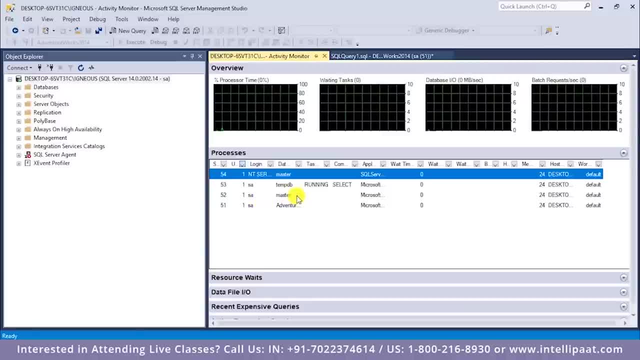 currently running processes on the sequel server databases and who are running those processes. so we have information for session ID, we have user process, we have login name and so on. right, so we see that these are the users over here and these are the databases which the users are currently working on. 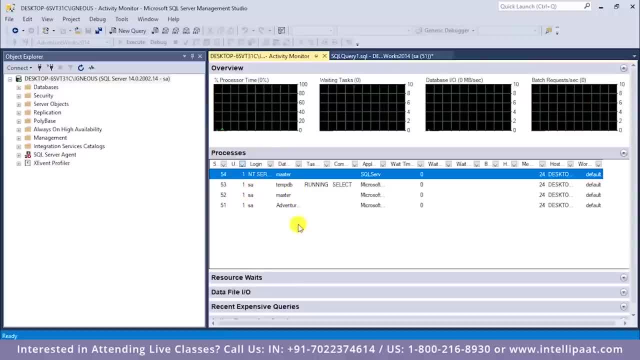 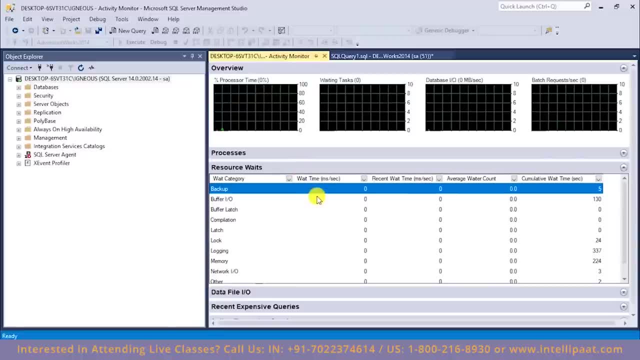 you see that the user essay has worked on temp DB, master DB and this adventure works DB. after that, we have the resource weights, pain, and this provides information with respect to a thread which is waiting for a key resource such as memory, CPU or network. so these are all of the threads which are waiting for something, and then we 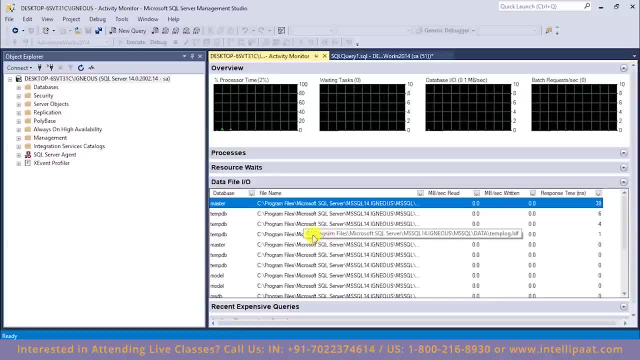 have the next pane, which is data file IO. so this pane shows information about the database files on the sequel server instance. so for each database all the files are listed. So we have all of the different databases over here- tempdb, master model and so on- and these are different files which are part of this database. 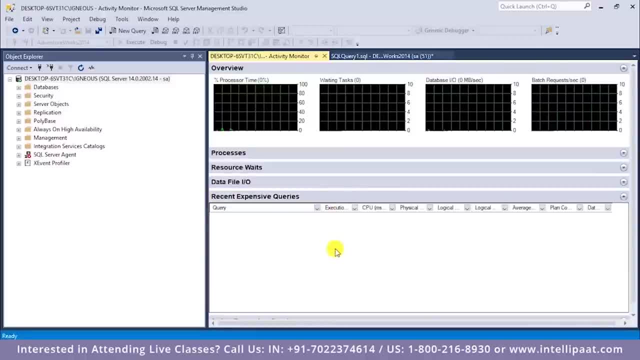 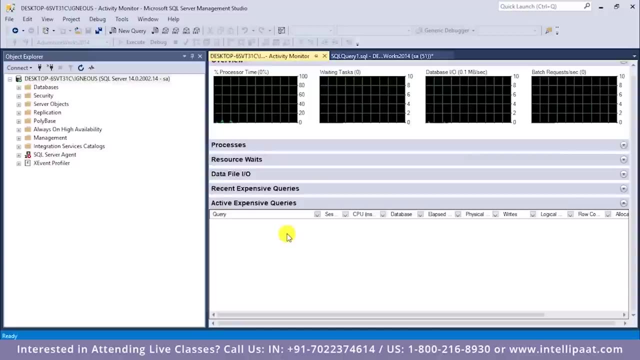 And then, following on, we have the recent expensive queries pane. So this pane shows all the expensive queries in the last 30 seconds which use up a lot of resources, whether it is memory disk or network. And finally we have the active expensive queries, which shows all the currently. 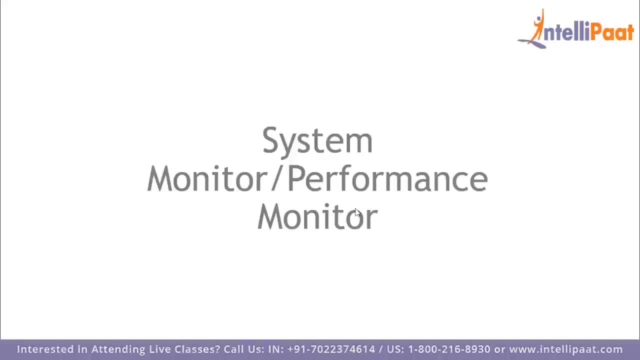 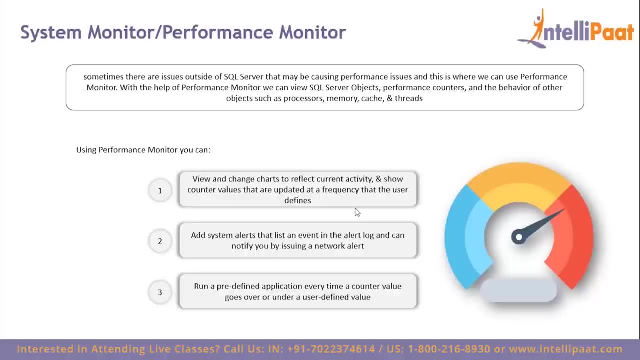 active, expensive queries running Now. we will work with the performance monitor Now. sometimes there might be issues which occur outside of SQL server that may cause performance problems in SQL server, So this is where we can use performance monitor. So performance monitor is a monitoring tool which is shipped with Windows and it helps in tracking various performance. 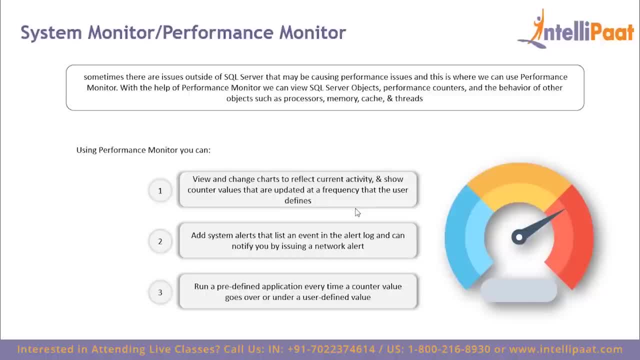 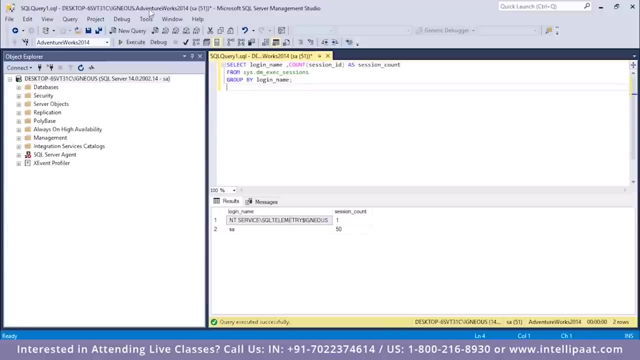 counters and monitors overall system and application performance, And these counter values are shown in real time graphs which can be saved in log files and be used for analysis. Now let's work with performance monitor in SSMS. So to open performance monitor, I'd have 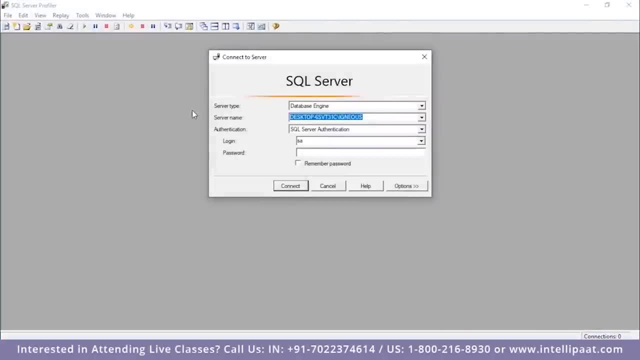 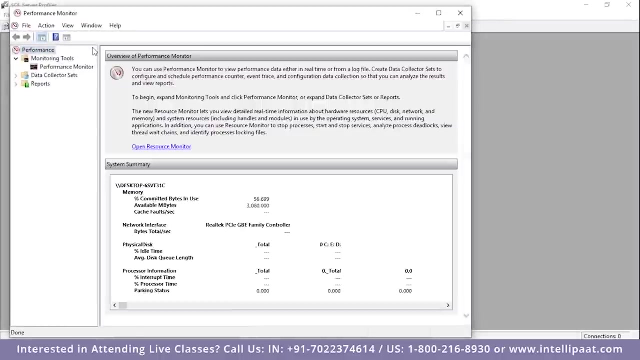 to click on tools and then select SQL server profiler. I will just give the connection name and the password over here. I will connect Now again inside the SQL server profiler. I have this tools tab, so I'll select this and then select performance monitor Over here. 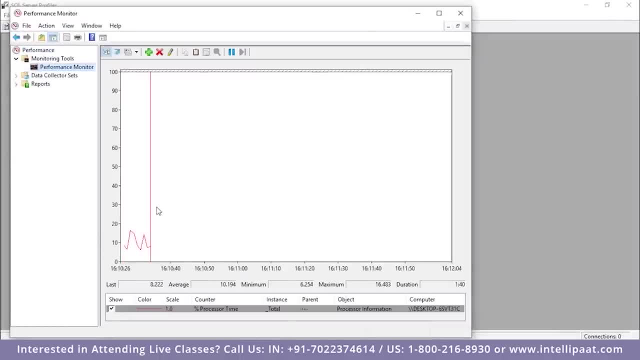 I will select performance monitor and we see that there is a graph which tells me about performance of the system. Now, if I want to add some counters, I would have to click on this plus symbol over here and I can add all of the performance counters. So let's say: 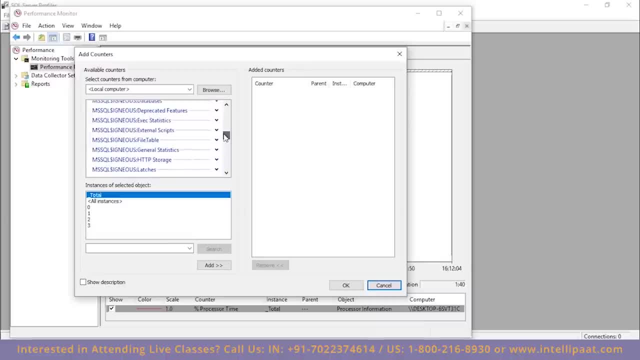 I want performance counters related to memory. So let me go to the memory section over here And inside memory. maybe I want to add available megabytes. I will add this. I will add committed bytes, free and zero page list bytes. So this is memory Again in logical disk. maybe I want. 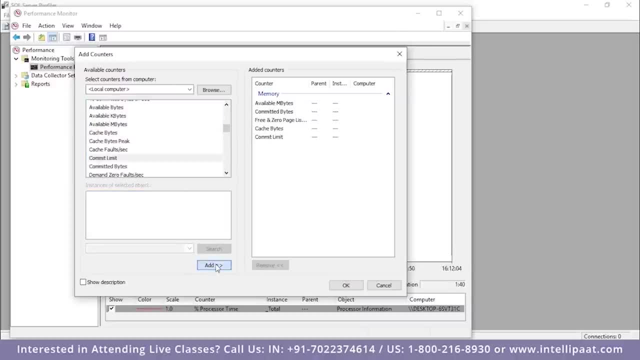 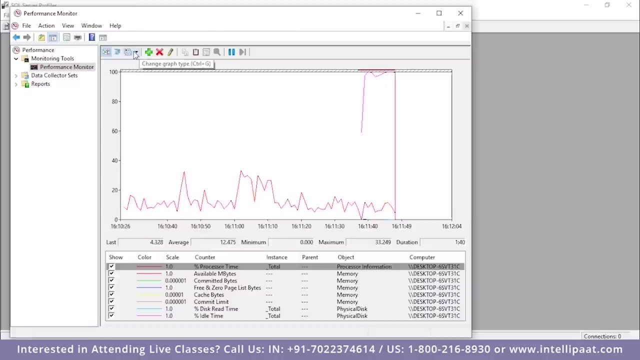 the cache bytes. I would also want the commit limit Now similarly under physical disk. I would want the disk read time and the idle time over here. Now all I have to do is click on OK Now if I want to get a report of this. we see this change graph type and I will click. 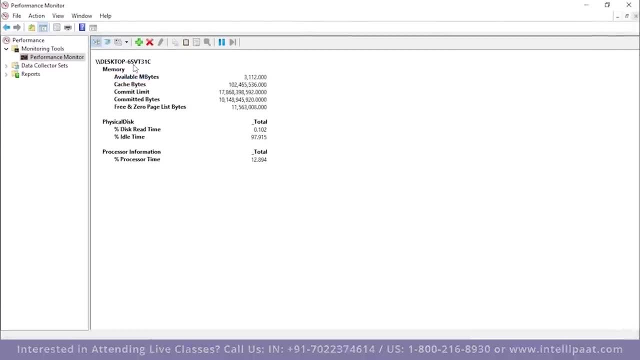 on report. So this is the report which I have. So we see that available megabytes- This is the available megabytes, cache bytes, committed limit, committed bytes and the free and zero page list bytes over here And we have the percent disk read time under physical disk. 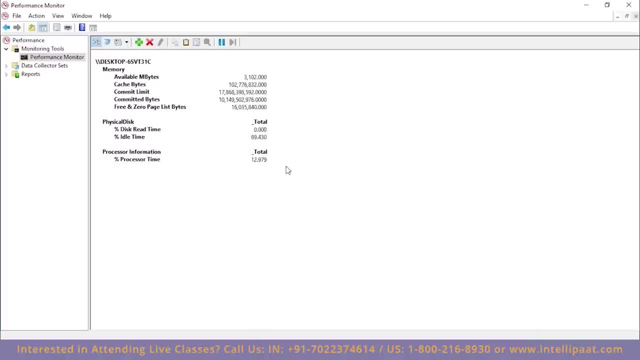 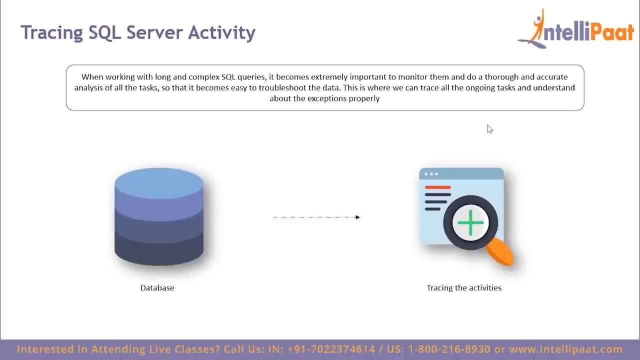 percent idle time under physical disk and we also have the processor time over here. Now let's see how can we trace SQL server profiler. So whenever we are working with really long and complex SQL queries, we have to make sure that all of those tasks are performed accurately. This is where tracing all these tasks becomes. 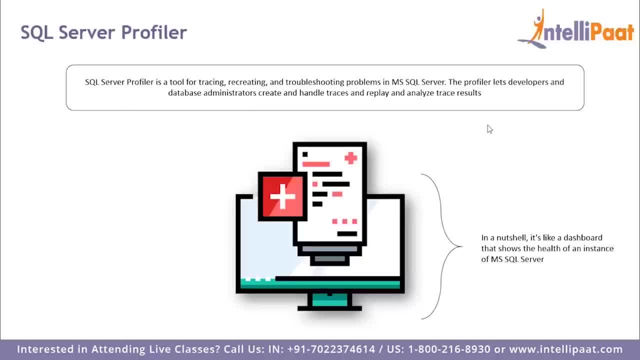 important. So SQL server provides a tool called as SQL server profiler for exactly this purpose. So profiler is a tool for tracing, recreating and troubleshooting problems in MS SQL server And it lets developers and database administrators trace all of these tasks And it lets developers 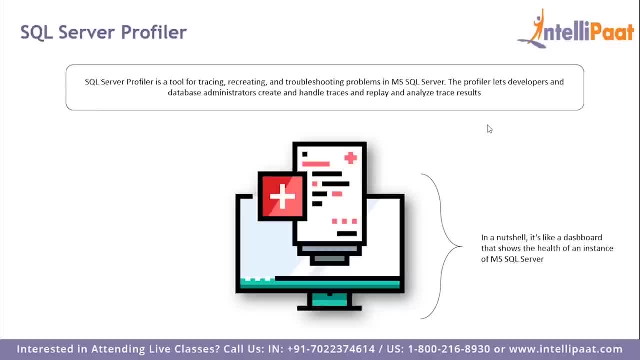 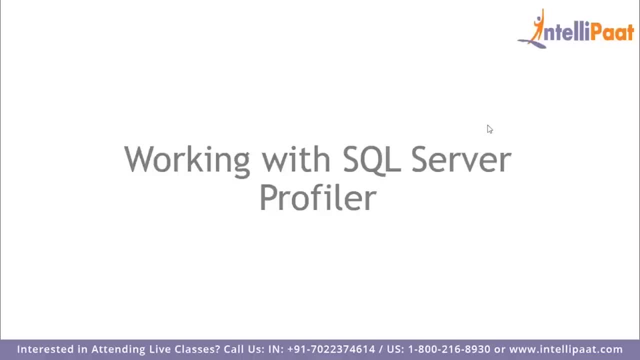 and database administrators trace all of these tasks And it lets developers and database administrators to create and handle traces and replay and analyze these trace results. Now let's go ahead and work with SQL server profiler in SSMS. So we are back to SSMS. 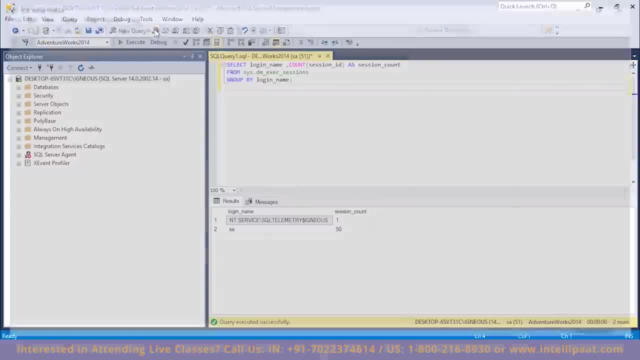 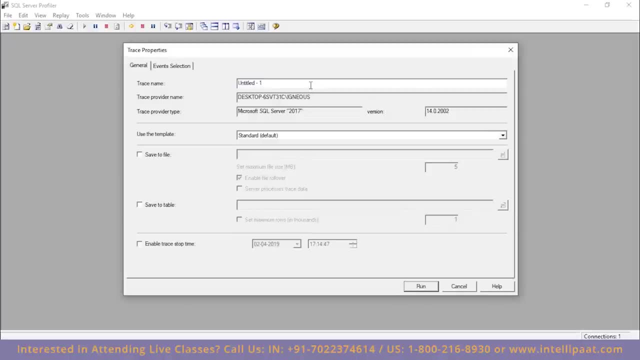 Now I'd have to click on tools and then select SQL server profiler. Again, I will give in the password and then establish the connection. Let me click on connect. Now I'd have to give a new name to this trace. So I will name this as new trace And then maybe I will also name 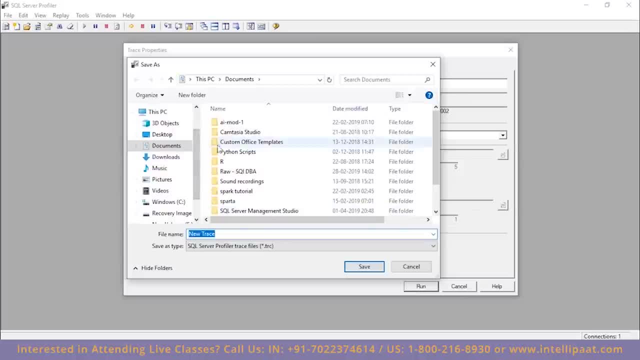 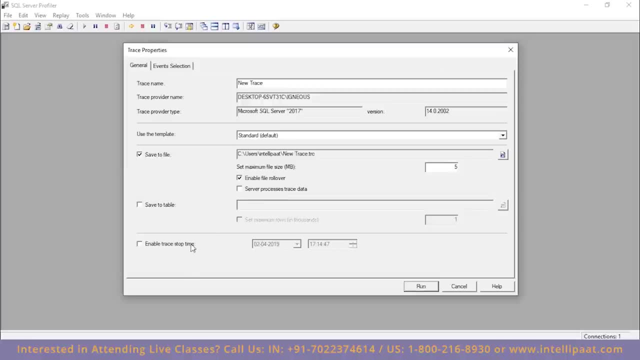 this as new trace And then maybe I will also save this to a file. So let me give in the destination So I'll save this in my C drive. I'll click on save over here. Now I can also set the trace time. So let me schedule it So. I want this SQL server profiler to run. 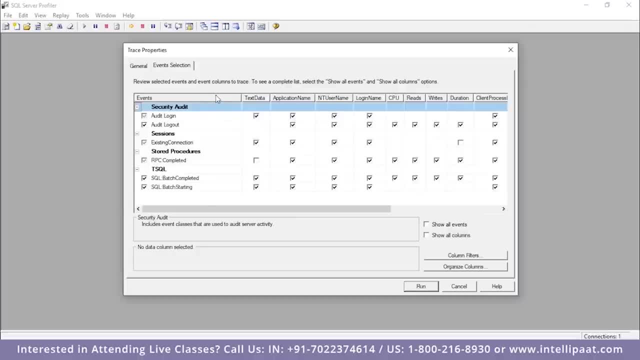 for at least one hour And again over here, event selection. So this is where I can set all of those events which I want to be traced. So I'll click on this show all events And let me add some events over here. So let's go ahead and click on show all events And. 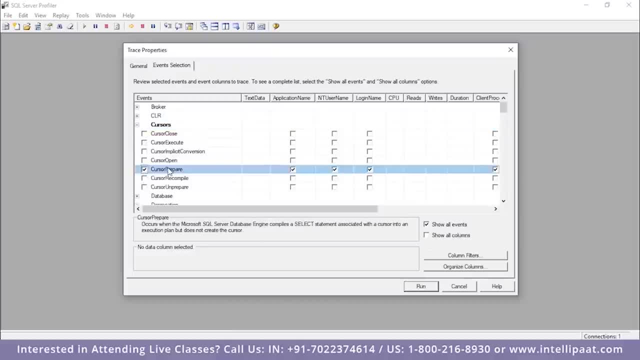 let me add some events over here. So let's say I want to do events over here, So I want, so I want to trace the cursor prepare cursor, unprepared option. and let me go to the objects tab over here and I want to know whenever an object is altered. 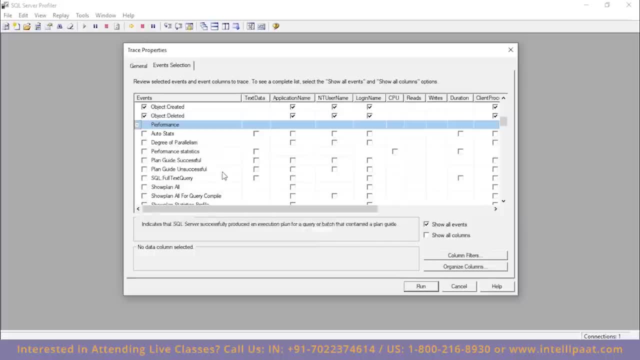 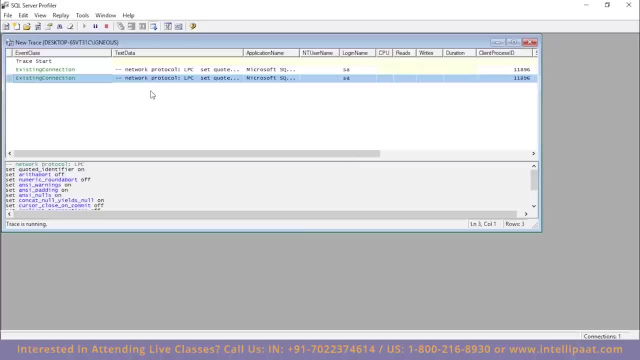 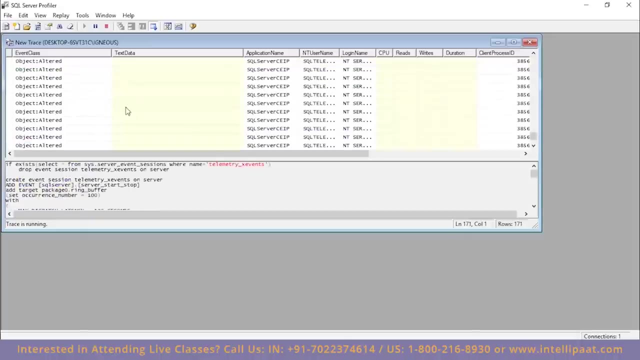 created or deleted. similarly, if we go to this performance tab and I want to know about all the stats, and now all I have to do is click on run so we see that the trace has started and we get all of the information over here, so we have the detailed information of whatever is happening, so you have the 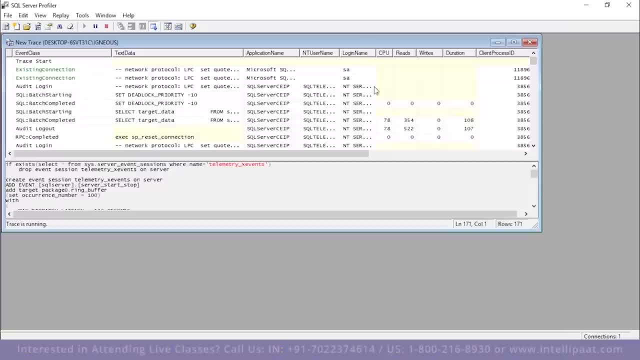 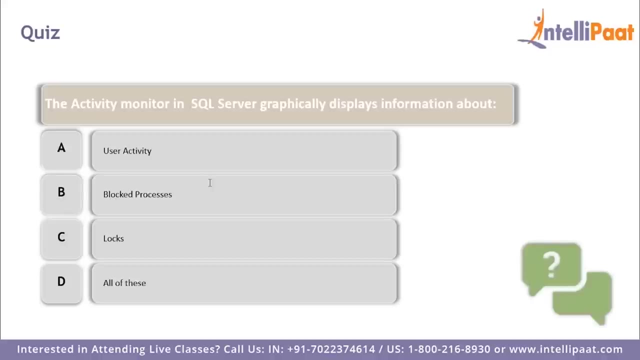 event, class text data, application name and the username, login name and so on, and we also have the reads rights and the duration for the reads and rights over here. so this is how we can work with secret server profiler. so now let's head on to the pop quiz. so you have this first question, the activity monitor, and 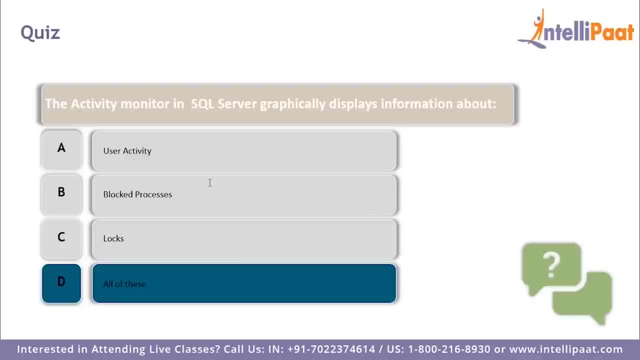 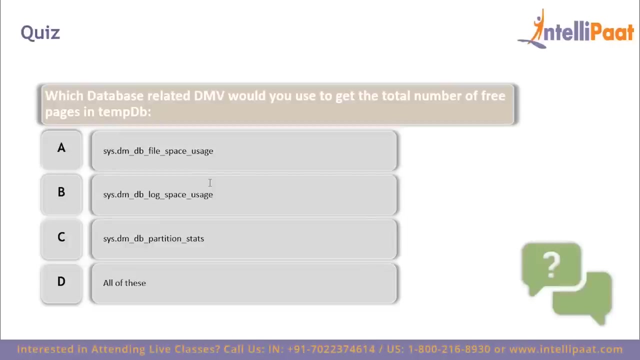 sequel server graphically displays information about what well it displays information about. of these, It gives us information about user activity, block processes and also locks. So the next question is: which database related DMV would you use to get the total number of free pages in tempdb? So what do you think is the 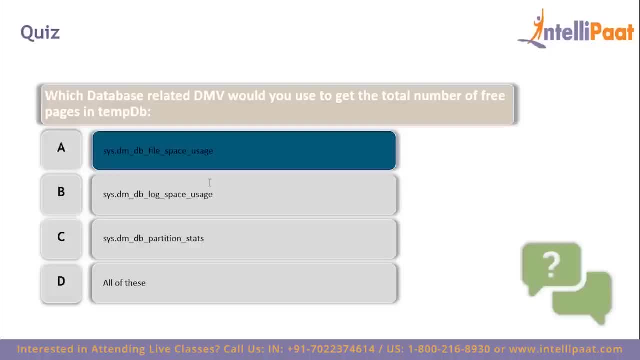 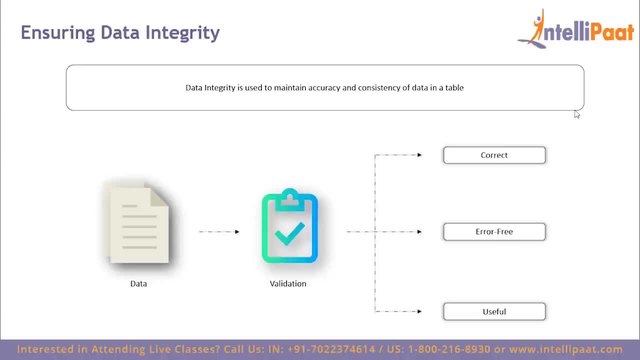 answer. The answer to this is db underscore- file space usage. So this is the DMV which we'll use to get the total number of free pages in tempdb. So why do we need data integrity? Well, data integrity is used to maintain accuracy and consistency of data in a table. So whatever data we have with us, 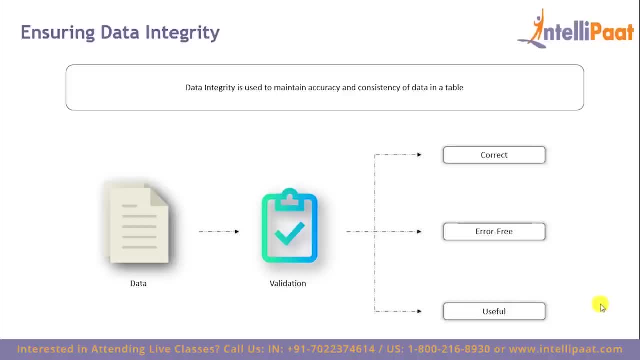 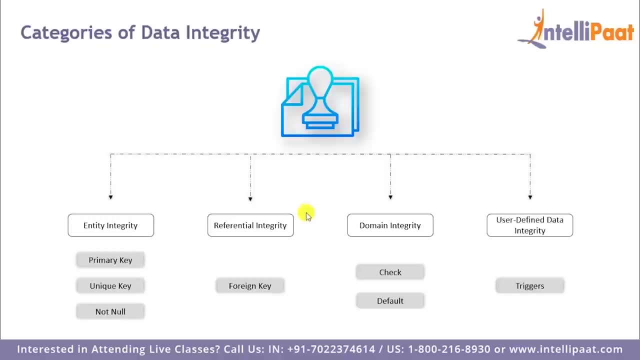 we need to make sure that it is correct, error-free and useful, And data integrity can be grouped into these categories. So we have entity integrity, referential integrity, domain integrity and user-defined data integrity. So entity integrity ensures that each row in a table is a uniquely identifiable entity. 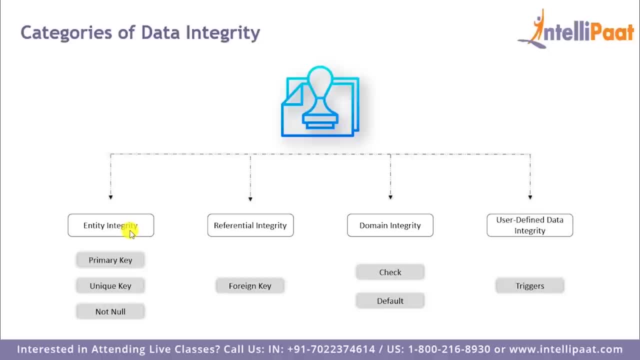 and we can apply any entity integrity to the table by specifying a primary key, unique key and not null. Then we have referential integrity, which ensures the relationship between two tables is proper, and we can apply this using a foreign key constraint. And then we have domain integrity, which ensures the data. 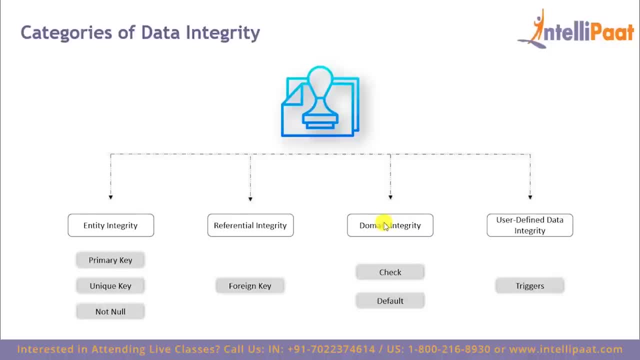 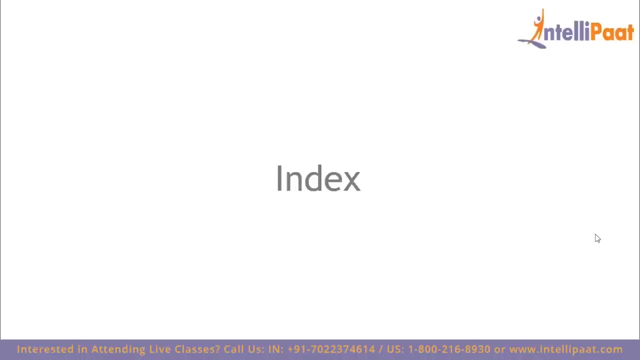 values in a database follow defined rules for values, range and format, and we can enforce these rules using check and default constraints. And finally, we have user-defined data integrity, which can be enforced through triggers. So now that we know about data integrity, let's learn about indexes in SQL Server. So indexes? 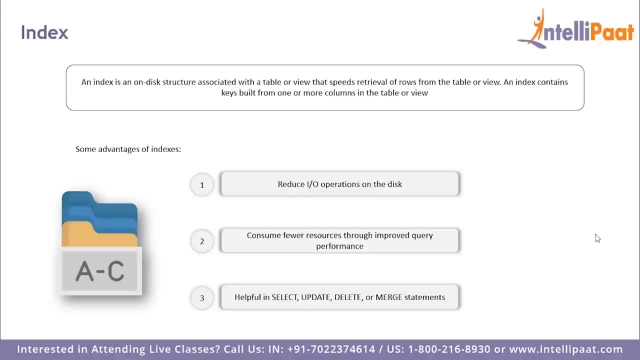 are special lookup tables that the database search engine can use to speed up data retrieval. Simply put, an index is a pointer to data in a table, So these indexes in a database are very similar to indexes at the end of the books, whose purpose is to find a topic quickly. 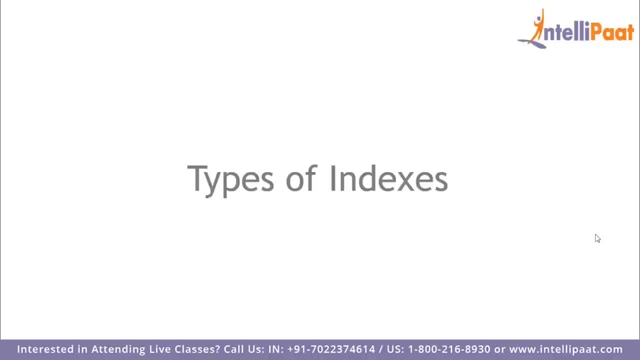 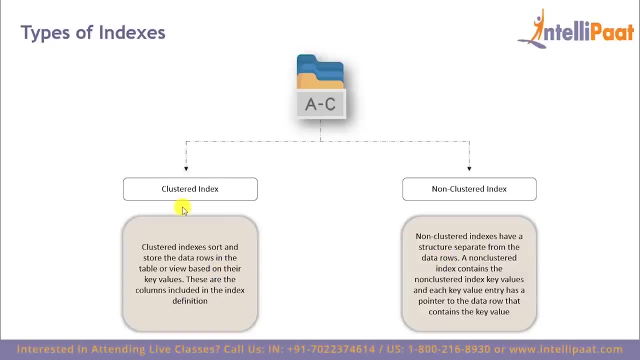 Now again that we know what exactly is an index, let's look at the types of indexes. So in SQL Server, indexes can be grouped into clustered and non-clustered. So a clustered index defines the order in which data is physically stored in a table and since table data can be sorted in only one way, therefore there can be 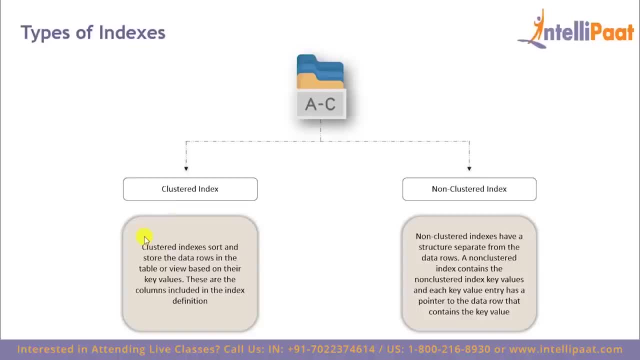 only one clustered index per table. So when SQL Server, the primary key constraint automatically creates a clustered index on that particular column, But when it comes to non-clustered index, it doesn't sort the physical data inside the table. In fact, a non-clustered index is stored at one. 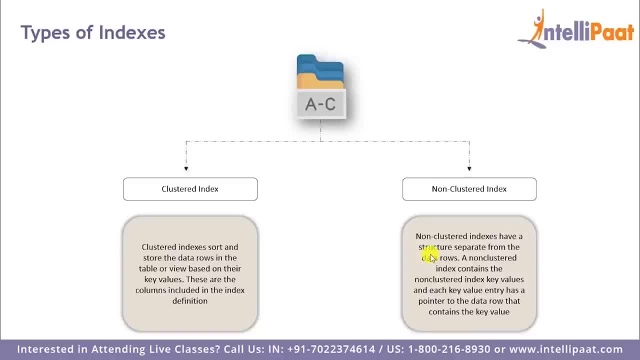 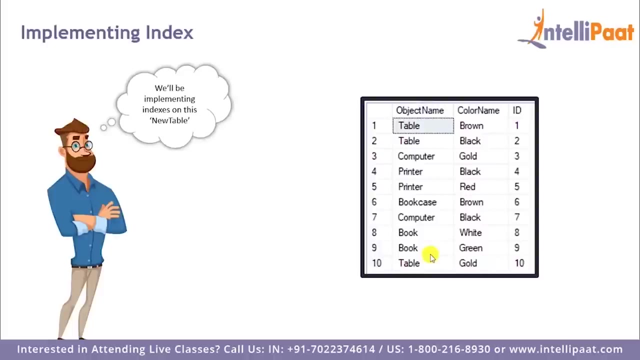 place and table data stored in another place, And this is actually similar to a textbook, where the book content is located in one place and the index is located in another, And this allows for more than one non-clustered index per table, And we'll be implementing indexes on this new table, which comprises of: 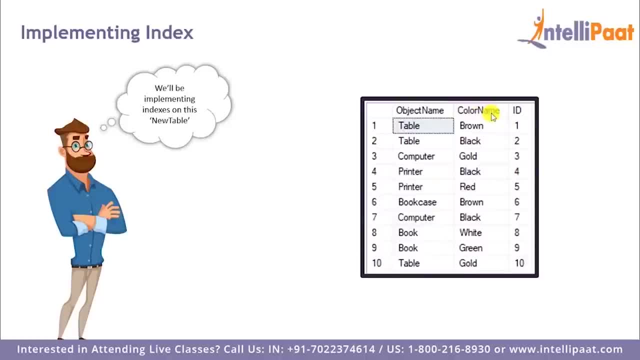 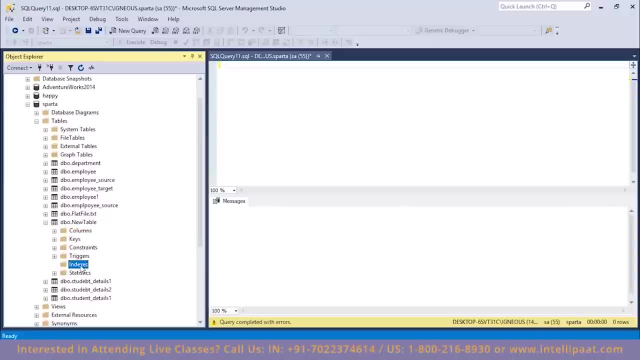 these columns: object name, color name and ID. right, so we have this new table over here. now, if I have to create an index on top of this, we have this index folder inside this table. so I would have to right click on this, select on new index and if I want to create a clustered index, I will select this option: clustered. 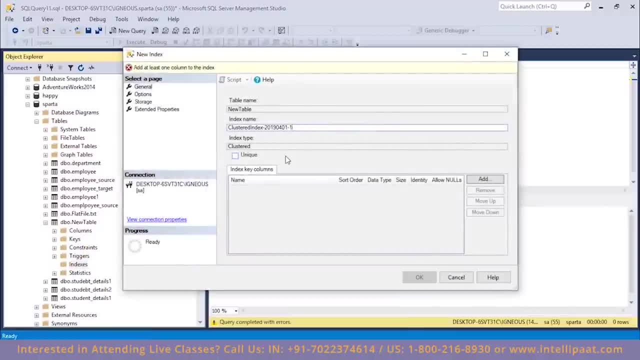 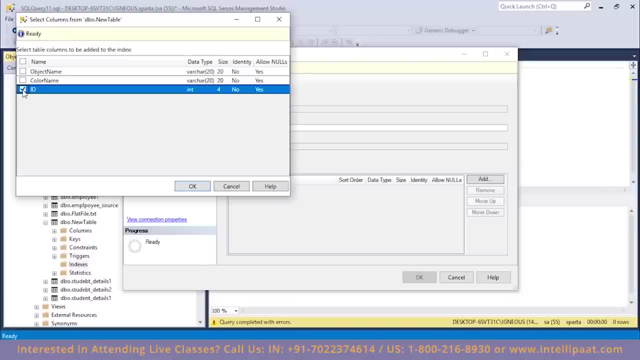 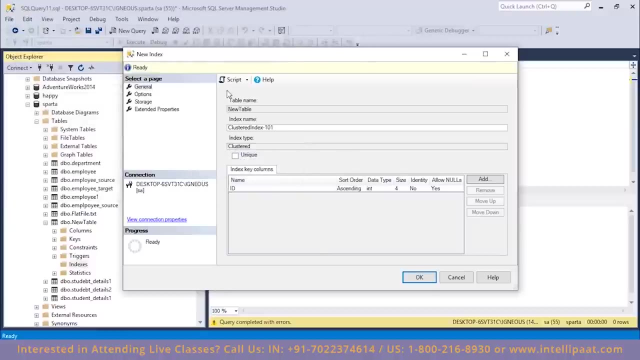 index and then give a name to this clustered index. so I will name this as clustered index 101 and I will go ahead and add this clustered index on top of the ID column of this table. I'll click on OK now again if I want the TSQL code. 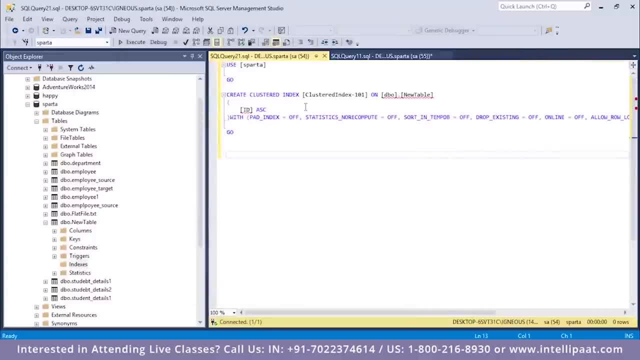 for it. all I have to do is click on script. so this is the TSQL code to create a clustered index with the name clustered index 101, and it is built on top of the ID column. so now, again, I will go to this dialog box and click on OK. 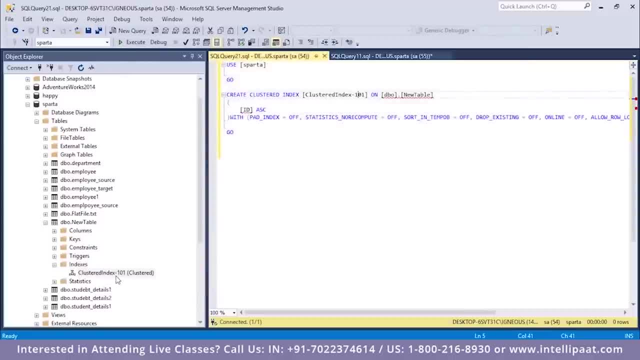 okay, so see that we have successfully created a clustered index with the name clustered index 101, which is on top of the ID column. now, similarly, if I want to create a non clustered index, I will right click on this folder, select new index and this time I will choose non clustered index and again I will give a name to this. so 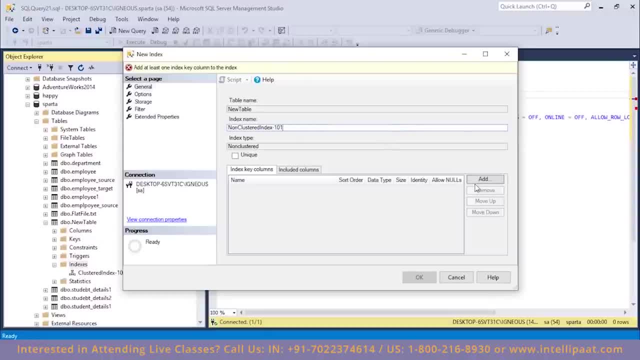 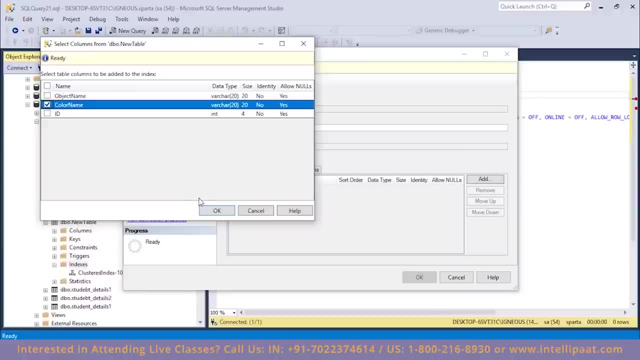 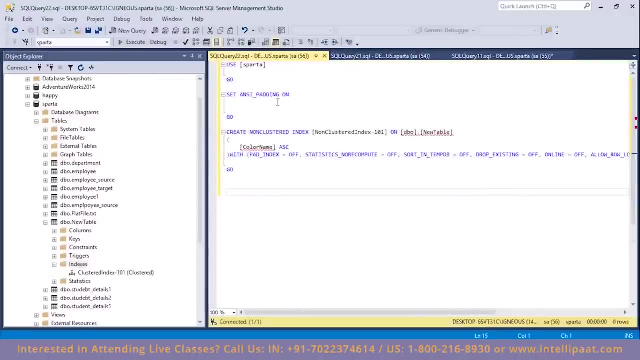 this will be non clustered index 101. I will go ahead and add a column on top of which this non clustered index is supposed to be. so I will choose the color name column. I'll click on OK again. if I need the code for this, I'll click on script. so this is the code to create a non clustered index. 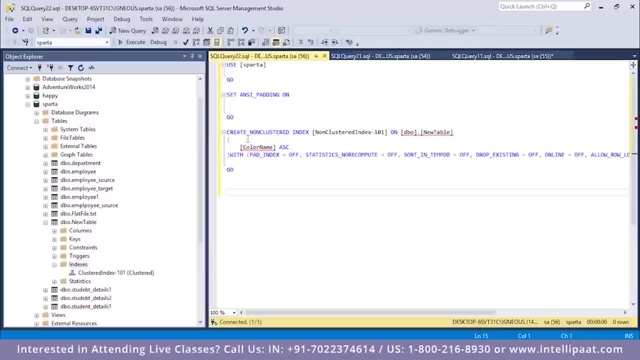 with the name non clustered index 101. and this is on top of the color name column. so again, I will finally click on OK. and we have also successfully created a non clustered index with the name non clustered index 101. now let's talk about one of the 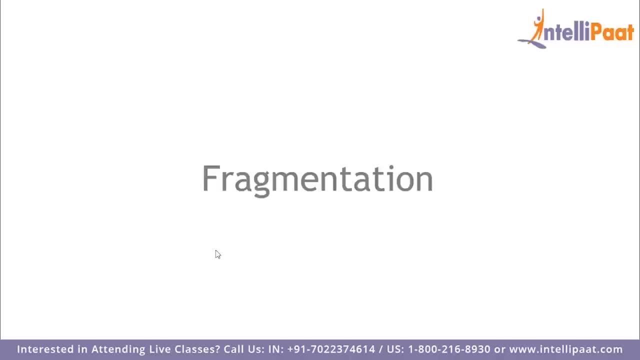 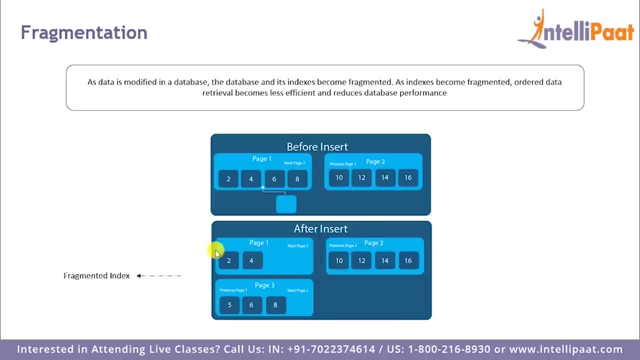 problem which is associated with indexing and that is known as fragmentation. so index fragmentation happens when the indexes are scattered all over the database. well, whenever SQL server performs IO operation, it initially reads the data from the disk, which is known as physical read. so it pulls everything into the SQL server buffer. so there is a load of. 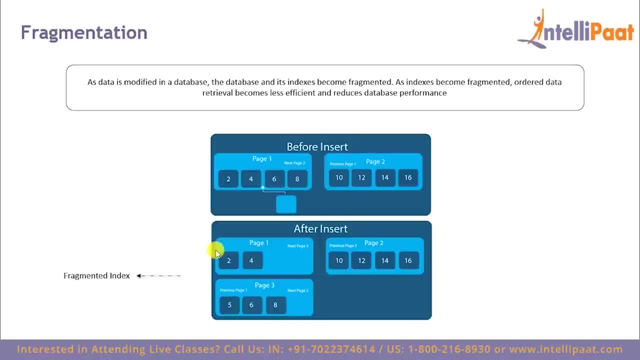 logical order in this buffer and Whenever the query runs again, instead of doing physical read, SQL server would look into the buffer and if it can't find the requisite data in the buffer, That is when it will do physical read from the disk. Now there might be a case where the logical order of the indexes is not. 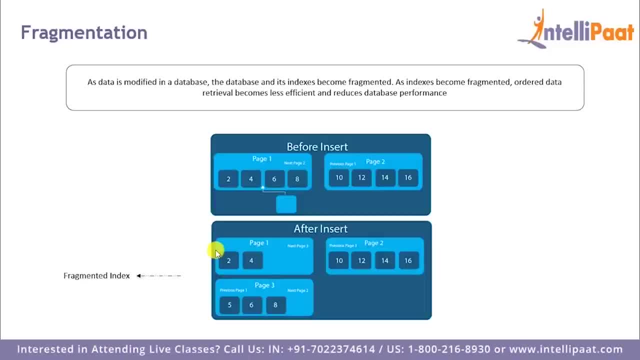 Equal to the physical order of the indexes, and this is called as index fragmentation. Now, why does it happen? Well, whenever we insert or update data, the indexes become fragmented and as indexes become fragmented, Ordered data retrieval becomes less efficient and reduces database performance. So let's actually take this example. 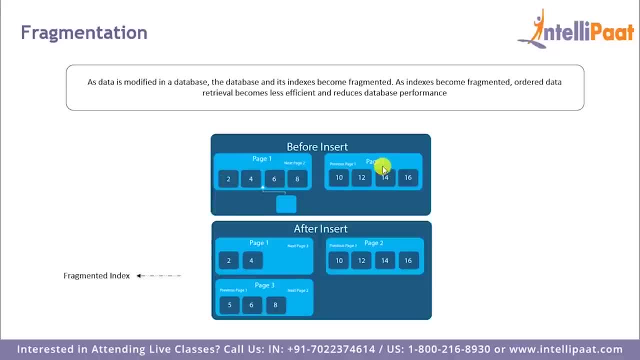 So initially we have two data pages for a table with a clustered index. Now a new row with the primary key file needs to be inserted and since it is a clustered index, New row is inserted. in order, And because the target page is full over here, The new row does not fit and SQL server splits the page roughly into two halves and 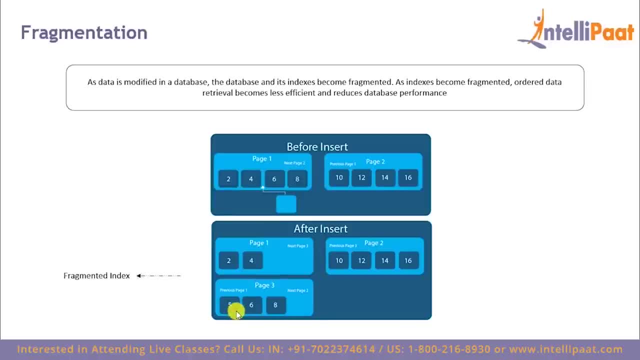 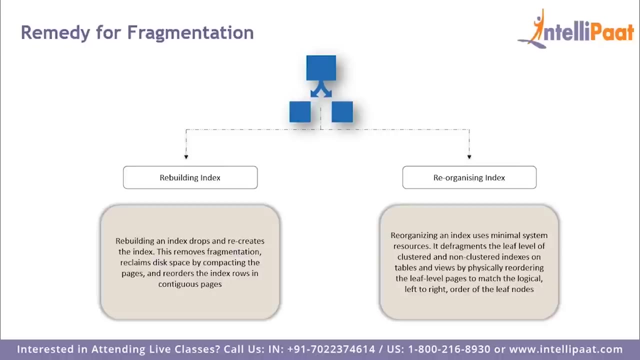 Insert the data into this new page. Now what happens is the logical order of the index does not match with the physical order, and this is when we say that the Index has become fragmented. now, to deal with fragmentation, We have two solutions. We can either rebuild the index or reorganize the index. 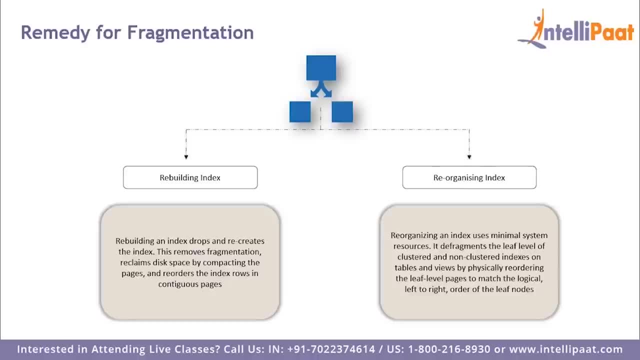 So rebuilding is the process of changing the whole b-tree There is all the existing indexes are dropped and new indexes are recreated, while reorganizing index is the process of cleaning, Organizing and defragmenting the leaf level of the b-tree. Now we'll go ahead and implement this concepts in SSMS. 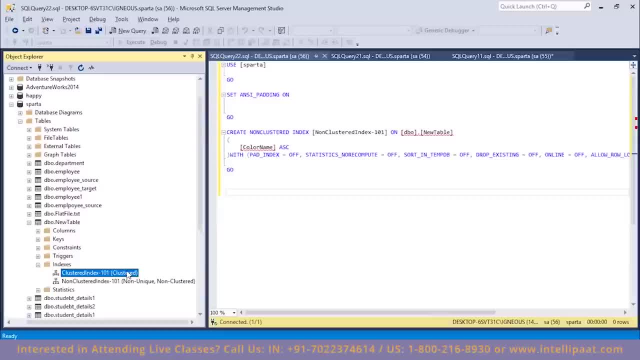 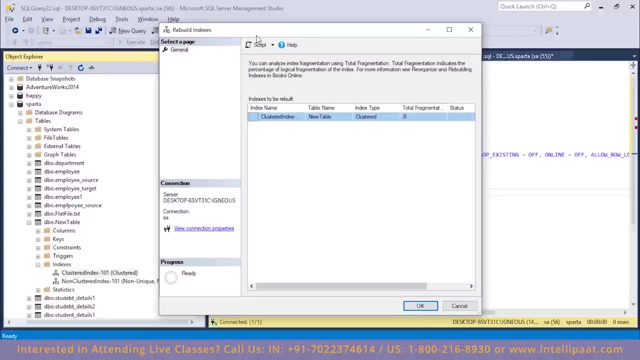 So I will take these clustered index and I want to rebuild this clustered index. So if I want to do that, I will right-click on it And I have this option to rebuild. I'll click on this now I. all I have to do is click on OK and again, if I need the TSQL code for this, 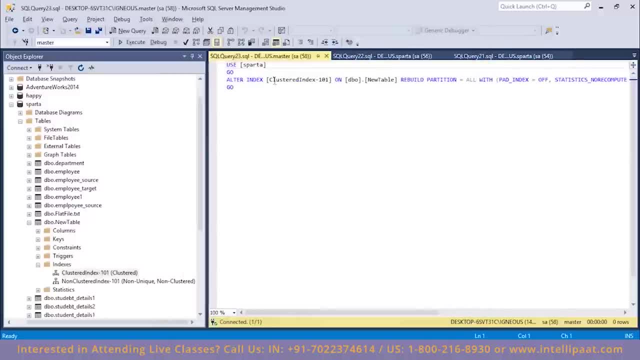 All I have to do is click on script- and this is the TSQL code- to rebuild this clustered index 101. So I will go ahead. click on OK and I have successfully rebuilt this clustered index. now I want to Reorganize this non clustered index, So this time I will right-click on it. 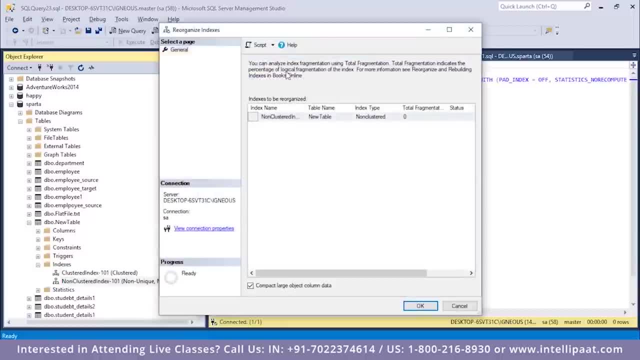 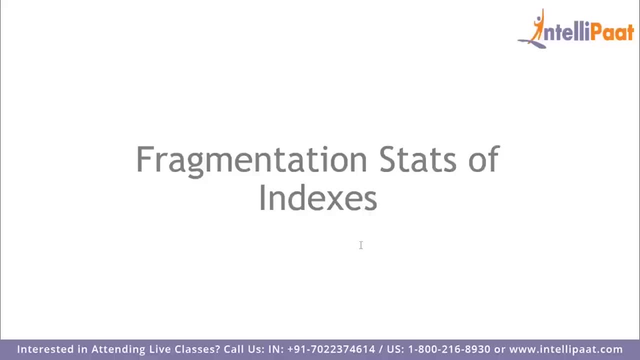 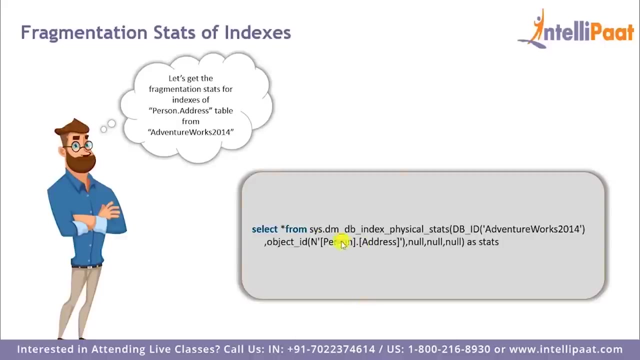 I will right-click on this, select reorganize, and again select this and click on OK. So this time I have successfully reorganized this non clustered index. now Let's see How can we get the fragmentation stats of indexes So we can use this dynamic management function. 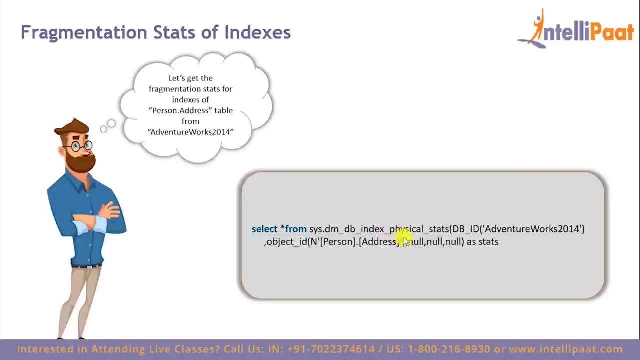 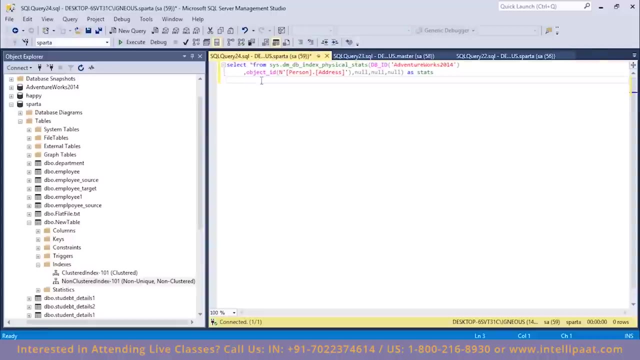 sysdm underscore DB, underscore index, underscore physical stats to get the fragmentation stats, and We'll be applying this on top of this person dot address table From the AdventureWorks 2014 database, So I'll just piece the code over here and I want these index stats for this table over here. 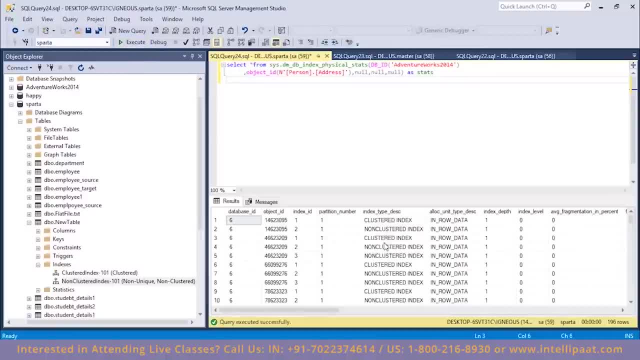 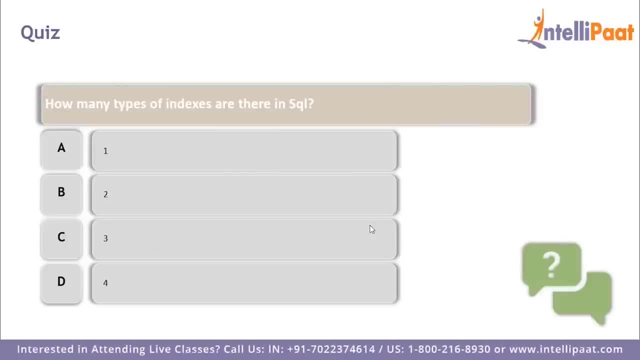 Person dot address. I'll click on execute and these are the fragmentation stats for this table. now We'll head on to the pop quiz. So we have this question over here: How many types of indexes are there in SQL? So, guys, what do you think? 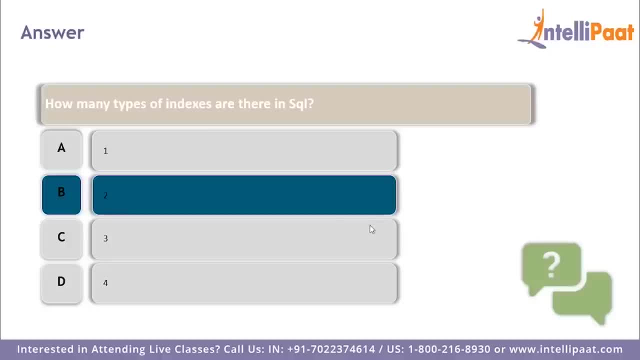 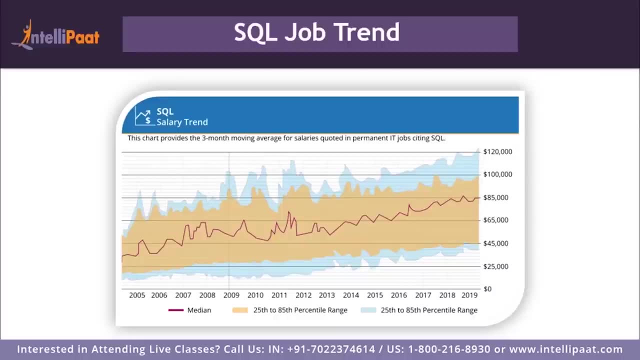 Well, the answer is two. we have clustered index and the non clustered index. Now let's start off by having a glance at the salary trends of sequel. So this graph tells us that the salary of sequel developers has been steadily increasing year by year, and as of 2019. 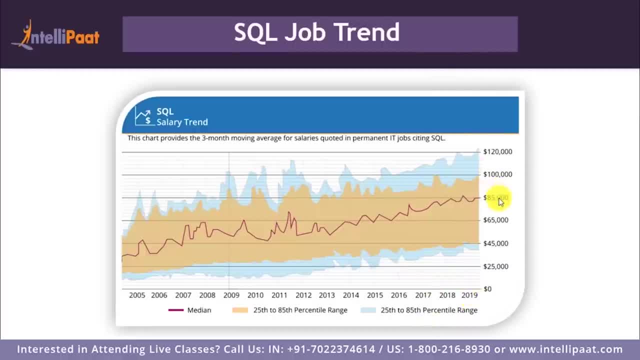 The median salary of a sequel developer stands at around $85,000, so there is a very high demand for professionals with knowledge in sequel. now that we've looked at the demand of sequel, Let's start the first question. So what exactly is sequel? So this is a very basic question. 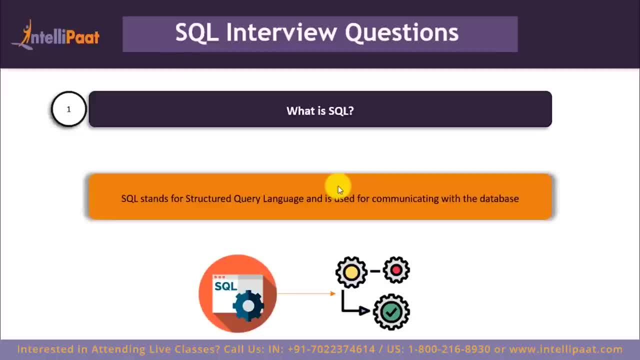 so, to answer this, SQL stands for the structured query language and according to ANSI, It is a standard query language for relational database management systems, which is used for maintaining the relational database and also to perform different he shun's of Data Manipulation on different types of data. 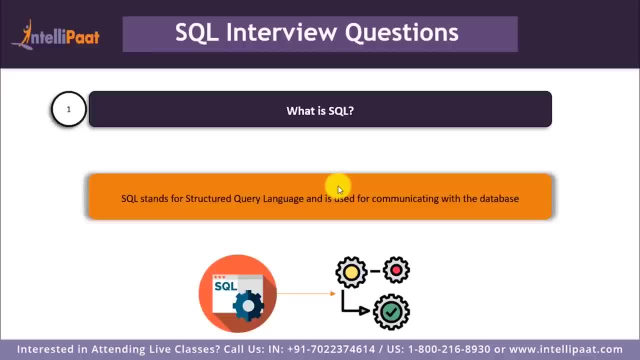 so sequel is widely used language for maintaining relational database and in AE 86 SQL became the standard of American National Standards Institute or ANSI. So basically it is a database language which is used for creation and deletion of databases and it can be used to fetch and modify rows from the table. 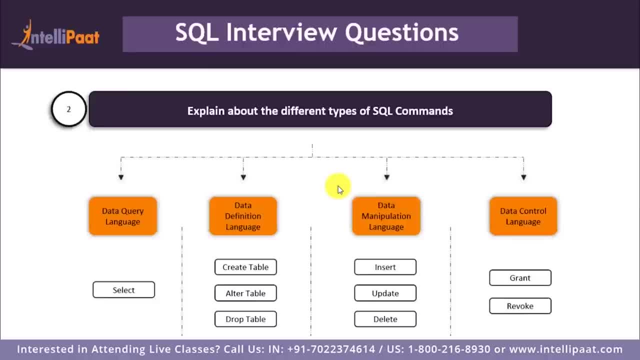 and also multiple other things. So let's head on to the next question. So we are supposed to explain the different types of SQL commands. So the SQL commands can be divided into four categories. So we've got data query language, data definition language, data manipulation language and data control language. So the data query 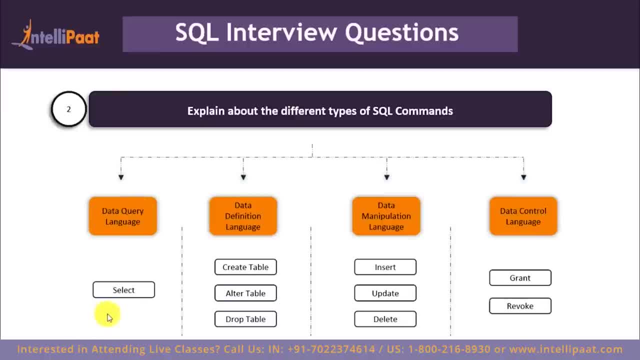 language comprises of just one command, SELECT, though it can be accompanied with many clauses to compose queries on a database. Then we have the data definition language. So DDL is that part of SQL which defines the data structure of the database in the initial stage when the database is about to be created. 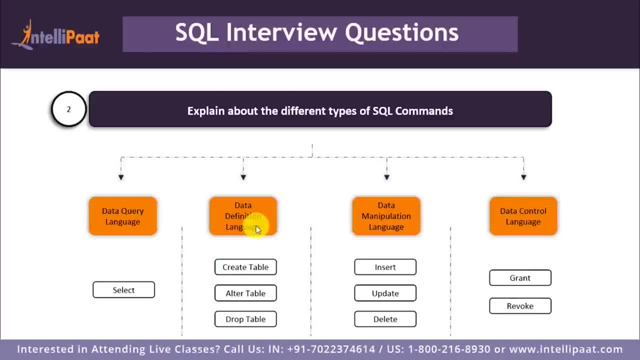 So it is mainly used to create and restructure the database objects. So you can see commands like create table, alt table and drop table in DDL and after that we have the database response. So this command is used to create- and data manipulation language. So DML is used to manipulate the already existing data in the 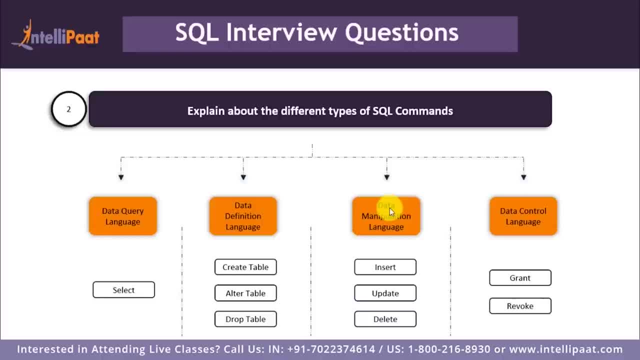 database, That is, it helps the user to retrieve and manipulate the data, And it is used to perform operations like inserting data into the database through the insert command, updating data in the database through the update command and deleting data from the database through the delete command. 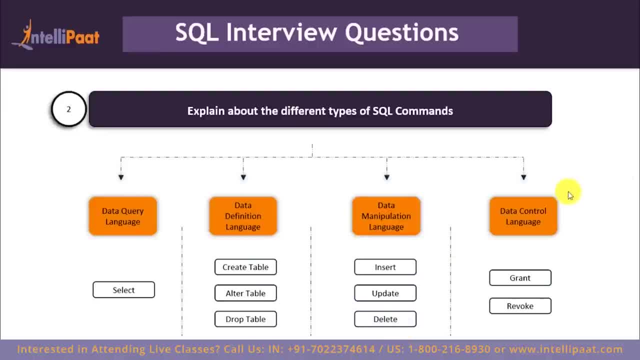 And finally, we have the data control language, which is used to control access to the data in the database. So these DCL commands are normally used to create objects related to user access and also to control the distribution of privileges among users, And you see commands such as grant. 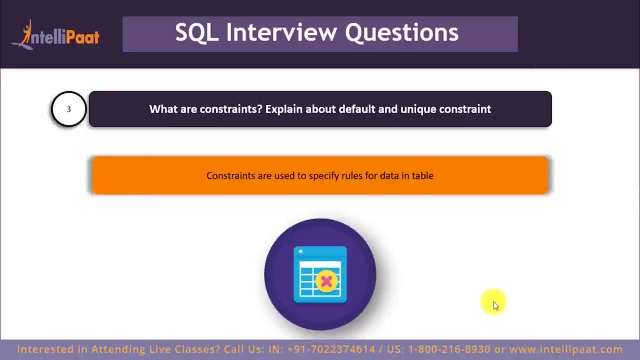 and revoke in DCL, Right? so this is the next question. So what exactly are constraints? And we are supposed to explain about the default and the unique constraint. So constraints are basically used to specify some sort of rules on the data and limit the type of data that can go into a 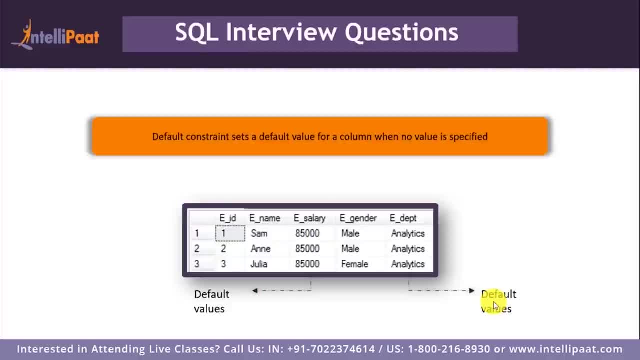 table. Alright. so let's understand about default constraint. So the default constraint is used to provide a default value for a column. So the default value will be added to all the new records if no other value is specified. For example, if we assign the default constraint to this eSalary column and set the default, 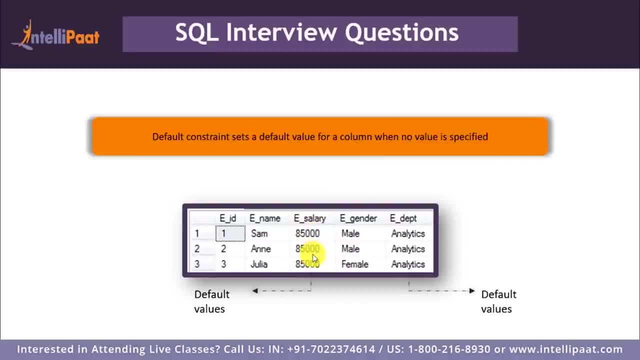 value to be equal to 85,000, then all the entries of this column will have a default value of 85,000 if no other value is assigned during the insertion. So similarly, we can also assign a default value of analytics to this EDEPT column, right. 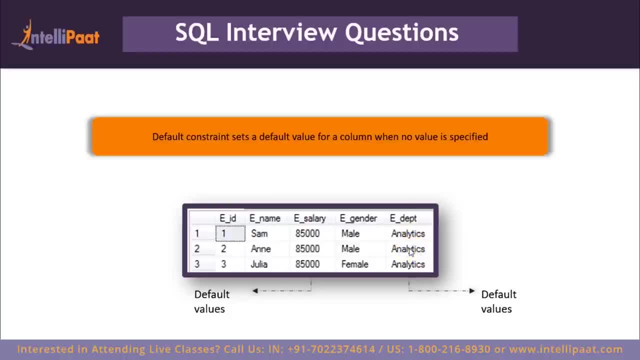 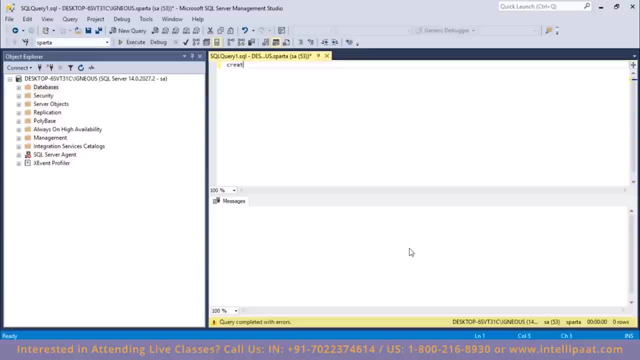 So now we'll go to SQL Server and we'll work with the default constraint. Now I'll start off by creating a new table and I'll add the default constraint to one of those columns. So I'll create a new table and I'll name this table as stu1.. 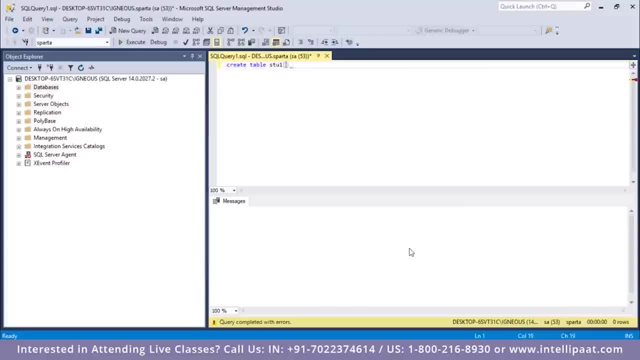 So the syntax would be: create table stu1, and this would comprise of these columns That would be sid, which basically stands for the student ID, and the data type of this column would be integer. After this, there is sname, which stands for student name, and the data type would be varchar. 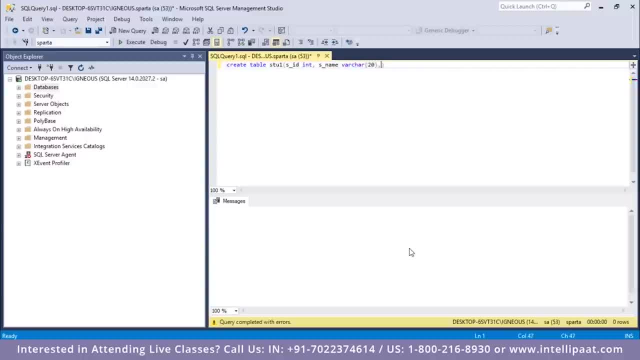 and the length of the string, or the maximum length of the string would be 20.. And then I'll finally have the marks code by the student, which would be smarks, and this would be of integer type. Now, after this, I will give in the default constraint and I will set the default value. 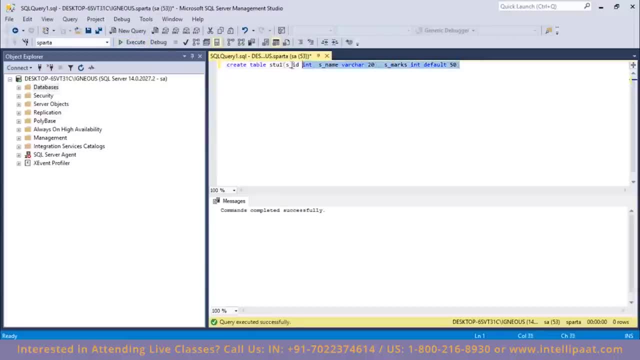 to be equal to 50, right? So I have successfully created this table. Now let me have a glance at this table first. So select star from stu1.. So this is our table, which is empty as of now. Now what I'll do is I will go ahead and insert some values into the table. 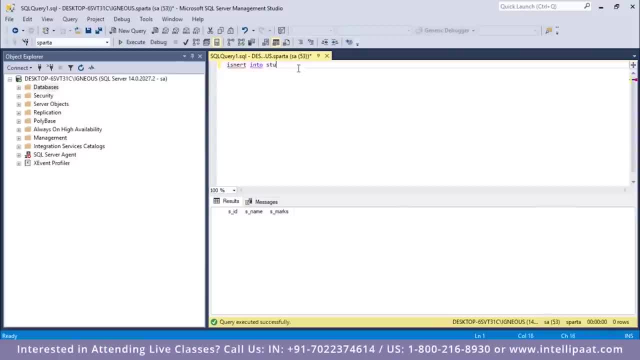 So I'll type in insert into stu1 and then I'll give in the name of the columns. so this needs to be insert. So the name of the first column is sid, and then I've got sname. Now I'll type in values and give in the values for these two columns. 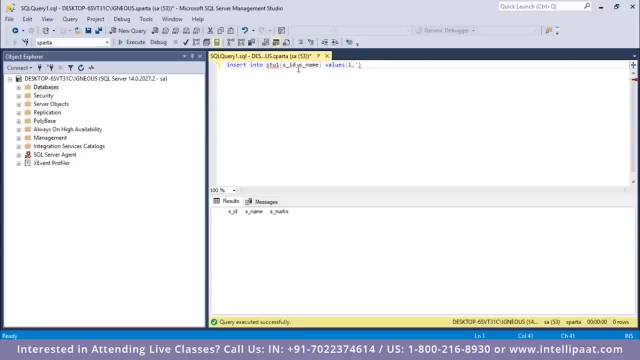 So let's say the first ID is 1 and the name of the student is sam. Now I'll click on execute. Now let me have a glance at this modified table now Select star from stu1.. So now we see that we have this default value of 50 in this s marks column, and this is because 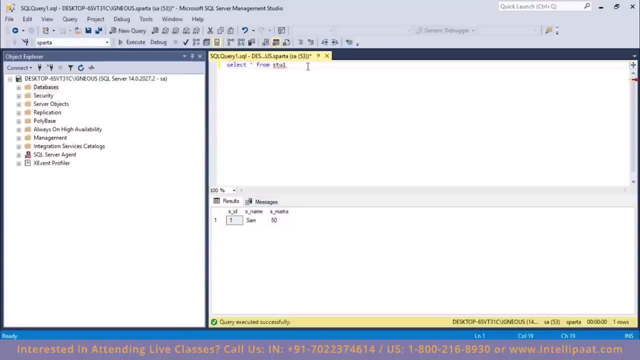 we had assigned the default constraint to this column. Now, similarly, let me add two more records into this table. So insert into stu1, sid sname- I'll give in values, so it'd be 2- and the name of the. second student is sam. So now we see that we have this default value of 50 in this s marks column and this is because we've assigned the default constraint to this column. So now we have this default constraint to this column and this is because we've assigned 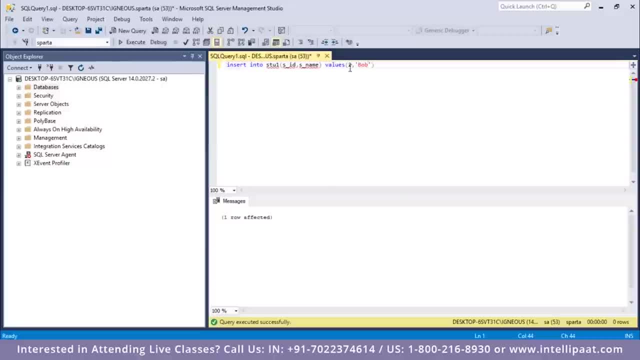 the default constraint to this column. So I've also added the second record. Now let me add in the third record. So the student ID is 3 and the name of the student is matt Right. so now I have three records in this table. 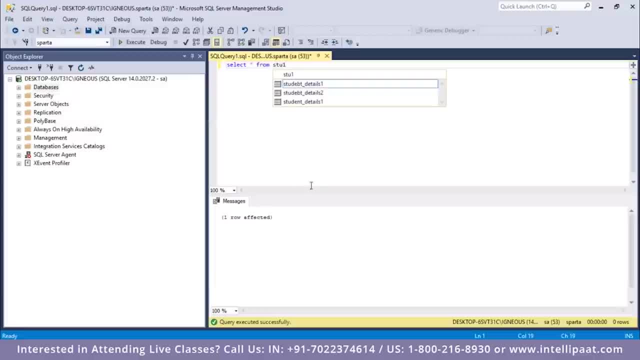 Select star from stu1.. So these are the two new records, and the default value is 50 for these two new records. So this is how we can work with the default constraint. Now comes the user guide. So here's how we can create a user guide. 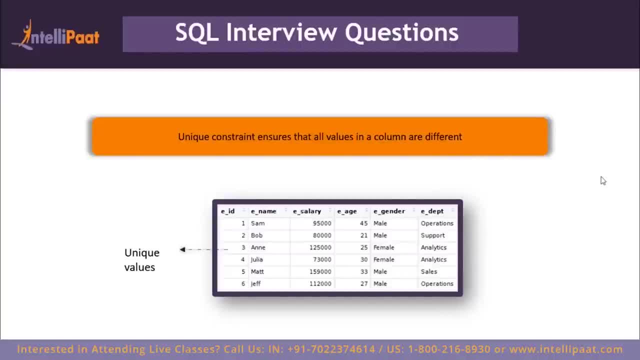 constraint. so the unique constraint ensures that all the values in a column are different. for example, if we assign the unique constraint to this ename column, then every entry in this column should have a unique value. so here we see that all the names of the employees are different. now again, let's go to 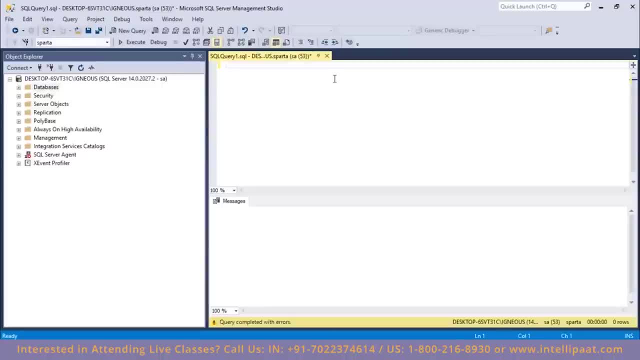 sequel server and work with a unique constraint. so again, I'll create a new table and add the unique constraint to one of the columns- create table- and this time the name of the table would be stu2. again there would be the ID and this is of integer type. now I would be assigning: 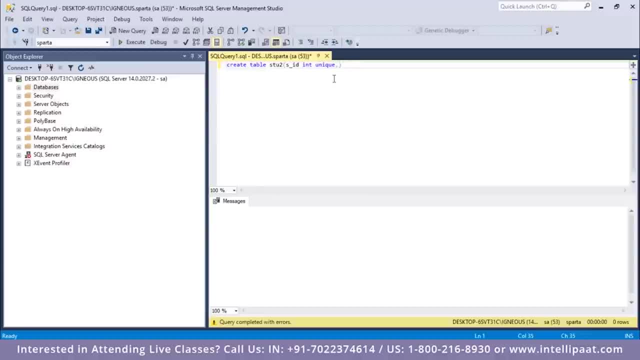 the unique constraint to this s ID column. and there would be a second column which is basically the student name, and this is of wirecard type. again, the length of the string would be 20. right now, let me have a glance at this table again. so select star from stu2. so this is our new table, which is: 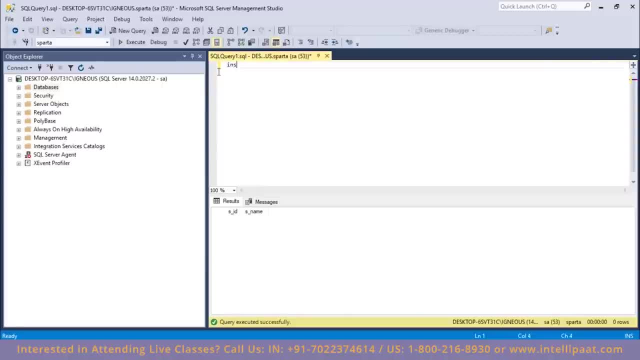 empty as of now. now let me go ahead and add values into this. so insert into stu2 values. I'll add in the first record. so 1, which would be the student ID name of the student, is Julia. now let me look at this table. select star from stu2. 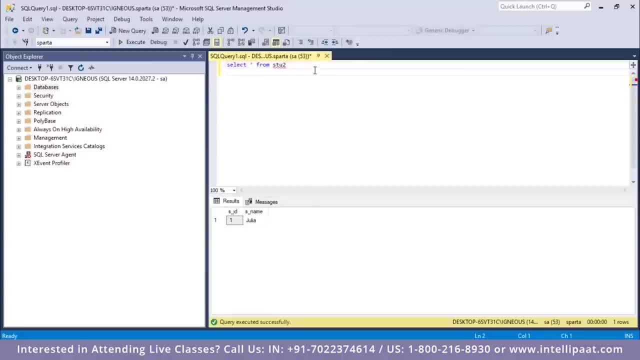 right. so we have successfully inserted this record. now let me add a new record. so insert into stu2 values. now what I'll do is I will again give the ID of the student to be 1 and the name of the student to be Matt, and let's see. 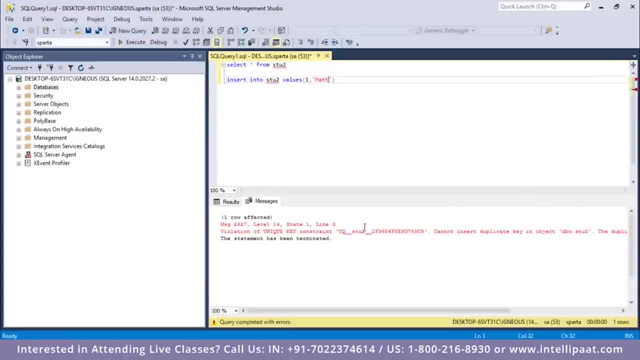 what happens. so this time we get a message, or a warning message, and the states that violation of unique key constraint and we cannot insert duplicate key in object DBO dot stu2 and that is because we had given the unique constraint to this s ID column. that is why this has to be. 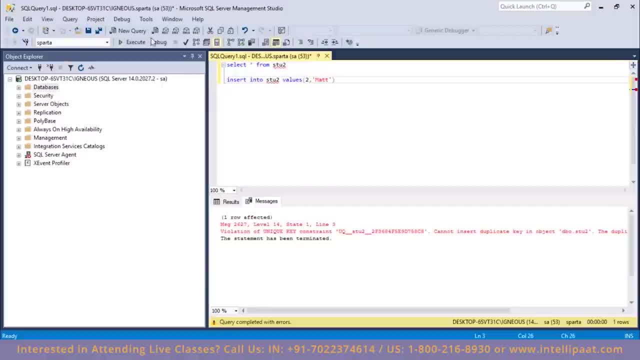 different. so let me change this to be 2 now. let me again run this right. so now, since this is a unique value, 2 is not a duplicate. that is why we were able to insert this record now. again, what I'll do is let me add another record with the 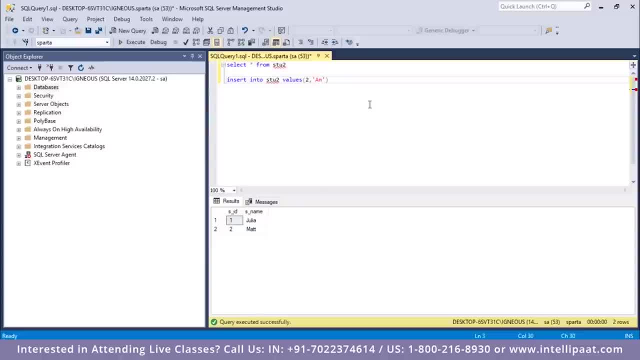 ID 2. so let's say, now the name of the student has Annie. now again we get this warning message because ID number 2 is already present. so let me change this to 3. now let me run this again. right, so now we are able to insert this record. so this unique constraint basically make 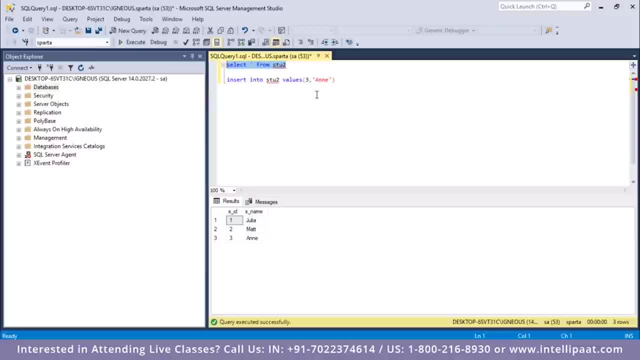 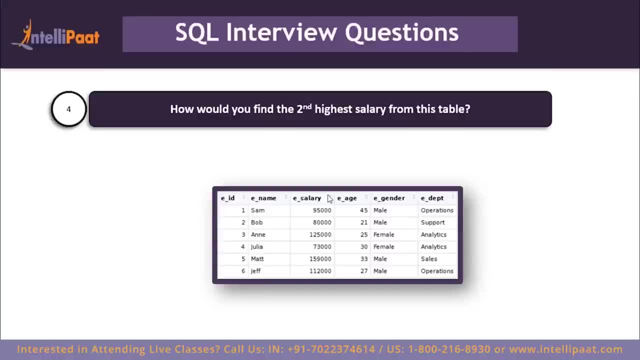 sure that there are no duplicate records inserted into this column. so now we have the next question. so again, we have this employee table with us and we are supposed to find out the second highest salary from this table. so let's go to sequel server and find out the solution. so let me start off by 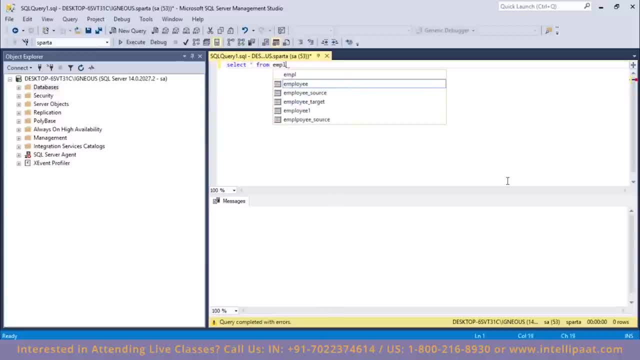 having a glance at the employee table, select star from employee right. so this is our employee table over here and we see that the highest salary is 159 thousand and the second highest salary is 125 thousand. so we are supposed to extract this particular value from this. 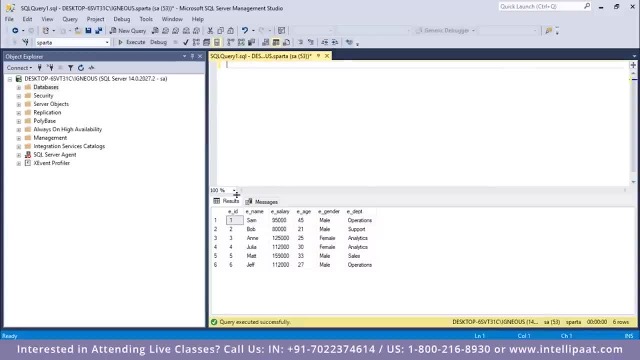 data set. now let's see how can we do this, so we can perform this operation with the help of sub query. now let me just type in the command select, and since you want the maximum value, I'll use the max aggregate function, and this would be E salary. so I want the maximum salary from the name of the table is: 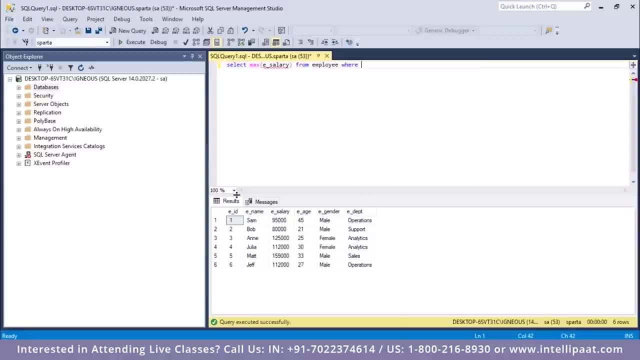 employee, I'll give in the where clause and, given the condition where E salary is not in after this, I will give in the sub query over here. so the sub query again would be the same. so select max of E salary from employee. so now, if you have a 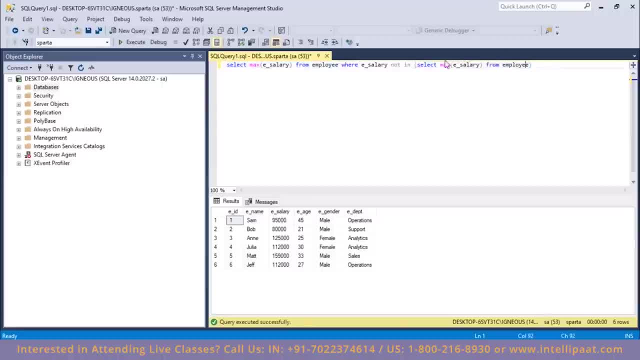 glance at this, you would see that both of these queries are same. so select max of E salary from employee and select max of E salary from employee. now this sub query would given this result, which is 159 thousand. so and then this main query over here we have to make sure that this salary does not lie in this. so this: 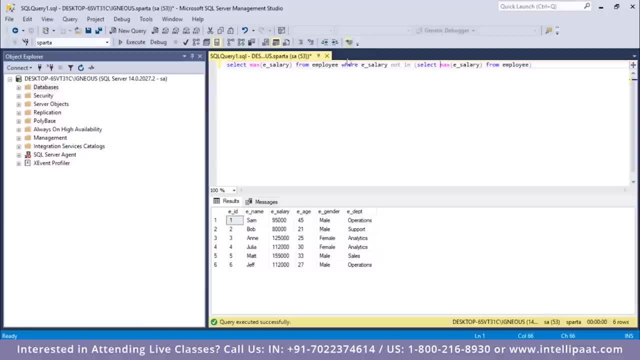 would give us the 125 thousand result. so select max of E salary from employee where E salary is not in 159 thousand. that would mean 125 thousand. so let me click on execute right. so we have successfully got the result, which is 125 thousand, and this is how we can extract the second highest salary. so we 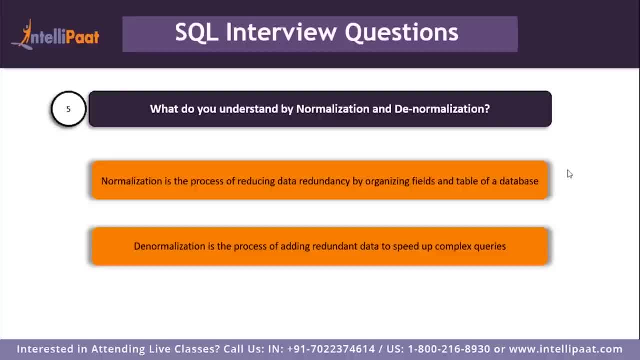 have our next question over here. so what do you understand by normalization and denormalization, which is very frequently asked during the interviews? so let's get to the answer. so normalization and denormalization are basically methods used in databases, and normalization is the process of reducing data redundancy. 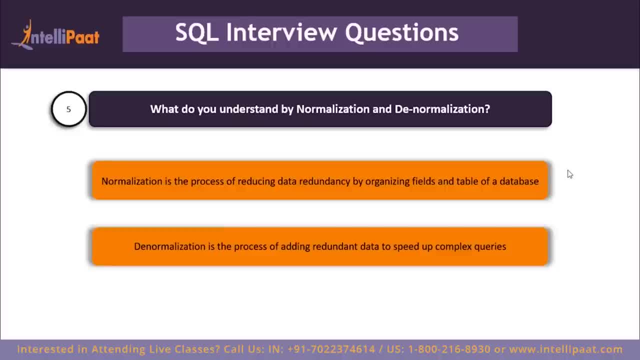 and dependency by organizing fields and tables of the database. so it involves constructing tables and setting up relationships between those tables according to certain rules, and the redundancy and inconsistent dependency can be removed using these rules in order to make it more flexible. so I am repeating it again, guys. so, simply put, normalization is the process. 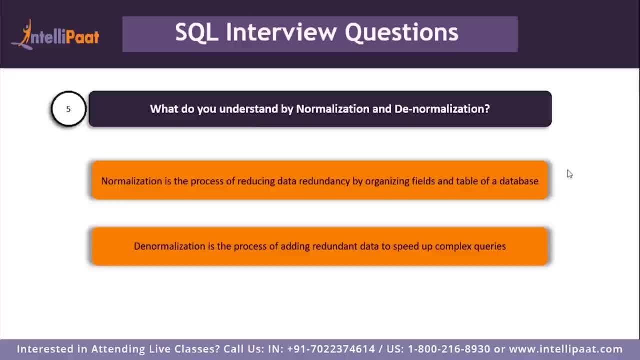 of reducing the data redundancy, and we are able to do this by organizing the fields and tables of the database. and then we have denormalization, which is a contrary process to normalization. so in denormalization we basically add redundant data to speed up complex queries involving multiple table joins. 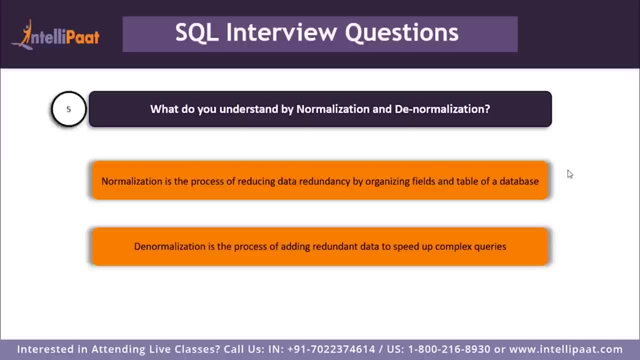 so in denormalization, we attempt to optimize the read performance of a database by adding different tables of the database and then in the process of reducing the data redundancy, and then, in the process of reducing the data redundancy, adding redundant data or by grouping the data right. so this is our next question. 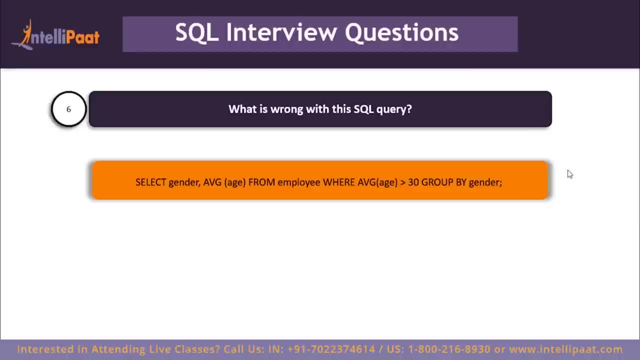 now we are supposed to find out what exactly is wrong with the sequel query. so this is the sequel query over here: select gender average of age from employee where average age is greater than 30. and again we are grouping this with respect to gender. so this is our employee table over here. now let me go. 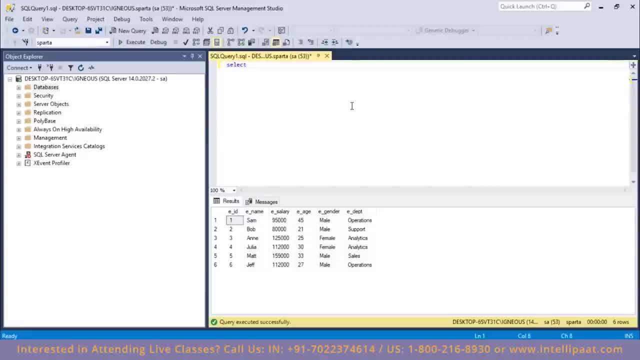 ahead and just type in the command which would be select e gender, and then I would want the average of age. so average of e age from the name of the table is employee, where again, the average of e age needs to be greater than 30, and this is being grouped with respect to gender. now let me go. 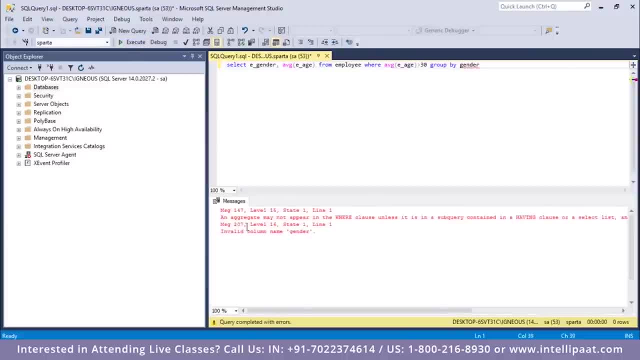 ahead, then we can execute. so let's see what is the error. so this warning message states that an aggregate may not appear in the where clause unless it is in a sub query contained in a having clause or a select list, and the column being aggregated is an outer reference. so this basically means that whenever we are 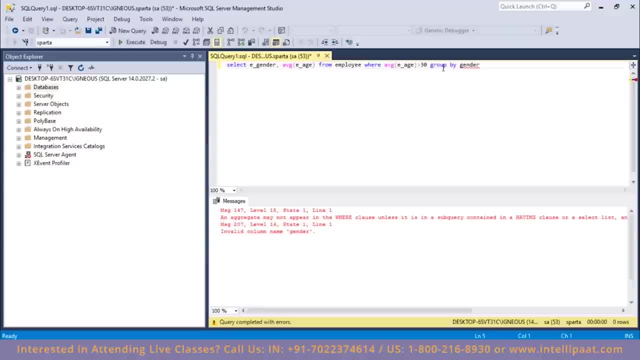 working with aggregate functions and we are using group by, we can't use the where clause, so instead of the where clause, you would have to use the having clause. now let me change this to having and let me click on execute. so now again we get an error over here and this error says that incorrect. 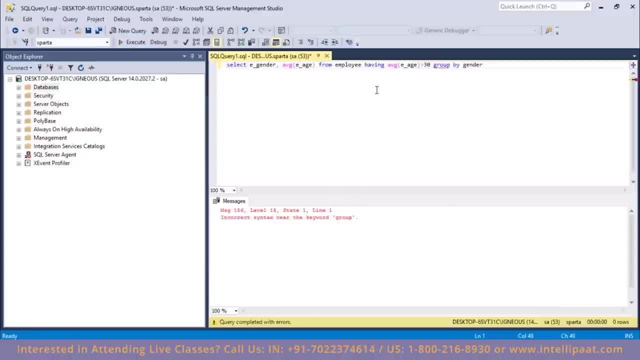 syntax near the keyword group, and this is because if we are using the having clause, then group by would come first and having would come second. now let me cut this over here and let me paste this before having. right now I click on execute, so this has to be e gender over here. now we've successfully got the 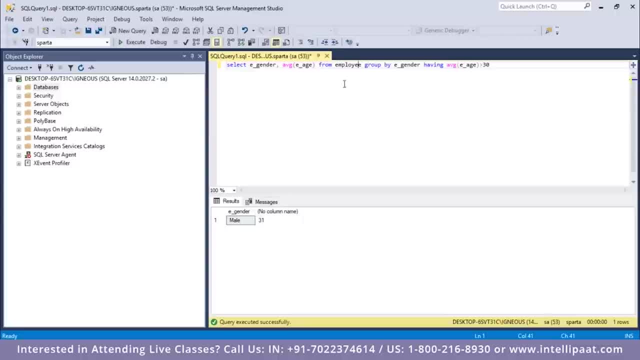 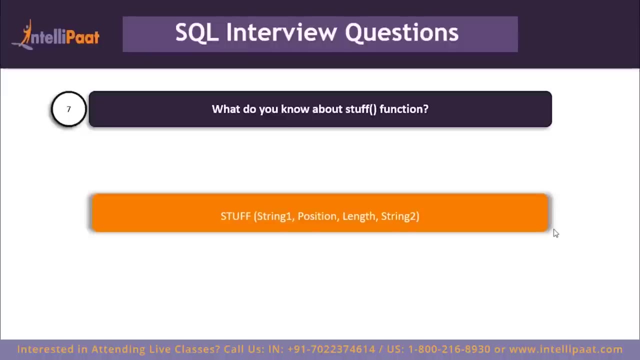 result. so just to reiterate the errors: whenever we are working with aggregate functions, we cannot use the where clause and we would have to use the having clause. and if you are also using group by with having, then group by would come first and having would follow it. so next question: so what do you know about the? 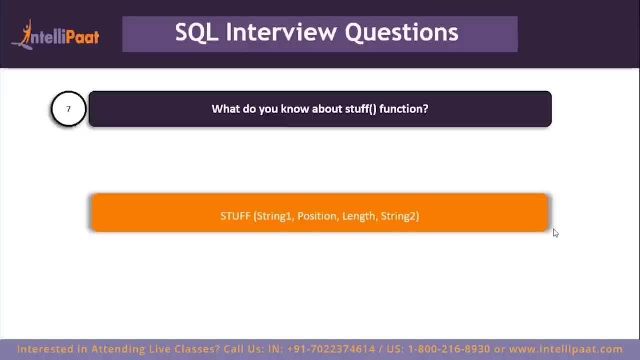 stuff function. so their stuff function deletes a part of the string and then inserts another part into the string, starting at a specified position. so this is the syntax of the stuff function. so stuff the stakes in these four parameters: string one, position, length and string two. so this string one is basically that string which would be overwritten. 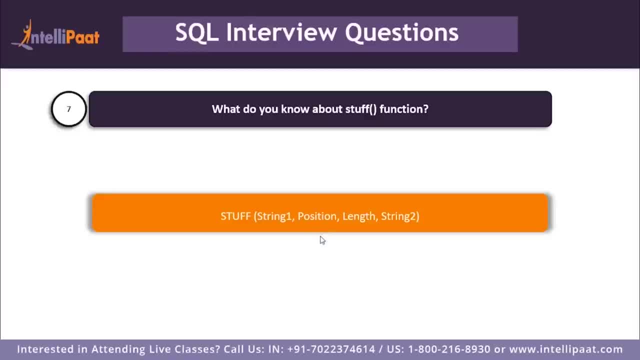 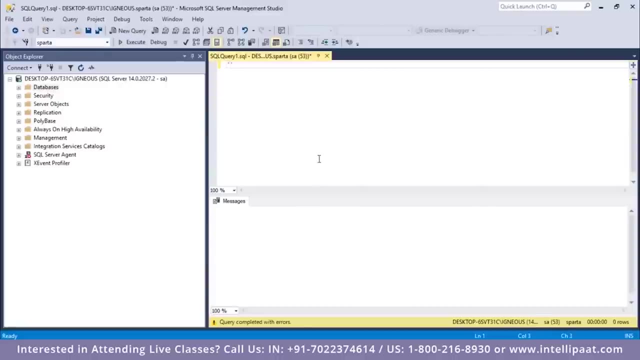 position would basically indicate the starting location for overwriting the string and length is the length of the substitute string. and string two is dart string, which would overwrite the string. so again let's go to SQL server and work with an example with the stuff function. so now let's say I have this: 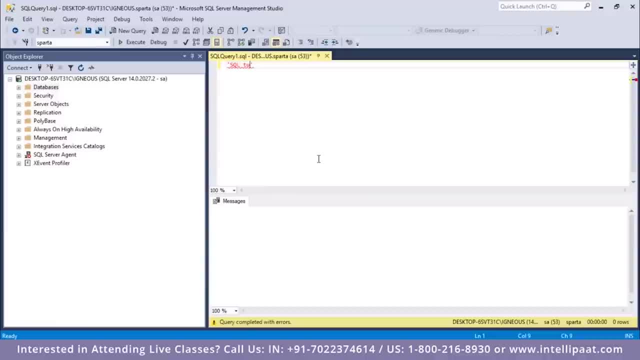 string which basically stands like this sequel tutorial. now I'd want to replace this sequel tutorial with Python tutorial. right, so for this purpose we can actually use the stuff function. so let me go ahead and write the syntax for that. it would be select. I'll give in the 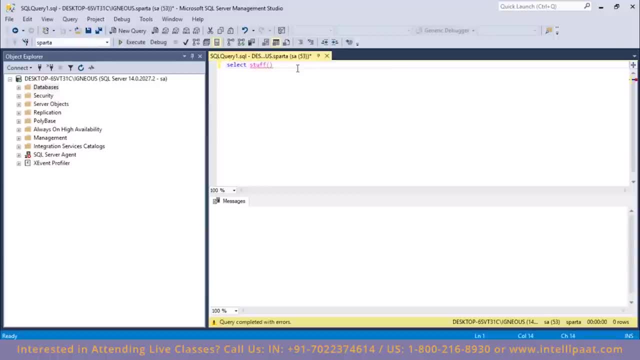 function stuff. so let me start with the force parameter, which is the string which is to be replaced. so the string which is to be replaced as sequel tutorial, and then I'll give in the second argument, which is the position. so the position would be one, that is, I want to replace this. so this is position number one, and then I would 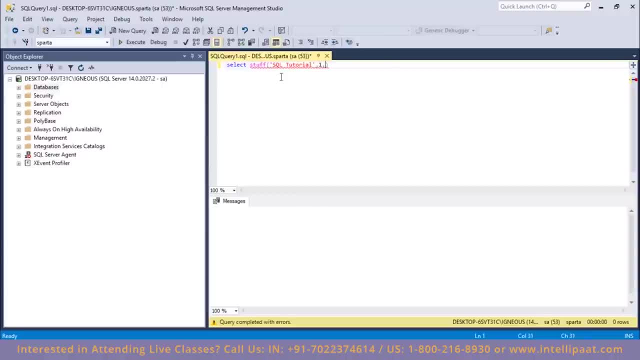 have to give in the length of the string which is substituted, right. so the length of SQL is three. I'll just type in three over here and then, finally, I will give in string two, which is basically that string which would replace this over here. so I would type in Python over here now. I'll execute so, initially our string. 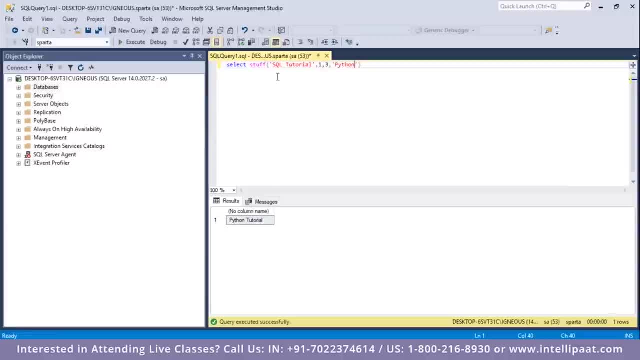 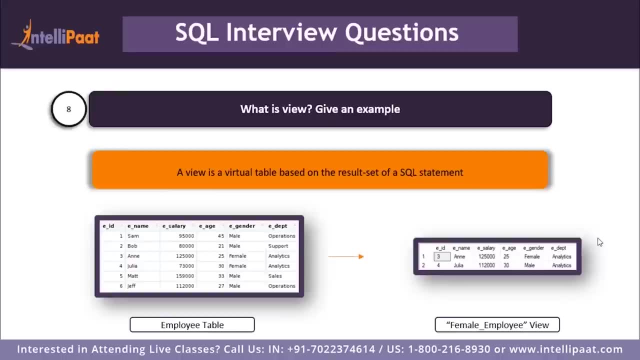 was sequel tutorial and with the help of the stuff function, you were able to change this from sequel tutorial to Python tutorial. so next up we'd have to explain about views and sequel- so what exactly is a view? and then we'd have to give an example of you so you can consider views. 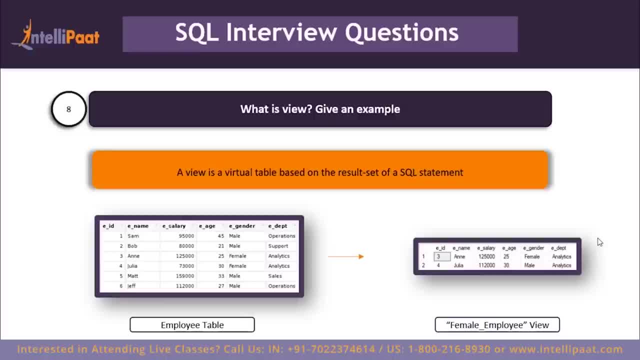 as virtual tables which are used to limit the information that we want to display, and these are actually nothing but the result of an sequel statement- which have a name associated with them, and since views are not virtually present, it takes less space to store. so let's take this example from this. 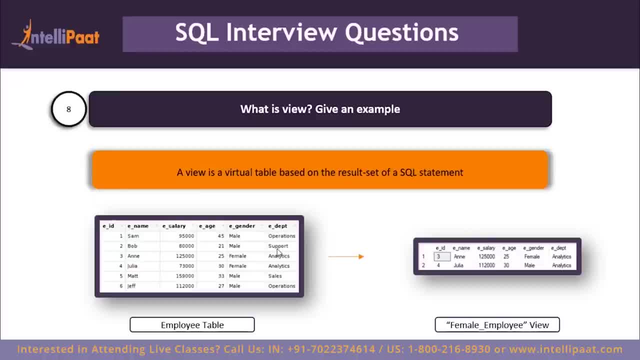 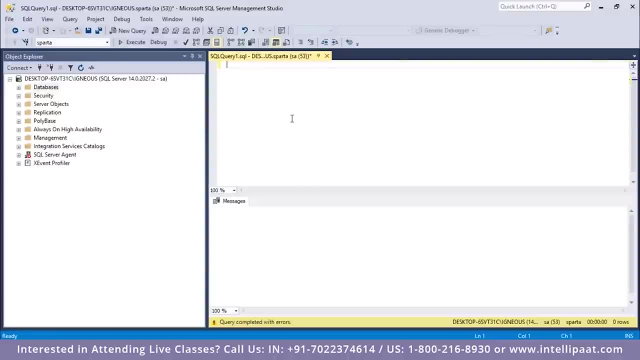 employee table. let's say we wanted to perform multiple operations on the records where the gender is female, so we can create a view only for the female employees from the entire employee table. so let's go ahead and perform this in sequel server. now let me type the syntax for this. so I would want to create a view. 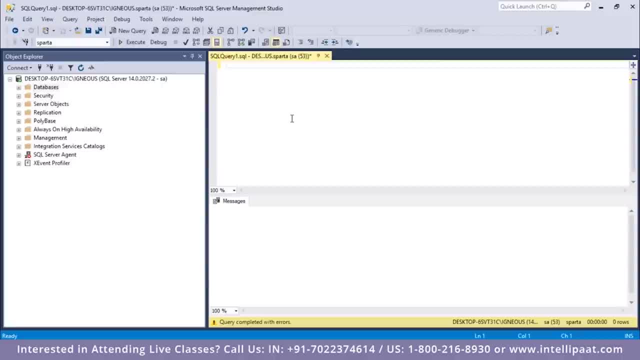 which would comprise of only the female employees from the entire employee table. now let me just have a glance at the employee table first. so select star from employee. now I would want a view which would comprise of just these two records. now let me go ahead and write in the syntax for the view, so it'd be create. 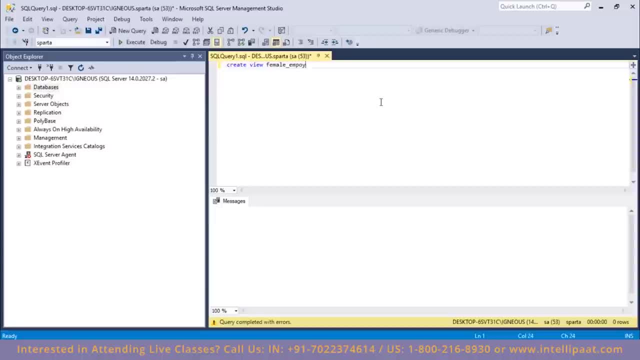 view and the name of the view would be female employee, and after this I will give in the keyword AS. after that I'll type in select and then I'll given the condition. so select star from employee where. after the where clause I will give in the condition which actually matters. so gender needs to be equal to. 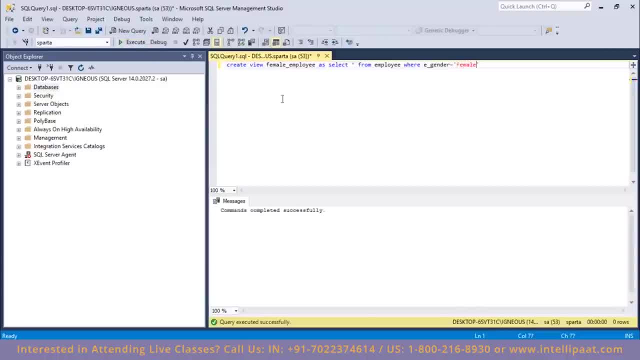 to female right. so I have successfully created this view with the name female employee, which would comprise of only the records of the female employees. now let me delete this and let me have a glance at the view which I've just created. so select star from female employee right. so this is our view, which 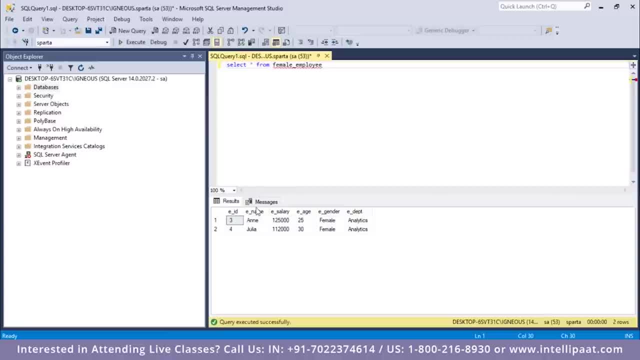 comprise of these two records, and the names of the employees are Anne and Julia. now, similarly, let's say: if I wanted to view, which would comprise of only those employees whose age is greater than 25, so let me go ahead and write the syntax for that. so create view and then let's say the name of the view. 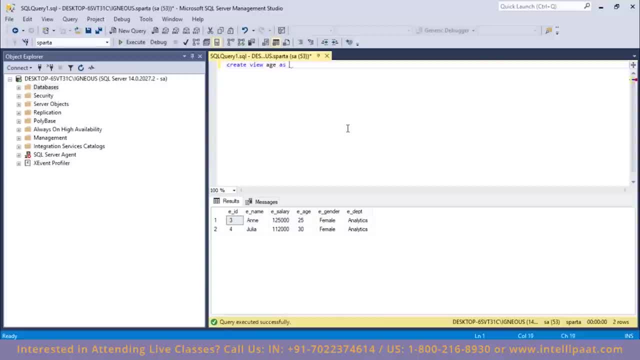 is age, and then I'll type in the keyword is select. now over here, let me give in the statement: so select star from employee, where condition would be: E age needs to be greater than 25. so we have created this view. now let me have a glance at this. so select. 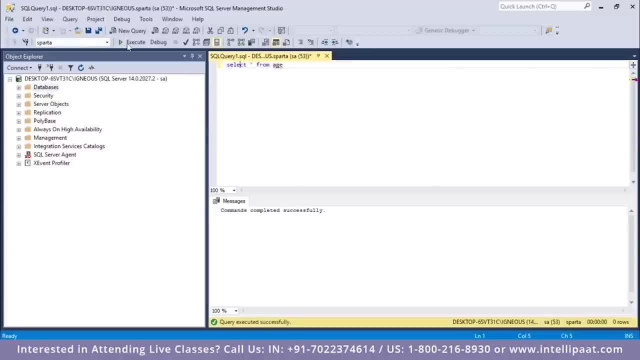 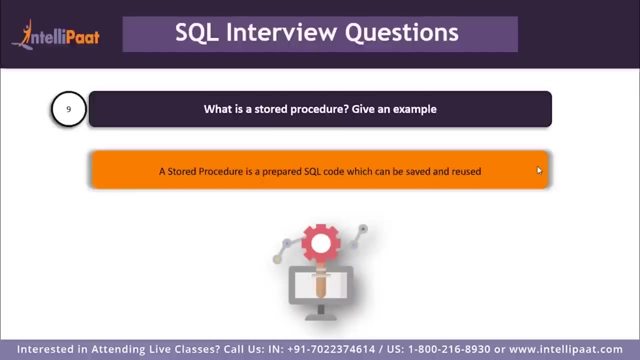 star from age, right? so this is a view which would comprise of only those records where the age of the employee is greater than 25, and we've got four records over here: Sam's age is 45, Julia's age is 30, Matt's age is 33 and Jeff's age is 27, right? so what is a stored procedure? and then, 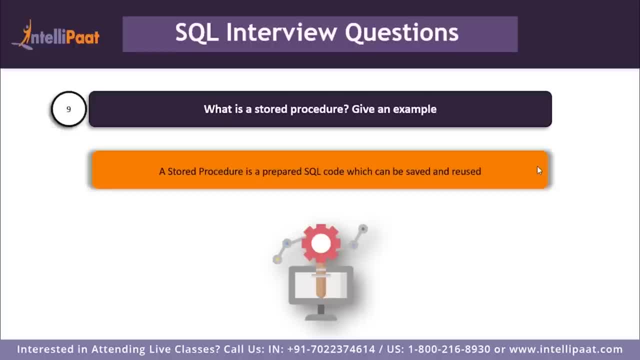 we'd have to give an example of stored procedure. so a stored procedure is a prepared sequel code which can be saved and reused, or in other words, you can consider a stored procedure to be a function consisting of many sequel statements to access the database system so we can consolidate several sequel. 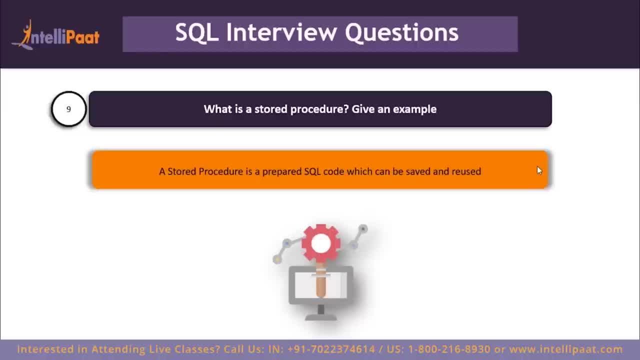 statements into a stored procedure and execute them whenever and wherever required. and the stored procedure can be used as a means of modular programming, that is, you can create a stored procedure once, store and call for several times whenever required. so this supports faster execution when compared to executing 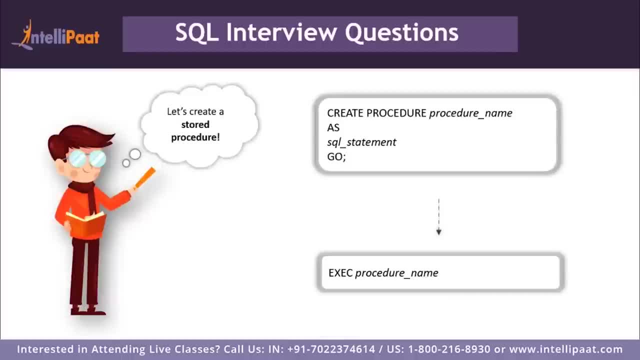 multiple queries. now let's look at the syntax of a stored procedure. so well, given the keywords create, procedure, and then we'll give the procedure name over here. after that we will give in the keyword E, S, and then we'll give the sequel statement for which we'd want to create the procedure, and then we'll 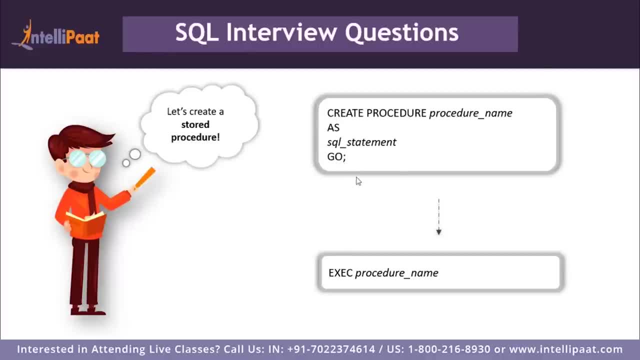 end the procedure with the No keyword. now, after we create a procedure, we need to execute it. so this is the syntax to execute the procedure. so we'll type in exe C and then give the name of the procedure which is to be executed. right, so again, let's have an example with the 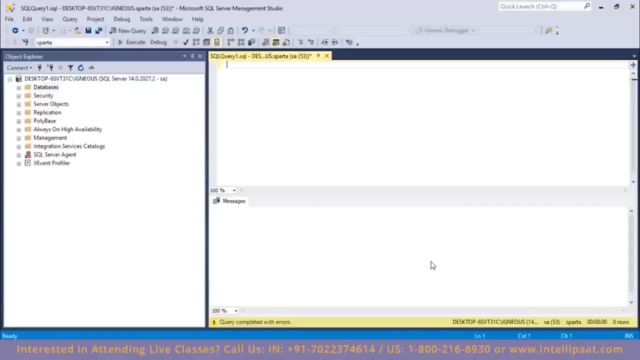 stored procedure. so now I'm going to create a stored procedure which would help me to extract the age of the employees in a very easy way. so let me type in the syntax for that create procedure and then I'll give in the name of the procedure. so this would be employee age. after this, I will type in: 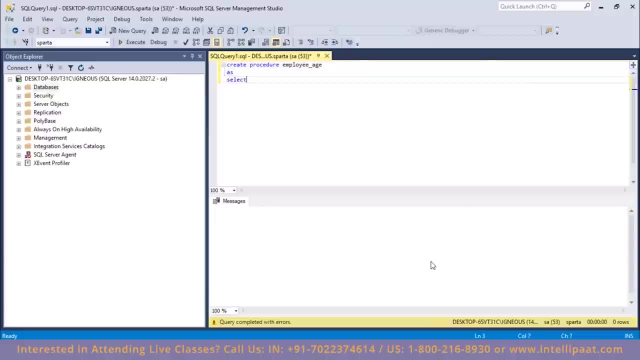 the keyword es and then I'll give in the select statement. so select eh from employee. now that this is done, I'll give in the go keyword right. so now I have successfully created the stored procedure with the name employee age. now I'll go ahead and execute this. so it'll be exe C or execute employee age. 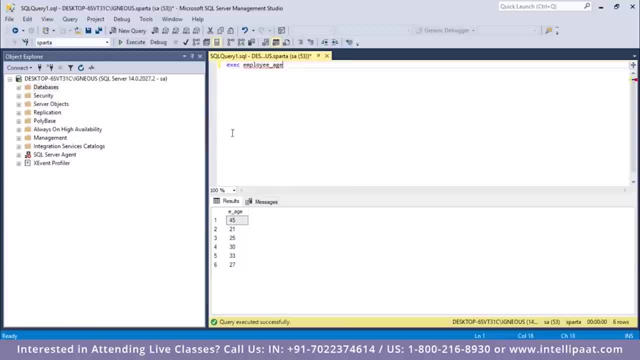 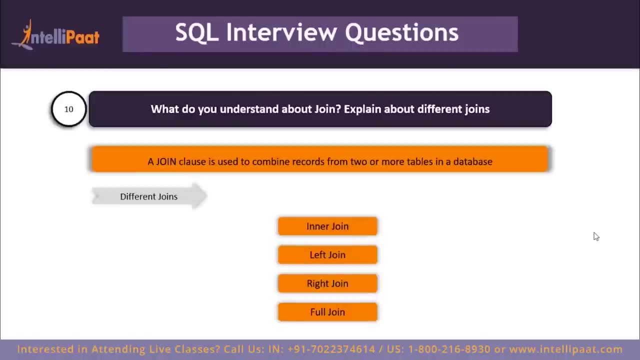 right. so we have created the stored procedure which would help me to easily access the age column from this employee table. so next question: what do you understand about join and explain about different joints? so what join clauses used to combine rows from two or more tables based on a related column between. 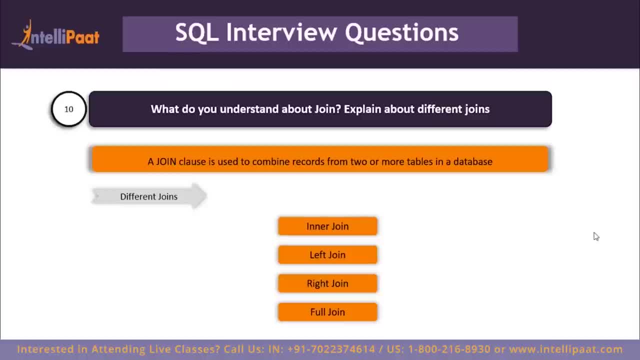 them. so there are. there are. there are various types of joints which can be used to retrieve data, and it depends on the relationship between tables. so first we have inner join, which basically returns records that have matching values in both the tables. then we have left join, so left join returns rows which are common between the tables and 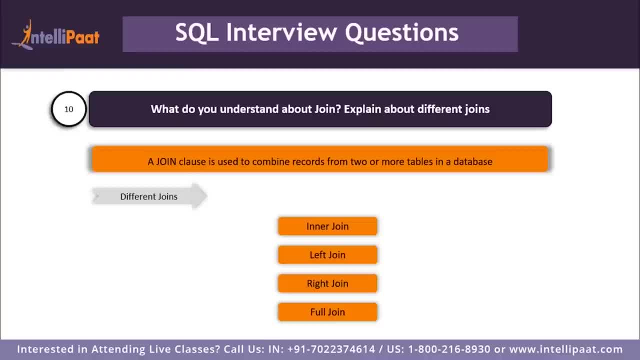 all rows of the left hand side table. that is, it returns all the rows from the left hand side table even though there are no matches in the right hand side table. then we have right join, so right join returns rows which are common between the tables and all the rows of. 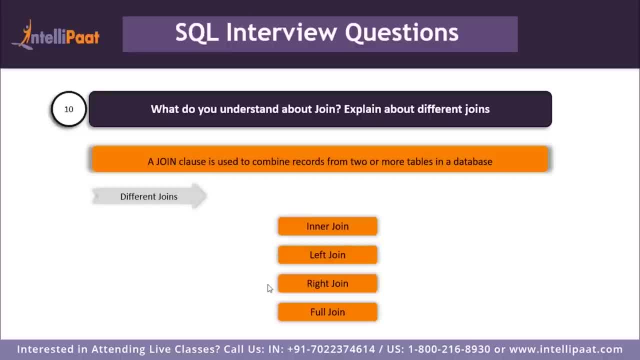 the right hand side table. there is. it returns all the rows from the right hand side table, even though there are no matches in the left hand side of the table, and finally we have the full join. so full join returns all rows on the left hand side table and all the rows on the right hand side table. so now we'd 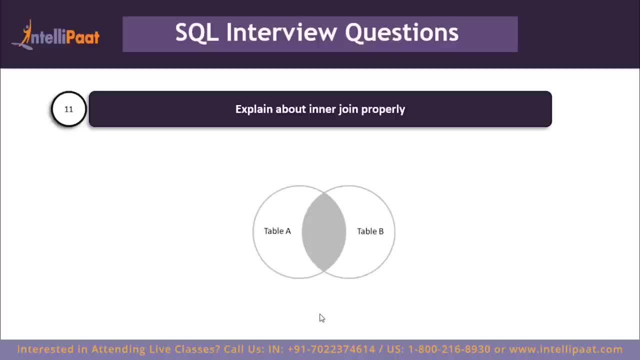 have to explain about inner join properly. so the inner join basically gives us those records which have matching values in both the tables tables. so we've already learned this. now let's say we have two tables, table A and table B, and when we apply inner join on these two tables, we'll get only those. 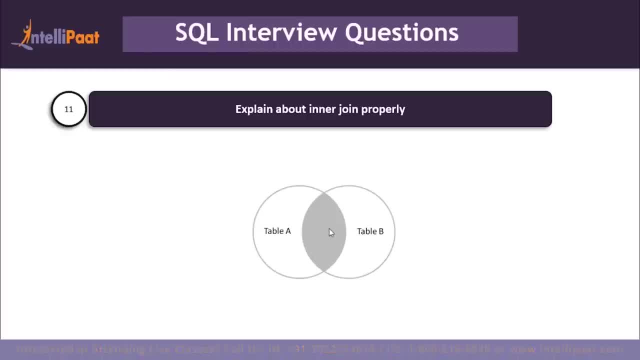 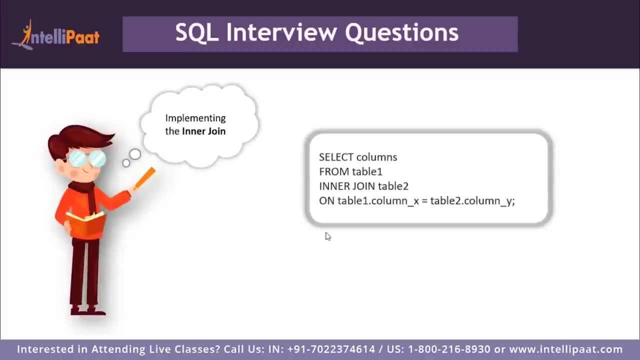 records which are common to both table A and table B. so this gray portion which you see over here. so this would be the result of the inner join. now let's look at the syntax of inner join. so we'll give the keyword select and then we'll 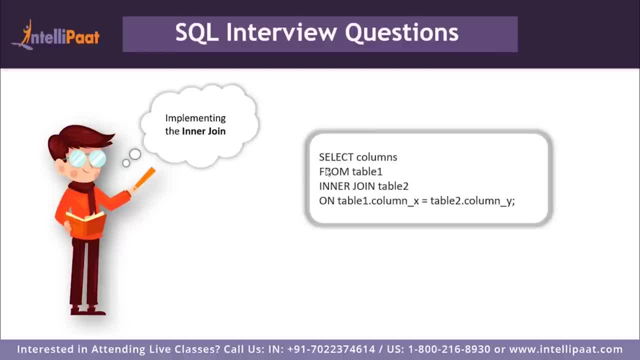 give in the list of the columns following, which will give the from keyword and then we'll give the name of the first table. then we'll use the keywords inner, join and then give the name of the second table, after which we'll gives in the on keyword. so this on keyword tells SQL that this inner. 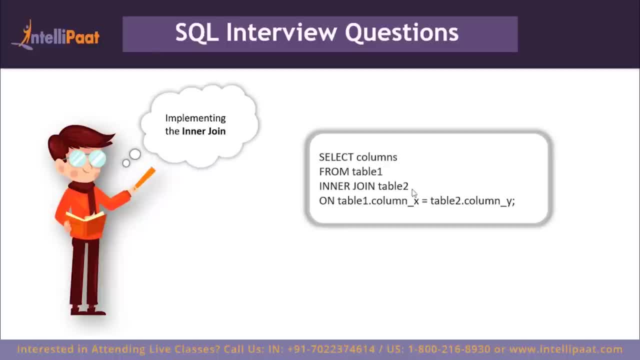 join needs to be done on some condition, and the condition over here states that the values from column X of table 1 should be equal to the values of column y from table 2. let me just retread this: the values of table 1 should be equal to the values of column y left over under table 2, enough. 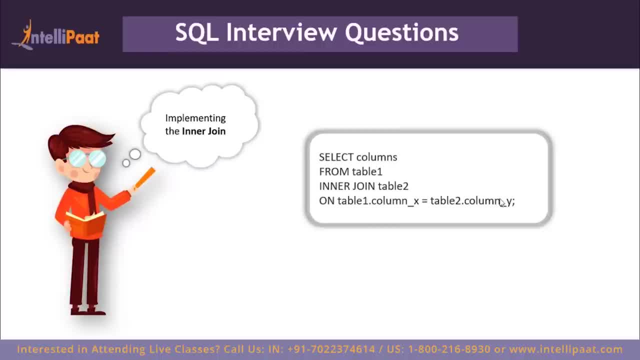 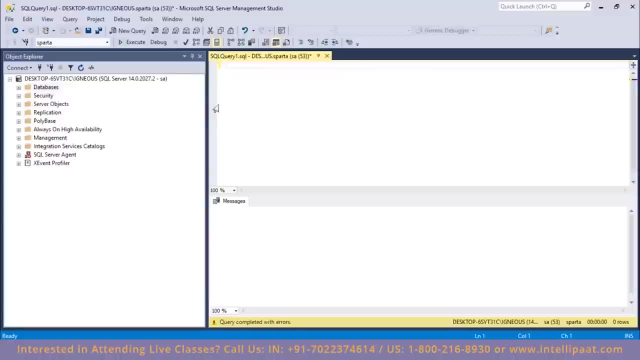 column x from table 1 should be equal to the values of column y from table 2.. Now let's go to SQL server and work with this inner join. So I have two tables over here. So the first table would be the employee table and the second table would be the department table. So let me have a 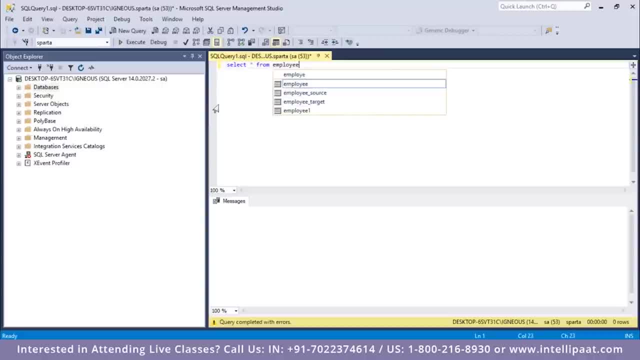 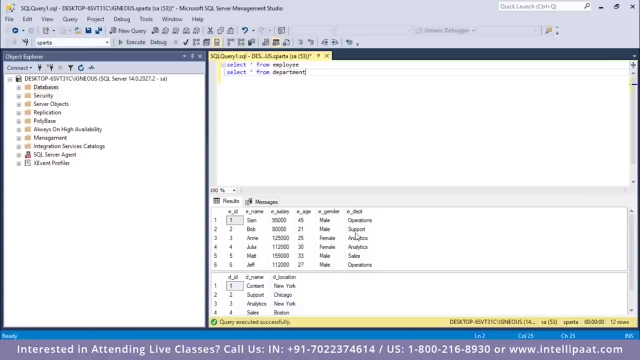 glance at both of the tables. So select star from employee. Now the second command would be select star from department. So this is the employee table over here, which we've already seen, and then we have this department table. Now I'd want to have an inner join on both of these tables where 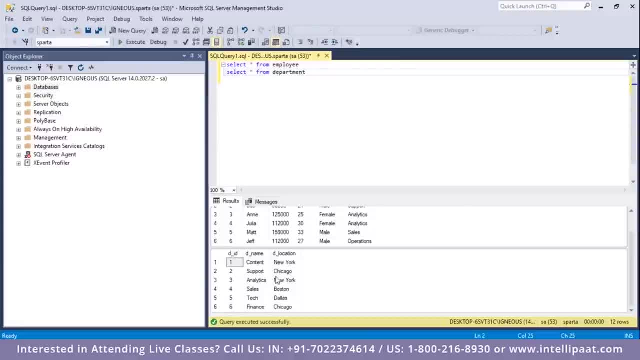 the edept column from this table is equal to the dname column from this table, That is, wherever the values from these two columns match. I'd want only those records. Now, let me go ahead and write the syntax for this, So I will type in: 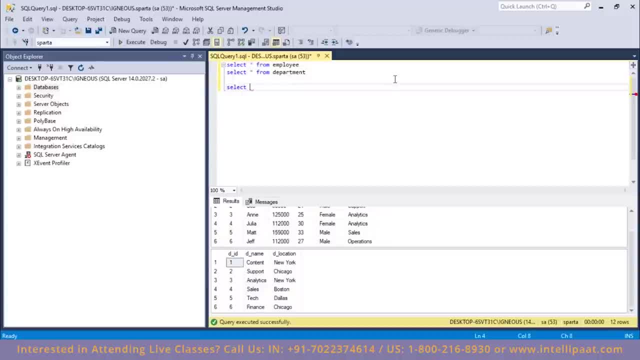 cd select and then I'll give in all of the columns which I want. So I want the ename column and edepartment column from the employee table. So this would be employeeename, Then I would want employeeedepartment. After that I would want the department name and the department location. 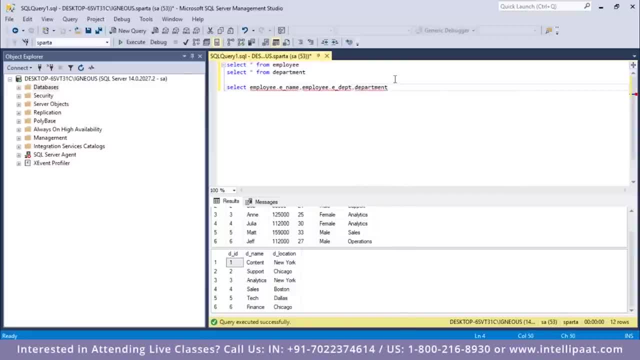 from the department table. So I'll type in departmentdename and then I'll type in departmentdelocation, Right? so these are all of the columns which I want from both the tables. Now, after this, I'll type in from and then I will type in the name of the first table, which is 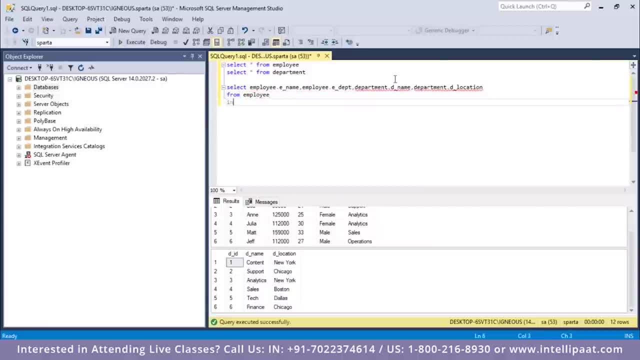 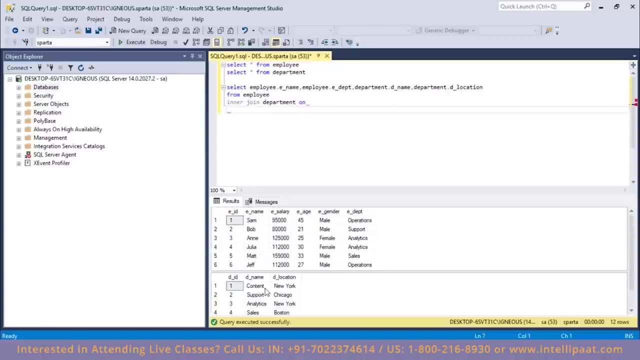 employee, and then I'll just type in inner join and then give in the name of the second table, which would be department. Then I'll give in the on keyword and then give in the condition. So here the condition is The values of the dename column should be equal to the values of the edept column, So employeeename. 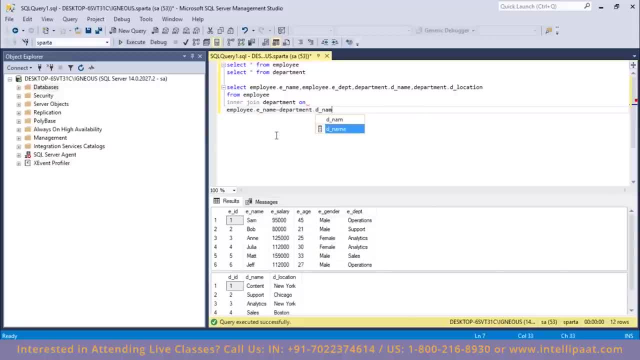 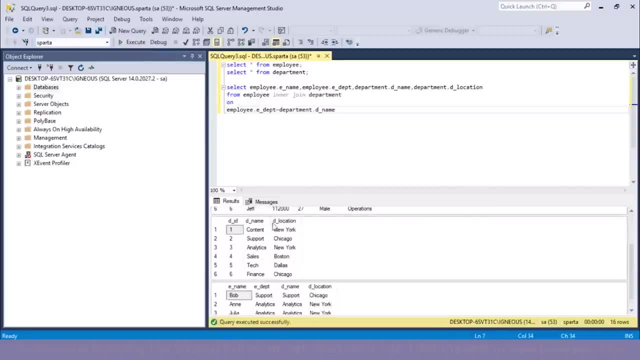 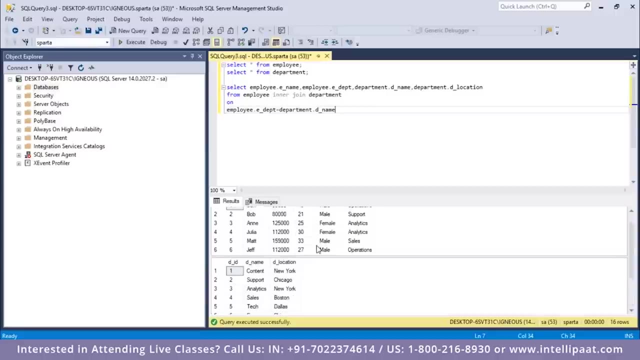 should be equal to departmentdename. Now I'll execute this Right. so this is the result. So we have our employee table over here, This is the department table and finally, this is the result of the inner join. So here we see that we've got only those records where the departments match in. 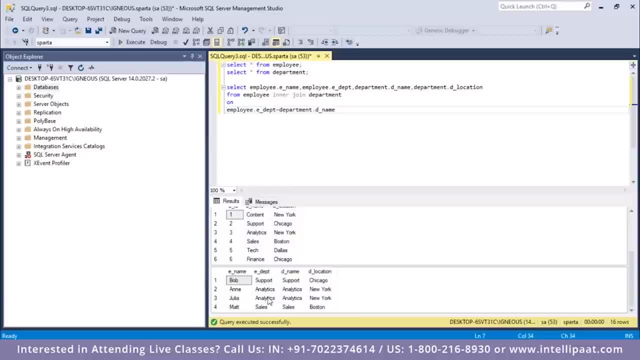 both of the tables. So the match departments are support analytics and sales. Right, so we've got support analytics and sales from over here, because only those departments are present in this department column. So next question: Well, what do you understand about temporary table? And then we'd 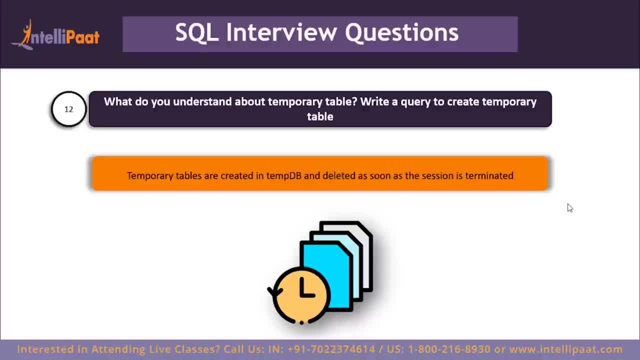 have to write a query to create a temporary table. So, simply put: temporary tables basically help us to store and process the intermediate results. Now these temporary tables are created in the tempdb and are automatically deleted, So we have to write a query to create a temporary table. 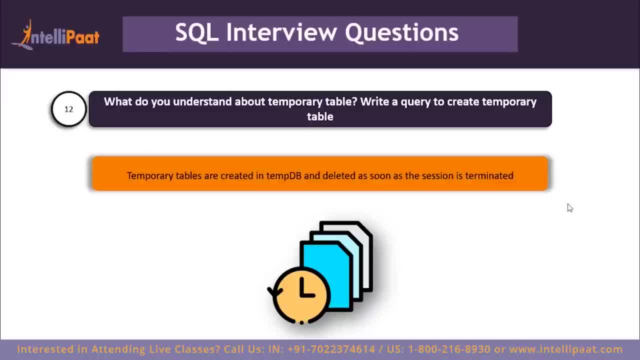 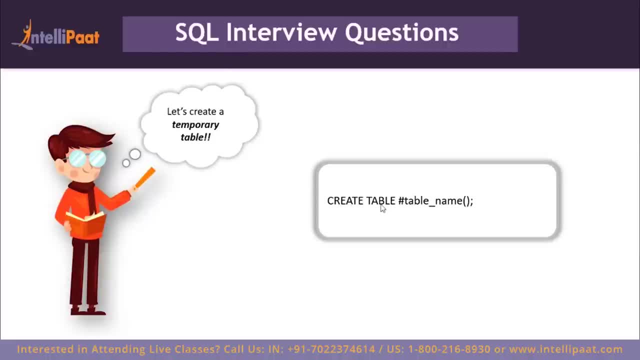 later we need to change the query name if we want to name it, And so that way we will be able to create a temporary table. and they are no longer used. So the temporary tables could be very useful in cases where we need to store temporary data. So now let's look at the syntax of a temporary 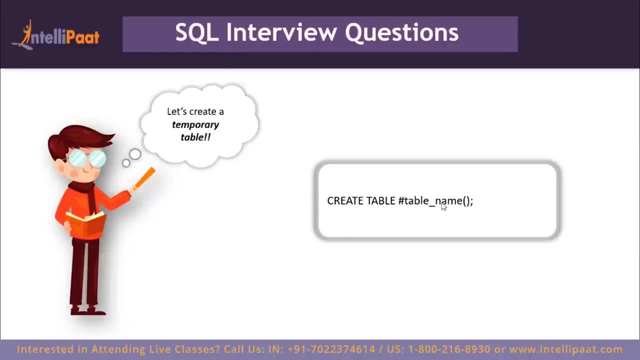 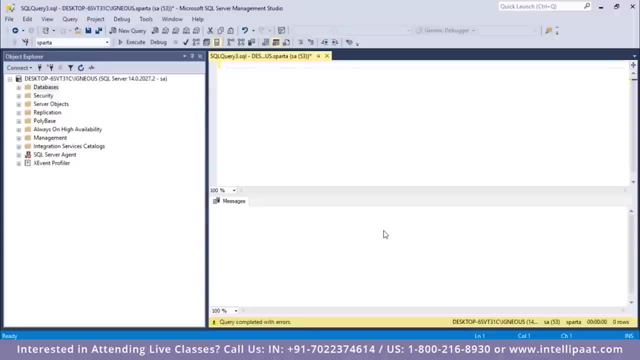 table. So first we will be given the keyword create table, And before we go ahead and give the name of the temporary table, we'll have to precede it with a hash. So again, let's go ahead and create a temporary table. So now what I'll do is I will create a temporary table and I will name this as: 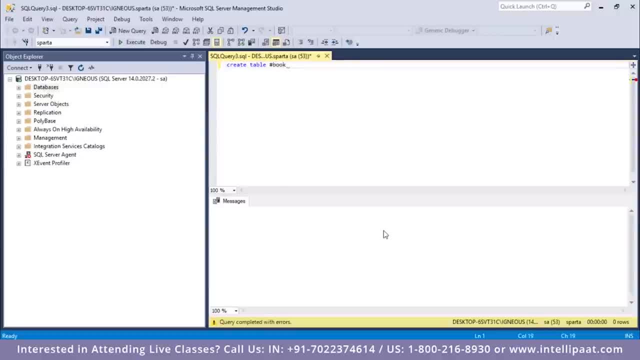 and then, before the name of the table, I'd have to precede it with a hash. right now. this would have two columns, so first would be the book ID, and this would be of integer type, and then this would have book cost, which is again of integer type. now let me execute this. now I'll refresh over here. I'll click on the. 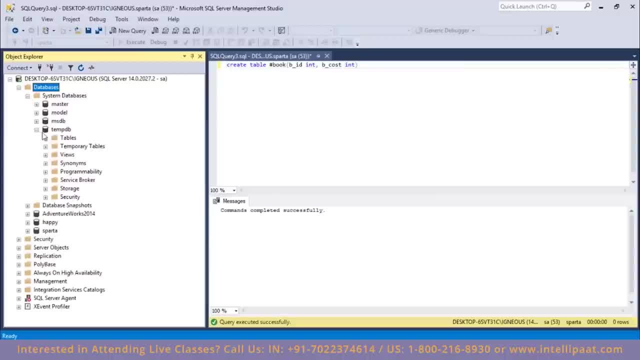 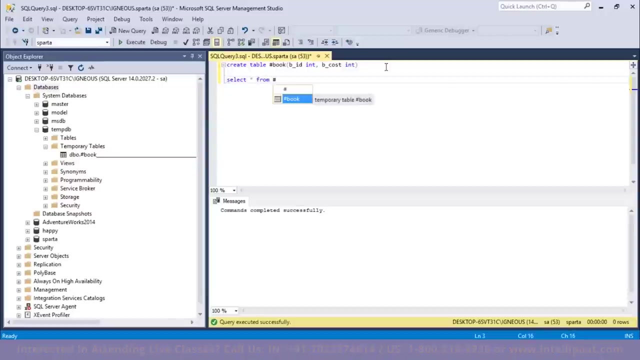 plus sign. I'll go into system databases and I'll go into temp DB and over here let me click on the temporary table so we see that we have successfully created this temporary table with the name book. now let me see what is present in this table. so I'll type in select star from. I'll put in the hash symbol over here. 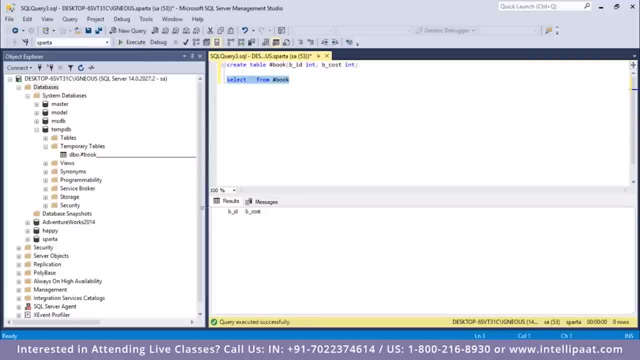 and then I'll give in book right. so as of now, this temporary table is empty. now let me go ahead then insert something into this table, so the command would pretty much be the same as the previous one. so I'll go ahead and insert something into this table, so the command would pretty. 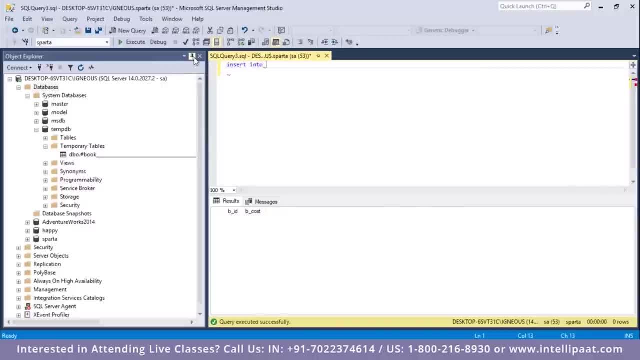 much be the same. so insert into and then LB book. I'll type in values over here. so the only difference which you see when you're creating or working with the temporary table and the normal tables is you would have to precede the name of the table with the hash. so as simple as that, rest everything would be. 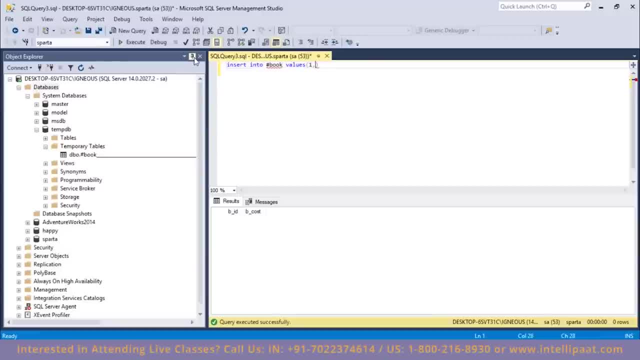 the same, and over here let me give in the values. so the book ID is one and the book cost us hundred. right now let me also add another record. so the second ID would be two and now the book cost would be, let's say, 232 all. 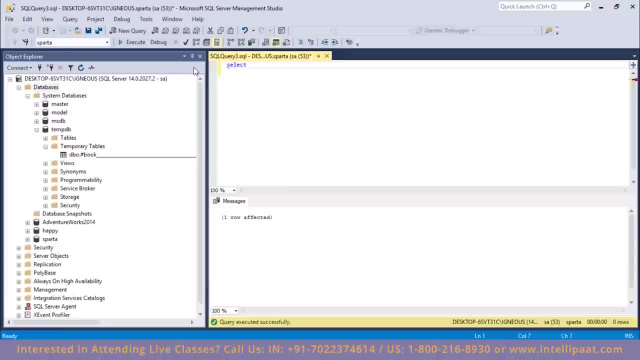 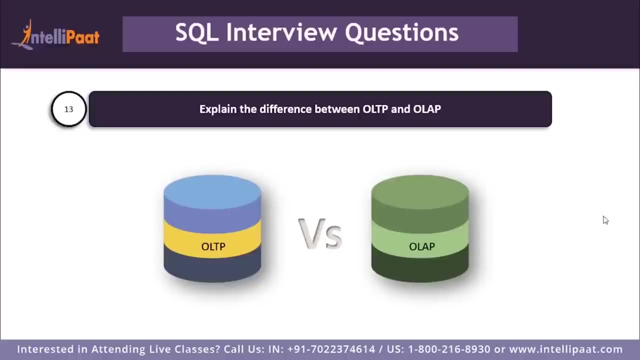 right now. let me have a glance at this modified temporary table. so select star from hash book, right? so we have added two records into this temporary table. so now we'd have to explain the difference between OLTP and OLAP. so let's start with OLTP. so OLTP basically stands for online transaction processing. 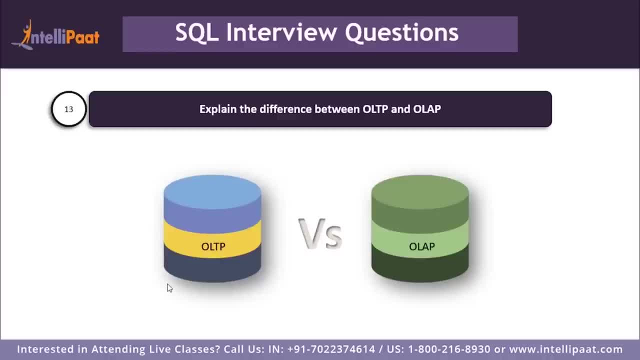 and you can consider it to be a class of software applications capable of supporting transaction oriented programs, and an important attribute of an OLTP system is its ability to maintain concurrency. so OLTP systems often follow over decentralized architecture to avoid single points of failure, and these systems are generally designed for a large audience of end-users who conduct 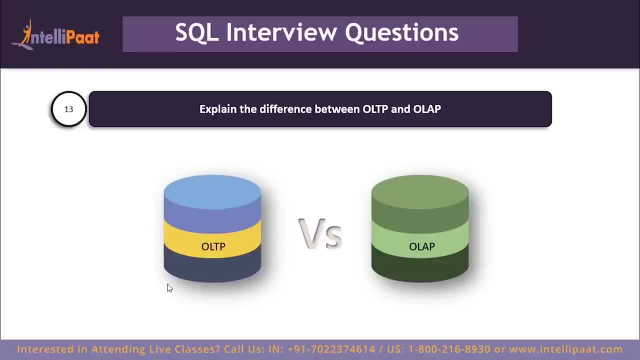 short transactions and queries involved in such databases are generally simple, need fast response times and return relatively few records, so the number of transactions per second acts as an effective measure for that systems. then we have OLAP. so OLAP stands for online analytical processing and it is a class of 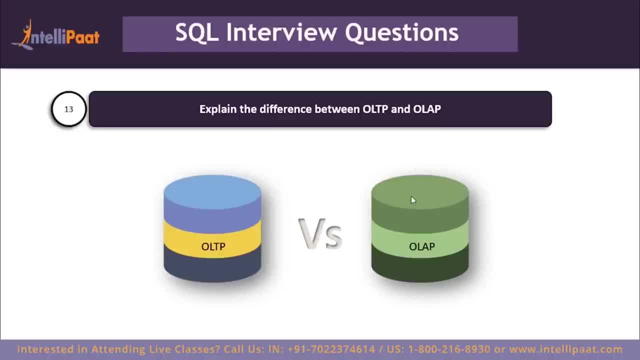 software programs which are characterized by relatively low frequency of online transactions, so queries are often too complex and involve a bunch of aggregations, and for OLAP systems the effectiveness measure relies highly on response time. so we have a class of software programs which are So such systems are widely used for data mining or maintaining aggregated historical data. 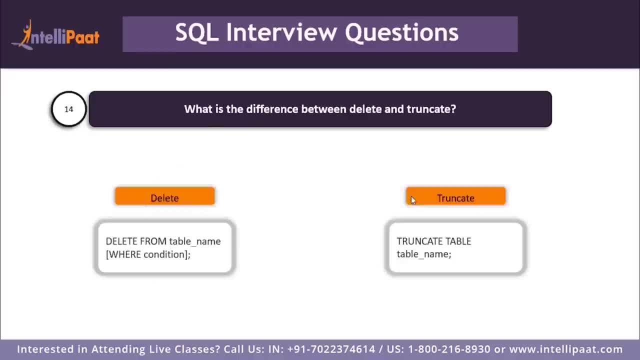 And this is usually used in multi-dimensional schemas. So then we have the next question. So what is the difference between the delete and the truncate command? So again, keep this in mind, guys. This is a question which is very frequently asked in interviews. 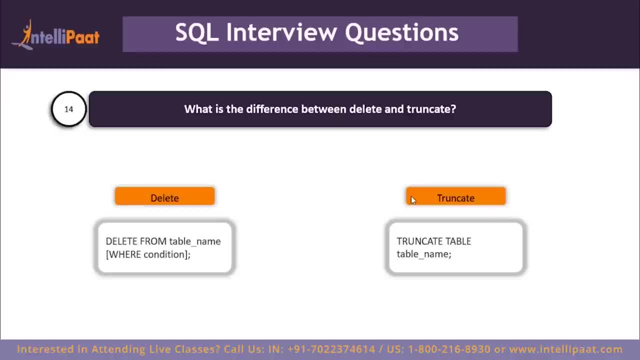 So let's start off with the delete query. So the delete query is used to delete or remove one or more existing tables. So let's have a look at the syntax. So we'll start with the delete keyword and then we'll put in the keyword from. 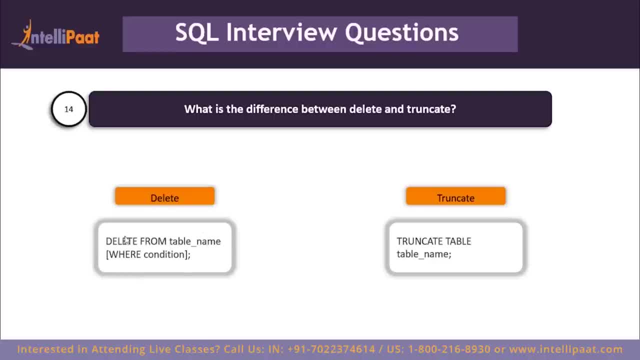 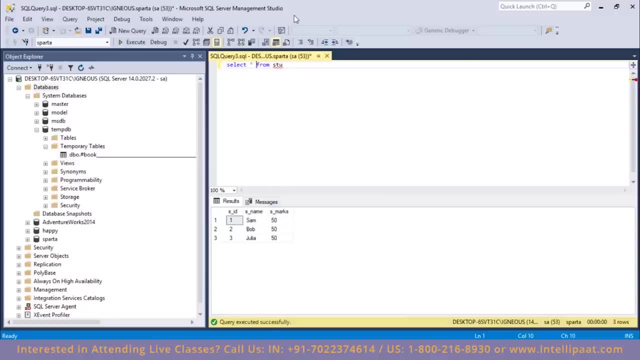 Then we'll specify the name of the table. After that we'll specify the where condition, but then that's optional. So let's see an example of this delete command. So we have this table. So the name of the table is STU, which basically is the student table. 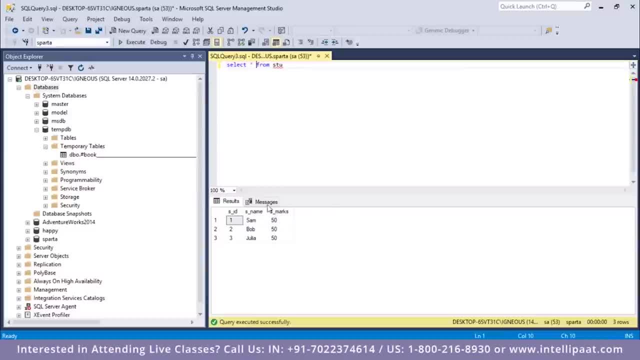 Now from this table. I'd want to delete the record where the name of the student is Bob. So let me write the syntax for that. So delete, Delete from, and then I'd have to give in the name of the table. So the name of the table is STU. 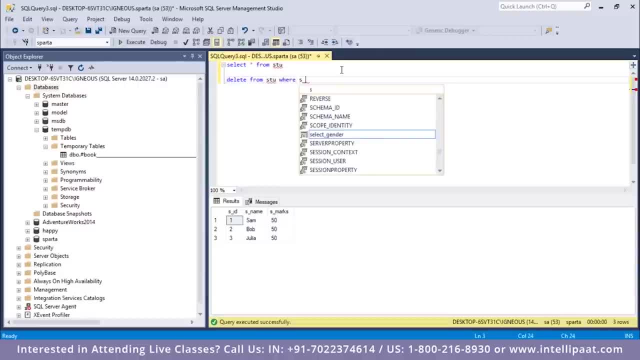 So delete from STU. After that I'll give in the where clause and give the condition where S name is equal to Bob. Let me execute this Right. So we have successfully deleted that record from this table, where the name of the student was Bob. 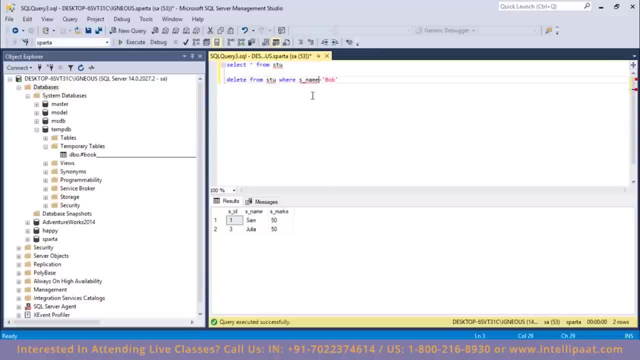 So, similarly, let's say: if I want to delete that record where the student ID is 3. So over here the condition would change. So delete from STU where S ID equals 3.. So now, this time we have deleted that record where the student ID was equal to 3.. 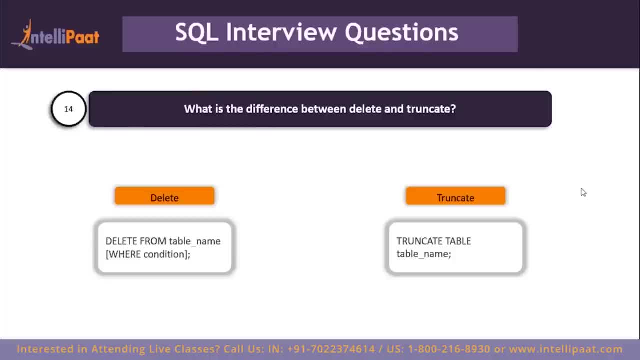 Now let's look at the truncate statement. So the truncate statement deletes all of the data inside the table. So here we'll give in the keywords truncate table and then give the name of the table. So let's go to SQL Server and work with this truncate command. 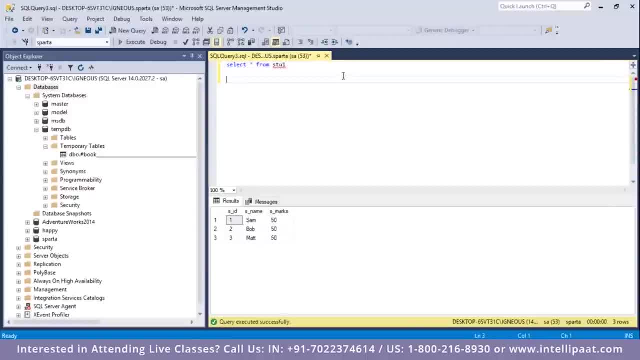 So now we have this STU1 table, So let me go ahead and use the truncate command of this table. So I'll type in truncate and then I'll give in the name of the table, which would be STU1.. So before that I'd have to type in tables: truncate table STU1.. 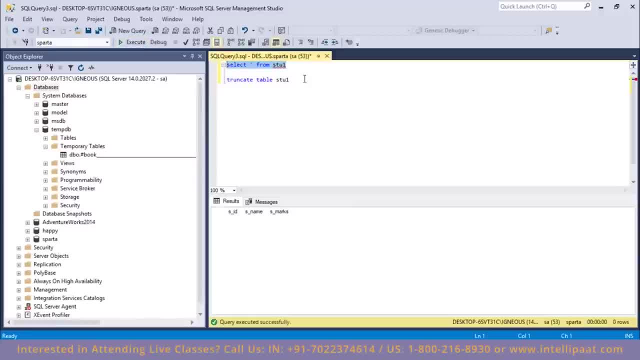 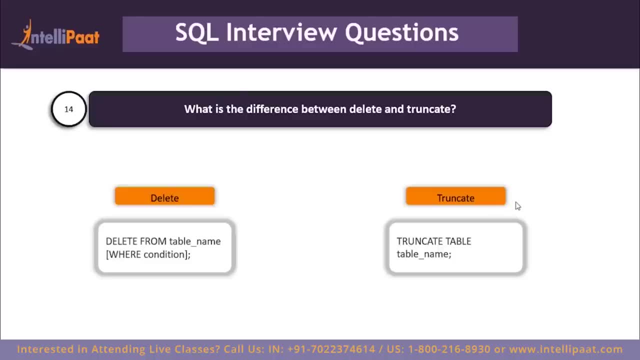 Let me run this Right. So we have deleted all of the records from this table. So this is how the truncate command works. Now let's understand some differences between the delete command and the truncate command. So, when it comes to the type of language, truncate would be your DDL command. 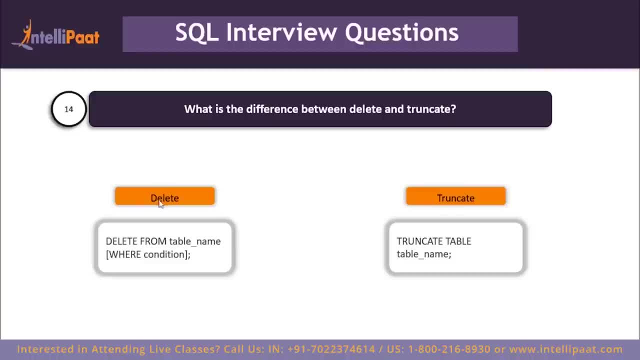 or a data definition language command, and delete is a DML command or a data manipulation command. Now, another difference would be we can't really execute a trigger in case of truncate, While with delete we can accomplish a trigger Now. also, if a table is different by any foreign key constraints, then truncate won't work. 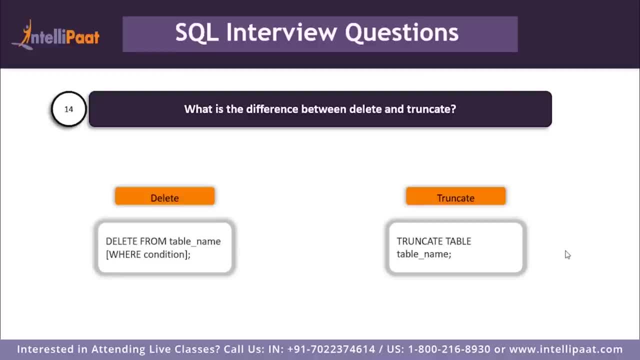 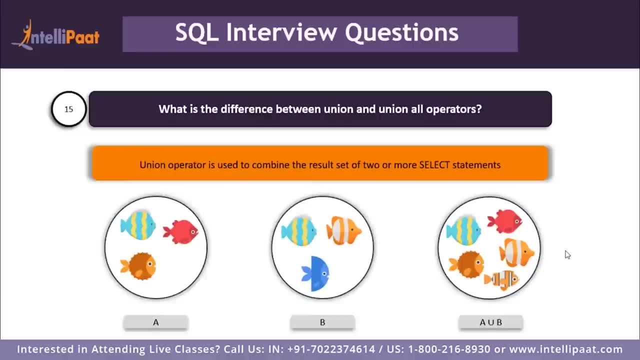 So if you have a foreign key, then you'd have to use delete and you wouldn't be able to use the truncate command. So next question: what is the difference between union and union all operators? So the union operator is used to combine the result set of two or more select statements. 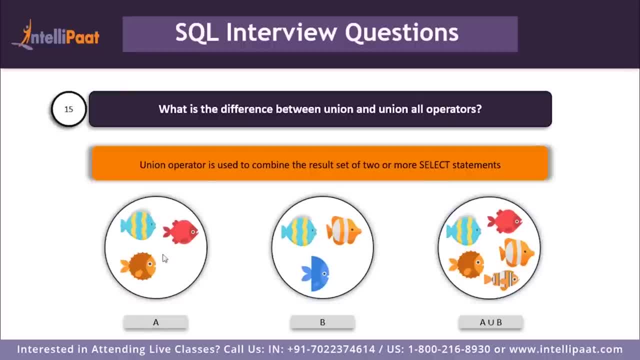 For example, if the first select statement returns these three fish and the second select statement returns these three fish, then the union operator would return the result of these two select statements, And if there is a record which is present in both the tables, we'll get only one of them in the final result. 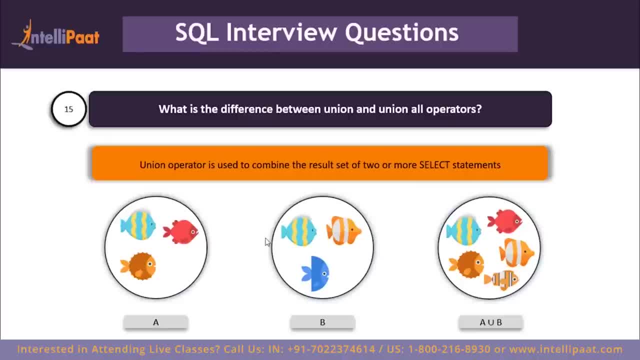 So here we see that this blue fish is present in both the tables A and B. Now when we apply the union operator on these two tables, the final result of A union B would have only one of these blue fish, And this is the syntax of the union operator. 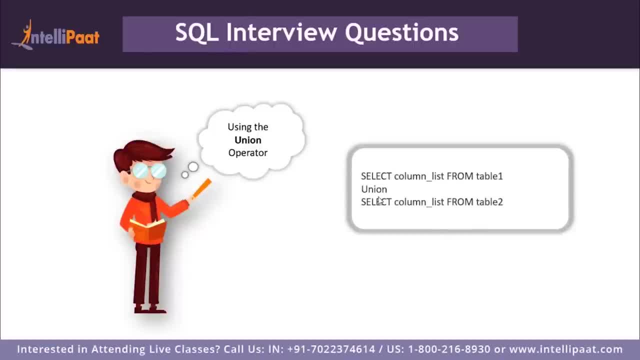 So we'll give the first select statement. After that we'll give in the union operator, following which we'll give the second select statement. Now you also need to keep in mind that the number and the order of columns must be same in both the select queries. 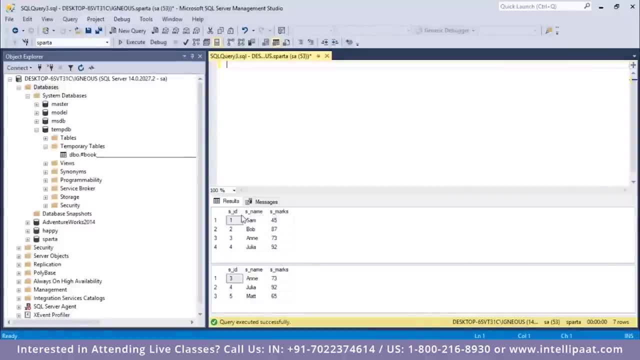 So let's work with this union operator now. So we have these two tables over here. So the name of this table is student details one and the name of this table is student details two. And if we have a glance at the columns, we see that both of the tables have three columns and the names of the columns are: 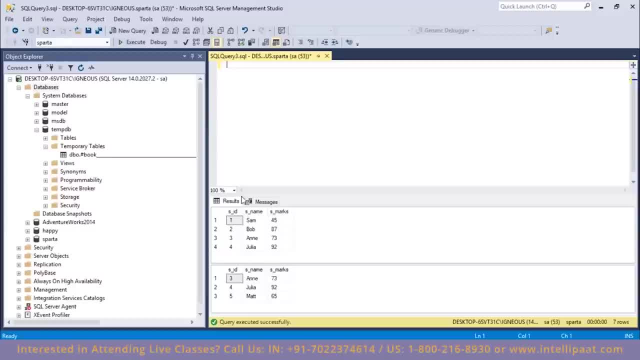 same and also the order of the columns are same. So here we have SID SNAME and DESMARKS. Similarly, over here we have SID SNAME and DESMARKS. Now let's go ahead and apply the union operator on this. So I'll type in the first select statement. 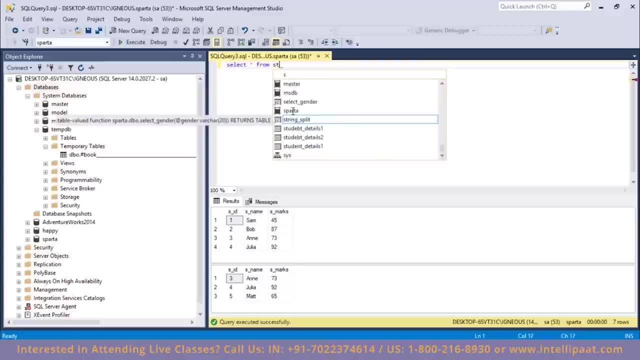 So it'll be SELECT star from student details one. So let me change the spelling to student details. After this I will apply the union operator and then give in the second select statement. So SELECT star from student details two. Now let me click on execute. 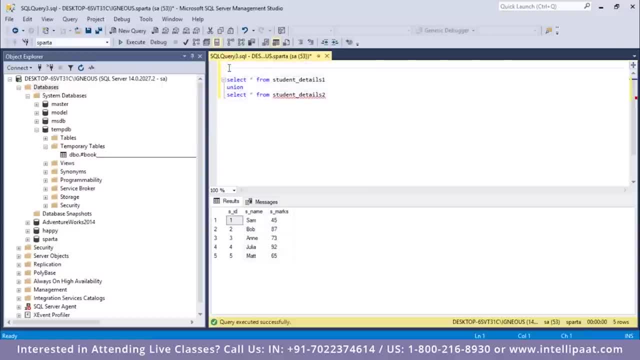 So this is the result over here. Now let me also print in the first two original tables. So SELECT star from student details one, And then I'll also put in SELECT star from student details two. So let me just change the spelling to student over here. 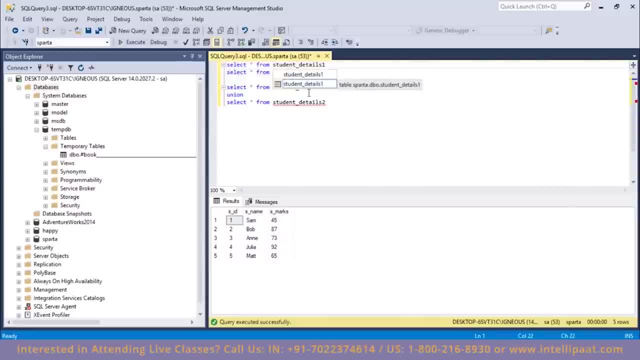 Let me also change this over here. So this will be student Right. So this is student details one. this is student details two, and this is the result of the union operator. Now, if you have a glance at these two tables, then you see that these two. 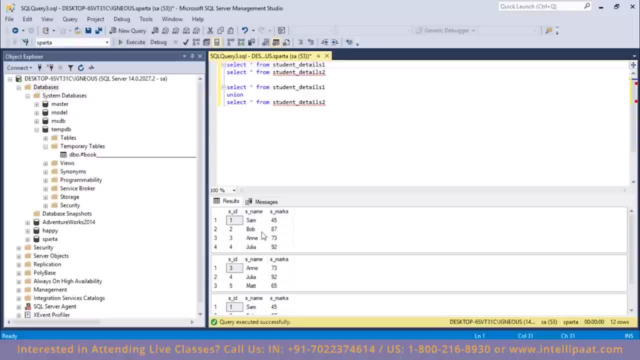 records are repeating over here, right? So there's Ann Julia over here in the first table And there's also Ann and Julia in the second table. Now, when we apply the union operator, then we just have one record coming from each of these tables. 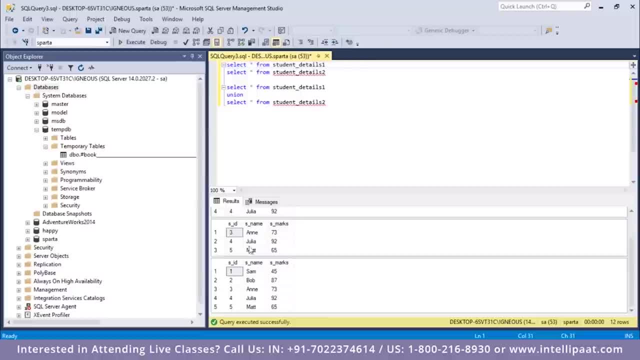 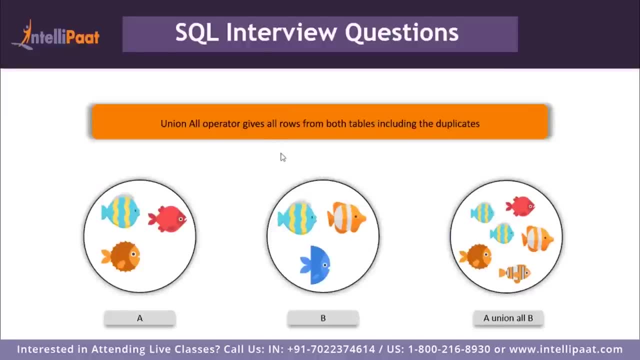 Right. So you've got Ann over here, We've got Julia over here And then we have finally have Matt, which comes from the second table. This is how the union operator works Right now. let's look at the union all operator. 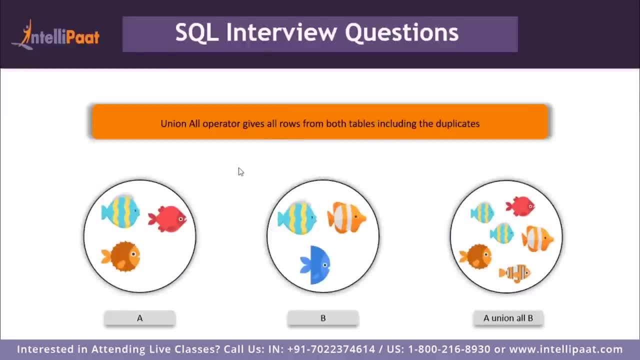 So the union, all operator, gives all the records from both the tables, including the duplicates as well. So here, since this blue fish is present in both the tables A and B, the final result of A union, all B would also have the duplicate value. 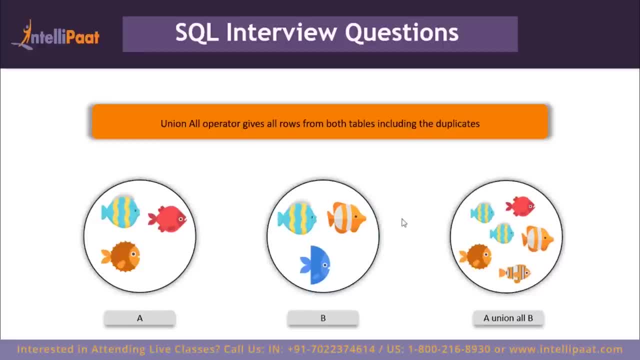 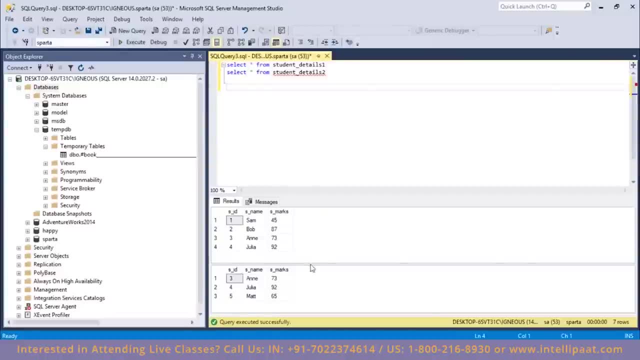 So here we see that we've got both of the blue fish from table A and table B. Now let's go ahead and implement this in SQL server as well. So here we have these two tables already ready, which are student details one and student details two. 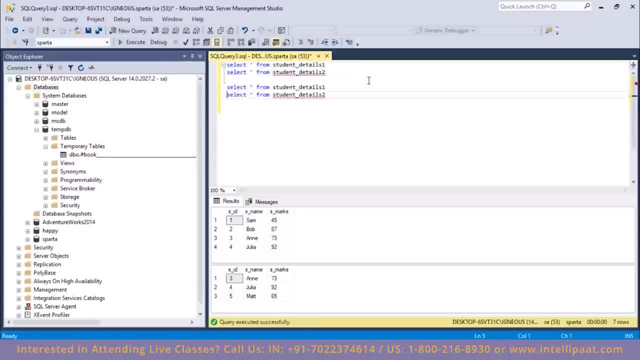 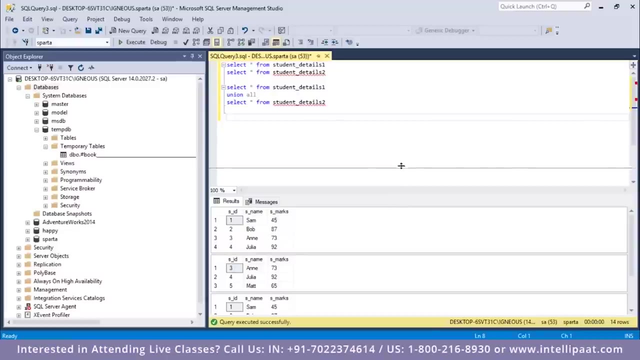 Now what I'll do is I will copy this, I'll paste this over here and just type in union all. So union all. I'll click on execute the student details one. student details two. Let me just expand this over here. Right, And this is the result of union all operator. 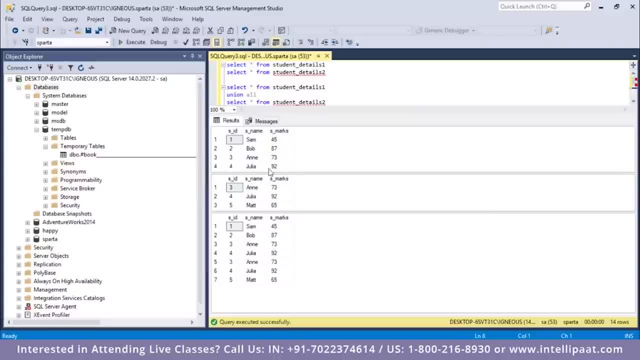 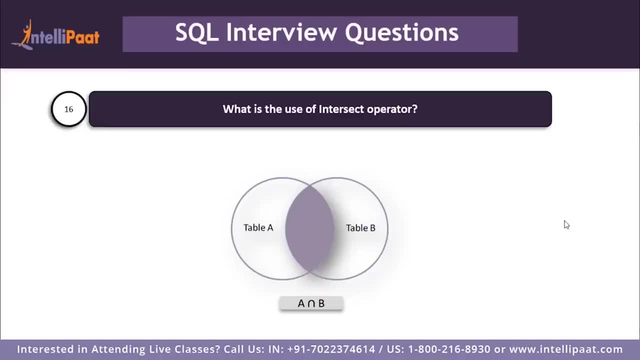 Right. If you have a glance at this, you'll see that these two are repeating, So we would have duplicate values. So we've got Anne twice over here and also Julia twice over here. So next question: well, what is the use of the intersect operator? 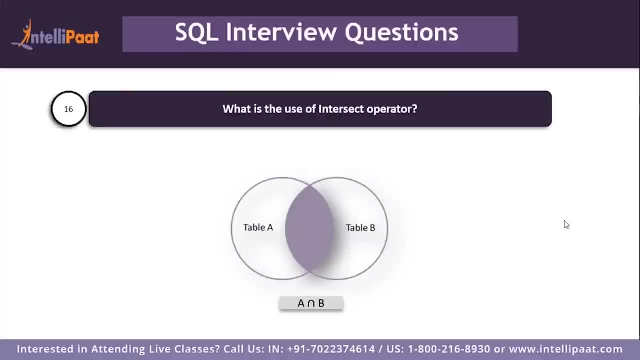 So the intersect operator helps to combine two select statements and returns only those records which are common to both the select statements. So if we've got table A and table B over here and if we apply the intersect operator on these two tables, then we'll get only those records which are common. 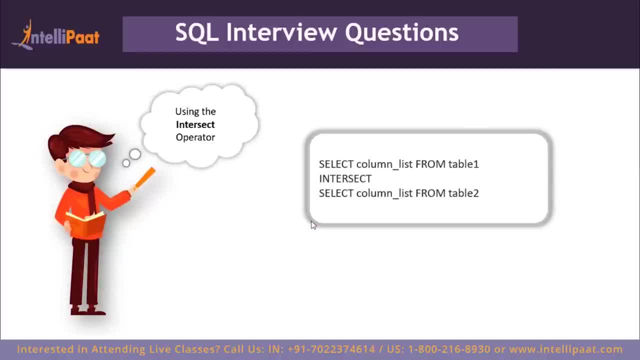 To the result of the select statements of these two. Now let's look at the syntax. So over here this is the syntax. So we'll start off by giving the four select statement and then we'll give the intersect operator, following which we'll give the second select statement. 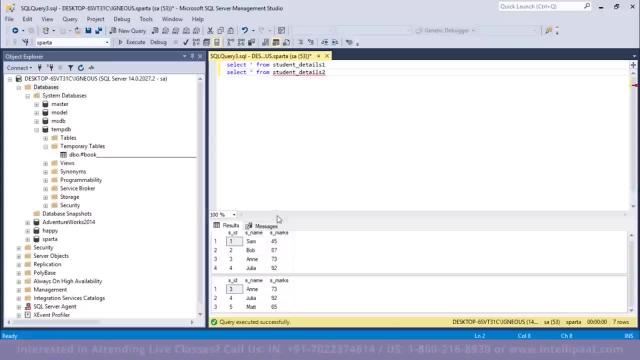 Now let's see an example on this. So again, we have these two tables over here: student details one and student details two. Now let me apply the intersect operator on these two. So let me just type in intersect over here and click on execute. 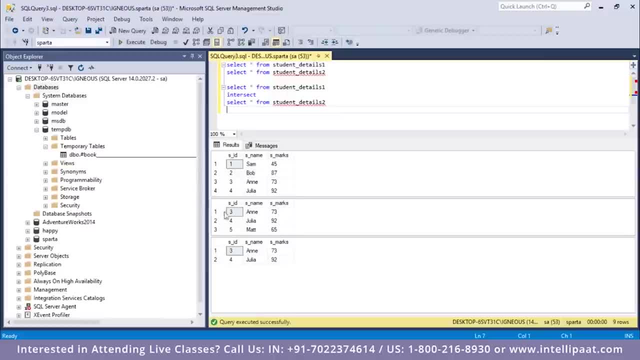 Now let me maximize this over here, Right. So student details one. student details two. And this is the result of the intersect operator. So we see that since Ann and Julia are common to both of these tables, this is the resultant of the select statement, right. 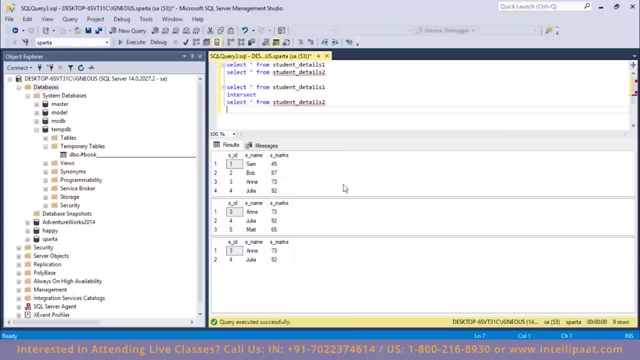 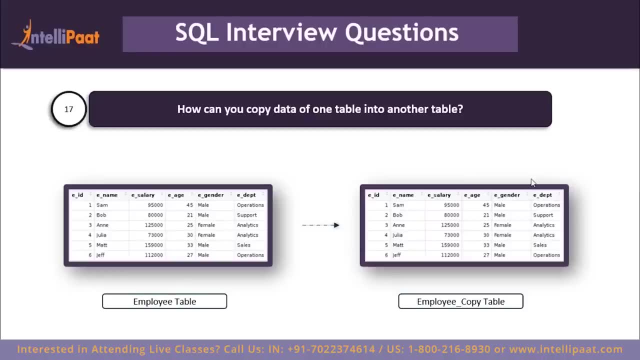 So the select statement on the first table gives out Ann and Julia, and the select statement from the second table also gives out Ann and Julia. So the intersection of these two would be this. So we have our final question Now. let's say you're given a table. 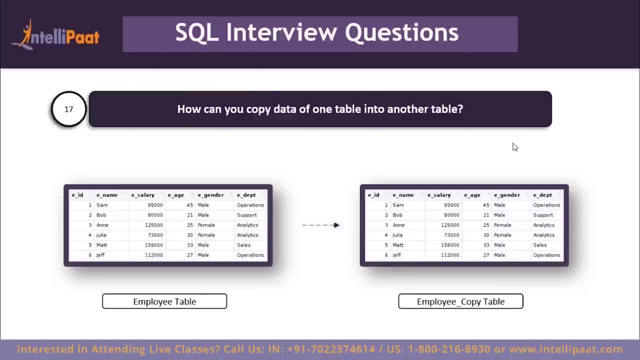 Now you'd have to copy the data of this table into another table. So you have this employee table. Now you'd have to go ahead and copy the data which is present in all of this table into another table. So let's see how can we do this. 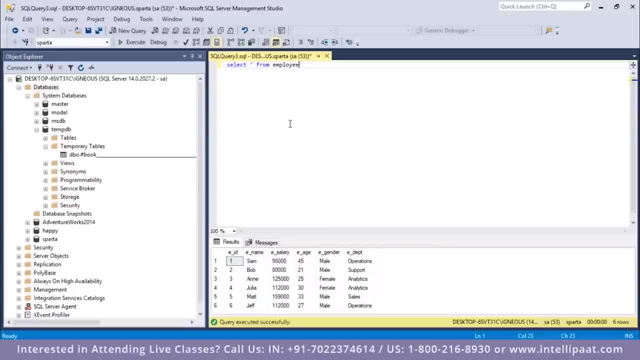 So this is our employee table over here. Now we'd have to copy all of this into another table. So for this purpose, we can use the insert into select operator. Now, before we go ahead and do that, we would also have to create another table which would have the same structure. 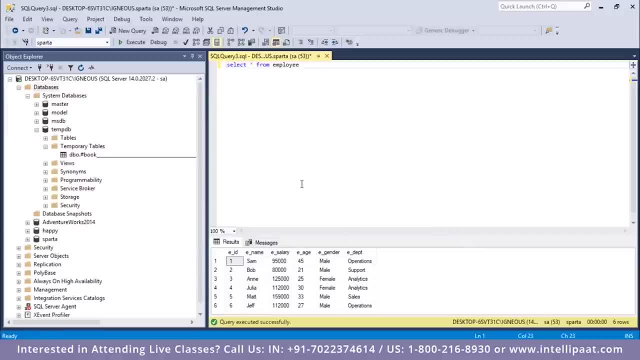 as this table. So the table doesn't have the same structure. Then you wouldn't be able to copy the data. So let me go ahead and create the table first. So I'll type in create table and I'll name this as employee duplicate. 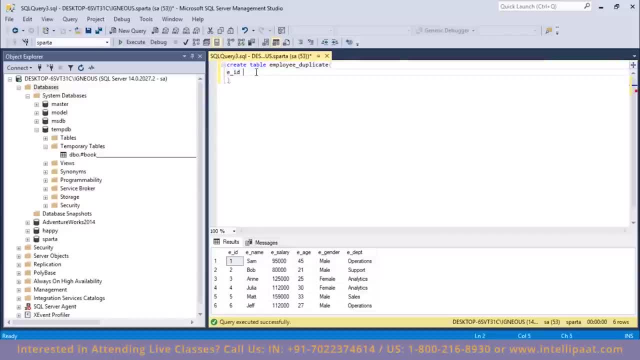 And then I'll give in all of the values over here. So my first column would be EID, and this would be of integer type. Second column would be E name, and this would be of varchar type And the length of the string would be 20.. 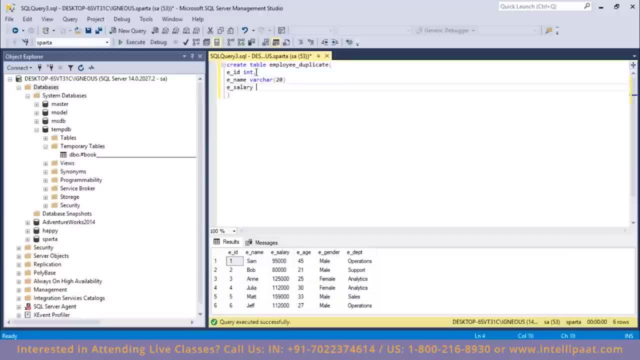 And then I would have the E salary over here. This would be of integer again. After this I would have the E age, which is of integer. Then I would have the gender of the employee. So the gender of the employee would again be of character type. 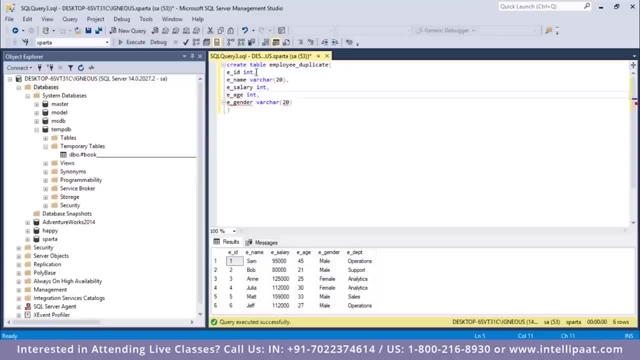 Now I'd have to make sure that I give in commas after all of these, So let me just put in a comma after this as well, And then the final column would be E, D, E, P, D, And this again would be of variable character, of length 20..